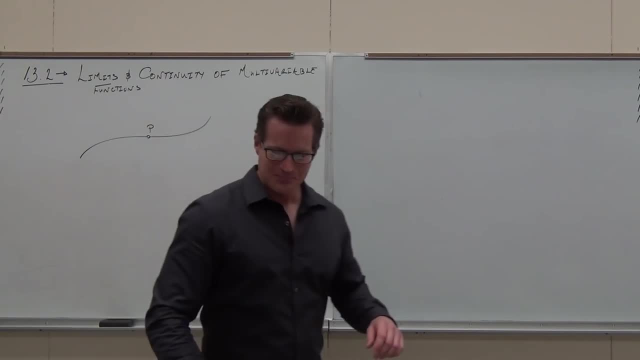 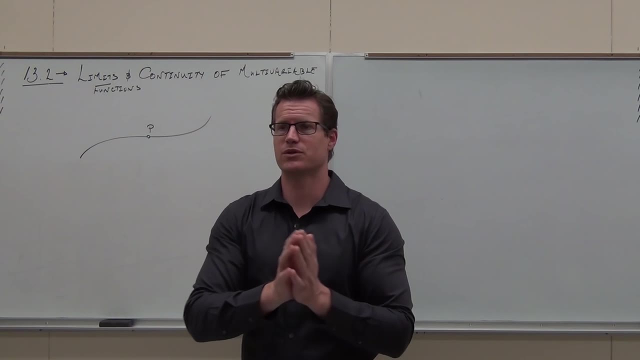 Well, good afternoon again. We're going to talk about section 13.2 right now. You see, we have this concept. It's how you start Calc 1.. It was called limits, and you learn to loathe them- Loathe is the right word. Until you really learn them, You go okay, this isn't so bad. So here's what we're going to do. We're going to talk about limits and continuity of multivariable functions. We'll see how this works. What I really want to focus on for about the first 20 minutes is what it means. 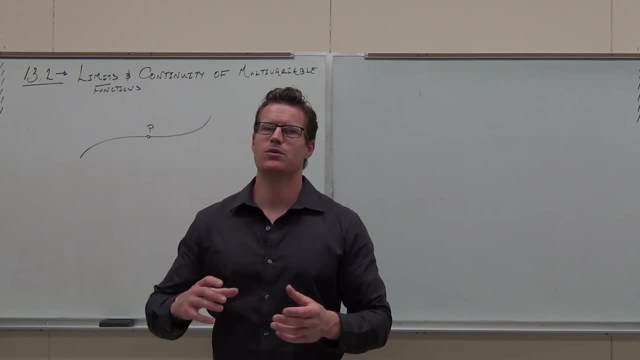 What are you doing when you're finding a limit? Because if you understand the concept, how we're going to do the rest of it makes a lot more sense. If you don't really get what we're doing- like why are we doing this? then they're not going to make sense at all. You're just going to have a set of rules that you're going to go through, probably never really get it and then eventually make a whole lot of mistakes on it Make sense. So I want to focus on what a limit means when we're talking about multivariable functions. 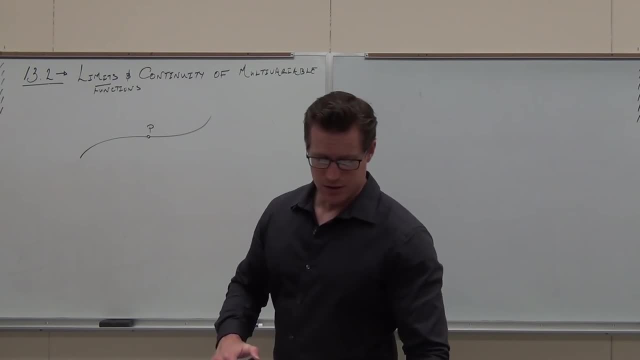 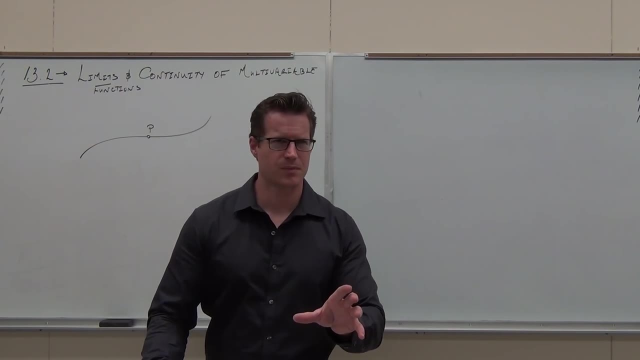 Let's start with something. Let's start with something about limits with functions in one variable And what we mean. of course, when I talk about variables, I mean independent variables. So when we have a function of one independent variable, what we get is we get this curve. 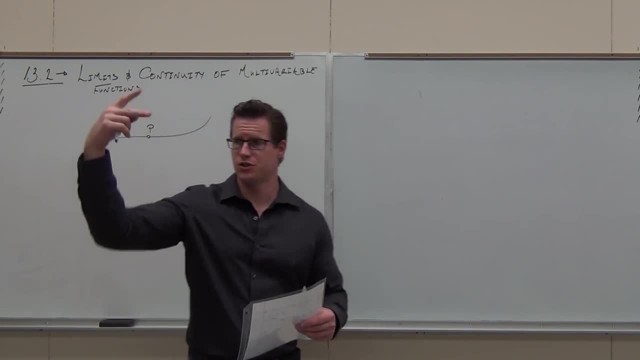 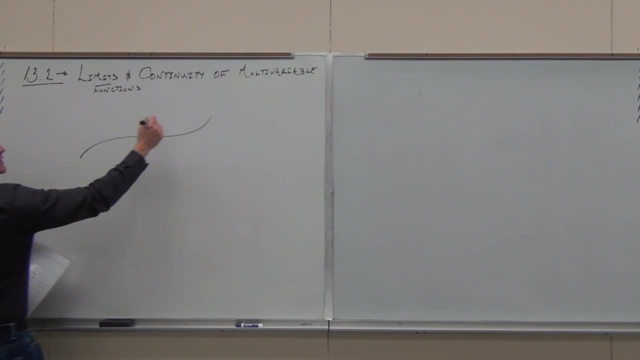 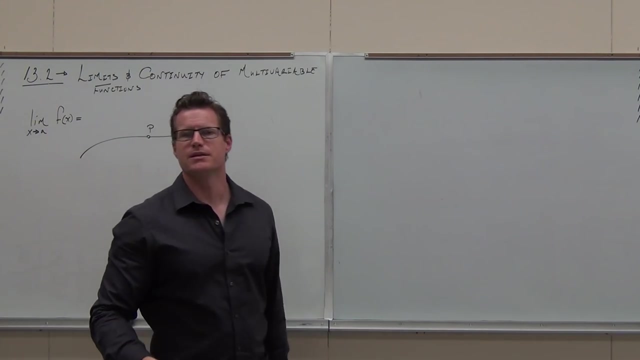 on a plane. that's entirely what we have: One variable, two dimensions. Remember talking about that a couple times ago or last time: One variable, two dimensions. So if this is my function, I say: well, how does a limit exist if we have a function in one independent variable? 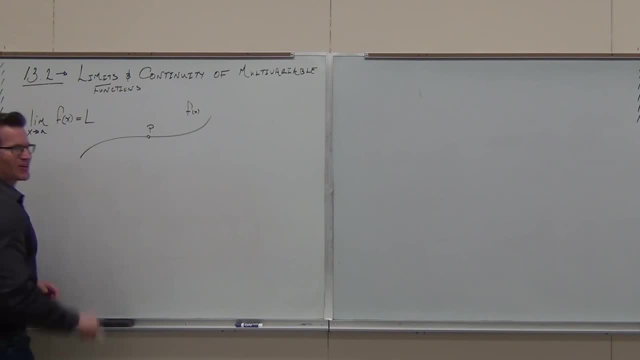 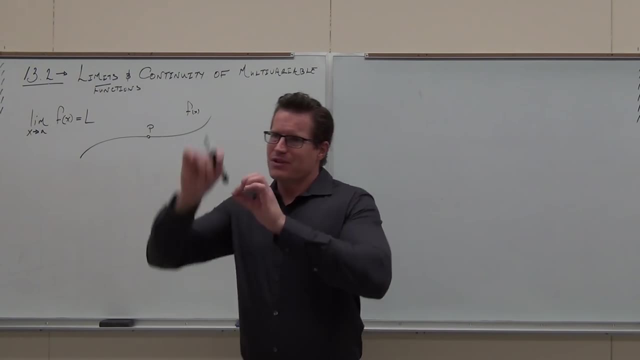 We go: well, it exists. if this limit equals a number, Yay, And it doesn't exist if that equals like an asymptote, and they're going opposite ways, or if we have different values. but more specifically, we say: here's what has to happen. 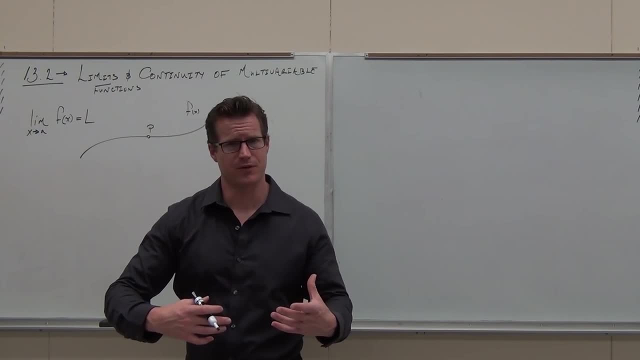 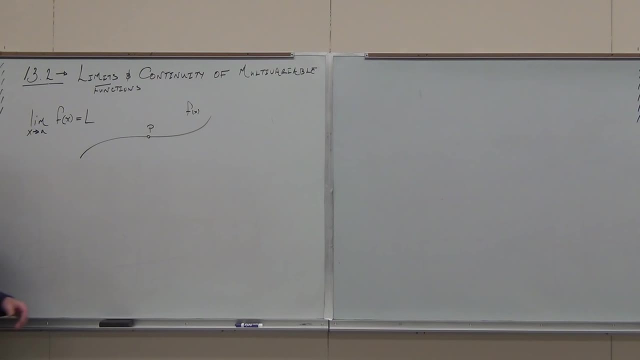 and this is the big part. okay, because this is going to change when we get to multivariable functions. Here's how we recognize that limits exist for functions in one variable. We go well. well, you know what. you know it. 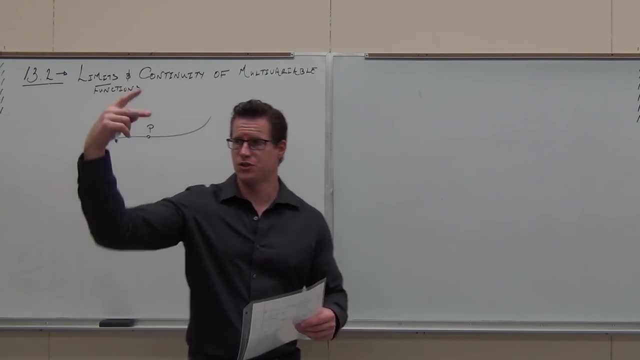 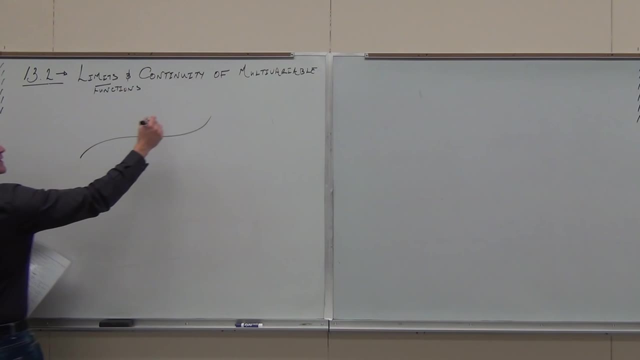 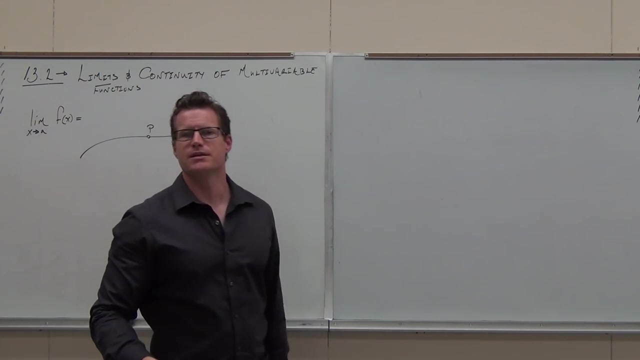 on a plane. that's entirely what we have: One variable, two dimensions. Remember talking about that a couple times ago or last time: One variable, two dimensions. So if this is my function, I say: well, how does a limit exist if we have a function in one independent variable? 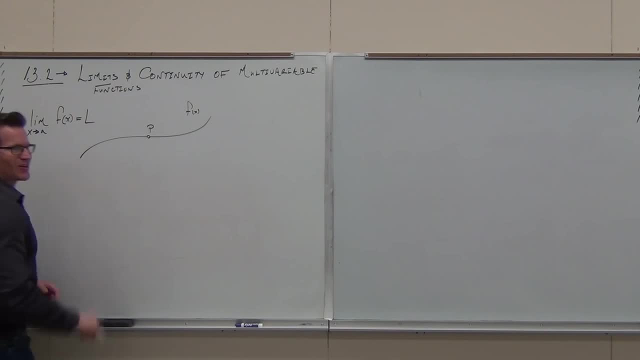 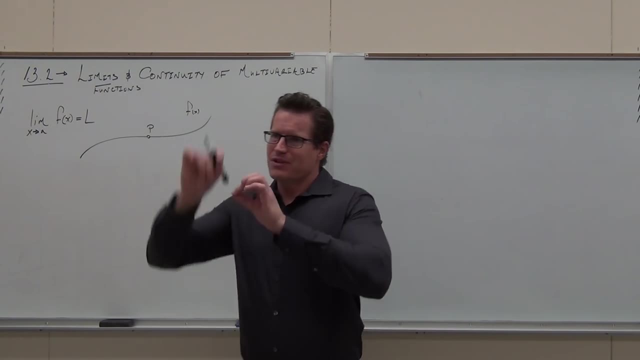 We go: well, it exists. if this limit equals a number, Yay, And it doesn't exist if that equals like an asymptote, and they're going opposite ways, or if we have different values. but more specifically, we say: here's what has to happen. 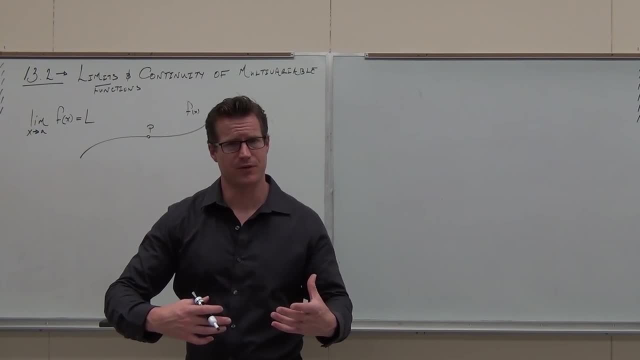 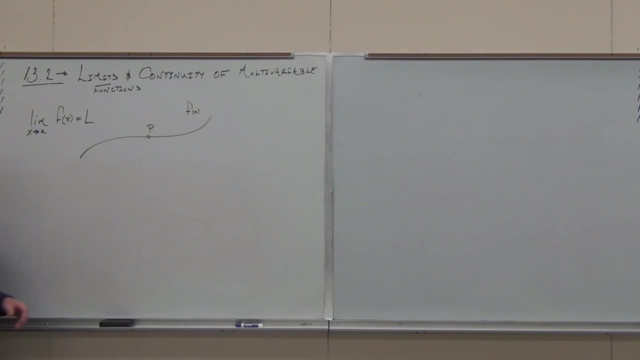 and this is the big part. okay, because this is going to change when we get to multivariable functions. Here's how we recognize that limits exist for functions in one variable. We go, well, you know it, How do we tell that limits exist for functions of one variable? 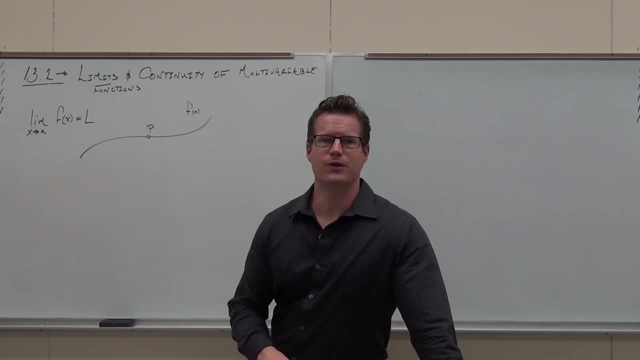 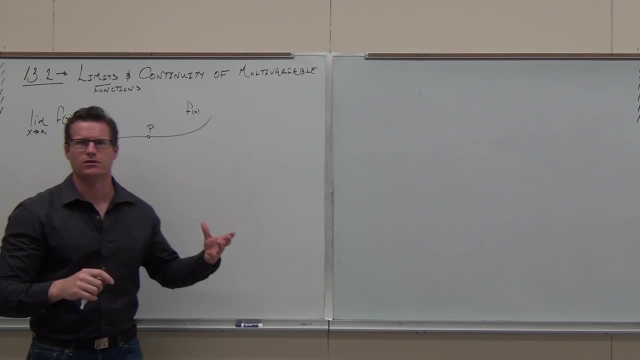 What do we do? Evaluate? How do you evaluate them? What do you If I say: does the limit exist here? Does it exist at the point P, yes or no, Why? Why does it exist? Does it exist? Does it exist at the value P here? 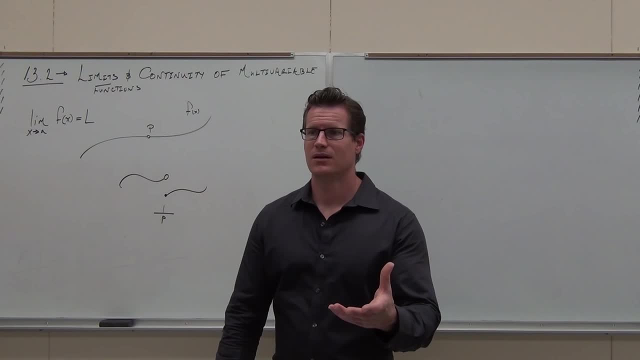 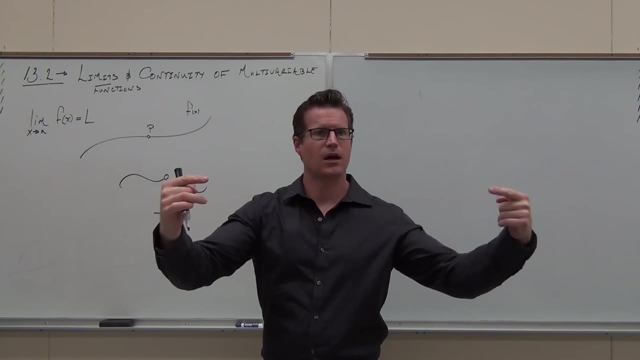 No, Okay, Why? Because not Both sides, From Both sides. So we have this idea of limits, of a left side and a right side. You guys remember that? It's a long time ago, I know. And that's how we determine that limits actually exist. 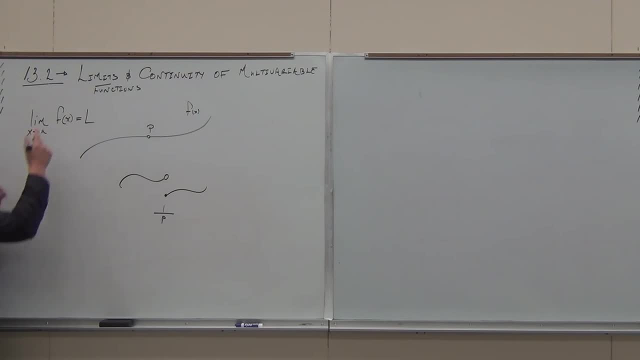 We say, okay, well, if this limit exists, what that implies, or how we got that, was that the limit as we approached along the axis of the independent variable, from the left to a certain value and from the right to a certain value were the same. 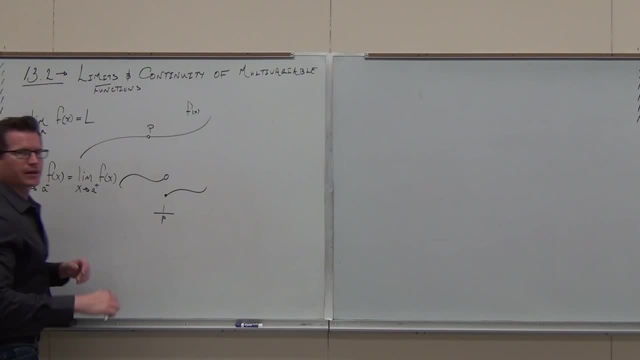 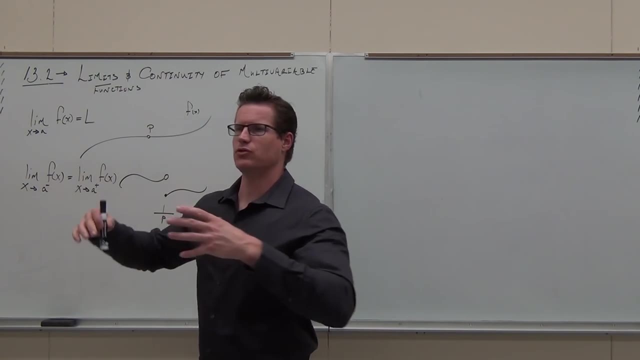 So we do this. Hey, let's come now. here's the big thing. Here's the big thing. This is what matters. This is what matters. This is what matters. How do where do we travel? What do we travel along when we're checking the limit of a function of one variable? 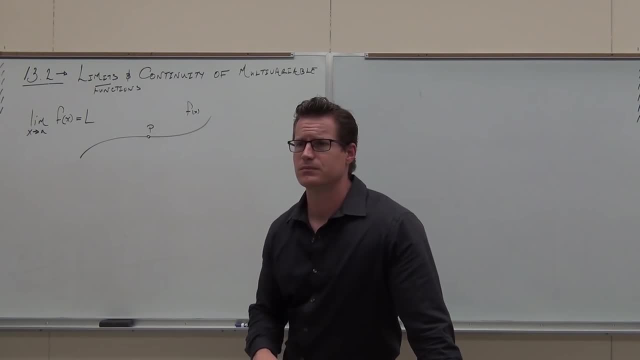 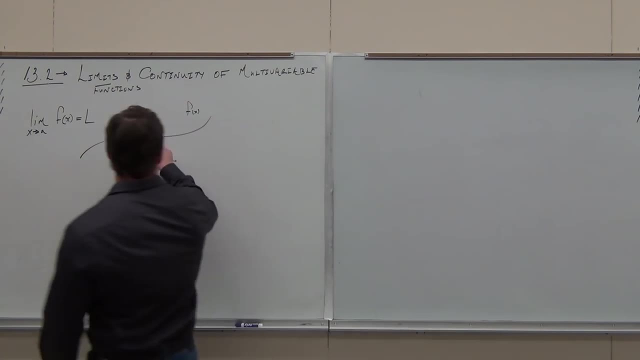 How do we tell that limits exist for functions of one variable? What do we do? Evaluate? How do you evaluate them? What do you if I say, does the limit exist here? Does it exist at the point P, yes or no? 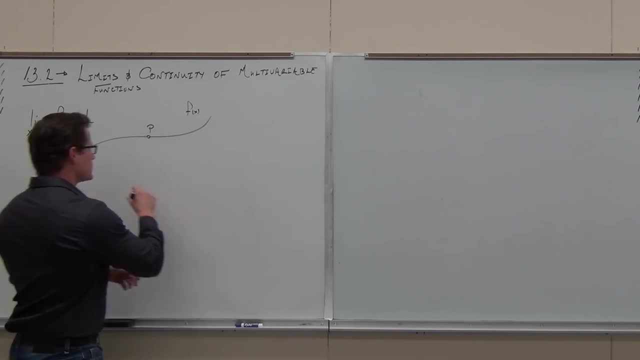 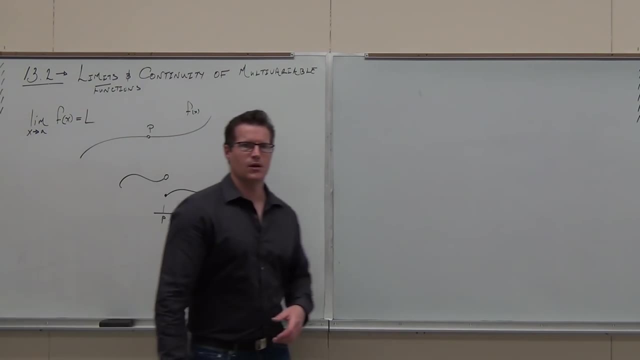 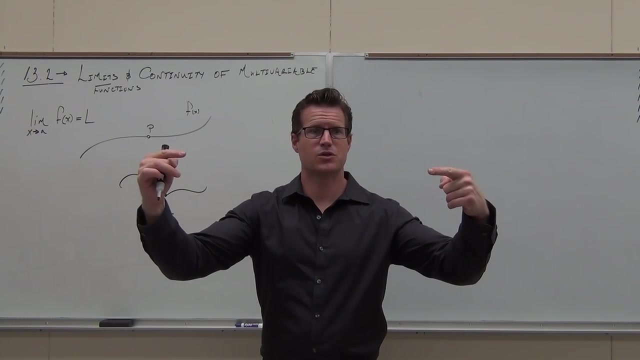 Y, Y. does it exist? Does it exist, Does it exist at the value P here? No, Okay, why? Because not Both sides, From Both sides, Both sides. So we have this idea of limits, of a left side and a right side. 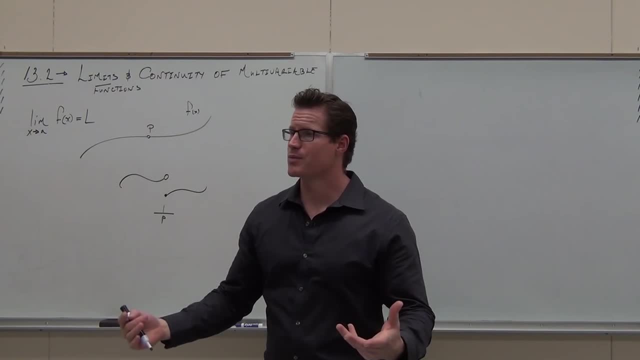 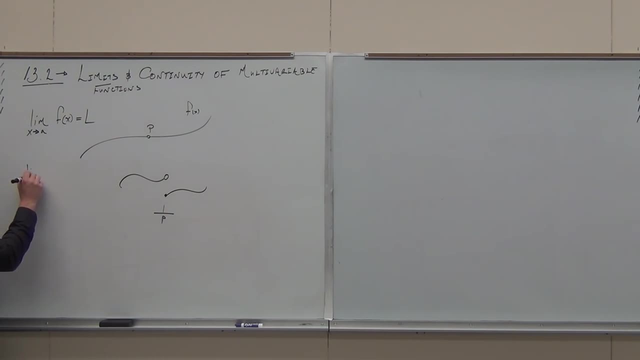 You guys remember that- It's a long time ago, I know. And that's how we determine that limits actually exist. We say, okay, well, if this limit exists, what that implies or how we got that, was that the limit as we approached along the axis of the independent variable from the left to a certain value. 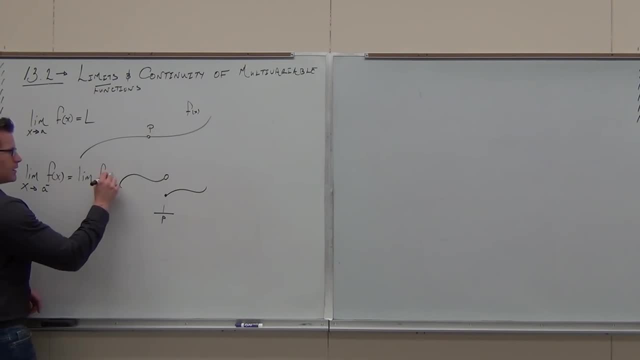 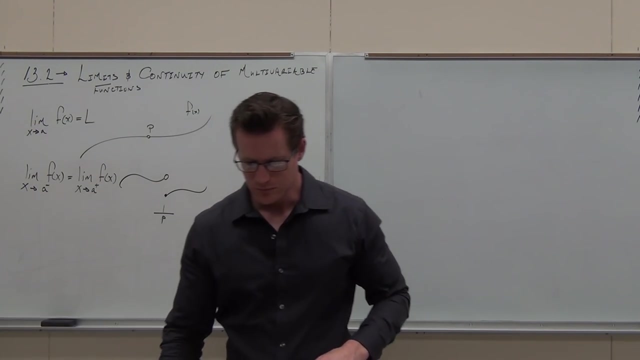 and from the right to a certain value were the same. So we do this. Hey, let's come Now. here's the big thing. Here's the big thing. This is what with what matters. where do we travel? what do we travel along? 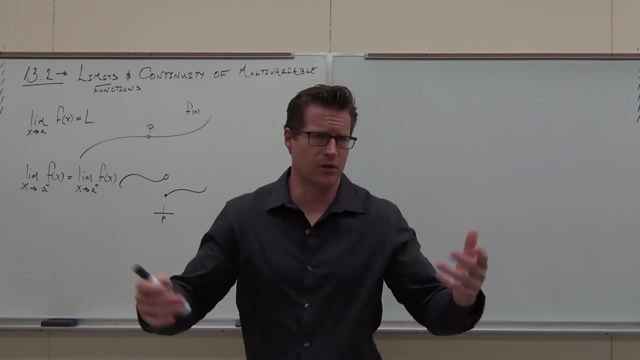 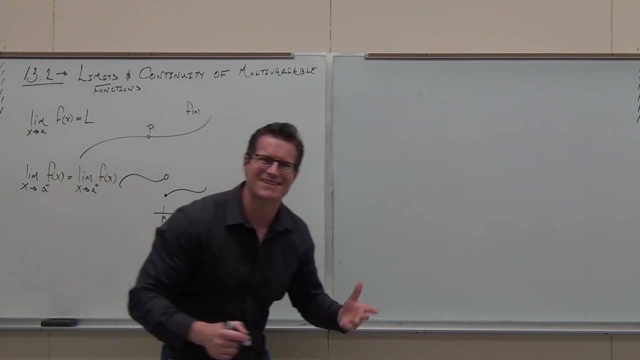 when we're checking the limit of a function of one variable. What do we travel along? Well, okay, so we're moving this way, but we travel along the actual curve. We don't travel along the x-axis, because in both these situations, 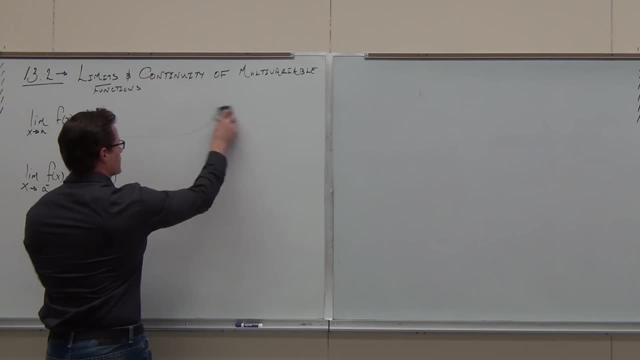 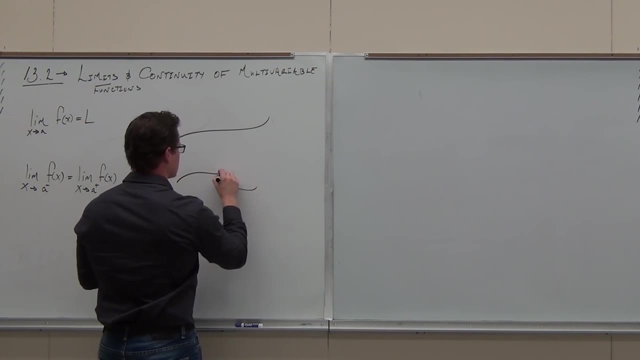 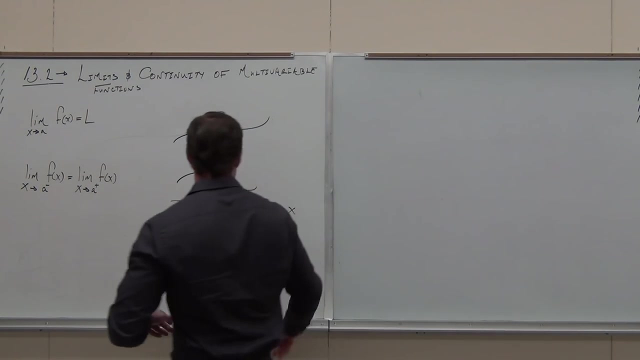 let me make them a little bit more on top of each other, okay. So let's see, Here's the x-axis, here's A. There's two different functions here, There's top function and bottom function. Say, hey, what's the limit as we approach A. 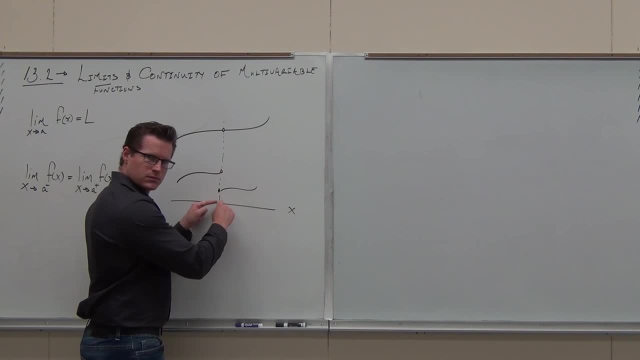 You don't go like this. You don't go um A Done, D for done, D for done. That's what you mean: D for done. We don't go this way. That's not what we do to check limits. 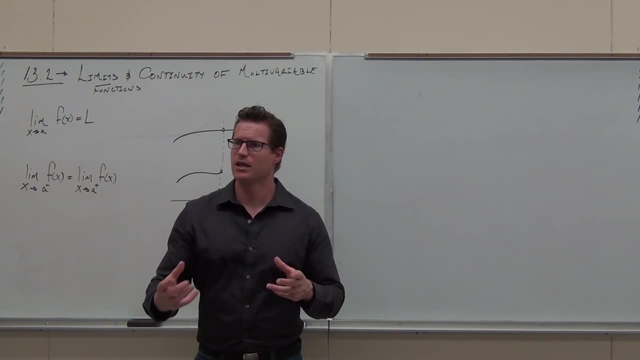 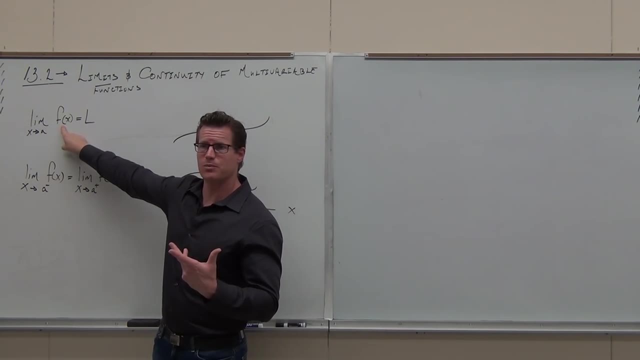 What do we travel along when we are evaluating our limits? Think back to what a limit means. A limit means: what's the height of your function, What's the function value as we're approaching that number on that axis? That's what it means. 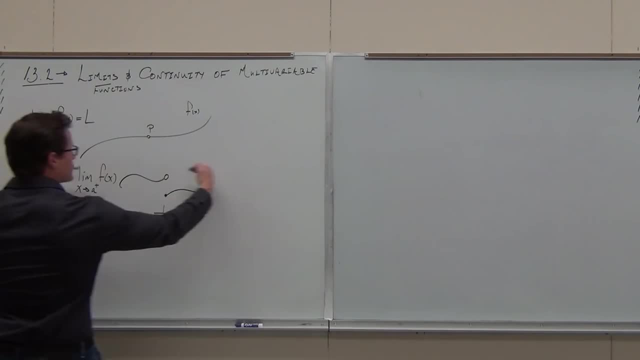 What do we travel along? Well, okay, so we're moving this way, but we travel along the actual curve, We don't travel along the x-axis, because if in both these situations, let me make them a little bit more on top of each other, okay. 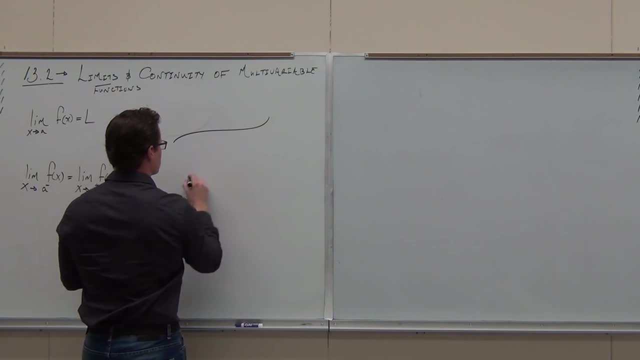 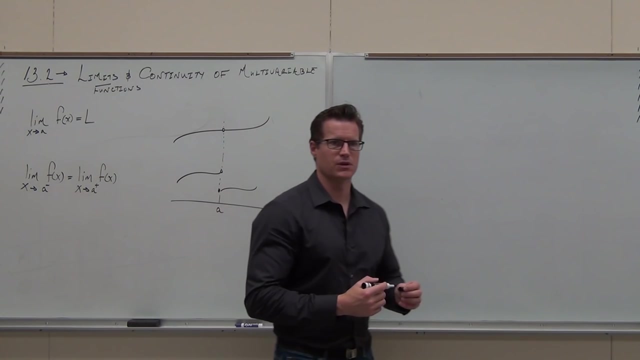 So let's see: Here's the x-axis, here's a. There's two different functions here. There's top function and bottom function. Say, hey, what's the limit as we approach a? You don't go like this. 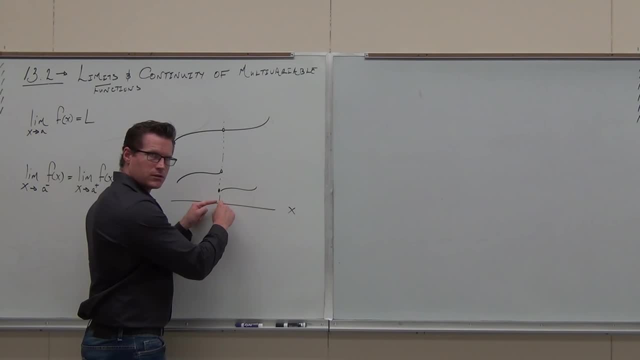 You don't go um a Done D for done, D for done, That's it, D for done. We don't go this way. That's not what we do to check limits. What do we travel along when we are evaluating our limits? 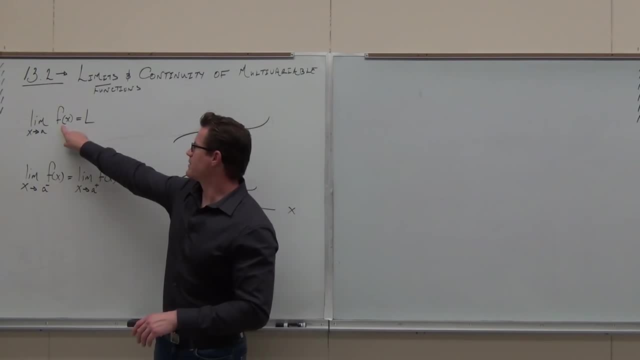 Think back to what a limit means. A limit means what's the height of your function, What's the function value, As we're approaching that number on that axis. that's what it means. What it implies is that we're approaching that number on that axis from both the left and the right. 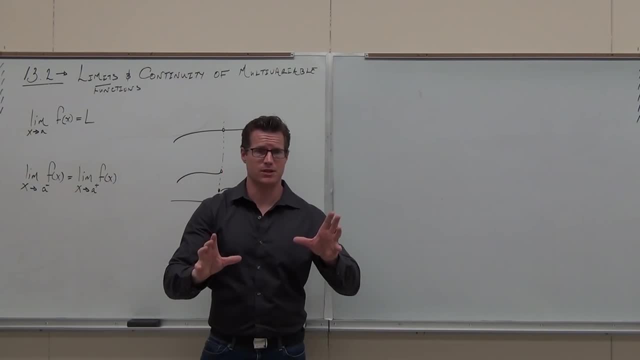 And the height of our function has to be equal for that limit to exist. You guys understand that concept. I don't want to have to go back and re-teach Calc 1, but I will Pause right now and watch the videos. 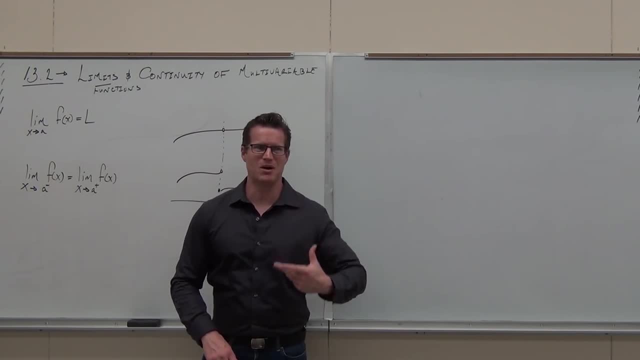 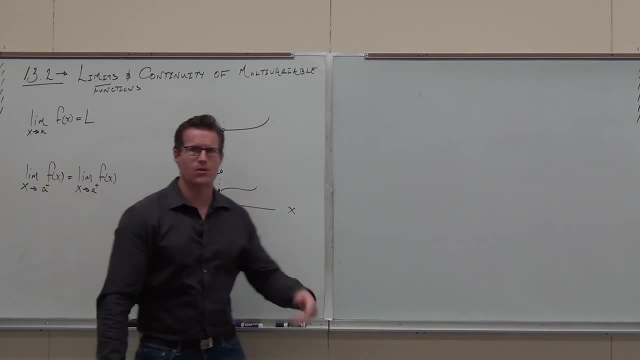 It's all of us together. Awesome, I'll get to soothe my voice. It hurts, man. It's hard work. That's what it means. So do we actually travel along the x-axis? No, No, We travel along the curve. 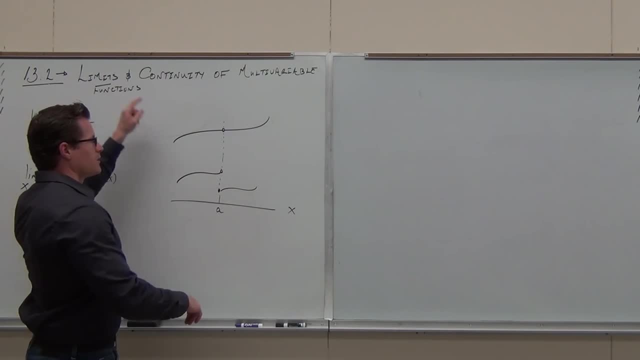 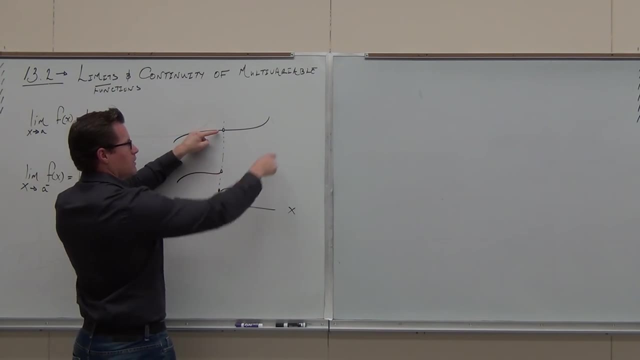 That's what we travel along, So we go okay here. Here's how we do it From the left. what's the height of my finger as we get close to our vertical dotted line, which is that a? Okay, it's right here. 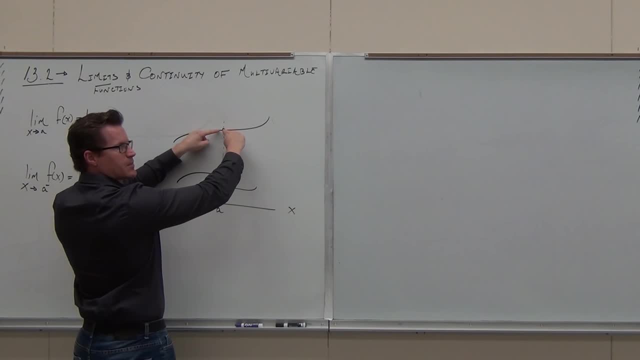 What's the height of my finger as we get close to that vertical dotted line? Oh, it's at the same height. That's how we know our limit exists. What's the height of my finger? Oh, it's over here As I'm traveling along the curve approaching this x-value dotted line. it's right here. 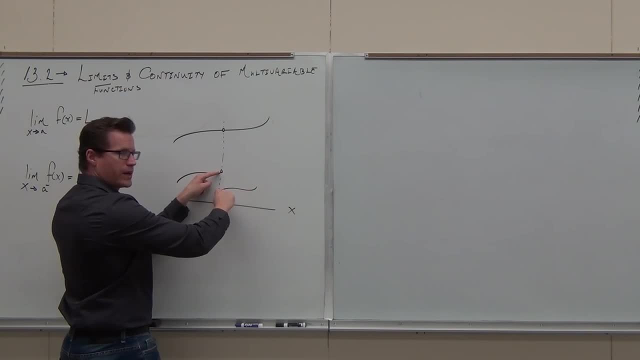 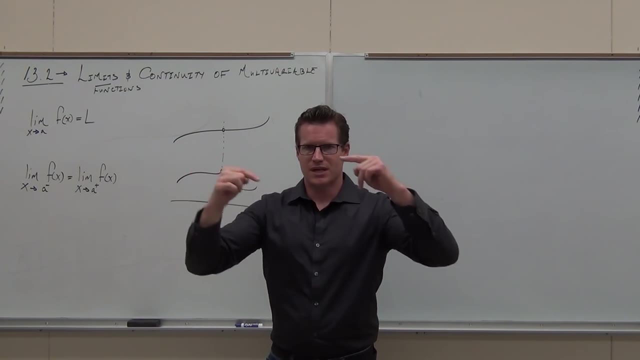 From the right-hand side, traveling along the curve. it's right here. Wait a minute, Those things are different. The height of my function, the height of the curve is different, as I'm approaching the same x-value, x-axis from left and right. 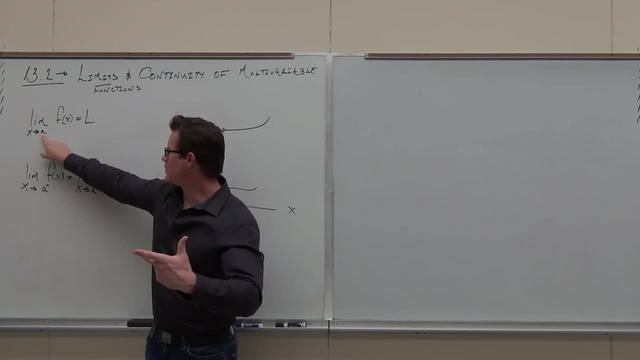 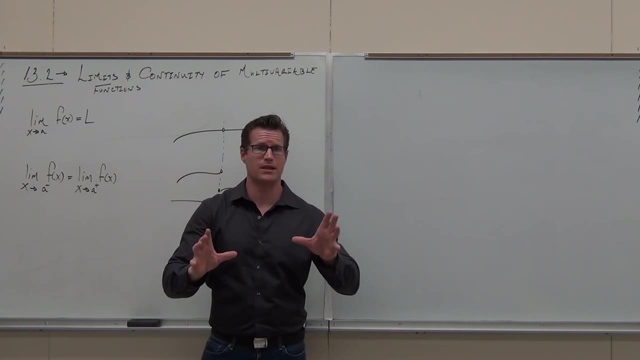 What it implies is that we're approaching that number on that axis from both the left and the right, and the height of our function has to be equal for that limit to exist. You guys understand that concept. I don't want to have to go back and reteach Calc 1, but I will. 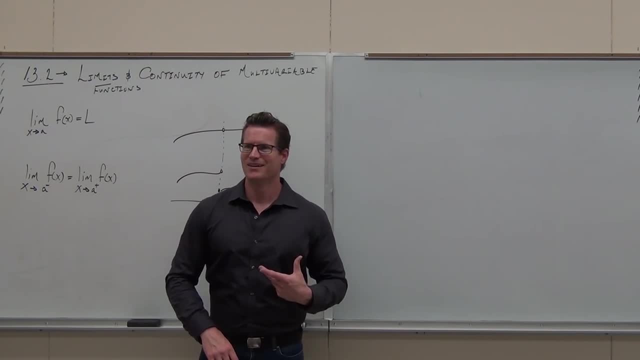 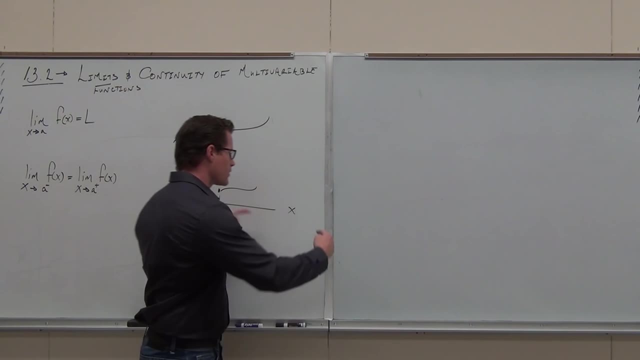 Pause right now and watch the videos. All of them together: Awesome. I'll get to soothe my voice. It hurts, man. It's hard work. That's what it means. So do we actually travel along the x-axis? 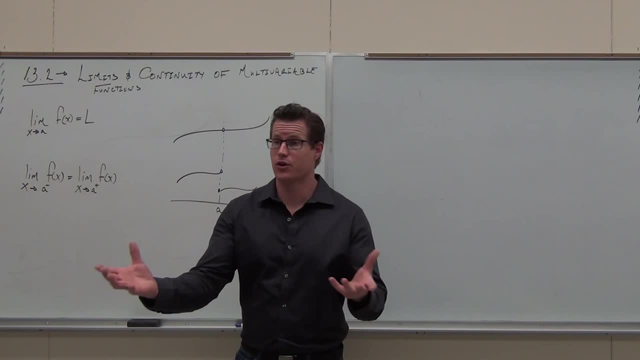 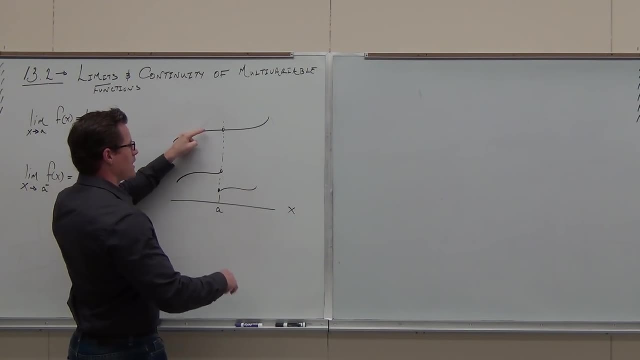 No, No, We travel along the curve. That's what we travel along, So we go okay here. Here's how we do it. From the left, what's the height of my finger as we get close to our vertical dotted line, which is that A? 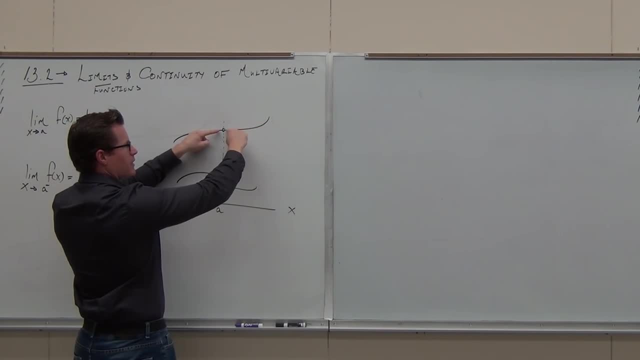 Okay, it's right here. What's the height of my finger as I get close to that vertical dotted line? Oh, it's at the same height. That's how we know our limit exists. What's the height of my finger? Oh, it's over here. 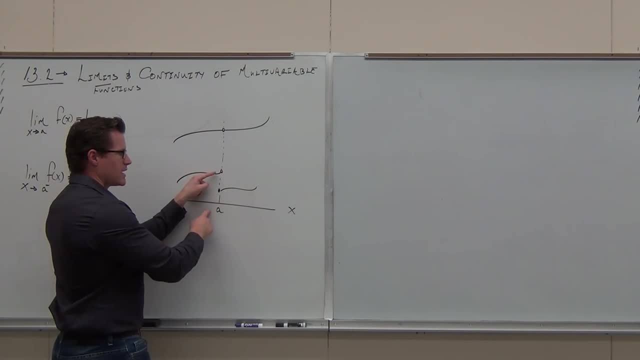 As I'm traveling along the curve, approaching this x-value dotted line. It's right here, From the right-hand side, traveling along the curve. it's right here. Wait a minute, Those things are different: The height of my function, the height of the curve. 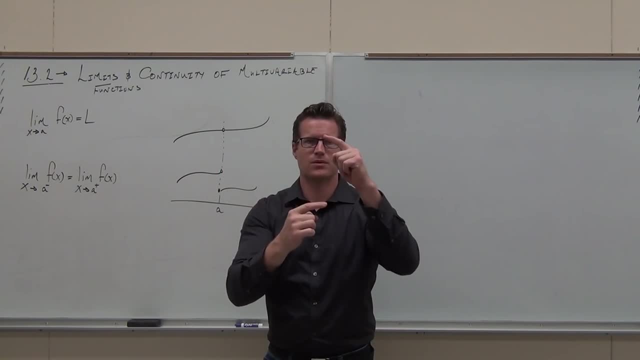 is different, as I'm approaching the same x-value, x-axis from left and right. Limit doesn't exist. Limit does exist, so it makes me okay with that one. Okay, Now we extend the concept. Okay, Let's consider something else now. 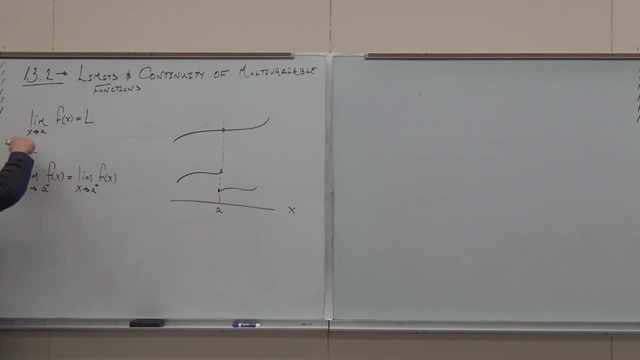 This happens. if this happens, The limit exists if, from the left and from the right, we approach the same value on our function. Now, what about this? What has to happen for a limit to exist if we have more than one x-axis? 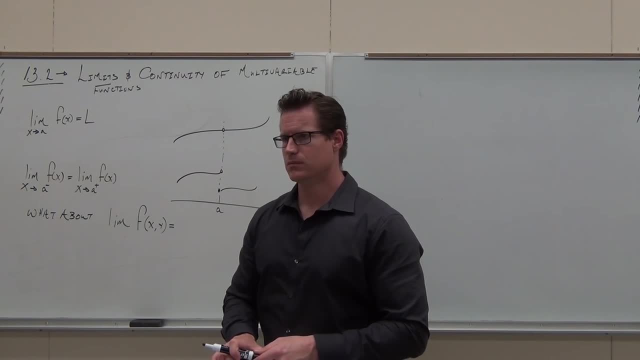 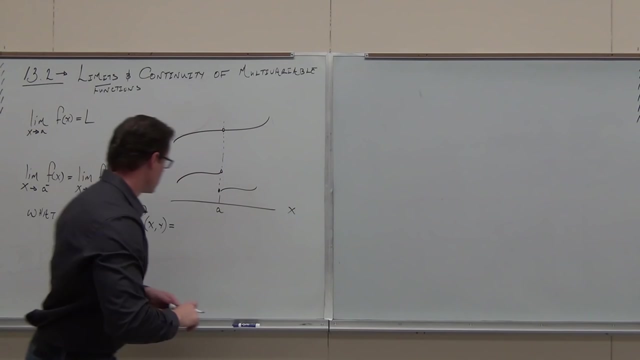 More than one independent variable. Well, there's an issue, right. The issue is a very huge ambiguity right now. Are we traveling along one axis of one independent variable? The answer is no. What we need to happen is that that order. 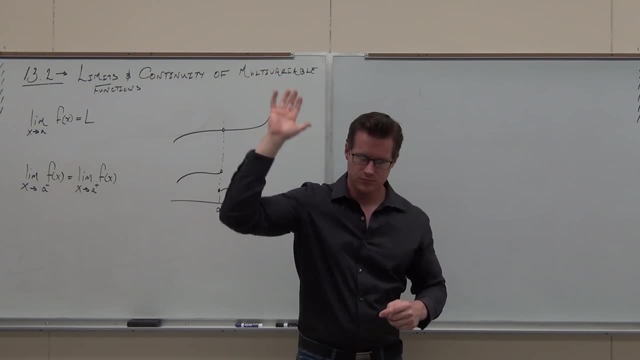 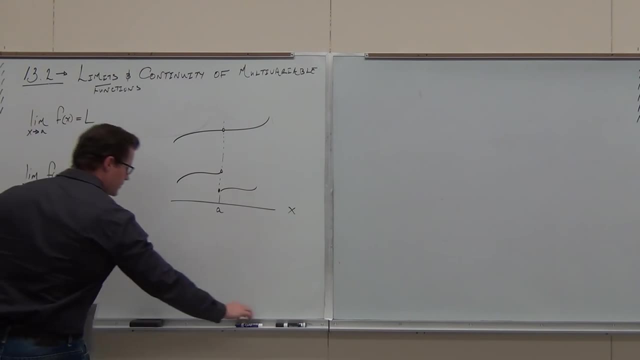 Limit doesn't exist. Limit does exist, so it makes me okay with that one. Okay, Now we extend the concept. Okay, Let's consider something else. now This happens. if this happens, the limit exists. if, from the left and from the right, we approach. 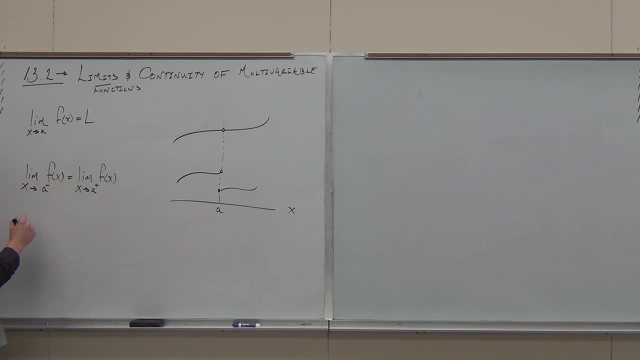 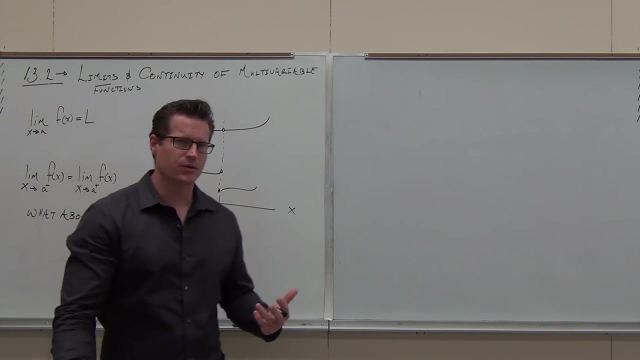 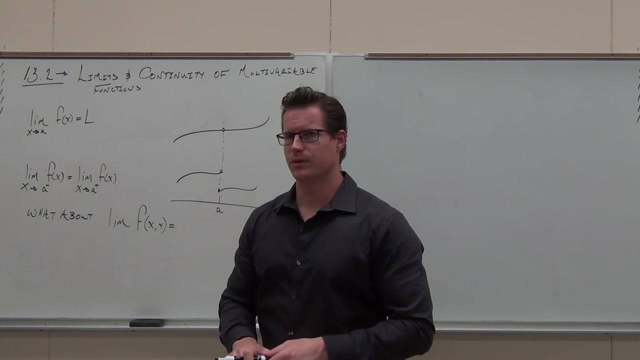 the same value on our function. Now, what about this? Okay, What has to happen for a limit to exist if we have more than one independent variable? Well, there's an issue, right? The issue is a very huge ambiguity right now. 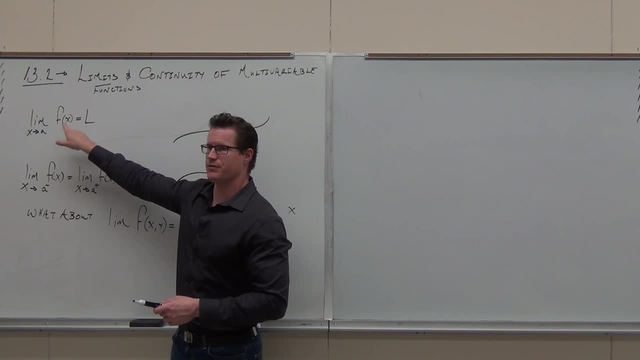 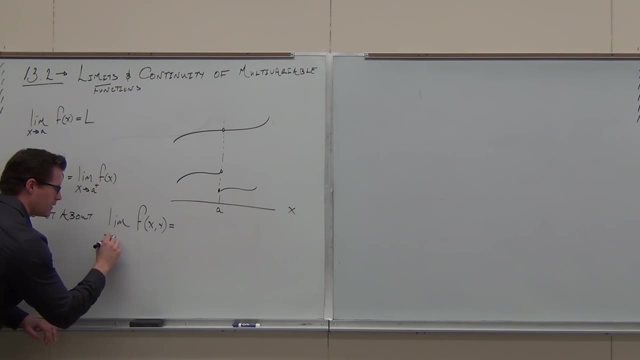 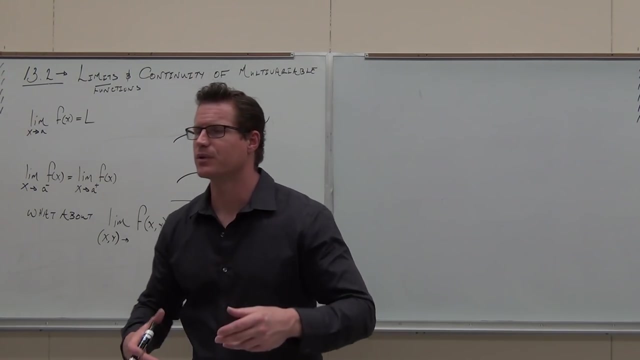 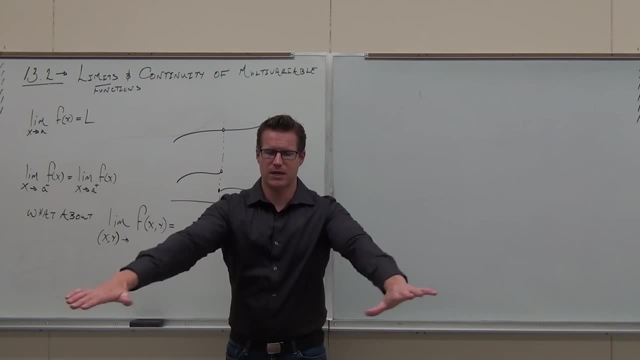 You know you've got to go back and kind of remember this. but what we're doing here is we're plugging in ordered pair. That ordered pair is along the xy plane. We're plugging in the pair. The ordered pair is giving us the height above the point on the xy plane. 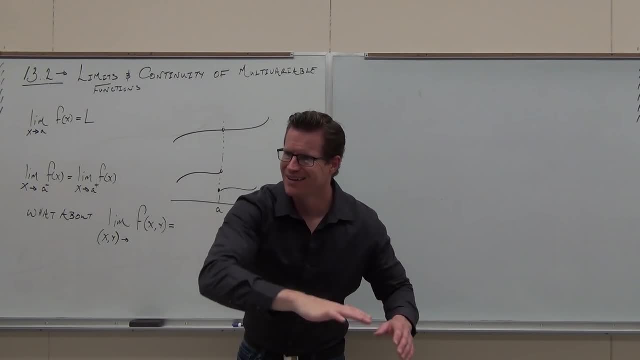 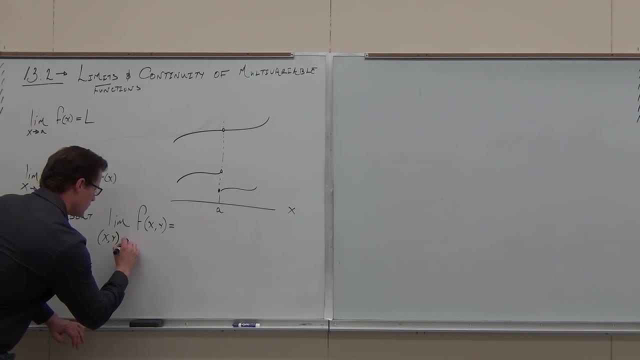 Does that make sense? So we have to traverse this plane. We have to traverse the plane now and see what's the height doing as we're traversing this plane. Well, How exactly is that? Yeah, ив, We did. That means, instead of approaching one number. 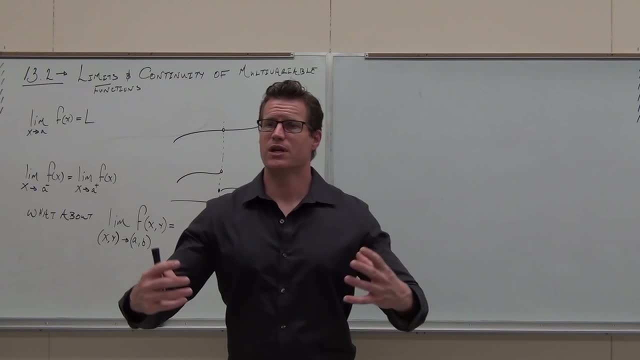 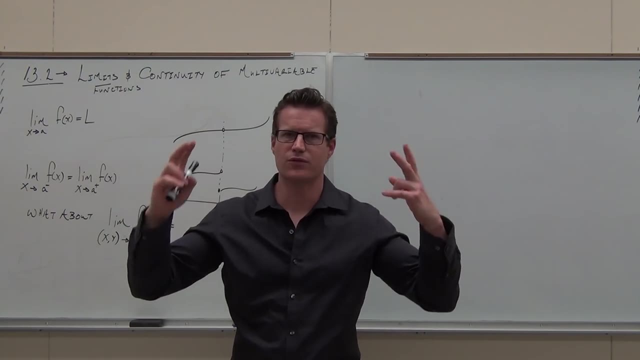 on one axis, we're approaching one point, but we're doing it from what? what? from what? from what direction? How are we doing this? What is the curve in this case? And this is the whole situation. How do we know this limit exists? 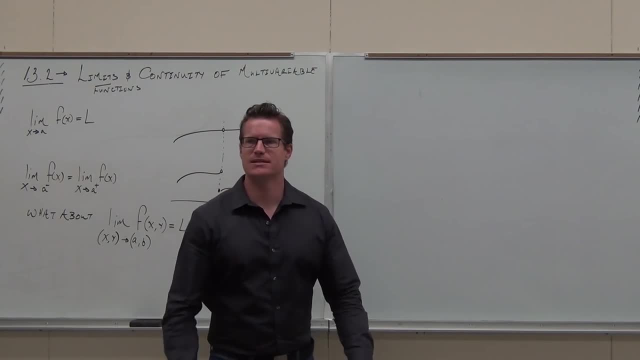 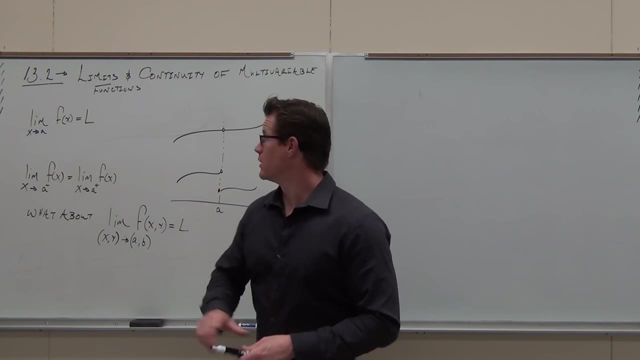 Well, if it equals L, done yay. that tells you nothing. It tells you nothing. Here's the issue, And we- we just covered part of it. What's that give you? What's a function in one variable? What's it give you? 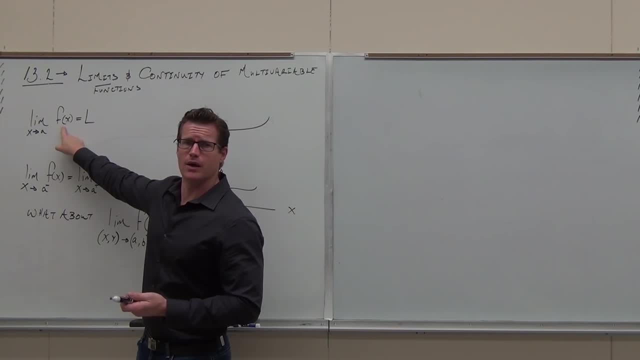 Come on, It gives you a curve, as you, as you said, on a on a plane. This is just a curve on a plane, That's all it is What does, and this is the whole reason why I had the last section. 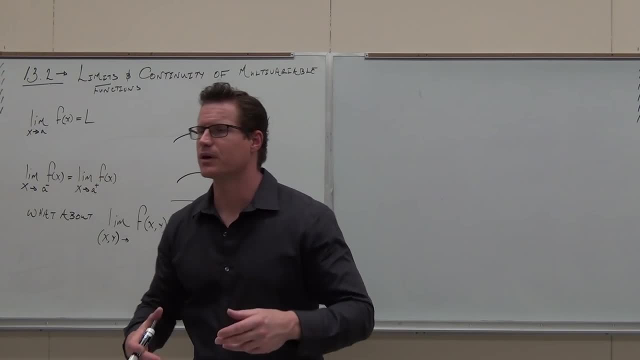 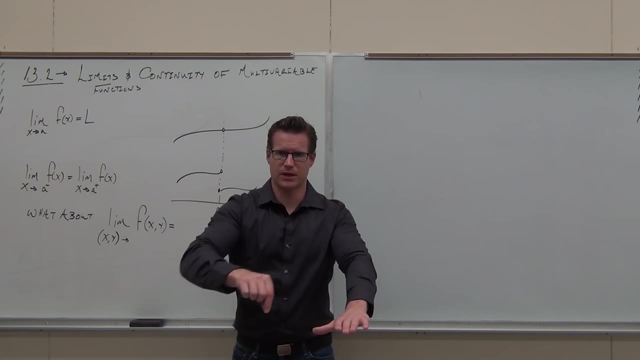 do you remember doing this from last section? You know you've got to go back and kind of remember this, but what we're doing here is we're plugging in order. That order pair is along the x-y plane. We're plugging in that pair. 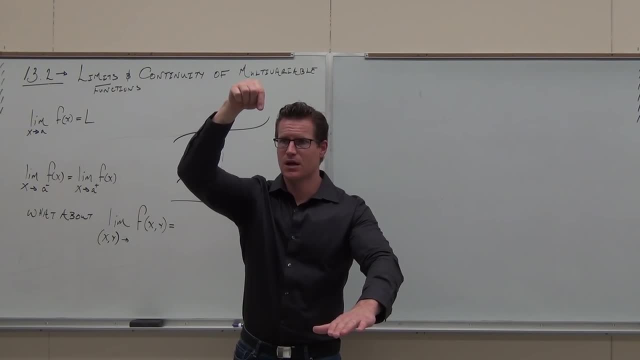 That order pair has given us a height above the point on the x-y plane. Does that make sense? So we have to traverse this plane? We have to traverse the plane now and see what's the height doing as we're traversing this plane. 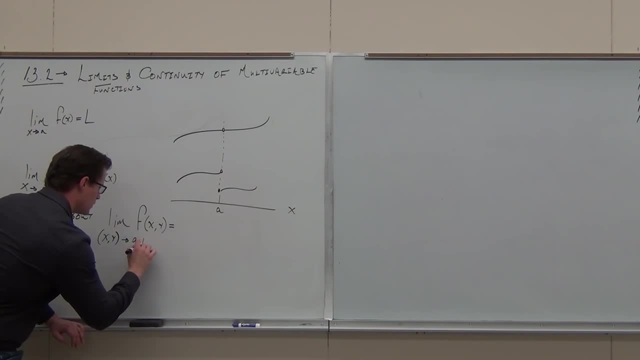 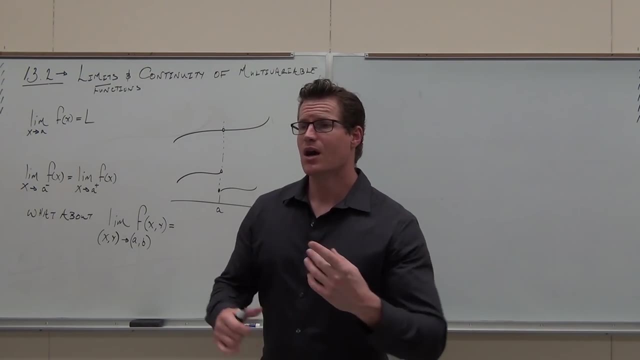 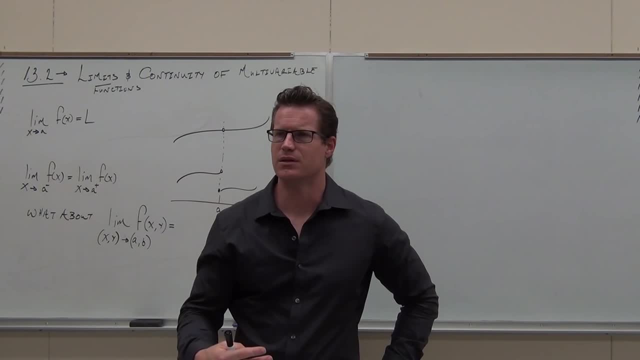 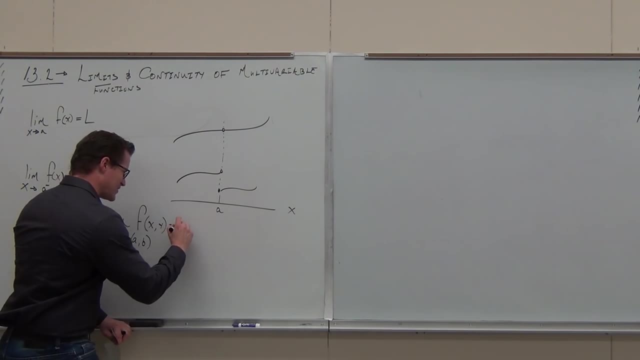 What, What, What, What. From what direction? How are we doing this? What is the curve in this case? And this is the whole situation? How do we know this limit exists? Well, if it equals L Done Yay, That doesn't tell you nothing. 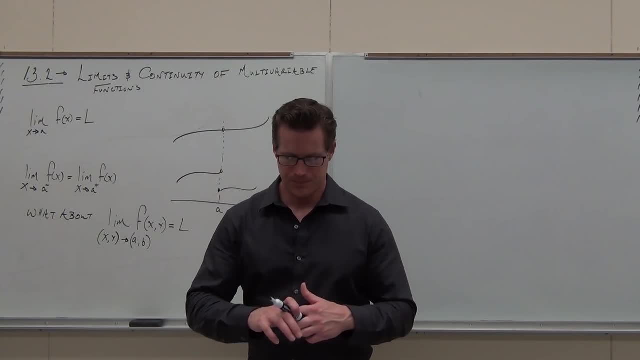 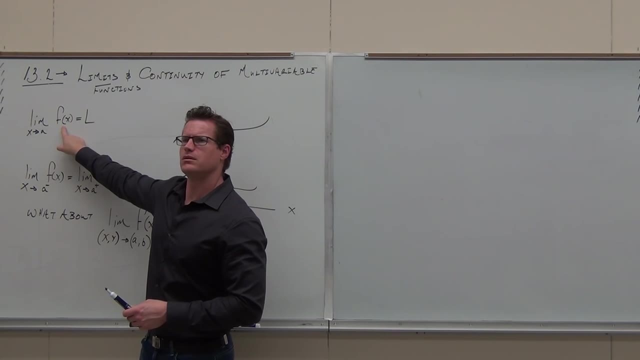 That tells you nothing. Here's the issue. We just covered part of it. What's that give you? What's a function in one variable? What's it give you? Come on, Gives you a curve. what you said on a. 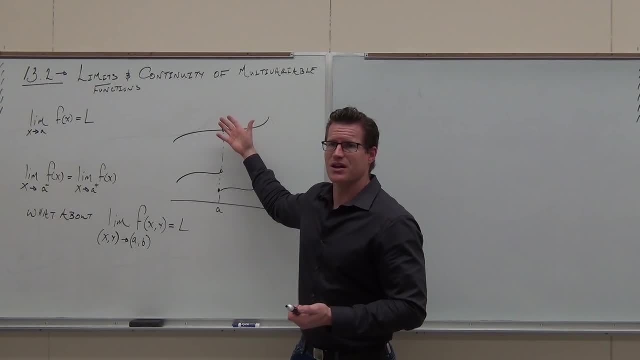 On a plane. this is just a curve on a plane. that's all it is. What does, and this is the whole reason why I had the last section, so you get really good at this. okay, What does a function in two independent variables give you? 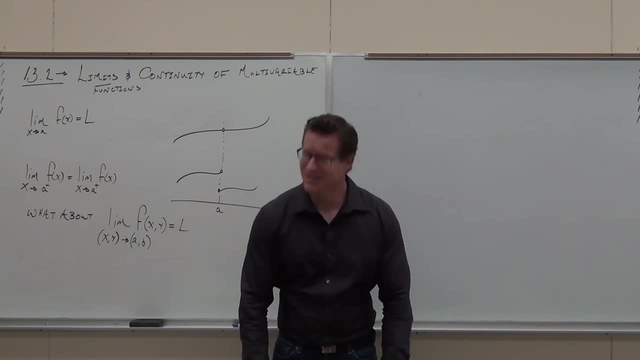 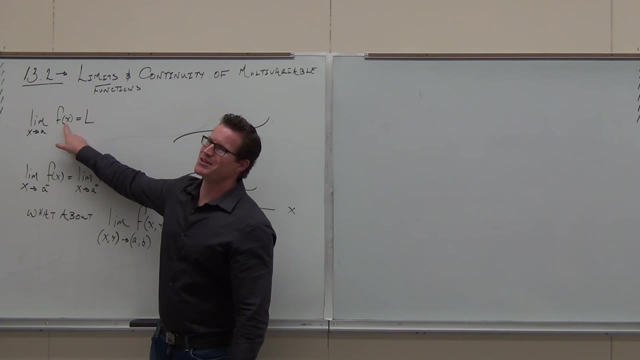 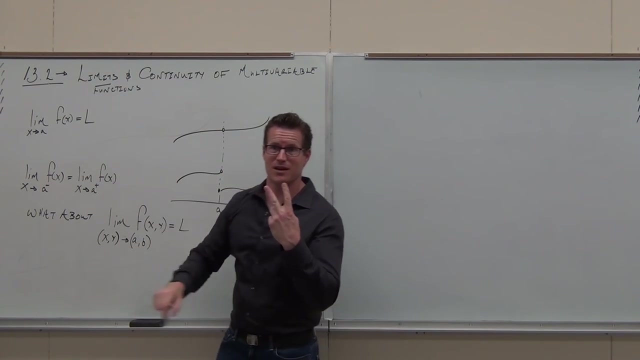 It's not a curve. that's the whole point. If it was a curve it would be easy. we'd have calc one again done. One variable you need: how many dimensions is the graphic Two? Ah, Don't make me drop this one dimension, okay. 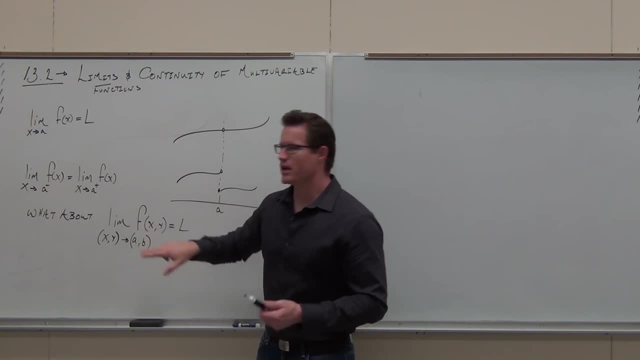 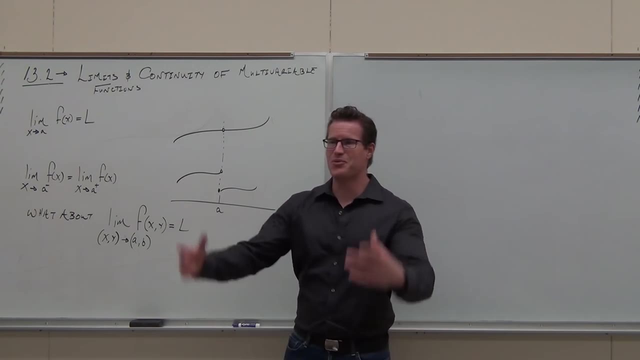 so you get really good at this. okay, What does a function in two independent variables give you? It's a curve on, It's not a curve. That's the whole point. If it was a curve, it'd be easy. We'd have calc one again done. 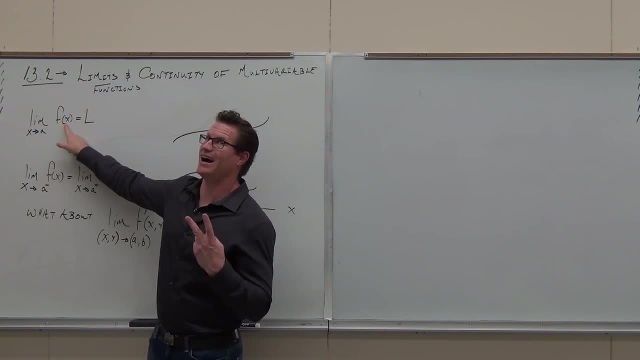 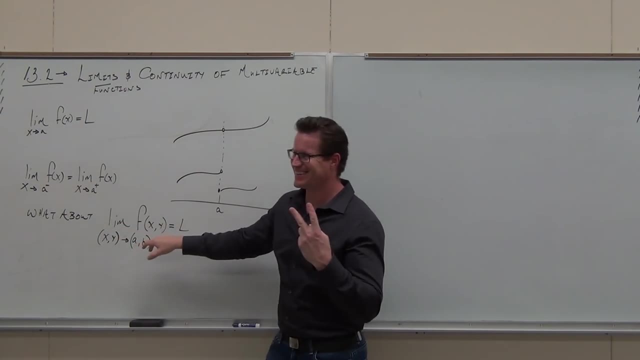 One variable. you need how many dimensions to graph it? Two: Ah, Don't make me drop this one dimension. okay, I'll do it. Two variables: how many dimensions do you need to graph a function with two independent variables? Three: 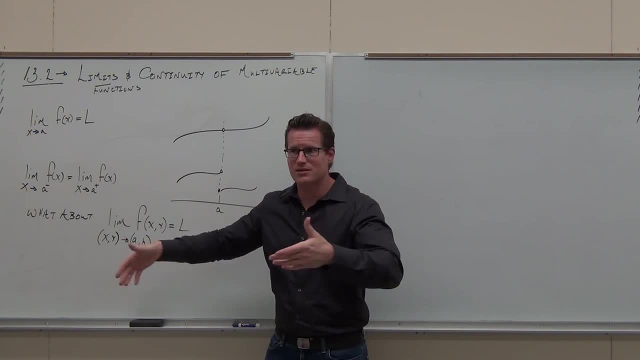 Three. That means it's a Service Service. Remember, we were just talking about this. You go to a point you get a high. My place is getting better, It's squeaky. come on, don't do that to me. 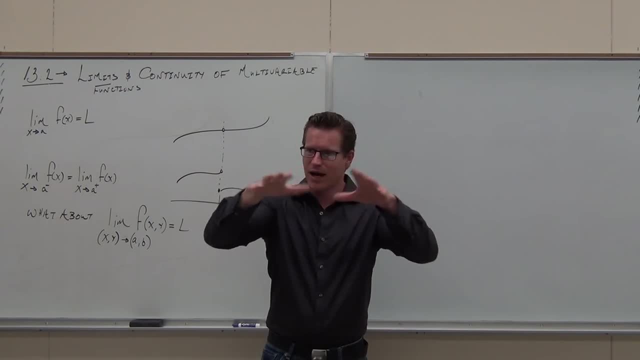 You go to a point on the plane, you get a height. A lot of different heights creates a service for you. What we're talking about on this situation is: what's the height of the function? doing as I'm allowing my point to get close, 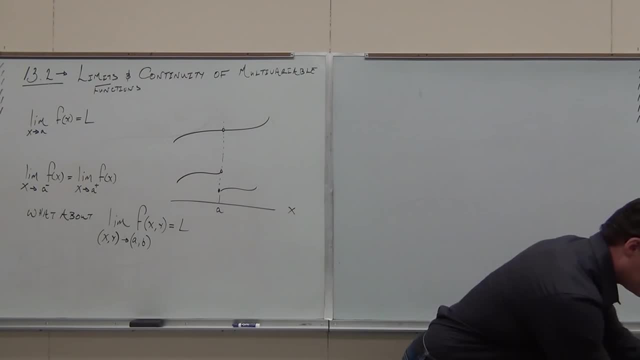 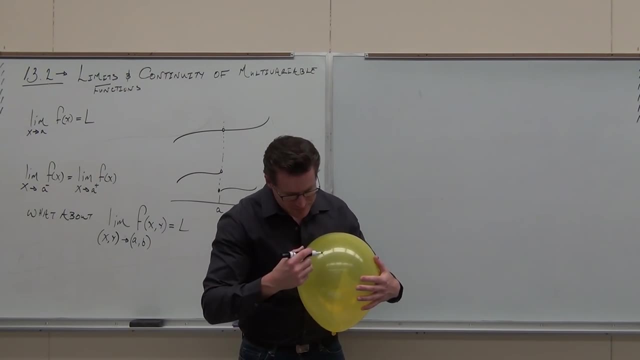 to here. but there's a big problem, and here's the problem: Service Point, Out of the point. how do you feel all the time in this class, right? Just kidding? Let's say that this is my point, all right? 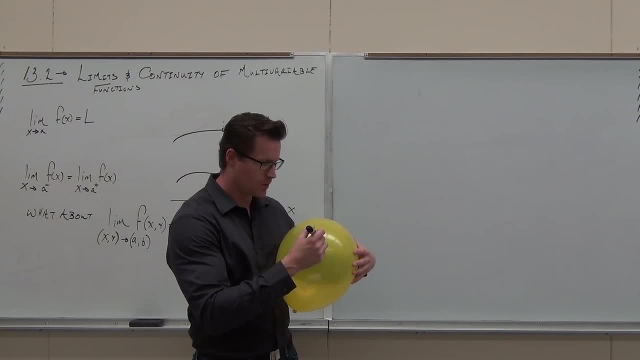 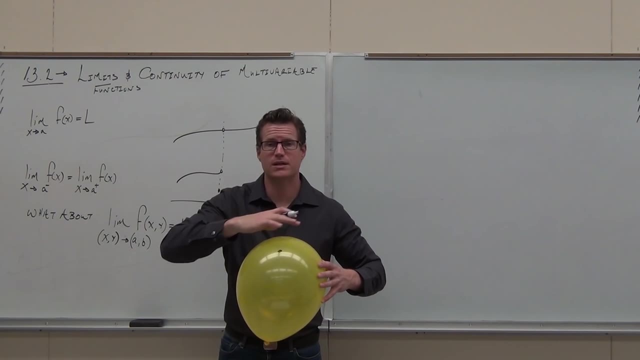 This is my point right here. This is the point AB or well, the height above the point. So you've got to imagine that this is the height, The whole idea here. the point is that this point is on the surface. 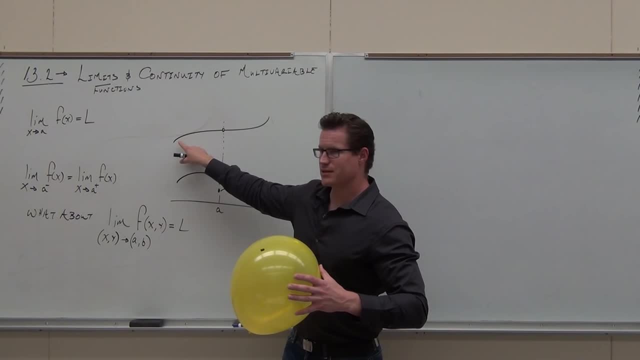 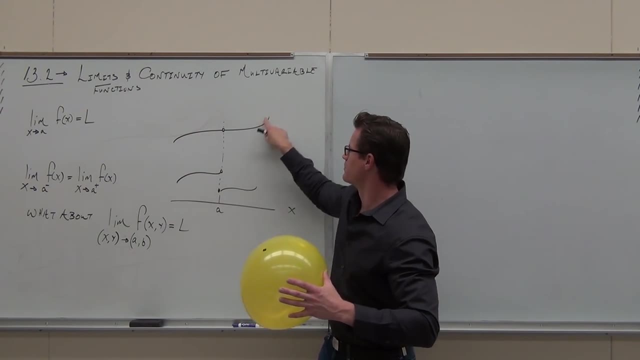 Here's my question: If the limit here says- and this is the whole reason why we did it- you have to travel not along the axis but along the curve, What's the height of the curve doing from both directions? What's the height of the curve doing from both directions? 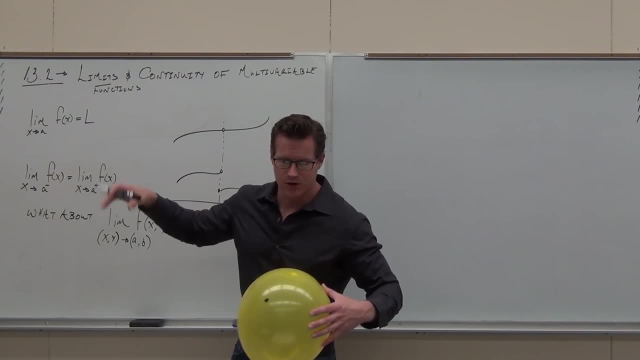 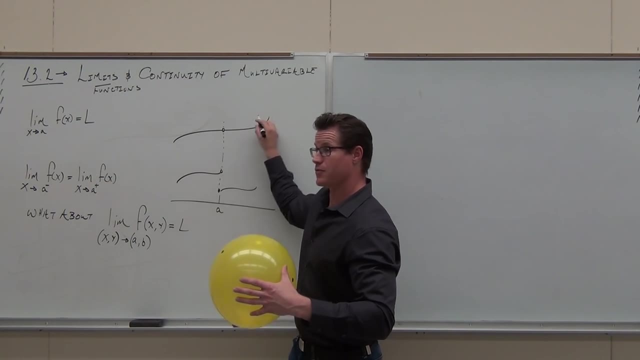 Well, that gives you one path. You see, on a curve there's a certain path. There's only two ways you can get to this value: from the left and from the right. That's two ways. If they equal, from the left and from the right, we say that's it. 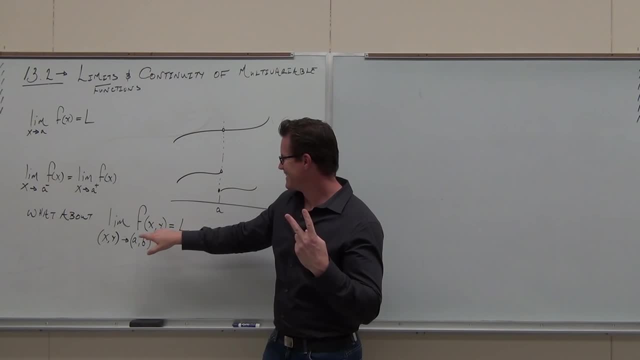 Okay, I'll do it. Two variables- how many dimensions do you need to graph a function with two independent variables? Three, That means it's a surface. Remember, we were just talking about this. You go to a point, you get a height. 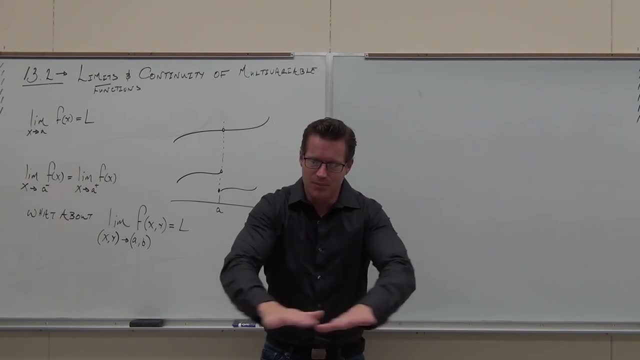 My place is getting squeaky. come on, don't do that to me. You go to a point on the plane. you get a height. A lot of different heights creates a surface for you. What we're talking about on this situation is: what's the height? 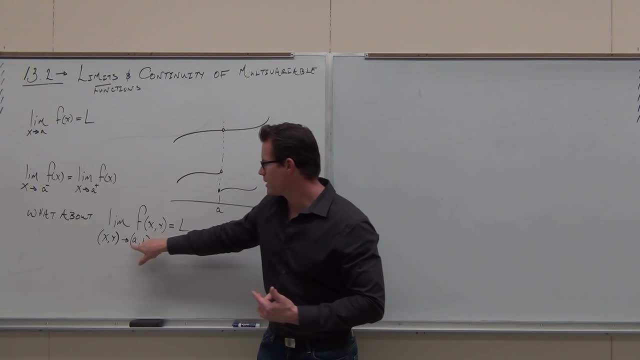 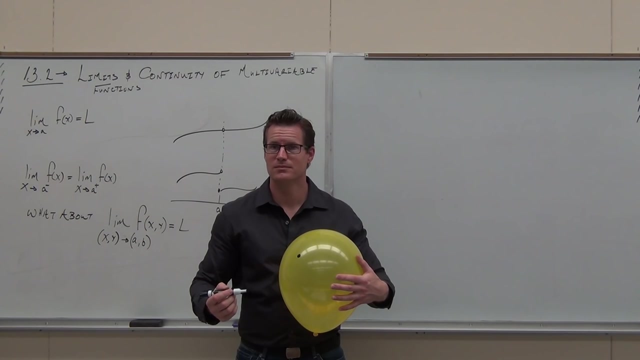 of the function, doing As I'm, allowing my point to get close to here. But there's a big problem and here's the problem: Surface Point. Other point: How you feel all the time in this class, right? Just kidding. 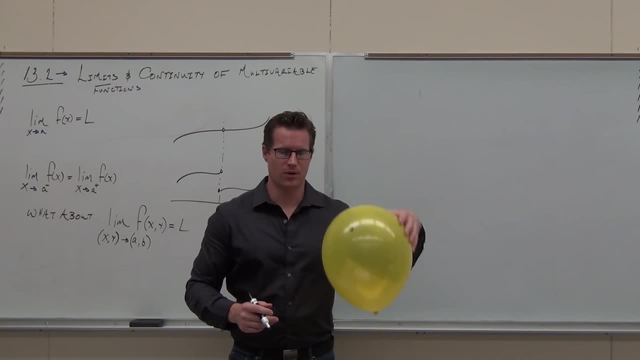 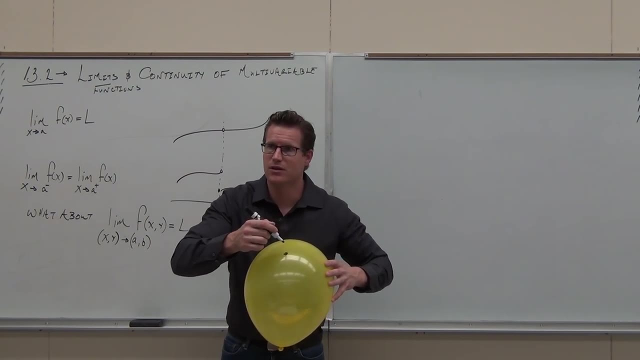 Let's say that this is my point. All right, This is my point right here. This is the point AB, or well, the height above the point. So you've got to imagine that this is the height. The whole idea here. the point is that this point is on a surface. 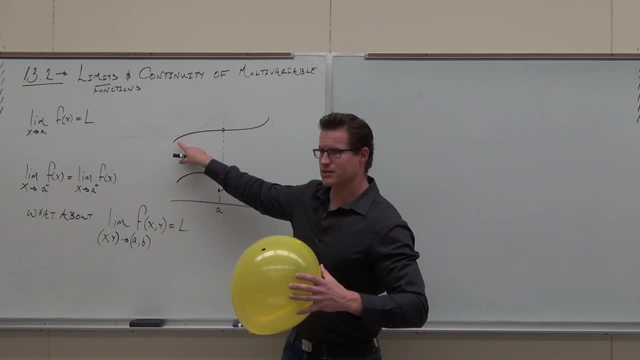 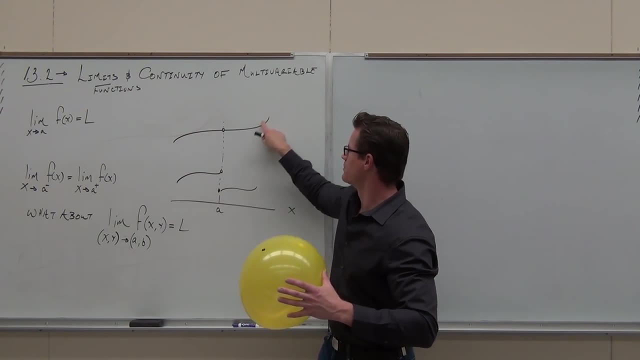 Here's my question: If the limit here says- and this is the whole reason why we did it- you have to travel not along the axis but along the curve, What's the height of the curve doing from both directions? What's the height of the curve doing from both directions? 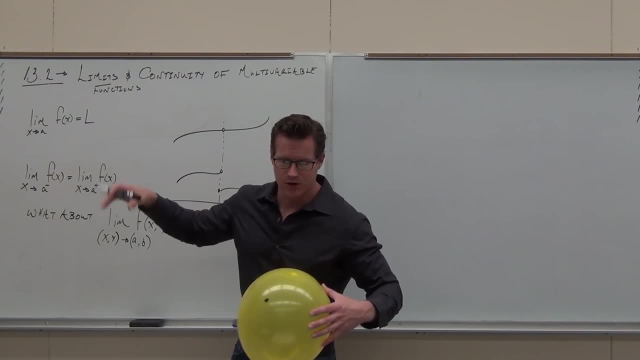 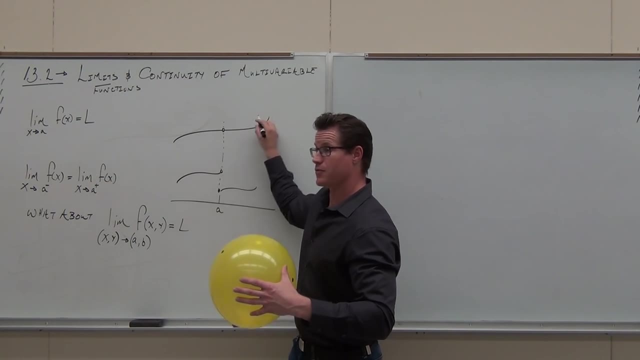 Well, that gives you one path. You see, on a curve there's a certain path. There's only two ways you can get to this value: from the left and from the right. That's two ways. If they equal, from the left and from the right, we say that's it. 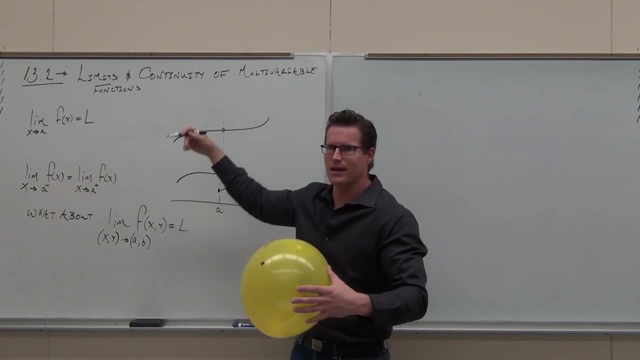 That's the only two ways you can get there. There's no magic third way, coming from imaginary land. all right, This isn't Harry Potter with a math wand Done. That's not what we're talking about. There's literally only two ways. 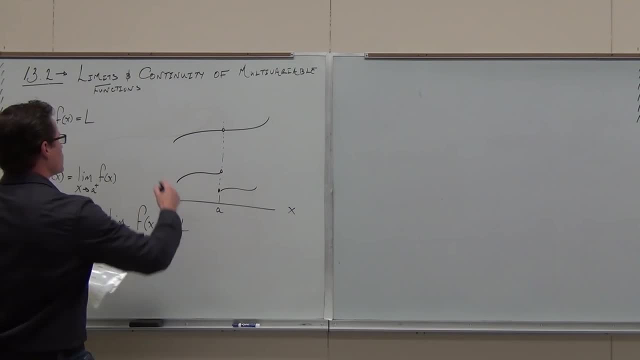 So when we're doing this, we say okay for one variable. it's kind of comfortable. I think I'm going to have to balloon all the time just because I'm running out of time. I'm going to have to press my arm right there. 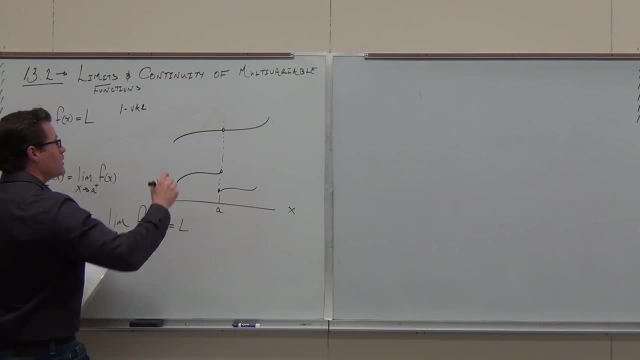 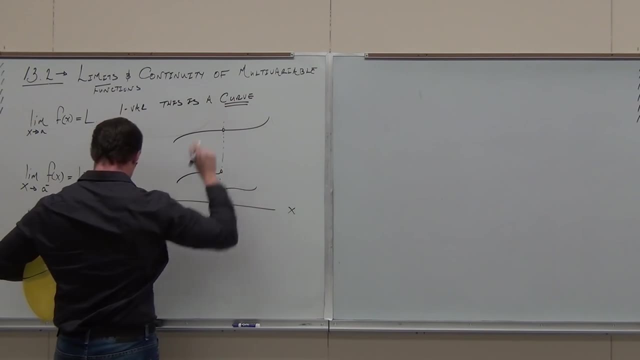 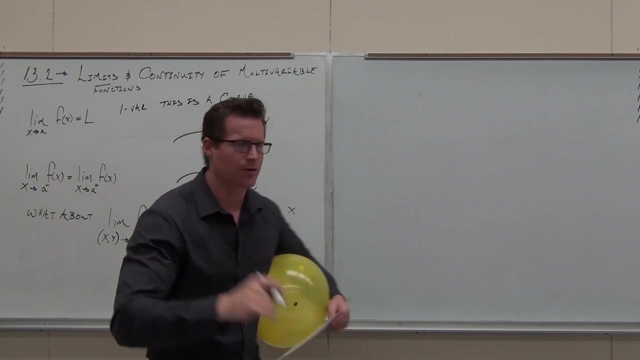 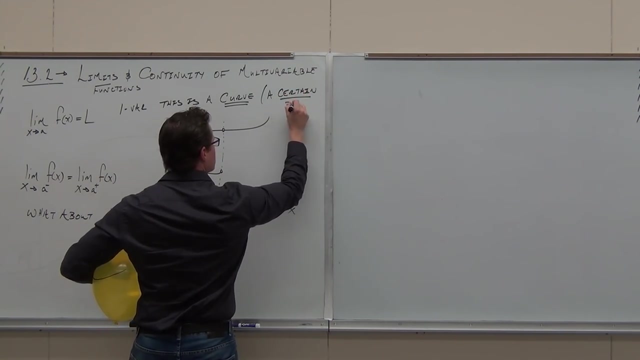 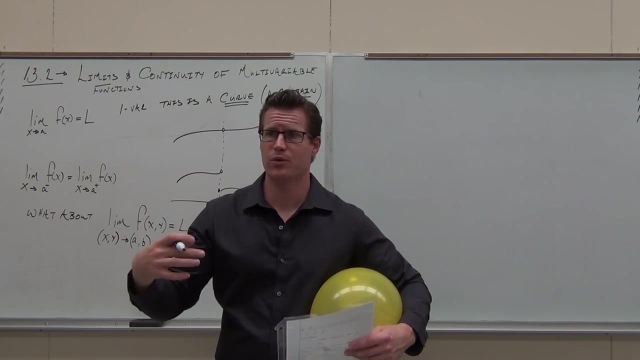 Perfect For one variable. this is a curve. It's a curve, It's a certain path. There's only one path, And what that means. the whole important thing about this, the reason why we're able to find limits so easily in Calc 1, is there are only two directions. you 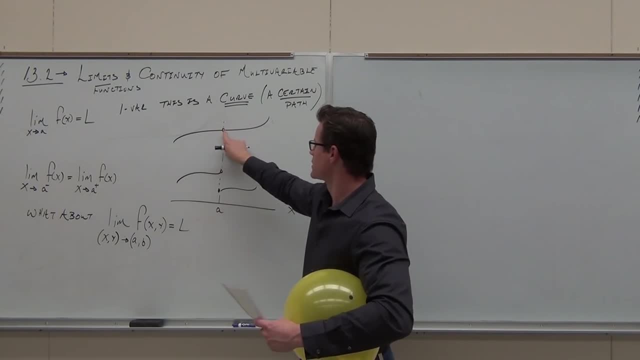 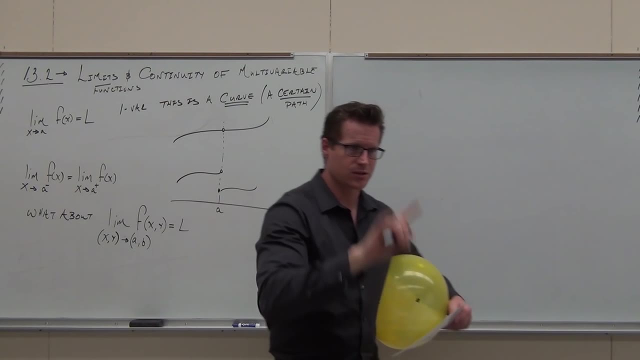 can take to get to this value. You can go from the left and you can go from the right. There's only two directions that you can take to this value: from the left and from the right, So that limits us to two directions. 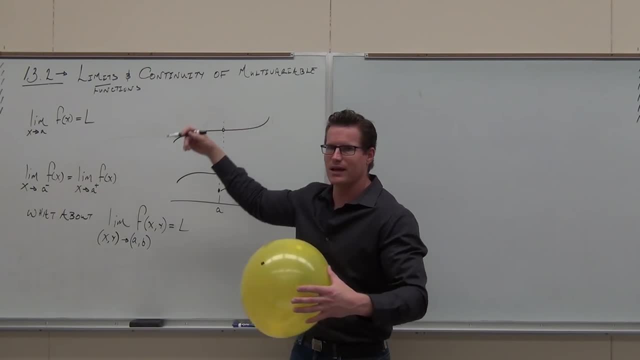 That's the only two ways you can get there. There's no magic third way, coming from imaginary land. all right, Doesn't Harry Potter, Harry Potter with a math wand Done? That's not what we're talking about. There's literally only two ways. 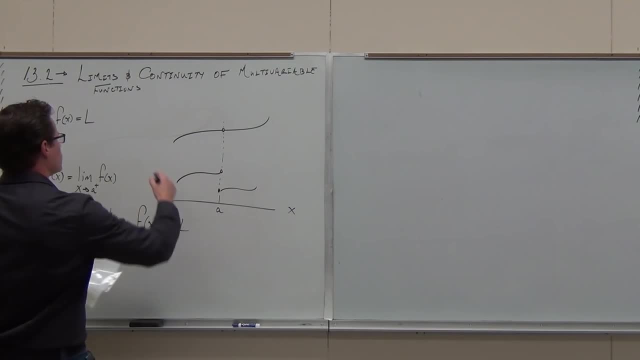 So when we're doing this, we say okay for one variable. it's kind of comfortable. I think I'm going to have to balloon all the time just because the rest of my arm is right there. Perfect For one variable. this is a curve. 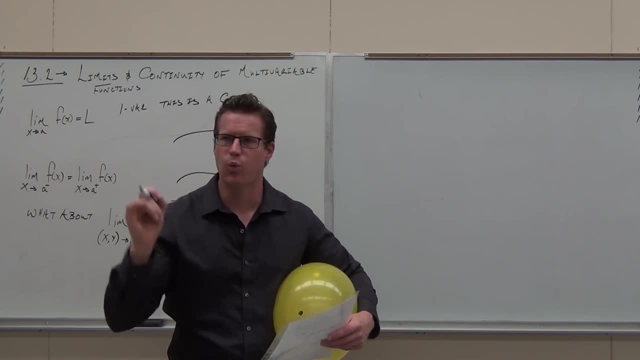 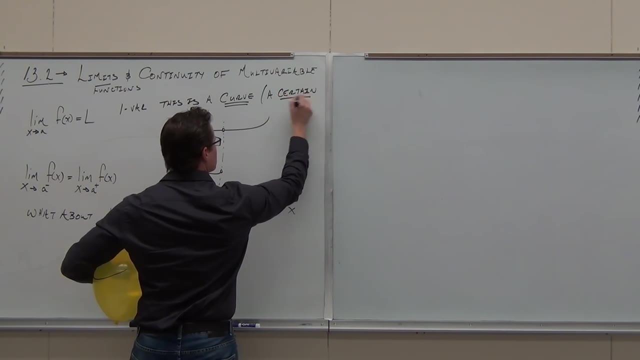 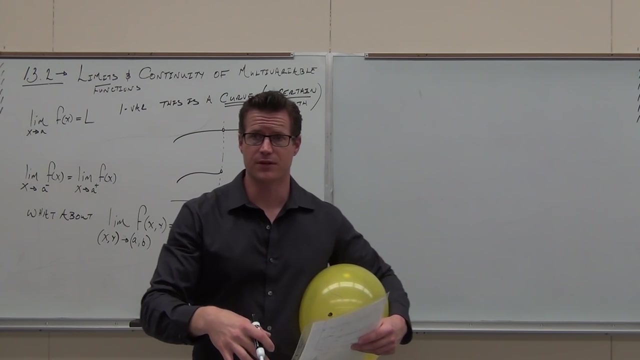 It's a curve, It's a certain value, It's a certain path. There's only one path And what that means, the whole important thing about this, the reason why we're able to find limits so easily in Calc 1,. 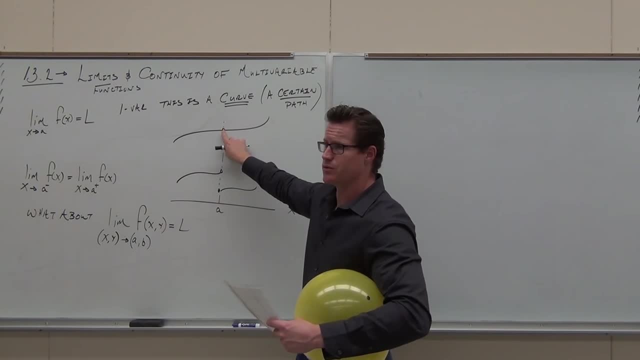 is. there are only two directions you can take to get to this value. You can go from the left and you can go from the right. There's only two directions that you can take to this value: from the left and from the right. 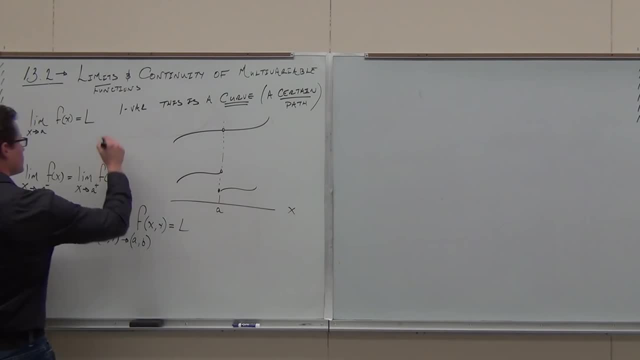 So that limits us to two directions. I'm going to say point. what I mean is the value. I'm going to say point, just so it makes a little more sense for this. But here's the whole point, Here's the whole idea. 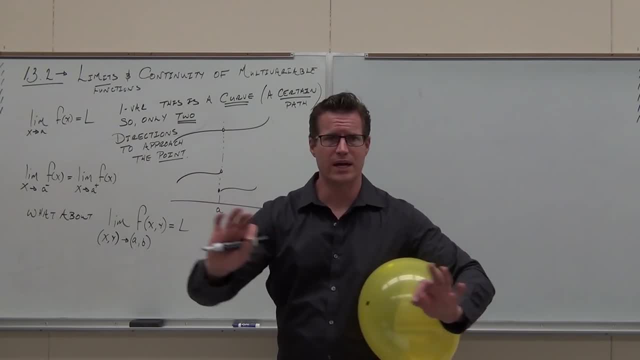 With one variable. you have one path, You have a certain path. There's only two ways you can approach that value, that point: From the left, from the right. show of hands. you understand the concept. Here's the idea now. 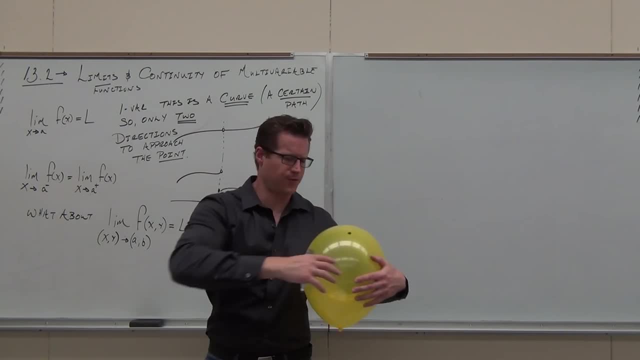 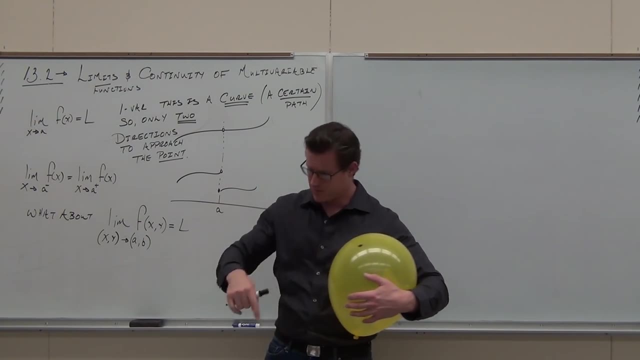 You've got a surface, I say: tell you what I want you. this is the function. all right, This is what this means. You already told me that two independent variables creates a surface. Let's pretend this is it, and I want to let my points. 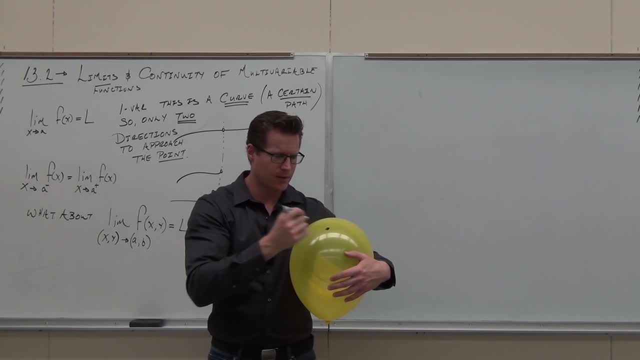 my things that are creating this height get to that value. How many ways can I approach that? This is the surface, right? Yeah, Which means that my function is going to get to that value. Yeah, My function is traveling along this. 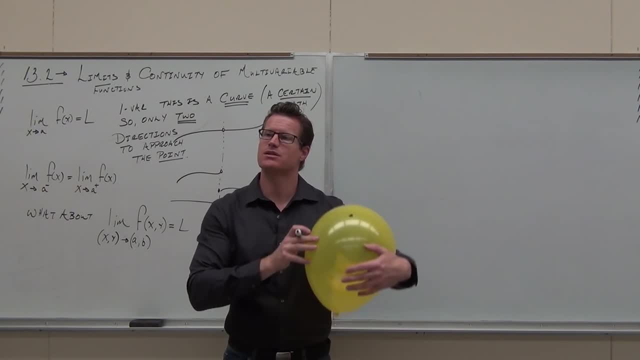 How many paths can I take to get here? Imagine, this is a mountaintop and here's a little cabin, That's a horrible cabin, And you say: hey, I want to get, I want to get to my cabin, And there's no roads. 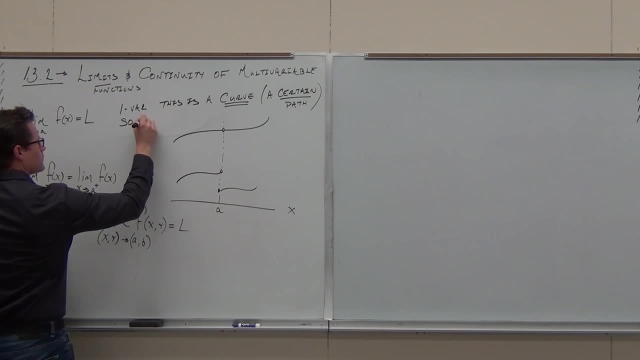 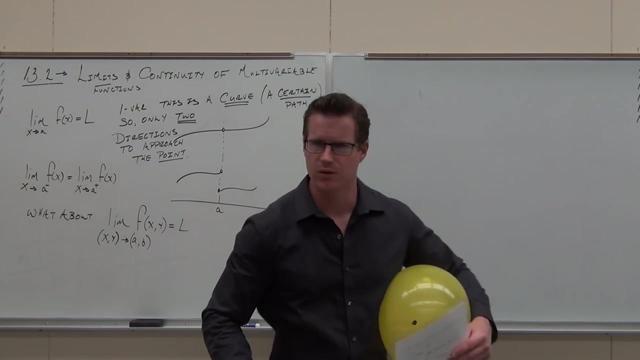 I'm going to say point. what I mean is the value. I'm going to say point just so it makes a little bit more sense for this. But here's the whole idea: With one variable, you have one path, You have two paths. 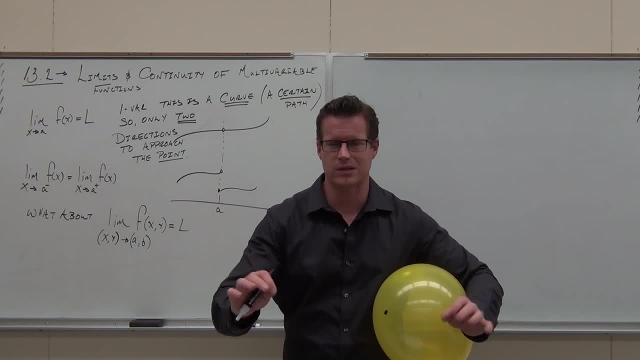 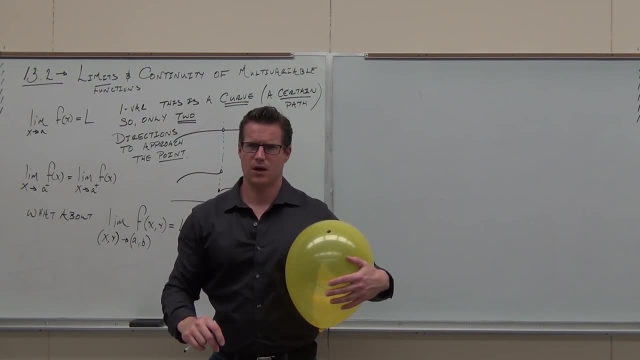 You have a certain path. There's only two ways you can approach that value, that point: from the left, from the right. Show of hands. you understand the concept, Here's the idea. now You've got a surface, I say: tell you what I want you. this is the function, all right. 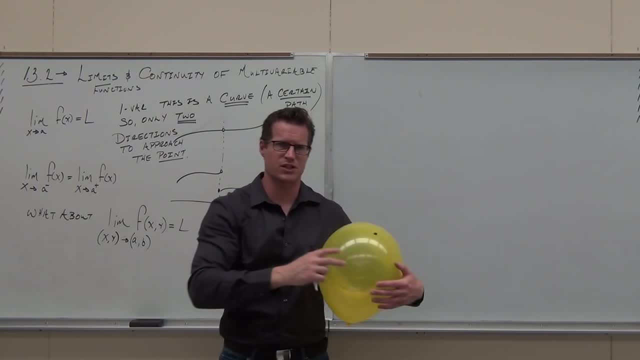 This is what this means. You already told me that two independent variables creates a surface. Let's pretend this is it And I want to let my points, my things that are creating this height, get to that value. How many ways can I approach that? 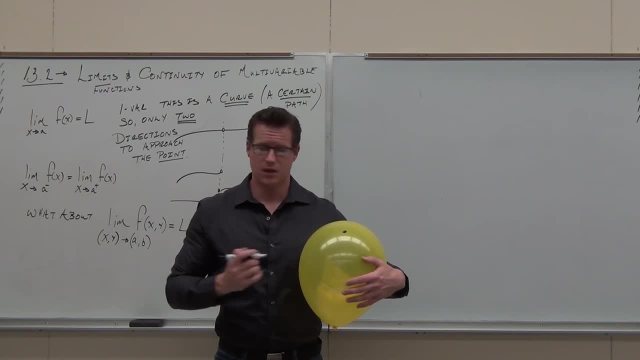 This is the surface right, Which means that my function is traveling along this. How many paths, How many paths can I take to get here? Imagine: this is a mountain top and here's a little cabin. That's a horrible cabin. 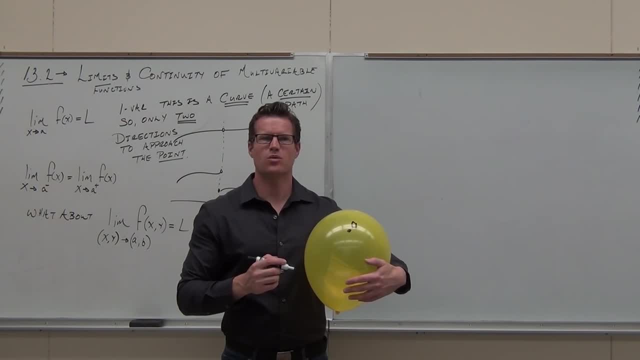 And you say: hey, I want to get to my cabin And there's no roads, Pick any roads you want. How many roads can you take to your cabin? I can do this right, I can take that road, or I could take this road, or I could go. 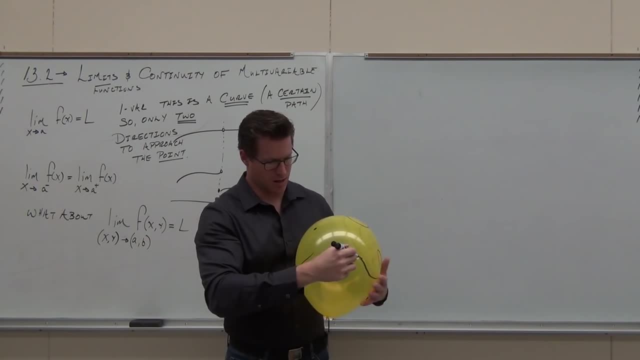 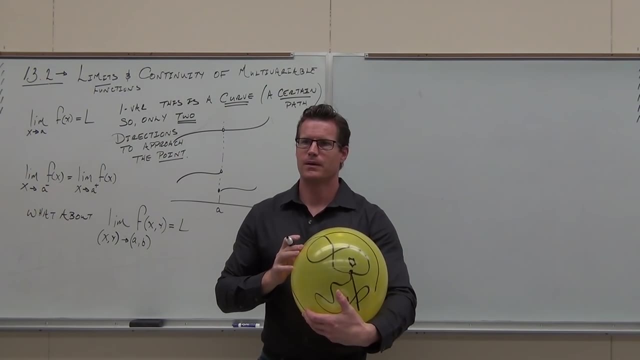 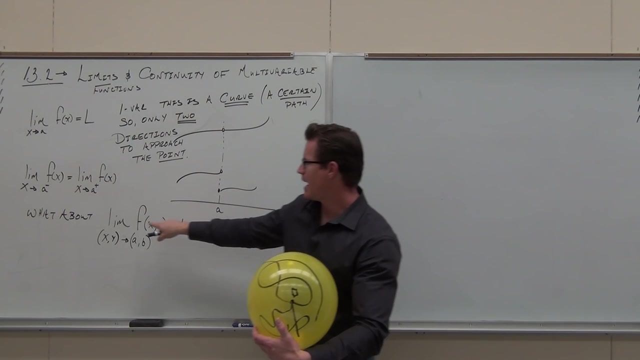 this way, or I can start over here and go. I like smiley, I want to start smiley, I'm not drunk And I go. what? Yeah, I'll go over here. Here's my question: How many paths, paths along your surface? how many paths along your surface could possibly? 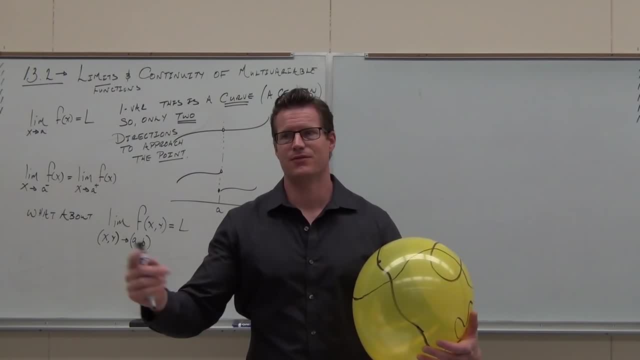 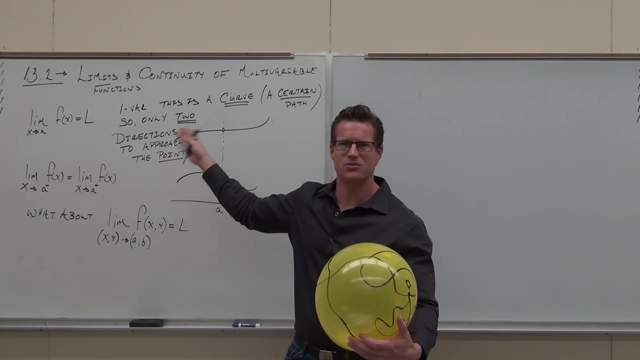 get you to that point? How many Infinite, Infinite. That blows this thing out of the water. There aren't just two paths anymore. Do you guys get the idea? Do you guys get the idea that curves are two paths? Left right done. 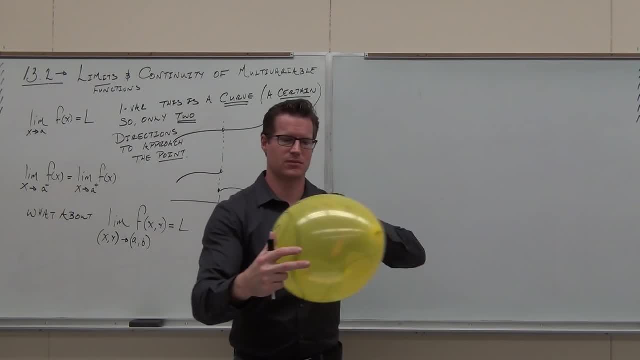 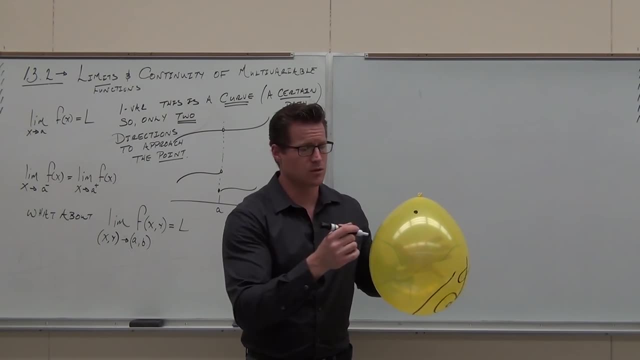 On surfaces. how many paths? wow, I completely kind of functioned that thing up, didn't I Really worked it out. So how many paths can you take to get to a point? An infinite many You could go left Doesn't make sense. 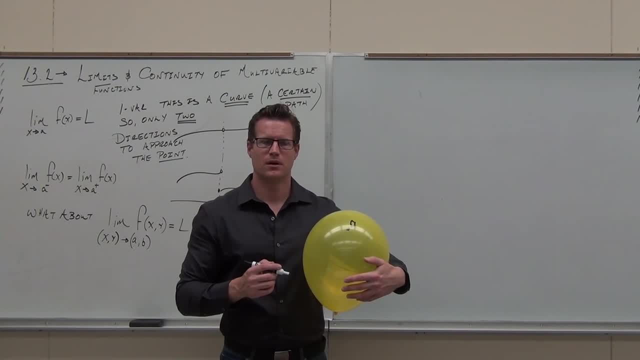 Pick any roads you want. How many roads can you take to your cabin? I can do this, right, I can take that road, or I could take this road, or I could, I could go this way, or I can start over here and go. I like smiley. 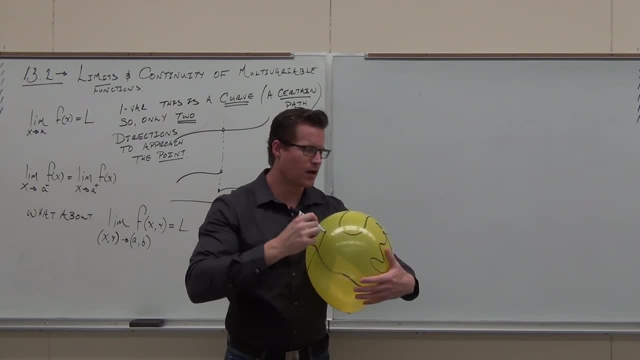 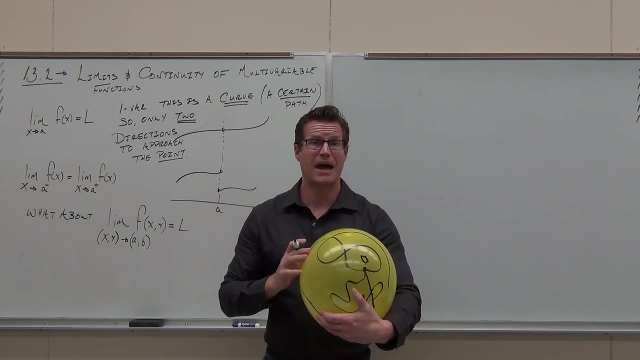 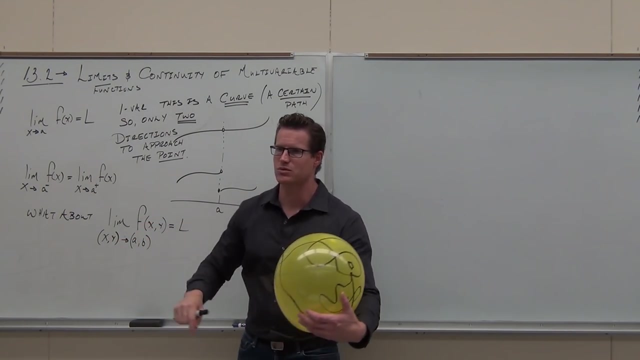 I'm going to start smiley. I'm not drunk And I go what? Yeah, I'll go over here. Here's my question: How many paths, paths along your surface, how many paths along your surface could possibly get you to that point? 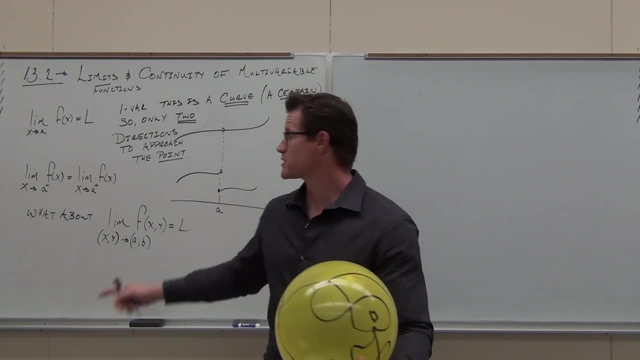 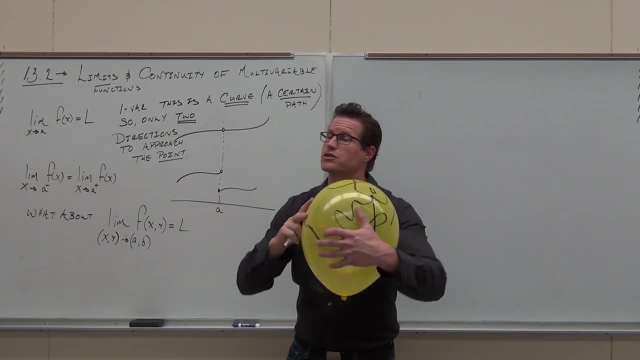 How many Infinite, Infinite. That blows this thing out of the water. There aren't just two paths anymore: Curves. do you guys get the idea that curves are two paths, Left, right, done On surfaces? how many paths? wow, I completely kind of functioned. 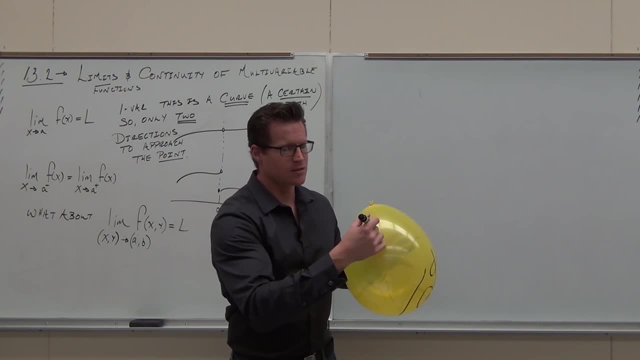 that thing up, didn't I Really worked it out? So how many paths can you take to get to a point? An infinite many. You could go. left doesn't make sense, Right doesn't be up down. You could go infinitely many paths to get to this point on a surface. 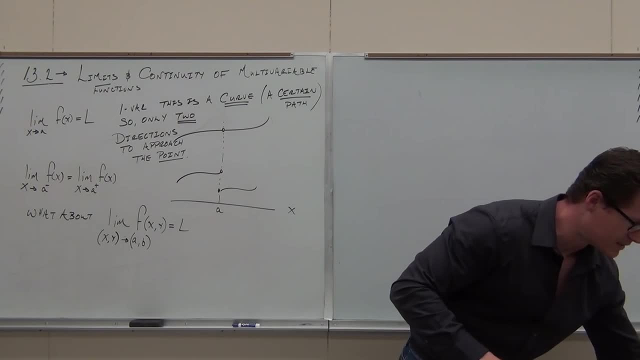 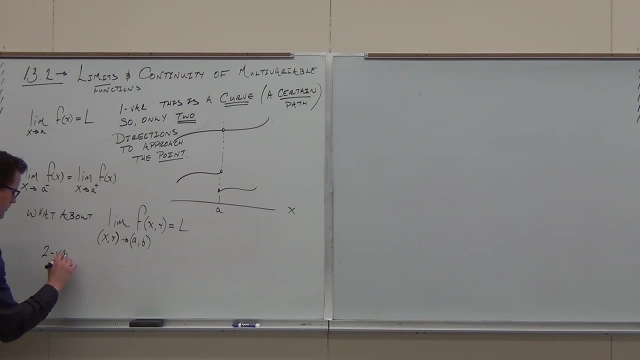 Do you guys understand the idea? Let's write out a couple of those ideas and then I'll show you what we can do, what we can't do. So for two variables. it's no longer a curve. This function is a surface. 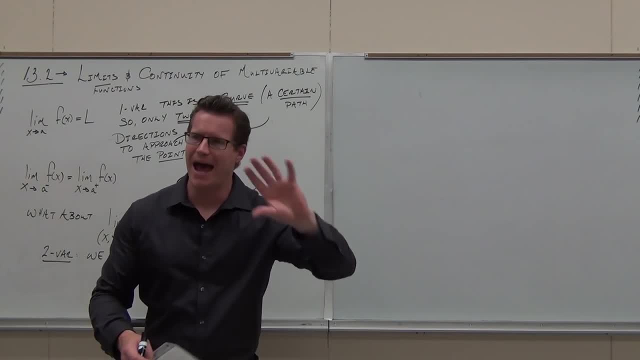 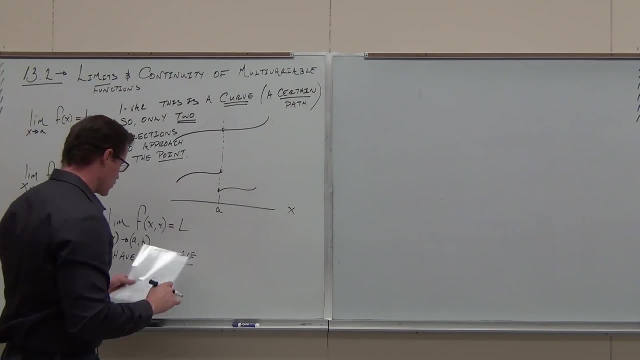 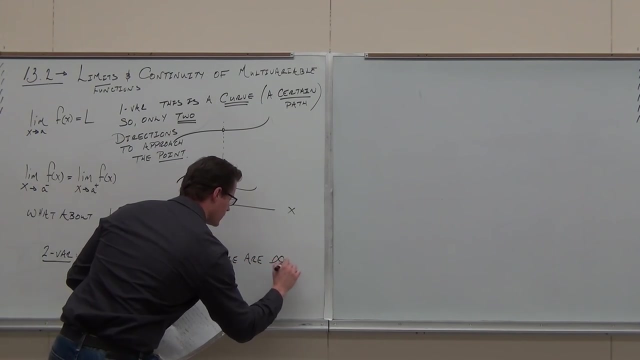 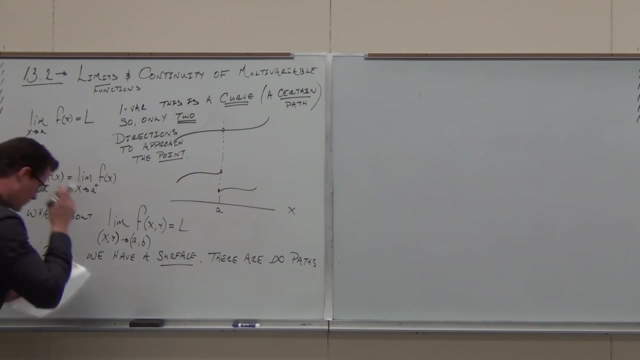 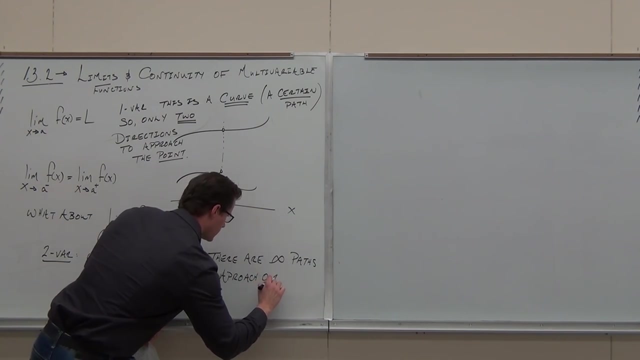 And the problem is there's an infinite number of paths along that surface that could intersect That point, that could get to that value on the function. And the answer to that is: the first step is to get to the point where the set of paths is greater than the set of paths. 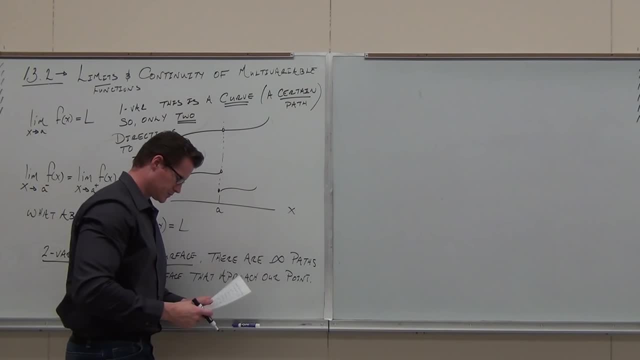 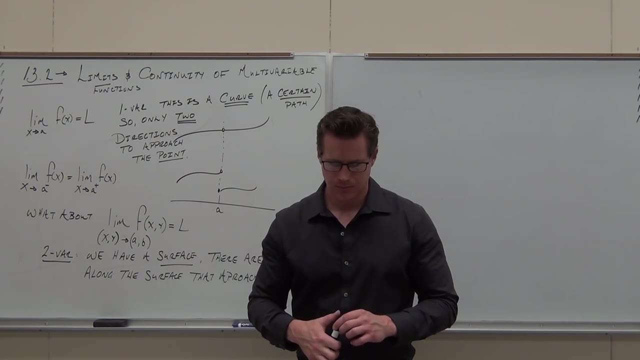 So the first step? the first step is to get to the point where the set of paths is greater than the set of paths. So you and I, in this case, we're going to write a set of paths. I know I've talked it for a while, so I'm just going to talk about it. 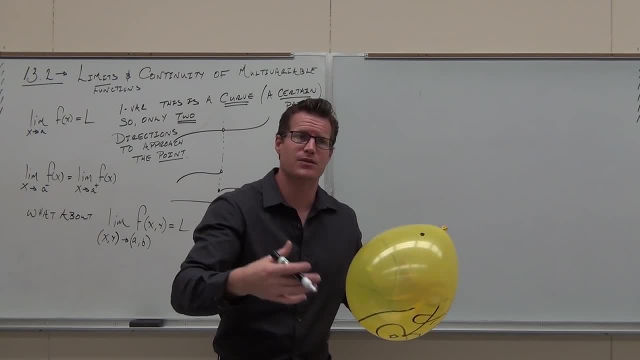 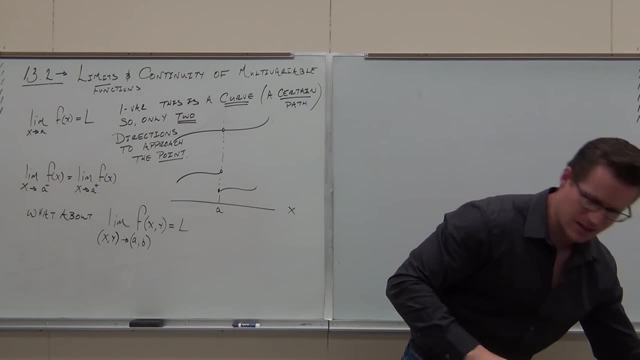 Right doesn't be up down. You could go infinitely many paths to get to this point on a surface. Do you guys understand the idea? Let's write out a couple of those ideas and then I'll show you what we can do and what. 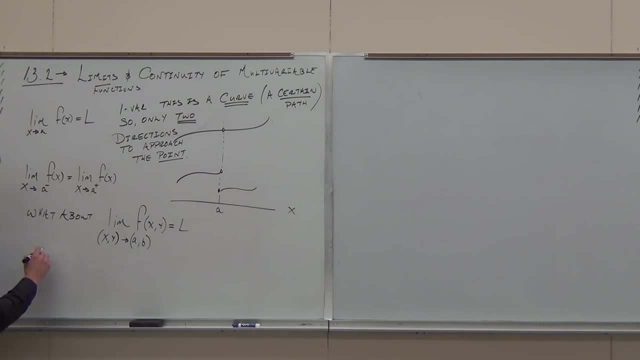 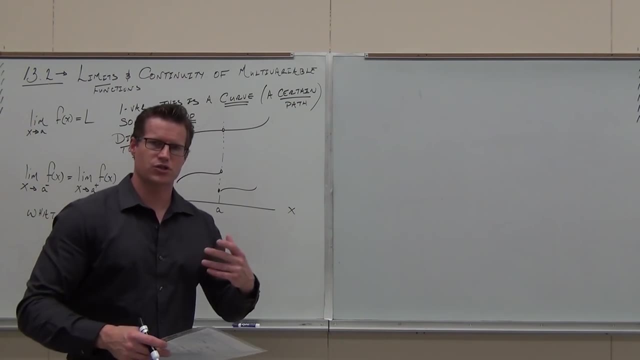 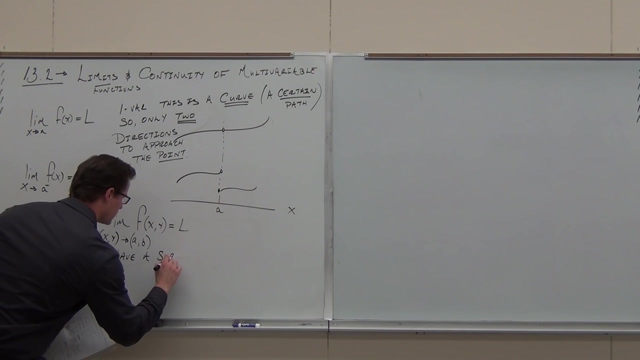 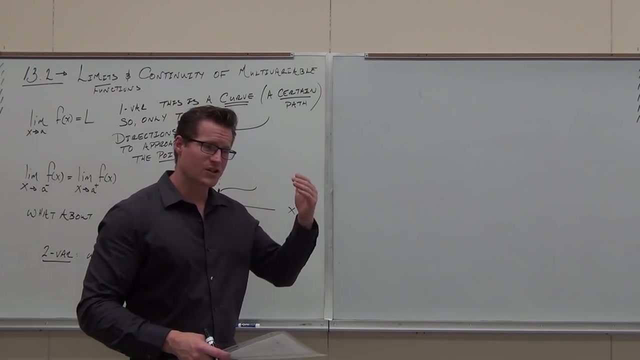 we can't do So for two variables. It's no longer a curve, this function is a surface, And the problem is there's an infinite number of paths along that surface that could intersect that point. So what we're going to do is we're going to put that value on the function. 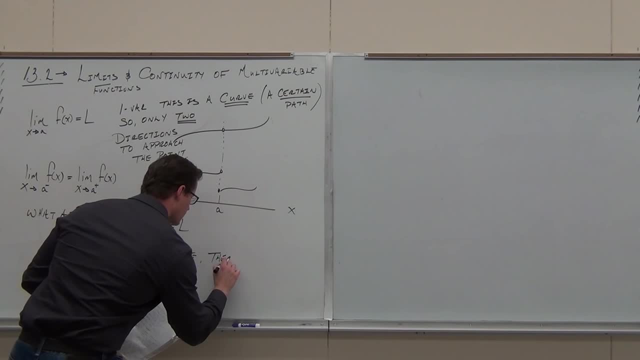 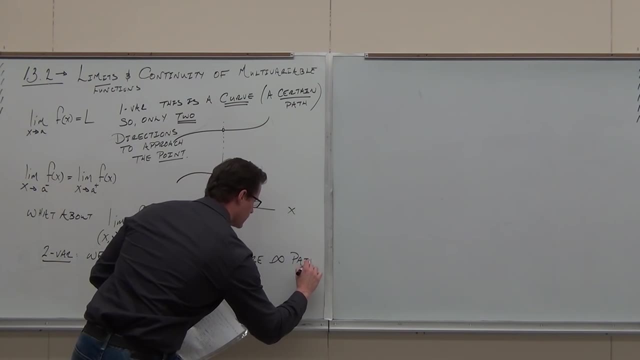 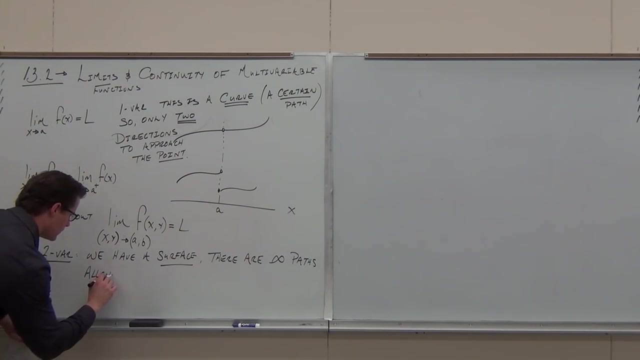 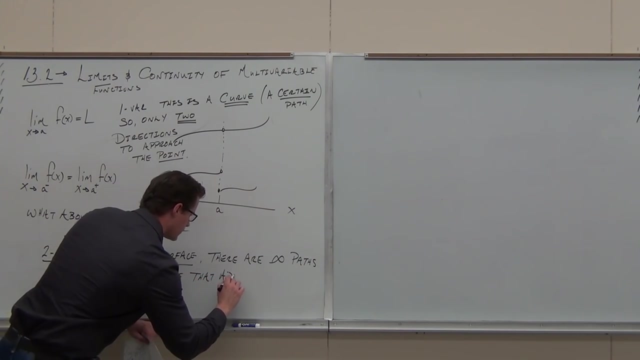 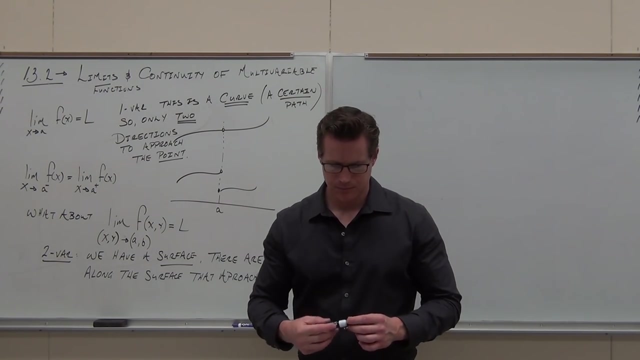 So what we're going to do is we're going to put that value on the function And then we're going to by the number of paths. So we're going to put that value here. I know I've talked it for a while. 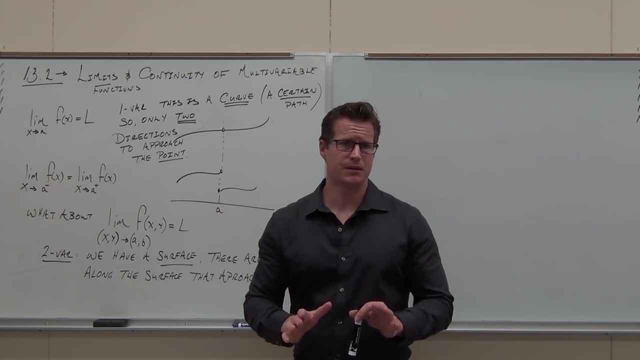 I said I was going to talk about it for about 10 minutes. just so we understand the idea, It's going to take another 10 minutes before we get to a– well, maybe not 10,, 10, to do our first example of why we're going to do that. 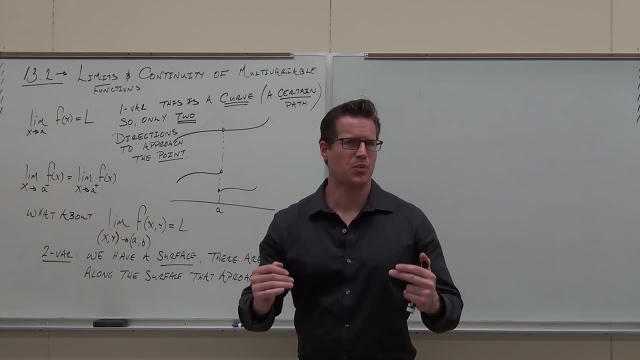 No, it's going to take another 10 minutes before we get to a– well, maybe not 10.. But do you understand the major, major problem between one variable and two or more variables Instead of one, where you have only two directions? 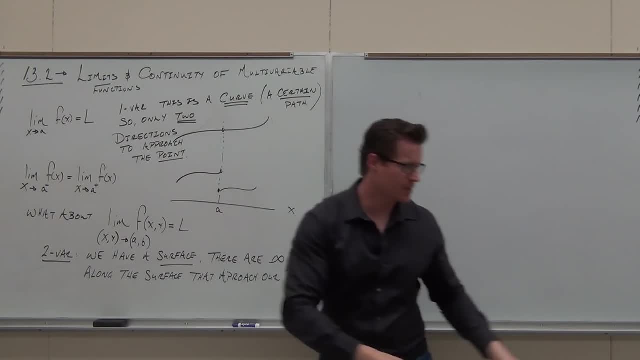 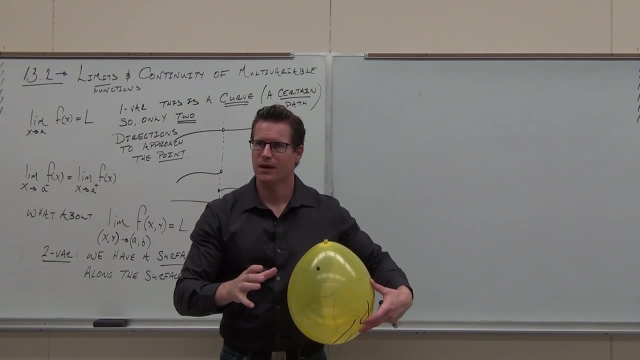 now we have an infinite number of paths that's getting us to our point. Infinite number. Here's the problem. If you wanted to prove that the limit exists on this surface at that value, you have to prove that along all of those paths they get to that point. 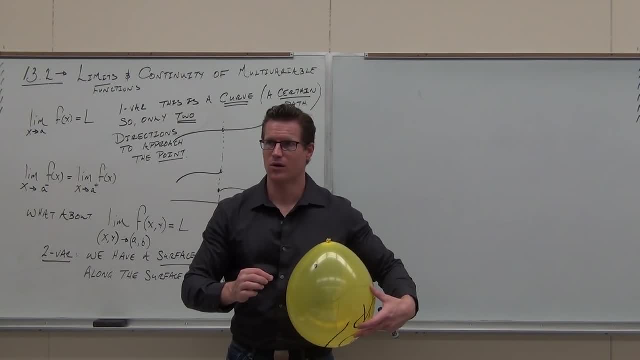 Is that easy to do? Do you want to write out all of the paths? You literally can't, because there's infinite many of them. There's infinite many vector functions, curves that are on the surface, that go here, Infinite many. So how do we do it? 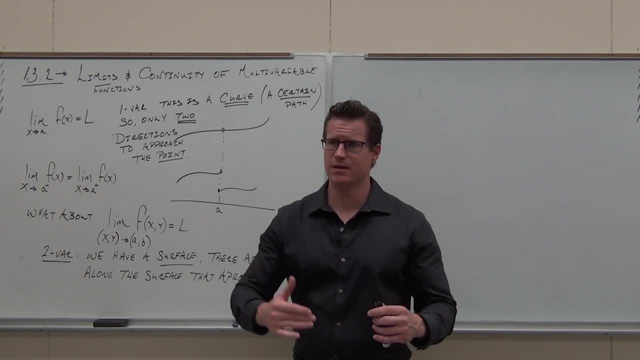 for about 10 minutes, just so you understand the idea. It's going to take another 10 minutes before we get to a- well, maybe not 10, to do our first example of why we're doing that. but do you understand the major? 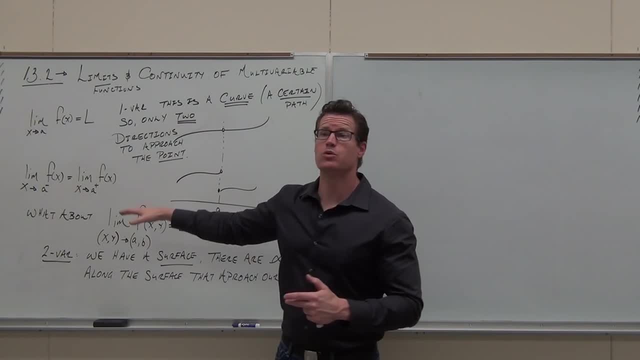 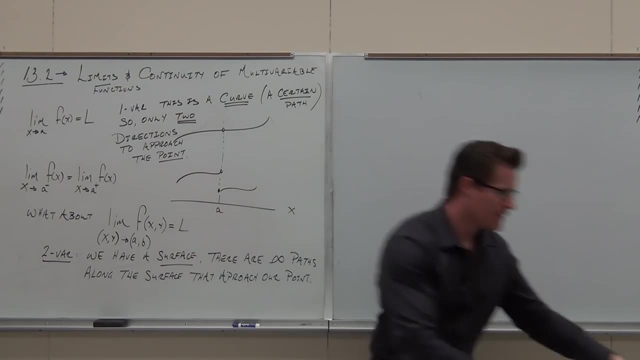 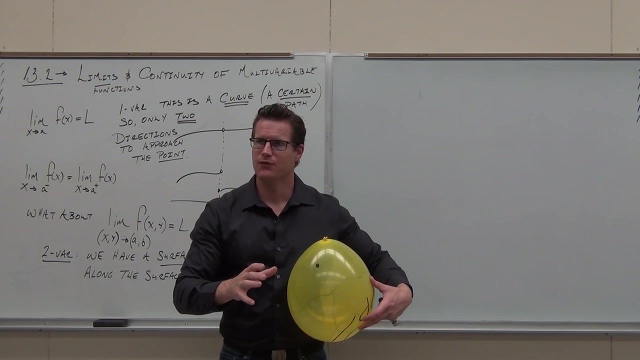 major problem between one variable and two or more variables, Instead of one where you have only two directions. now we have an infinite number of paths. that's getting us to our point: infinite number. Here's the problem. If you wanted to prove that the limit exists on this surface at that value, 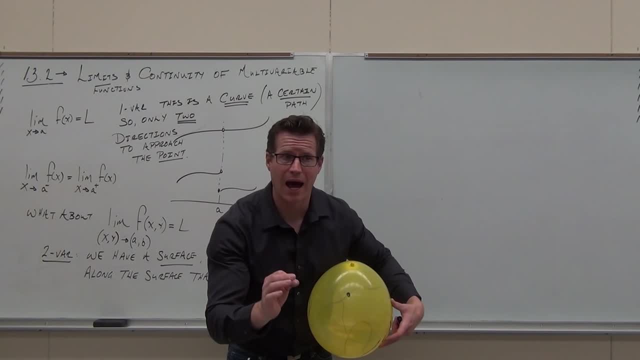 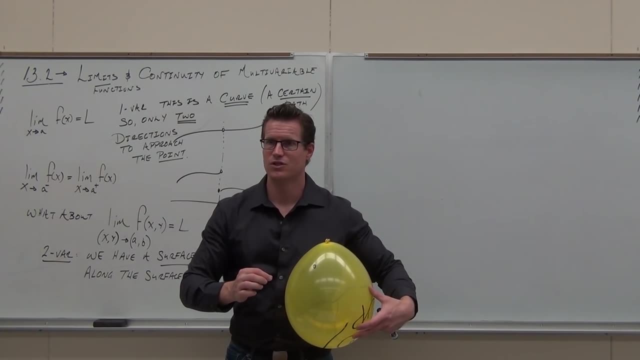 you have to prove that along all of those paths they get to that point. Is that easy to do? Do you want to write up all of the paths? You literally can't, because there's infinite many of them. There's infinite many vector functions, curves. 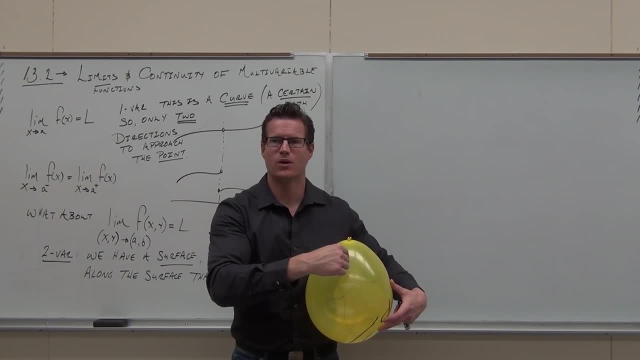 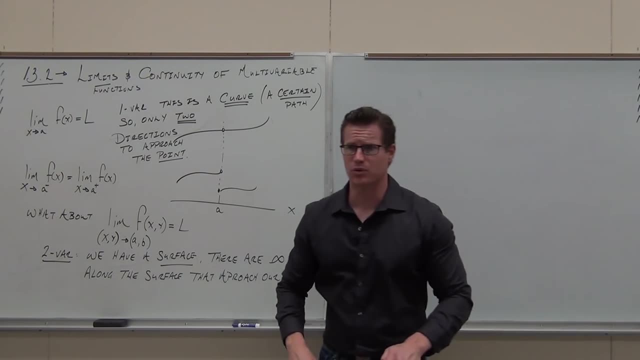 that are on the surface, that go here, infinite many. So how do we do it? Well, it's really hard to do. You should read that: impossible in most cases to do that. We can do it with something called the squeeze theorem. 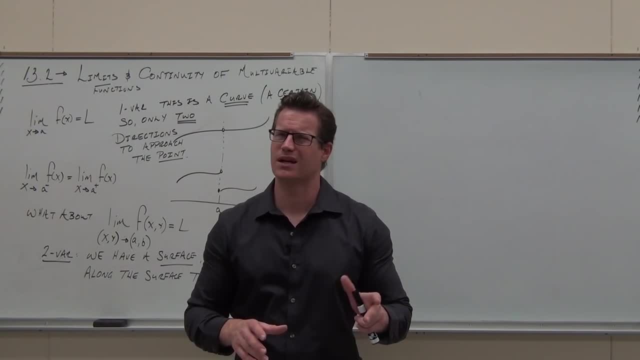 calc one concept, but we're going to use it again. All right, We'll do it later. It's hard, It's not that easy to do. I'll show you how you can prove that limits exist with the squeeze theorem. Do we generally do that? 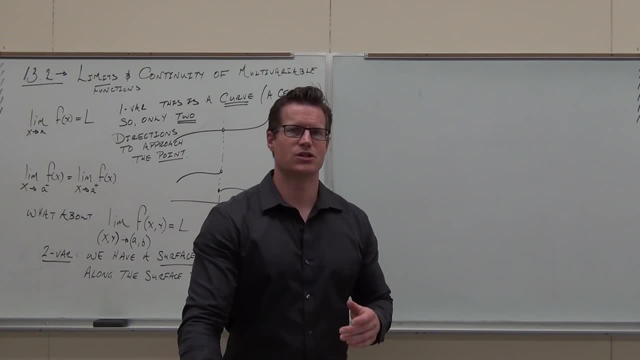 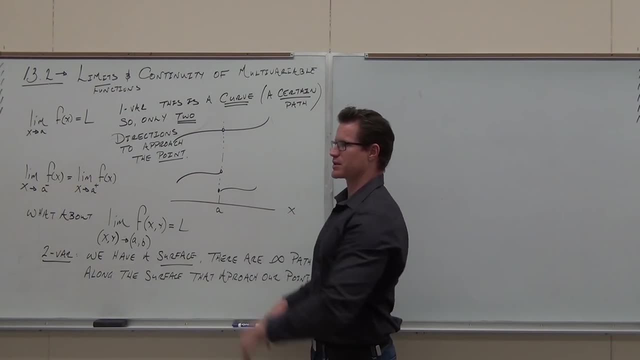 Not really. Here's why It's a lot easier to do two things. One, it's a lot easier to prove limits don't exist. It's really easy: Left side doesn't meet right side, Or one path doesn't meet the other path. 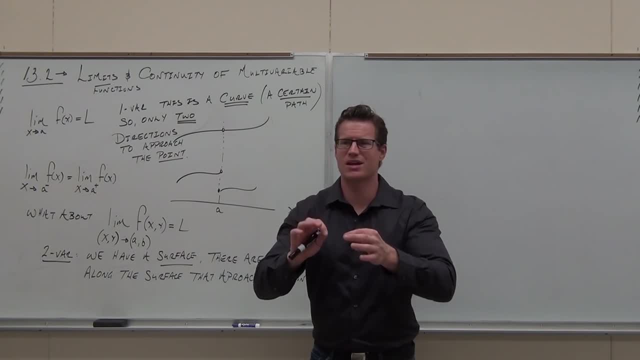 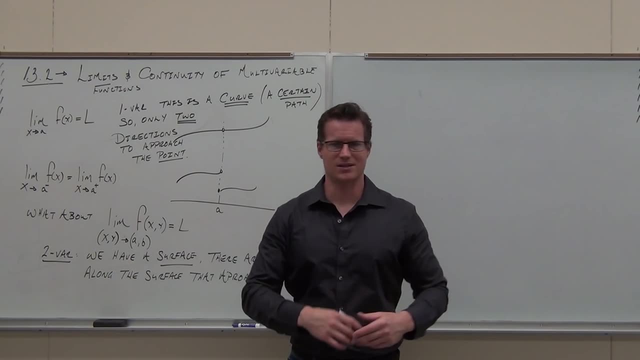 It only takes one example And you can prove. a limit doesn't exist. You guys understand the idea. To prove something is true, you got to prove it for all the cases. To prove something is not true, you just got to unprove it for one case. 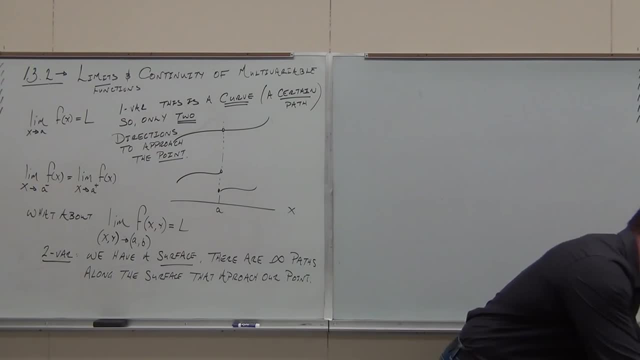 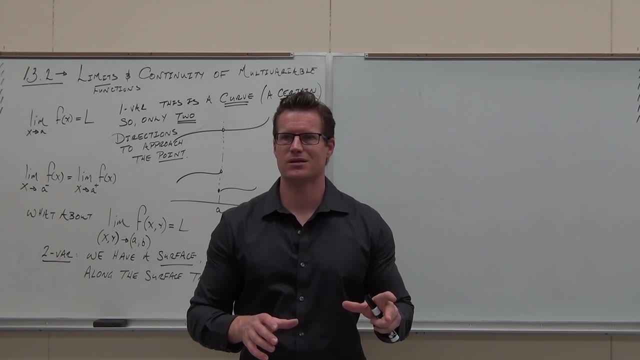 Well, it's really hard to do. You should read that: impossible in most cases to do. We can do it with something called the squeeze theorem, Calc 1 concept. We're going to use it again. We'll do it later. It's hard. 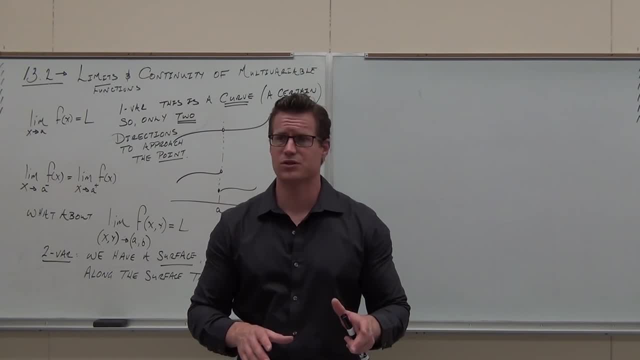 It's not that easy to do. I'll show you how you can prove that limits exist with the squeeze theorem. Do we generally do that? Not really. Here's why It's a lot easier to do two things. One: it's a lot easier to prove limits don't exist. 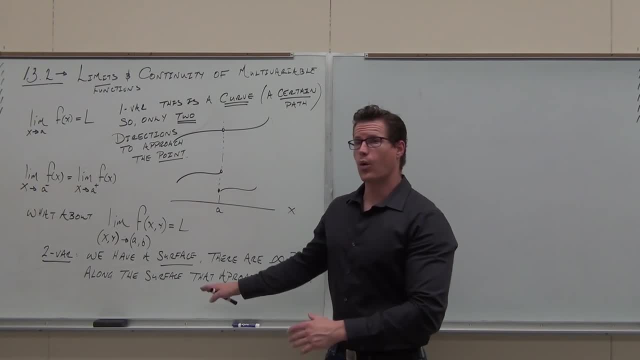 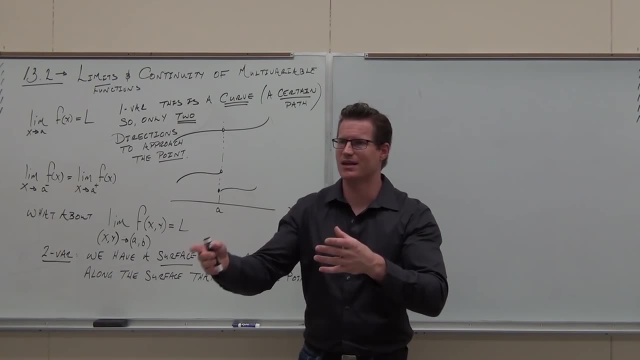 It's really easy: Left side doesn't meet right side, Or one path doesn't meet the other path. It only takes one example And you can prove a limit doesn't exist. You guys understand the idea. To prove something is true, you got to prove it for all the cases. 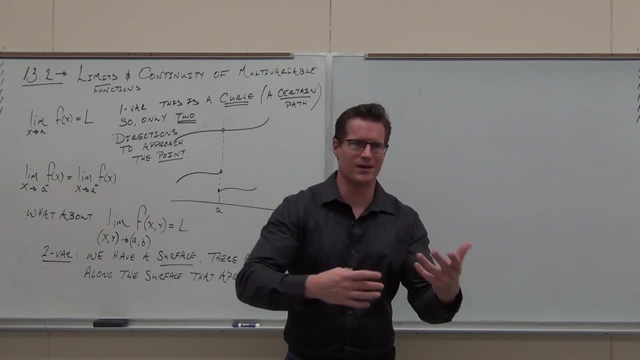 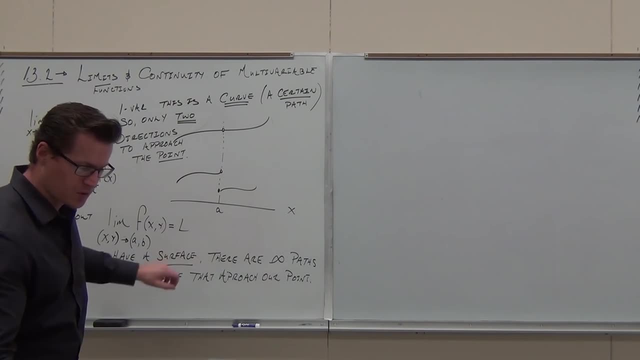 To prove something is not true, you just got to unprove it for one case Done. So a couple things about this And we're going to get through it here in a second. So to prove that this exists, you have to prove that along all the paths. 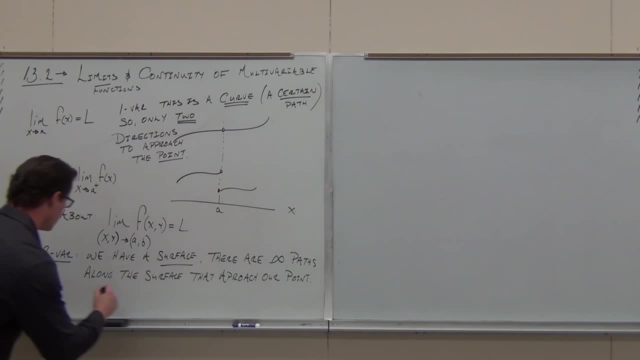 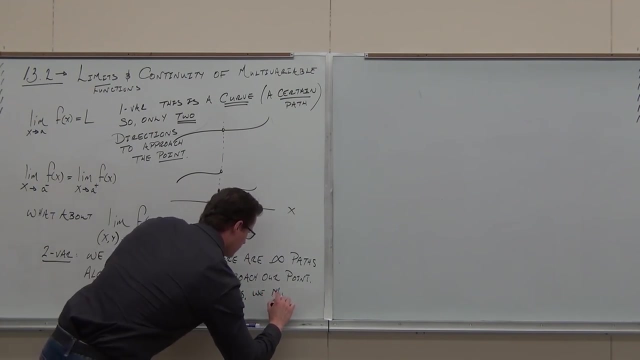 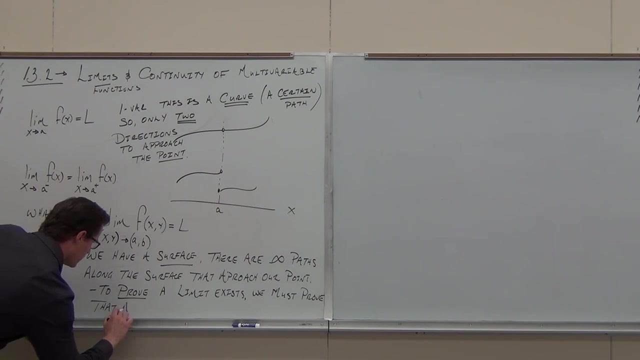 we approach the same height. as we approach that point All paths, All infinity of them. We get to prove that along all paths we approach the same point. We don't leave to to one right time This might be the same. we have to prove it. 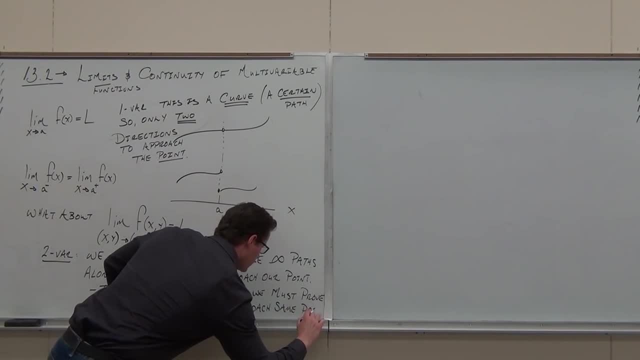 The point of proof is really simple: to trust that something exists doesn't exist. You help us think that we have to make a comparison here. You need to tell us who this is. That's what you're going to do, And you have to answer us, okay. 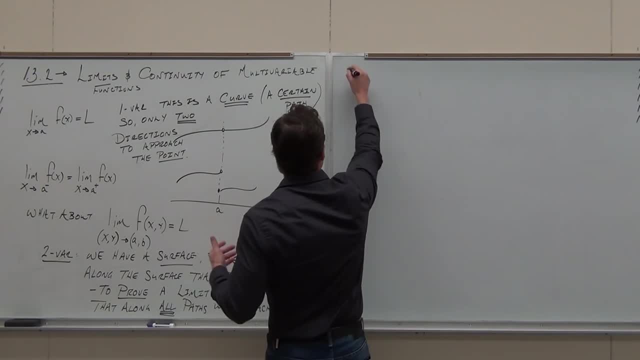 What if we broke? because something exists? What if we broke? What if we broke? What if we say: this is what we're doing with the effective video? Speak up in front of your right DOM. You don't just answer with that. Yes, everyone. 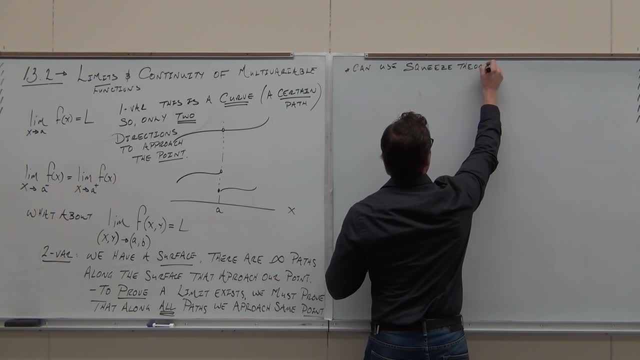 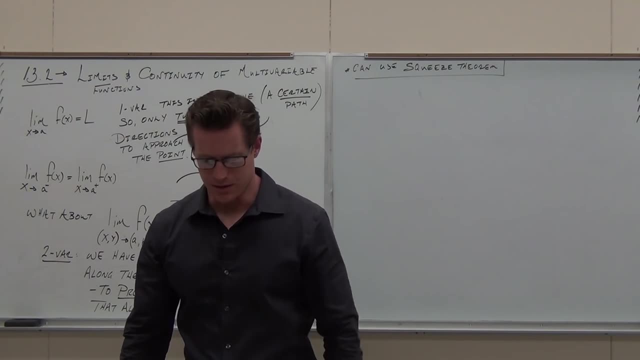 Okay, If you spoke up and said it's right, It doesn't actually mean it exists, right. But then you say: where are you coming from? It means the same, but it doesn't. I'm going to come back, I'm going to prove that, but that's going to be the end. 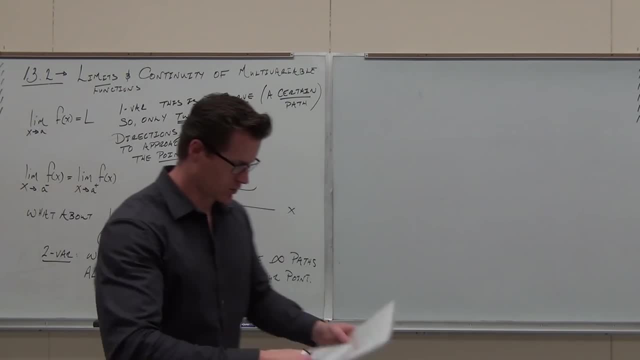 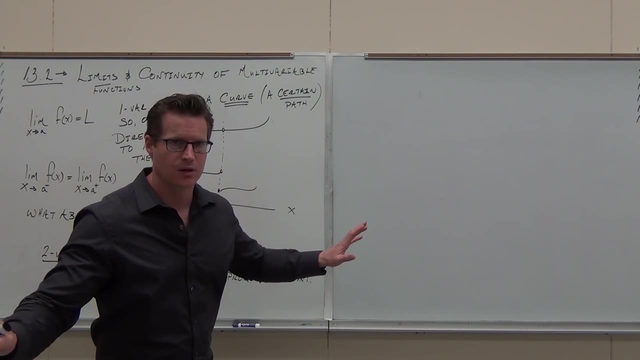 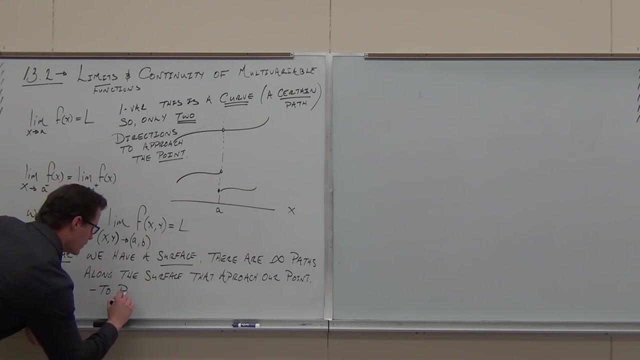 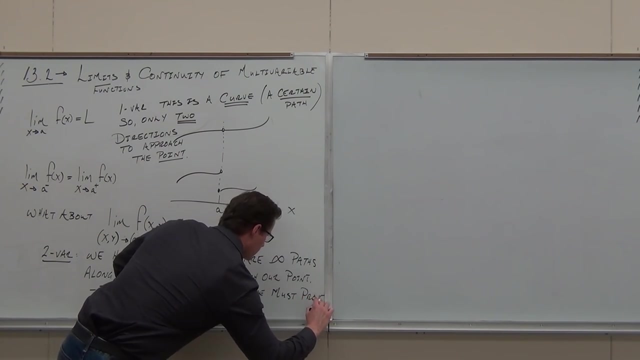 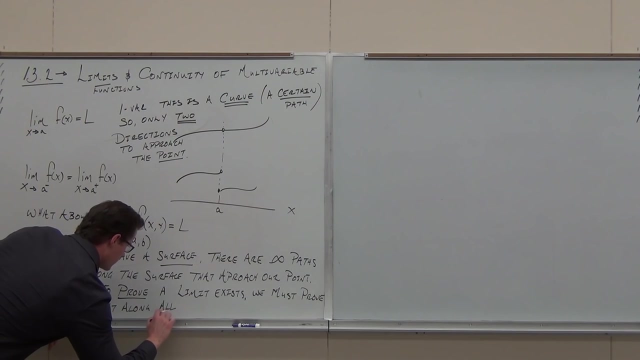 Done. So a couple things about this and we're going to get through it here in a second. So to prove that this exists, you have to prove that along all the paths we approach the same height as we approach that point. All paths, all infinity of them. we get to prove that along all paths we approach the same point. 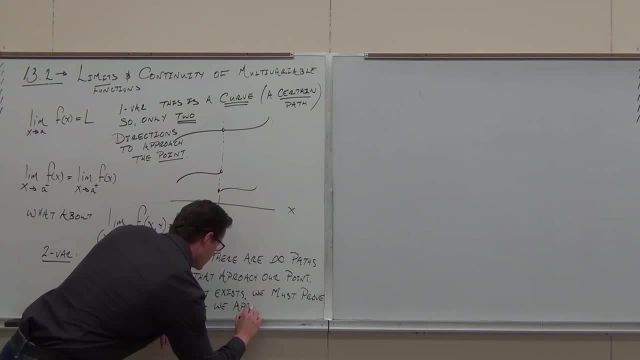 All paths, all infinity of them. we get to prove that along all paths we approach the same point. All paths, all infinity of them. we get to prove that along all paths we approach the same point. Really hard Squeeze theorem would do it. 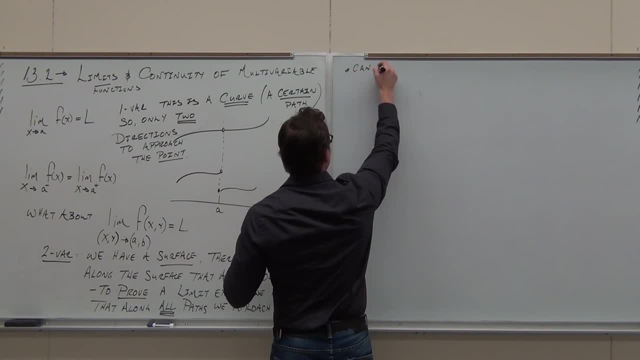 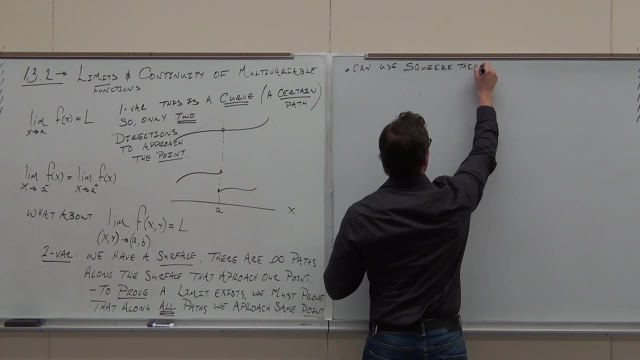 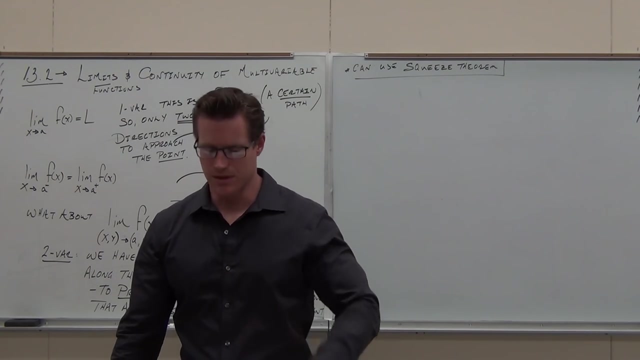 We can use squeeze theorem: I'm going to come back, I'm going to prove that, But that's going to be the end, All right. So we're going to come back, But it's not easy in general. Sometimes it's impossible. 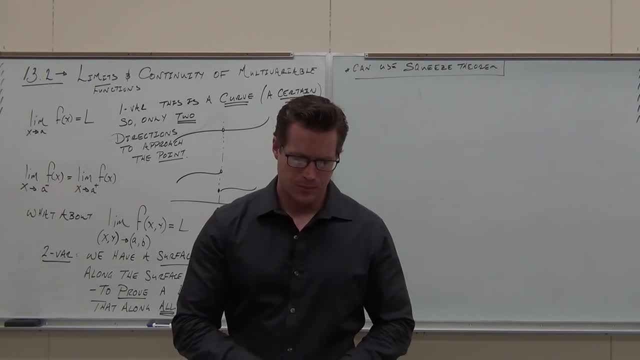 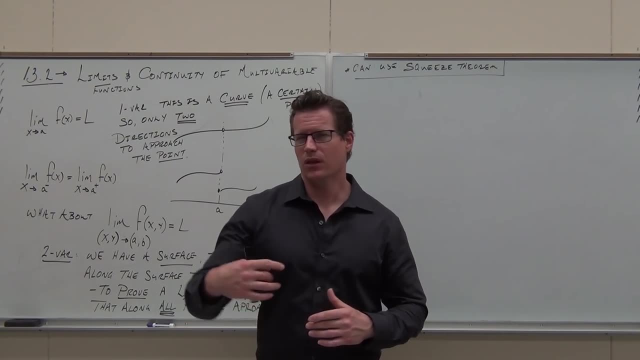 We just can't do it. So how do we prove these things exist? One of them is squeeze theorem. The other way is that we use a lot of the principles about functions that we know. For instance, we're going to talk about continuity. 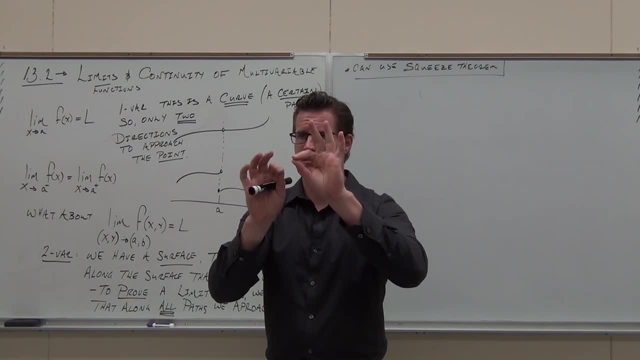 If you remember Calc 1, if you have a function that's continuous, the limit has to exist at every single point. Do you remember talking about that? Say, hey, it's continuous here. Continuous, No jumps, No gaps, No. 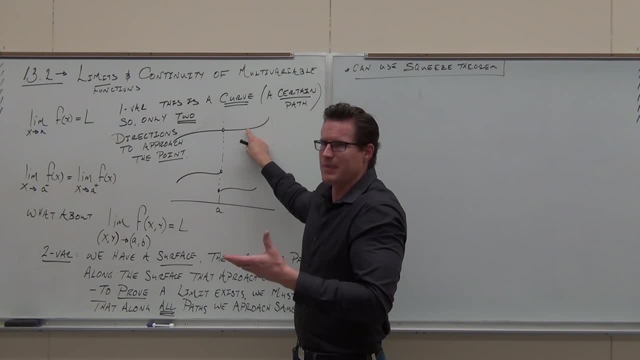 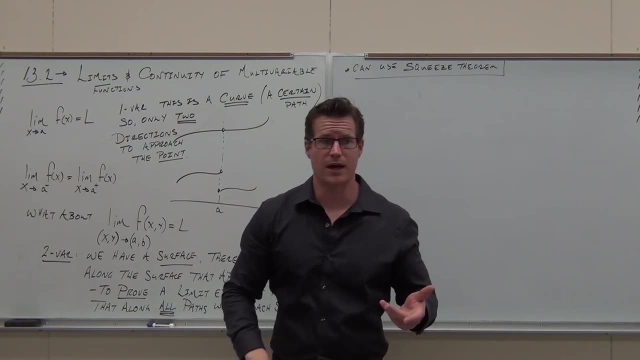 No holes, No whatevers, No, Nothing that makes it undefined. The limit's going to exist at every single one of those points And it will equal the function value of those points. We can use stuff like that. So we're going to use continuity to help us out with some of these limits. 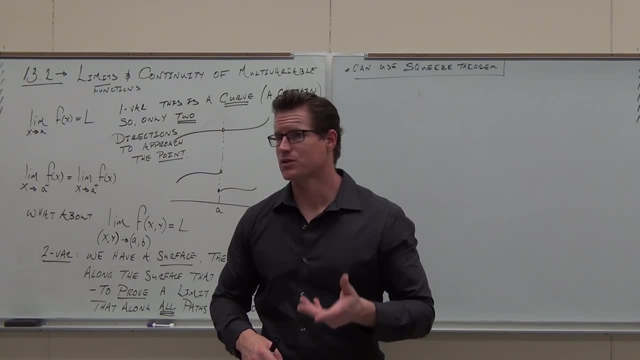 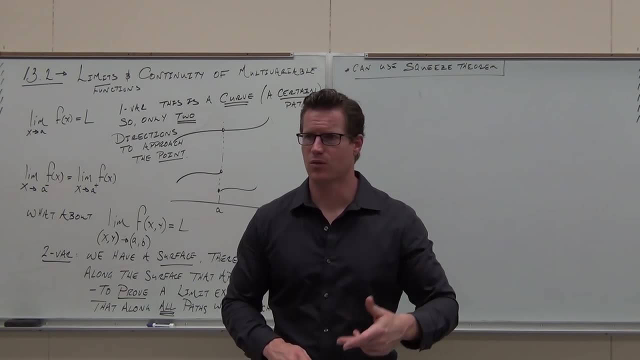 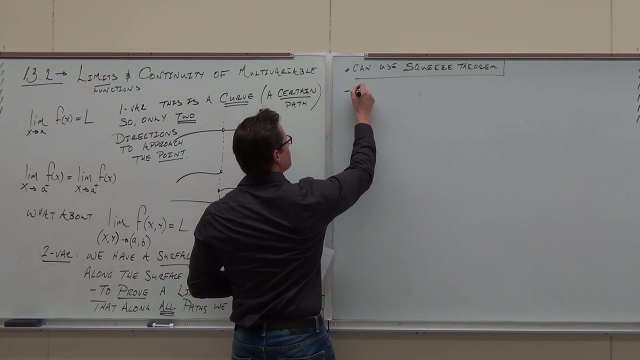 to let us evaluate them really quickly. That's pretty nice, So we can do that. So squeeze theorem is one way. Using some of the properties of limits from Calc 1 is another way. Other than that, other than that, we can easily, relatively easy, prove when a limit doesn't exist. 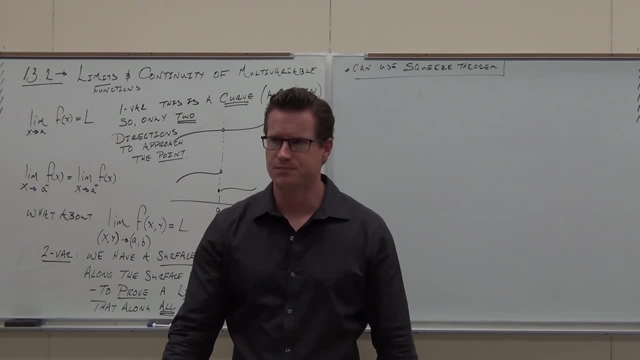 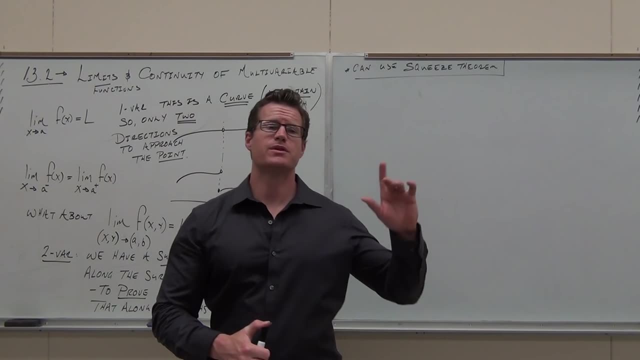 But it's not easy in general. Sometimes it's impossible, but we just can't do it. So how do we prove these things exist? One of them is squeeze theorem. The other way is that we use a lot of the principles about functions that we know. 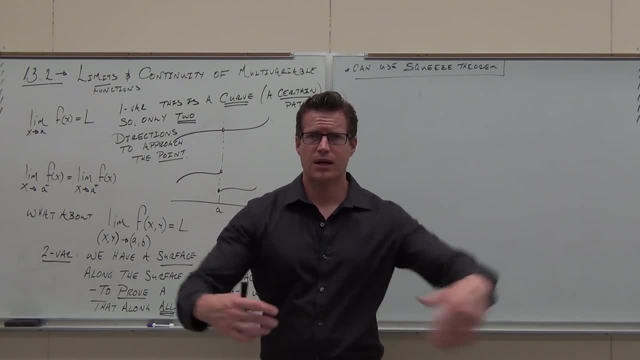 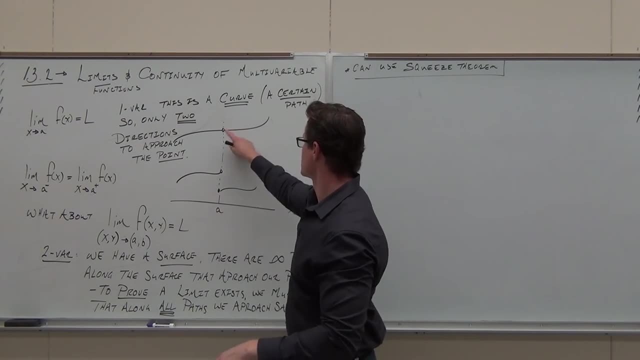 For instance, we're going to talk about continuity. If you remember Calc 1, if you have a function that's continuous, the limit has to exist at every single point. Do you remember talking about that? Say, hey, it's continuous here. 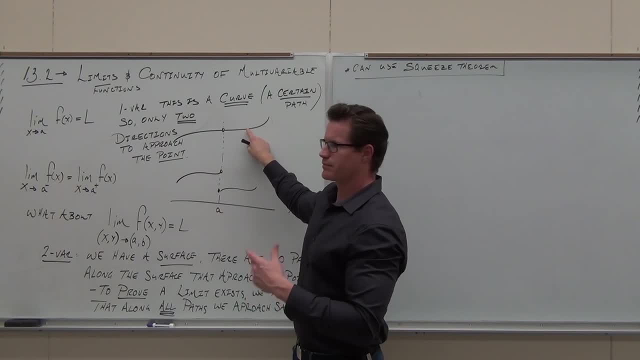 Continuous: no jumps, no gaps, no holes, no whatevers. nothing that makes it undefined. The limit's going to exist at every single one of those points and it will equal the function value at those points. We can use stuff like that. 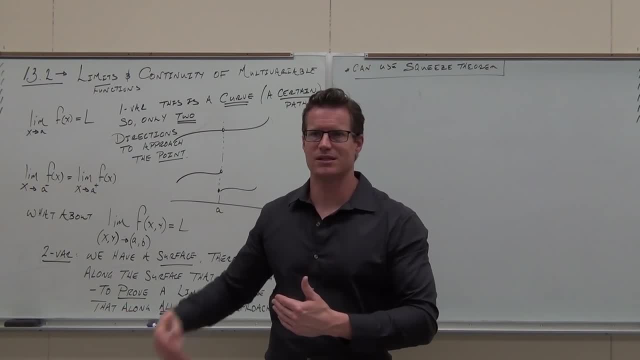 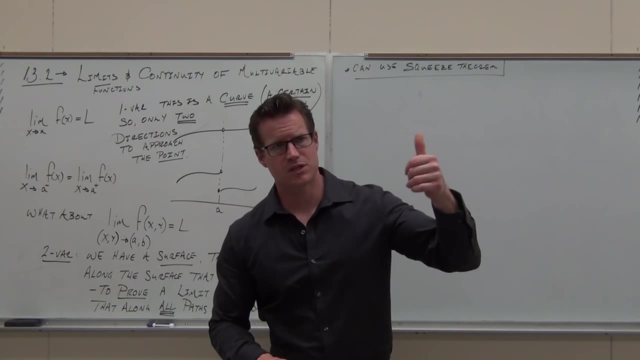 So we're going to use continuity to help us out with some of these limits, to let us evaluate them really quickly. That's pretty nice So we can do that. So squeeze theorem is one way. Using some of the properties of of limits from Calc 1 is another way. 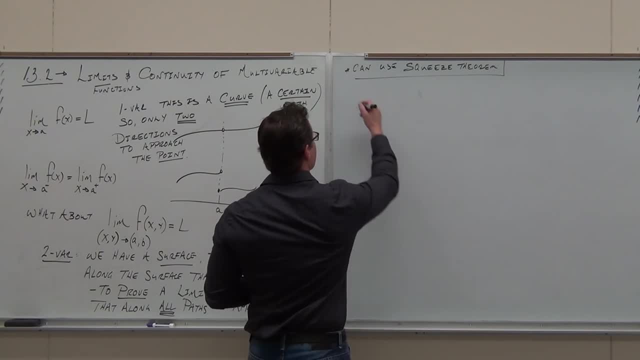 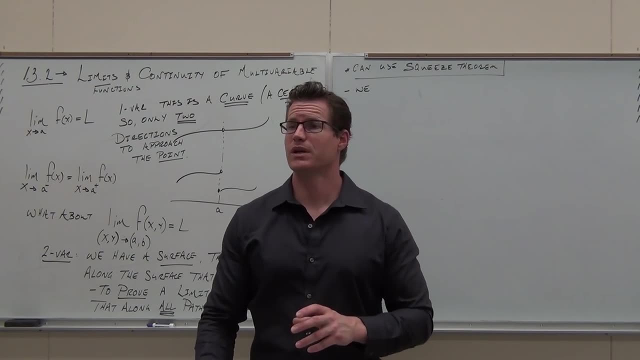 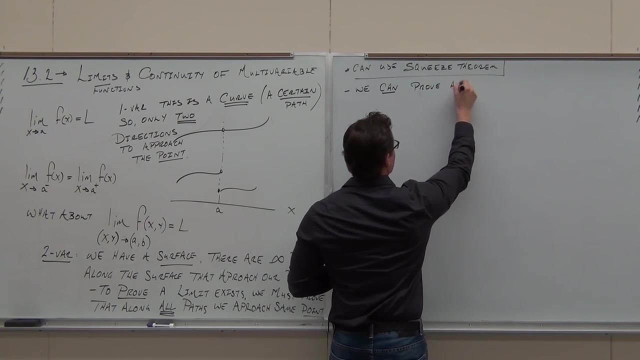 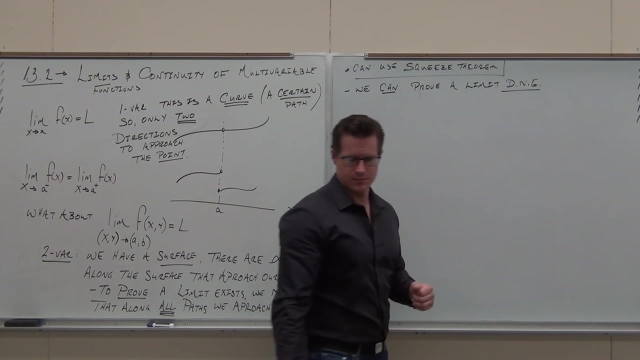 Other than that, other than that we can easily- relatively easy- prove when a limit doesn't exist. It's really akin to to what we're doing here: From one direction and from another direction along the curve, we're equaling a different value. 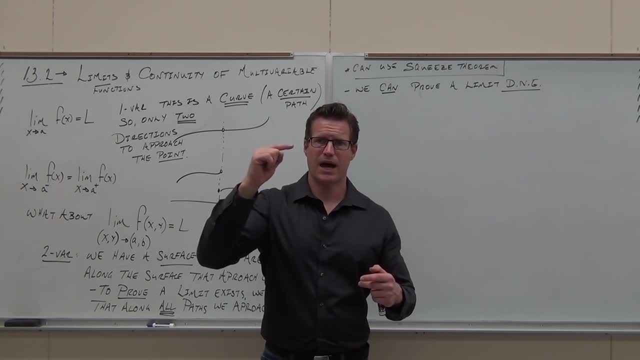 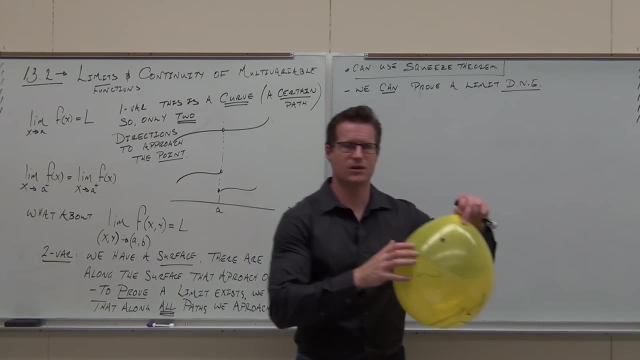 That, that that's. that's the idea. On a surface it's from one path and another path. we'd equal a different value. I can't show you with this, because this is, and we're going to show this a little bit later. 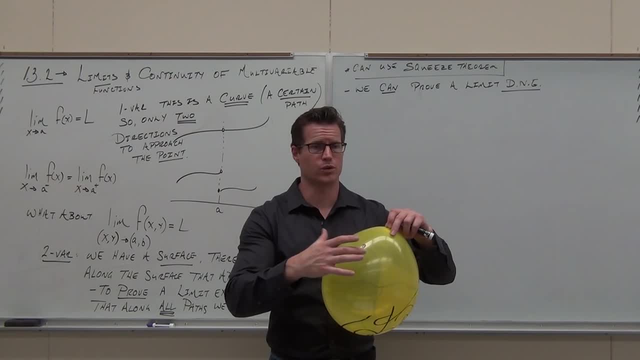 This will be continuous at any path because it's defined everywhere. There's no holes. There's no no asymptotes in 3D. Those look weird, But there's nothing like that. asymptotic planes There- there's nothing like that. 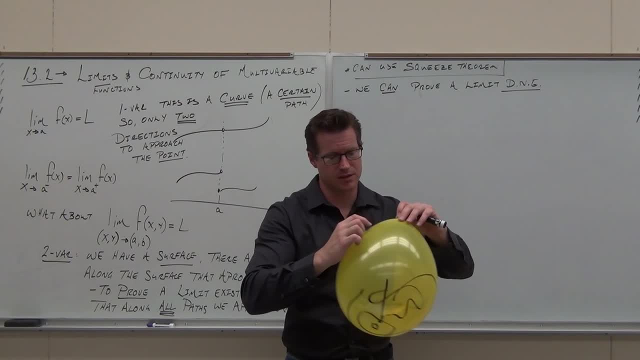 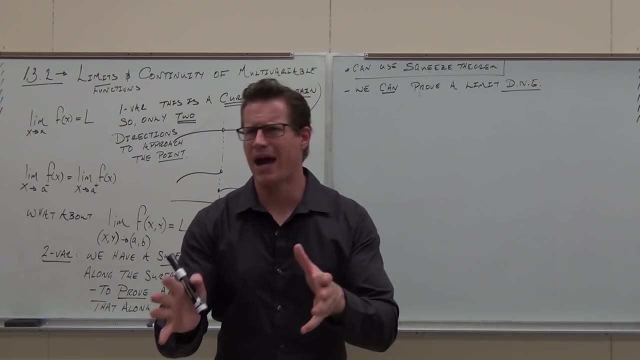 So this will be continuous everywhere, which means that all paths lead to this one point at that point. So that's okay. But in general it says this: It says: just find me two paths. that when we approach my point x, y, it gives me a different height. 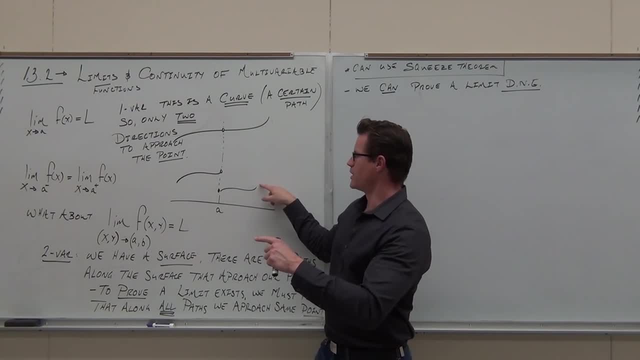 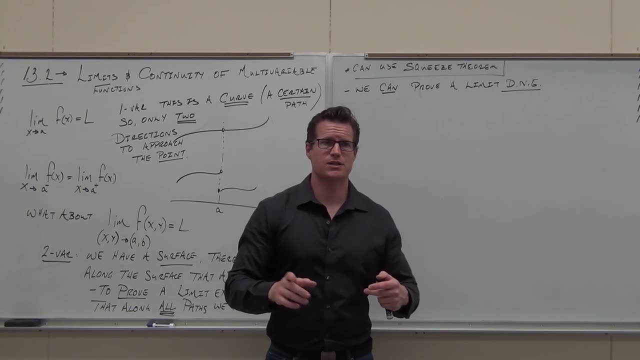 It's really akin to what we're doing here: From one direction and from another, From another direction, along the curve, we're equaling a different value. That's the idea On a surface. it's from one path and another path, we'd equal a different value. 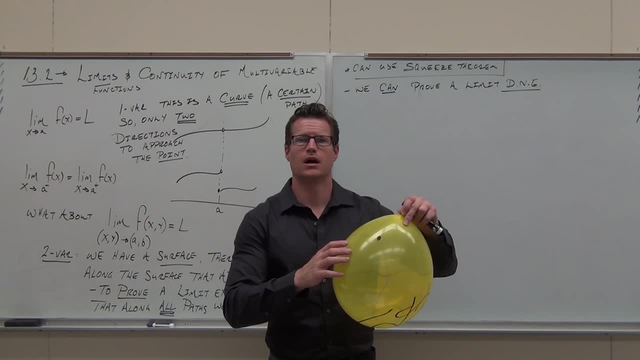 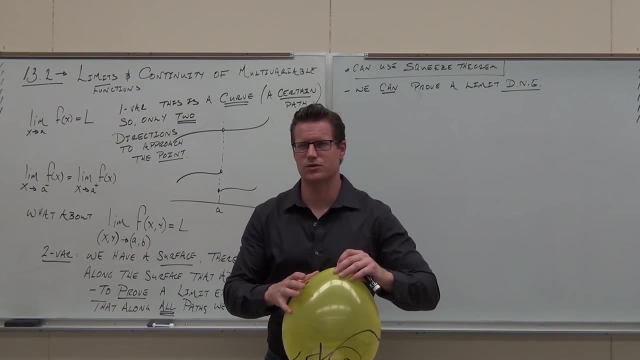 I can't show you with this, because this is going to- and we're going to show this a little bit later. This will be continuous at any path, because it's defined everywhere. There's no holes, There's no asymptotes in 3D. 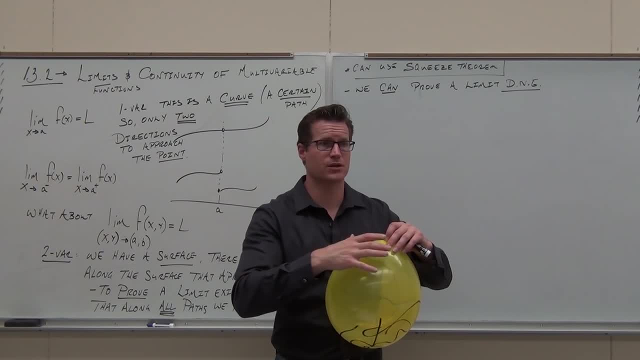 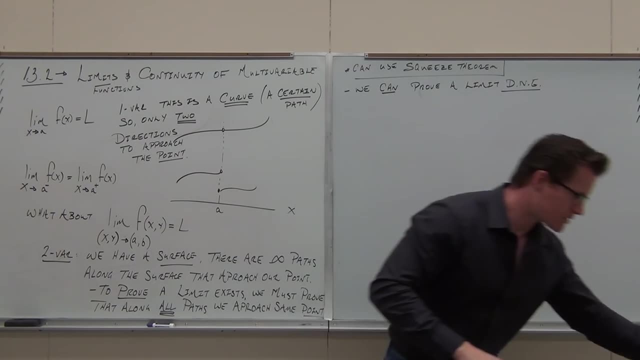 Those look weird, But there's nothing like that. Asymptotic planes: There's nothing like that. So this will be continuous everywhere, which means that all paths lead to this. that one point at that point. So that's okay. 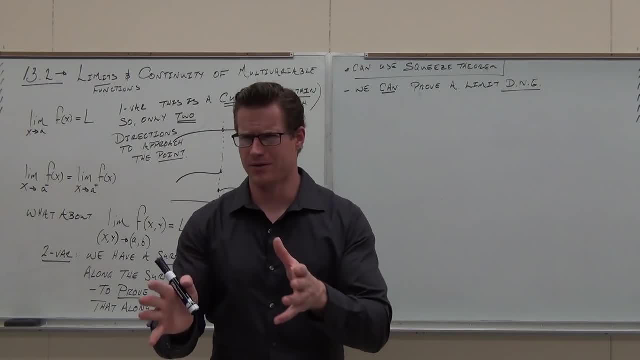 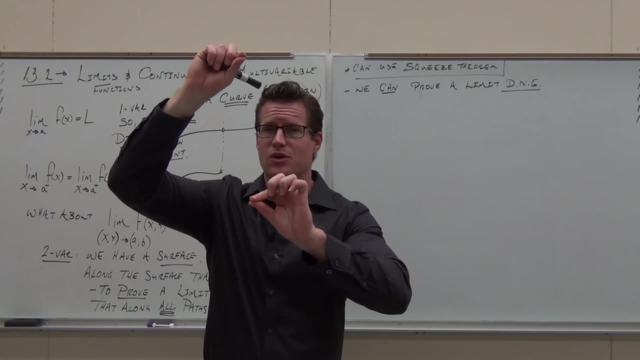 But in general it says this. It says: just find me two paths that when we approach my point x, y, it gives me a different height. I'm going to say that one more time so it sinks in, because some of you guys are zoning out already. 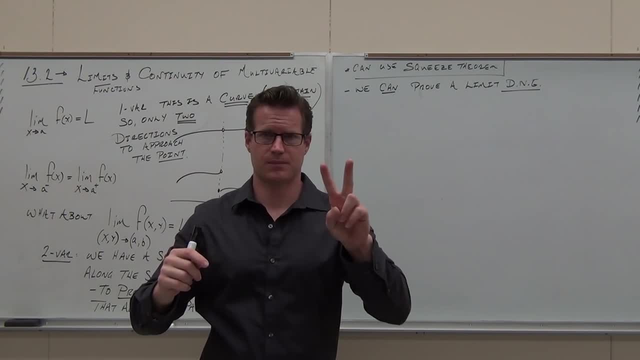 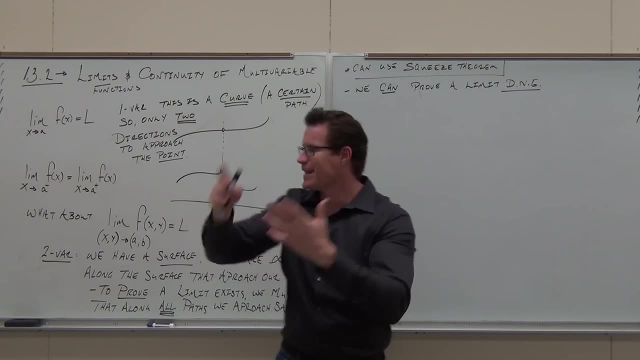 All right, I'm going to say this: Find me two paths that when I get to my x, y, when I get to this, it gives me out two different heights. That is what this situation would be in 3D. You go, hey, along one path. I'm up here. 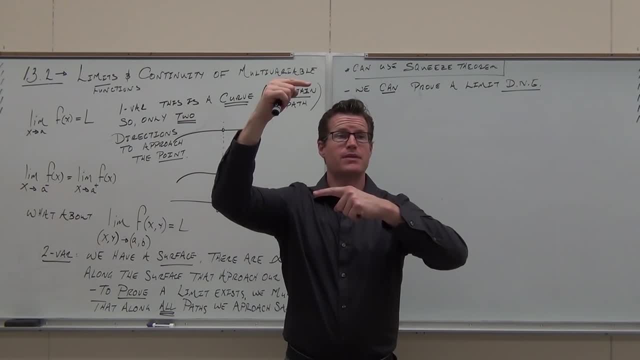 Along another path. I'm up here. Along another path, same surface. I'm down here. Okay, That right there tells you you're not continuous at that point and therefore the limit does not exist at that point. That's what we're doing. 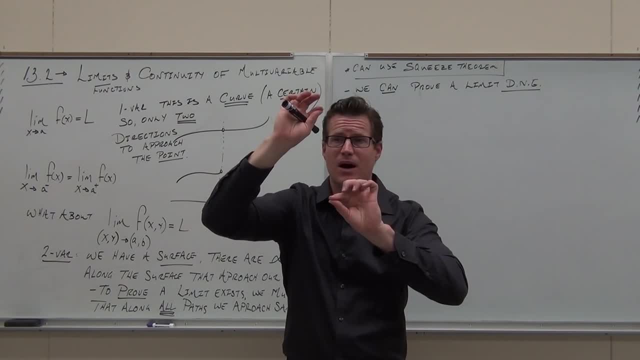 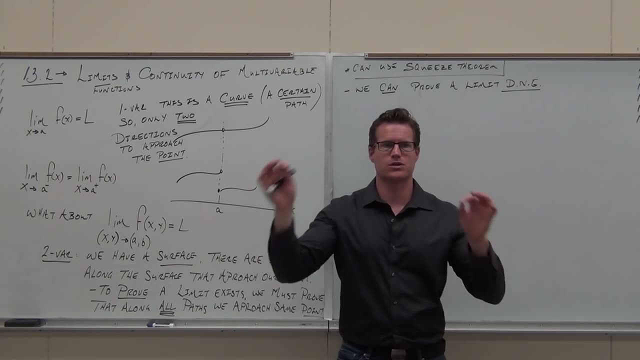 And it only takes two paths. because if we can show two paths don't equal the same height, that right there is enough to say the limit doesn't exist. Why? Because for the limit to exist, we have to show that every single path goes to the same value. 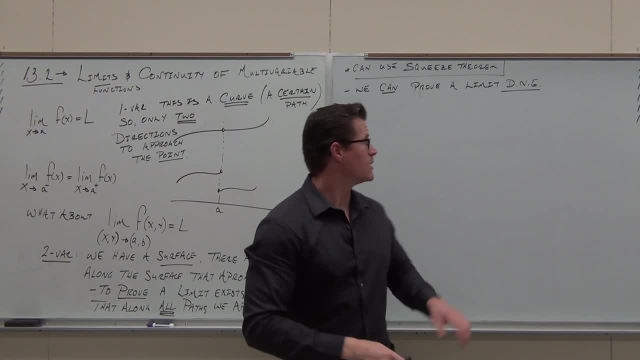 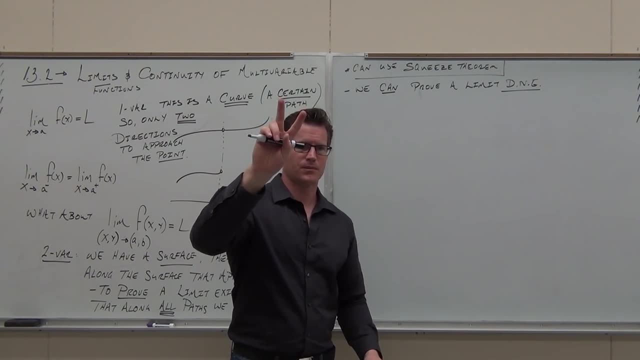 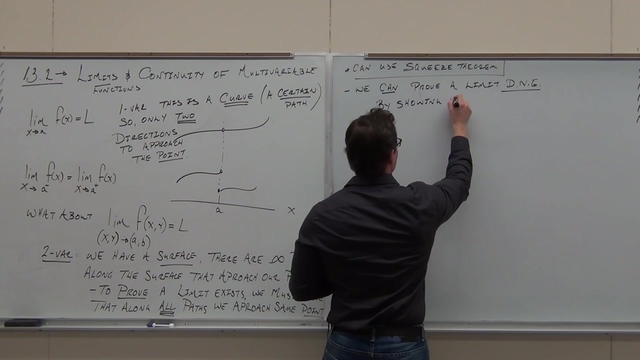 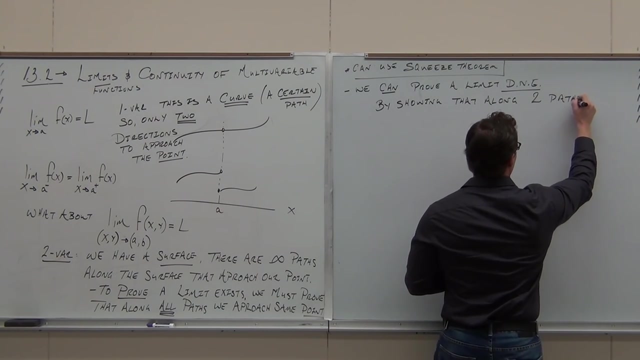 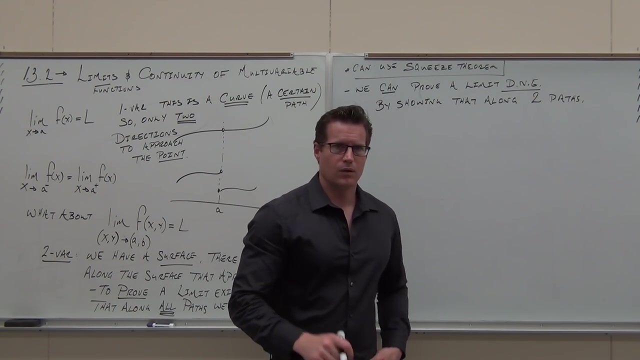 If we prove that two don't, we've proven that wrong. That's the point. So we can easily prove a limit does not exist by showing that along two paths- Along two paths, We get a different value as we approach the same point. 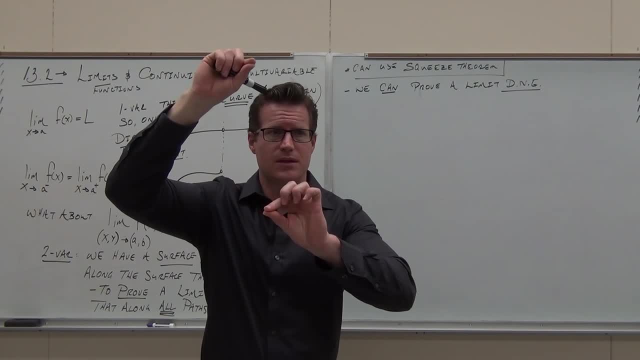 I'm going to say that one more time so it sinks in, because some of you guys are zoning out already. all right, I'm going to say this: Find me two paths that, when I get to my x, y, when I get to this, 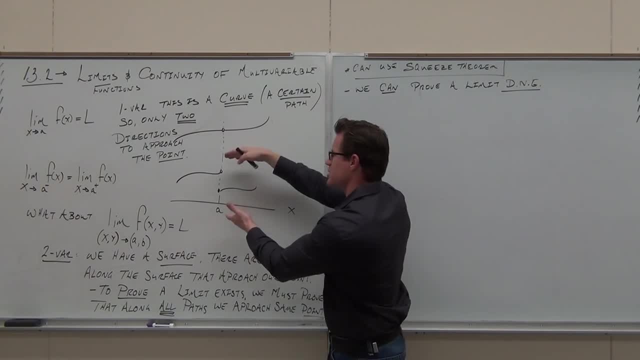 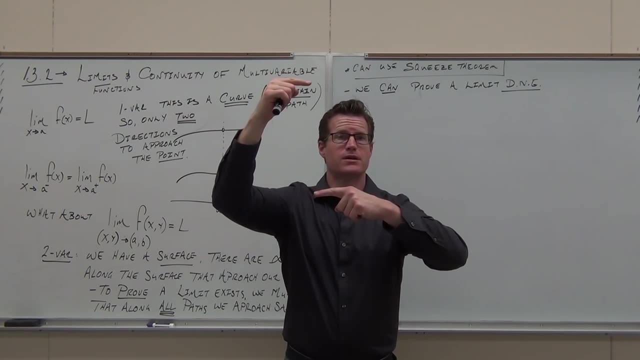 it gives me out two different heights. That is what this situation would be in 3D. You go, hey, along one path, I'm up here. Along another path, same surface, I'm down here. Okay, That right there tells you you're not continuous at that point. 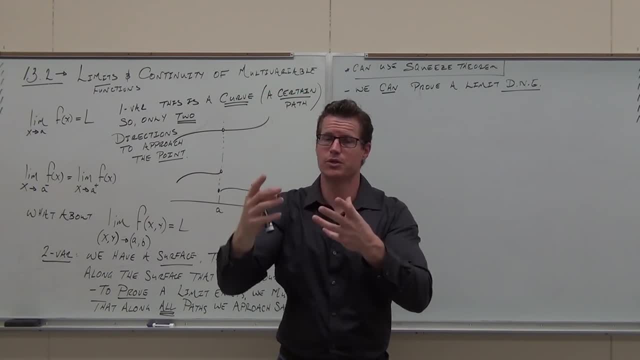 and therefore the limit does not exist. at that point. That's what we're doing, And it only takes two paths, because if we can show two paths don't equal the same height, that right there is enough to say the limit doesn't exist. Why? Because for the limit to exist, we have to show that every single path goes to the same value. If we prove that two don't, We've proved that two don't, We've proven that wrong. That's the point. So we can easily prove a limit does not exist by showing that along two paths. 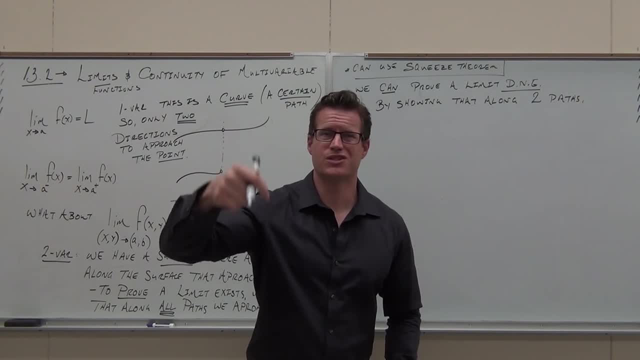 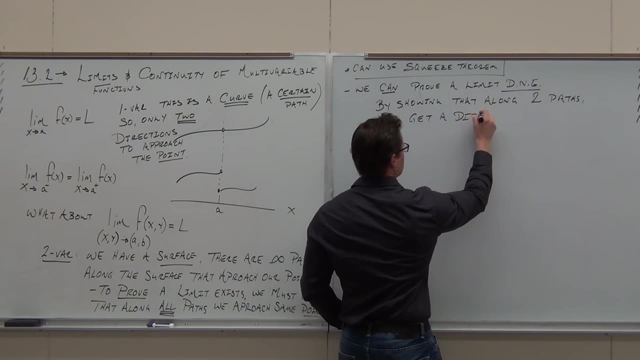 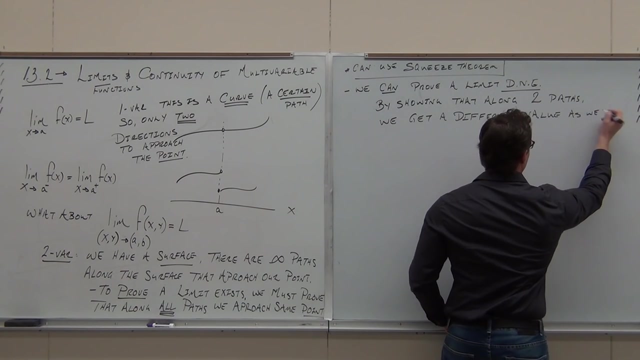 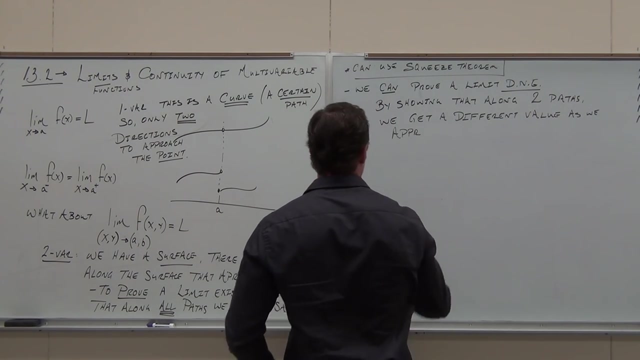 We get a different value as we approach the same point. Did you spell approach wrong like 14 different times I did. Sorry, I don't even know which one it is anymore. Yeah, Did you ever do that Like? you know it's one way, but then you write it two different ways. 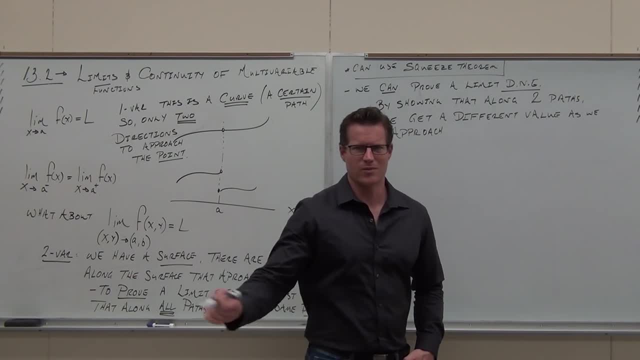 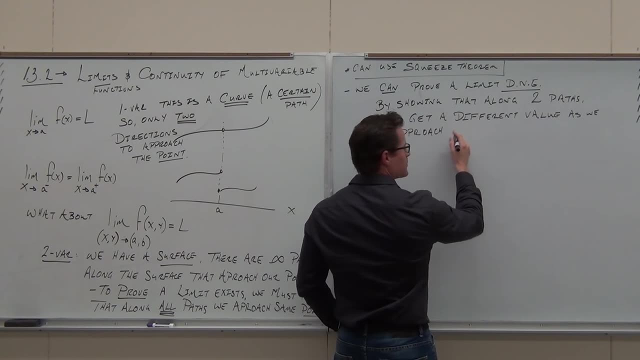 and you can't tell anymore. I'm pretty sure these two are wrong down there. Don't ignore those, Just white them out on the, on the whatever Draw it in there. Typical math teacher, right Typical. This shouldn't even let me write words. 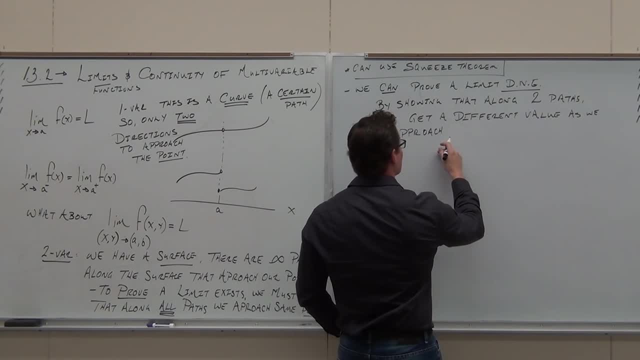 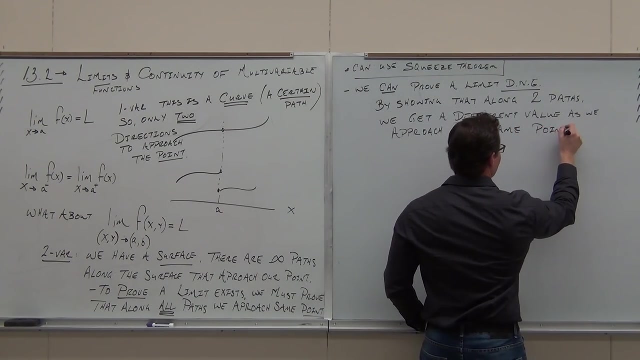 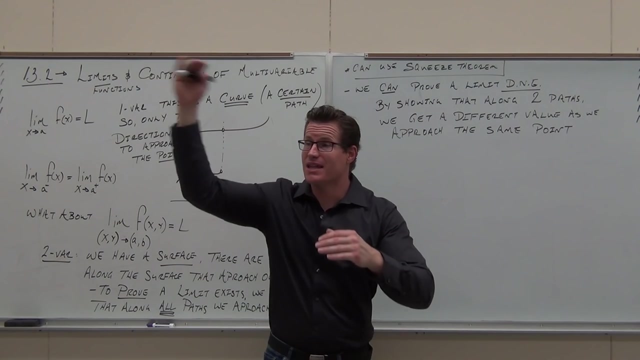 I don't ignore math anymore. What was that Approach? Approach, Thanks, That was really helpful for us. One, two, we're good. Okay, We're good. We get a different value. The different value is the height of your function. 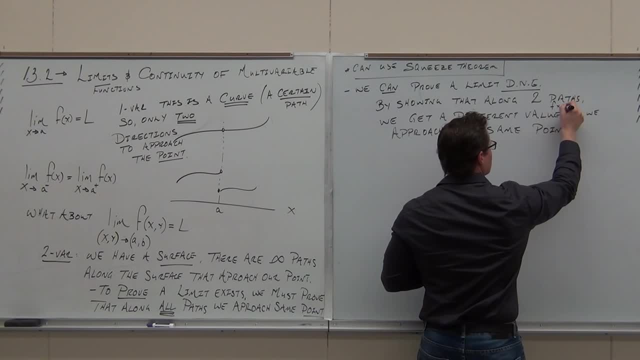 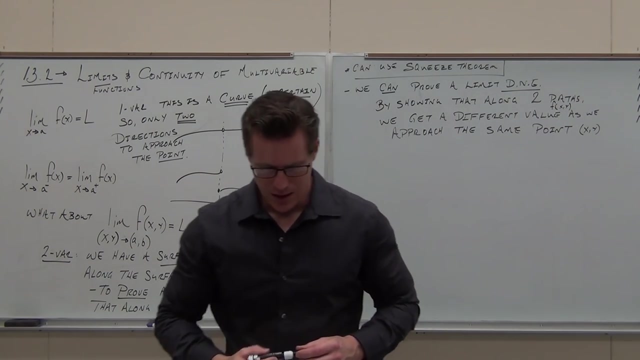 It's on the surface, F of XY as we approach the same point. XY, That's a horrible XY. I really don't feel like explaining this anymore. I have to explain it a little, if you guys understand the main concepts. One variable, easy, don't exist, done. 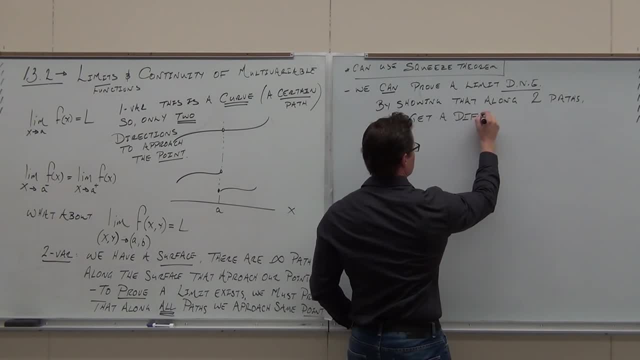 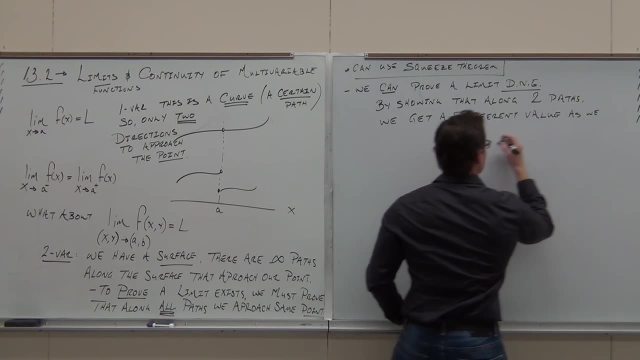 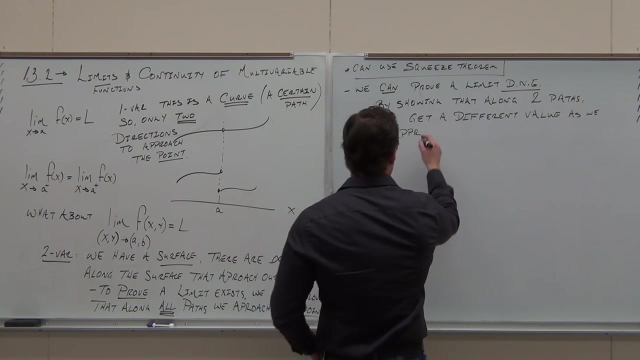 Any questions? Are you supposed to approach wrong like 14 different times? I did Sorry, I don't even know which one it is anymore. Do you ever do that Like you know it's one way, but then you write it two different ways. 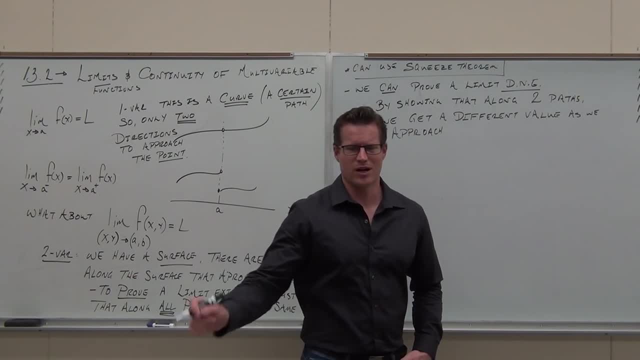 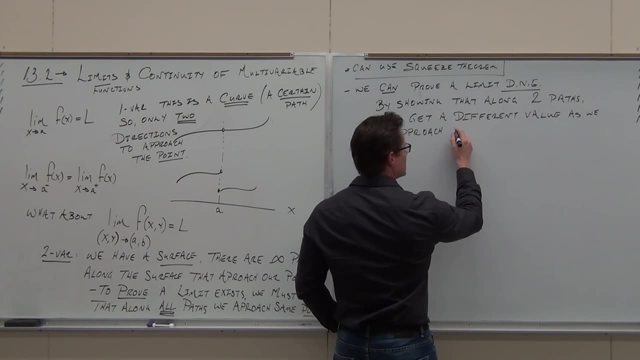 and you can't tell anymore. I'm pretty sure these two are wrong down there. Don't ignore those. Just white them out on the table on the whatever. draw it in there. Typical math teacher, right Typical. They shouldn't even let me write words. 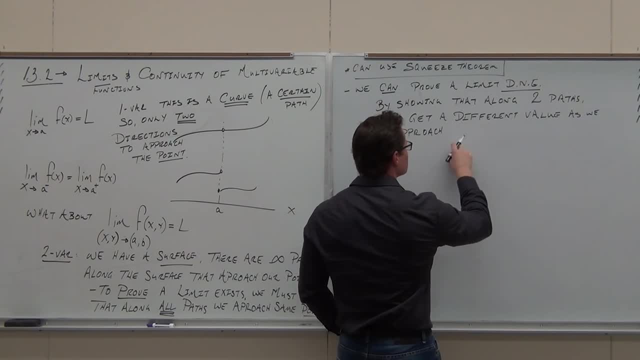 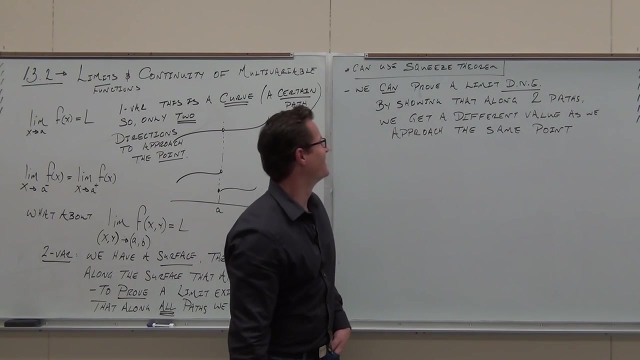 I don't even know how to math anymore. What was that? Approach, Approach. thanks, That was really helpful for us. One, two, we're good. okay, We get a different value. The different value is the height of your function. 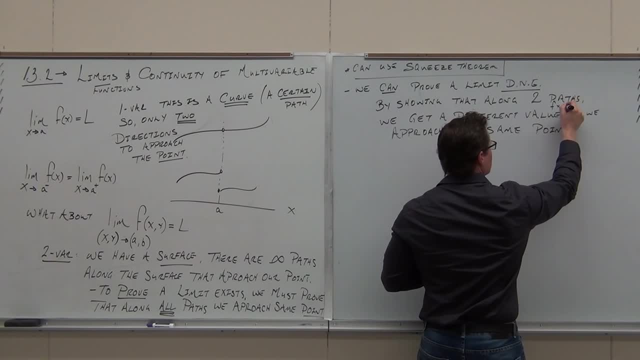 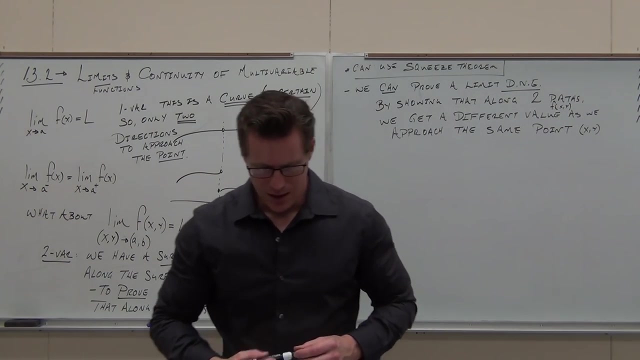 It's on the surface F of xy as we approach the same point. xy, That's a horrible xy. I really don't feel like explaining this anymore. Have they explained it? I don't know if you guys understand the main concepts. 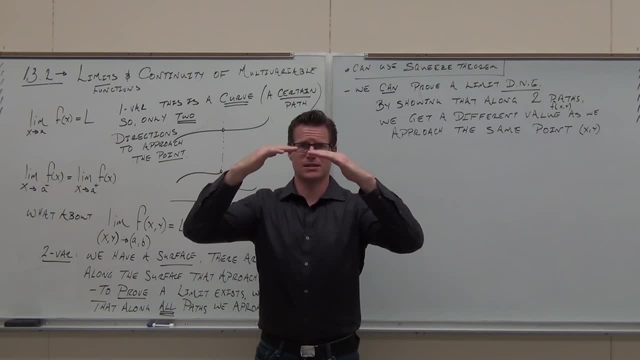 One variable Easy, don't exist. done One variable easy exist For two variables- not easy. You have to prove every path has the same value. Not easy to do. To prove it doesn't exist, it is easy. 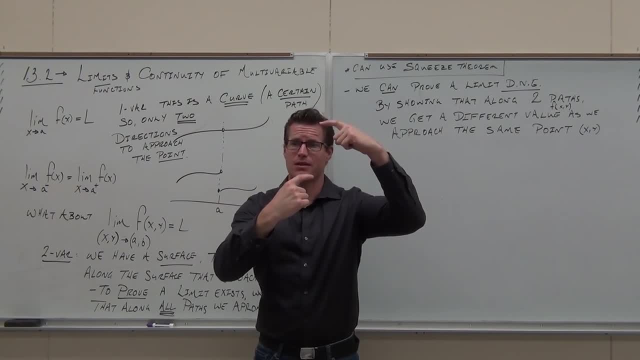 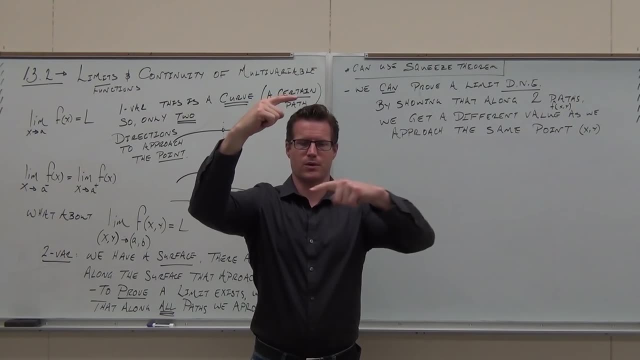 Just prove at least two. At least two paths have different heights when we are getting to the same x value. So here, xy, what's going on? From one way we're up here, From another way, we're down here. 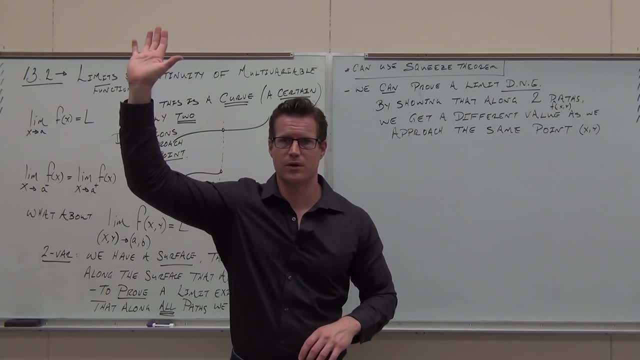 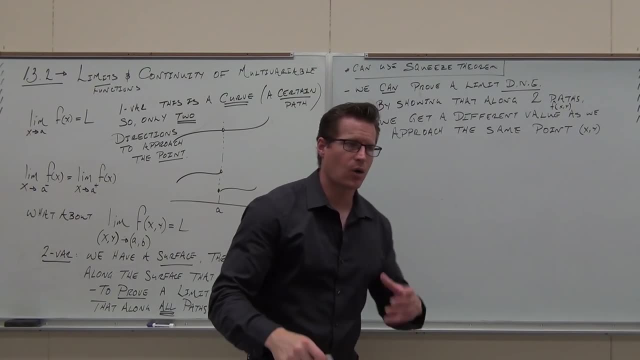 Those are different heights. Limit does not exist because we failed that Show of hands. if you're okay with that one, Let's do a quick example. Some of these are very easy, very easy to do. I'm going to show you exactly how you go about telling. 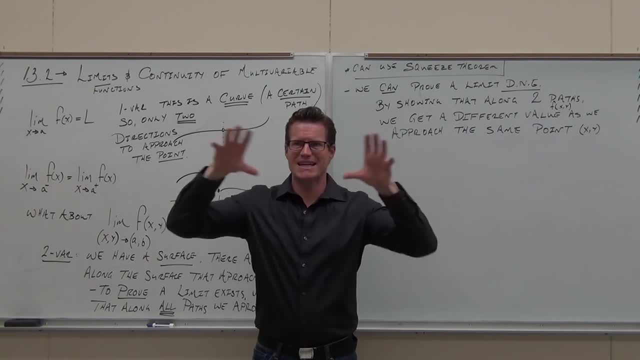 One variable- easy. exist For two variables? not easy. You have to prove every. every path goes the same, has the same value. Not easy to do. To prove it doesn't exist, it is easy, Just prove. prove at least two. 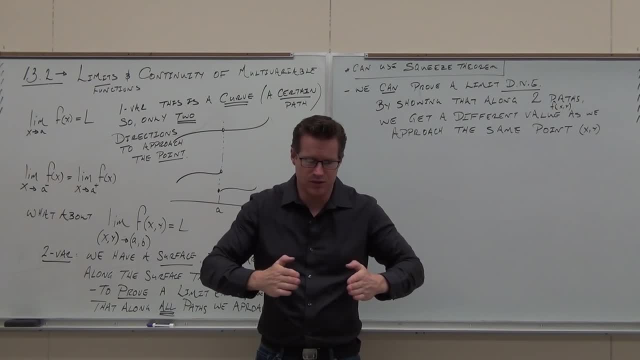 At least two paths have different heights when we are getting to the same X value. So here, XY, what's going on? From one way, we are up here, From the other way, we are down here. Those are different heights. 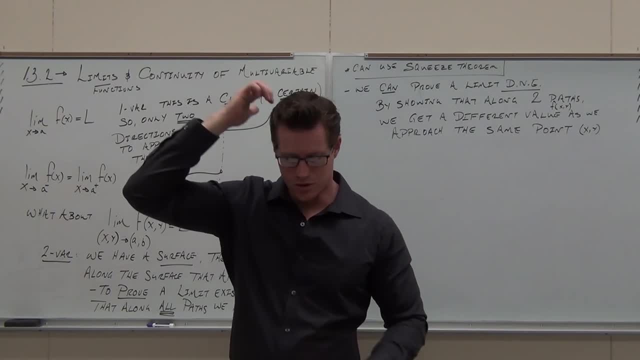 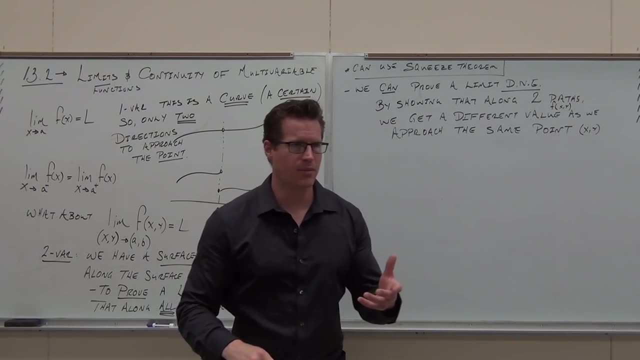 Limit does not exist because we failed that Show. fans feel okay with that one. Let's do a quick example. Some of these are very easy, very easy to do. I'm going to show you exactly how you go about telling what you should do and when you should do it. 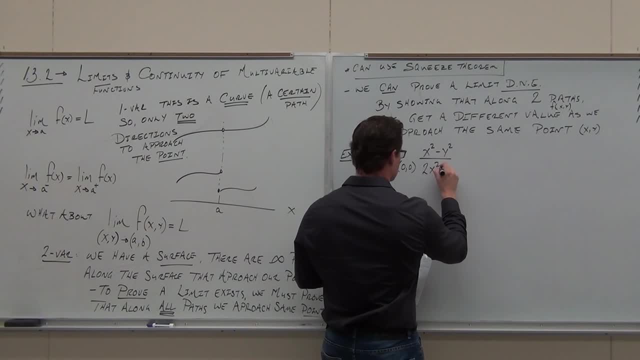 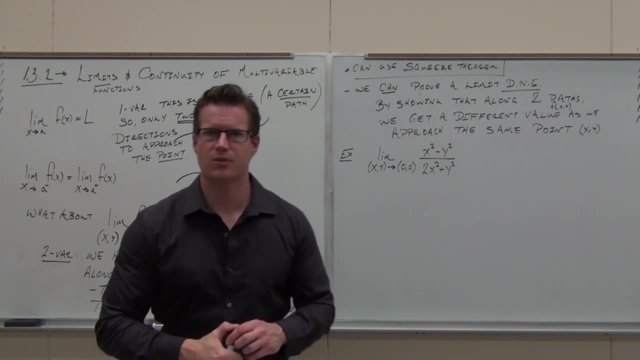 So you know. just to kind of recap a couple things, ladies and gentlemen, how many independent variables do you see right now? Very good, Everybody come on. How many independent variables? What would this graph look like? 2D, 3D, 4D. 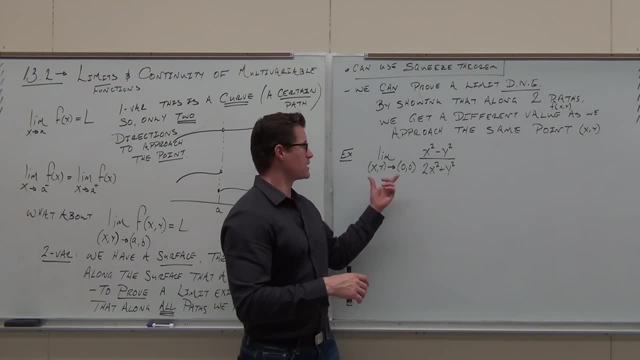 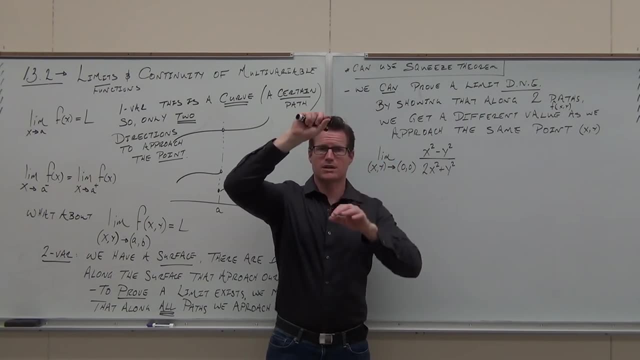 This is a surface in 3D. What I'm asking you is: does the limit exist on this function? So is the height of this function, so the surface continuous at that point? Do we have Continuity? Do we have the limit existing from every path can go to the same place? 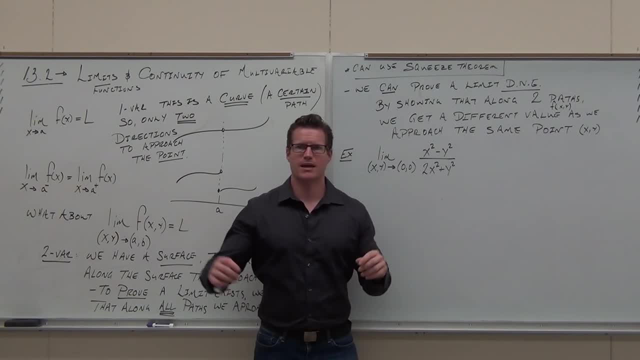 I don't know What I'm saying is. at this particular point, as X and Y, the point approaches 0, 0.. From what direction It's on a plane, ladies and gentlemen, There are no directions. Any direction you could get to 0, 0 on the plane. 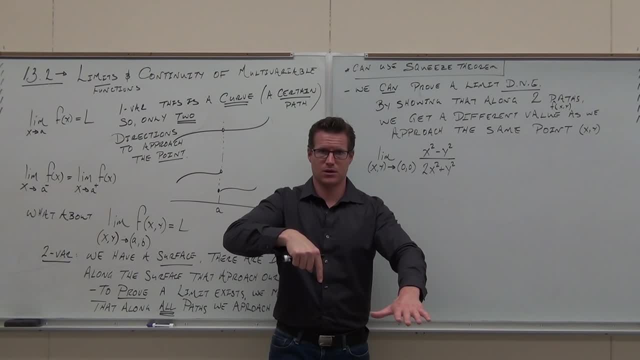 You can think about it that way too. Here's a plane, Here's 0, 0, the origin On the plane. how could you get there? Infinite number of ways. There's not just one axis, There's not just one direction. 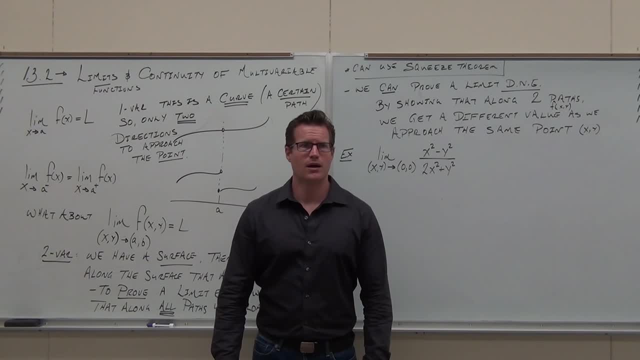 Make sense. Also, I don't like that band one direction, But anyway It's the wrong direction. So can we prove it exists? Listen, I'm going to cheat. I'm going to tell you some backwards things that we're going to get later, but you use them now. 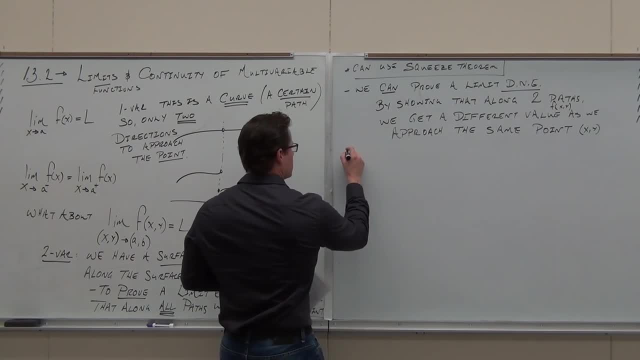 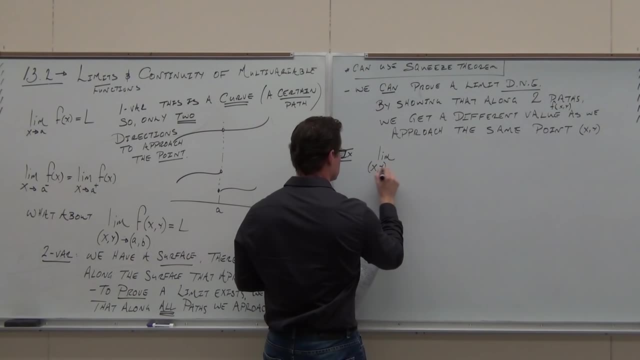 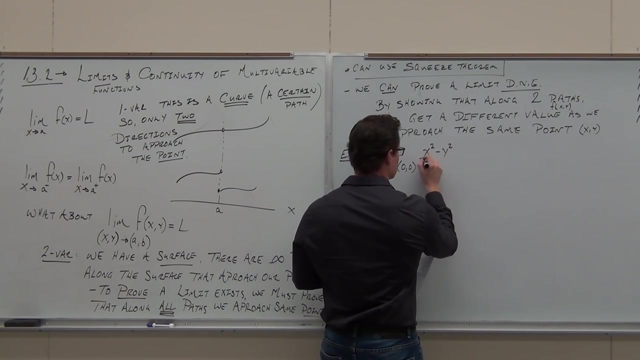 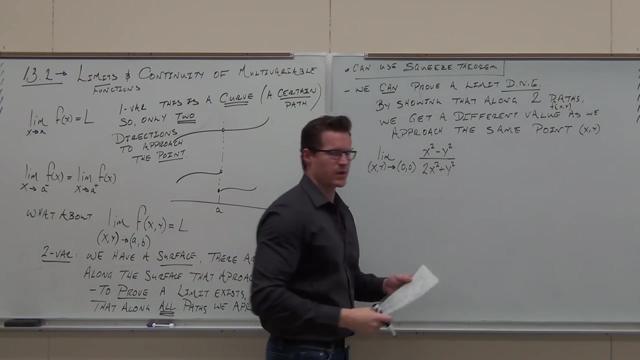 what you should do and when you should do it. You know. just to kind of recap a couple of things, ladies and gentlemen, how many independent variables do you see right now? Very good, everybody, come on. How many independent variables. 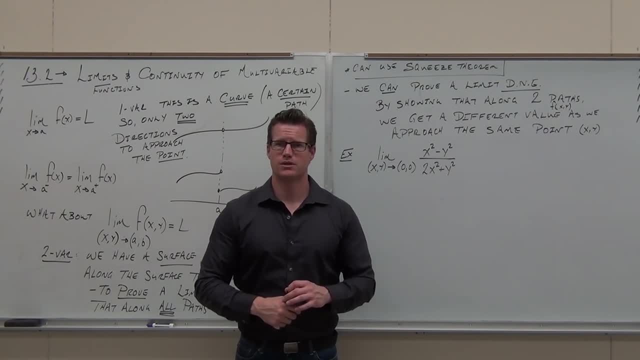 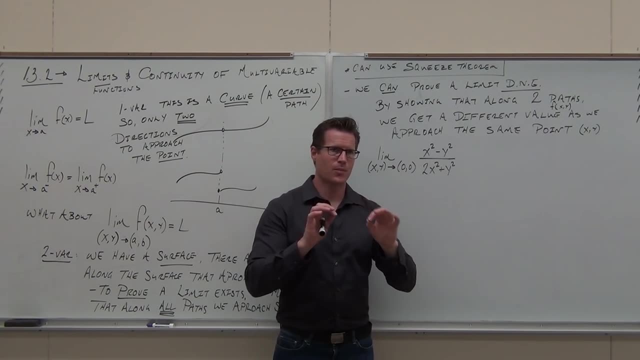 What would this graph look like? 2D, 3D, 4D, 3D. This is a surface in 3D. What I'm asking you is: does the limit exist on this function? So is the height of this function? 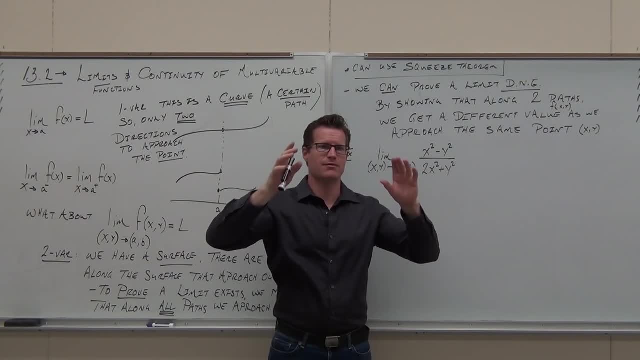 so the surface continuous at that point, Do we have continuity? Do we have the limit existing from every path can go to the same place? I don't know What I'm saying is. at this particular point, as x and y, the point approaches 0, 0. 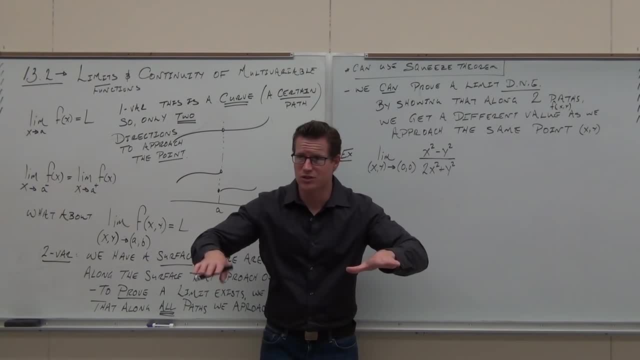 From what direction It's. on a plane, ladies and gentlemen, There are no directions. Any direction you could get to 0, 0 on the plane. You can think about it that way too. Here's a plane. Here's 0, 0, the origin. 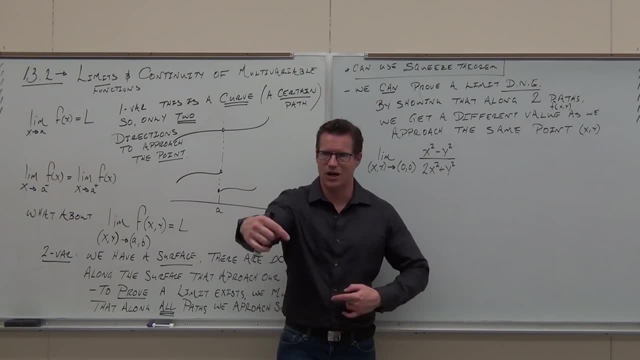 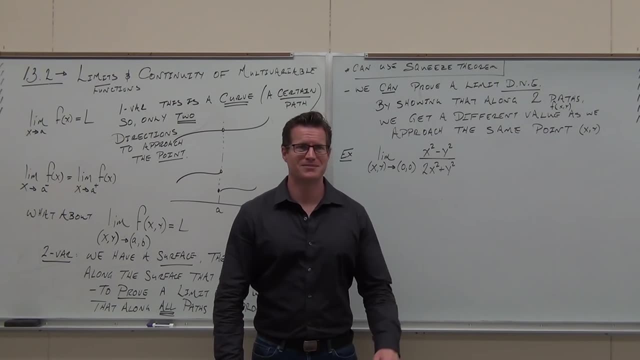 On the plane. how could you get there? Infinite number of ways. There's not just one axis, There's not just one direction. Make sense. Also, I don't like that band. one direction, But anyway it's the wrong direction. 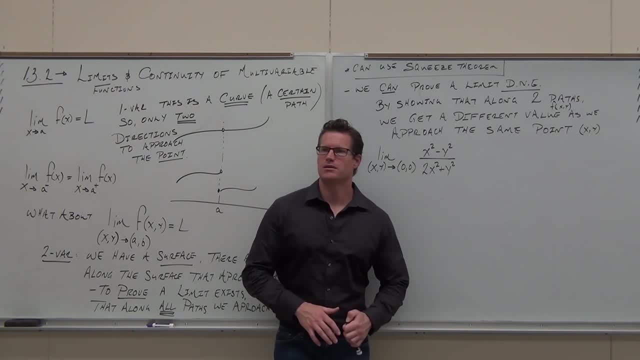 So can we prove it exists? Listen, I'm going to cheat. I'm going to tell you some bad stuff, Some backwards things that we're going to get later, but you use them now. So I'm going to teach circularly. 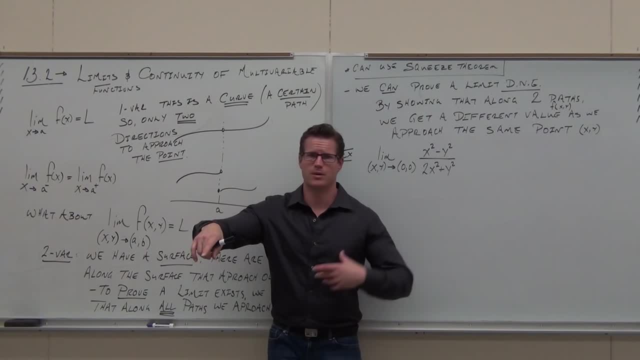 I don't care anymore. I'm going to kind of use something that I'm going to prove later And then I'm going to use that thing to prove it later. So it's going to be a little circular. Here's the deal, because I just want. 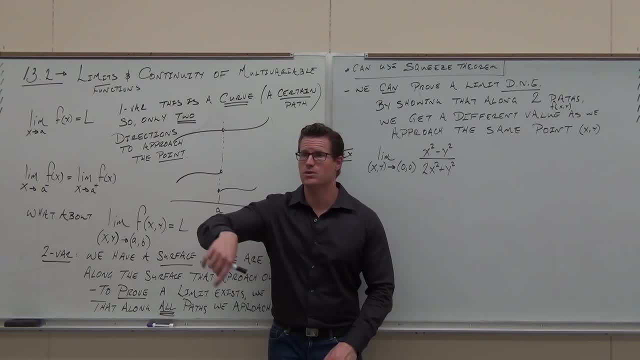 So I'm going to teach circularly. I don't care anymore. I'm going to kind of use something that I'm going to prove later And then I'm going to use that thing to prove it later. So it's going to be a little circular. 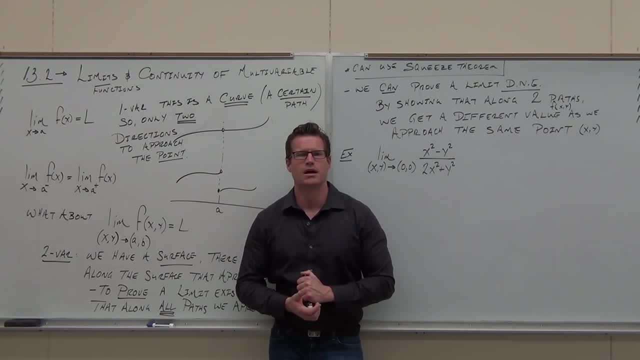 Here's the deal, because I just want you to be able to do it pretty easily, And we're going to use continuity to do it. The first thing you should do every single time when you get a limit from back to back from Calc 1, is what. 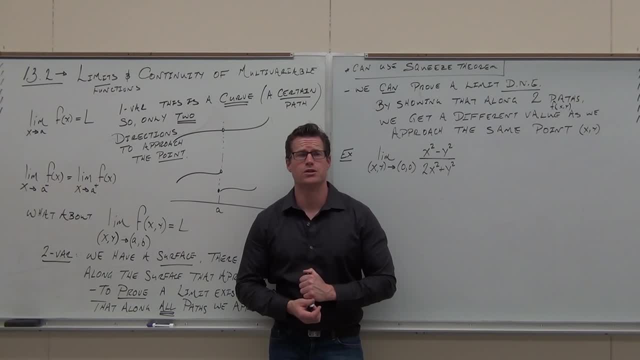 you to be able to do it pretty easily, And we're going to use continuity to do it. The first thing you should do every single time when you get a limit from back to back from calc 1 is what? Just plug it in. 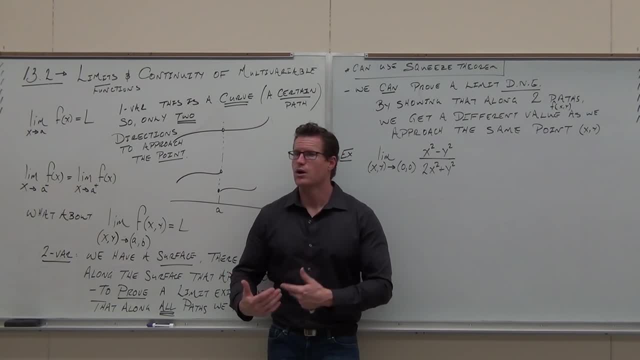 Just see if it actually works, And we're going to use that later, So try to plug it in Now. what do you get? 0 over 0.. L'Hopital's. Oh crap, Can we do? L'Hopital's. 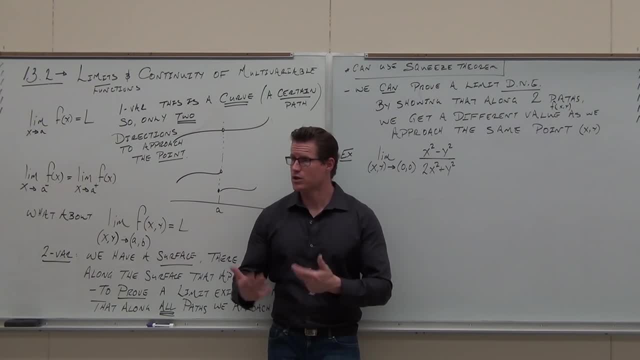 Plug it in. Just plug it in, Just see if it actually works. And we're going to use that later, So try to plug it in Now. what do you get? Zero, Zero over zero. L'Hopital's, Oh crap. 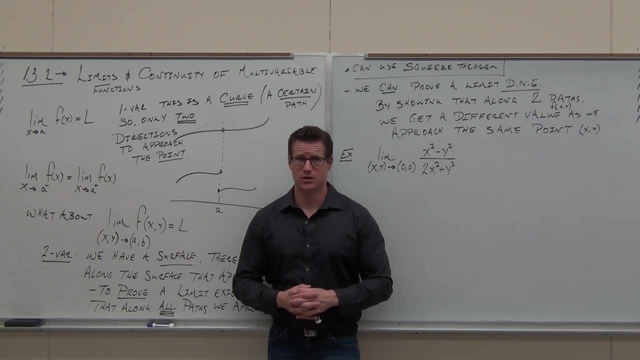 Can we do L'Hopital's? Do you know how to take derivatives with two independent variables? Yes, You do. How, Oh crap? Yeah, You have this, You have this. You've done physics, don't you? 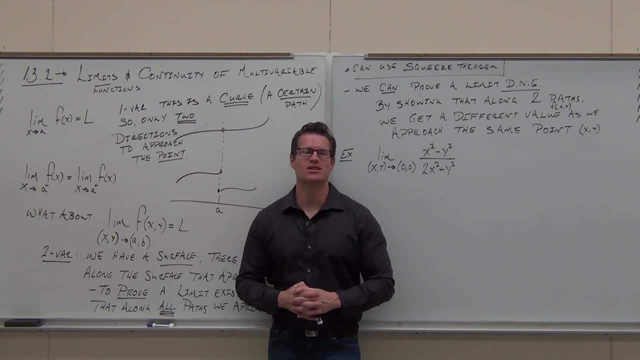 Suckers, Not yet. Next section: yeah, Changed a little bit. It's weird, But no, because what would you do with your partials right, Partial derivatives? what are you going to do with that? as far as your limit's concerned? 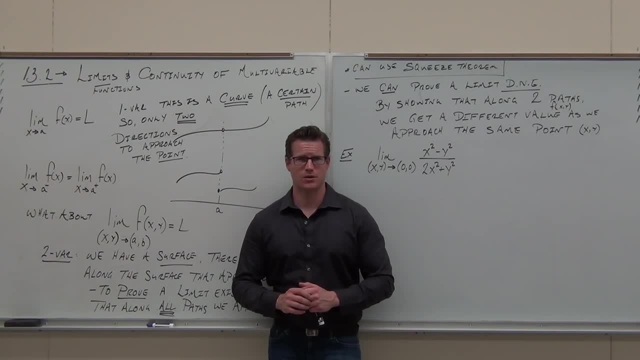 All that would do, because all you know right now from your physics class is that there are these things called partial derivatives. Some of you do not even know what they mean yet. You just know that you have to do them, And this is how you do them. 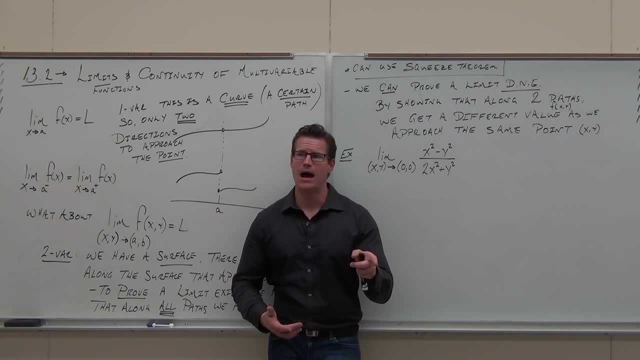 What they will do for you is: they will give you a path that is over, over a certain axis. that's all they do. They limit your travel along a surface over a certain axis. I will explain that in the next section. So will they help us? 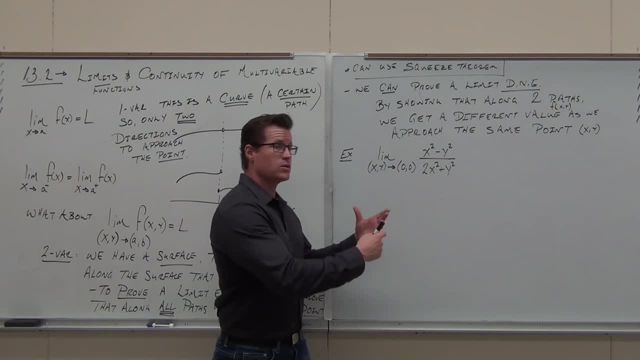 They could, but not generally. No, What we do is first you try to plug in, you get zero over zero, You go okay. well, that's a problem If it worked out to a number that's defined done. 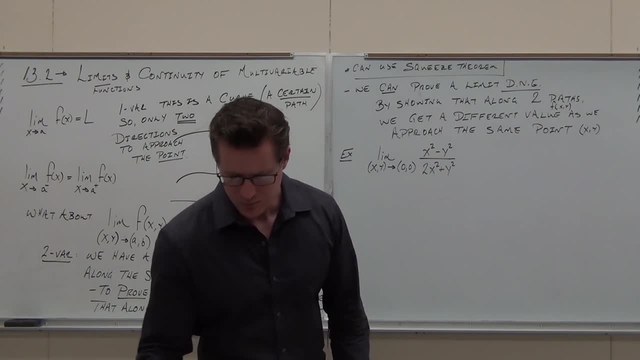 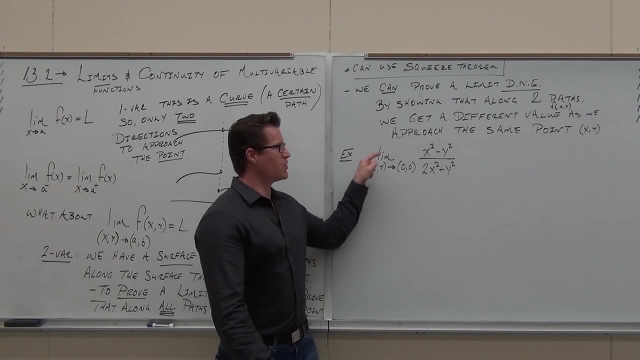 You're done. I'll show you why later. We'll talk about continuity later, But you'd be done. Here's what we're going to try to do now. What I'm going to ask you specifically for is show that this limit does not exist. 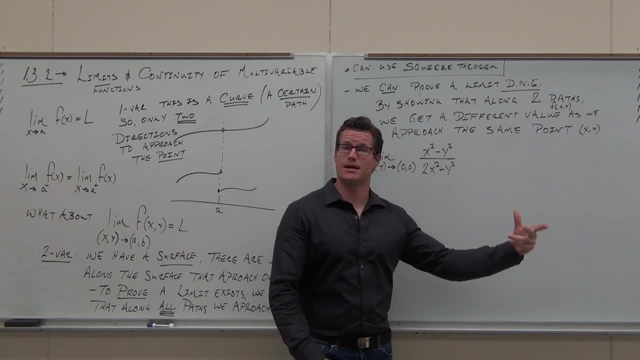 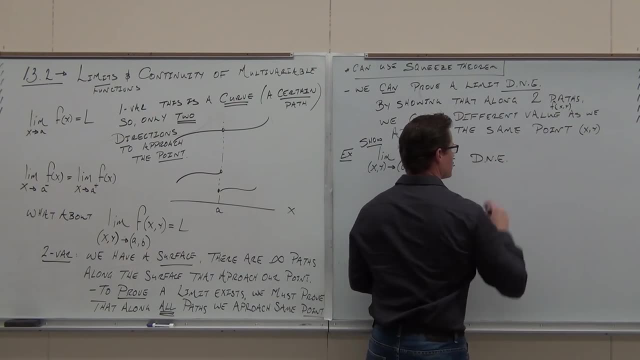 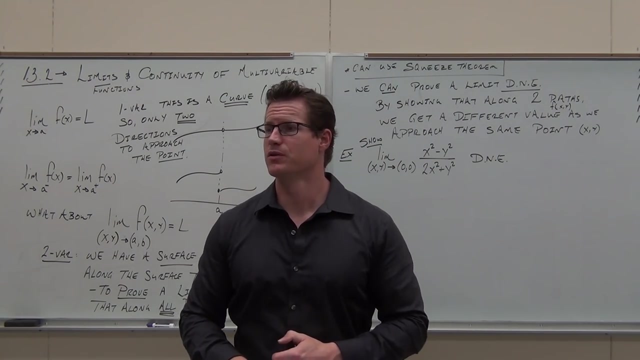 Not try to prove that it does exist, because it's not going to, But show that it doesn't exist. How, How? How many paths do we need to prove a limit exists- Infinite? How many paths do we need to prove a limit doesn't exist? 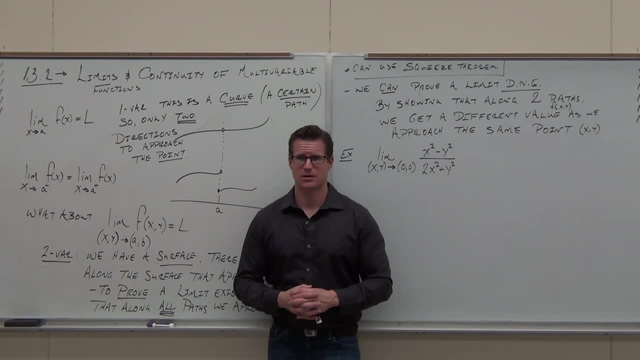 Do you know how to take derivatives with two independent variables? You do, How, Oh crap, you have physics, don't you Suckers? Not yet. Next section: yeah, Changed a little bit. That's weird, But no, because what would you do with your partials, right? 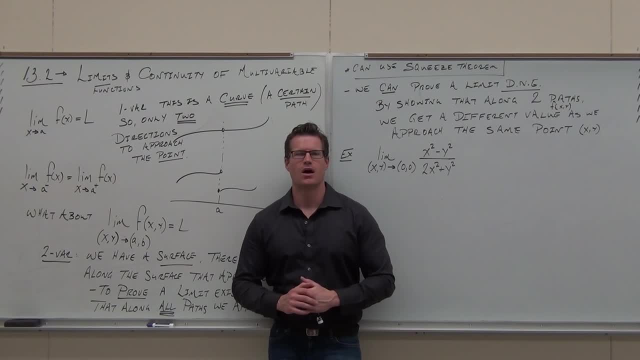 Partial derivatives. what are you going to do with that? as far as your limit's concerned, All that would do, because all you know right now from your physics class is that there are these things called partial derivatives. Some of you do not even know what they mean yet. 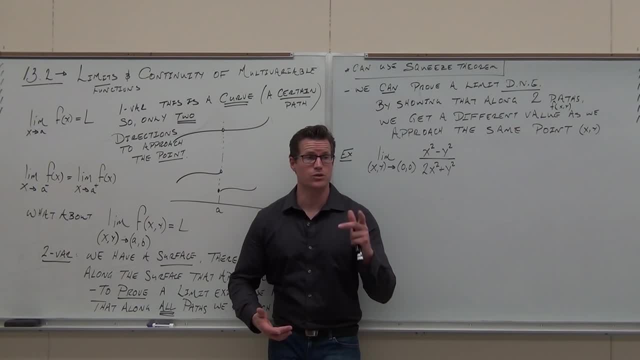 You just know that you have to do them, And this is how you do them. What they will do for you is they will give you a path that is over a certain axis. That's all they do. They limit your travel along a surface over a certain axis. 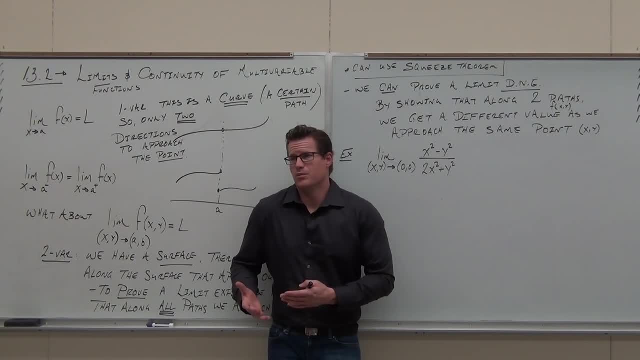 I will explain that in the next section. Will they help us? They could, but not generally. No, What we do is: first you try to plug in. you get 0 over 0. OK, well, that's a problem. 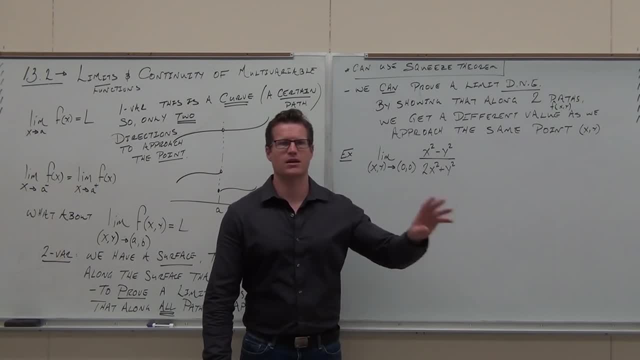 If it worked out to a number that's defined, done, You're done. I'll show you why later. We'll talk about continuity later, But you'd be done. Here's what we're going to try to do now, What I'm going to ask you specifically for. 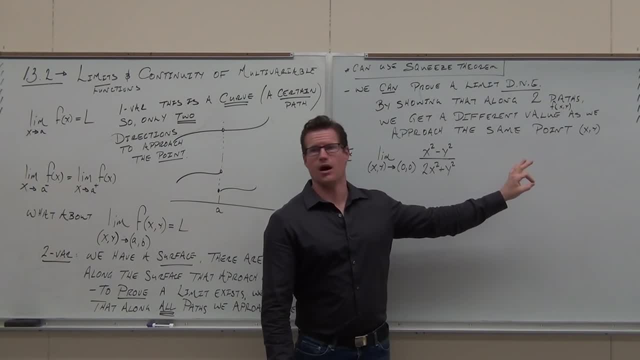 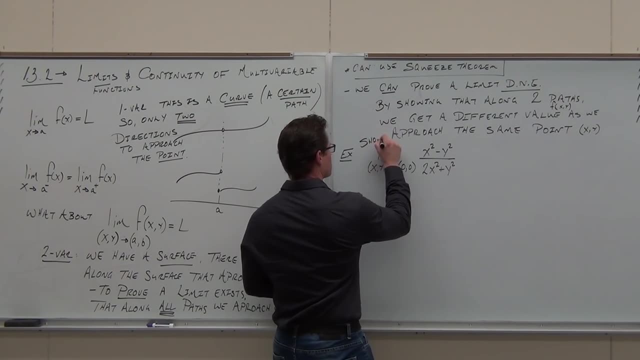 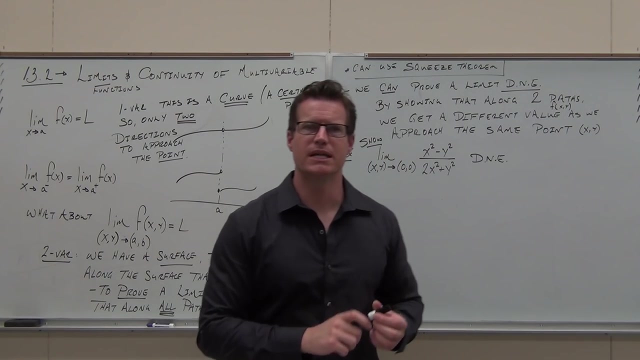 is: show that this limit does not exist. Not try to prove that it does exist, because it's not going to, but show that it doesn't exist. How many paths do we need to prove a limit exists- Infinite? How many paths do we need to prove a limit doesn't exist? 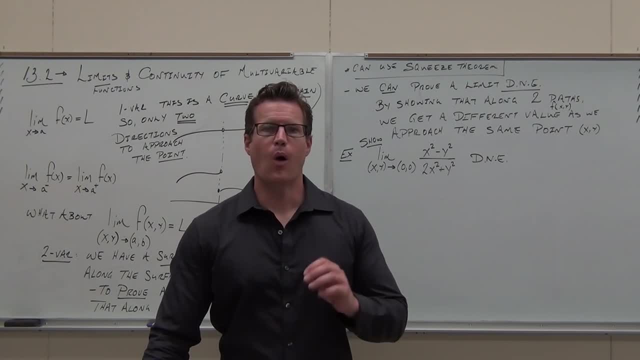 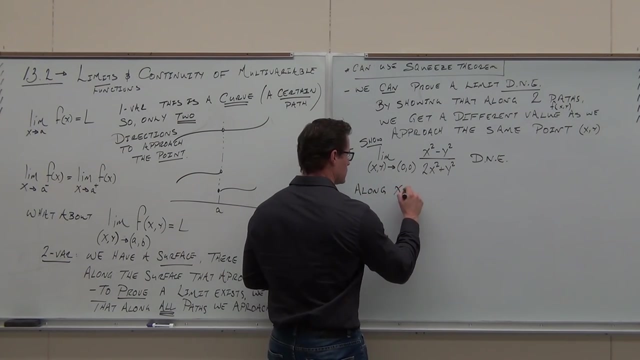 So let's pick two paths. I'll tell you something right now: Always pick x or y equals 0 as one of them. That's the easiest path. Now I'll show you that. So we're going to put along Along x equals 0.. 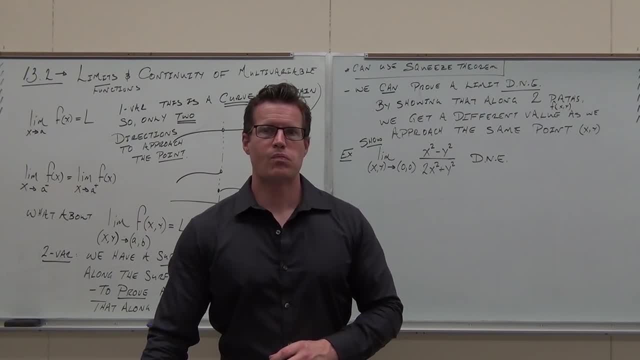 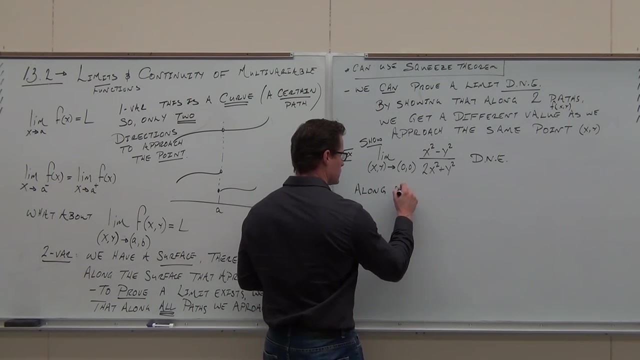 Two. So let's pick two paths. I'll tell you something right now: Always pick x or y equals zero as one of the two paths, One of them. That's the easiest path. Now I'll show you that. So we're going to put along along: x equals zero. 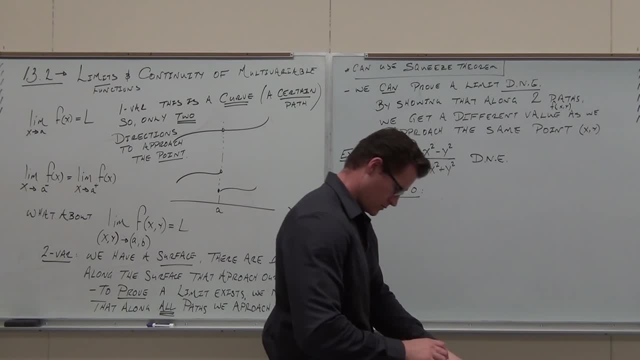 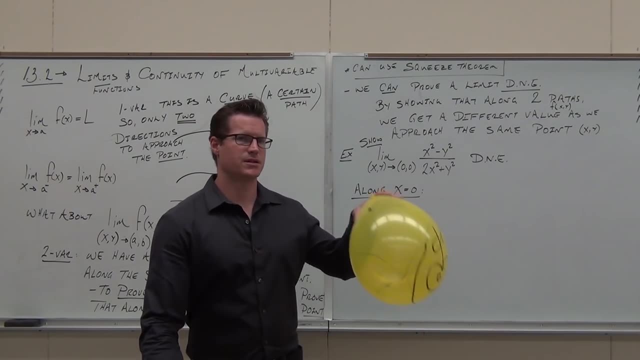 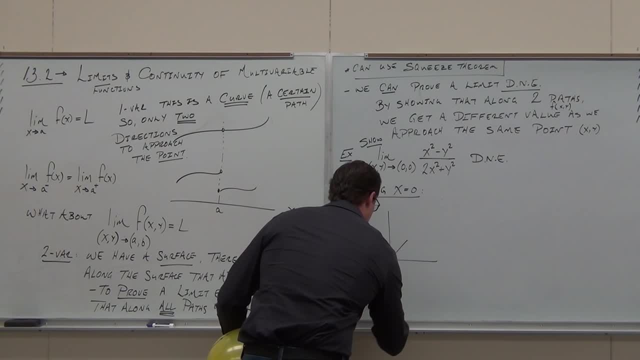 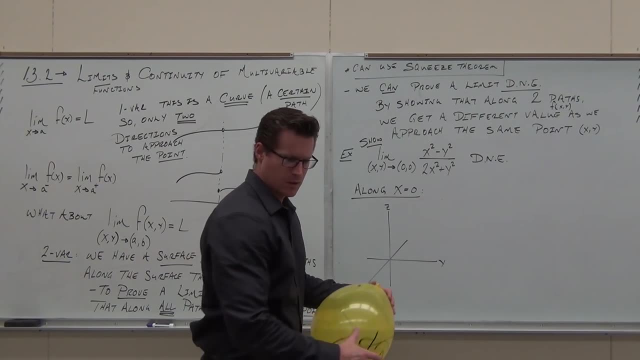 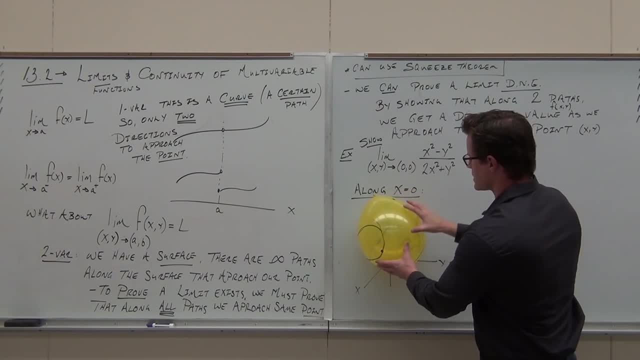 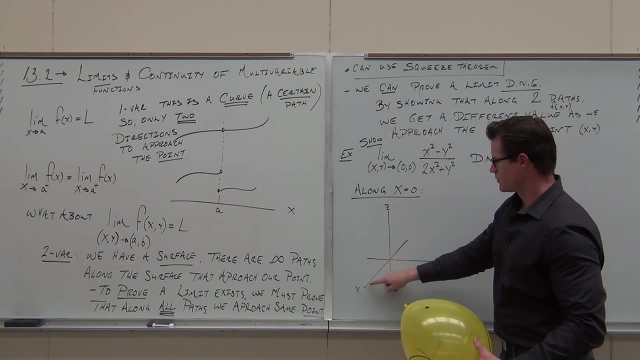 with that point is right right above the z. Okay, So this is the axis. Here's what's happening. If I let you do x equals zero- x equals zero goes way back here. then what's the only variable that we have? 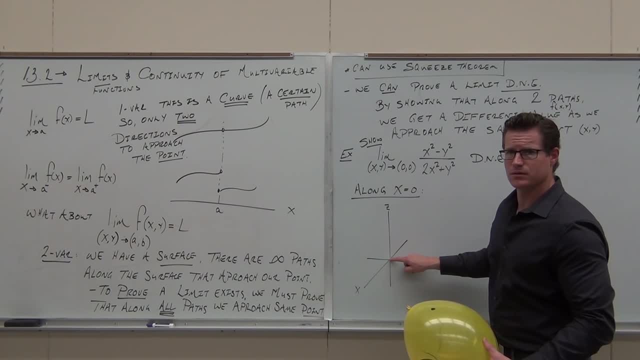 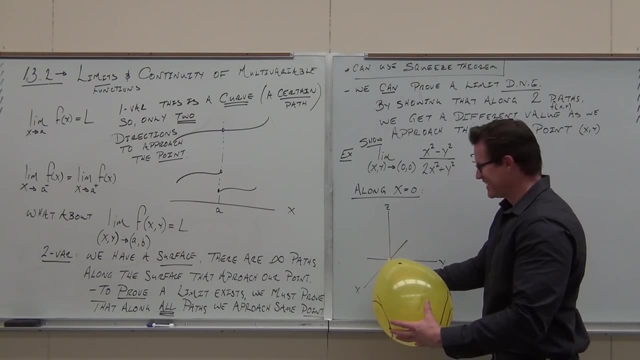 have left because I asked you: Oh, that was funny, come on. and it's y. I know, If I let x equal 0, then I say let's force that to be 0. We would be traveling along the y axis. 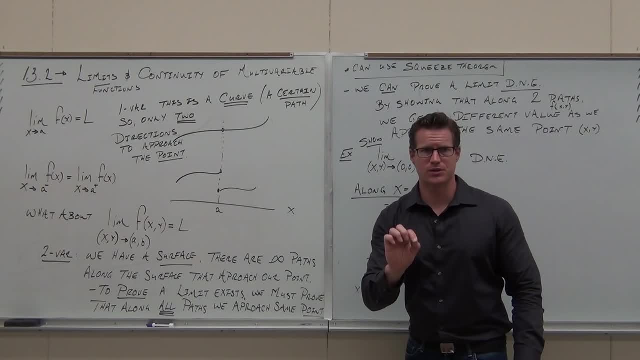 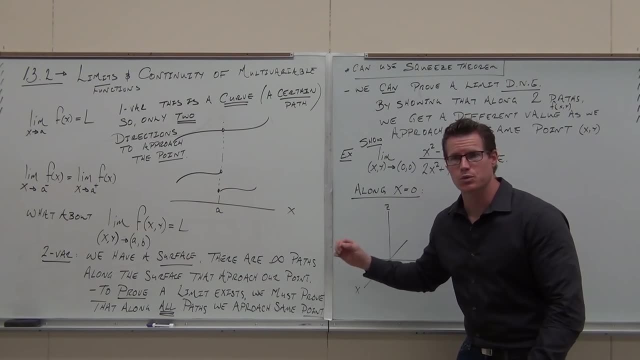 Please notice something right now. I'll explain it a little bit later as well. reiterate it, but notice something: 0, 0 is along the y axis. Do you see that We have to? whatever we restrict, it's got to be a solution. 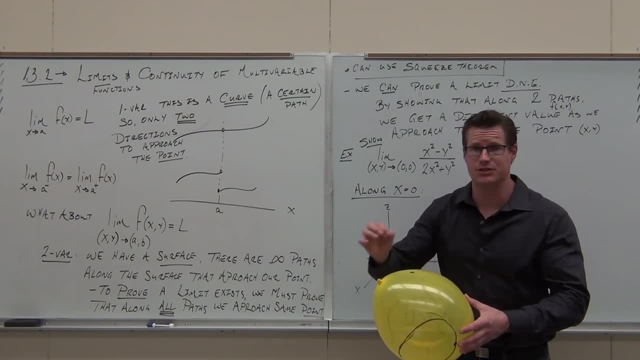 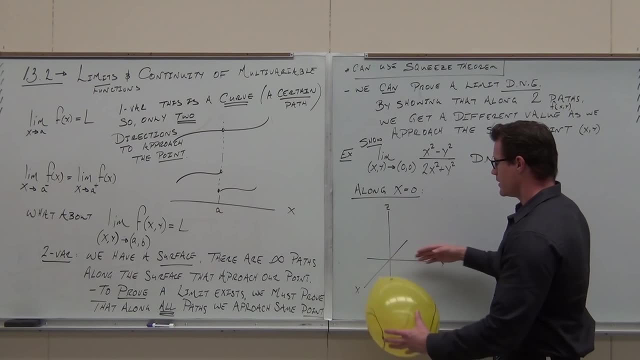 have that point as a point. on that line. We have to do that. We can't go. I don't want to go over here. We've got to travel over whatever we're restricting this to. So if I say let's let x equal 0, then what this implies is that I'm going. 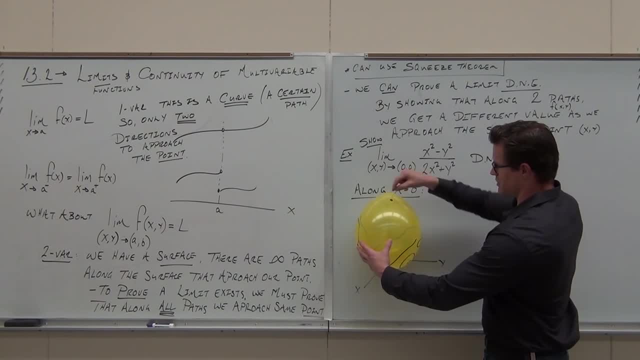 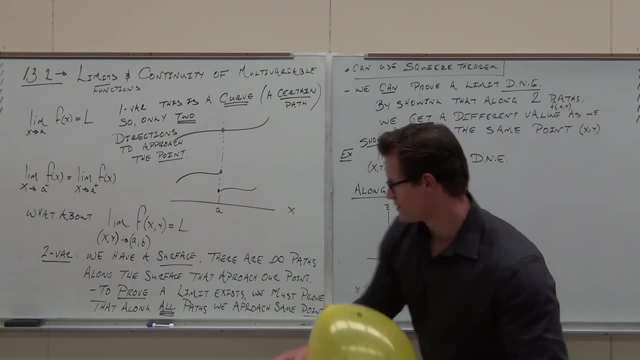 to be approaching that point, the point down here, and here's the function value, but only along the y direction. So this would be the curve that's doing this. So I'm going to take the path Where x is 0, that's right along. I'm going to try to do it this way, so you see it. 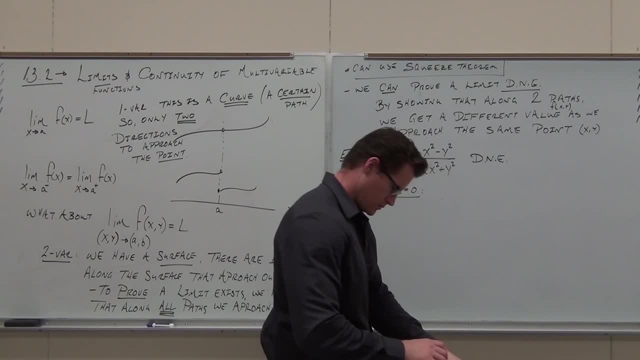 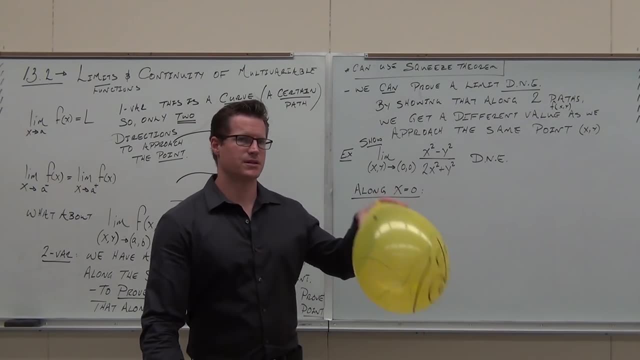 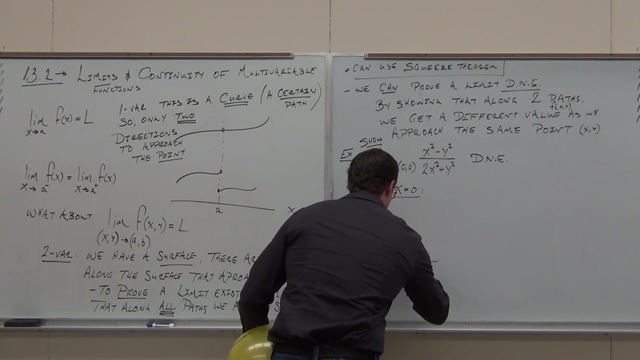 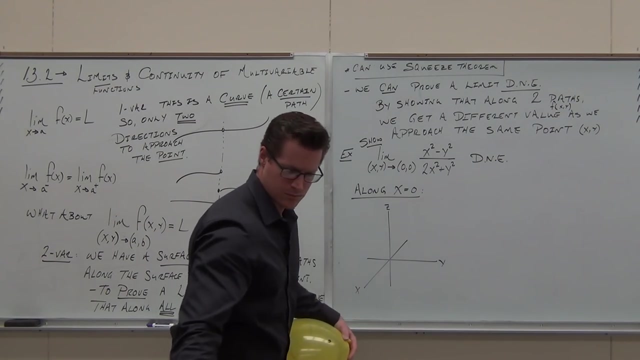 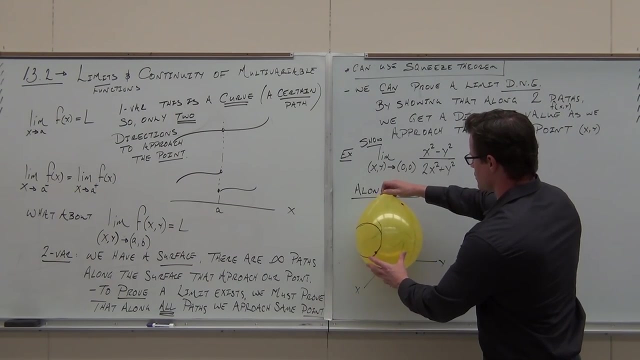 Oh man, I need another balloon. Along. x equals 0.. Here's what this does. Can you imagine? Can you imagine this? So along x equals 0.. Imagine this at the origin, with that point is right above the z, OK. 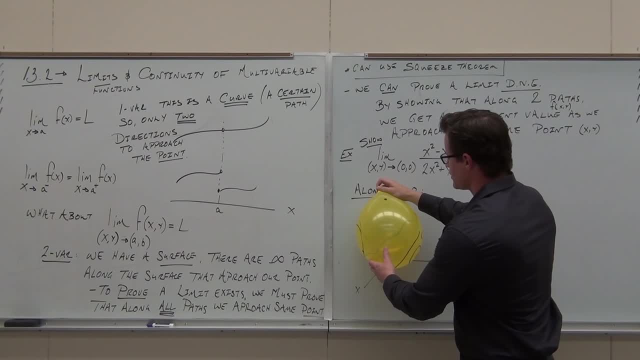 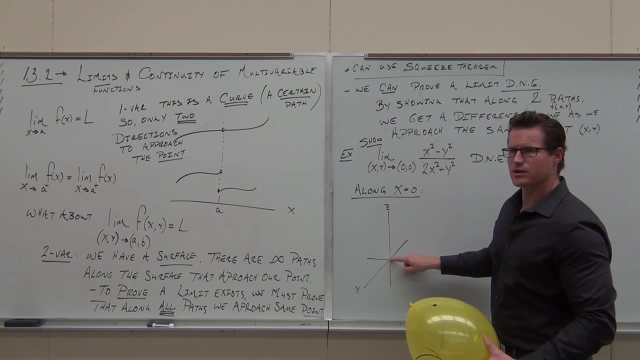 So this is the axis. Here's what's happening. If I let you do: x equals 0, x equals 0 goes way back here. Then what's the only variable that we have left? 1. Because I asked you. Oh, that was funny. 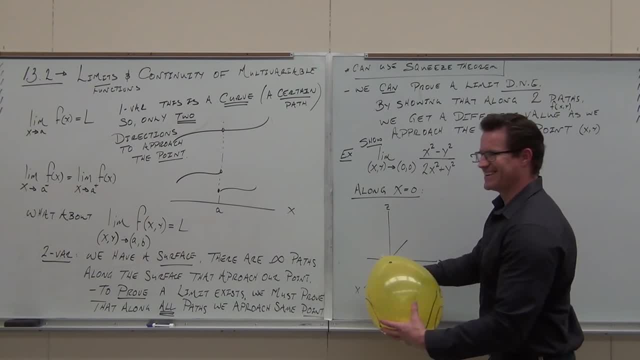 Come on, And it's y. I know, If I let x equals 0, then I say let's force that to be 0. We would be traveling along the y-axis. Please notice something right now. I'll explain it a little bit later as well. 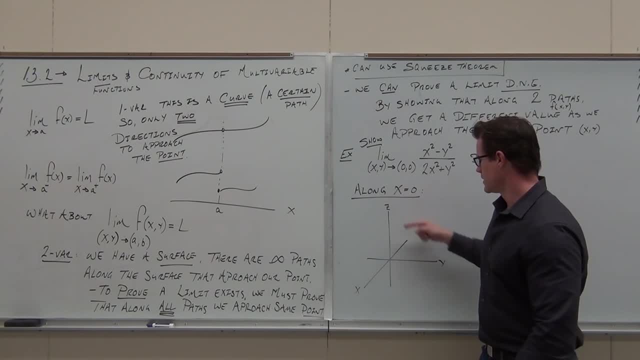 I'll reiterate it, But notice something: 0, 0 is along the y-axis. Do you see that We have to? Whatever we restrict, it's got to be a solution. Have that point as a point on that line. 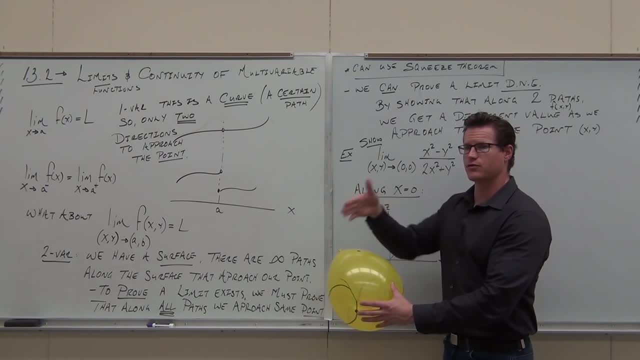 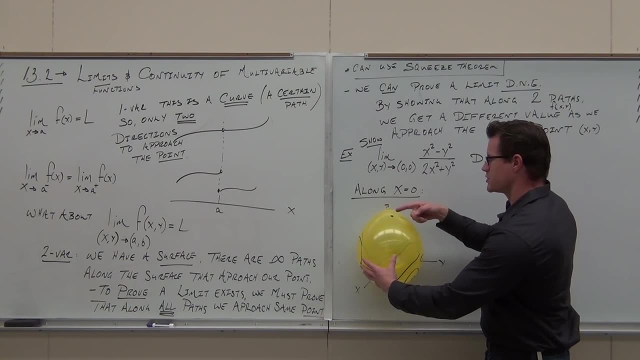 We have to do that. We can't go Now. I'm going to go over here. We've got to travel over whatever we're restricting this to. So if I say let's let x equals 0, then what this implies is that I'm going to be approaching that point, the point. 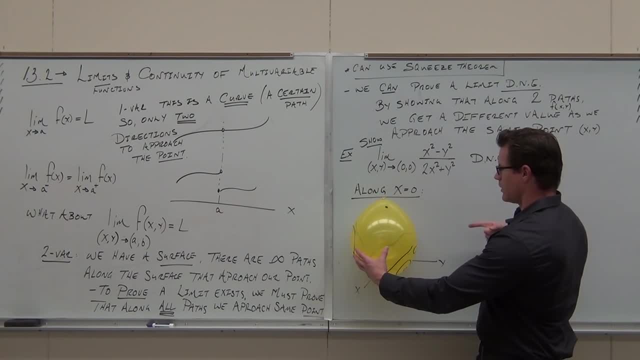 down here and here's the function value, but only along the y-direction. So this would be the curve that's doing this. I'm going to take the path where x is 0.. That's right along. I'm going to try to do it this way, so you see it. 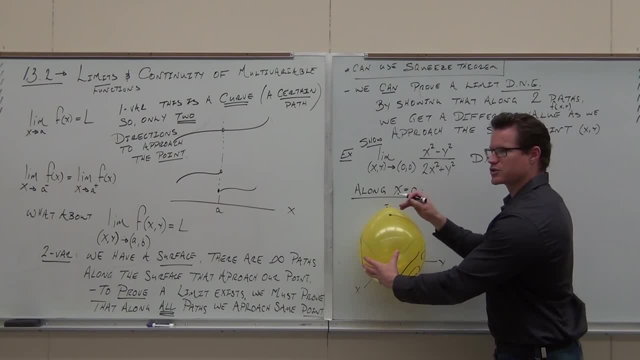 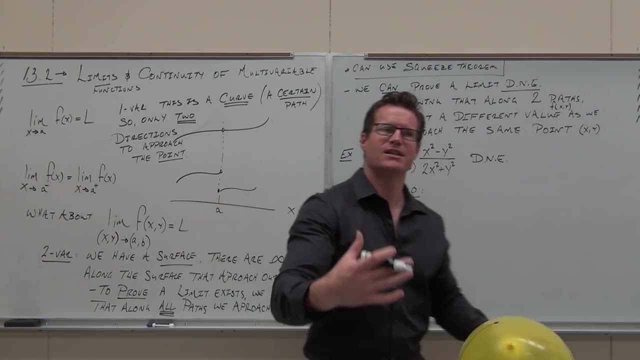 Right along, just the y-direction, Just right over or under the y-axis. Do you guys get what I'm talking about? So if I let this go along, x equals 0,. what about the z? The z is the height. I don't have to worry about that. 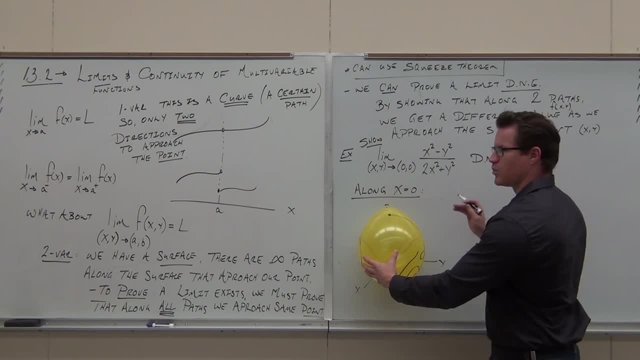 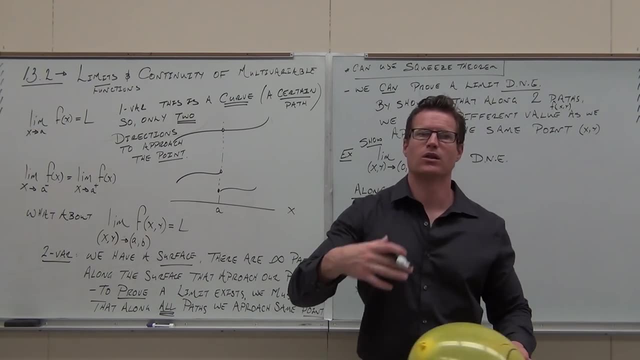 Right along, just the y direction, Just right over or under the y axis. Do you guys get what I'm talking about? So if I let this go along, x equals 0,. what about the z? The z is the height. I don't even have to worry about that. 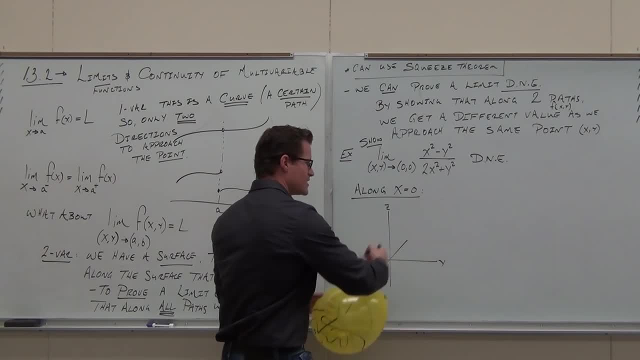 That's a dependent variable. I'm only worried independent. So if I let x equal 0, what I'm doing is I'm traveling over the surface, right over the y axis. Do you guys see that? Do you guys get that? So this right here is traveling along the surface, directly over the y axis. 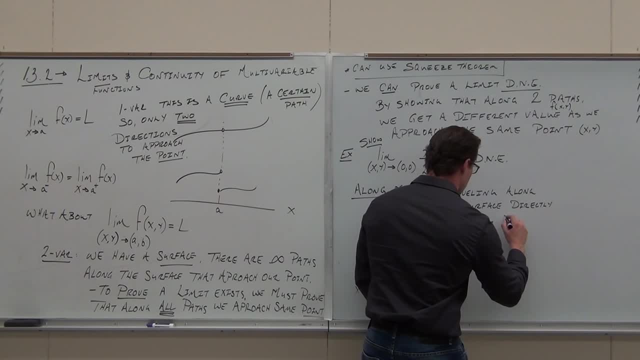 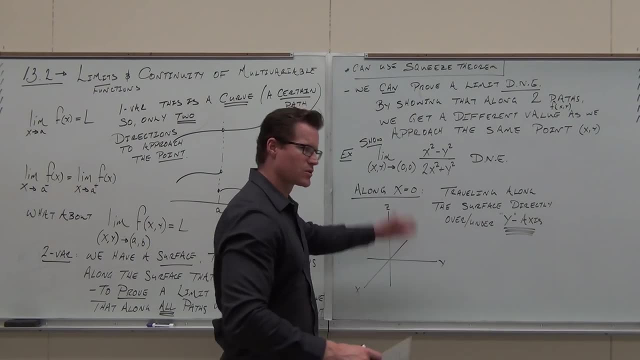 Now what I'm doing is I'm told to let x equal 0.. Not the x. X equals 0 is not over the x axis. X equals 0 is over the y axis. Now let's see what it does mathematically. 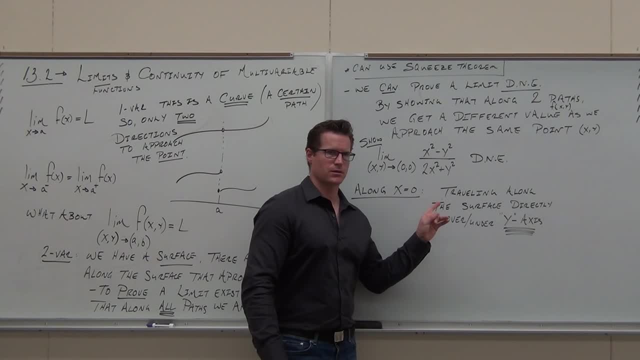 If I force x to be 0, look, look, stop writing, just look for a second. If I force x to be 0, what happens to my x? 0. 0. 0. 0. 0.. 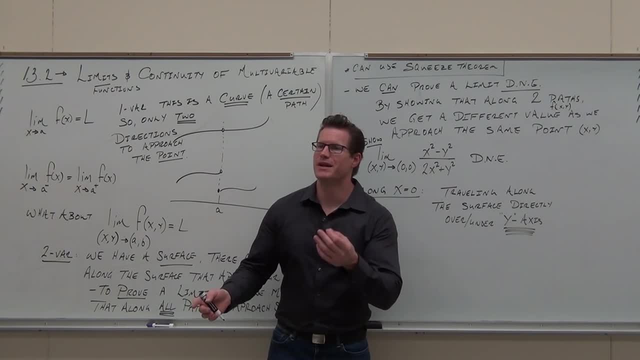 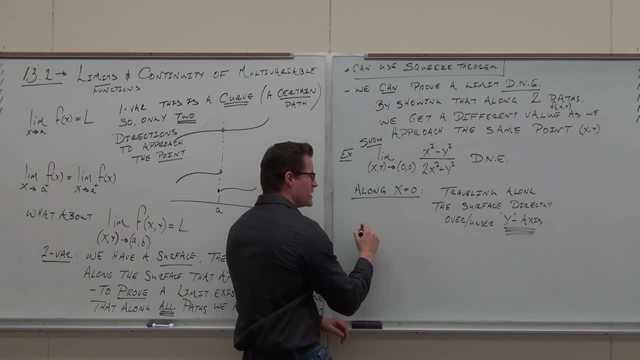 If I go along, X equals zero. all my X's are zero. This limit now becomes a limit of what's on the numerator. If X is zero, well, you know what we'll do it. How much is X Zero? 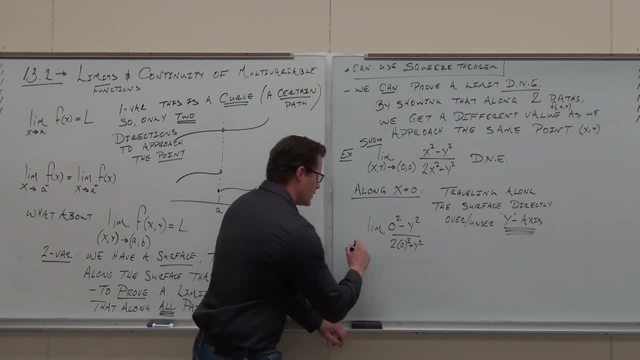 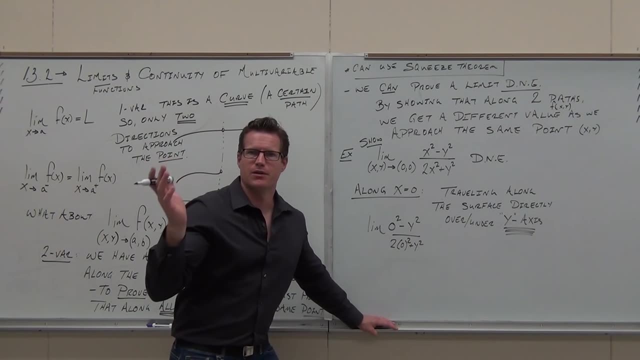 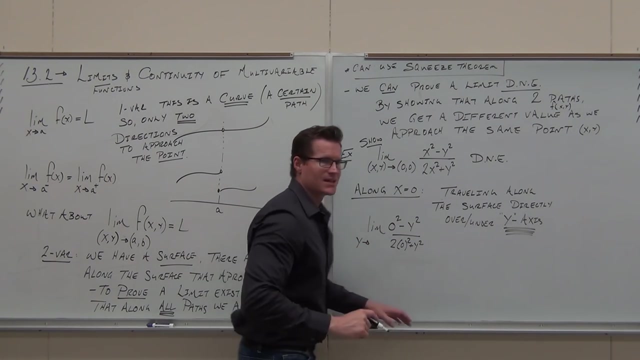 As: but wait, wait for it, As what approaches? what Is X approaching anything anymore? No, we don't even need it because X is fixed. So what that allows us to do is basically take a 2,- sorry, 3D- limit and change it into a 2D limit. 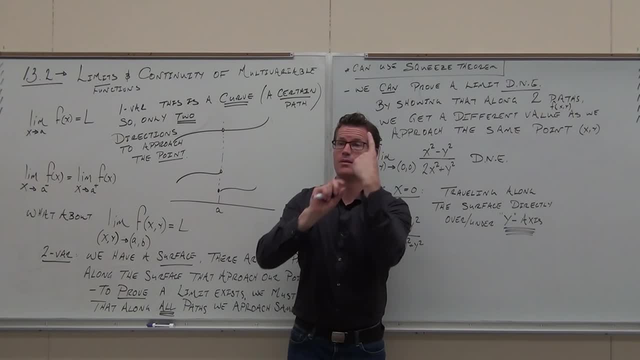 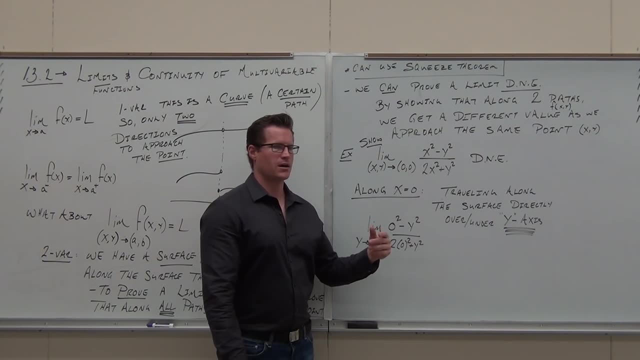 Or take two independent variables and make it- let's see which one- this one- make it one independent variable. So, instead of X1.. Y approaching zero, zero. forget it, man. I'm already stuck here. I've already let X go to zero. 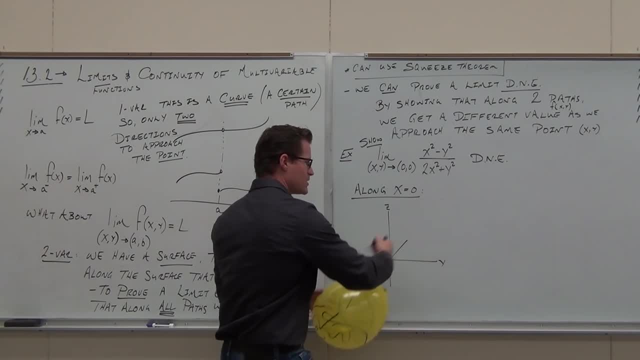 That's a dependent variable. I'm only worried independent. So if I let x equal 0, what I'm doing is I'm traveling over the surface, right over the y-axis, Did you guys get that? So this right here is traveling along the surface directly. 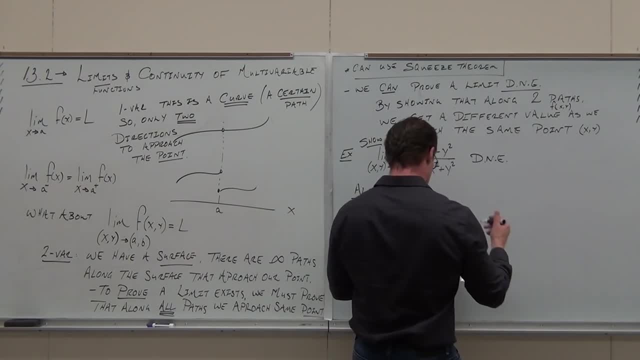 over the y-axis. So I'm going to do x equal 0 right here, And when I'm at the center of the y-axis, I'm going to take the path. here I'm going to seems like I'm going to make a difference. 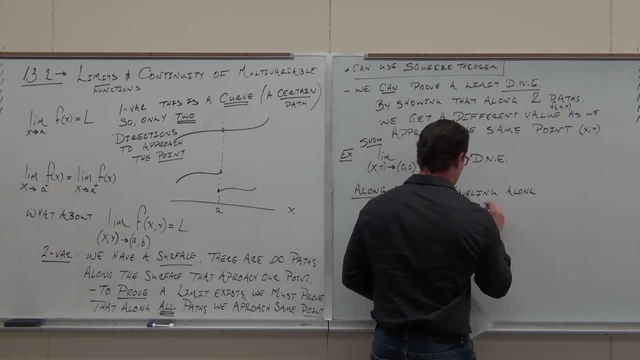 over all of this And I'm going to say that this, this is the y-axis. I'm going to say I didn't do it, I just did it because that was theve of y, that I did. So, right over this value. I'm going to say: 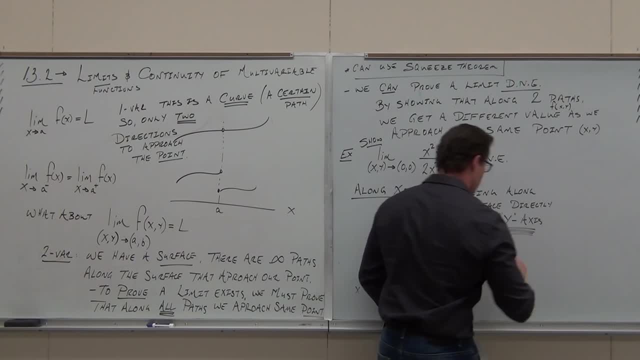 here is the y-axis And that's the z. So I'm going to say: here is the y-axis And I'm just going to say: here is the y-axis, Not the x. x equals 0, is not over the x-axis. 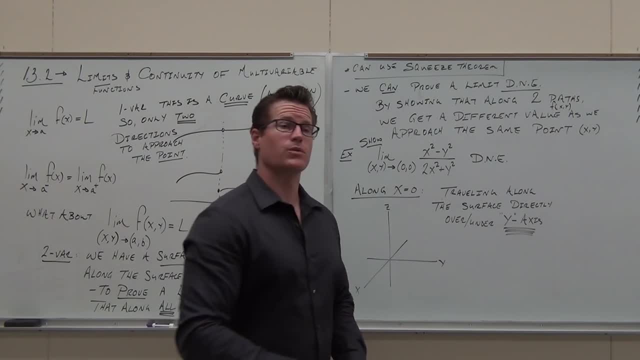 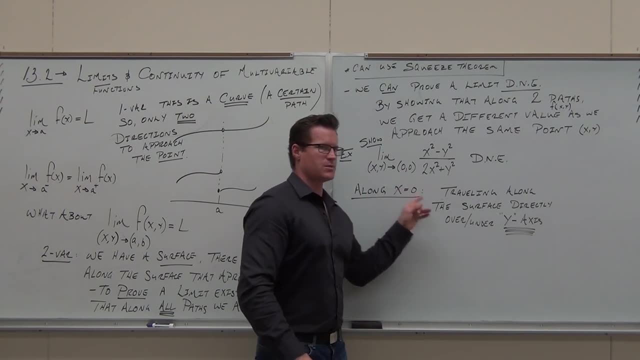 x equals 0 is over the y-axis. Now let's see what it does mathematically. If I force x to be 0, look, look, stop writing, Just look for a second. okay, If I force x to be 0, what happens to my x's? 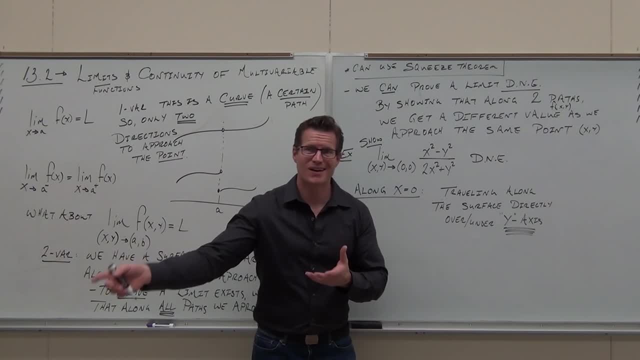 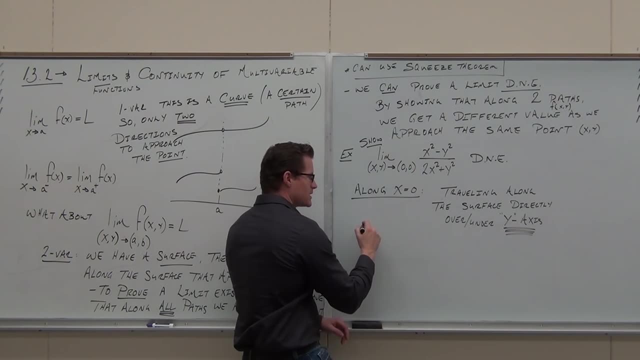 They are 0.. The only variable that now changes is The y, The y variable. That changes our limit completely. If I go along, x equals 0, all my x's are 0. This limit now becomes a limit of what's on the numerator. 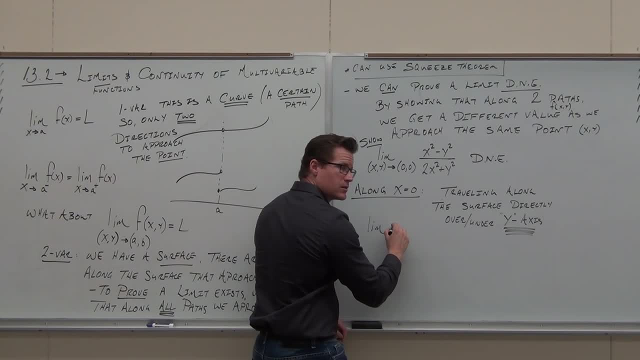 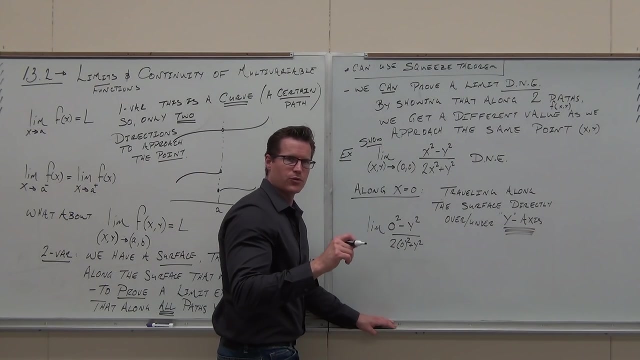 If x is 0, well, you know what We'll do it. How much is x 0. As? but wait, wait for it, As what? A plus A plus, So what is x approaches what? 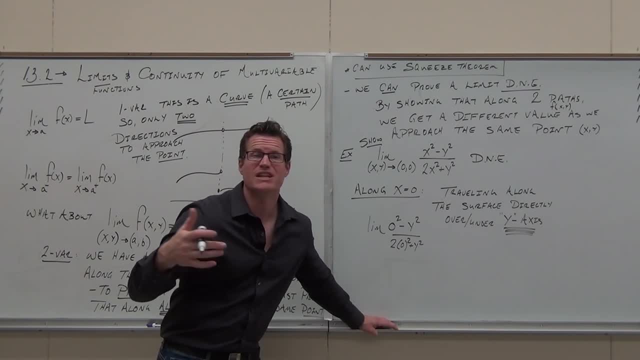 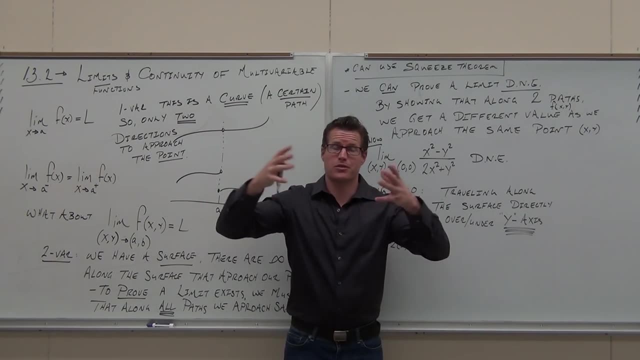 Is x approaching anything anymore? No, No, we don't even need it because x is fixed. So what that allows us to do is basically take a 2,- sorry, 3D- limit and change it into a 2D limit. 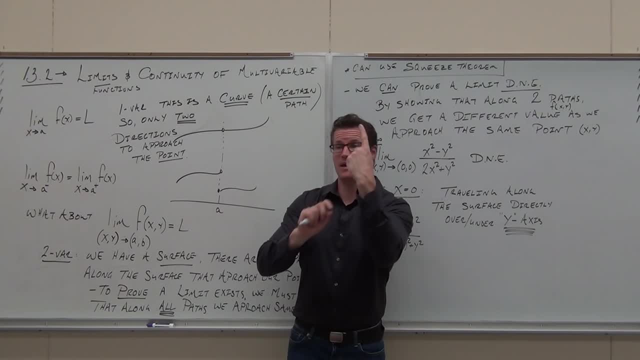 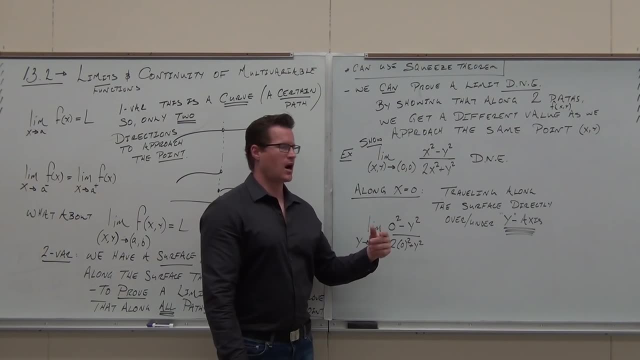 Or take two independent variables and make it- let's see which one- this one make it one independent variable. So, instead of x, y approaching 0, 0, forget it, man, I'm already stuck here. I've already let x go to 0. 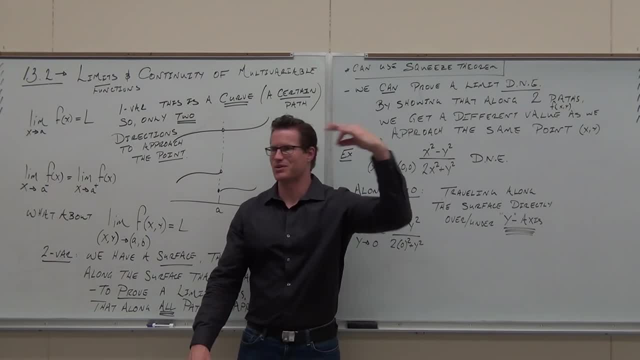 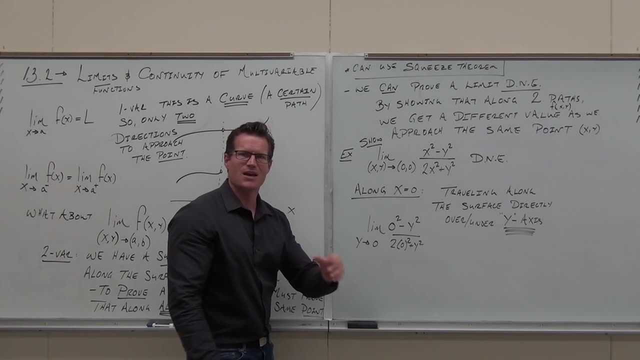 I'm just along that path. Of course it's going to hit X equals zero at some time at somewhere along the surface, But now I'm only letting the Y change. Does that make sense to you? If I'm along the Y, man, I hope it's sinking in. 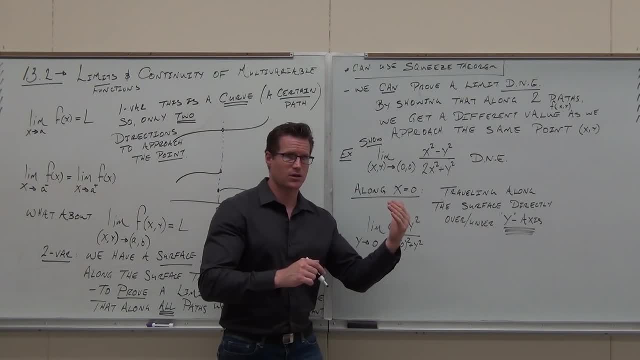 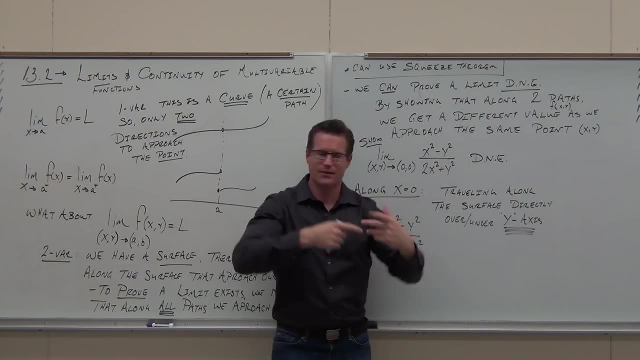 If I'm letting along, X equals zero. that's literally solely above the Y axis, Do you guys get it? Which means that the only thing that can be changed is the Y? I'm right over that. That's it. Well, let's make it easy. 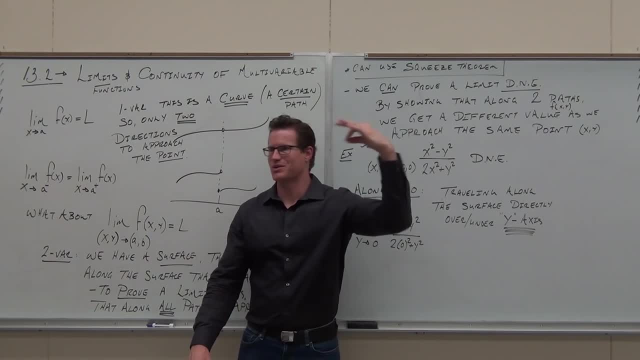 I'm just along that path. Of course it's going to change. I hit x equals 0 at some value, at some time at somewhere along the surface, But now I'm only letting the y change. Does that make sense to you? 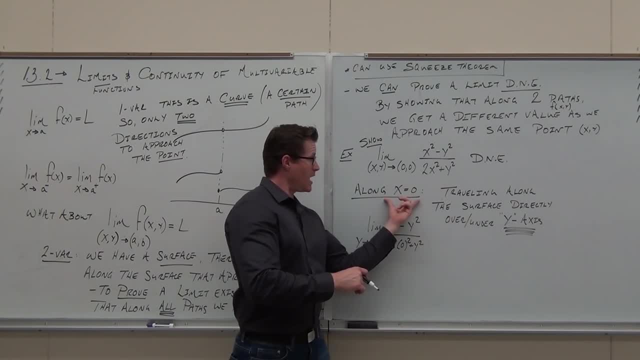 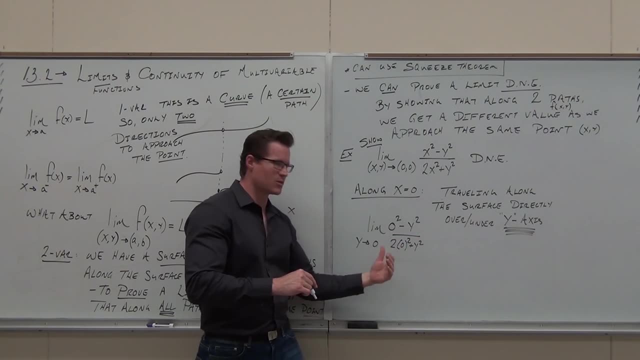 If I'm along the y man, I hope it's sinking in. If I'm letting along, x equals 0, that's literally solely above the y axis, Do you guys get it? Which means that the only thing that can be changing is the y. 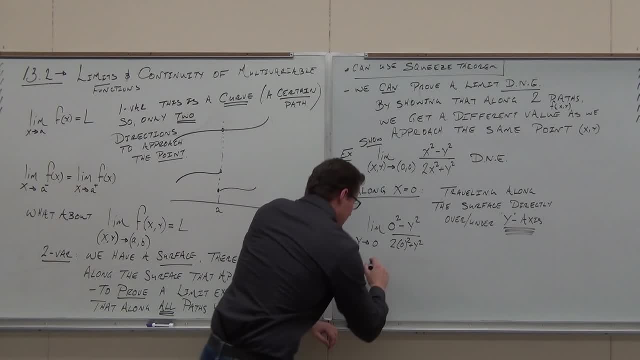 I'm right over that. That's it. Let's make it easy. Negative y squared over y squared. I don't care how fast or slow you are, You do your limits at this point. Once we change it, here you're done. 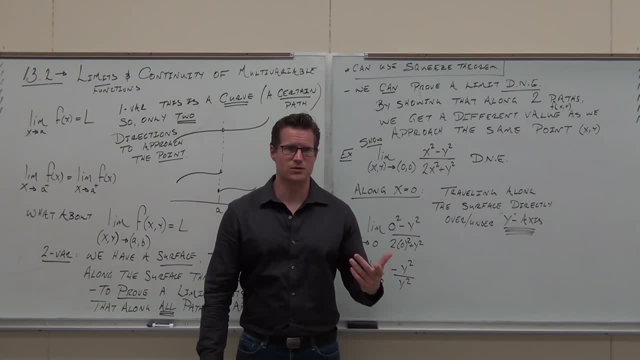 If you want to match degrees, which is always a great idea, you can do it. If you want to do lobitoles two times fine, Divide by the large power of the denominator, I don't care. What are you going to get out of this thing. 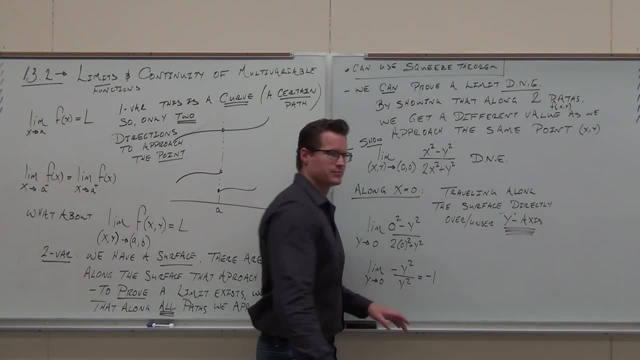 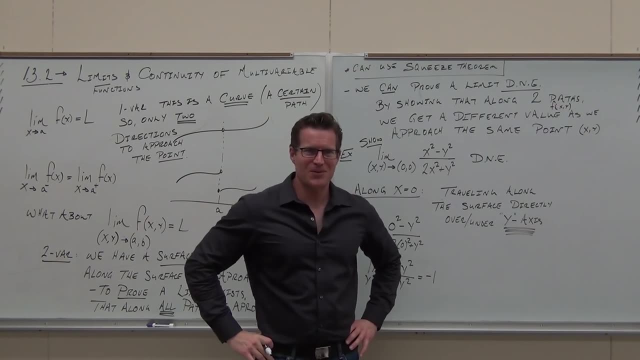 I'm going to get a 1. Perfect, That was heaven saying I love these answers. No, no, it's just Adam's fault. That's okay. Question: Did that prove the limit exists? Yes, No. Have we shown every possible path? 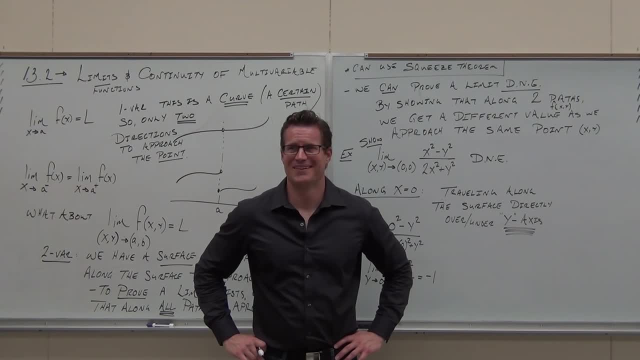 Yes, No, Definitely. You've shown one, The one that's right. Let's talk about every possible. I don't have infinite time to do that. We have one path right here. All we have to do is show one path. 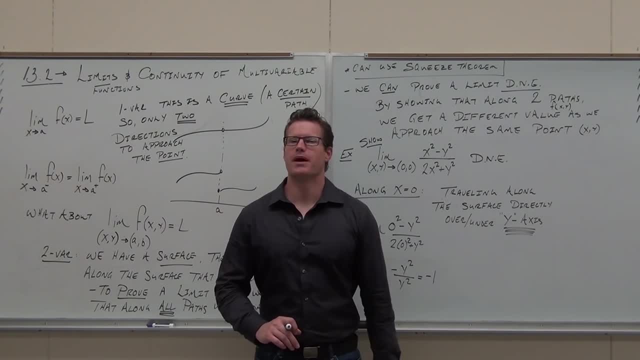 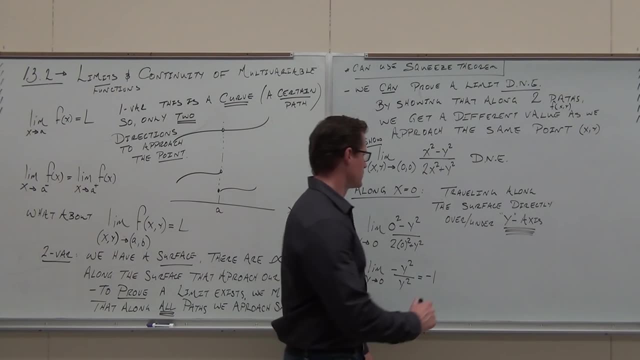 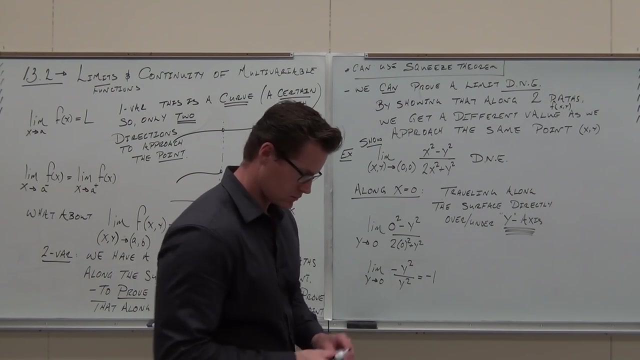 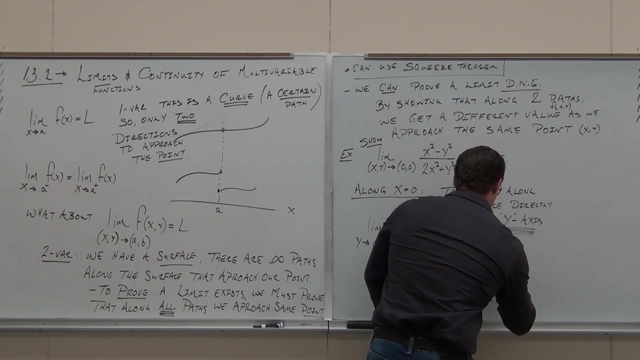 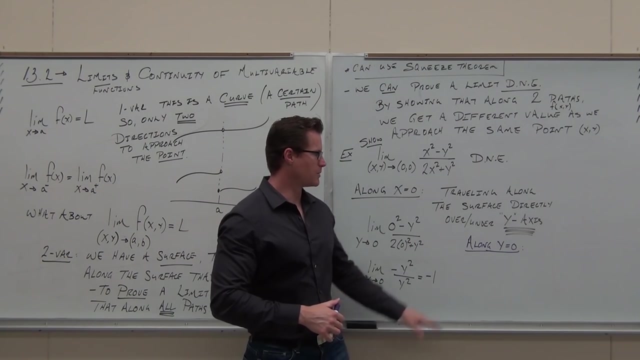 So it doesn't exist? all right, That's literally the point. Show me one other path along. what do you think Intuitively? What do you think? Let's try that. Why don't you set that up? As you're writing this, I'm going to say a little blurb. 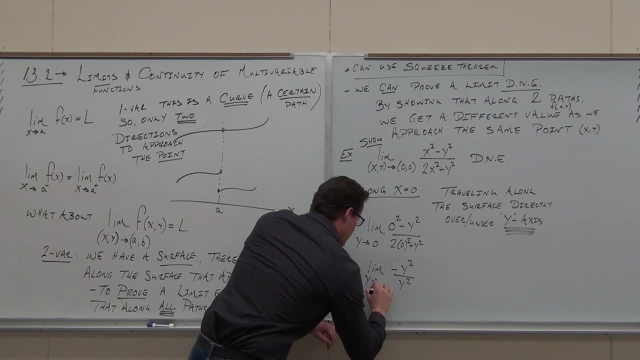 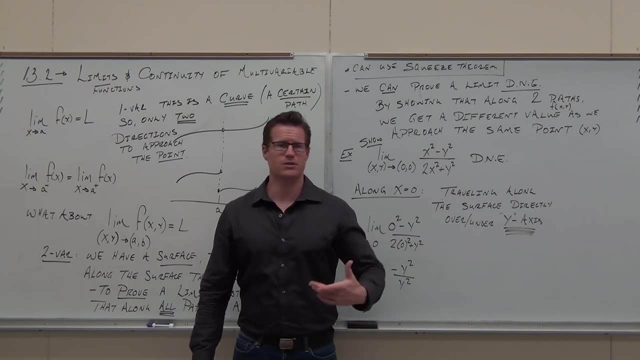 Negative: Y squared over Y squared. I don't care how fast or slow you do your limits at this point. Once we change it here, you're done. If you want to match degrees, which is always a great idea, you can do it. 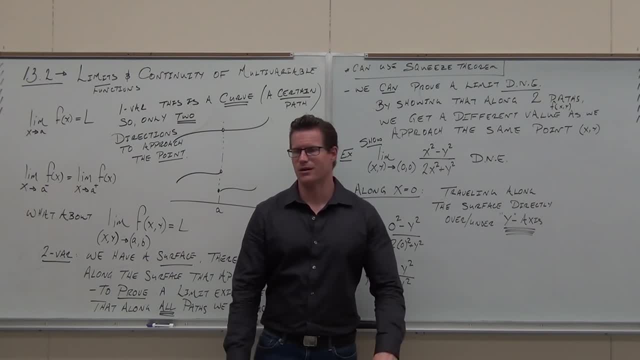 If you want to do Lobitols two times, fine. Divide by the large power of the denominator. I don't care What are you going to get out of this thing. I'm going to get one here and one there, Perfect. 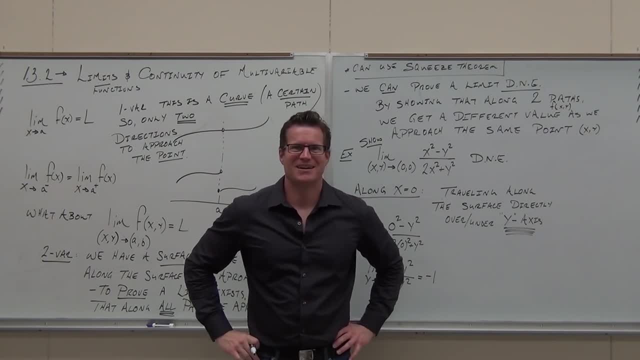 That was heaven's saying. I love these answers. All right, We're still here. No, It's just Adam's phone. It's okay. Question: Did that prove the limit exists? Yes, No, Have we shown every possible path? 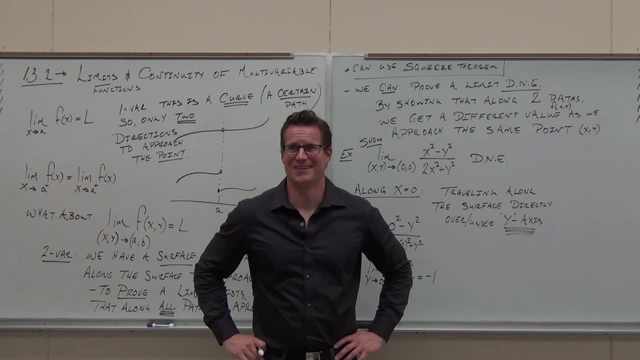 Yes, No, Definitely. We've shown one, The one that's right. Let's talk about every possible. I don't have infinite time to do that. We have one path right here. All we have to do Is show one path. 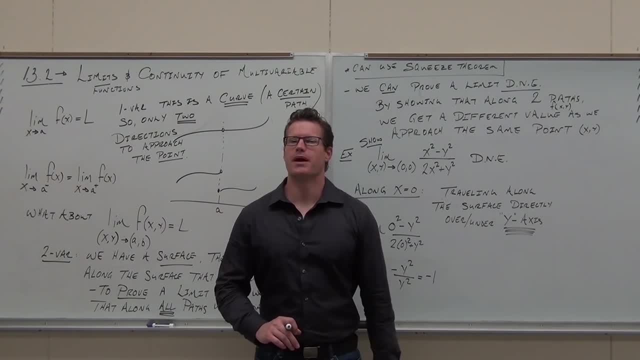 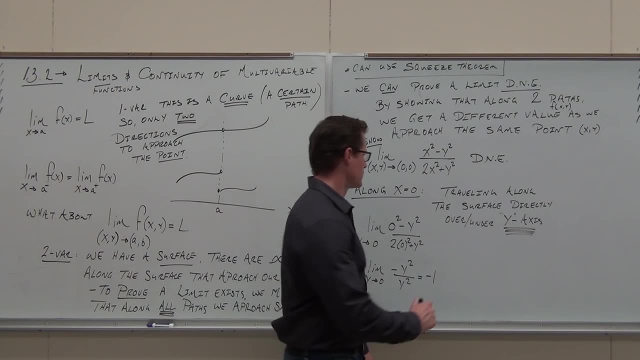 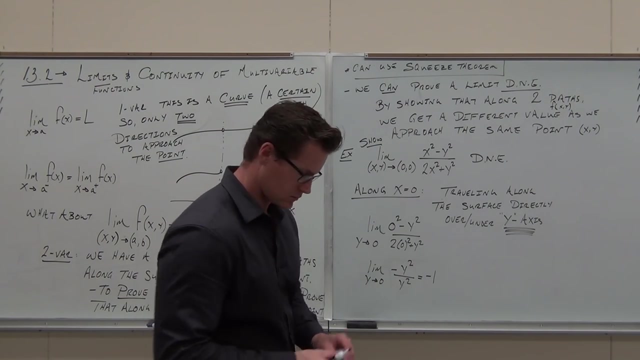 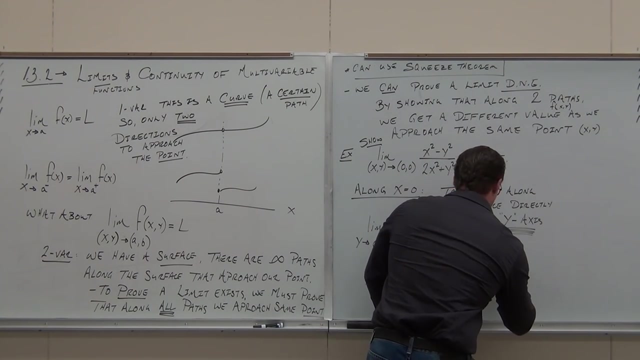 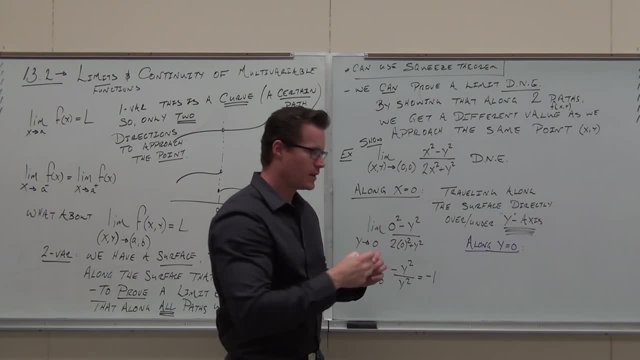 Twenty minutes, Okay, Bye, bye. 10 minutes, See you, Bye. Okay, Bye, Bye. As you're writing this, I'm just going to say a little blurb Along: y equals 0. shuts down the y-axis. 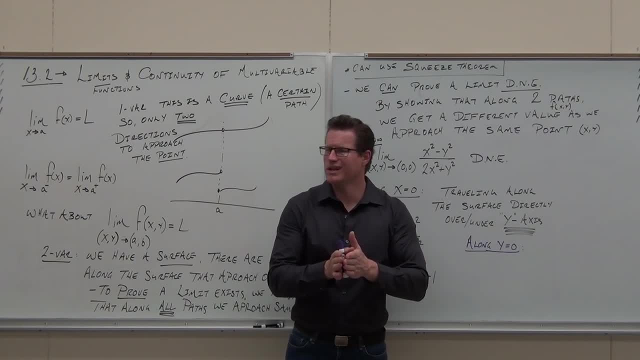 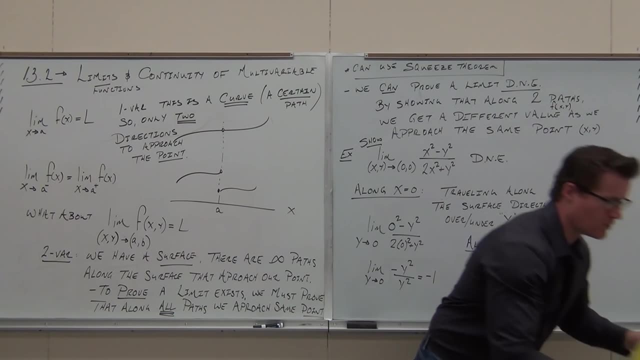 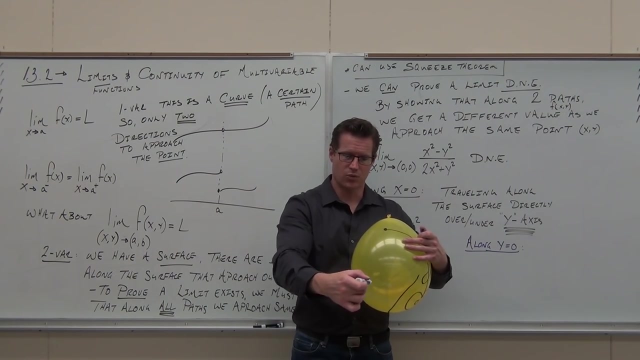 It forces you to only travel the surface, right above your only other independent variable, which is x. So this would be traveling the surface right along the x-axis. That's it. It would give you this. So if this is the y, the x would be traveling this way, so traveling on the surface, but right above the x-axis. 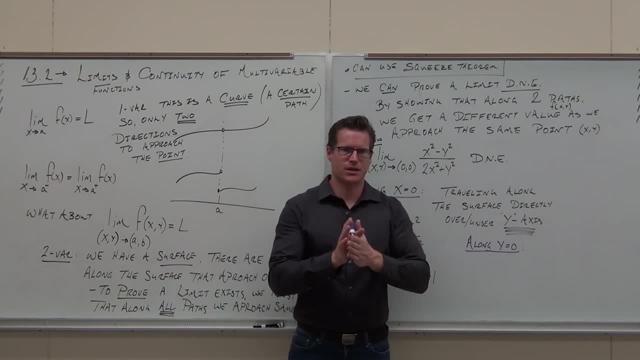 Along y equals 0 shuts down the y axis. It forces you. It forces you to only travel the surface right above your only other independent variable, which is x. So this would be traveling the surface right along the x axis. that's it. 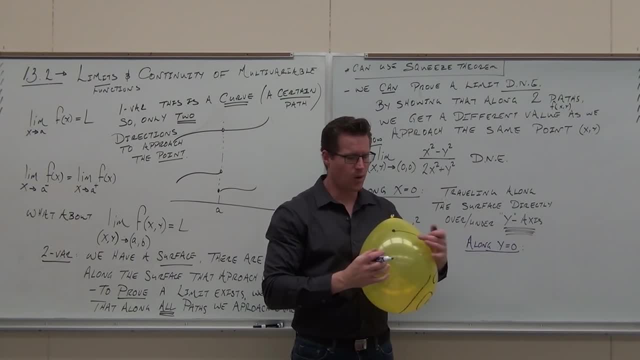 It would give you this. So if this is the y, the x would be traveling this way, so traveling on the surface, but right above the x axis. It would be trying to give you this idea. Now, what I'm going to try to show you here is: 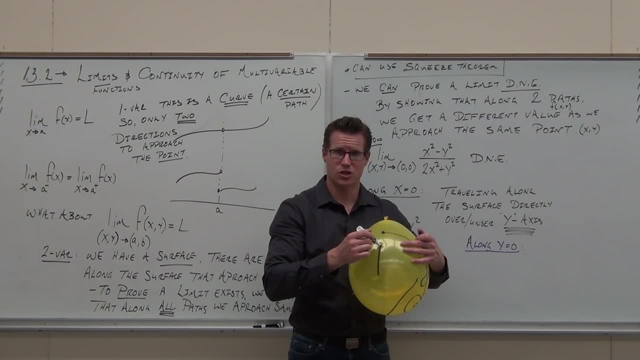 It would be trying to give you this idea. Now what I'm going to try to show you here is that these things don't match up On this balloon. they would match up. This would not be good for us. I'll show you what to do in that situation in just a minute. 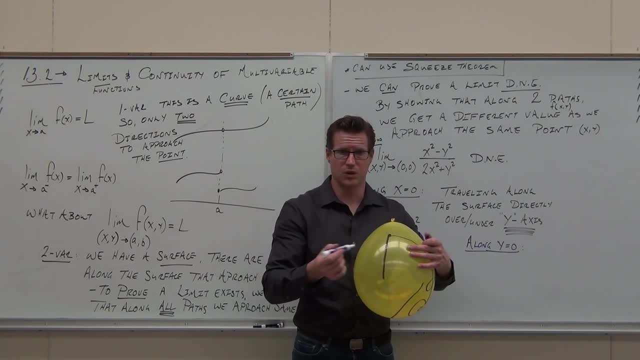 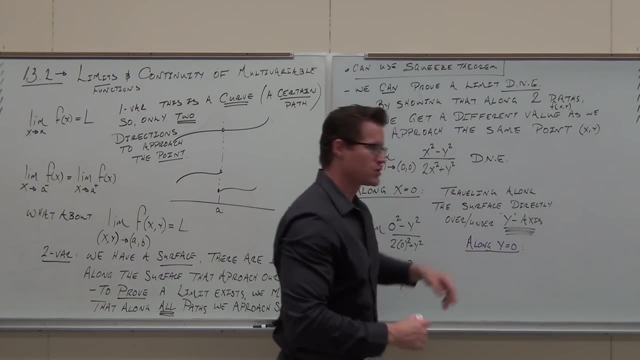 that these things don't match up On this graph, on this balloon, they would match up. This would not be good for us. I'll show you what to do in that situation. Just a minute. Did you at least let your y value go to 0?? 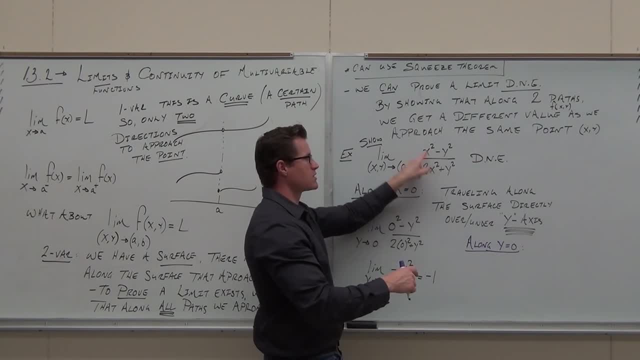 If you do, then this is 0,. this is 0. These are still x's, but since you let y equal 0, you're right above the x axis. The x axis is your only legitimate independent variable. left. You're saying: if I'm over the x axis, the x axis is only. 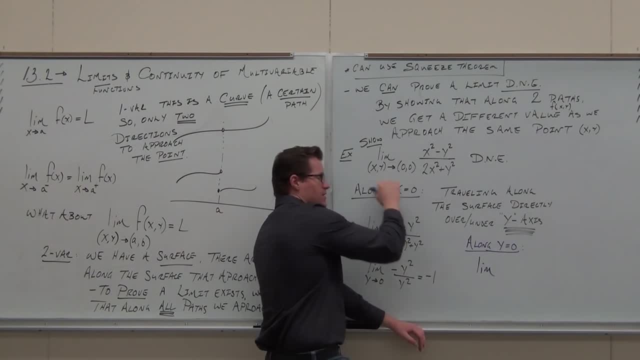 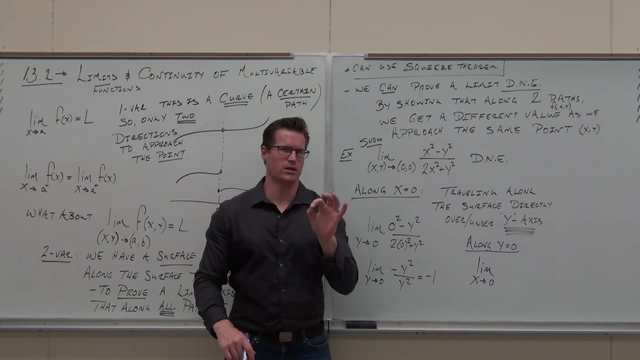 the x variable is the only thing that can change. So I don't have this anymore. I just let x approach. Do you see why x would still be approaching 0, though I still need to make it to that point, I've already taken y equals 0, so it's going to. 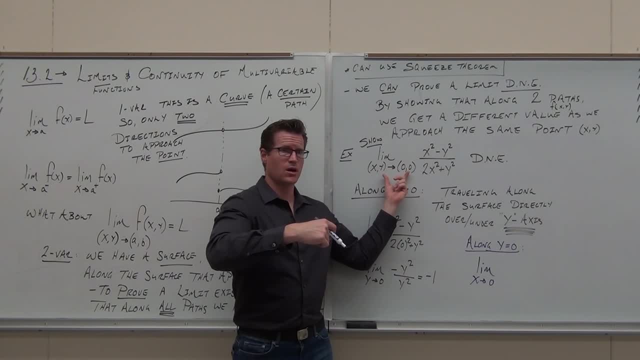 whatever path I do, it's going to make it through that y equals 0 value, but I also want x to go to 0 because I need to make it to 0, 0.. Those two ideas have to be kind of cohesive. 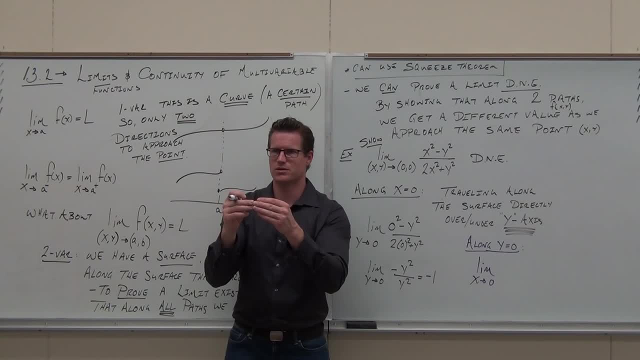 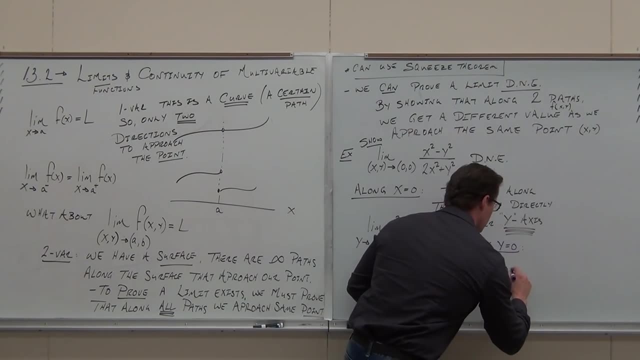 Does that make sense to you? I just did a whole lot of words and some of you are like: what are you going to do with that If you let y equal 0 already and change this all so it's only x squared minus 0, okay, done. 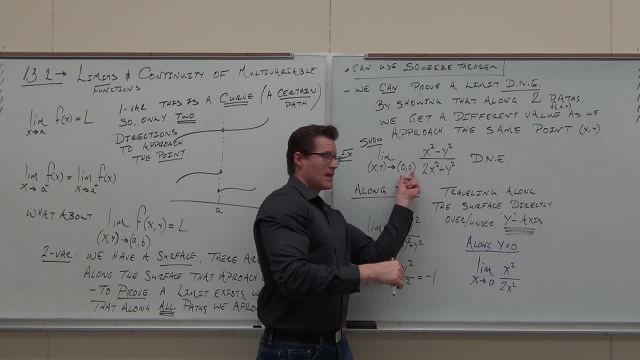 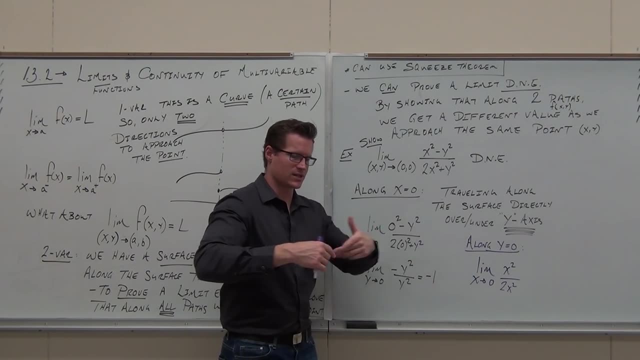 over 2x squared plus 0,. done, you're trying to get to that point. correct, You have to make it to that point. If y equals 0, I now need to say, okay, I know, my y is 0,. 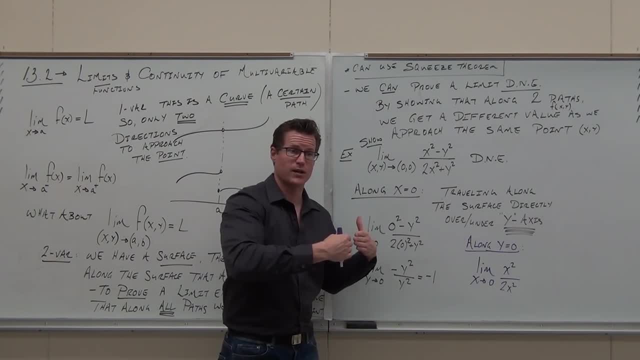 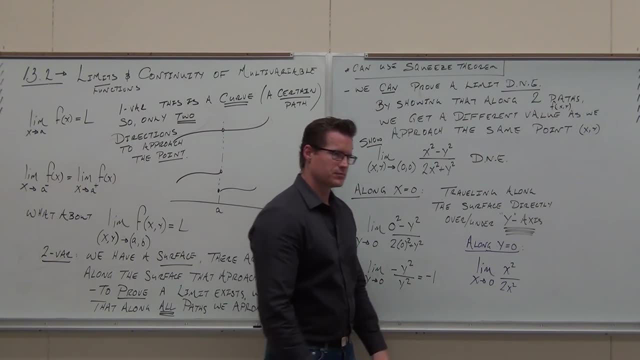 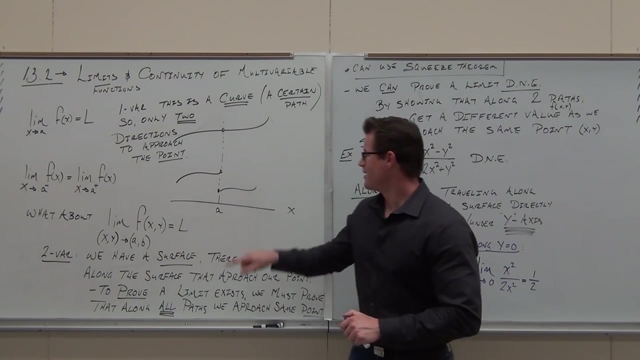 right over x. I need to let my x coordinate approach that 0 value so that I hit 0, 0.. Make sense, We should do it one at a time. How much is that? You have just shown this situation on a surface. 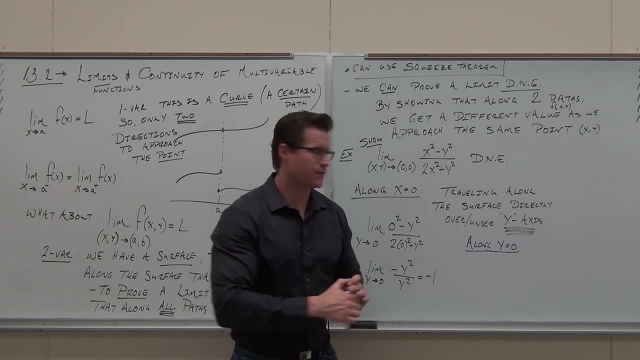 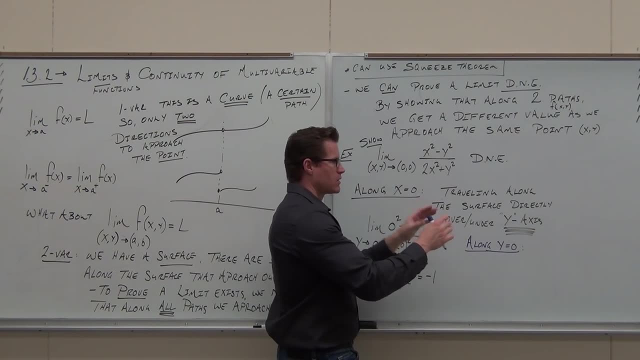 Did you at least let your y value go to 0?? If you do, then this is 0,, this is 0.. These are still x's, but since you let y equal 0,, you're right above the x-axis. 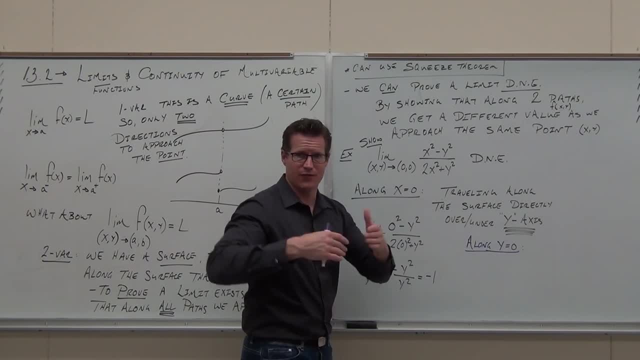 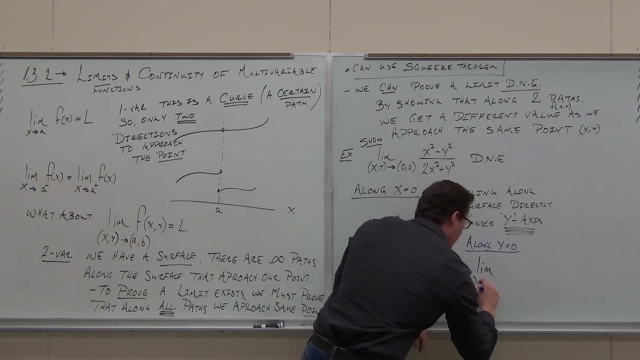 The x-axis is your only legitimate independent variable left. You're saying: if I'm over the x-axis, the x-axis is only the x variable. The x variable is the only thing that can change. so I don't have this anymore. 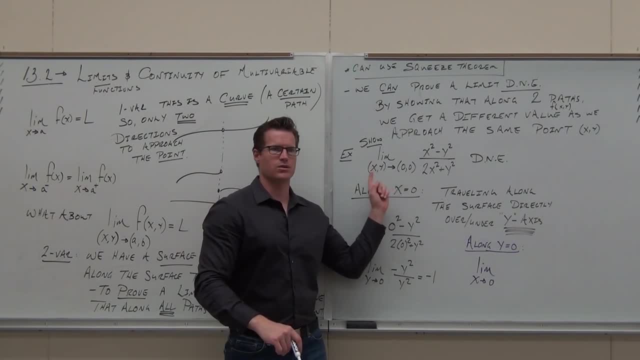 I just let x approach. Do you see why x would still be approaching 0,? though I still need to make it to that point, I've already taken y equals 0, so whatever path I do, it's going to make it through that y equals 0 value. 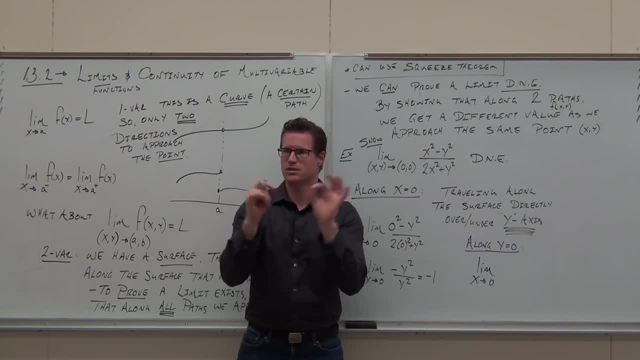 but I also want x to go to 0, because I need to make it to 0, 0. Those two ideas have to be kind of cohesive. Does that make sense to you? I just did a whole lot of words and some of you are like what? 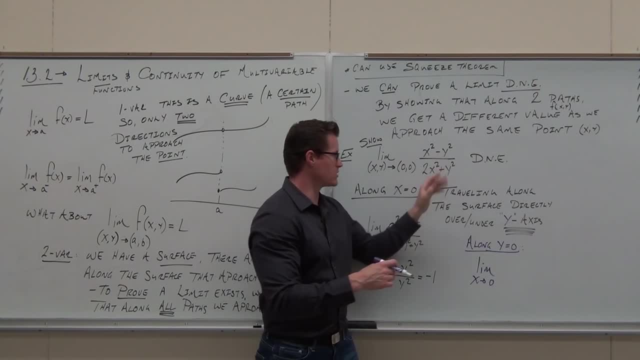 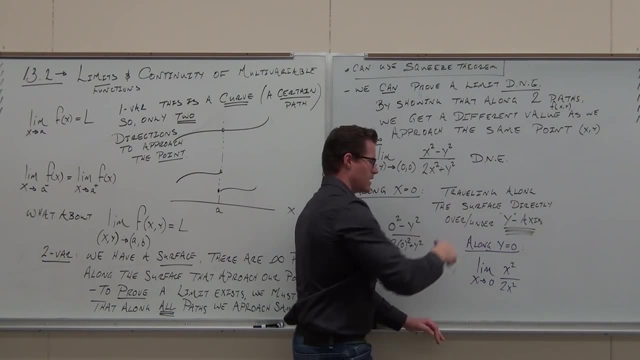 If you let y equal 0 already and change this all so it's only x squared minus 0, okay, done, over 2x squared plus 0, done, You're trying to get to that point, correct, You have to make it to that point. 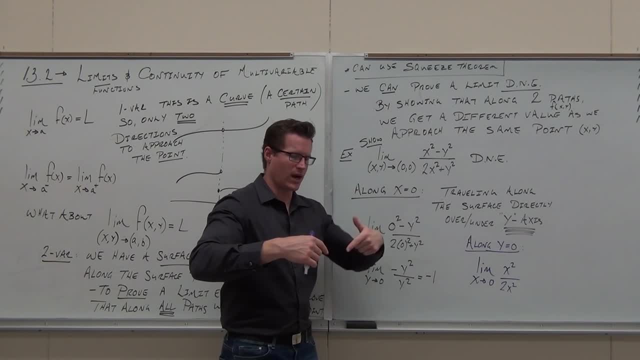 If y equals 0, I now need to say, okay, I know my y is 0 right over the x. I need to let my x coordinate approach that 0 value so that I hit 0, 0. Make sense. 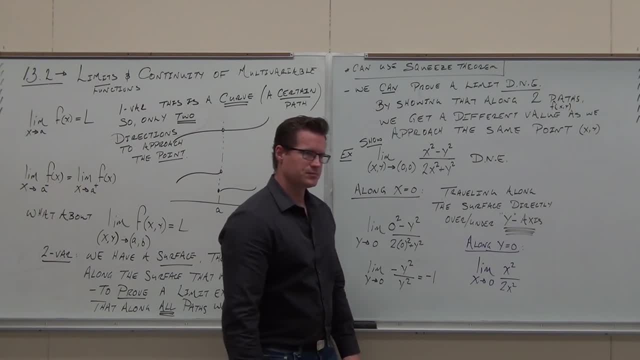 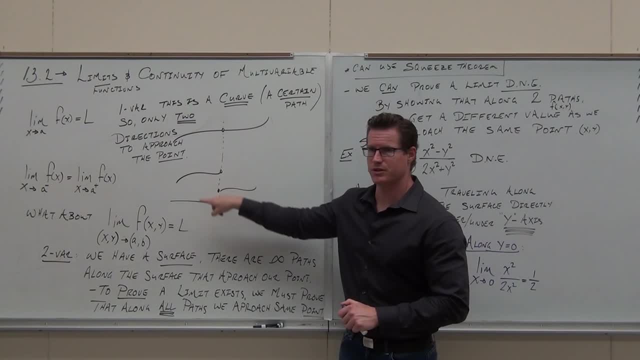 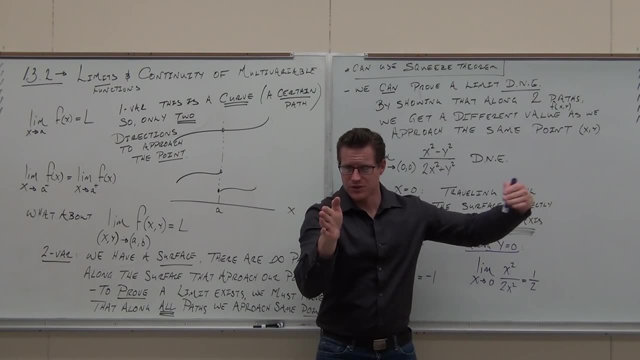 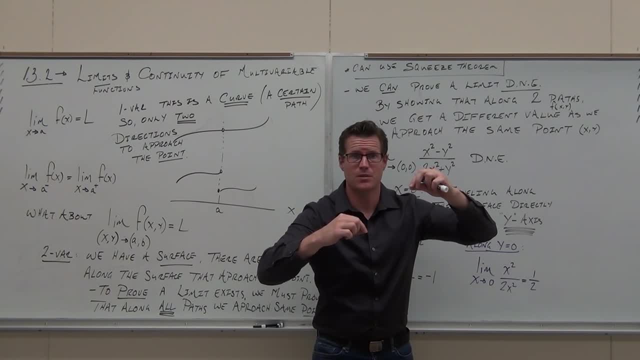 you're getting two different heights. There's infinite paths, but I just need to show along the surface, along two curves, two paths, that I get different heights at one point, just above one point, and that's exactly what I've done. 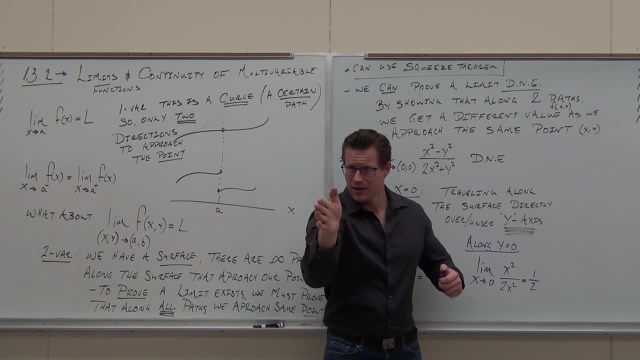 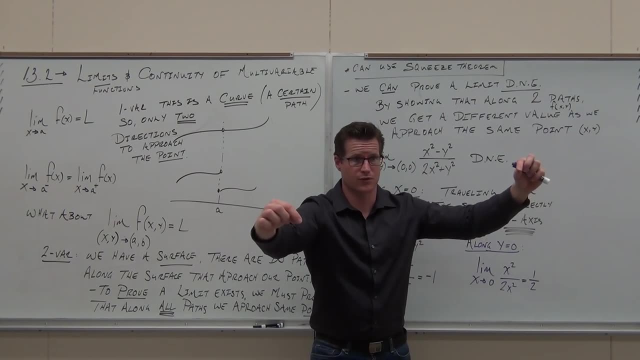 It's practically the same. It's just that from this way and from this way, you're getting two different heights. There's infinite paths, but as you can show along the surface, along two curves, two paths, that I get different heights at one point, just above one point. 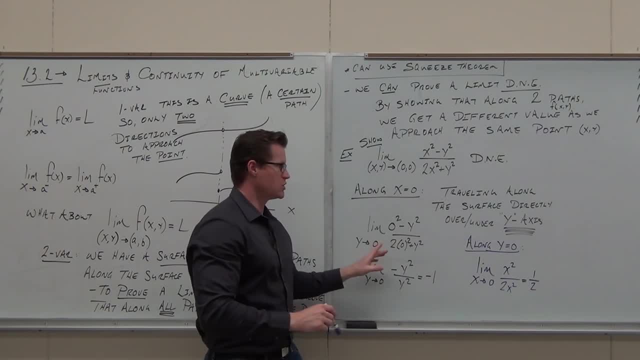 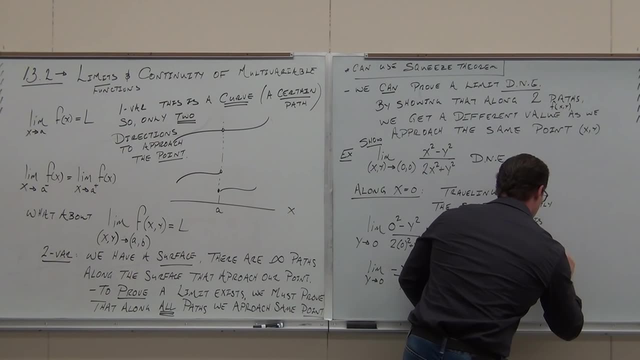 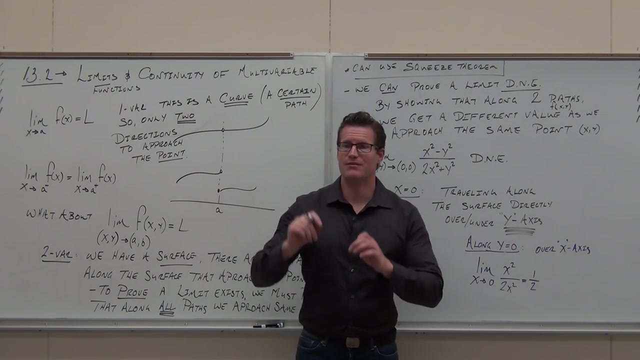 And that's exactly what I've done. So by showing that along two paths- what paths? Right over the y axis, right over the x axis, Along those two paths, I have a different value for my surface and that says the limit does not exist, because along all paths, 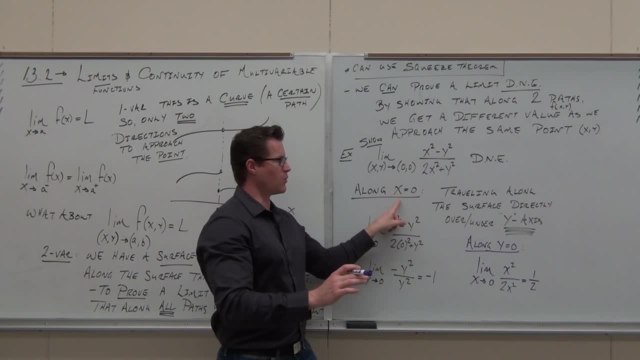 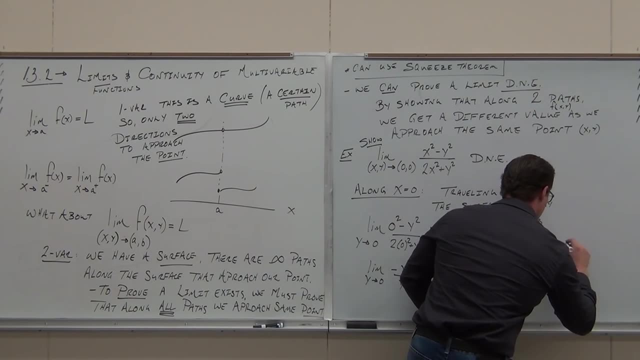 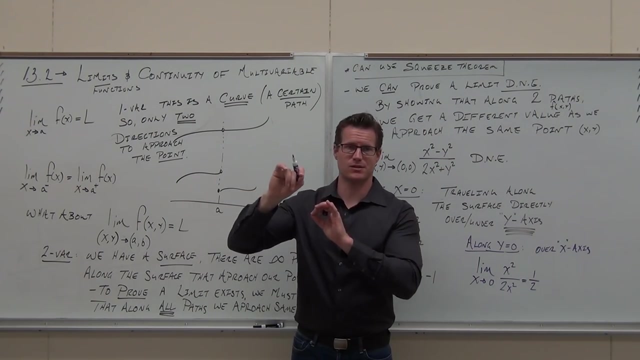 So by showing that Along two paths, What paths? Right over the y-axis, right over the x-axis, Along those two paths, I have a different value for my surface and that says the limit does not exist, because along all paths. 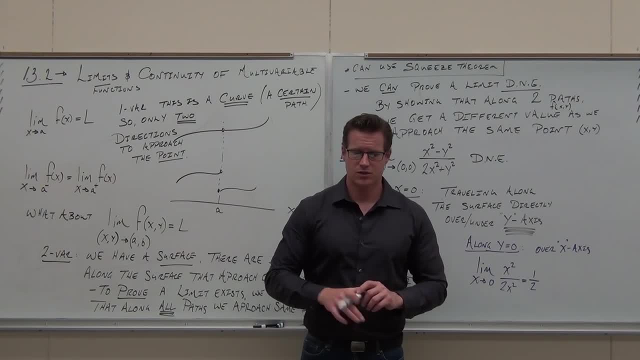 we have to come to the same value for our function, the same value for our surface. So it has to be okay with that. So we'll wrap this up here. Say you showed it in your test, You say hey, negative 1.. 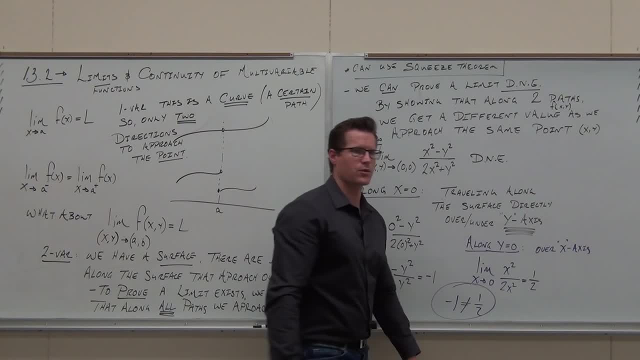 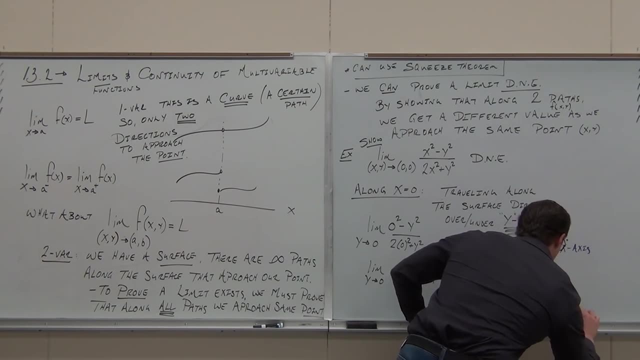 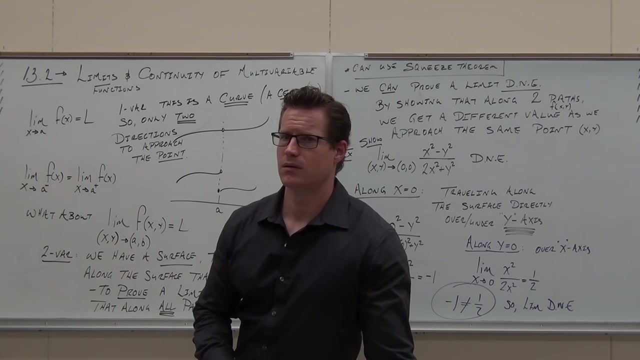 Negative 1 does not equal 1 half. Therefore the limit does not exist. Please be very careful on your verbiage here. The limit doesn't exist. at what point? Zero, zero, Zero, zero. At the input: zero zero. 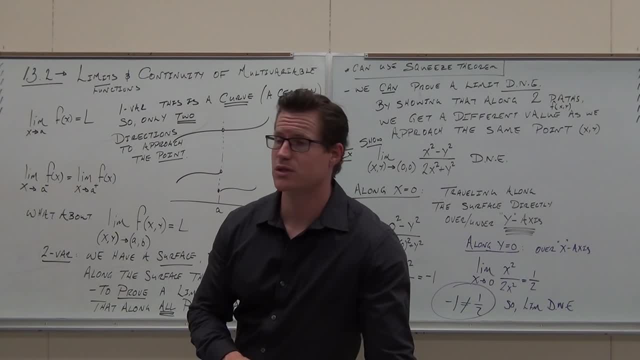 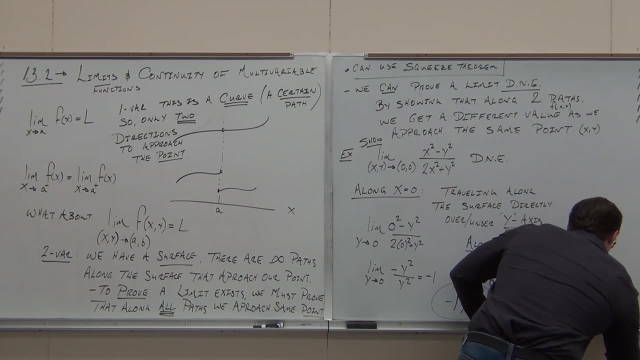 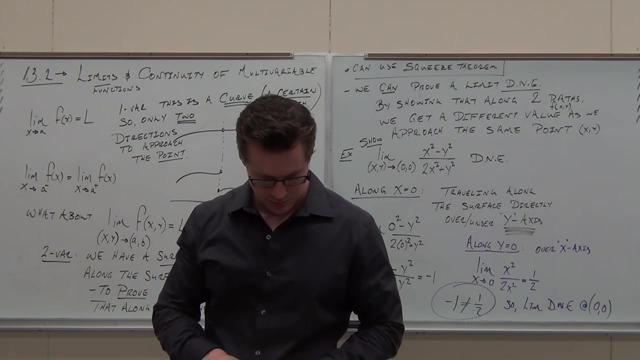 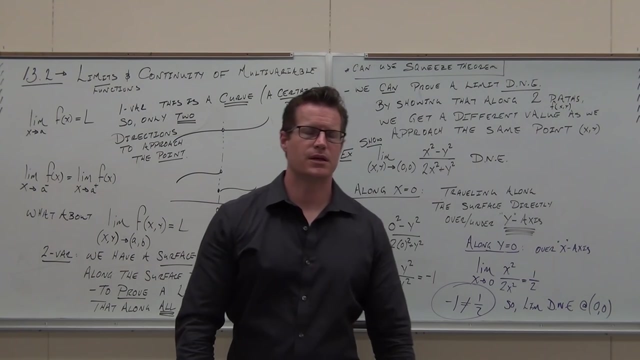 Other points? sure it's going to exist Most other points. Can I give you a couple hints that's going to really help you out? Here's the quickest, easiest, simplest way to do limits or to show the limits don't exist. 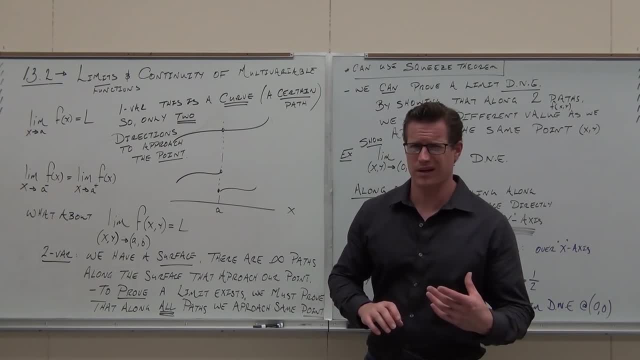 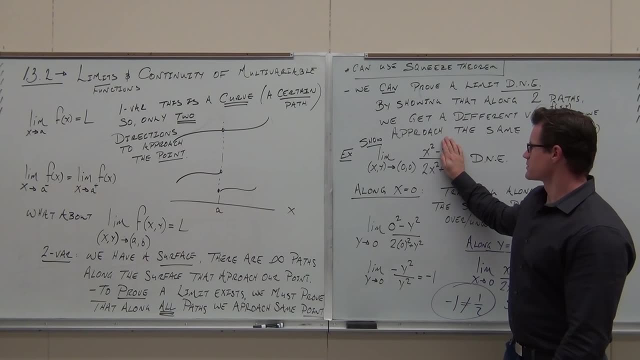 But you've got to listen carefully, because I'm not going to write a whole. I'll write a couple things out, but not a lot. Check it out. Ready, Ready Cover if you're wise. Ready Cover if you're wise. 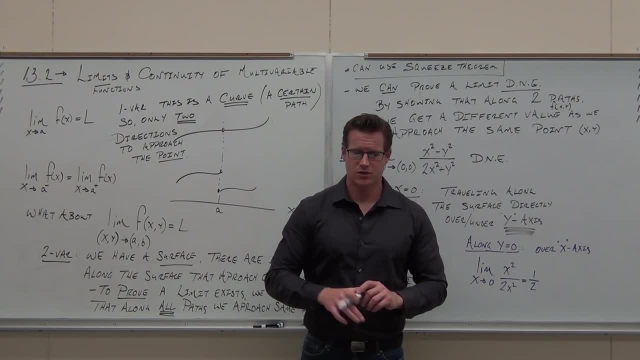 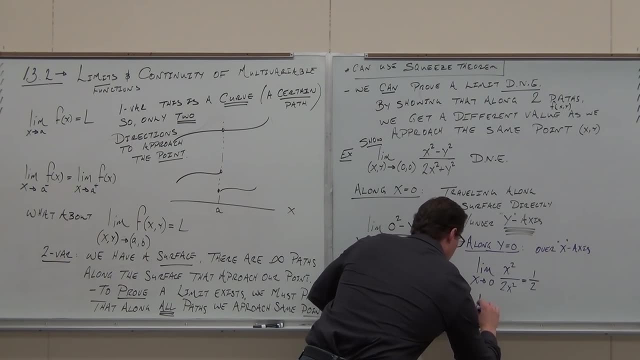 we have to come to the same value for our function, the same value for our surface. So it has to be okay with that. So we'll wrap this up here. So you showed in your test you say, hey, negative 1 does not equal 1 half. 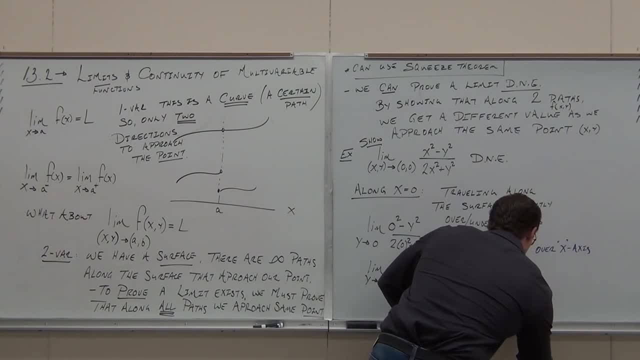 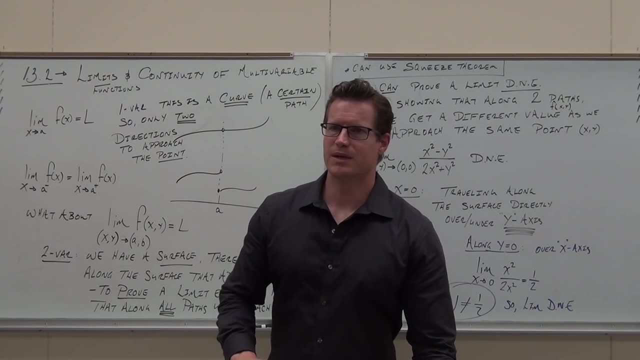 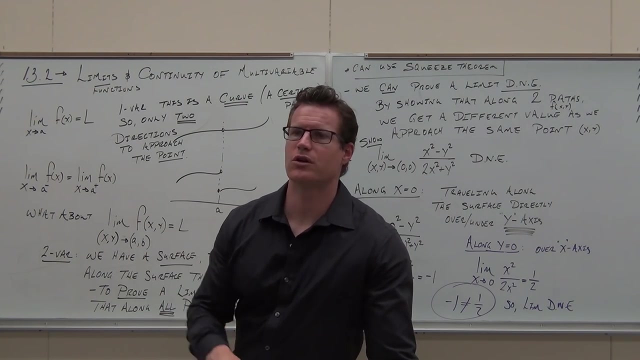 Therefore the limit does not exist. Okay, Please be very careful on your verbiage here. The limit doesn't exist. at what point? Zero, zero, Zero, zero. at the input: zero, zero. Other points: sure it's going to exist most other points. 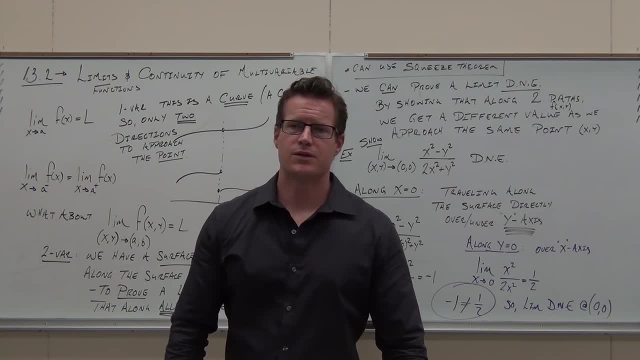 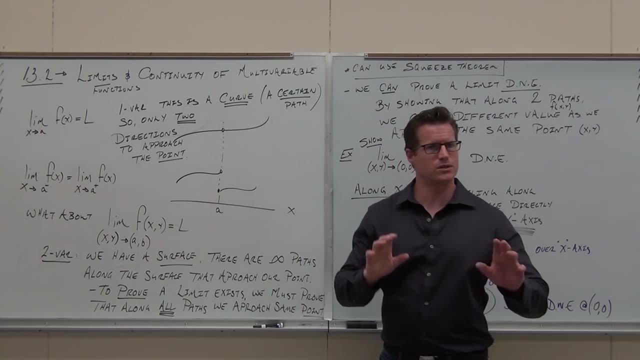 Can I give you a couple hints That's going to really help you out. Here's the quickest, easiest, simplest way to do limits or to show that limits don't exist. But you've got to listen carefully, because I'm not going to write a whole 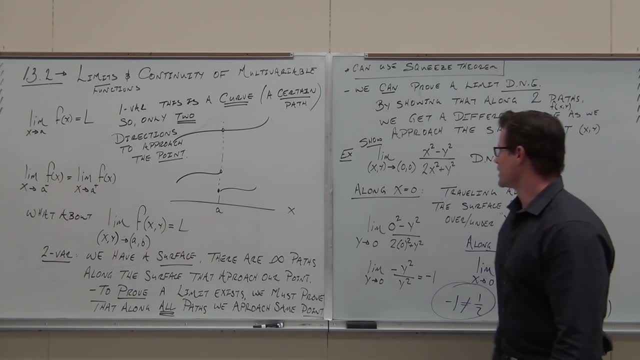 I'll write a couple things out, but not a lot. Check it out: Ready, Ready. Cover up your y's, do the limit in your head. you get 1 half. You see it. Cover up your x's, do the limit in your head. 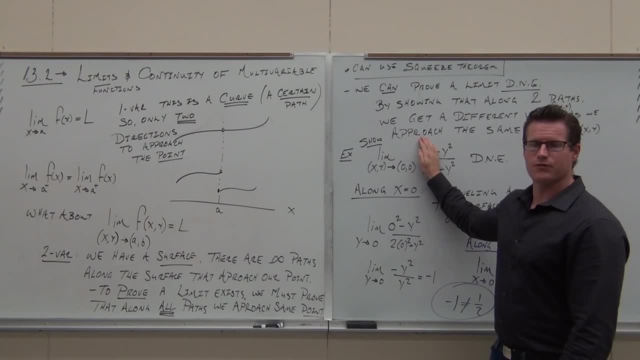 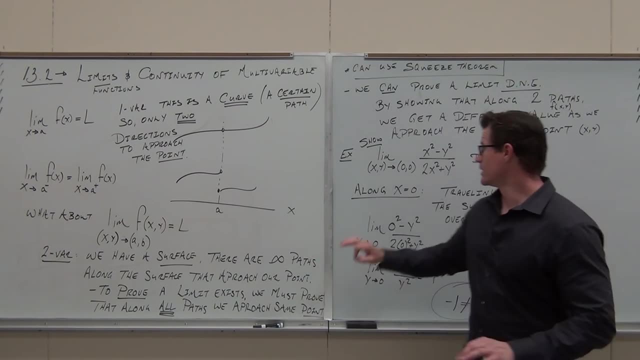 you get negative 1.. Did you catch that? If those numbers are different, go along: x equals 0 and y equals 0, done, Because that's exactly what we did. We left the y equals 0, 1 half. we left the x equals 0, negative 1,. 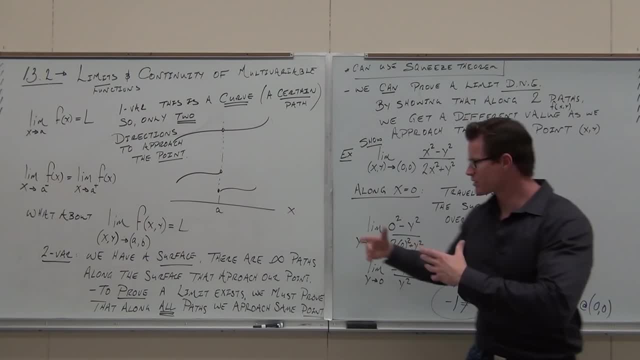 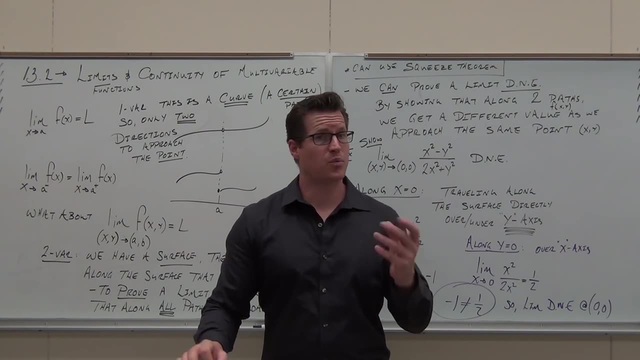 different values, different height done, Just go, just show your work. go along: x equals 0,, y equals 0, and you're done. Does that make sense to you? That's the easiest way to go about it. The problem is what happens when we go along: x equals 0. 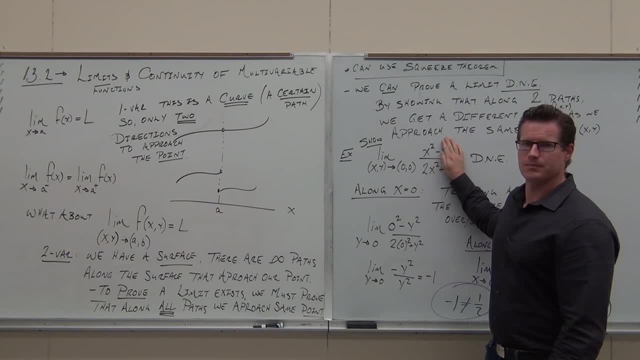 Do the limit in your head, You get 1, half. You see it Cover. if your x's Do the limit in your head, You get negative 1.. Did you catch that? If those numbers are different, go along. x equals 0. 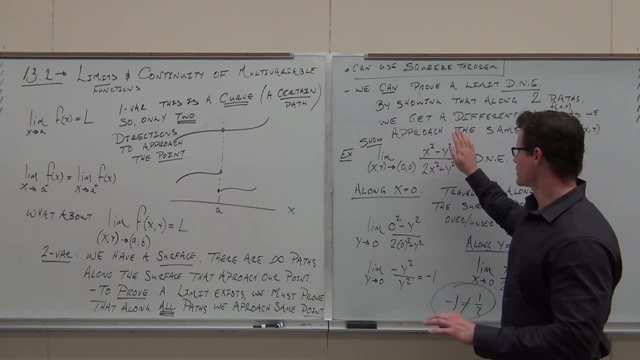 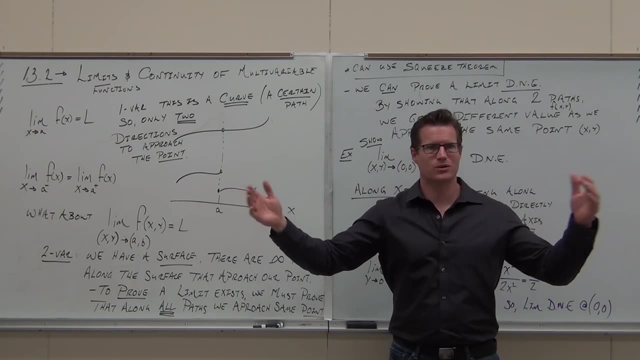 and y equals 0, done, because that's exactly what we did. We let the y equals 0, 1 half. We let the x equals 0, negative 1.. Different values, different height: done, Just go, just show your work. 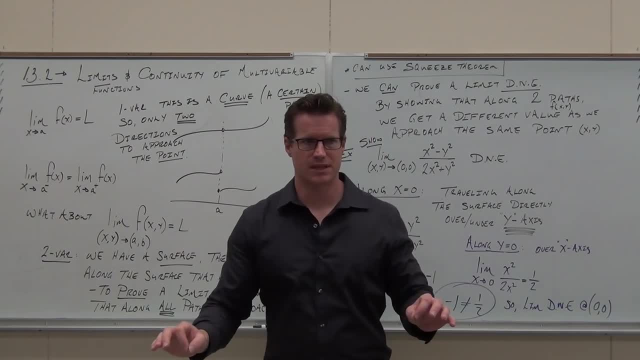 Go along: x equals 0,, y equals 0, and you're done. Does that make sense to you? That's easy. That's the easiest way to go about it. The problem is what happens when we go along: x equals 0. 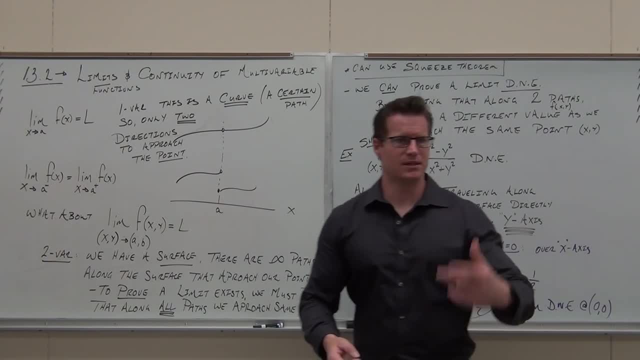 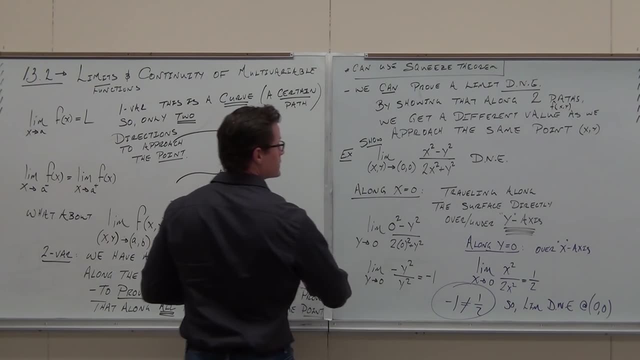 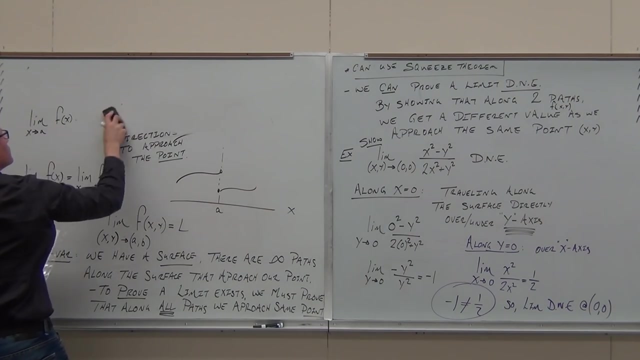 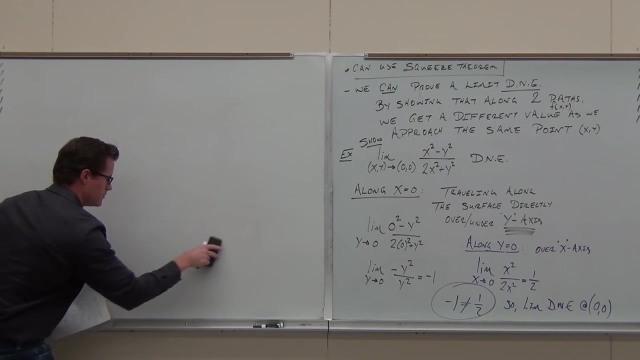 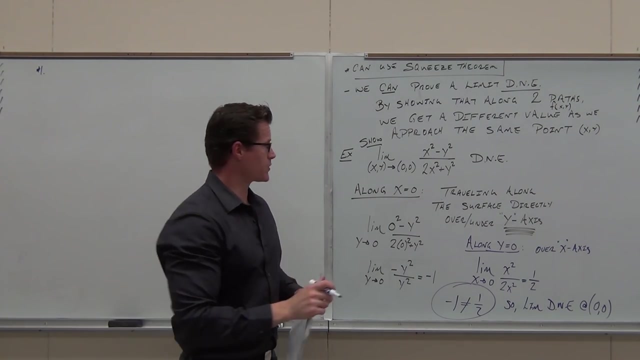 and y equals 0, and we get the same value still, And that's the nature of the next couple questions that we have. So a few notes, Let me continue. So number 1. Try: x equals 0 and y equals 0. first in your head. 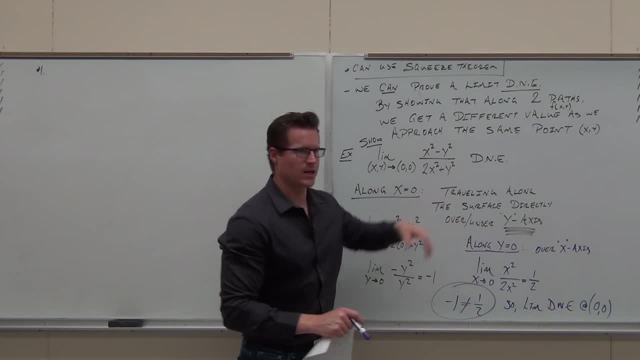 Don't even write them out yet, Just in your head. just cover up the variables and see if you get different numbers. If you do, then only x equals 0, y equals 0, that's it. That's all you got to do. 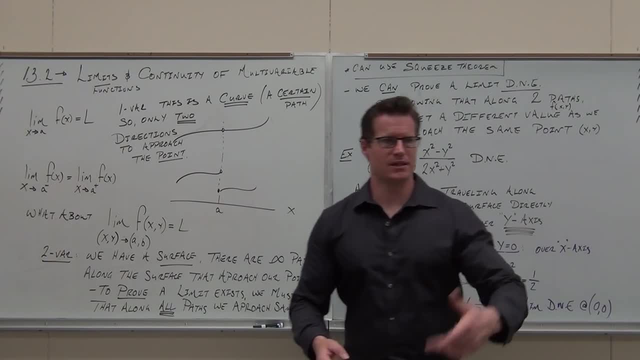 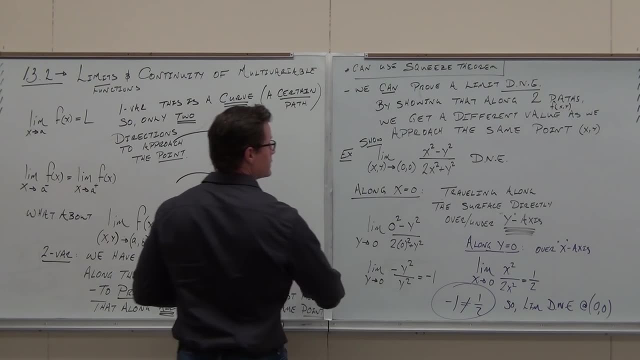 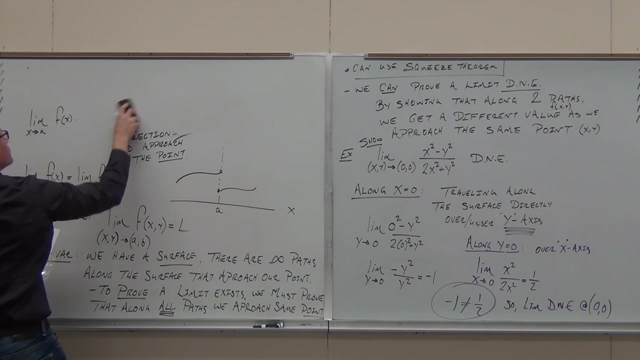 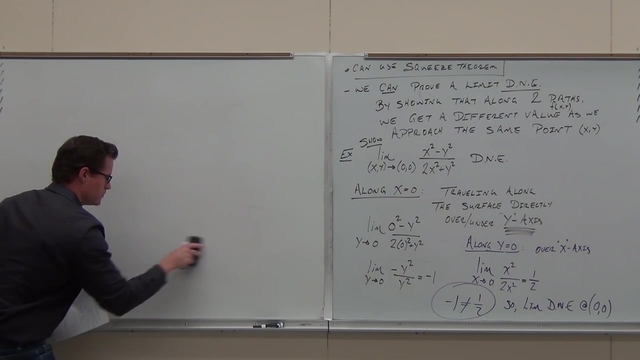 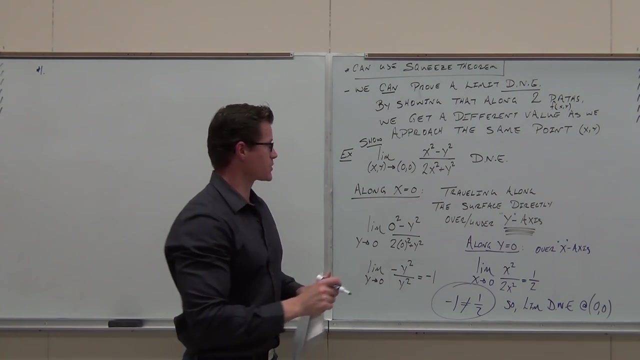 and y equals 0, and we get the same value still, And that's the nature of the next couple questions that we have. So a few notes, Let me continue. So, number one, try: x equals 0 and y equals 0. first in your head. 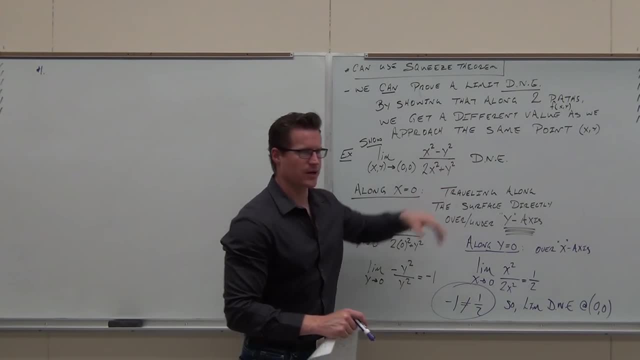 Don't even write them out yet, Just in your head. just cover up the variables and see if you get different numbers. If you do, then only x equals 0, y equals 0. That's it. That's all you got to do. 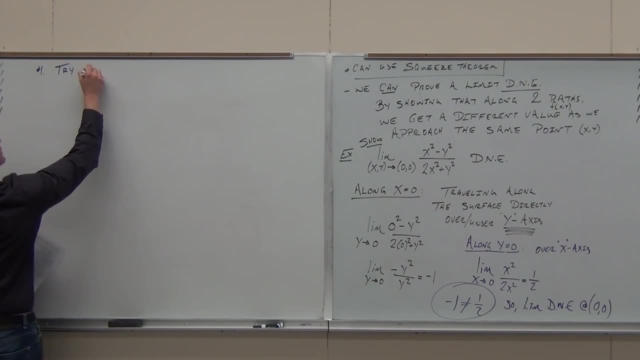 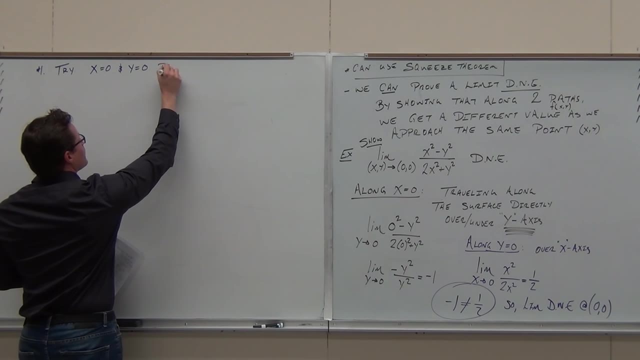 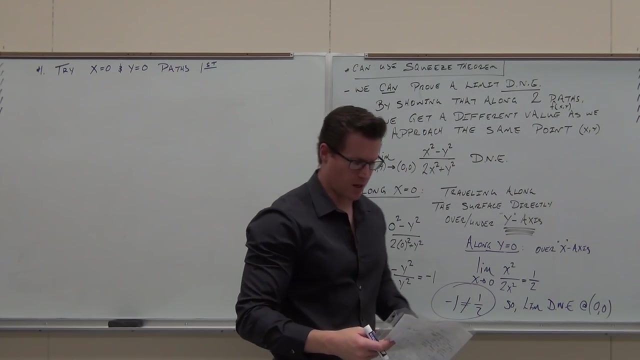 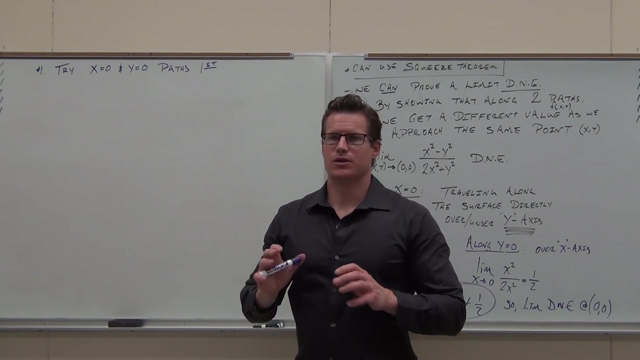 So try These paths first. The reason why is because you can do them in your head very, very fast. that's why Listen carefully. This is not going to work all the time. If it doesn't work, so that means you do. x equals 0. 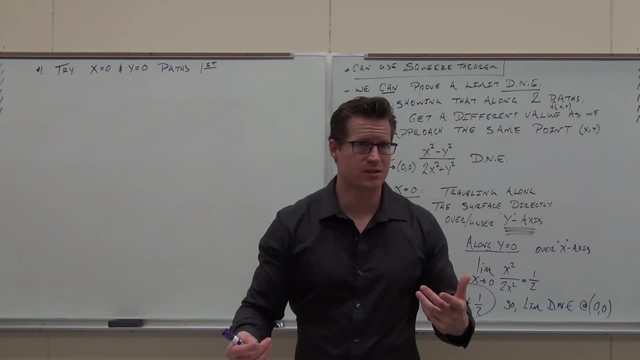 and y equals 0 and you get the same value still. Have you proved something exists? Have you proved something doesn't exist? No, That's the worst case scenario. Then you go okay. well, what do I do now? Try another path, but always use at least. 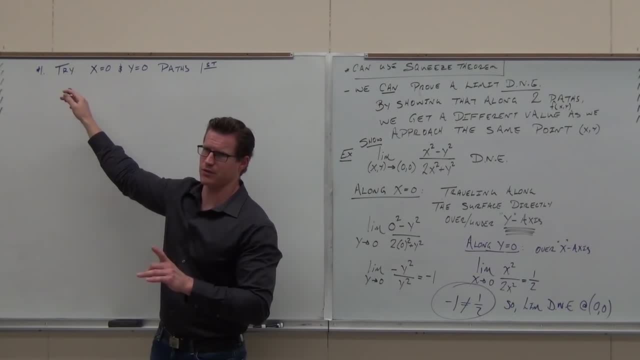 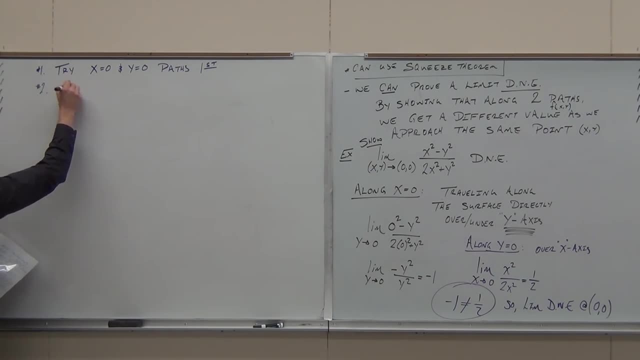 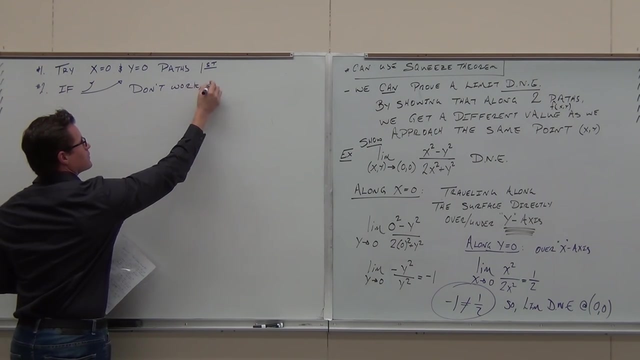 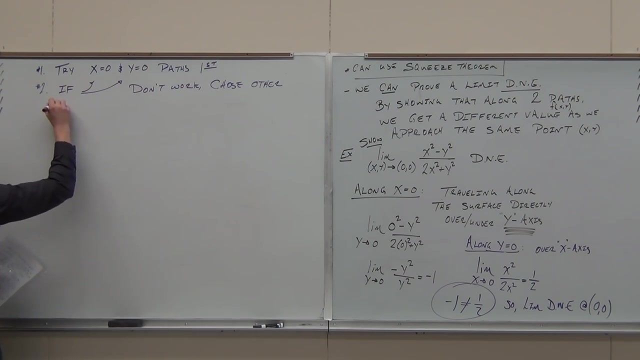 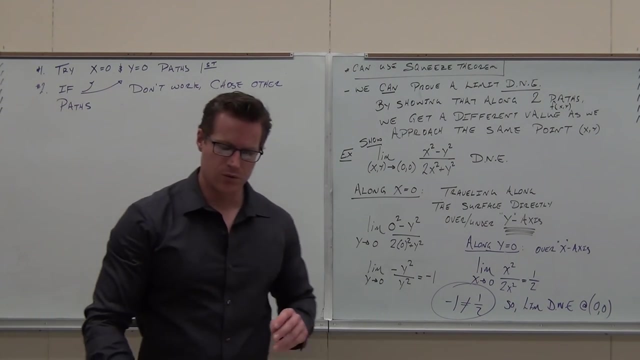 always use one of these to do one path, okay, So always use one of those. If these don't work, Choose other paths. A few notes here. There's a couple that I want you to know that are really going to help you. 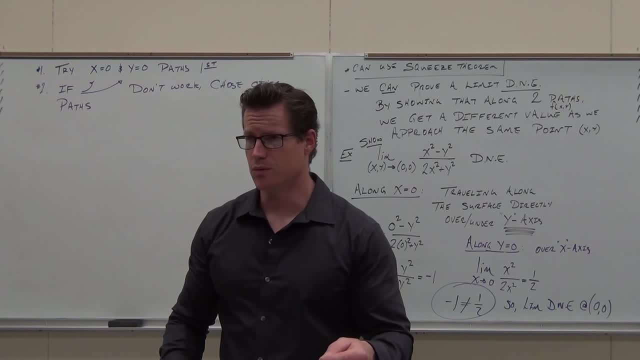 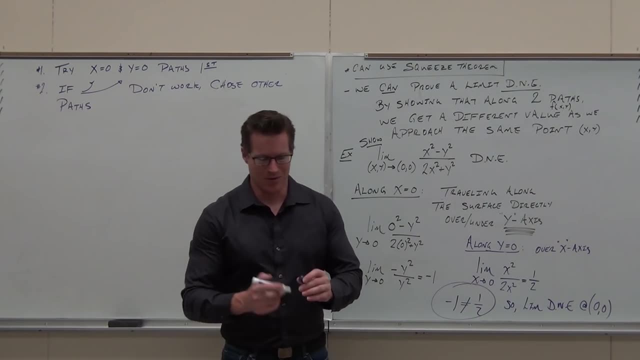 Number one: whatever path you choose must contain that point. That has to be the case. Play with it, Go okay. I want a path. I want to check the limit at 0, 0, so let's go through 5, 2.. 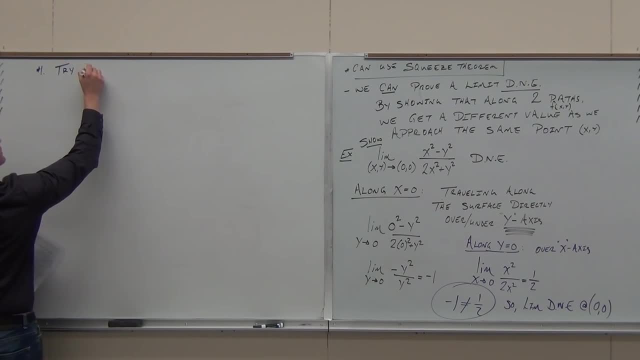 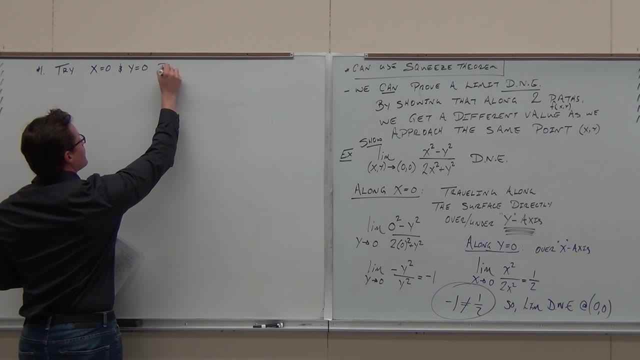 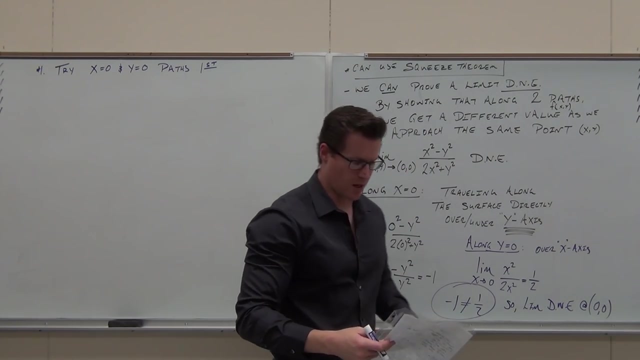 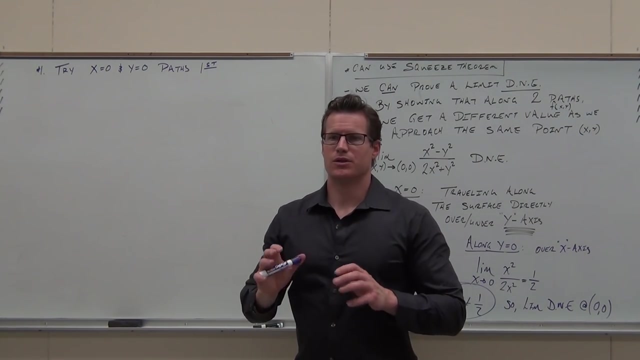 So try these paths first. The reason why is because you can do them in your head very, very fast. That's why Listen carefully. This is not going to work all the time. If it doesn't work, so that means you do. x equals 0. 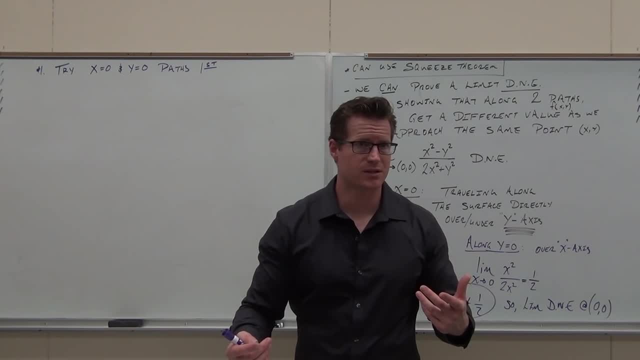 and y equals 0,. you get the same value still. Have you proved something exists? Have you proved something doesn't exist? No, That's the worst Okay Scenario. Then you go, okay, well, what do I do now? 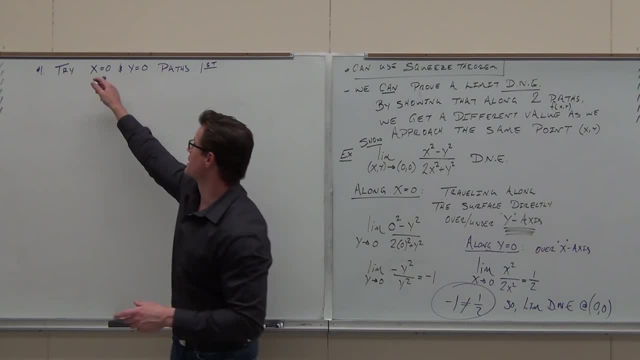 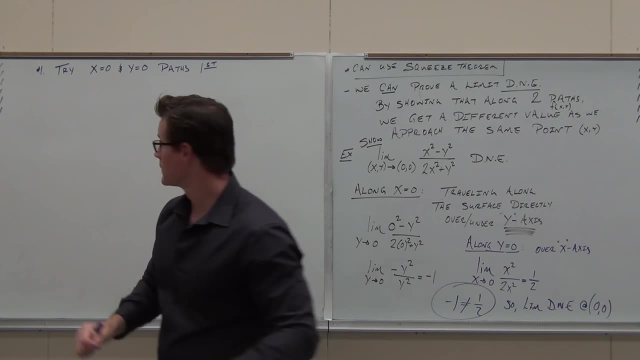 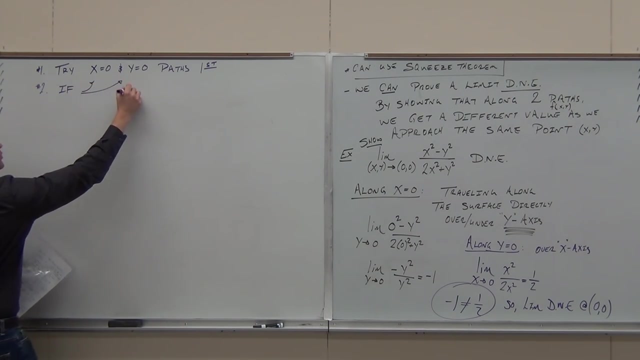 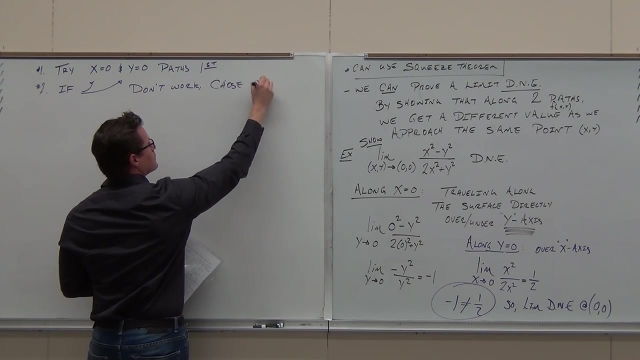 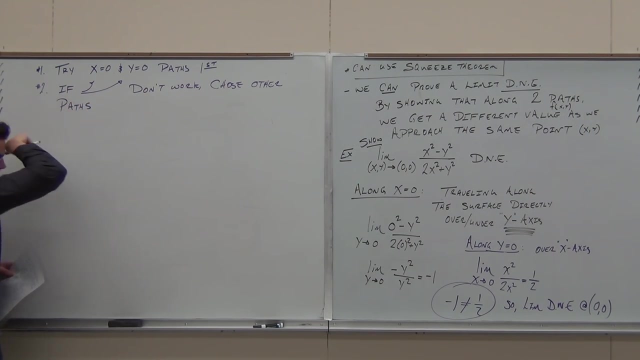 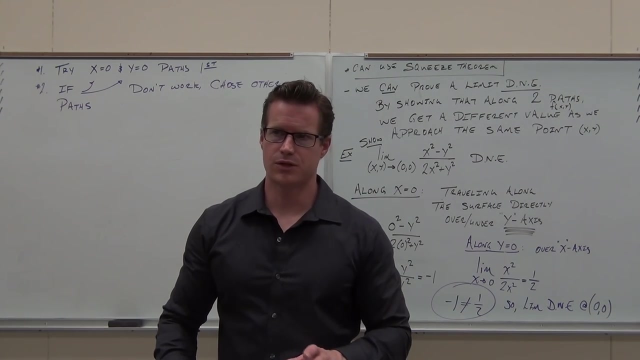 Try another path, but always use- at least always use- one of these to do one path. okay, So always use one of those. If these don't work, Choose other. A few notes here. There's a couple that I want you to know. 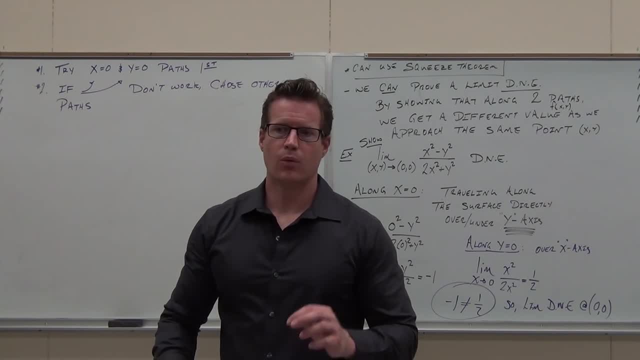 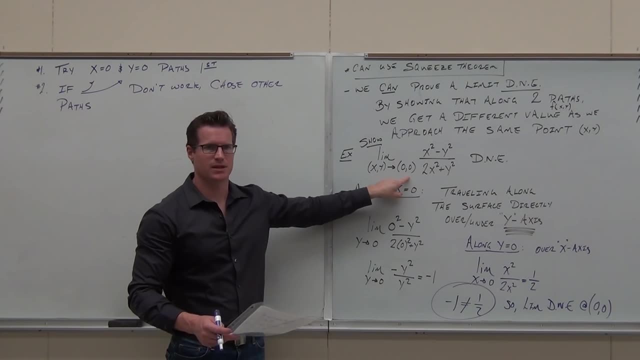 that are really going to help you. Number one: whatever path you choose must contain that point. That has to be the case. Play with it, Go. okay. I want to check the limit at 0, 0.. So let's go through 5, 2.. 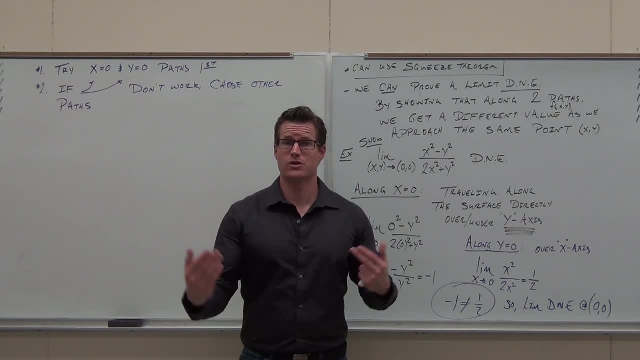 Yeah, Does that make sense? No, You want to make sure that path actually contains that point. So, number one thing: make sure the path you're choosing contains that point. Does x equals 0 at some point contain 0, 0?? 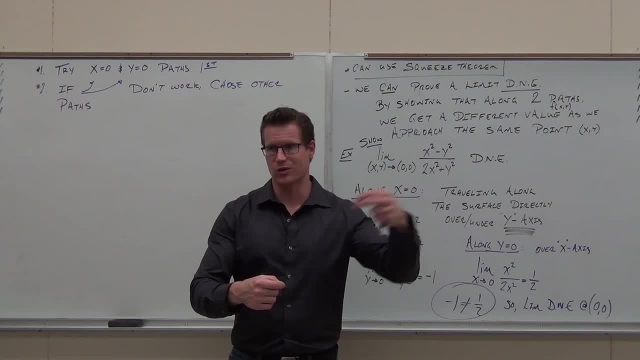 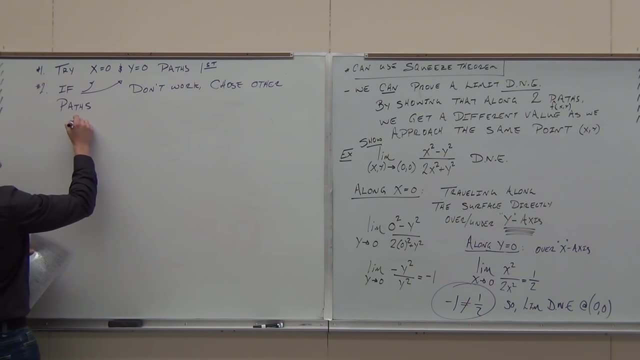 Yeah, When x is 0 and then when y becomes 0. That's why you got to go along y, okay. So make sure that happens for any substitution you make, any path you choose, But if you're not able to do that, then it's going to take you a long time. 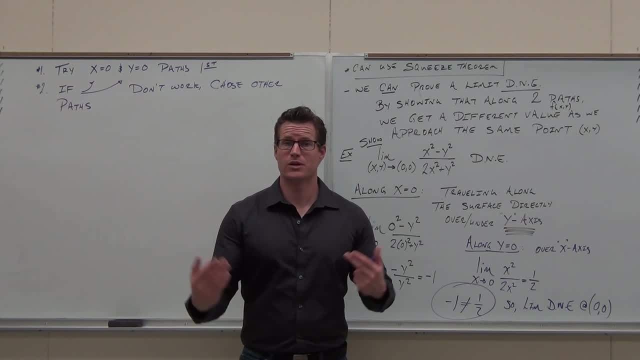 Yeah, Does that make sense? No, You want to make sure that path actually contains that point. So, number one thing: make sure the path you're choosing contains that point. Does x equals 0 at some point contain 0, 0?? 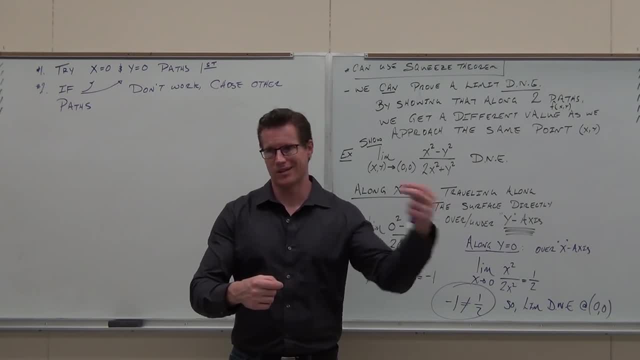 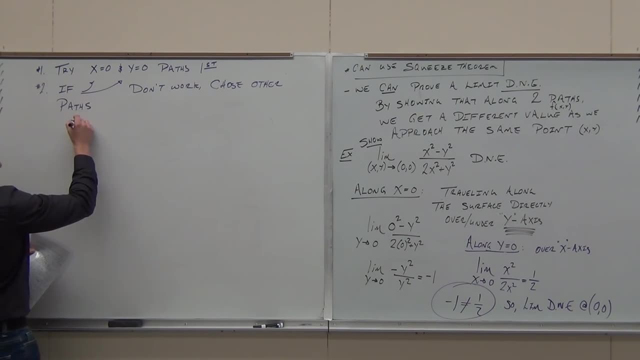 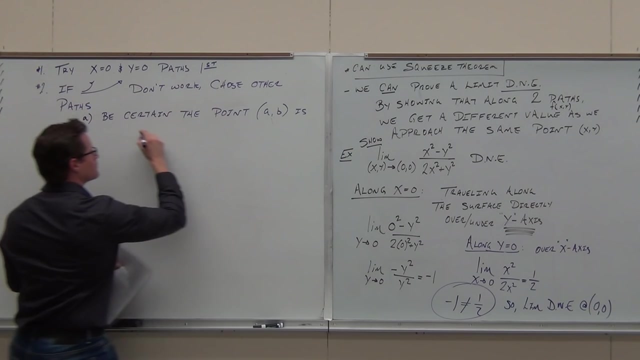 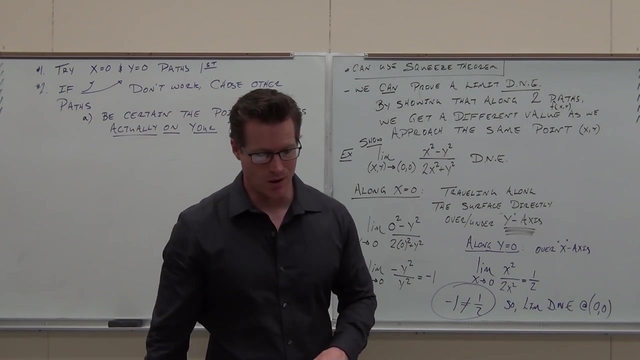 Yeah, When x is 0 and then when y becomes 0. That's why you got to go along y, okay. So make sure that happens for any substitution you make, any path you choose, Be certain your point is actually on your path. 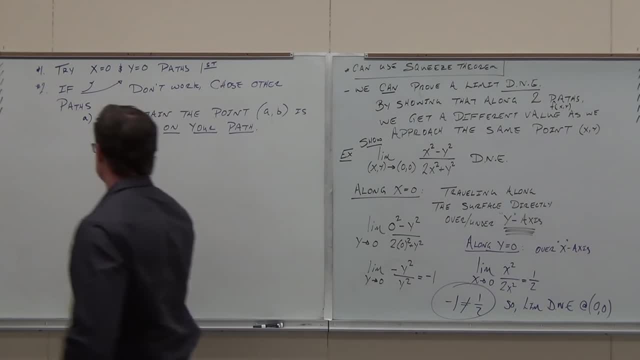 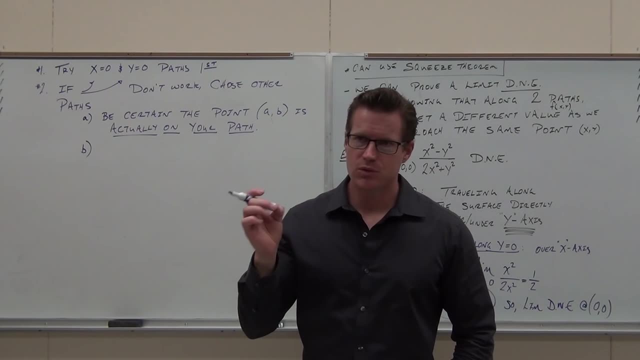 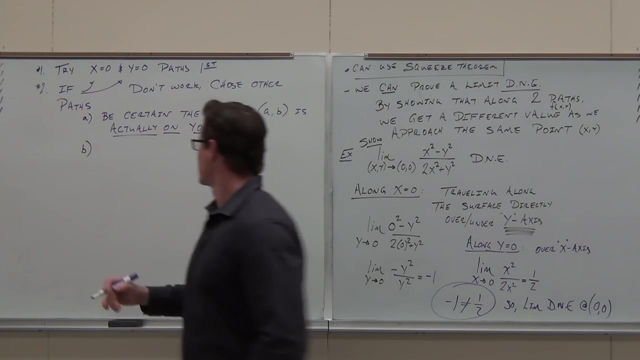 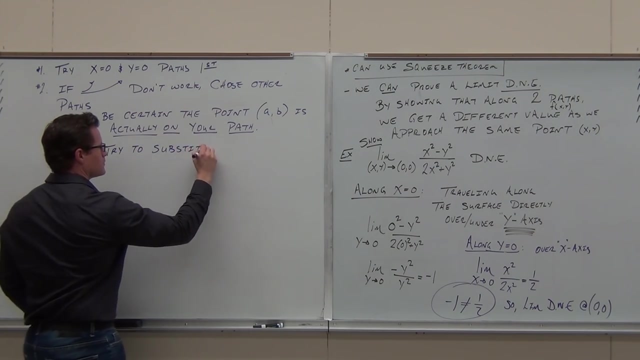 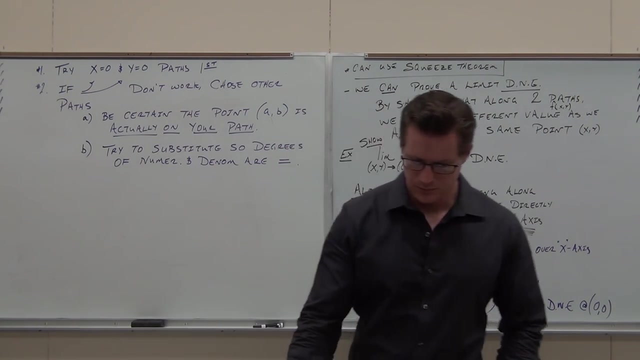 Second, Make sure your point is actually on your path. Second, Make sure your point is actually on your path. Second, When you're doing this, it often helps to substitute so that the degrees on your numerator and denominator become the same. So make sure you can do this with any answer. 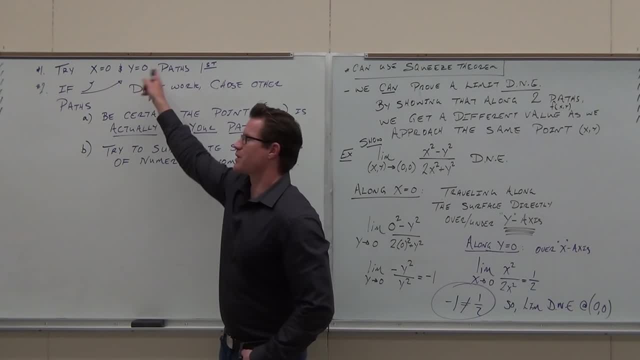 And thirdly, for one of your paths, always choose one of these. Always choose one of those because it's the easiest one. we can do so. always pick one of those if you can. Almost 90 percent time you can, Okay. 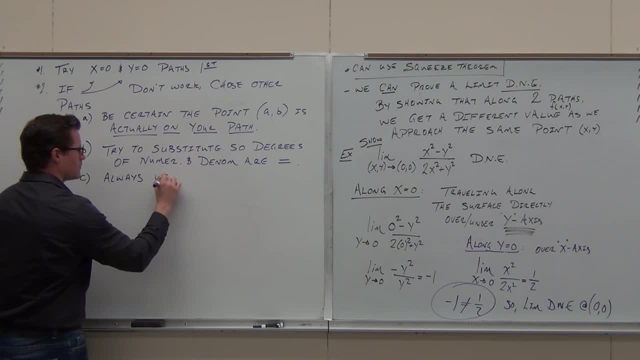 Go ahead, All right. When you're doing this, when you're doing this, make sure your point is zero, and then, when you're doing it, make sure that every point is zero. So make sure you don't make the right choice. 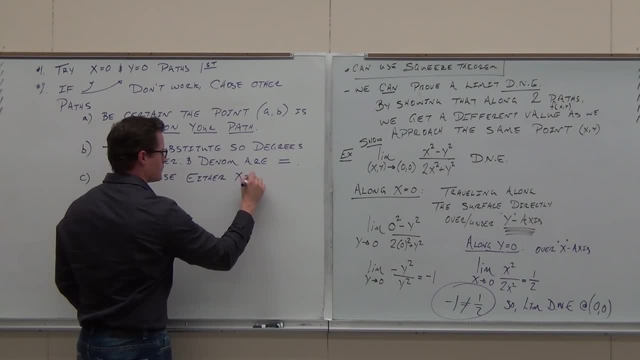 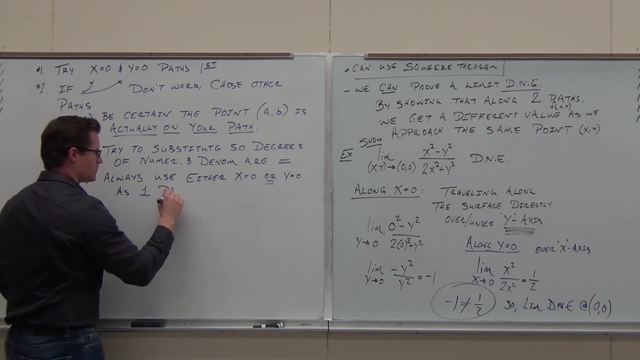 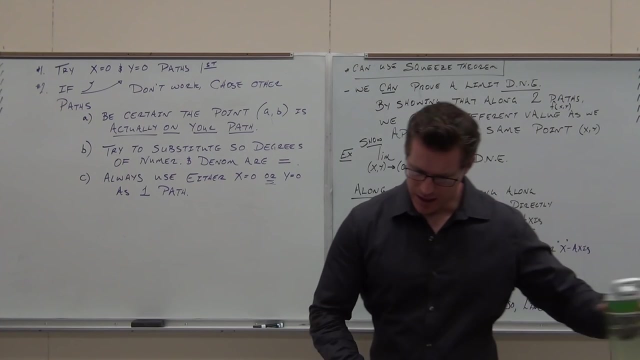 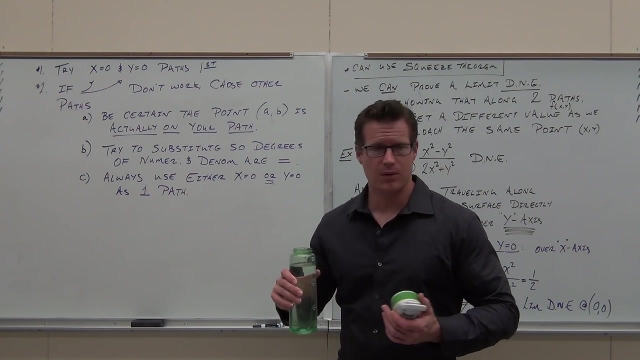 Okay, It generally does not matter which one you do. I would like to try just three examples. We'll talk about having more than two variables. We'll go to three variables. After that we'll talk about continuity, and that wraps this section up. 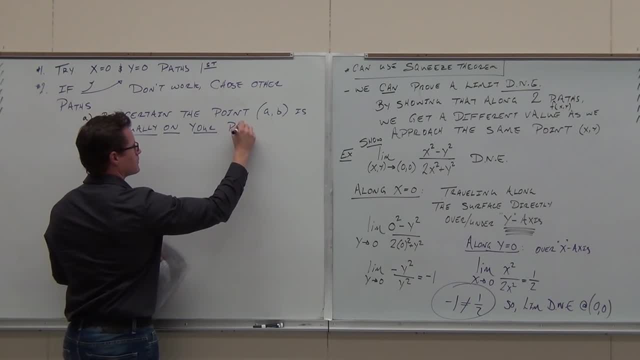 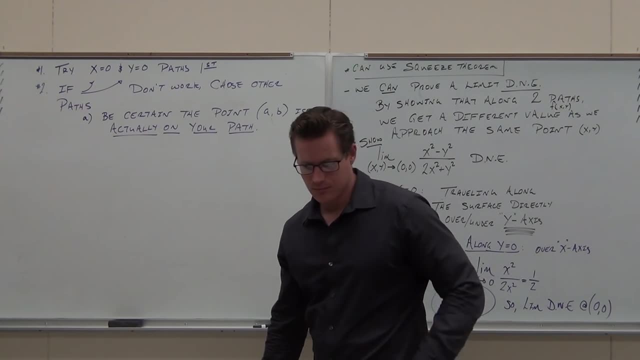 So remember, we're not just going to specify the path. it's going to take you some time. Our point is actually on your path. Okay, That's going to be the case for this long path. Let's go to number two. 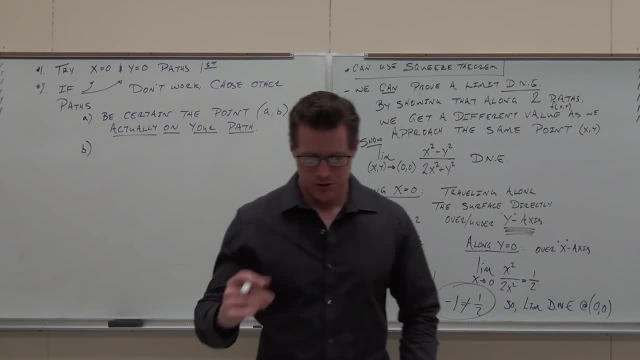 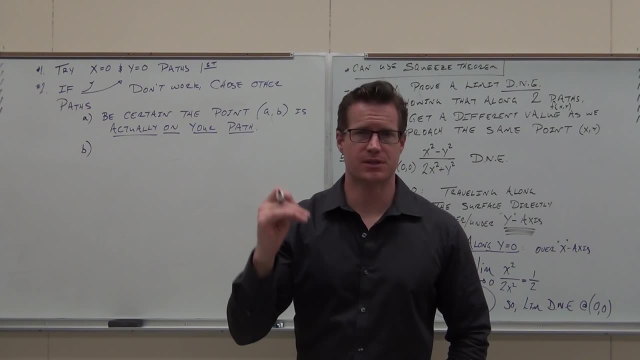 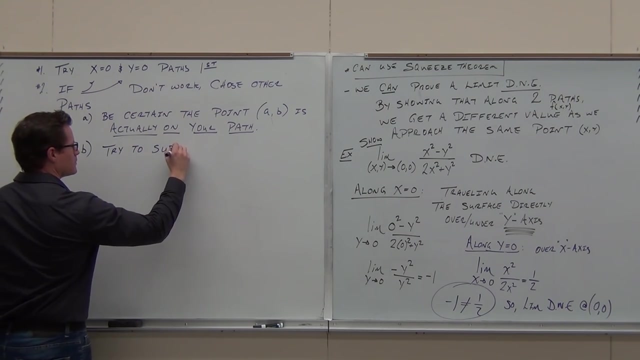 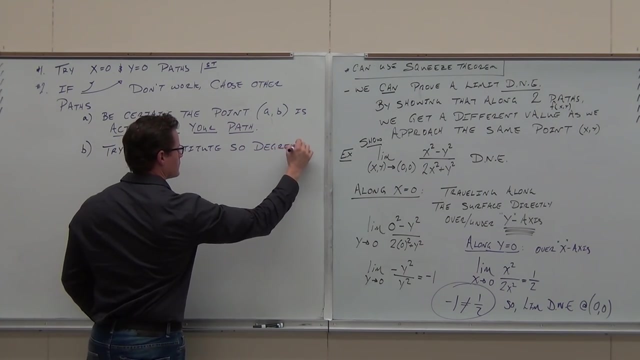 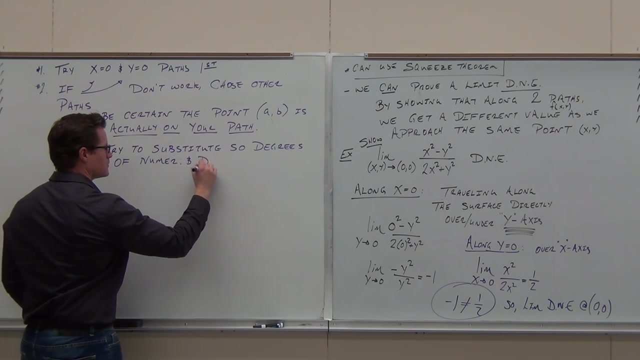 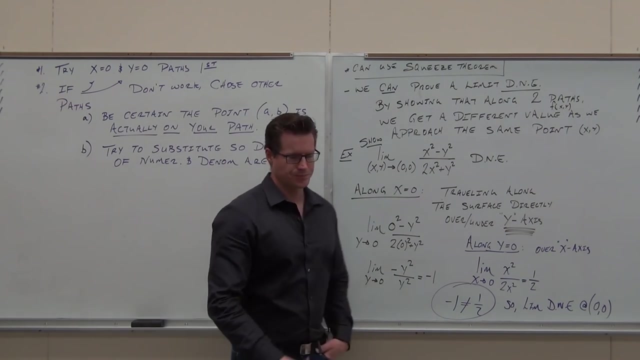 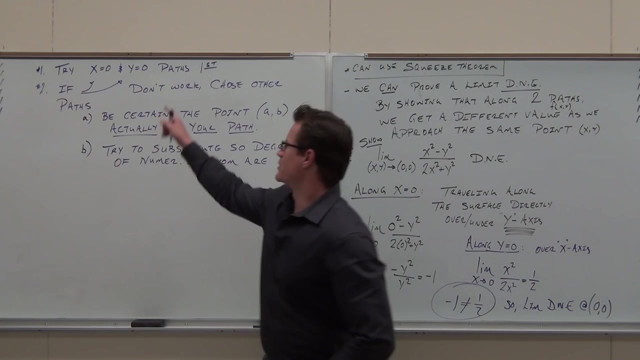 Number two: be certain your point is actually on your path. it often helps to substitute so that the degrees on your numerator and denominator become the same. And thirdly, for one of your paths, always choose one of these. always choose one of those because it's the easiest. 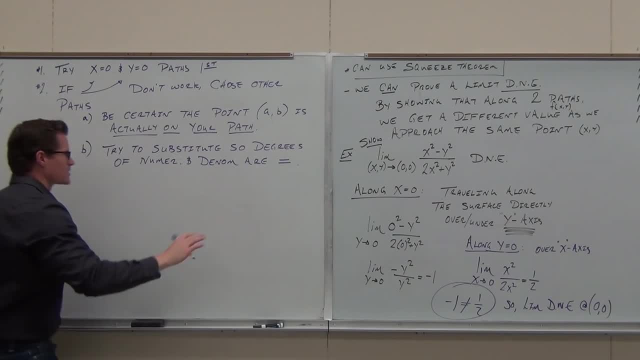 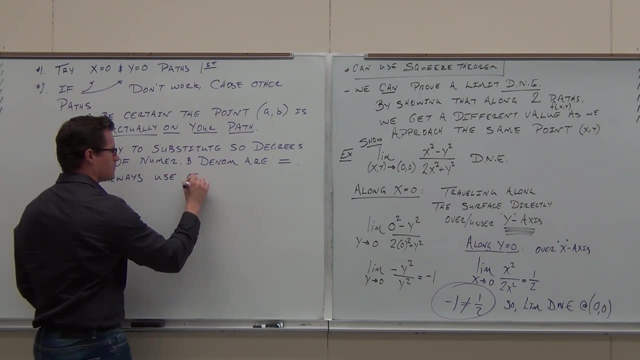 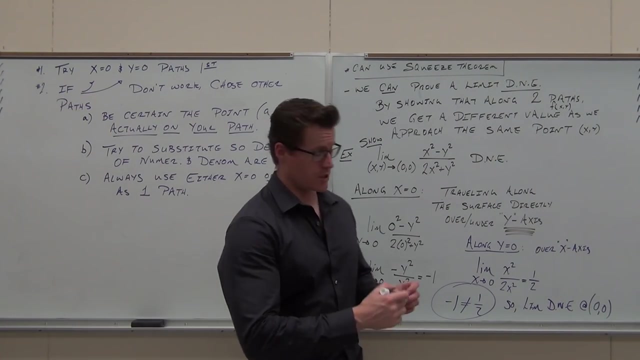 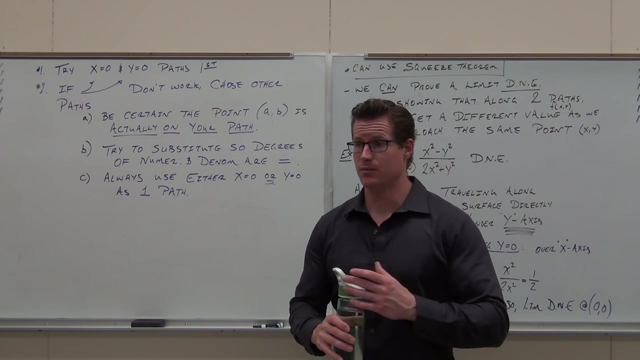 one we can do so. always pick one of those if you can. Almost 99% of the time you can, It generally does not matter which one you do. I would like to try just three examples. We'll talk about having more than two variables. we'll go to: 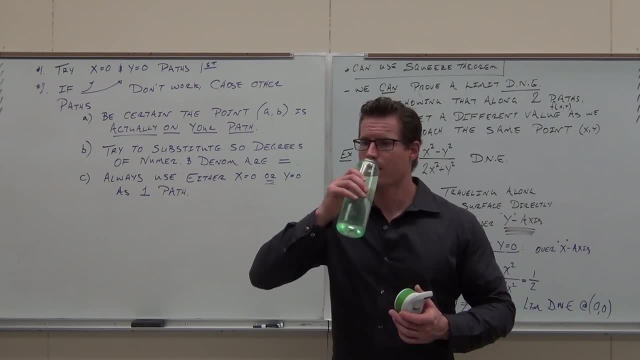 three variables. After that we'll talk about continuity and that wraps this section up. Sounds like only a little bit. It's going to take us a little while because I want to fully explain this Again. limits: as you know from Calc 1, right limits are one. 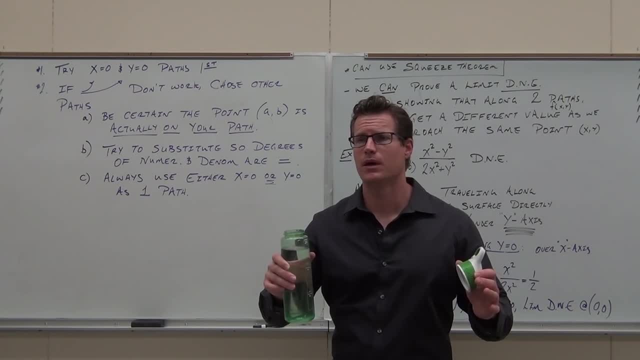 of the fallbacks for people, They go. I hate limits Why? Because they don't understand them. I want to make sure you actually understand this. Do you understand so far what we've been doing for real? Don't just nod your head and go: yeah, I get it. 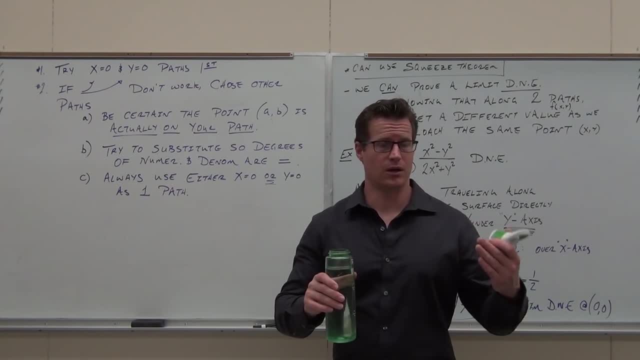 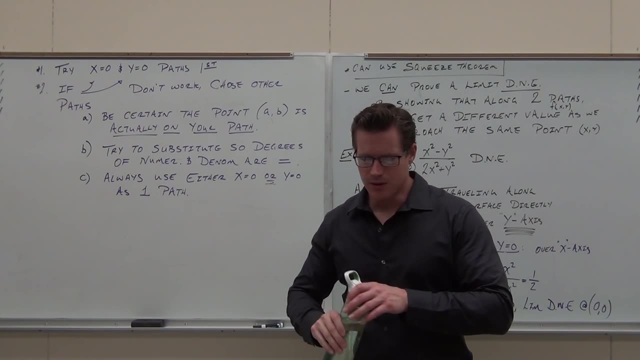 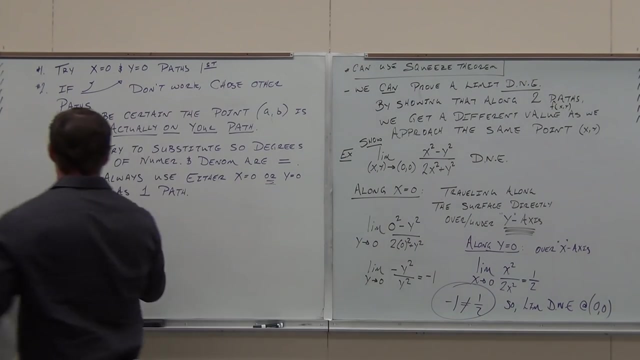 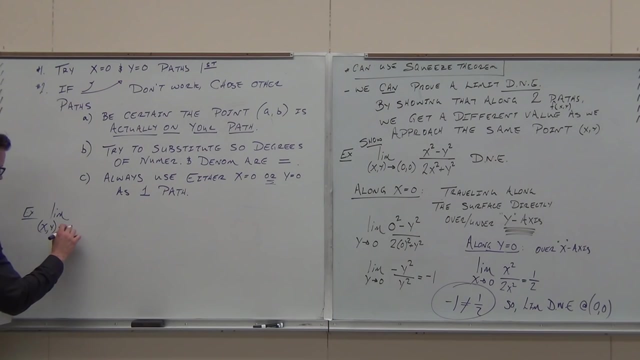 Do you actually get the idea of what we're doing? Yes, The over the surface, sorry, along the surface, over a particular path. you guys get that Okay, So let's try this. Let's do the limit Here. 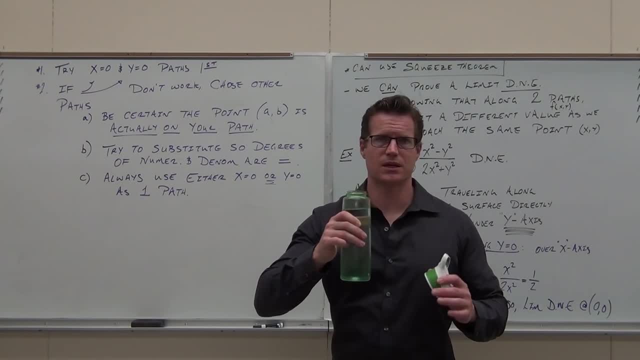 Sounds like only a little bit. It's going to take us a little while because I want to fully explain this Again. limits: as you know from Calc 1, right limits were one of the fallbacks. for people They go. I hate limits. 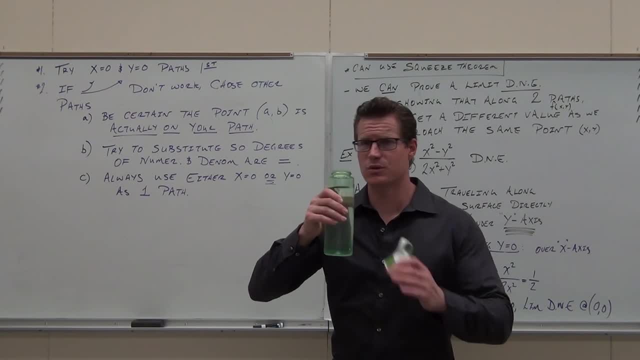 Why? Because I don't understand them. I want to make sure you actually understand this. Do you understand so far what we've been doing for real? Don't just nod your head and go: yeah, I get it. Do you actually get the idea of what we're doing? 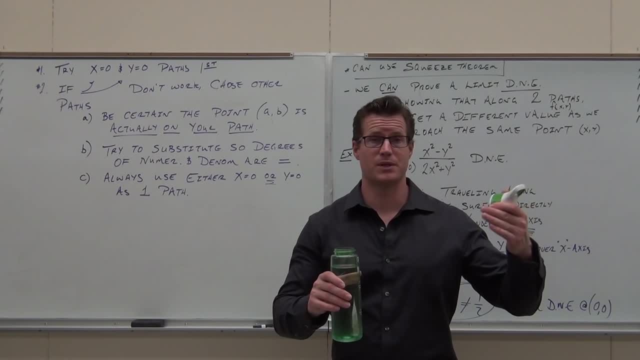 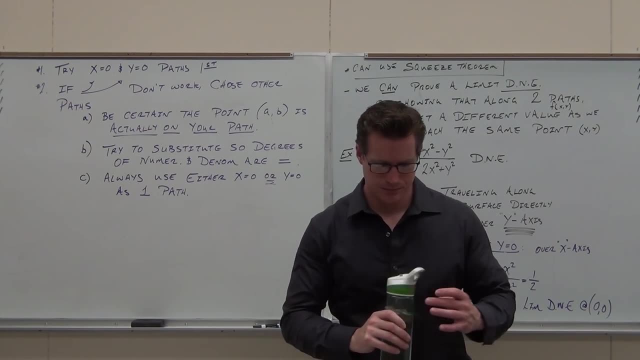 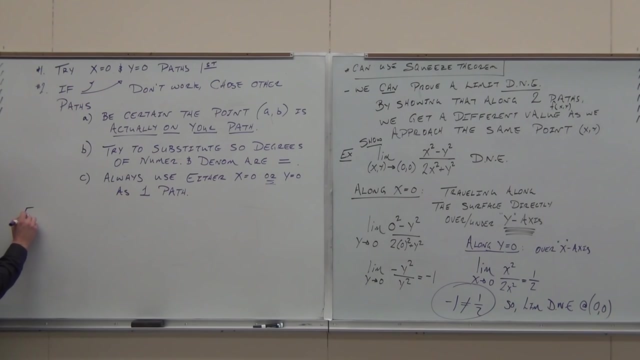 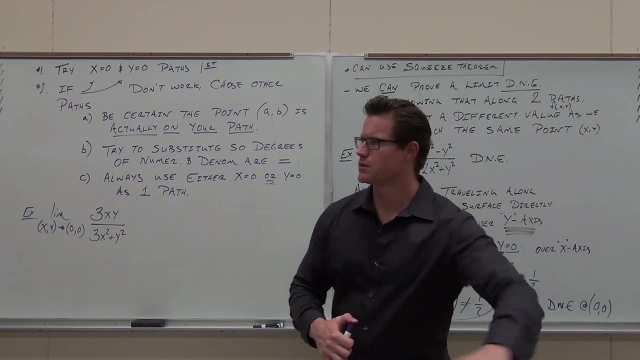 Yes, The over the surface, sorry, along the surface, over a particular path. you guys get that Okay, So let's try this. Let's do the limit here, There, Everyone in class right now. how many independent variables do you have? 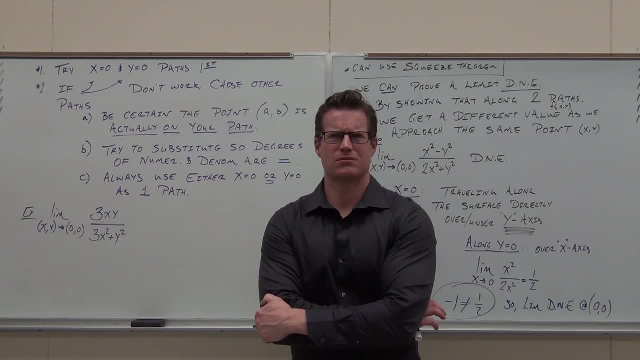 Two, Okay. So this is going to be a? what type of Surface? It's a surface 3D. Okay, 3D surface, Great. What point are we approaching? Zero, zero, zero. What should you do every single time? 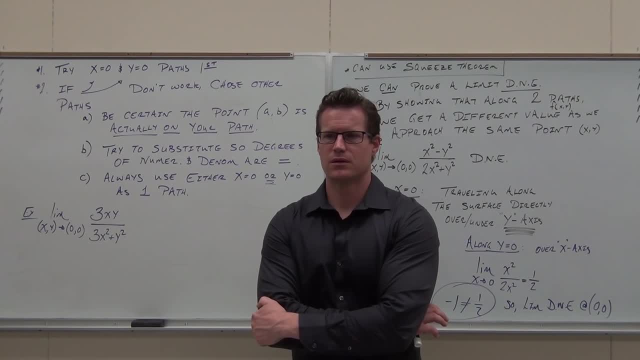 with the limit, no matter what. I don't care what class you're in. What do you do with the limit? Just try to plug it in. What are you going to get here? Zero, Okay, Well, that kind of sucks. 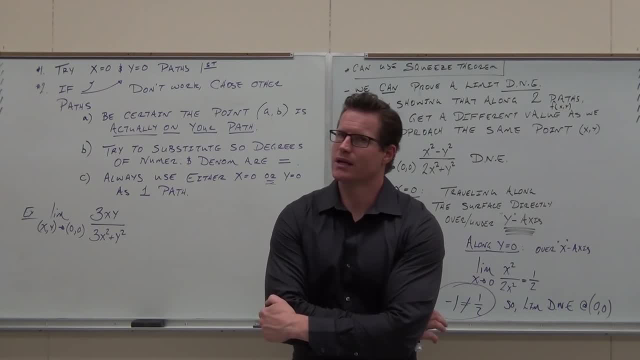 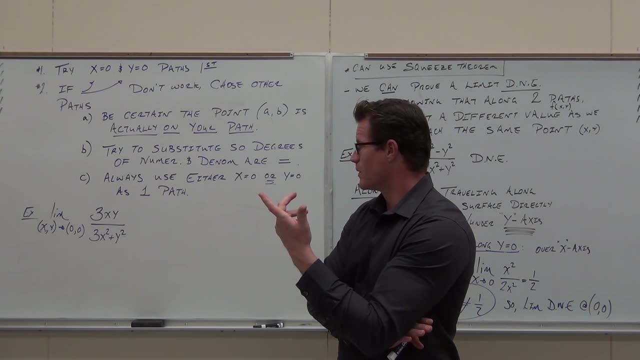 So we can't just plug in the value, because we get zero over zero. We don't really know how L'Hopital's rule works. If it does work, we don't even know. So, goodness gracious, what are we going to do? 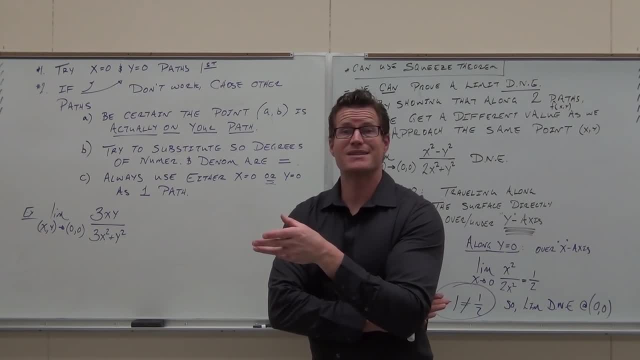 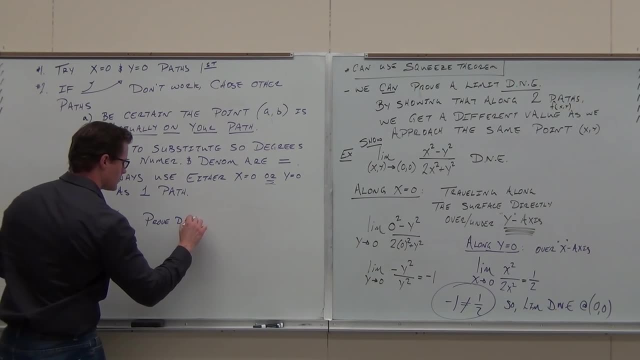 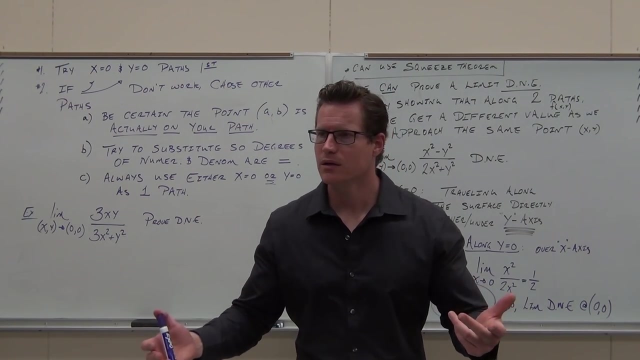 Well, what I'm going to ask you here is not to prove that it does exist. prove it doesn't exist. That makes your lives easier, Because all you need is how many paths? Two paths, You can't do one, because it doesn't make sense. 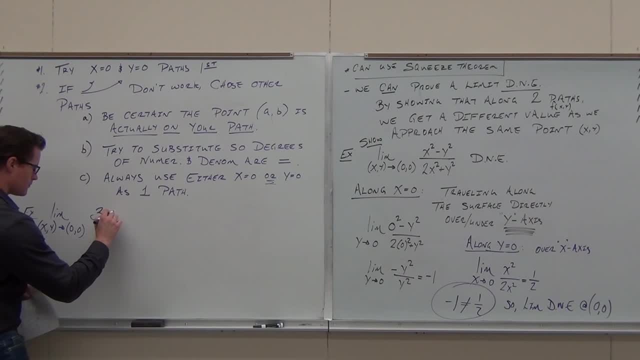 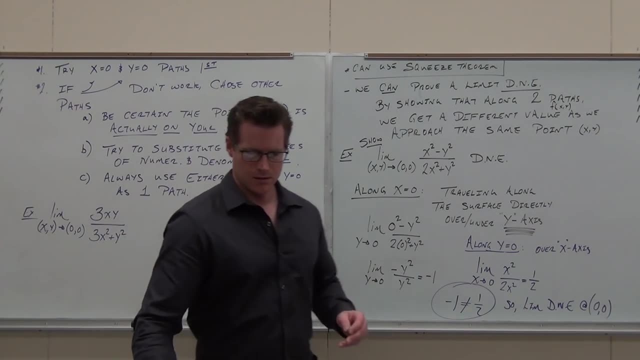 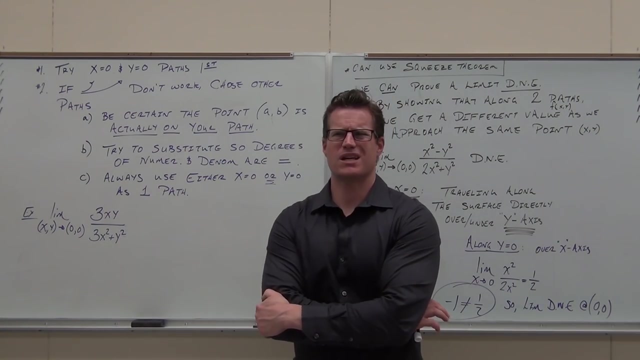 There, Everyone in class right now. how many independent variables do you have? Two, Okay, So this is going to be a. what type of Surface? It's a surface 3D surface. Great, What point are we approaching? 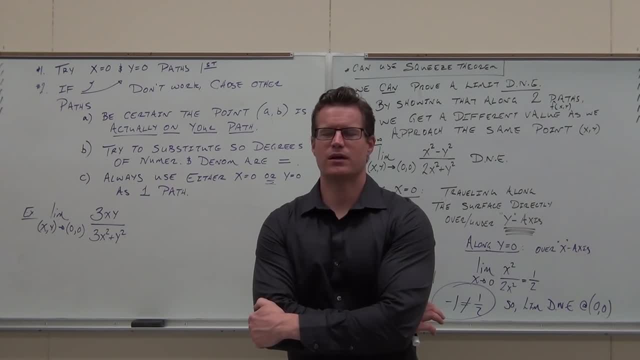 Zero, zero, zero. What should you do Every single time with the limit? no matter what, I don't care what class you're in. what do you do with the limit? Plug it in, Just try to plug it in. 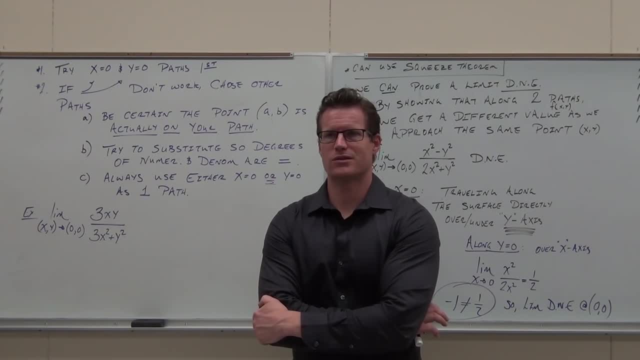 What are you going to get here? Zero, Okay, Well, that kind of sucks. So we can't just plug in the value because we get zero over zero. We don't really know how L'Hopital's rule works. If it does work, we don't even know. 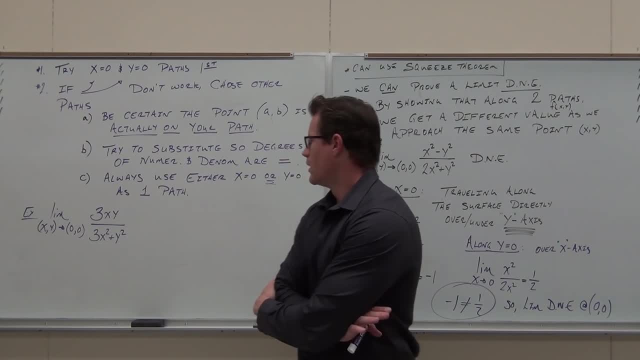 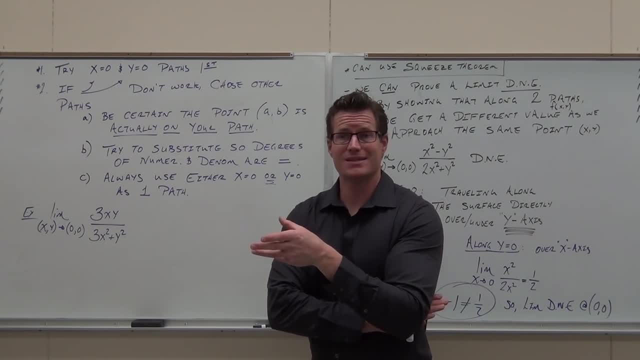 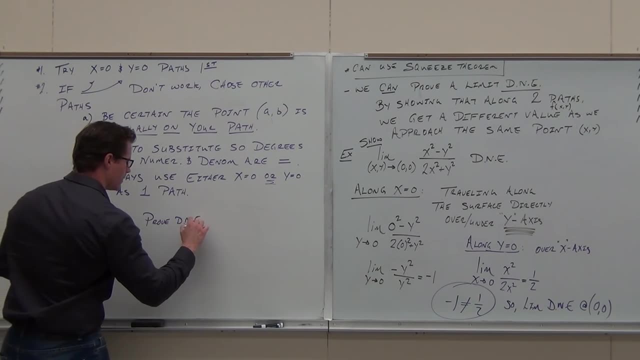 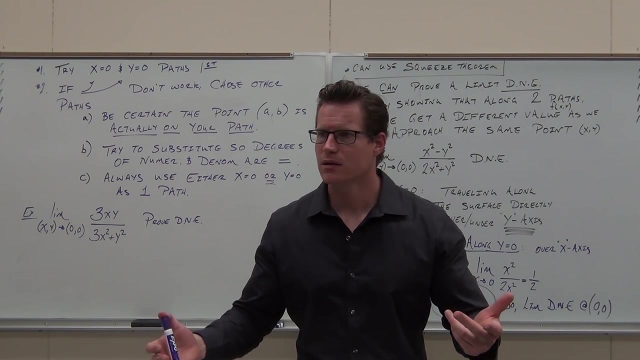 It doesn't exist. It doesn't exist. If it does exist, prove it doesn't exist. That makes your lives easier, because all you need is how many paths? Two paths, Two paths. You can't do one because it doesn't make sense. 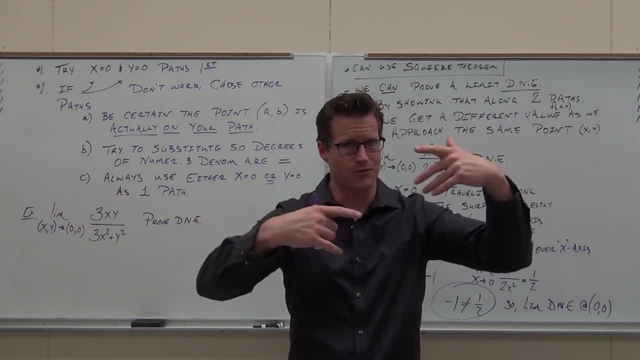 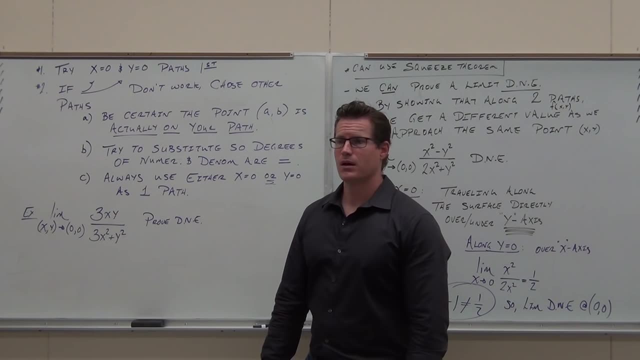 You've got to show that we're getting different values, just like from left and right side we're getting different values. So we need two paths to go. Here's the cover-up method that I would encourage you to try. first off, Okay. 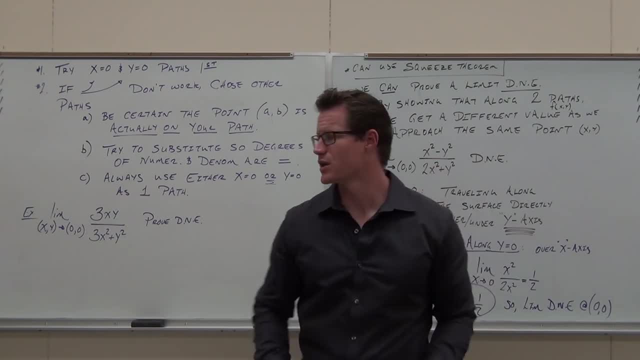 You've got to show that we're getting different values, Just like from left and right side we're getting different values. So we need two paths to go. Here's the cover-up method that I would encourage you to try. first off, Okay, Check it out. 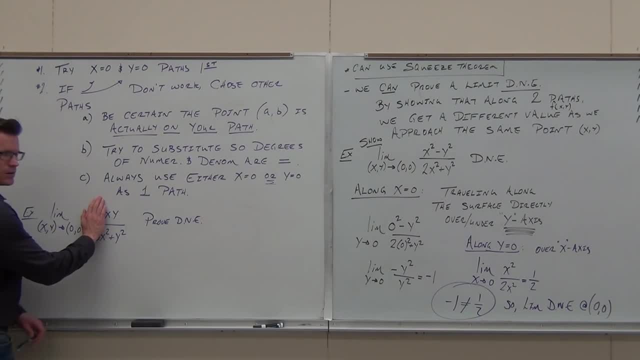 Cover up your X's. What's the limit there? Oh, silence. Oh, here, That's good. You know what? We've got to use one of those anyway. So let's try. X equals zero. Let's see what happens. 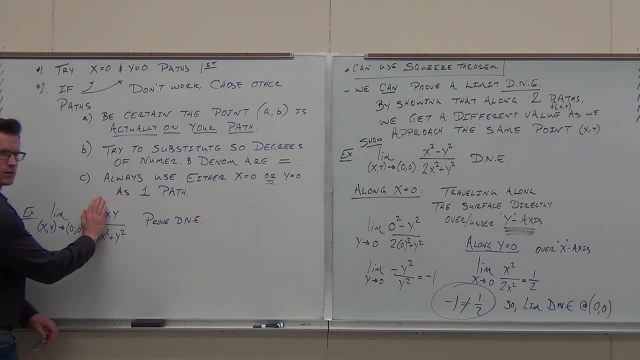 Check it out. Cover up your X's. Okay, What's the limit there? Oh, silence, Oh here, That's good. You know what? We've got to use one of those anyway. So let's try. X equals 0.. 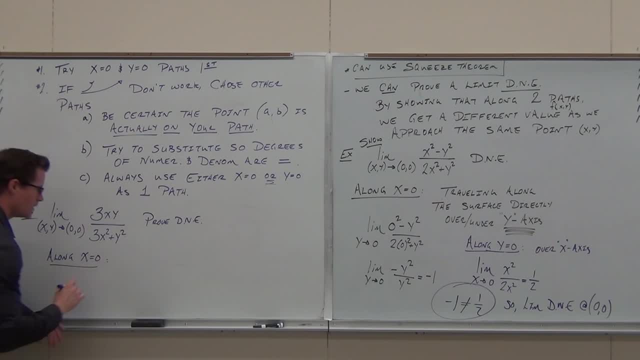 Let's see what happens. Can you- at least left-siders, can you tell me what I should rewrite if I'm letting X go to 0?? Tell me, please Anything you want, So just do it. Tell me what it is. 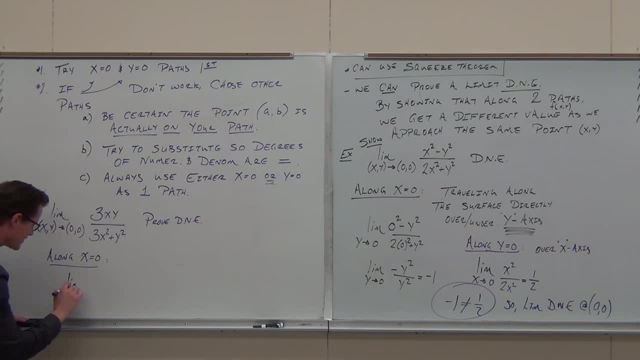 The limit? Y, Oh, the limit. Oh good, I still have those. Good, What variables do I have? Y, Y, Where's it going? 0.. Can you verify something for me, That this point 0, 0 is somewhere along the Y axis, which is X equals 0. 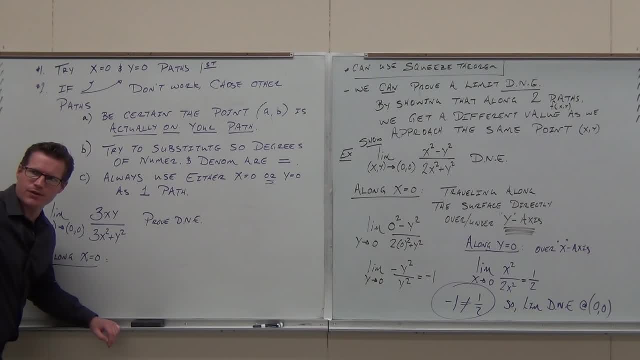 Can you at least left-siders- can you tell me what I should rewrite if I'm letting X go to zero? Tell me please Anything you want, So just do it. Tell me what. it is The limit Y. 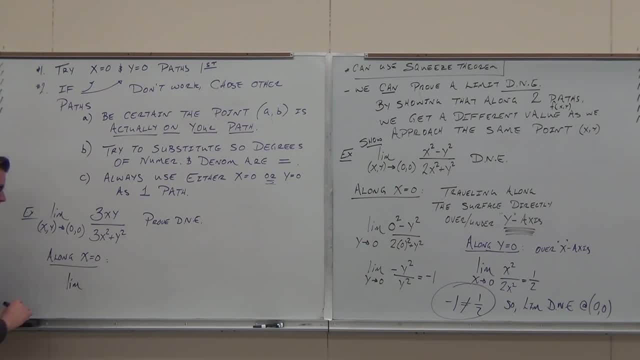 Oh, the limit. Oh good, I still have those. Good, What variables do I have? Y, Y, Where's it going? Zero. Can you verify something for me That this point zero, zero is somewhere along the Y axis? 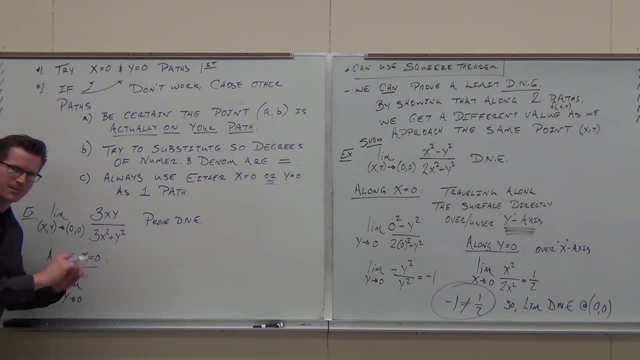 which is X equals zero. Can you verify that? for me It's somewhere along there. You have to have that happen. If it doesn't happen, you're wasting your time. What happens when It happens when I let X go to zero? 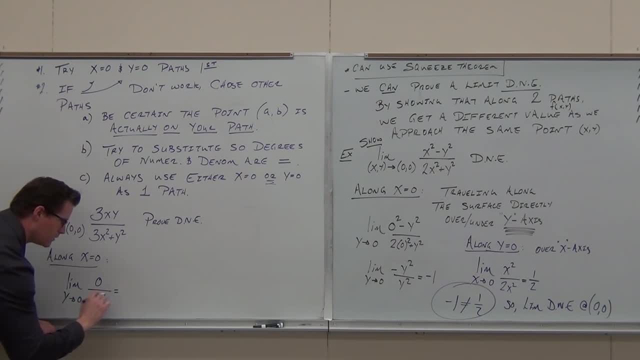 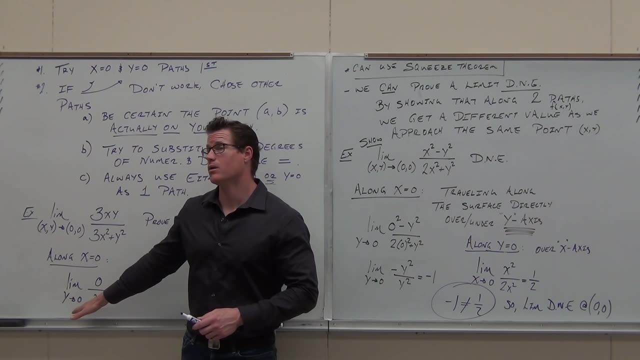 Over One. What is that? It's zero. Two ways you can prove it. One, oh wait, wait. How many independent variables do you have now? One: Does L'Hopital's rule work? Yeah, Now it does. 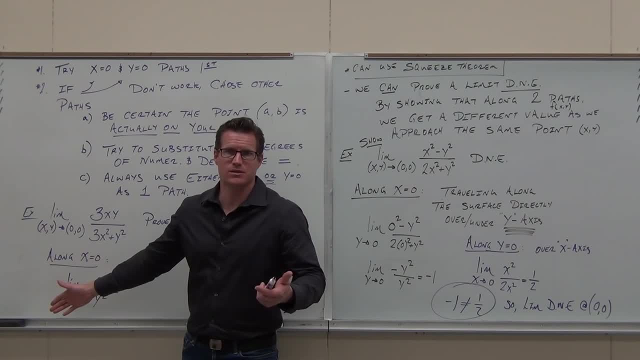 Easily. You have zero over two. If you want to do L'Hopital's rule twice, fine, Or you just go. well, that's an actual zero. This is only approaching zero. So it's zero divided by an actual number, not zero. 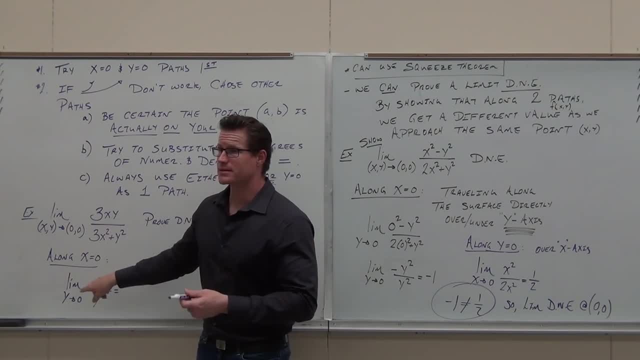 Keep in mind. what limits Do they say? I'm getting really gross. So that's zero for sure, And not if you're okay with that one. You can do that by just going: hey, let's cover this up. Can you still do L'Hopital's rule? 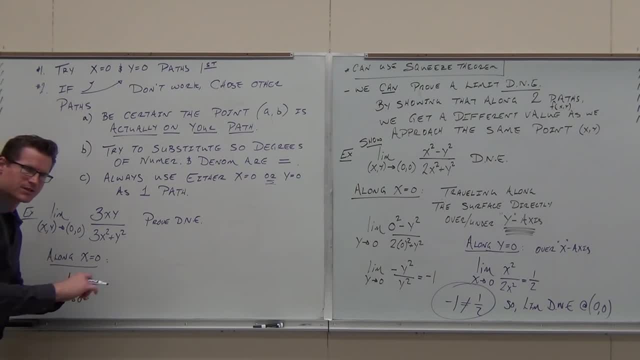 Can you verify that for me? It's somewhere along there. You have to have that happen. If it doesn't happen, you're wasting your time. What happens when I let X go to 0? Over 1.. What is that? 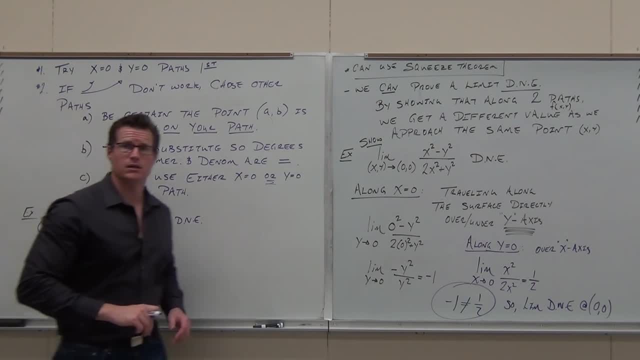 It's 0.. It's 0.. Two ways you can prove it. One: oh, wait, wait. How many independent variables do you have now? One: Does L'Hopital's Rule work? Yeah, Now it does Easily. 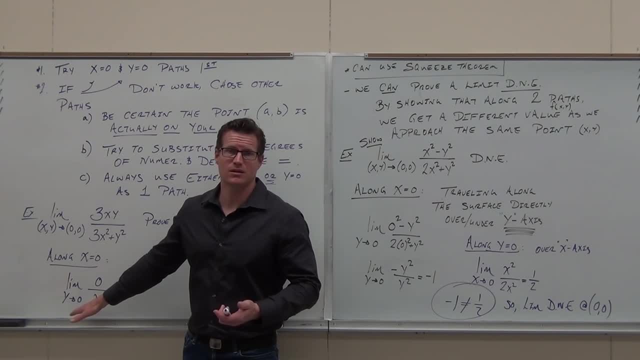 You get 0 over 2. if you want to do L'Hopital's Rule twice, Fine, Or you just go. well, that's an actual 0.. This is only approaching 0.. I'm just going to go back to the previous one. 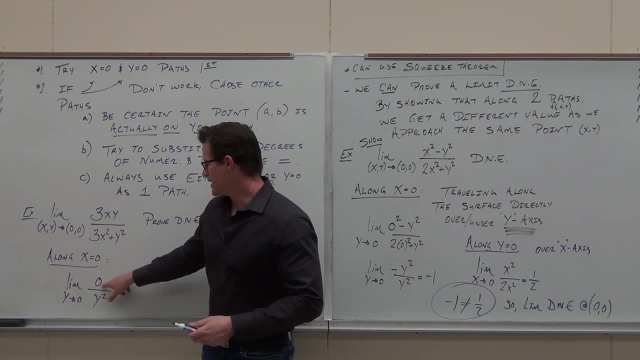 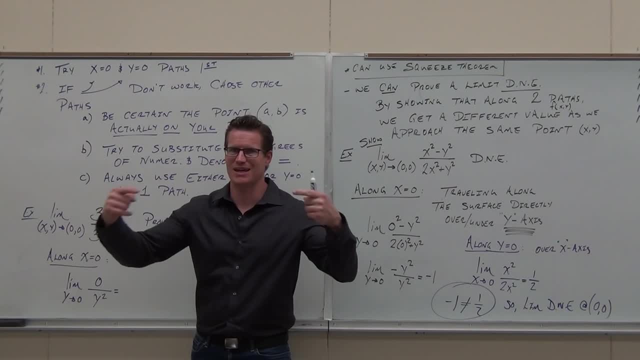 Keep in mind. what limits do? They say I'm getting really gross, So that's 0 for sure. I don't know if you're okay with that one. You can do that by just going. hey, let's cover this up. 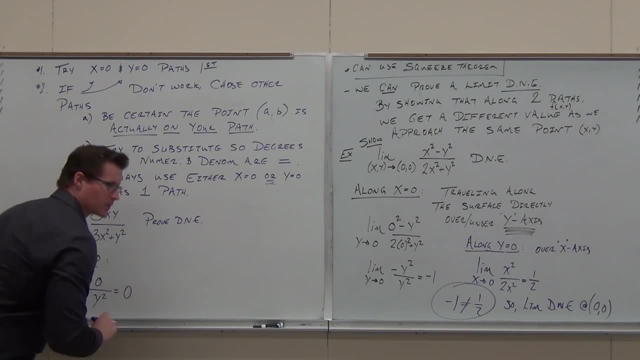 Can you still do L'Hopital's Rule? Yeah, You get 1 over 2Y, which is 0 over 2.. It's 0.. Now try this: What if I cover up the? you should be on this side. 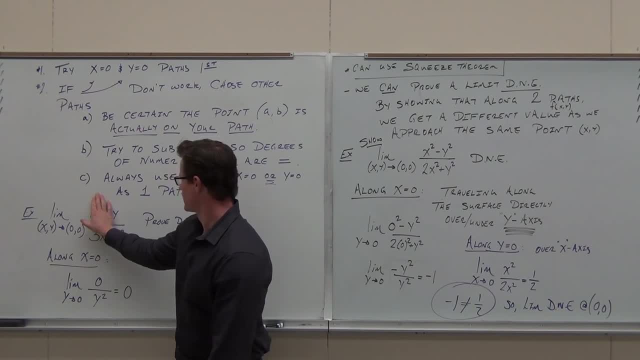 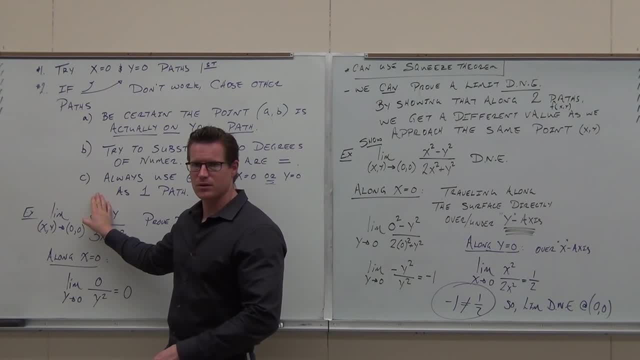 Let Y equal 0.. What if I cover up the Ys? Let Y equal 0.. And here's my number 2.. It's 0.. Now try this. What if I cover up the? you should be on this side. 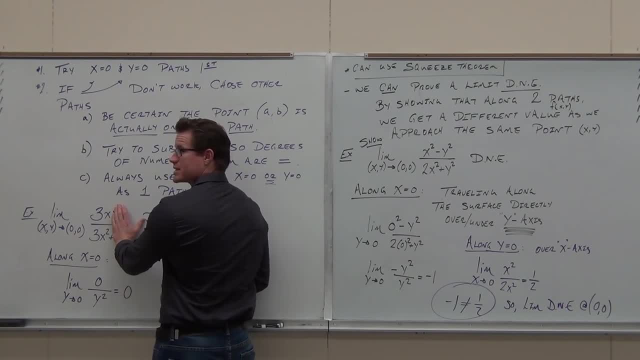 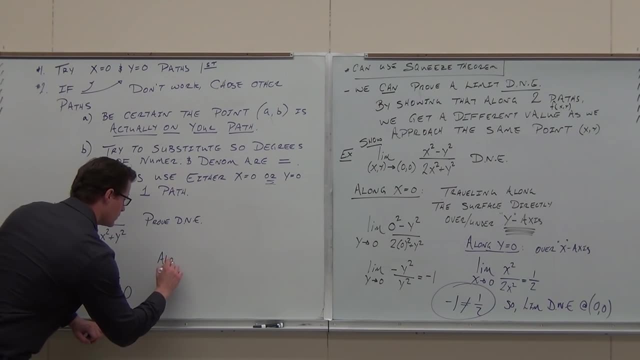 What if I cover up the Y? Let Y equal 0.. Do I still get 0?? Yes, That's a problem and I'll show you right now. If I go along, Y equals 0, then I'm fixing the Y. 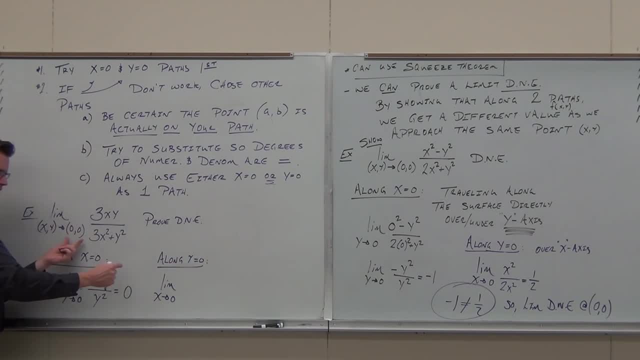 I still need the X to go to 0.. Notice: 0, 0 is along that path. If I let y go to 0, then I still get 0, but I have 3x squared. Do you guys see where the 3x squared came from, where the 0 came from, yes or no? 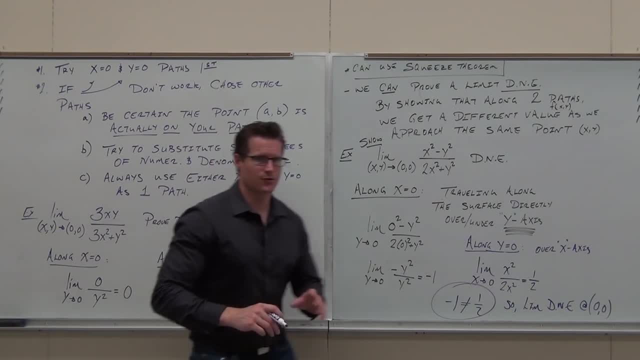 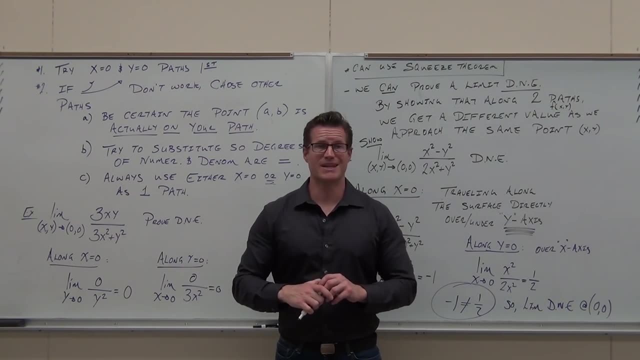 How much is that limit? Now, if you didn't get it the first time, let's get it this time. I got 0 along this path. I got 0 along this path. Does it prove the limit exists? How many paths can get to this point? 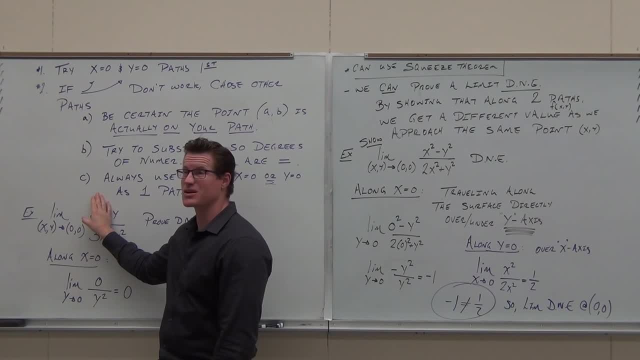 Yeah, You get one over two Y, which is zero. over two, It's zero. Now try this: What if I cover up the should be on this side? What if I cover up the Y's? let Y equal zero. Do I still get zero? 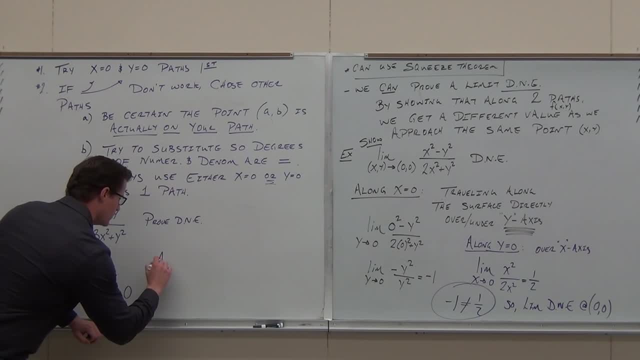 That's a problem And I'll show you right now. If I go along, Y equals zero, then I'm fixing the Y. I still need the X to go to zero. Notice: zero, zero is along that path. If I let Y go to zero, then I still get zero, but I have three X squared. 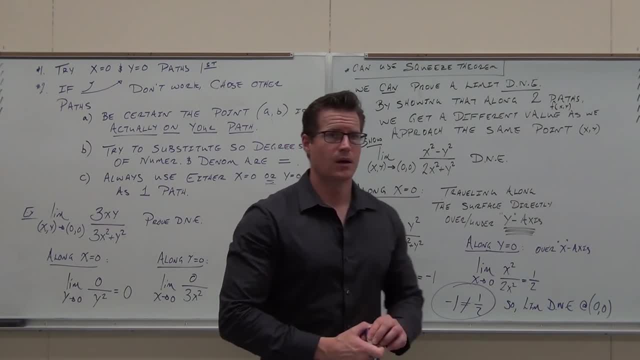 Do you guys see where the three X squared came from, Where the zero came from? Yes or no? Mm-hmm, How much is zero? How much is that limit Zero Now? if you didn't get it the first time, let's get it this time. 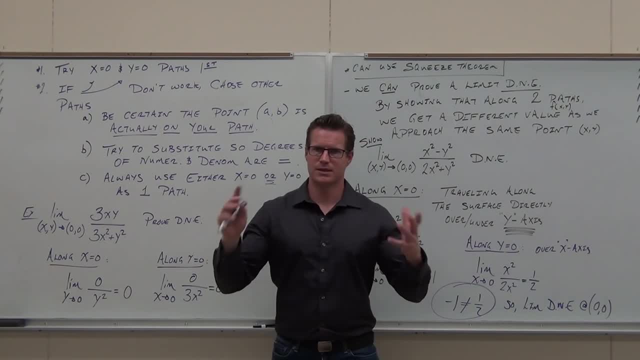 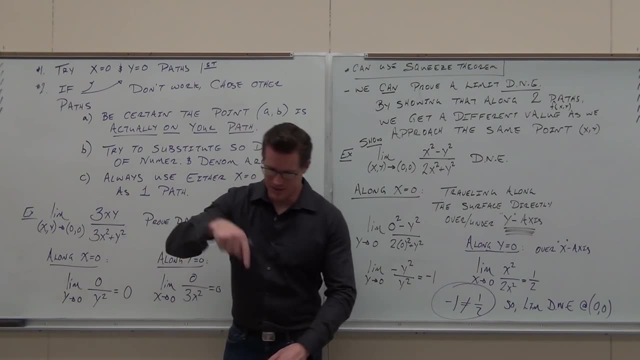 I got zero along this path. I got zero along this path. Does it prove the limit exists? No, How many paths can get to this point? Infinitely many. It's the origin on a plane. Infinitely many lines, paths, curves, whatever get to that value. 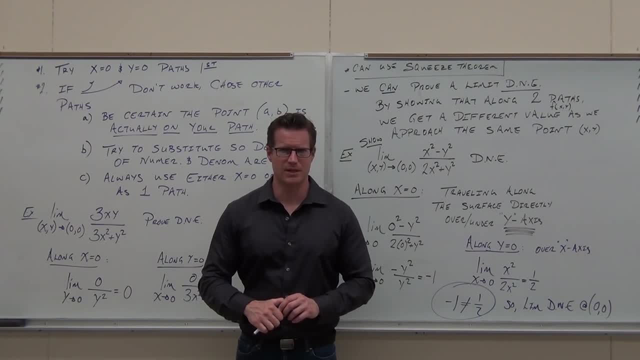 I've shown two that exist. Have I proven that the limit exists? Have I proven the limit doesn't exist? No, Which is my question? anyway, I've done nothing. I've done nothing so far Now, not nothing. One of these is good. 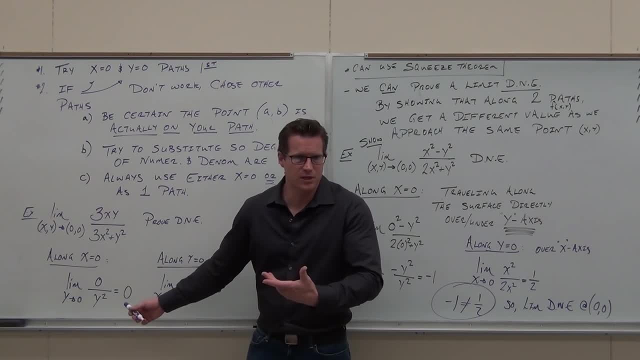 Okay, this is at least one path. Now both of them are. you don't need both, but choose one of these because it's really easy to find. So either one, I don't care, But it's not enough. Verify that this is not enough, one would please? 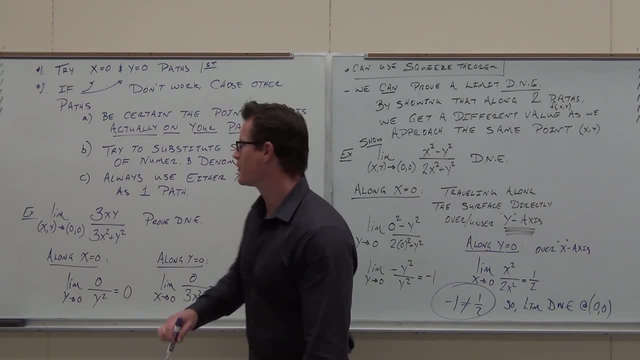 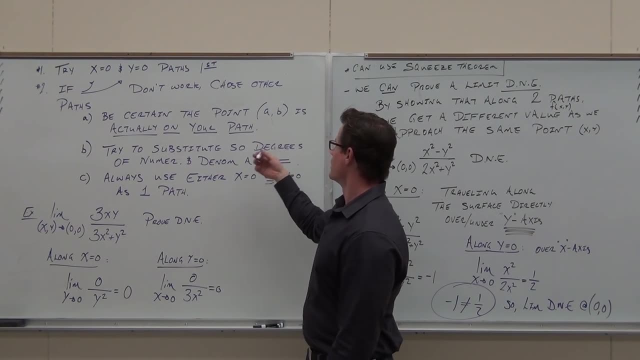 Let's pick another path. Here's how to pick the other path. First, be certain the point you pick is actually on your path. We're going to do that. Substitute so that the oh, this is the big one. Substitute so that the oh, this is the big one. 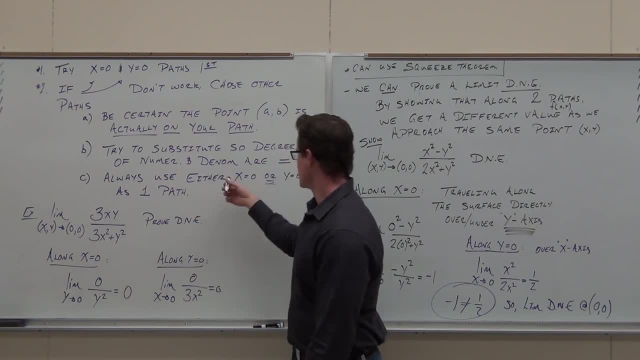 Substitute so that the oh, this is the big one. Substitute so that the degrees of the numerator and denominator are equal, and always use either oh, here we go. we got that one down, So here's the other path I would choose. 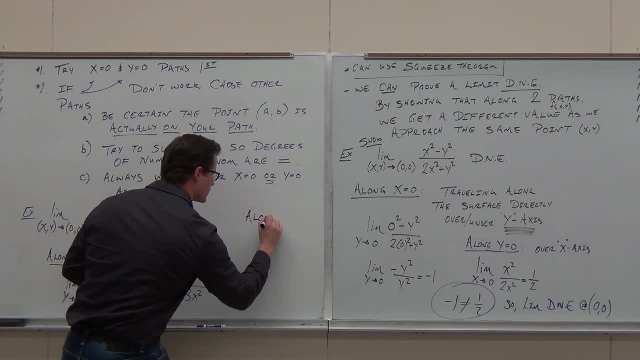 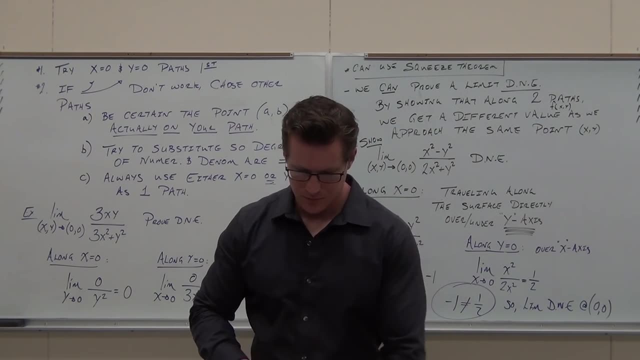 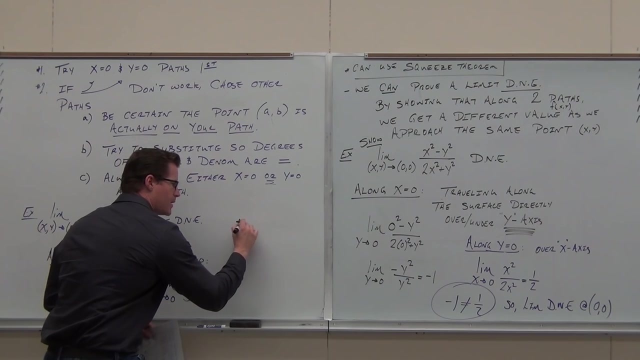 I'm going to look over here and I'm going to choose. you know what. I'll make it look a little sad. now I'm going to choose so that this happens. I want to pick y. I'm going to pick y equals a function of x or x equals a function of y. 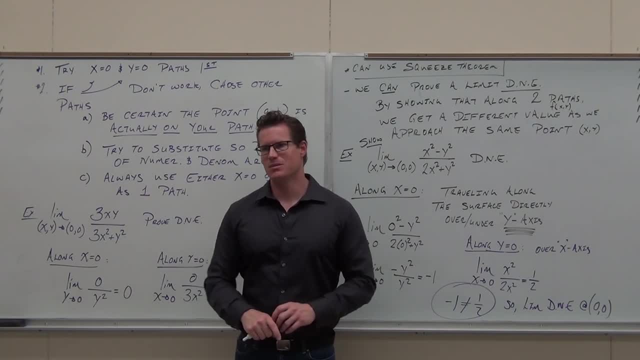 Infinitely many. It's the origin on a plane. Infinitely many lines, paths, curves, whatever, get to that value. I've shown two that exist. Have I proven that the limit exists? Have I proven the limit doesn't exist, which is my question anyway? 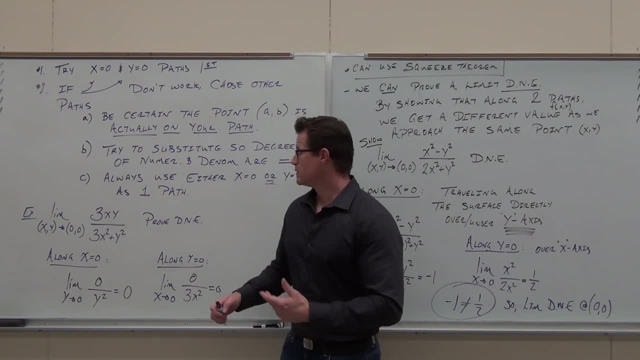 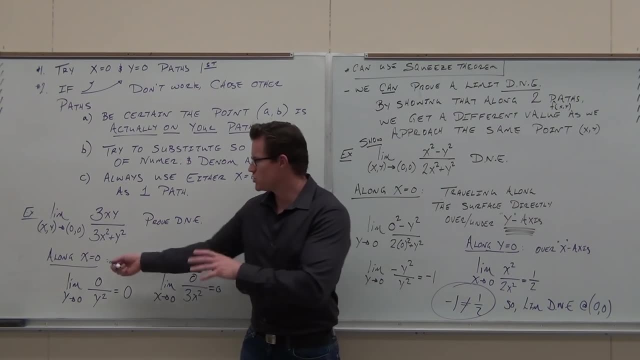 I've done nothing. I've done nothing so far, Now, not nothing. One of these is good. This is at least one path. Now, both of them are. you don't need both, but choose one of these because it's really easy to find. 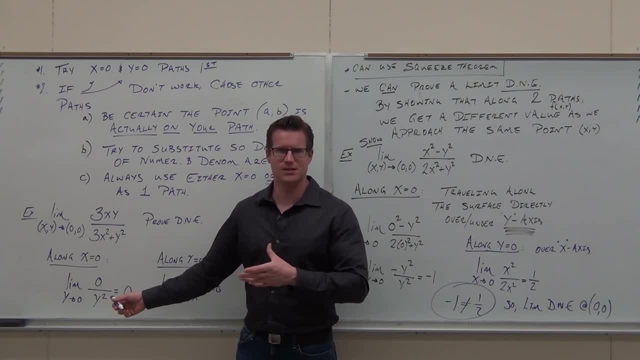 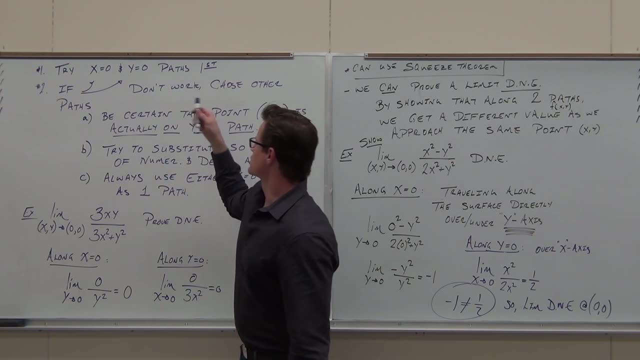 So either one, I don't care, But it's not enough. Verify that. this is not enough. limit, please. Let's pick another path. Here's how to pick the other path. First, be certain the point you pick is actually on your path. 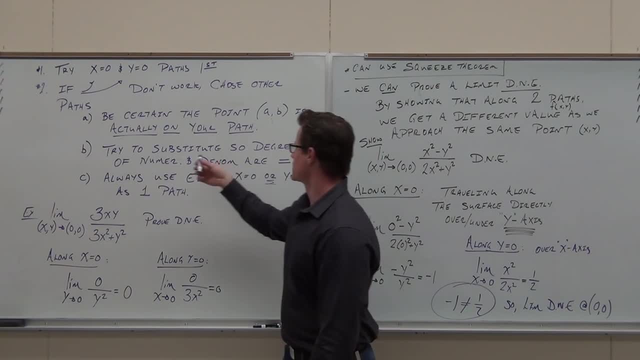 We're going to do that Substitute so that the oh, this is the big one, so that the degrees of the numerator and denominator are equal and always use oh, here we go. we got that one down, So here's the other path I would choose. 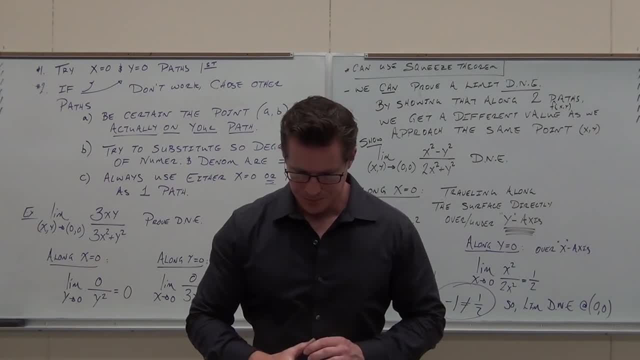 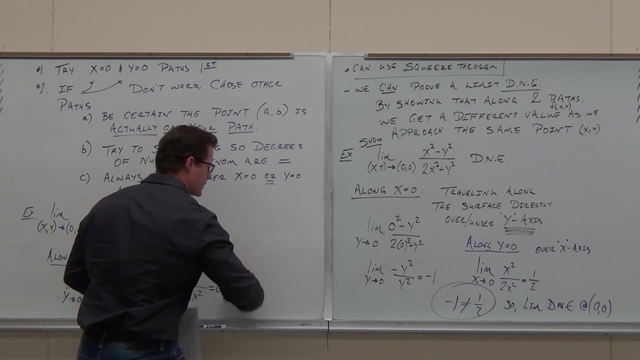 I'm going to look over here and I'm going to choose. you know what. I'll make it look a little sad. now I'm going to choose. so that this happens, I want to pick: y equals a function of x or x equals a function of y. 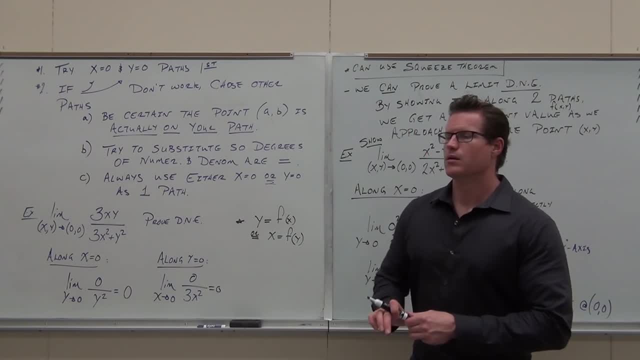 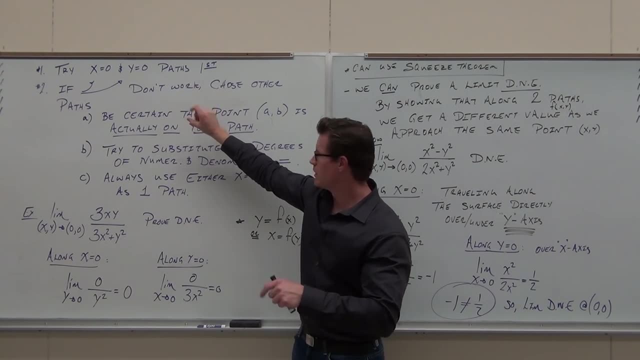 I'm going to pick that, but I want to do it so that these conditions are met, so that I still have this as a solution- Okay, It's got to be there- and so that my degrees are equal. There's multiple ways to do it sometimes, but here's the one I'm going to pick. 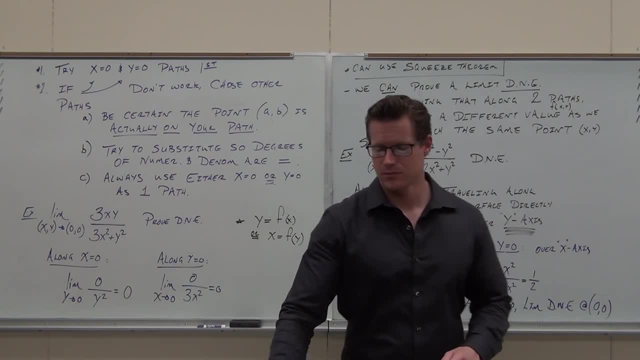 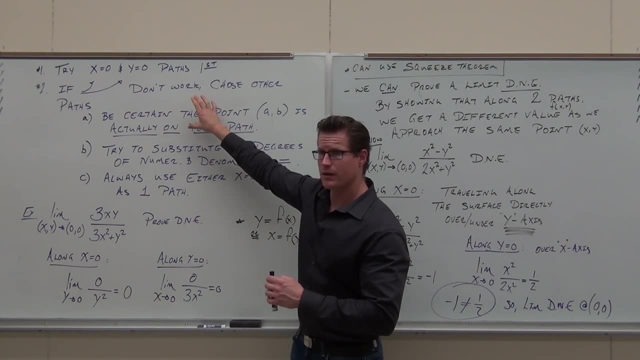 I'm going to pick that, But I want to do it so that these conditions are met, So that I still have this as a solution- It's got to be there- And so that my degrees are equal. There's multiple ways to do it sometimes. 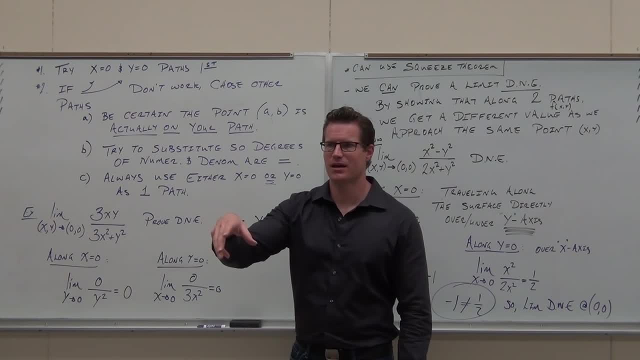 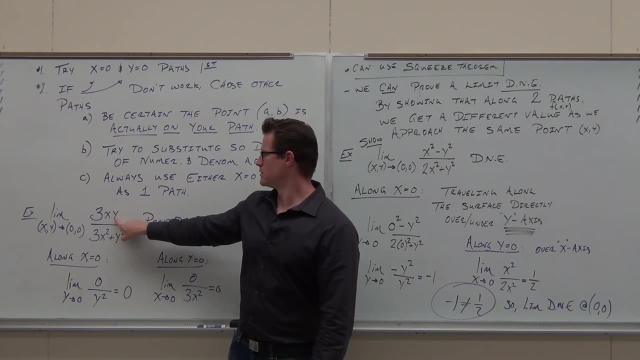 But here's the one I'm going to pick, because I like setting y equal to x's. You guys get that, So check this out. Let's imagine something. Let's imagine if this y was actually an x, Could you multiply those? 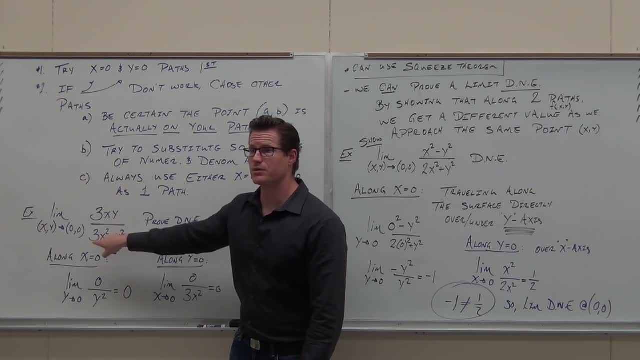 What would you get If this y was actually an x? could you add those And you would get 4x squared. Do you see how I'd be matching up the degree of the numerator and denominator? That's real nice. That's what I'm looking for. 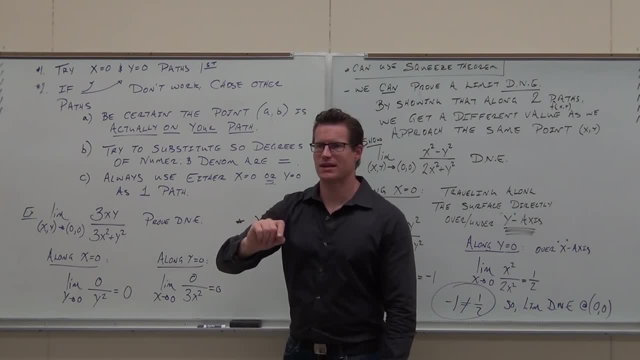 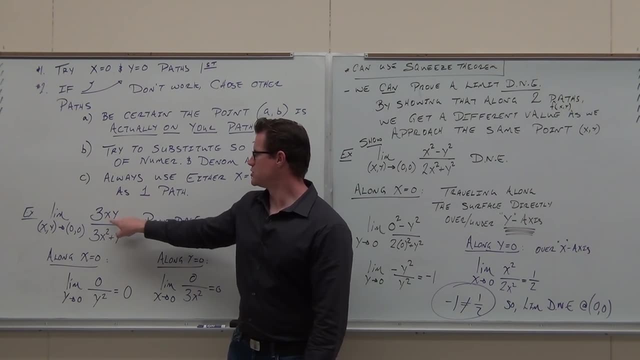 because I like setting y equal to x's. You guys get that, So check this out. Let's imagine something. Let's imagine if this y was actually an x. Could you multiply those. What would you get? If this y was actually an x, could you add those and you would get 4x squared. 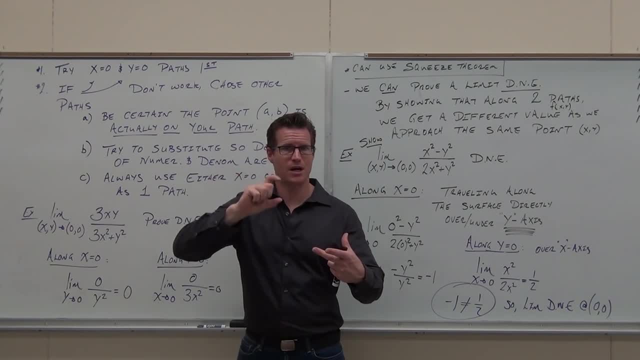 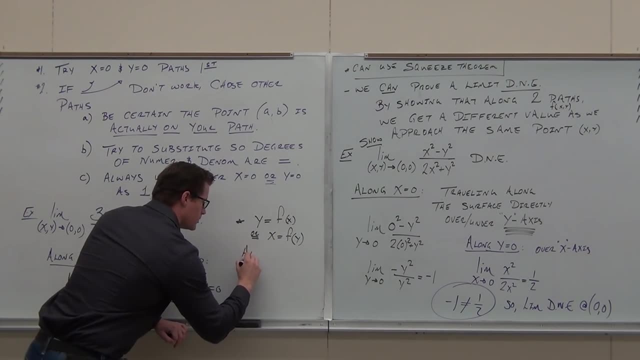 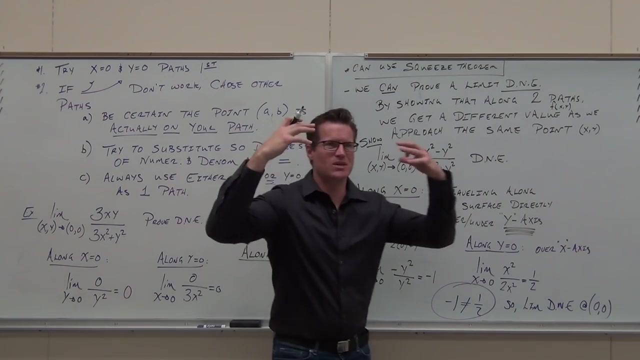 Do you see how I'd be matching up the degree of the numerator-denominator? That's real nice. That's what I'm looking for Also, just so it sinks in. so you get it. I probably don't have to explain it anymore. 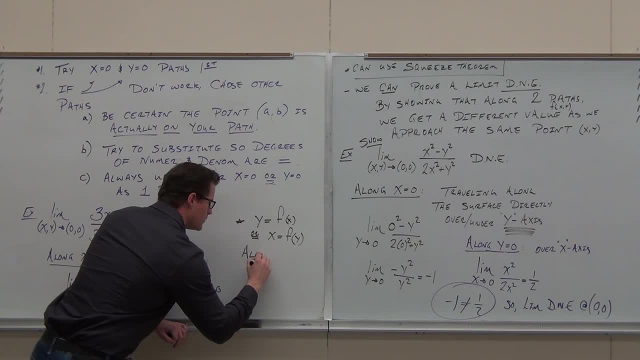 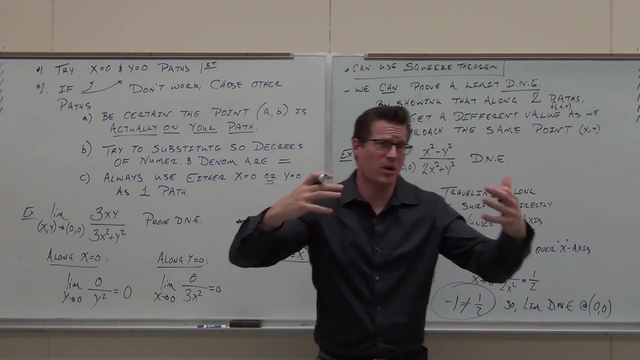 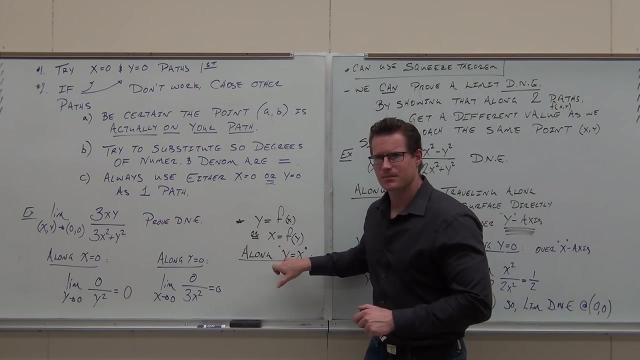 Also, Just so it sinks in. so you get it. I probably don't have to explain it anymore, But just so it sinks in. Notice something: If you were to graph y equals x, Look, If you were to graph y equals x, is that a curve? 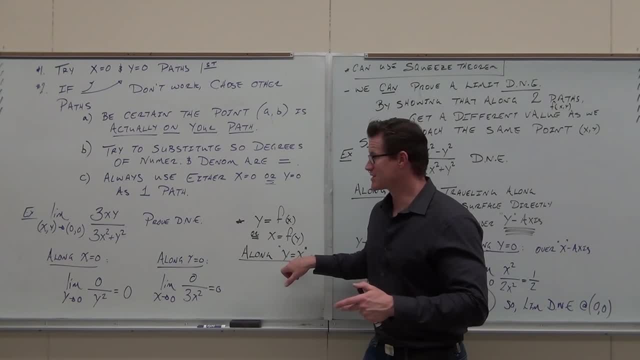 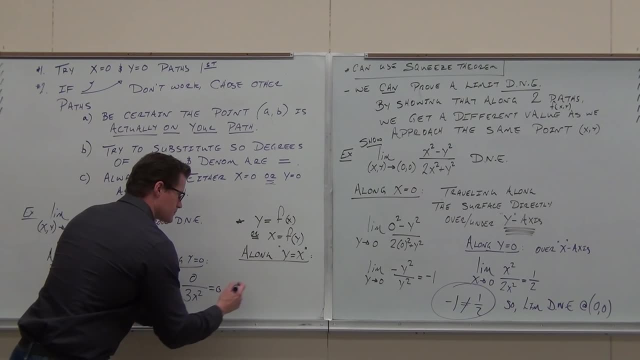 Yeah, Well, okay, We call lines curves. Is that a curve? Yeah, Does it go through that point? Yeah, Aha, Can you make a substitution? If you did, you'd go okay. Well, what's the only variable remaining now? 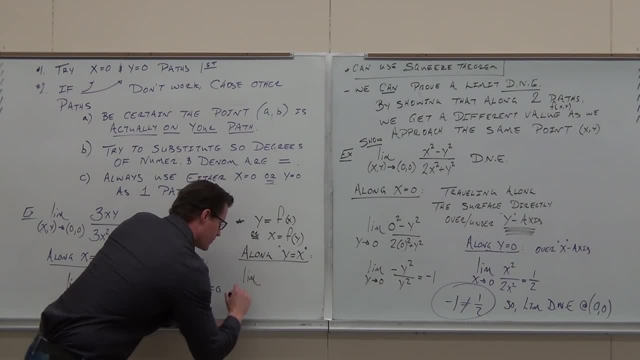 If I let y equal x, I have a limit. I have 3x times. what am I letting y equal? Notice how you could do it the other way around. You could let x equals y, It doesn't matter, But just change it so you only have one variable: y. 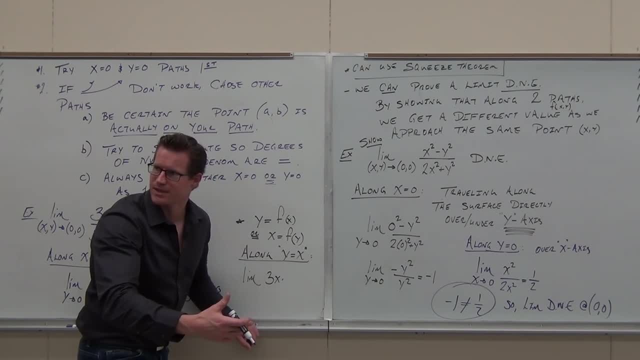 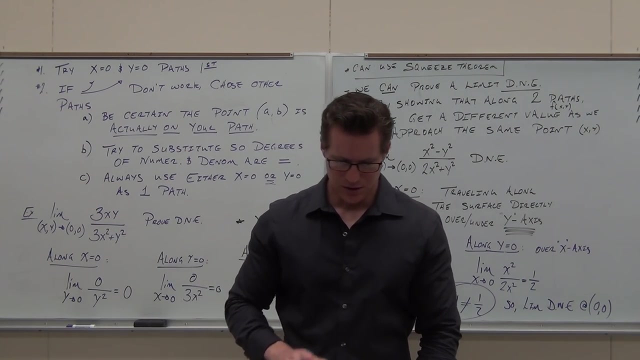 Well, because we know how to deal with limits with one variable. Does that make sense? So, oops, Let y equal x. Let y equal x. Seriously, though, are you guys okay with that one? Now, if we're only in terms of one variable? 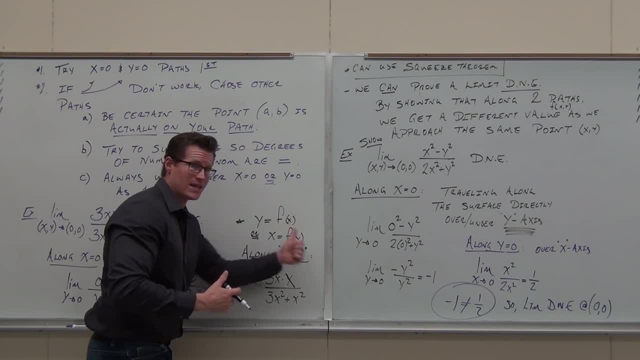 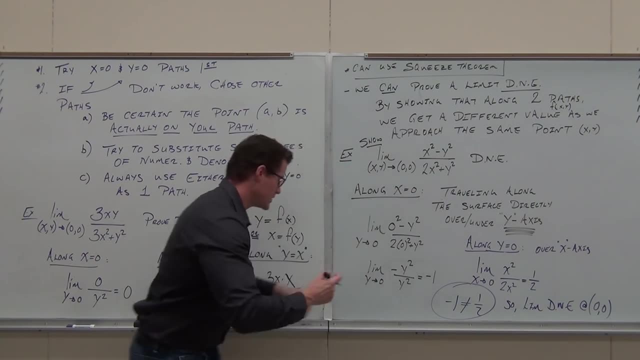 I really don't need to let y approach anything. I let y equal x. That's fixing the y. That's fixing it. That's fixing it to the x value. It's making it now depend on the x, which means the only thing I let float around is my x. 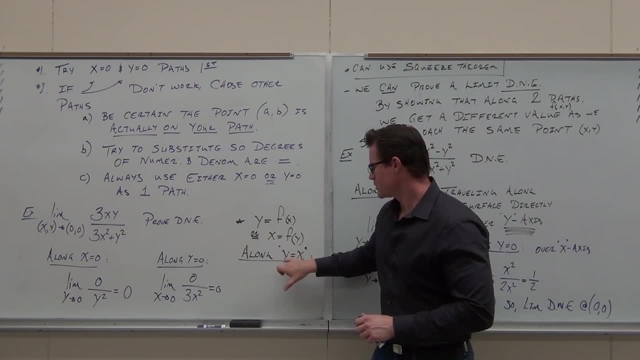 but just so it sinks in, notice something. If you were to graph y equals x, look, if you were to graph y equals x, is that a curve? Yeah well, okay, we call lines curves. Is that a curve? 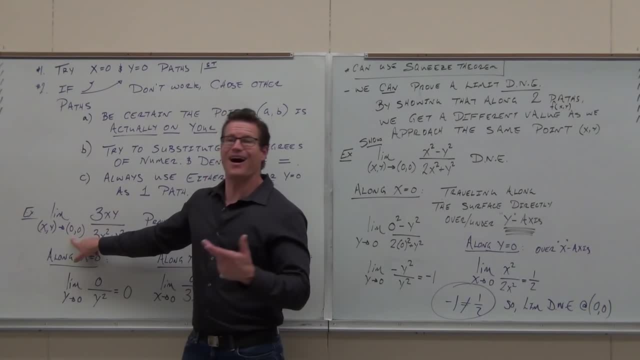 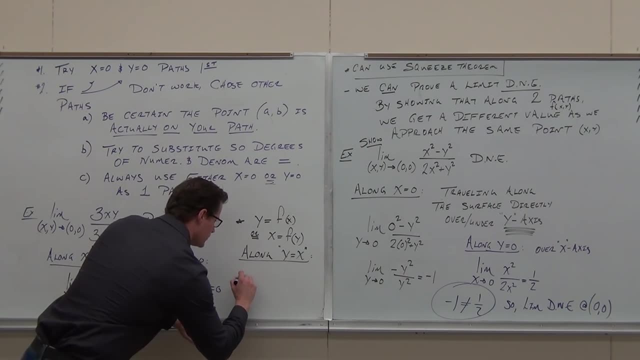 Yeah, Does it go through that point? Yes, Ha, Can you make a substitution? If you did, you'd go okay. well, what's the only variable remaining now? If I let y equal x, I have a limit. 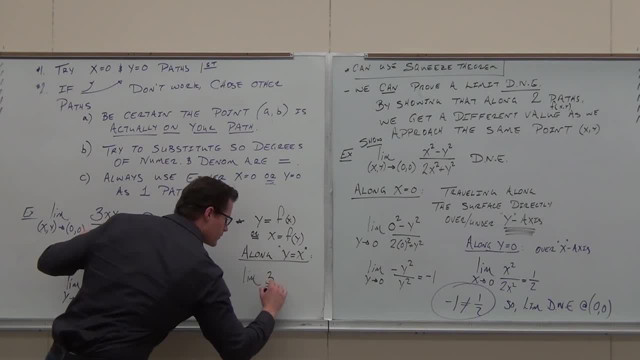 I have 3x times. what am I? letting y equal x. Notice what? Let's say, you could do it the other way around. You could let x equals y. It doesn't matter, but just change it. so you only have one variable. 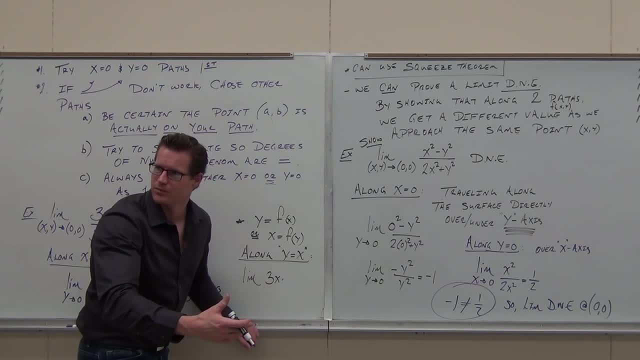 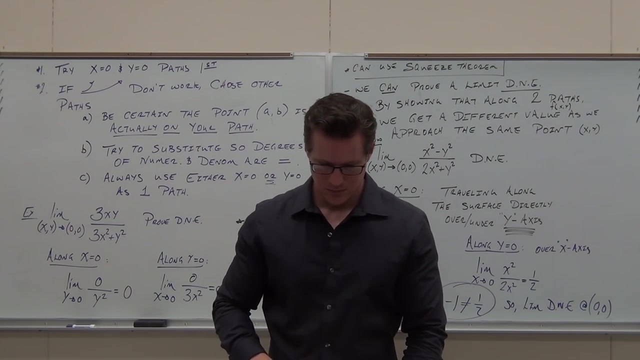 Why? Well, because we know how to deal with limits with one variable. Does that make sense? So, oops, let y equal x. Let y equal x. Seriously, though, are you guys okay with that one? Now, if we're only in terms of one variable? 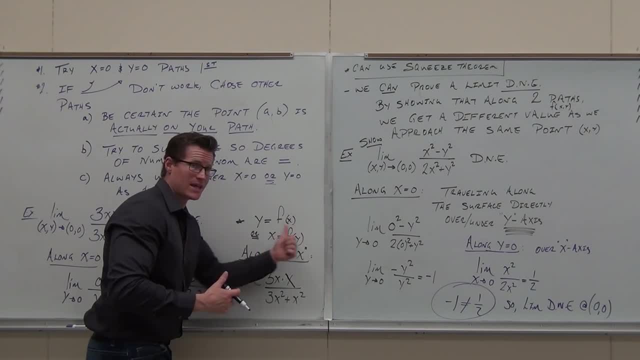 I really don't know how to do it. I don't know how to do it. I don't know how to do it. I don't need to let y approach anything. I let y equal x. That's fixing the y, That's fixing it to the x value. 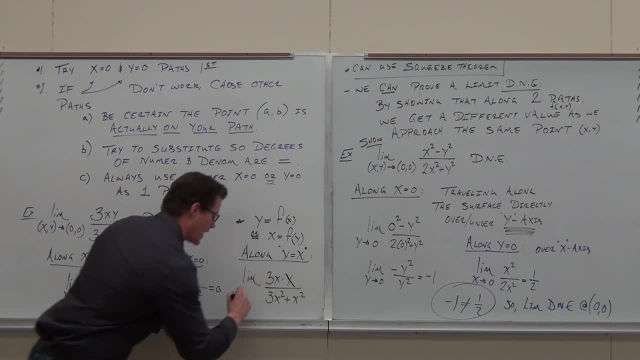 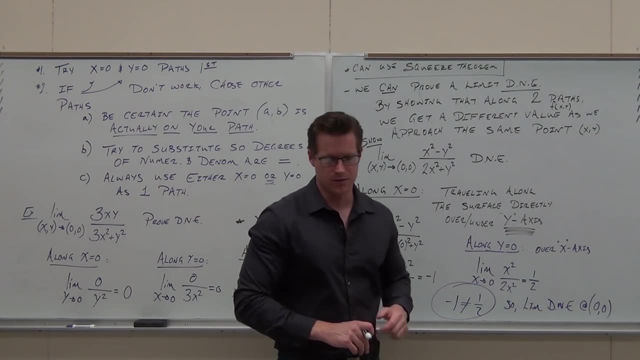 It's making it now depend on the x, which means the only thing I let float around is my x and it still has to go to 0. It's still got to approach that same value For real. yes, no, Are you picking up what I'm kind of like? 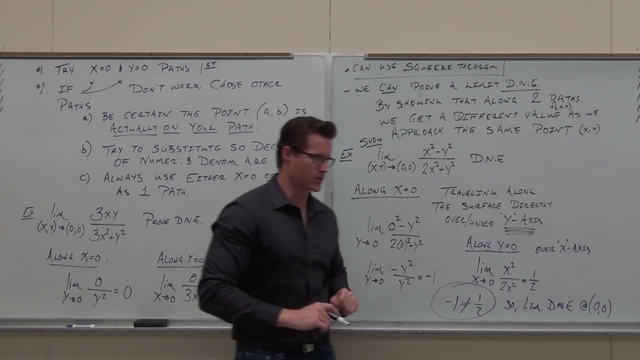 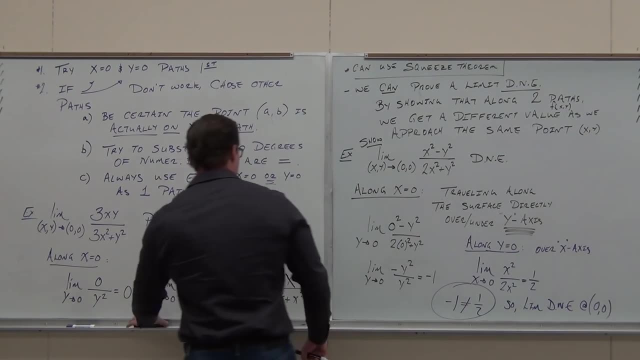 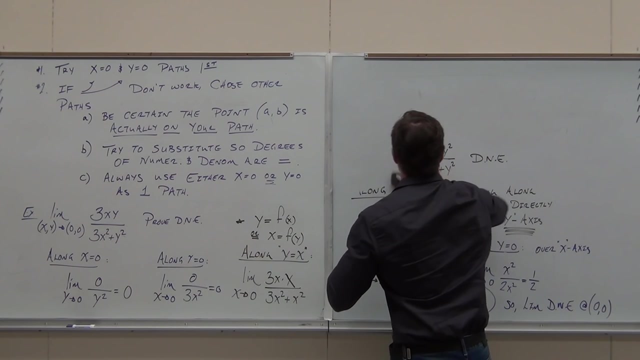 And it still has to go to zero. It's still got to approach that same value For real. Yes, no, Are you picking up what I'm kind of like? Yes, Now, let's do this. So here, if I change this to make it a little bit nicer, 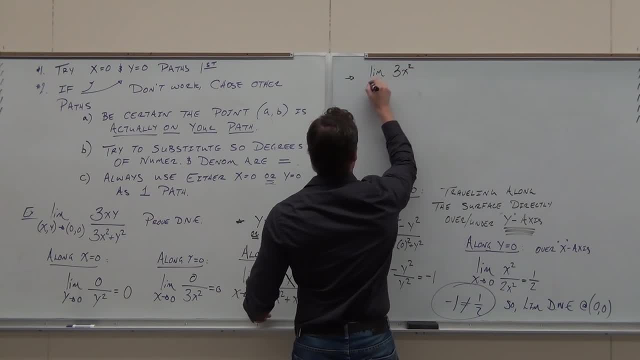 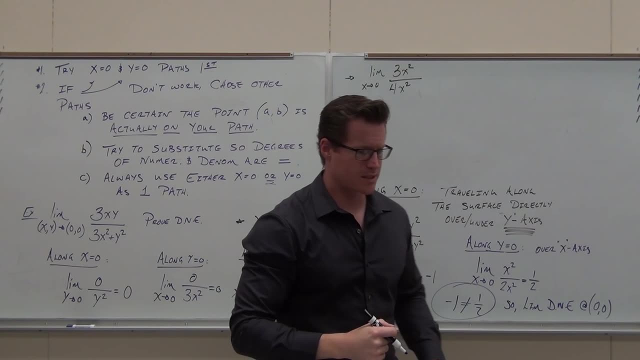 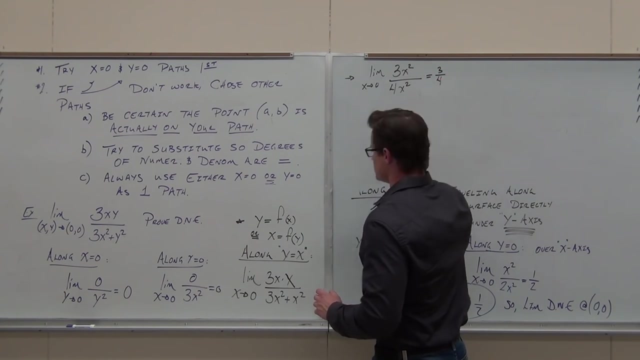 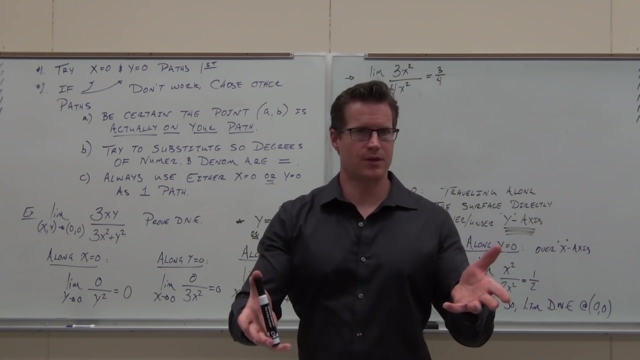 again a little bit. Limit 3x squared. we're not going to waste time doing limits real, real slow. What's that limit? By a variety of techniques. Now here's the question: Does that prove that the limit of this function at that point does not exist? 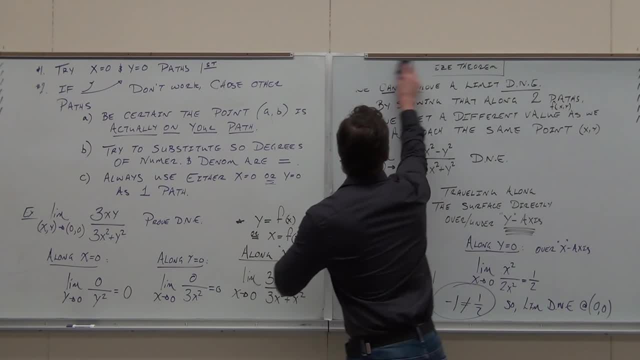 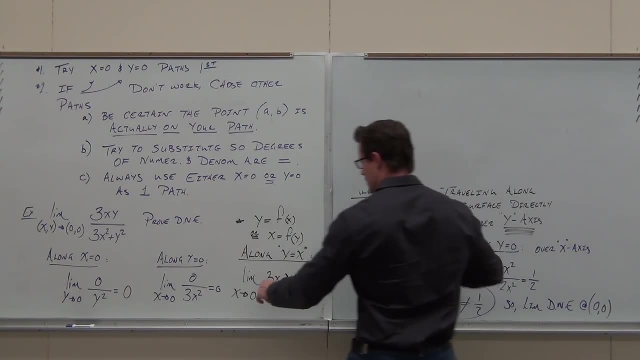 Yes, Now, let's do this. So here, if I change this to make it a little bit nicer, 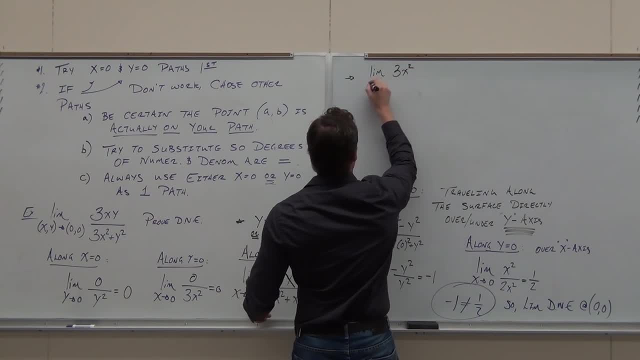 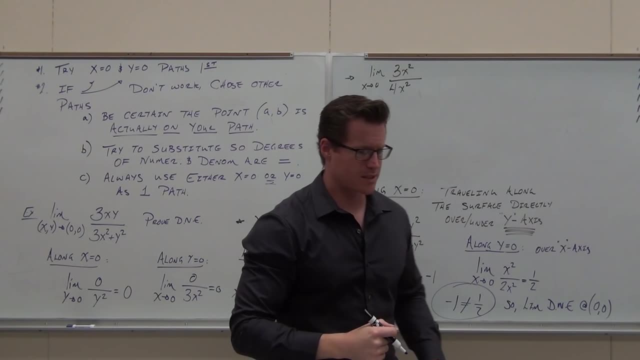 I got a limit 3x squared. We're not going to waste time doing limits- real, real slow. What's that limit? 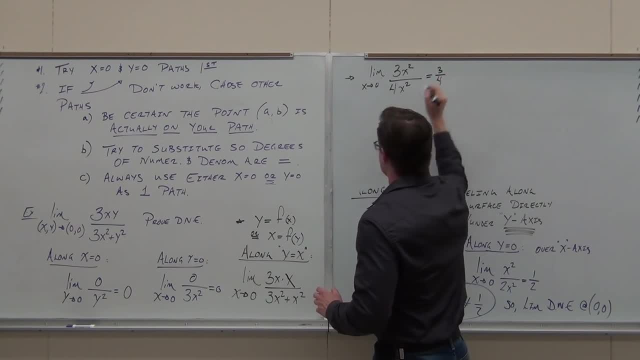 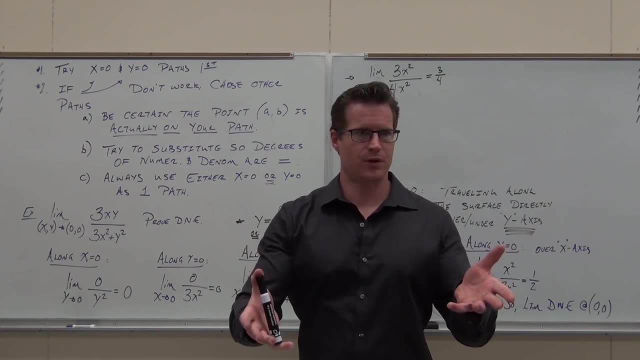 By a variety of techniques. Now here's the question: Does that prove that the limit of this function at that point does not exist? Does that prove it? 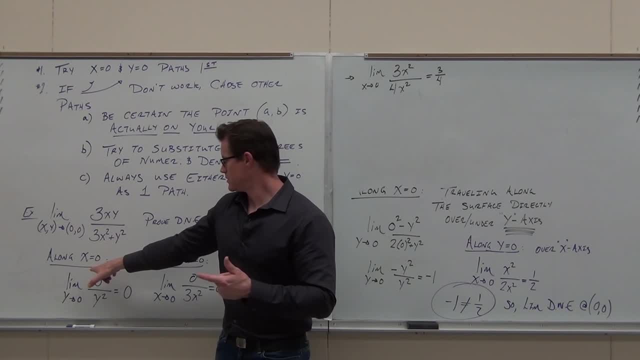 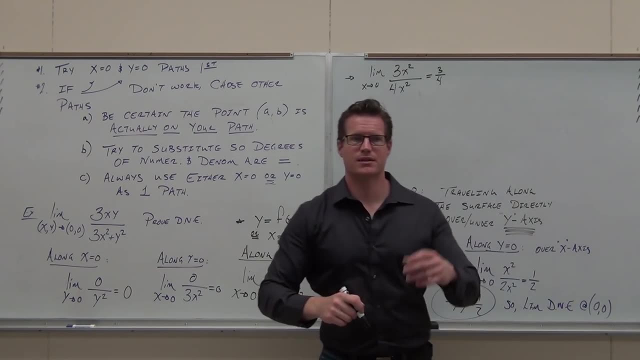 Does that prove it? Yes, Along one path, We got to zero. Along another path We got to. that didn't prove anything. Along a different path, we got to three-fourths Since zero. choose either one, I don't care. 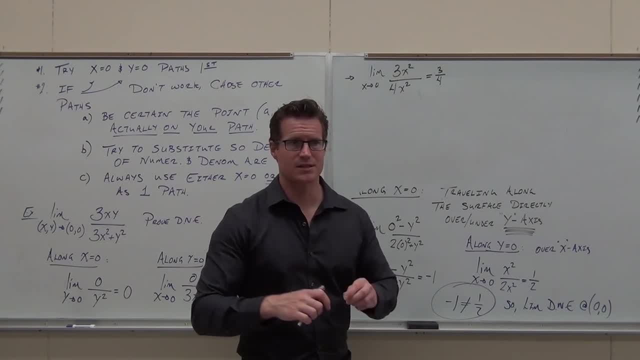 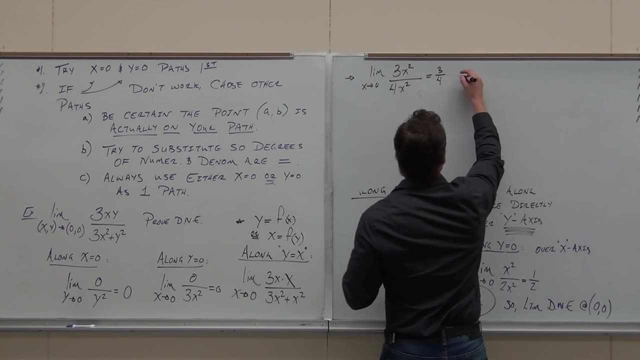 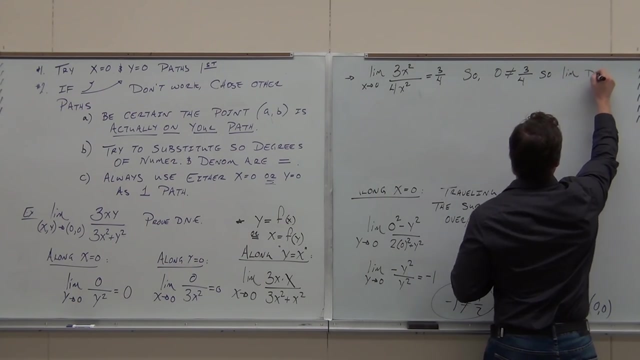 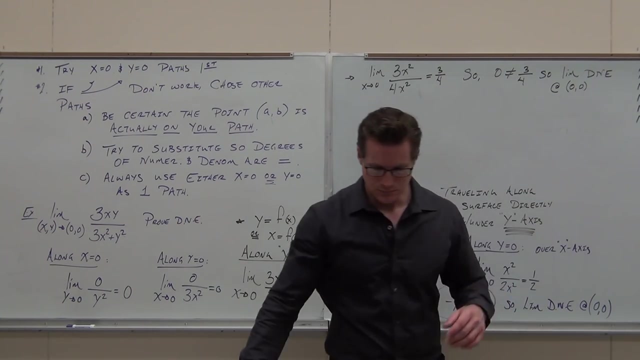 Since zero does not equal three-fourths, that proves that the limit does not exist at x equals or, as the function approaches zero, zero on the xy plane. So what do we get? Let's do zero at xando, at x equal, or what? 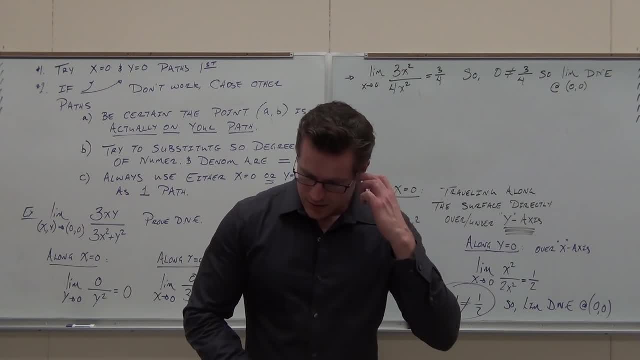 Zero, Zero. 于. Here we are. We get zero, Zero One, Zero, Zero, Zero, Zero, One, Zero, Zero, Zero Zero. I'll give you a little message Just to keep you on track. Oh yes. 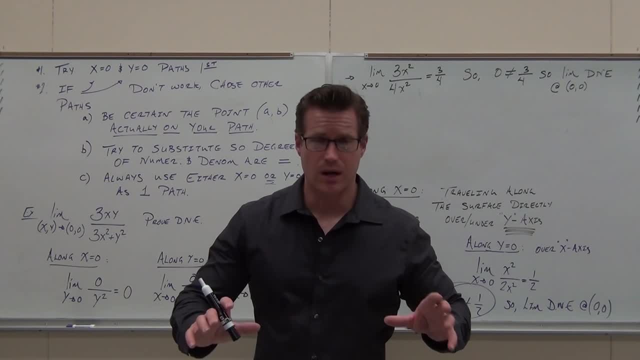 Okay, Here's whatever job I was so adept at. That job is a little easier because, even if it's a little bit closer, it's always been a little chaotic in that area, and Azure Cloud Training, The other way of speaking about. 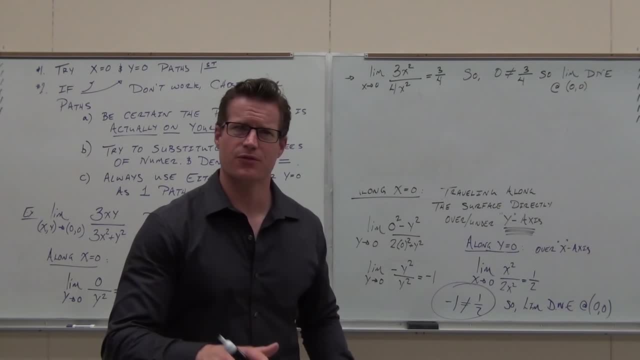 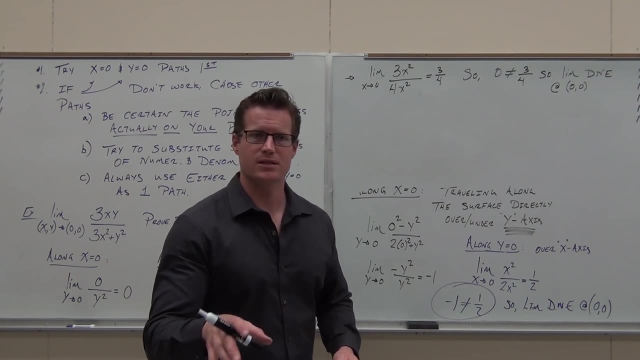 Why are you always going to take the lead ofodes? It's a hot topic being rolled out on the. Okay, I'm probably going to forget, So let's try one more. to get you know what. tell you what. I want you to try this one on your own, at least the first couple steps of it. let's see. 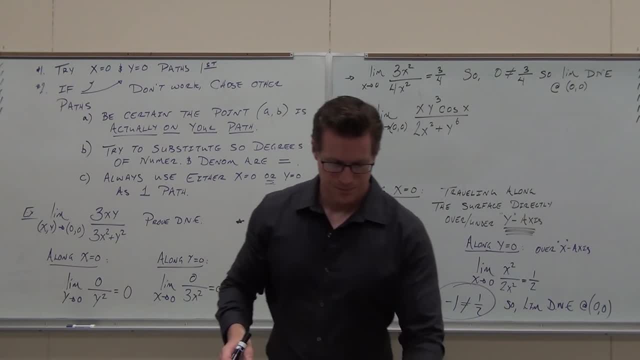 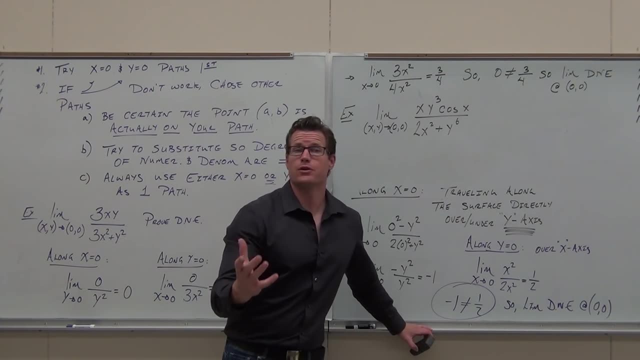 So, as I'm erasing, here's what I would like for you to do. I'd like for you to go along the two paths that we pretty much always start with. okay, well, actually, I want you to plug in the number: what are you going to get? 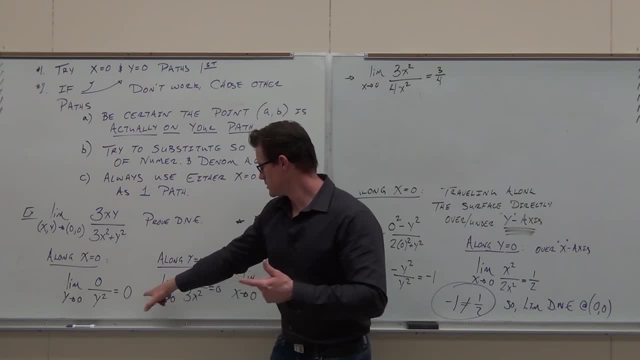 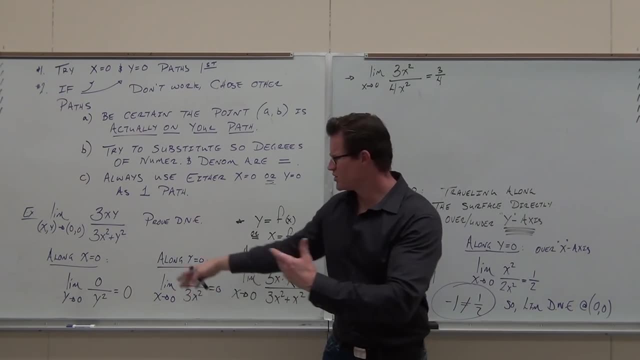 Yeah, Along one path we got to zero. Along another path we got to. that didn't prove anything. Along a different path, we got to three-fourths Since zero. choose either one, I don't care, Since zero does not equal three-fourths. 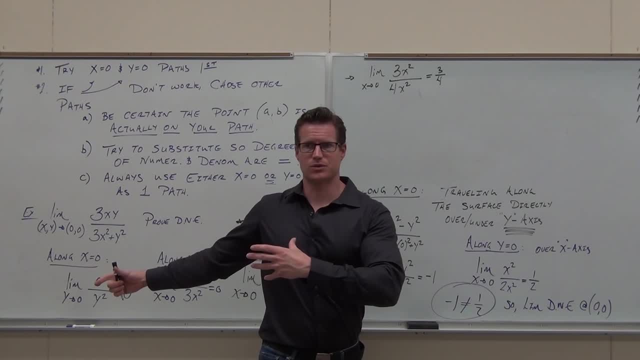 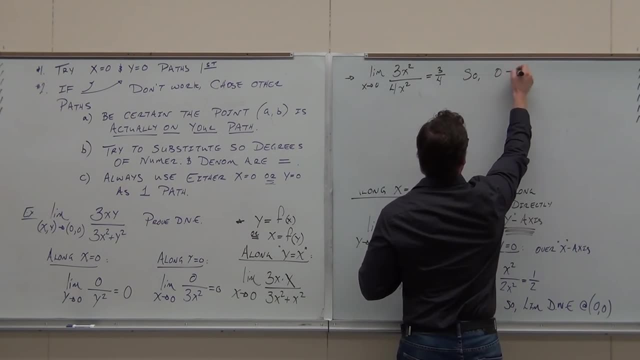 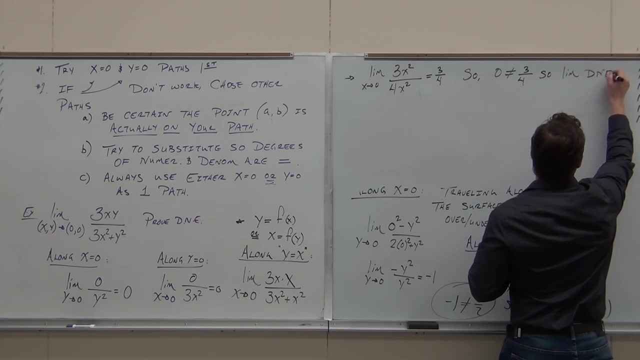 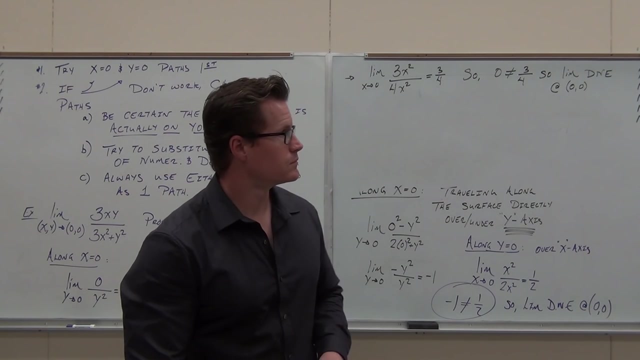 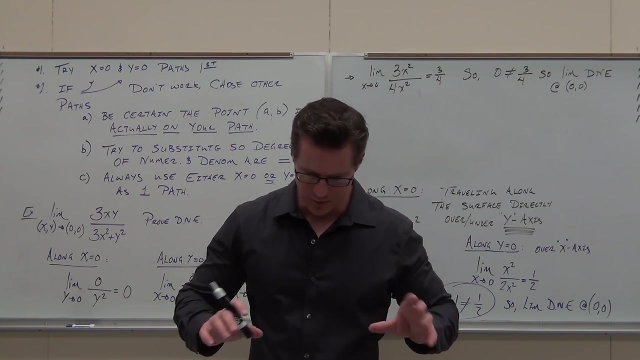 that proves that the limit does not exist at x equals zero as the function approaches zero. zero on the xy plane. Tell you what I wanted. I'd like to do two more, since we're right on this. We only they're going to go a little bit quicker. 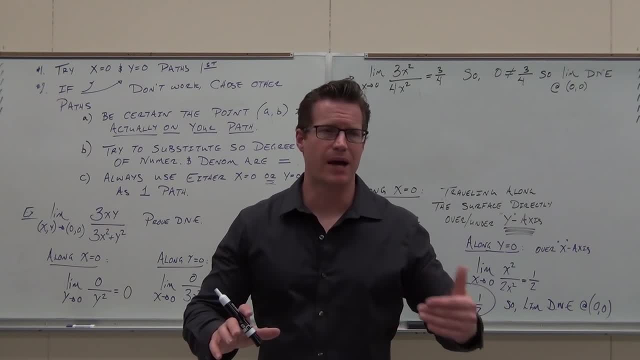 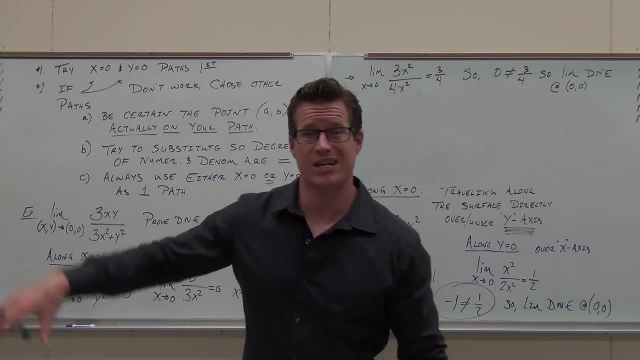 Since we're right in the middle of this concept, and when we come back from our break, I'll talk about how to deal with three variables. It's actually, it can be a little bit easier because you don't have real nasty, nasty substitutions, and you'll have this idea down. are you guys ready for this? so? 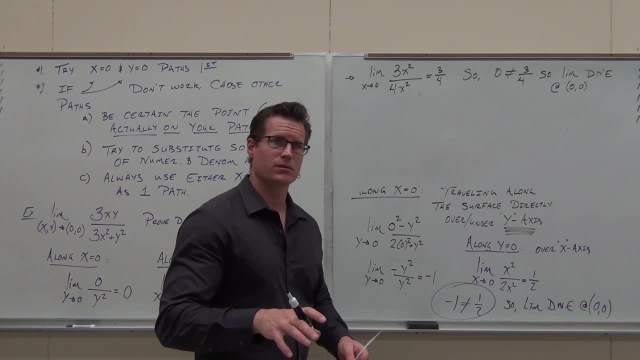 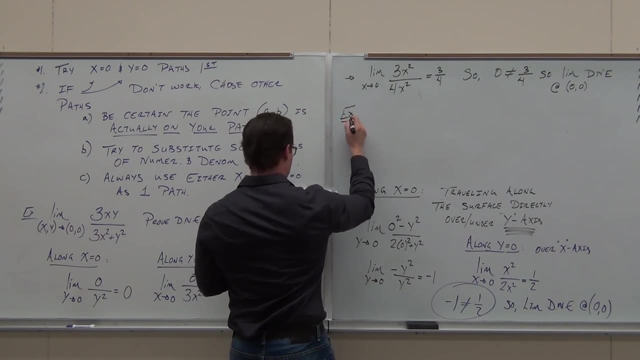 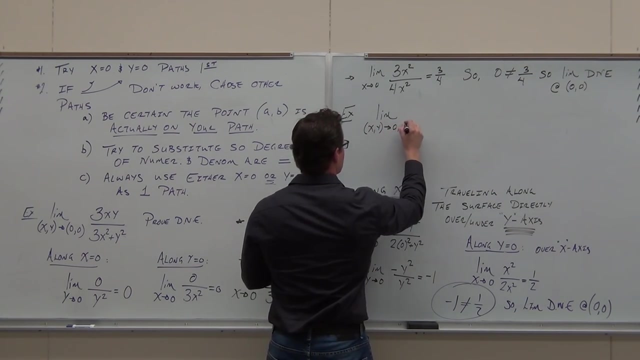 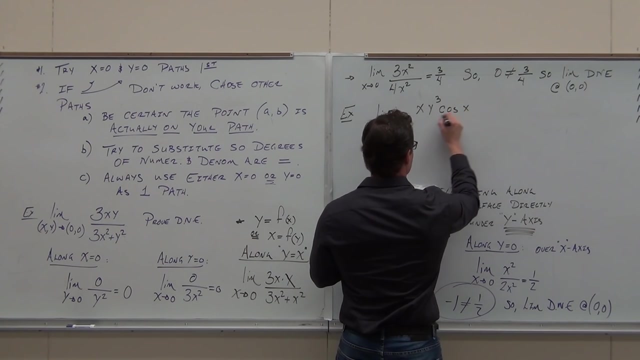 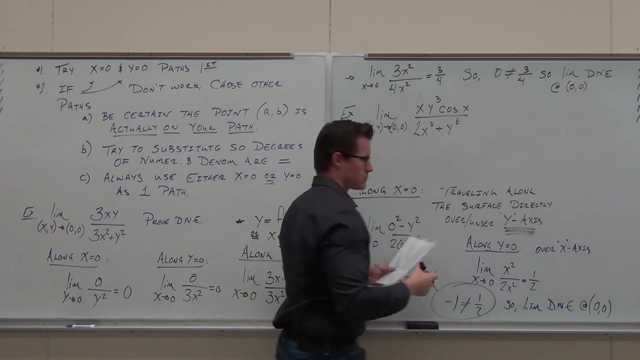 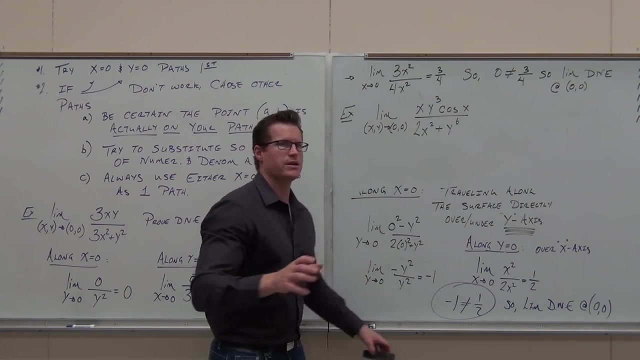 let's try. let's try one more to get tell you what I want you to try. this one your own, at least the first couple steps of it. let's see. so, as I'm erasing, here's what I would like for you to do. I'd like for you to go along. 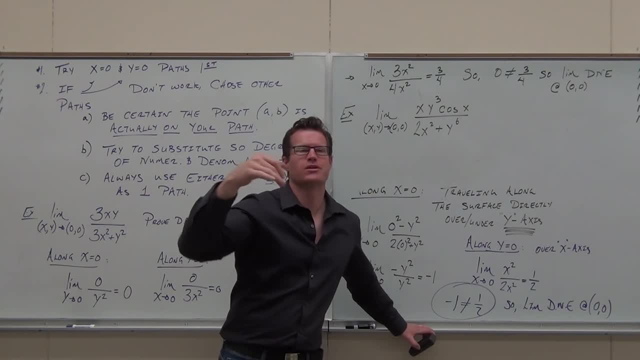 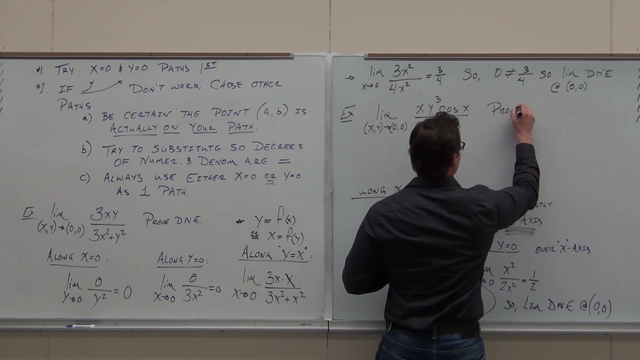 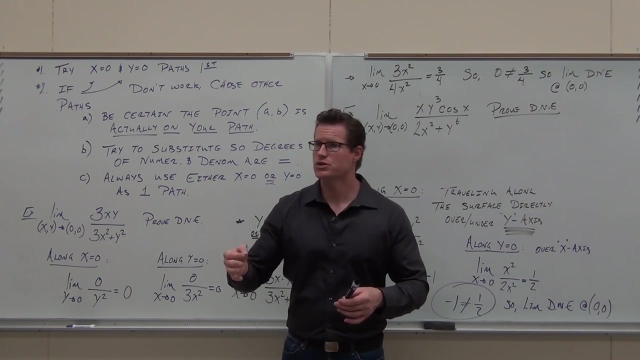 the two paths that we pretty much always start with: okay. well, actually, I want you to plug in the number. what are you gonna get? zero, zero. so that means okay. I want you to prove that this doesn't exist right now. how I want you to start these. I want you to either in your head or write out these: 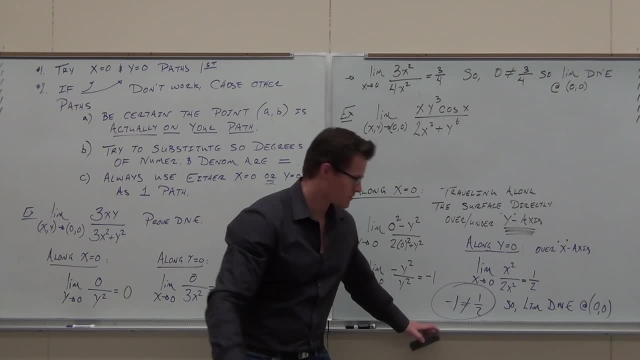 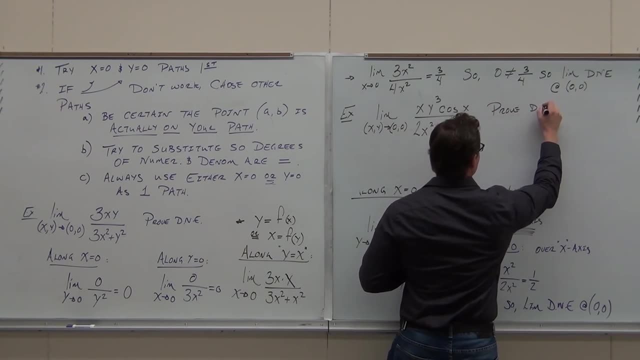 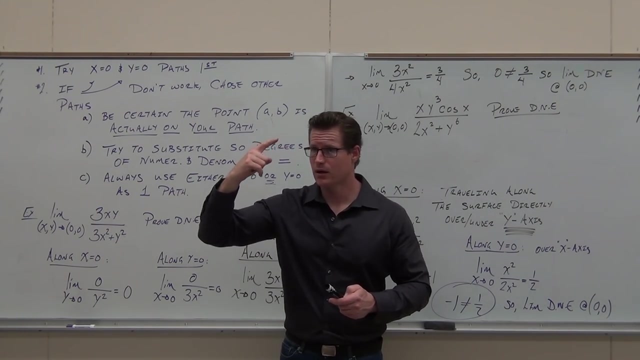 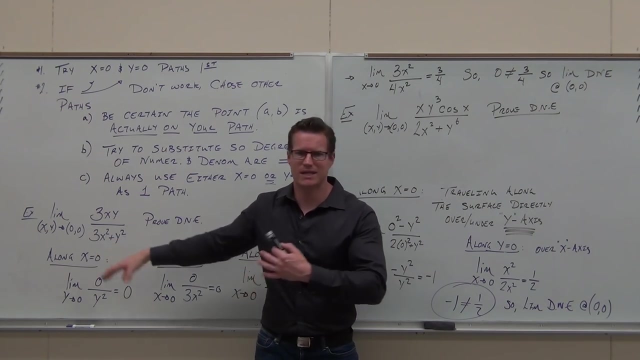 Zero over zero. so that means okay, I want you to prove that this doesn't exist. So right now, how I want you to start these. I want you to either in your head or write out these paths. if you can do it in your head, do it in your head, but you've got to write at least one of them. you always have one of those paths. 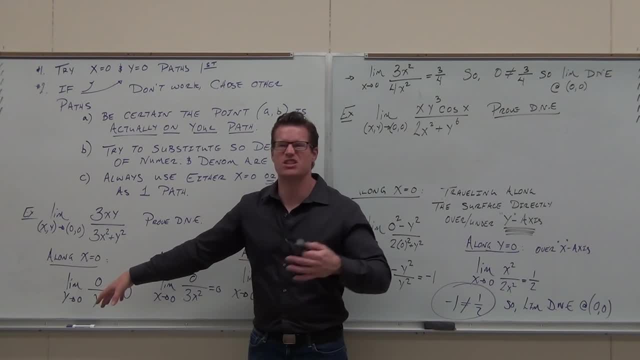 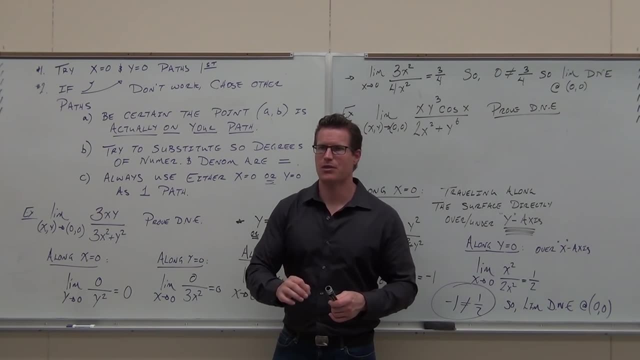 So I'd write this one out and I'd go with x equals zero and see what happens then in your head. or write the y equals zero one: if you've got different numbers, you're done. if you don't, then you've got to pick a different path. that's the hard part here. 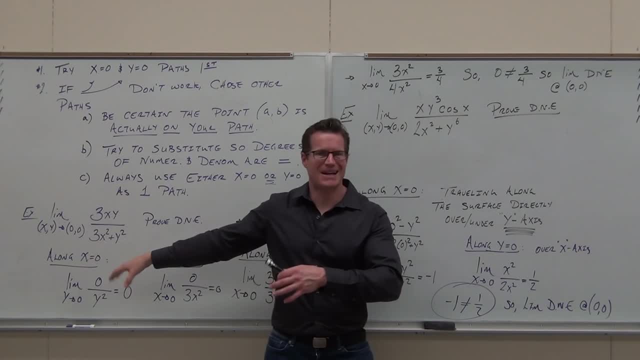 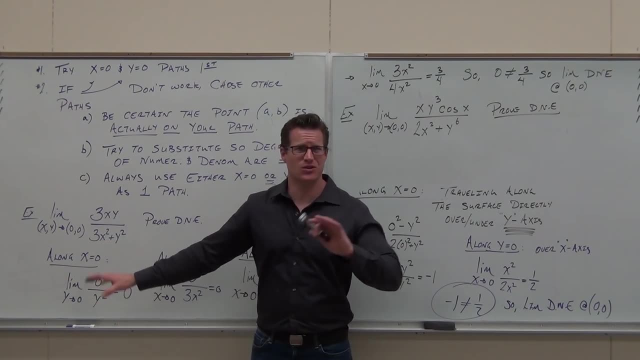 paths. if you can do it in your head, do in your head. but you got to write at least one of them. you always have one of those paths, so I'd write this one out and I'd go with x equals zero and see what happens then in your head. or write the y equals zero one if you got different numbers. 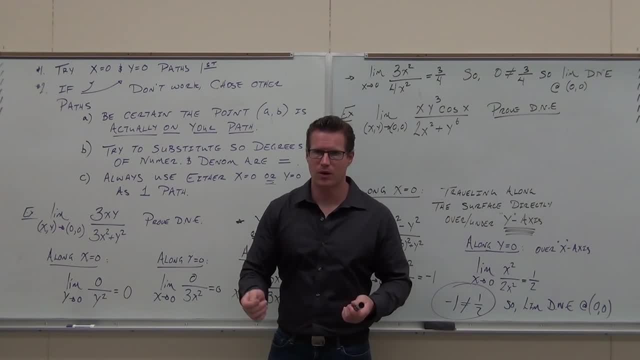 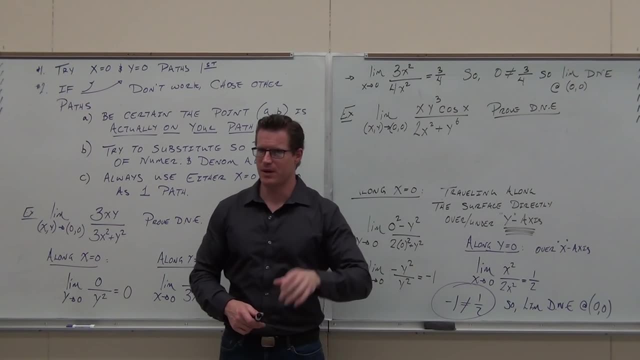 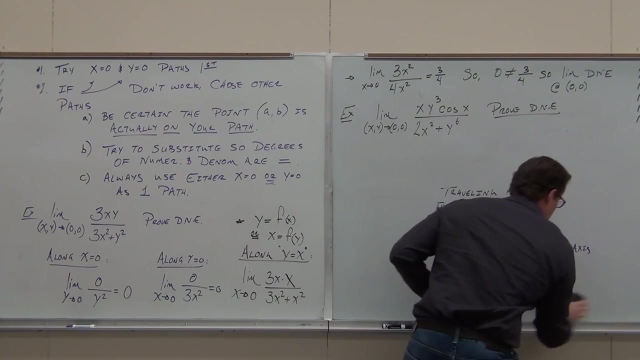 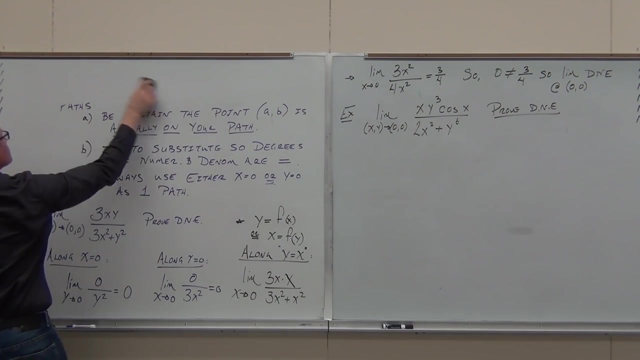 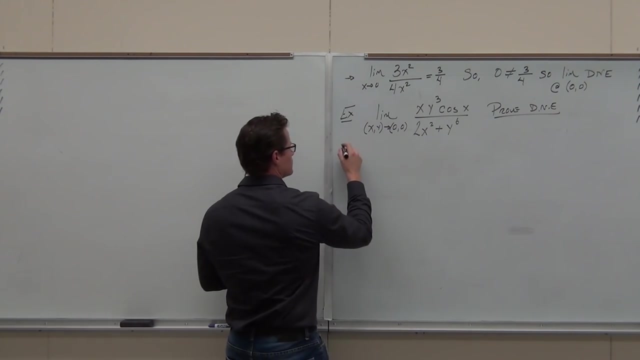 you're done. if you don't, then you got to pick another one and you're done. that's the hard part here. so I want you to try the x equals zero, y equals zero thing, see what you get and then work on finding a different path. all right, so we've got all the paths in there, all. 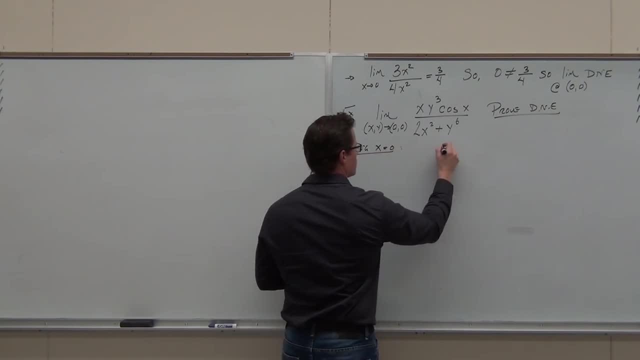 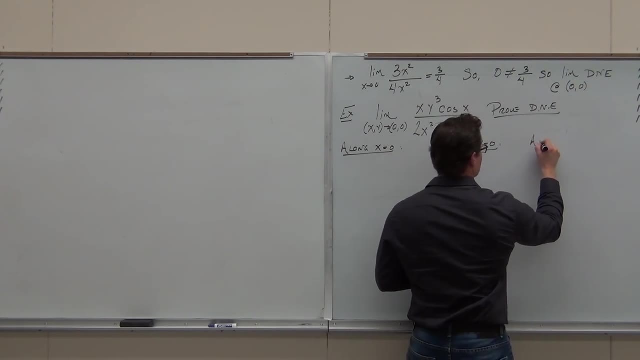 we've got this path coming out, representing the concepts all of us have on them. this would be info number you'll want to be able to type into your notebook. this would be info number. two will help you. my friend will going to write it down. you'd want to come up with a name for that. 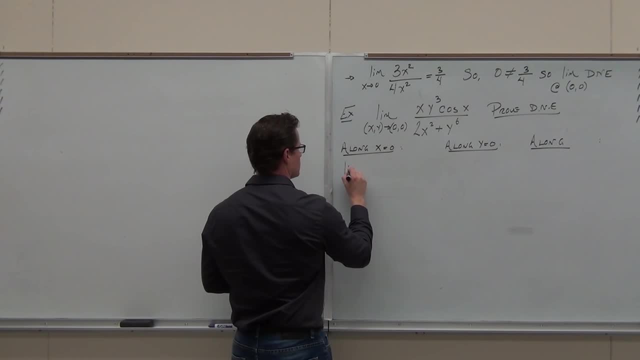 this would be the type if you don't use that name, and it'd make it greater fit if you're going to. yeah, the two at the end with these sheets. so this would quickly over here. tip, this would be an overview of what the loud are over here. okay, my friend. lot of play. don't go over these. one more also easy: create a link here and then you're already done and I've made some abilities out of it, so you'll just gotta start溥 and like me, of course, for the whole thing. that's what I've done, lovely, and I can describe it to you- doing an aff случае. 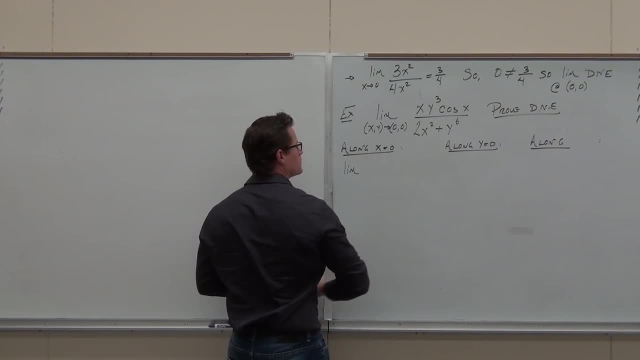 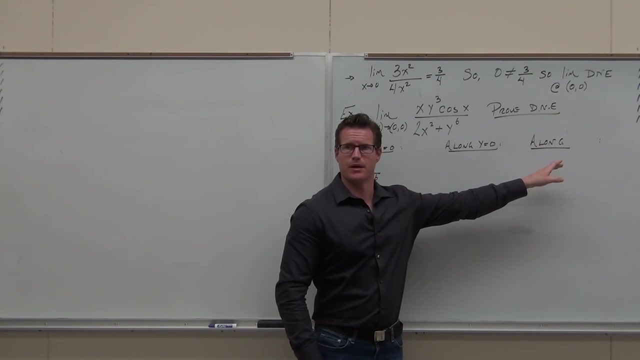 let's just stop for a second. I know you're still working. I know you're probably thinking about that path. right now, at least, I hope you've made it that far. let's think about this: if I let x equal 0, I'm traveling along the y axis. 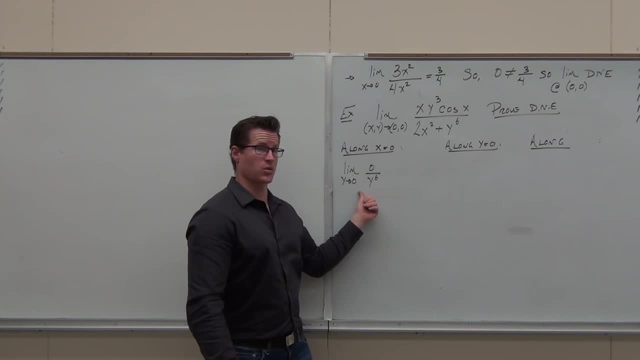 0,. 0 is on the y axis. that's great. I also know that 0 if x is 0, that's 0. the whole thing is 0. if that's 0,, I get y to the 6th and this is 0. 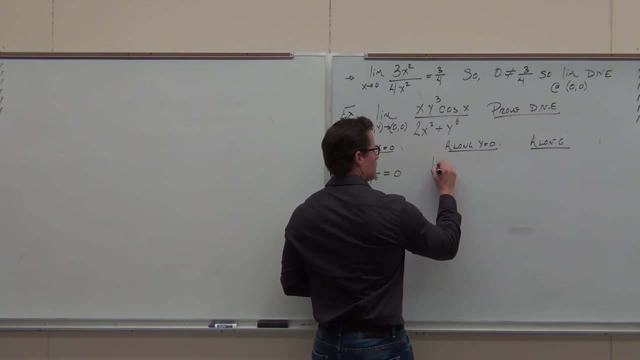 if I let y equal 0, the only independent variable left is x. it still has to probe 0. I know that y equal 0 still contains that point. I know that y equal 0, that's 0, that's 0. we get 2x squared and that's 0. 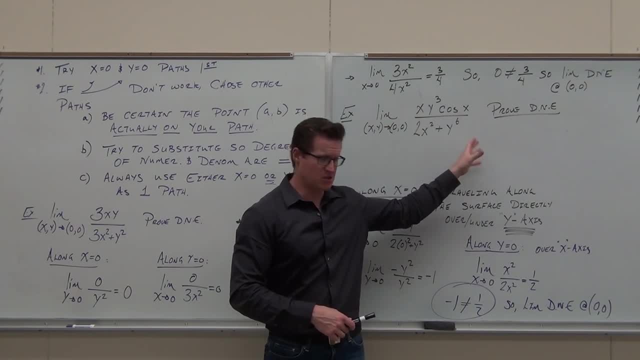 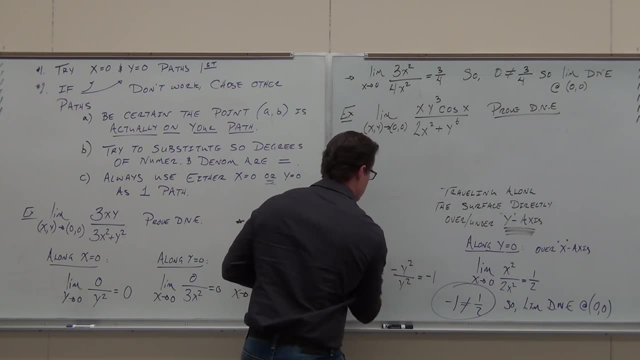 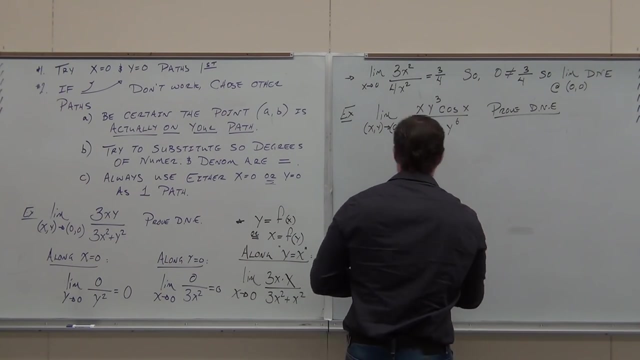 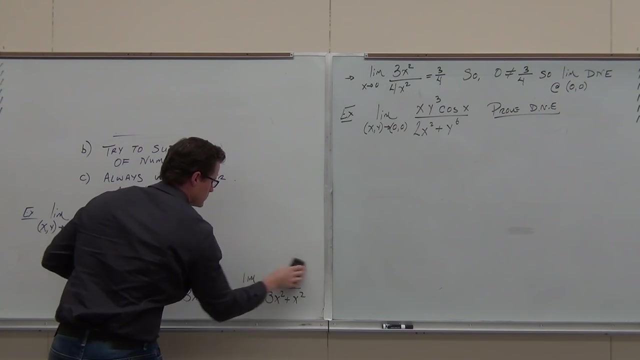 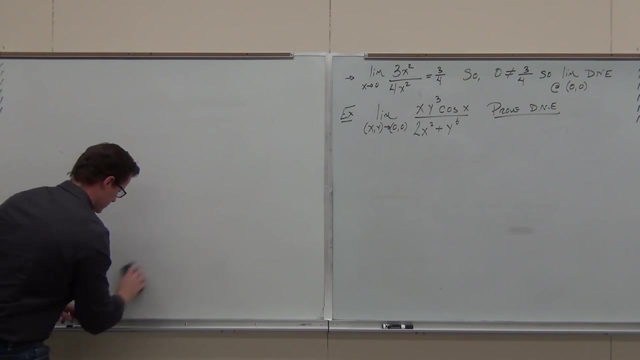 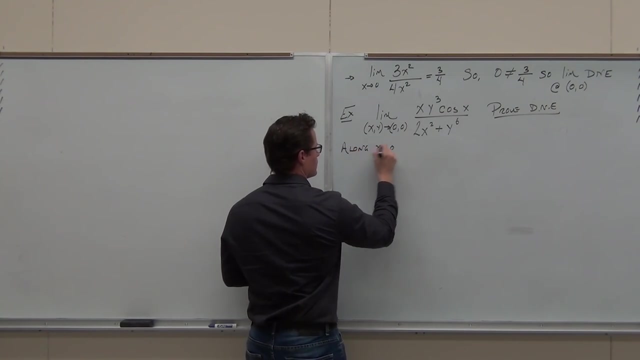 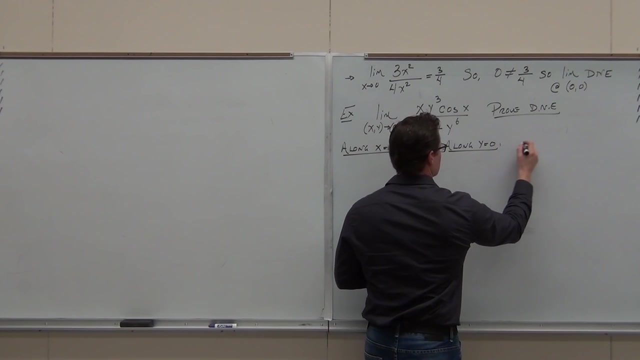 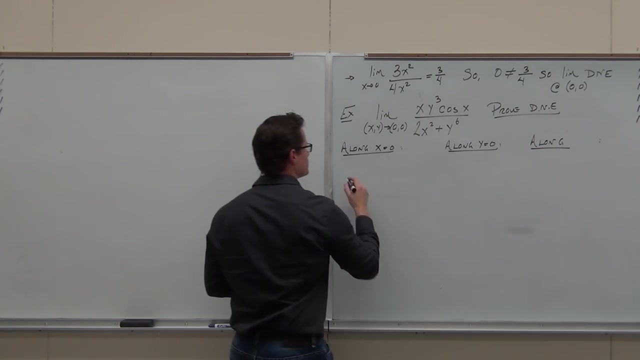 so I want you to try The x equals zero, y equals zero thing. see what you get and then work on finding a different path. Let's see. Let's just stop for a second. I know you're still working. I know you're probably thinking about that path right now. 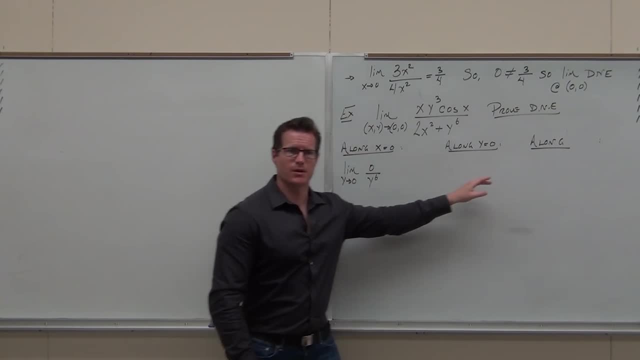 At least I hope you've made it that far so far. Let's think about this: If I let x equal 0, I'm traveling along the y-axis. 0, 0 is on the y-axis, That's great. I also know that. 0, if x is 0, if that's 0, the whole thing is 0.. 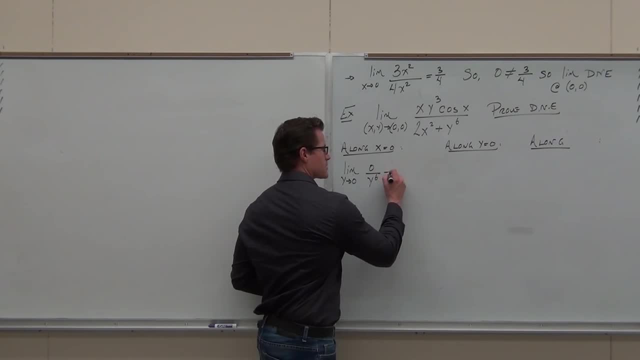 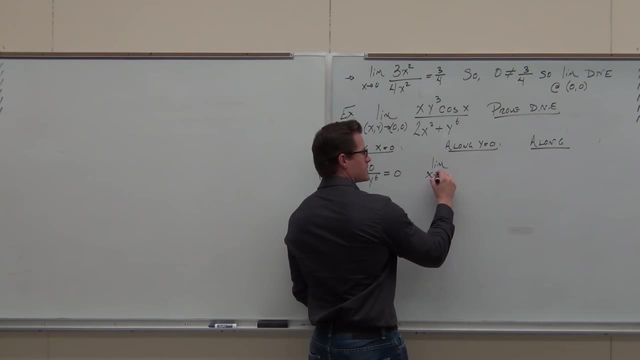 Gone. If that's 0, I get y to the sixth and this is 0.. If I let y equal 0, the only independent variable left is x. It still has to probe 0.. I know that y equals 0. still contains that point. 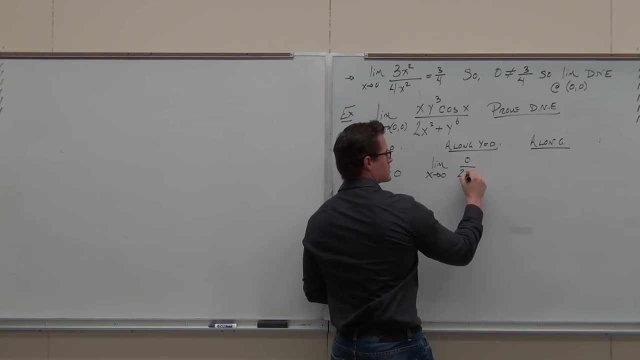 I know that y equals 0, that's 0.. That's 0.. We get 2x squared and that's 0. That does nothing for you. That gives you about 1 point out of 10 on the test. 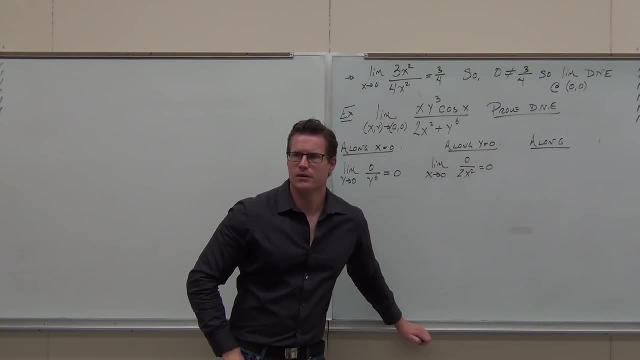 Because what have you done? Literally nothing. You haven't done anything. You haven't proved it exists, You haven't proved it doesn't exist. You've done nothing. So along, let's pick another point and let's do this: 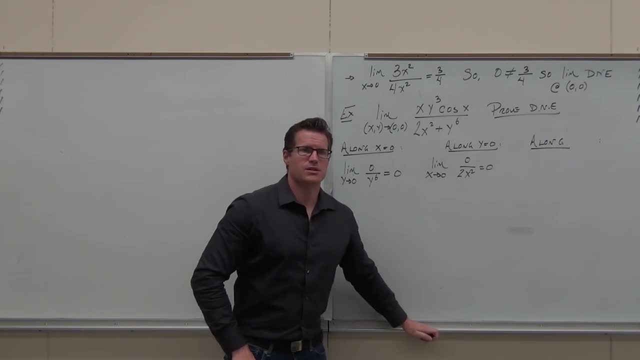 Let's try to pick a substitution that not only contains this point but makes the degrees the same, if we can. That's what I want to do, So let's see how to do that. If we're going to try to make the degrees the same, here's a little hint I'd like to. 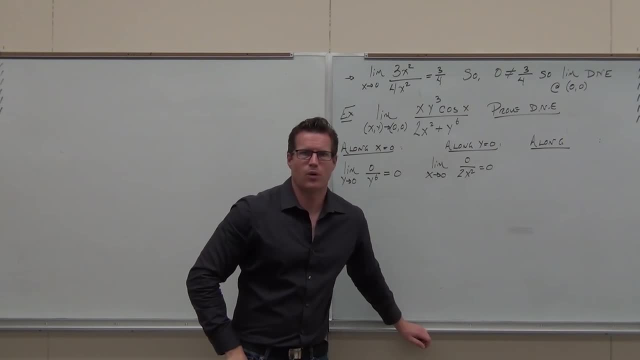 that does nothing for you. that gives you about 1 point out of 10 on a test. because what have you done? literally nothing. you haven't done anything. you haven't proved it exists. you haven't proved it doesn't exist. you've done nothing, so along. 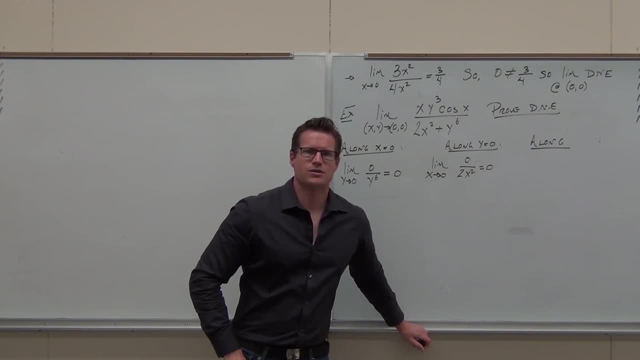 let's pick another point. let's do this. let's try to pick a substitution that not only contains this point but makes the degrees the same. if we can, that's what I want to do, so let's see how to do that. if we're going to try to make the degrees the same, 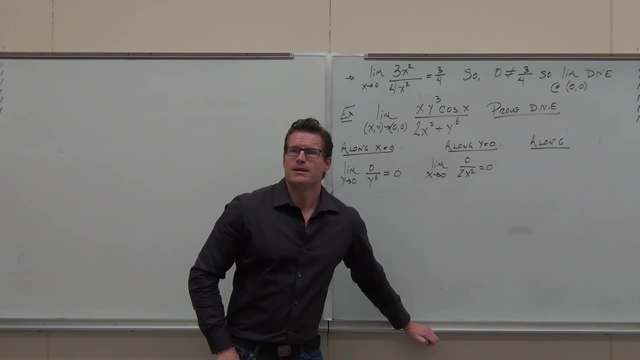 here's a little hint I'd like to write down. maybe you should know this. maybe you should write it down. take the variable with the smaller degree and try to make it into the variable with the larger degree. otherwise it's kind of hard, because if I want to change 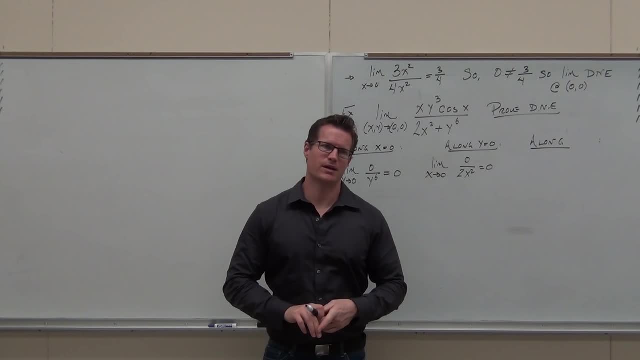 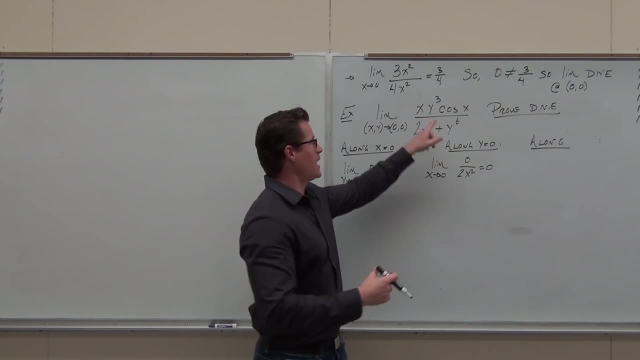 well, what's got the larger degrees here, x's or y's, y's do. if I try to change y's into x's, I'm going to have to cut powers. does that make sense? it's hard, it's easier to grow powers. so if I say I want x to equal something in y, 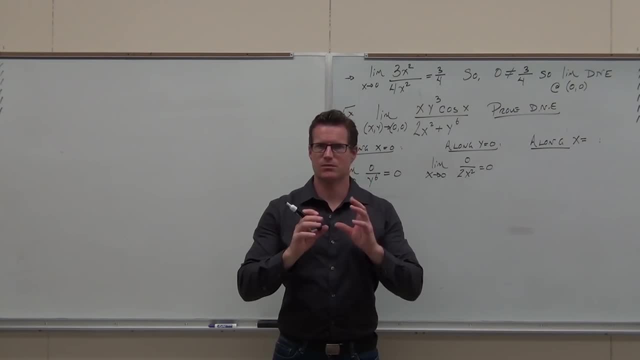 such that the variables have the same value as x and y the same degree. can you see the substitution right now? what is it? x equals 1 to the 3rd. good, so I'm going to take the smaller degree variable and try to change it into having that power. 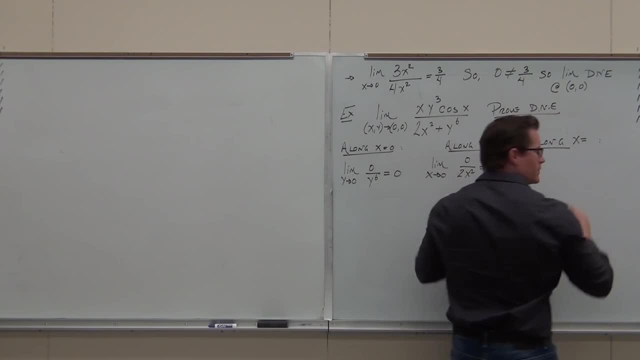 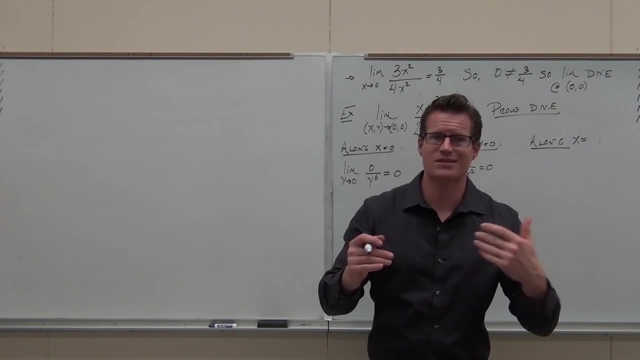 so if I say I want x to be equal to, did you guys get the concept that I'm going to have to eliminate a variable right? because I can't do this stuff in two variables very easily. so I'm going to have to eliminate one. so I'm going to change x's into y's. 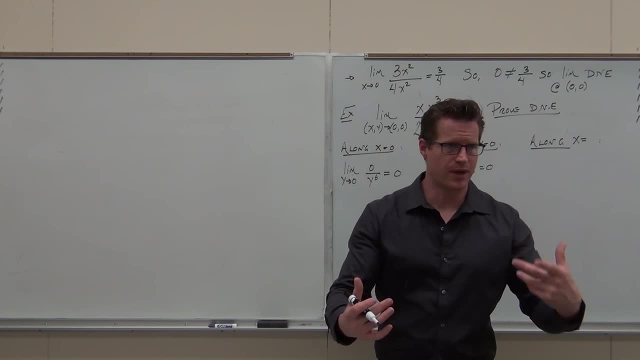 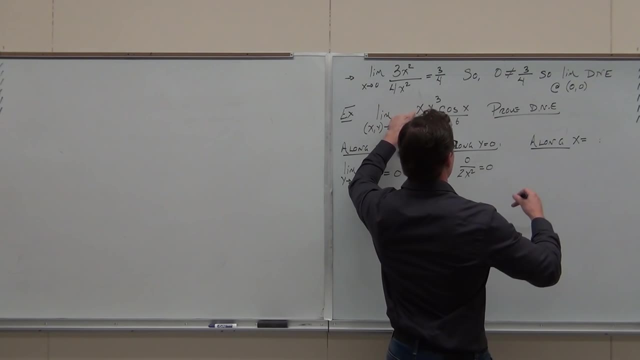 or y's into x's. I also want to do it so that my degrees become the same, because the limits are way easier that way. the limits, you just basically cover them up. so I'm going to say, hey, let's go along the path. x equals y to the 3rd. 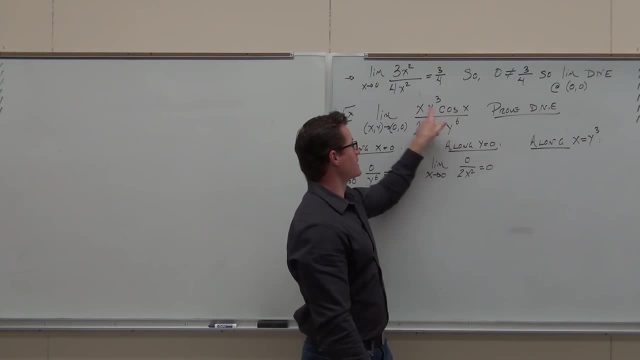 do you see why we might want to do that if I let x? if this is a y to the 3rd, that's y to the 6th. if that's a y to the 3rd, that's y to the 6th. 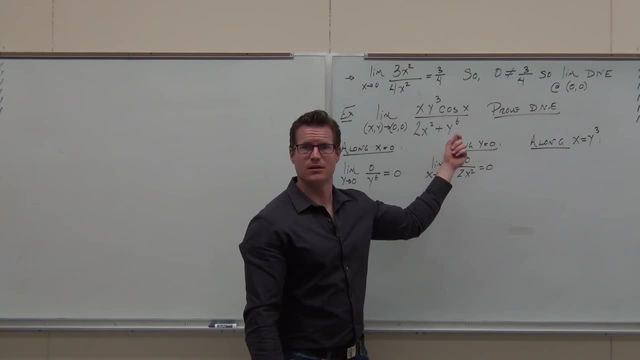 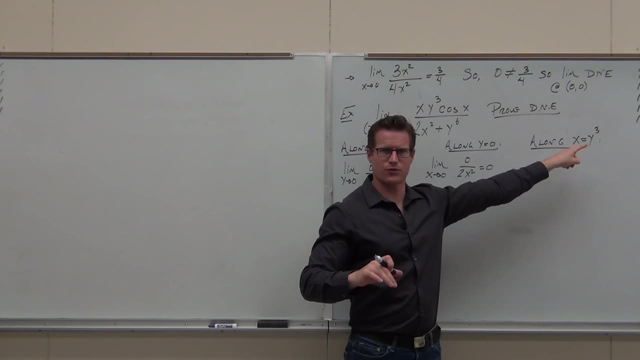 and I can add them and then it's very nice, very easy. so it makes me feel okay with that one also. one more thing you've got to double check: this is 0, 0 on that curve. notice, it is actually a curve, right. 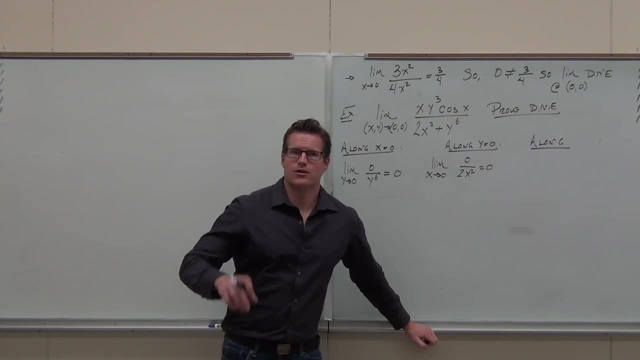 write down. Take the variable with the smaller degree and try to make it into the variable with the larger degree. Otherwise it's kind of hard because if I want to change, well what's got the larger degrees here, X's or y's? 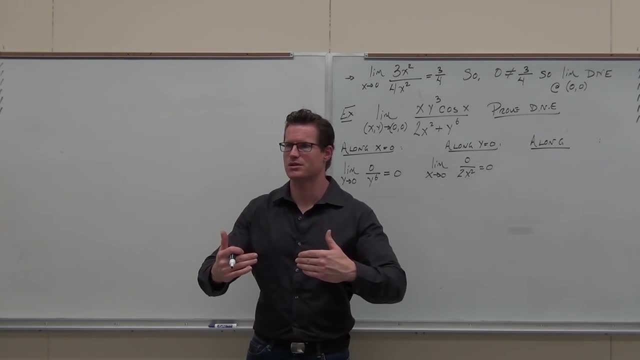 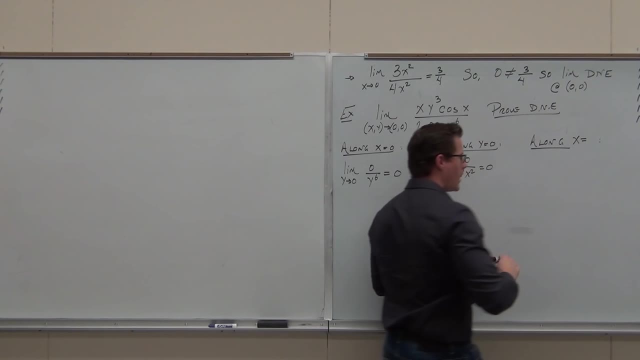 Y's, Y's do. If I try to change y's into x's, I'm going to have to cut powers. Does that make sense? It's hard. It's easier to grow powers. So if I say I want x to equal something in y, such that the variables have the same, 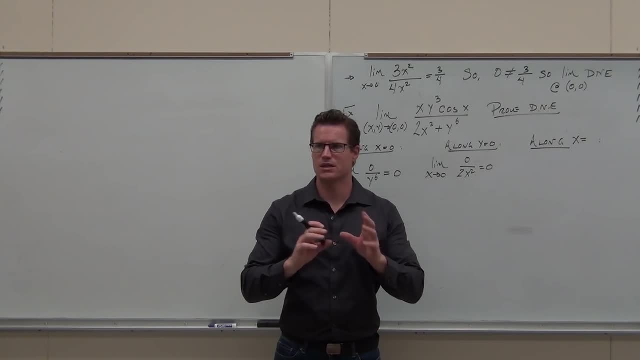 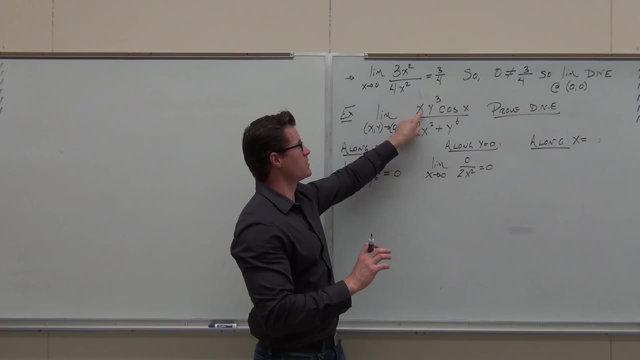 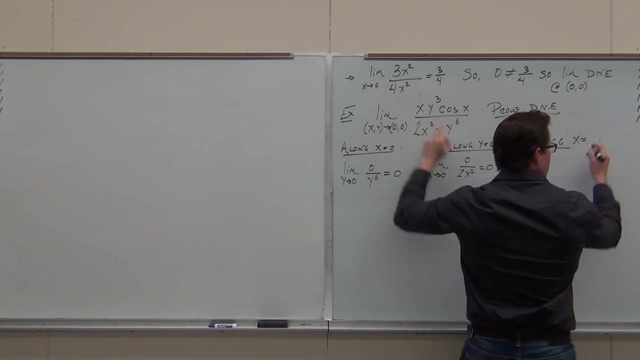 the variables have the same degree. Can you see the substitution right now? What is it Good? So I'm going to take the smaller degree variable and try to change it into having that power. So if I say I want x to be equal to, did you guys get the concept that I'm going to have? 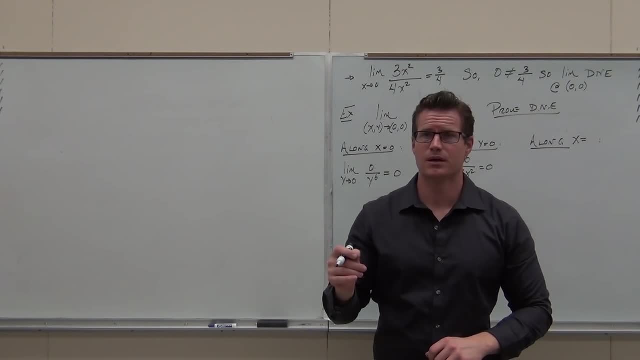 to eliminate a variable, right? Because I can't do this stuff with two variables very easily. So I'm going to have to eliminate one. So I'm going to change x's into y's or y's into x's. I also want to do it so that my degrees are the same. 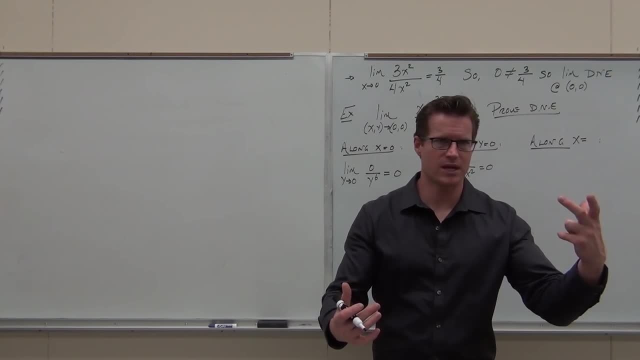 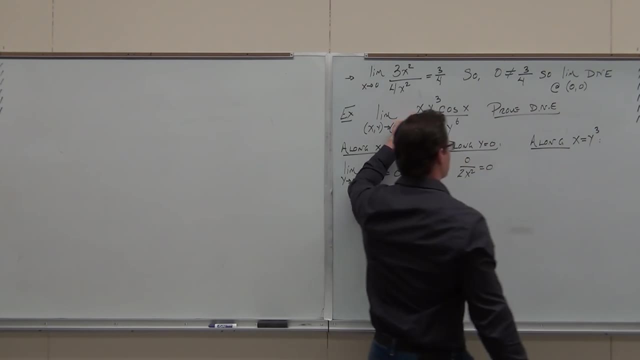 Okay, So my degrees become the same because the limits are way easier. that way, The limits, you just basically cover them up. So I'm going to say, hey, let's go along the path. x equals y to the third. Do you see why we might want to do that? 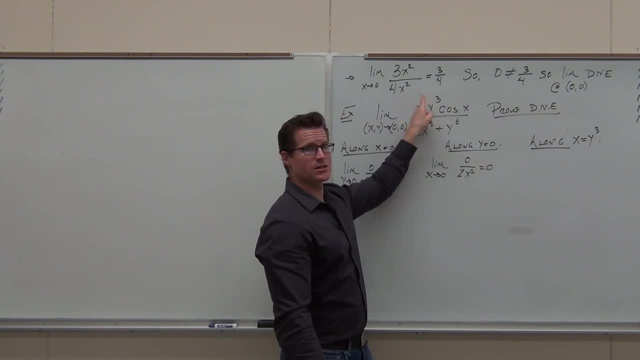 If I let x, if this is a y to the third, that's y to the sixth. If that's a y to the third, that's y to the sixth, and I can add them, And then it's very nice, very easy. 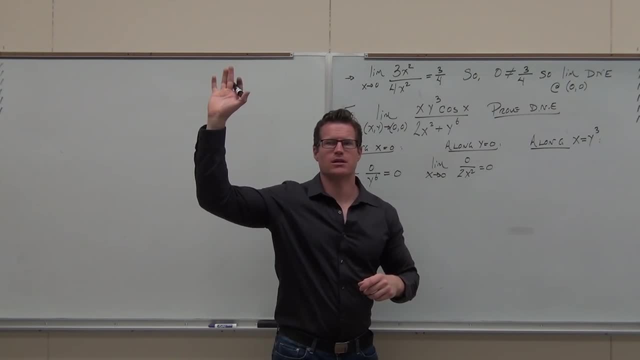 So things will be okay with that one. Also, one more thing You've got to double check. this Is 0, 0 on that curve. Notice it is actually a curve right now. It's not a line, It's a curve through space. 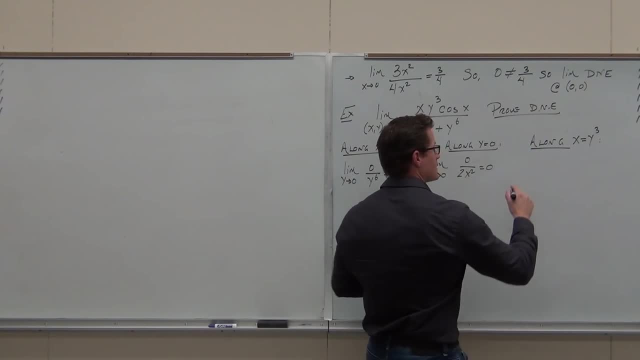 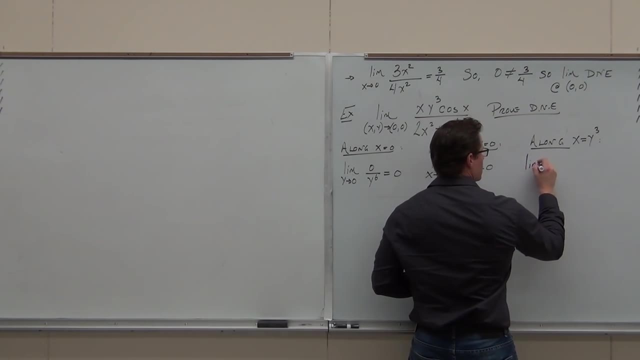 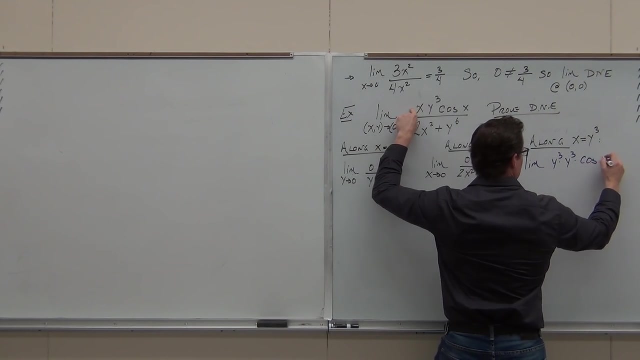 Is it on that curve? Yes, 0 equals 0? Done. So that says that if we let all x's change to y's, y to the third's, then this is y to the third times, y to the third times, cosine y to the third. 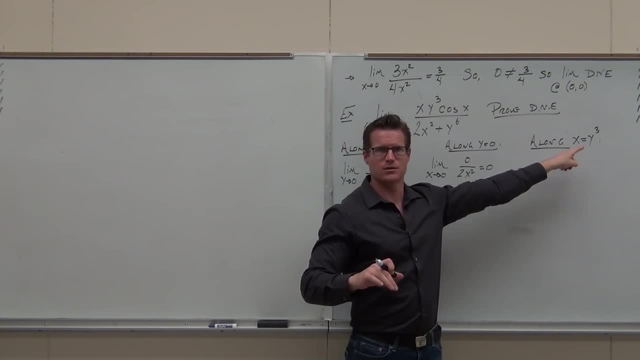 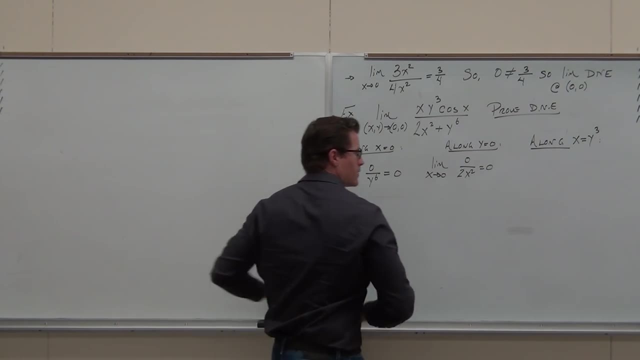 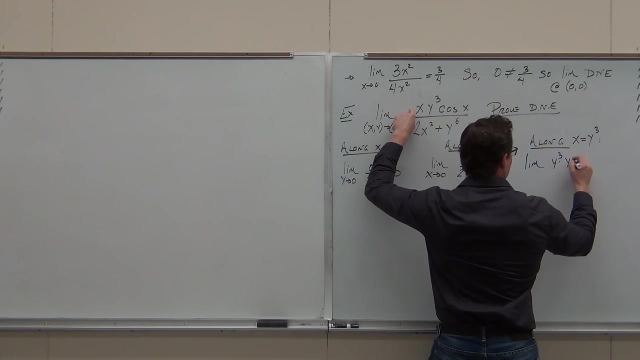 now, it's not a line, it's a curve through space. is it? on that curve, 0 equals 0? done so that says that if we let all x's change to y's- y to the 3rd- then this is y to the 3rd. 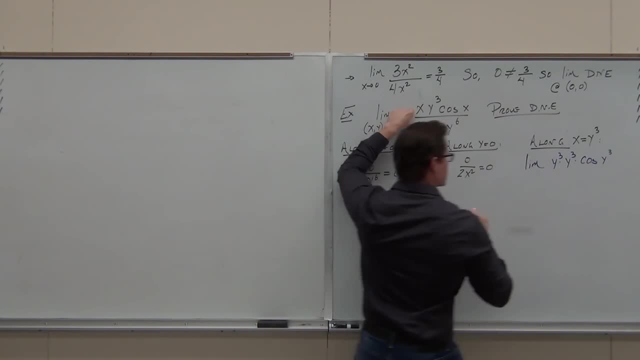 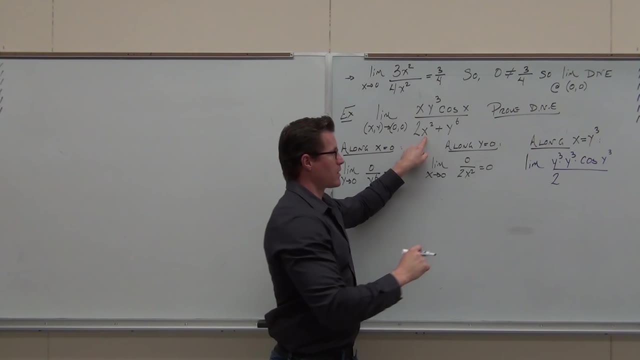 times y to the 3rd times. cosine y to the 3rd, x was y to the 3rd, now x is y to the 3rd. now, if x is y to the 3rd, I get y to the 3rd, y to the 3rd squared. 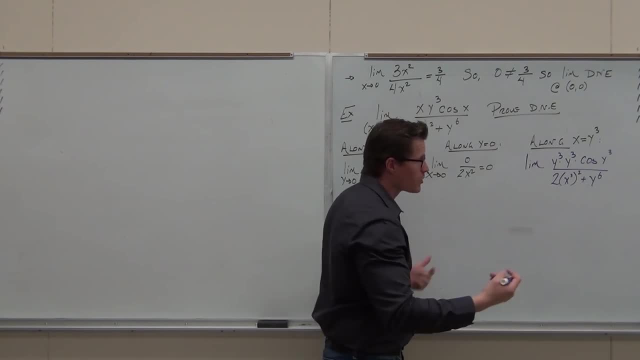 plus y to the 6th, what's the only independent variable left? so let's let that y go to where it's supposed to go to for real show of hands, if you're okay with that one. it's kind of a weird one. are you guys back there, okay with it? 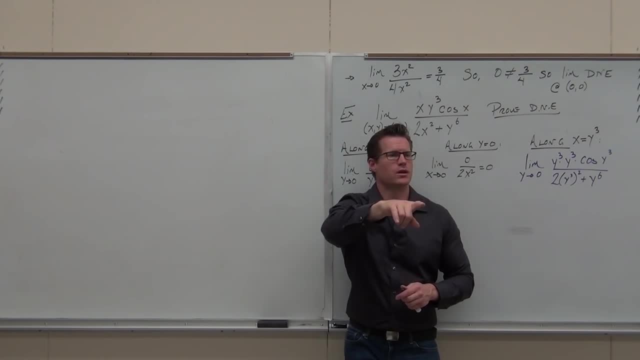 you sure, right side, I don't want to lose you. we spent too much time doing this for me to just lose you now. this should be the kind of funner stuff, interestiner stuff. that's a word. can you simplify it? let's try. 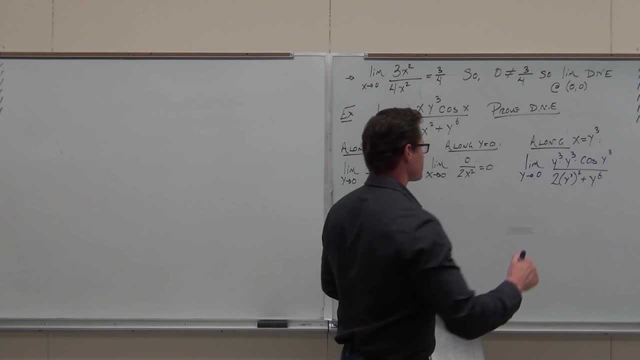 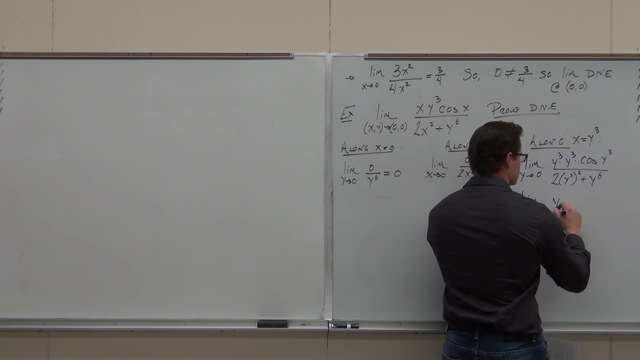 how much? what is 6?? what is 6?? this is 2y to the 6th plus 1y to the 6th plus 2y to the 6th plus 1y to the 6th plus 1y to the 6th. 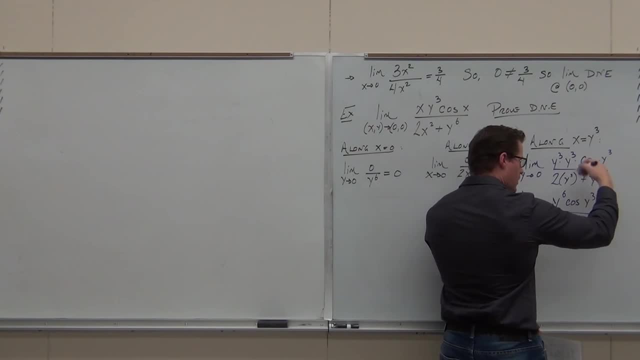 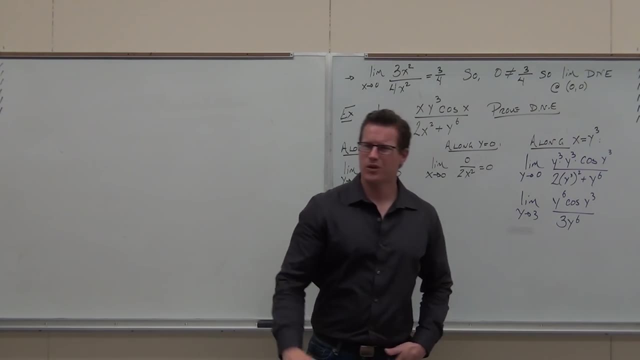 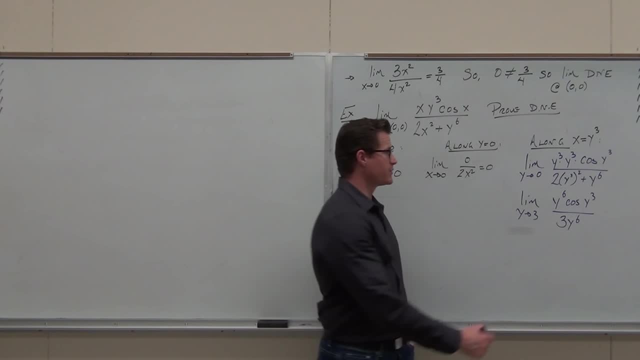 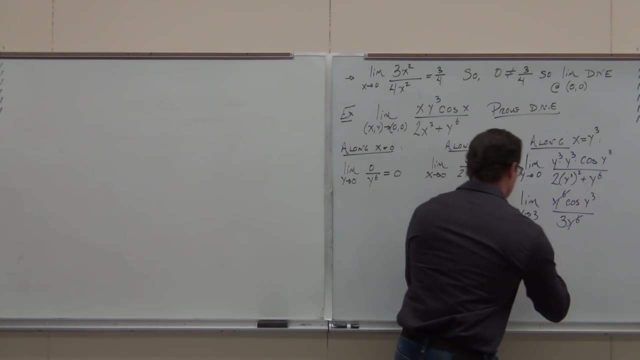 Ladies and gentlemen, this is why we try to make the degrees the same, Because, if we can, we can do some basic basic math operations Gone, Get them gone. That's great. Oh my gosh, I'm sorry. Why, why? 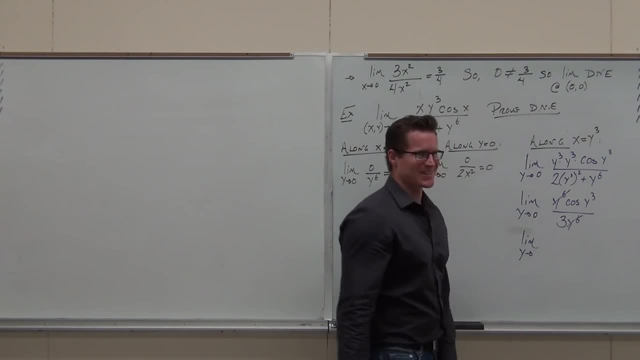 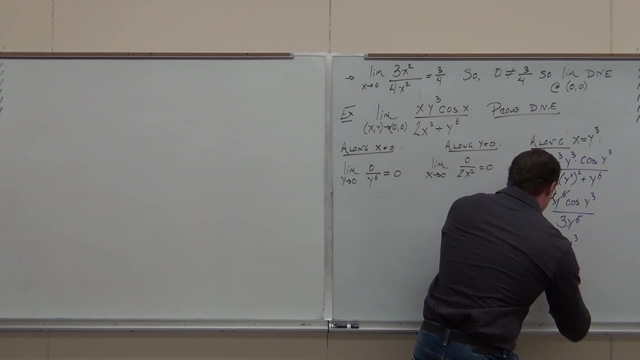 Why do you people- let me do that, Goodness gracious, I just like 3's today, I don't know- Wrote so many of them? that's why. So we're left with cosine y to the 3rd over 3.. 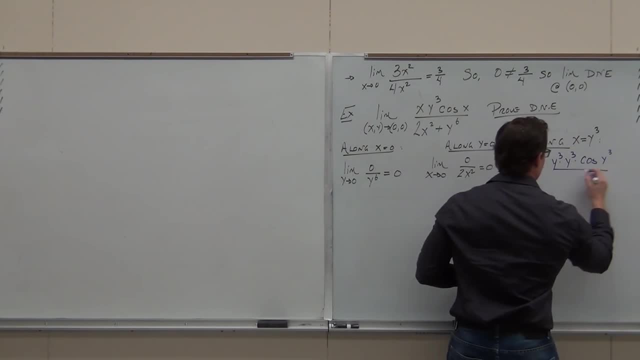 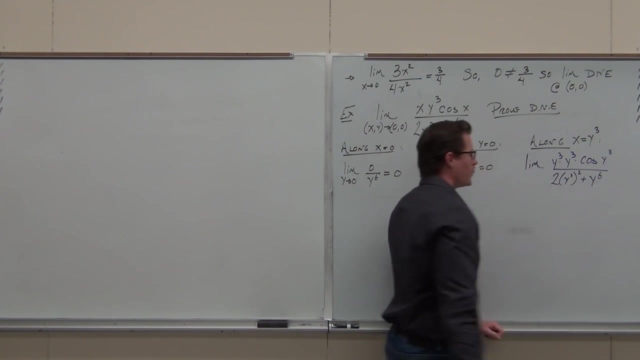 X was y to the third. now X is y to the third. now, Okay, So y to the third. I get y to the third squared plus y to the sixth. What's the only independent variable left? So let's let that y go to where it's supposed to go to. 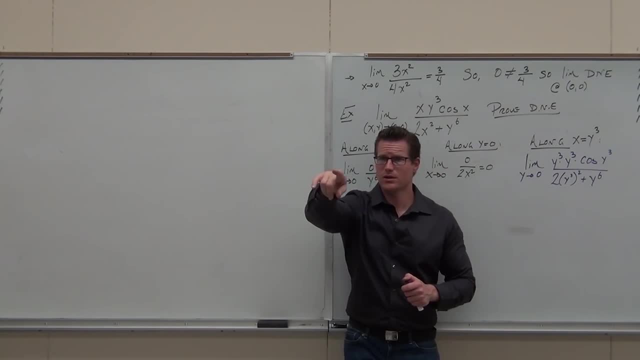 For real show of hands, if you're okay with that one. It's kind of a weird one. Are you guys back there okay with it? Are you sure? Right side, I don't want to lose you. Okay, We spent too much time doing this. 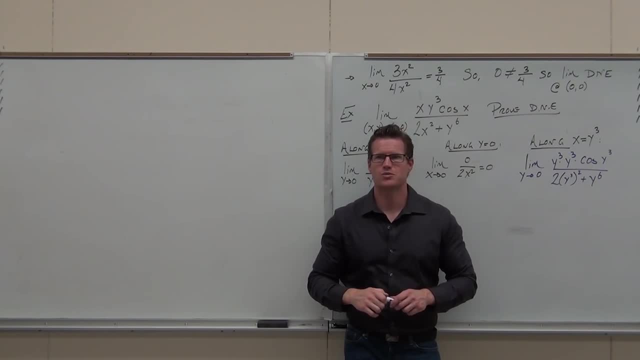 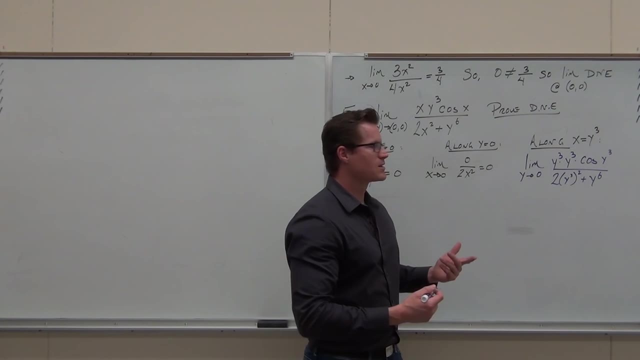 We're going to do it again. I don't want to waste too much time doing this. for me to just lose you now. This would be the kind of funner stuff: interest in your stuff. It's a word. Can you simplify it? 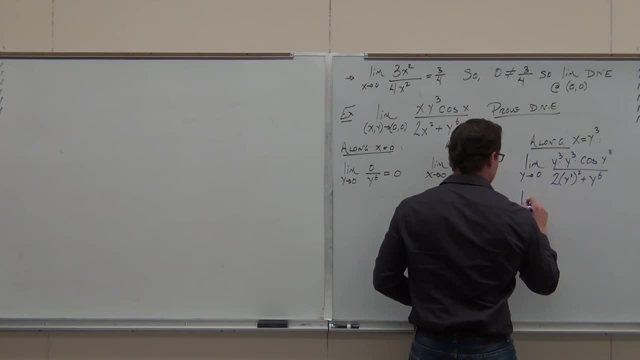 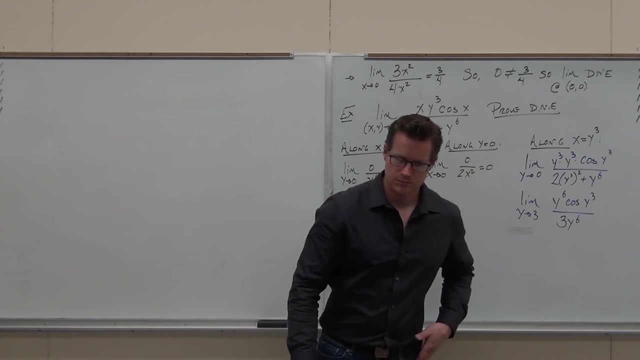 Let's try How much. What is this? This is 2y to the sixth plus y to the sixth Plus 1y to the sixth. we get 3y to the sixth With me. Yeah, No, Can you simplify that? 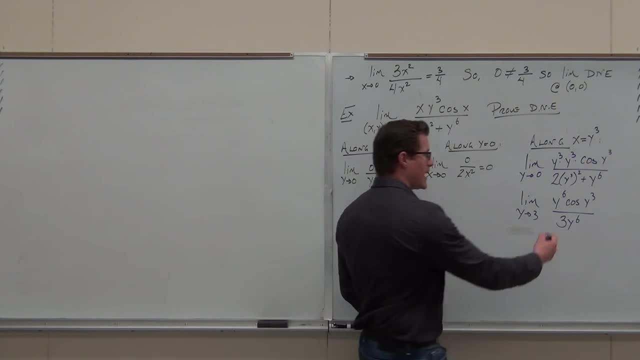 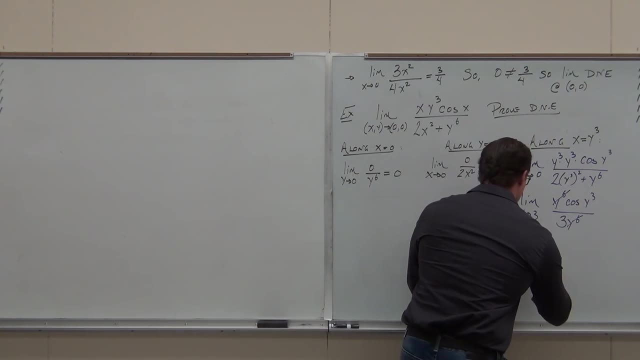 Ladies and gentlemen, this is why we try to make the degrees the same, Because, if we can, we can do some basic basic math operations Gone, Get them gone, That's great. Oh my gosh, I'm sorry Why? 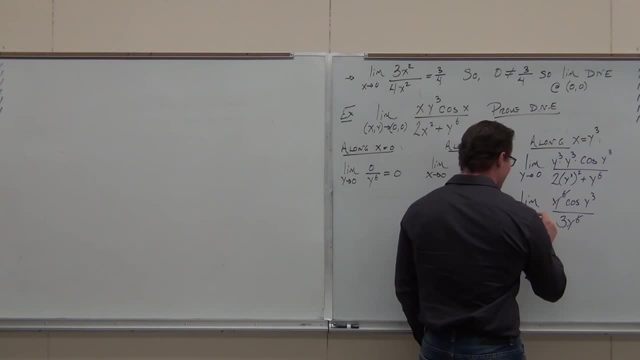 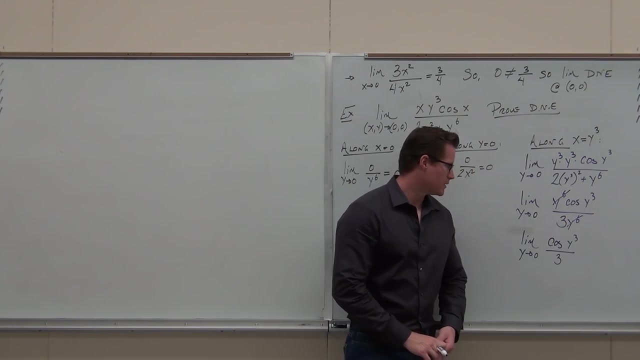 Why? Why do you people- let me do that, Goodness gracious. Yeah, I just like threes today, I don't know Wrote so many of them, that's why. So we're left with cosine y to the third over 3.. 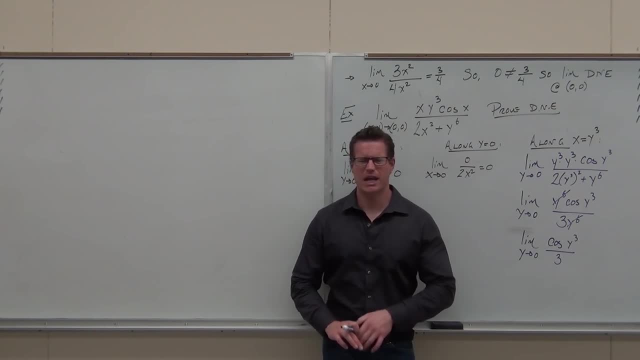 What do you do every time in Calc 1 when you do anything with a limit? What do you try, over and over and over again. What do you try now? Plug it in. Plug it in. Hey, what's y to the third if y is 0?? 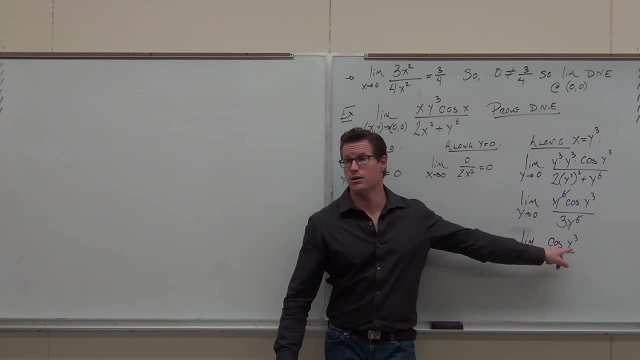 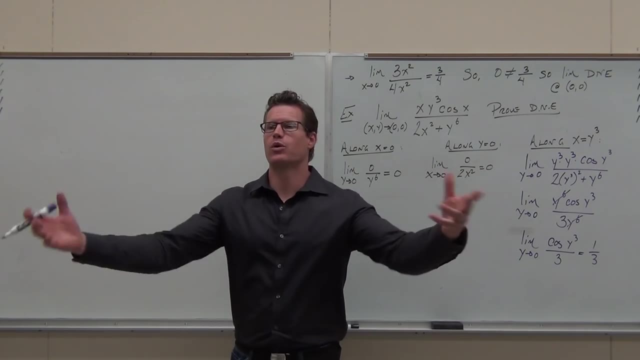 0.. What's cosine of Of 0.. 0.. Does that prove anything? Yes, Everyone. what's it prove? The line limit is not Why. Why? Because along those two paths, this one, a curve along the xy plane which we're floating. 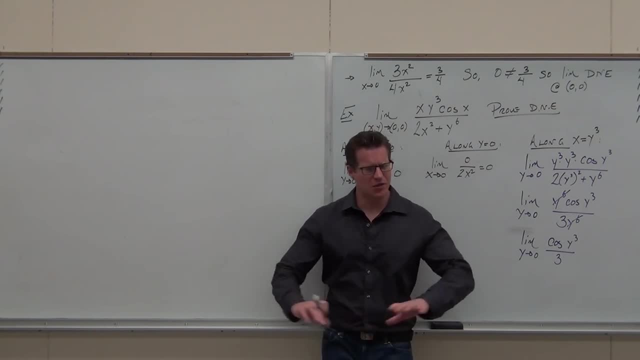 What do you do every time in calc 1, when you do anything with a limit? What do you try, over and over and over again. What do you try now? Plug it in. Plug it in. Hey, what's y to the 3rd if y is 0?? 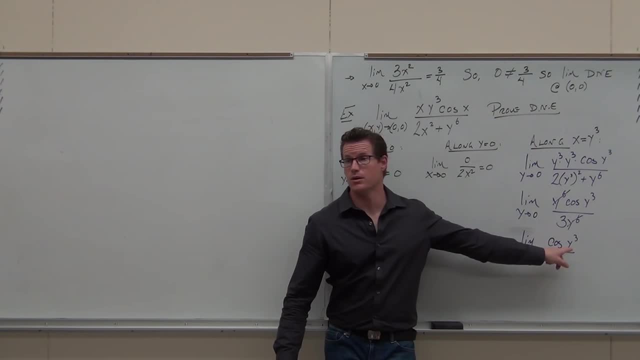 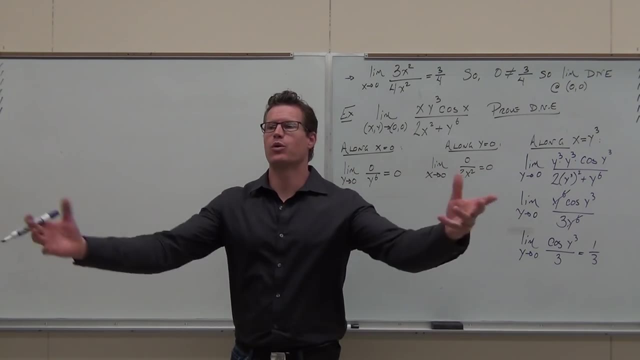 0.. What's cosine 0. 0.. What? 0. 0. 0. 0.. Does that prove anything, Everyone? what's it prove? Why? Why? Because, along those two paths, this one, 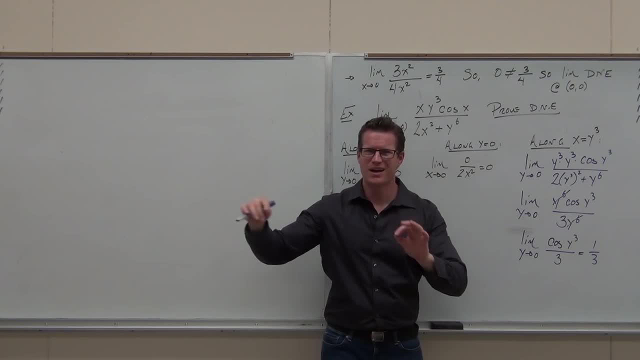 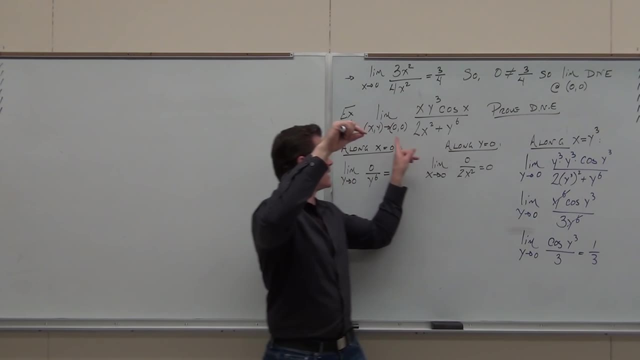 a curve along the xy plane which we're floating on. this is weird, right? This is like an s curve. So we're floating on the surface above that s curve And we're getting to this value, that point, We're getting to that value. 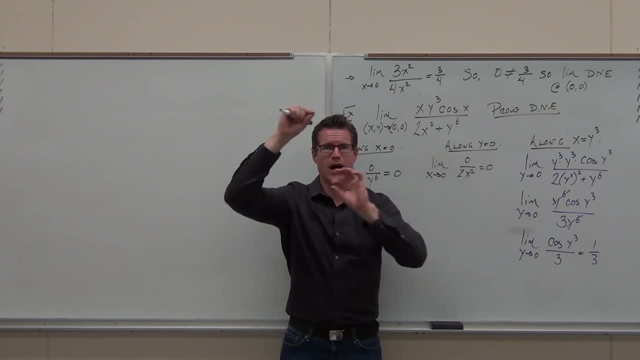 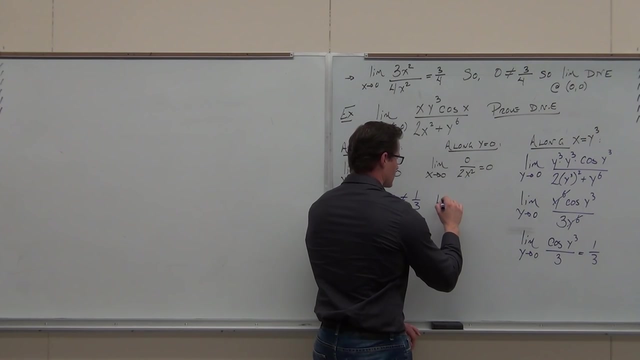 And then we're right above either one of these axes and we're getting to a different value. So the height of the surface is a different value as I'm approaching along the surface over those two curves. So since 0 does not equal 1, 3rd limit does not exist. 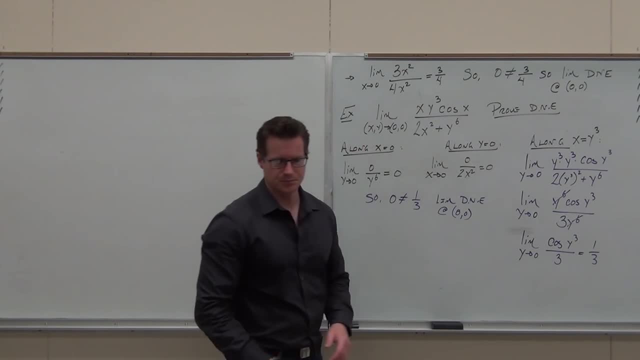 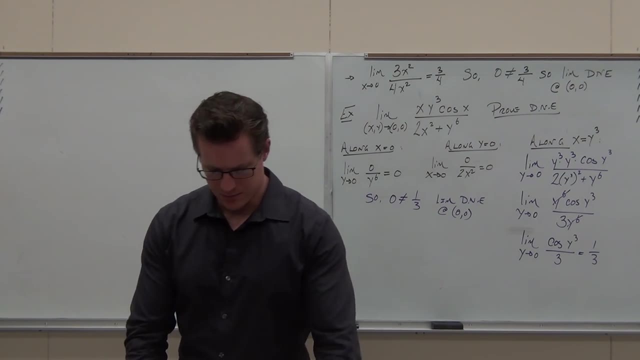 At that point. Yeah, yes, no, Okay, I'll tell you what One more I'm going to. I'm basically just going to do this one for you. I'm going to talk through it just to show you some weird things that can happen. 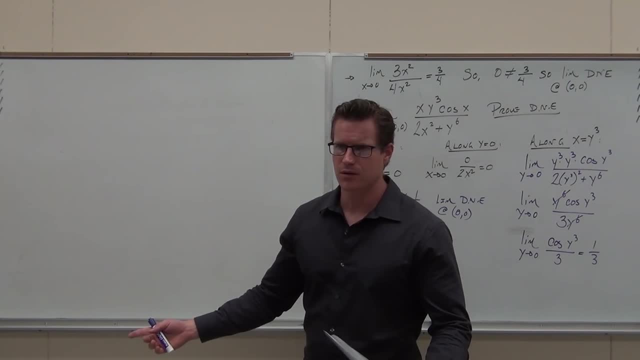 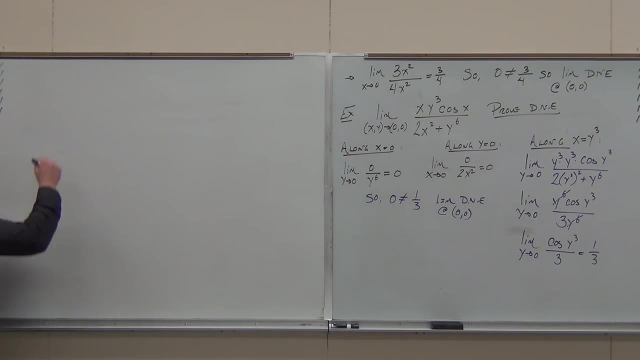 Because this doesn't tell the whole story. We're not always going to 0, 0.. Your substitution is not always going to be x equals y or y equals x. It's not how it is all the time. So I want to do one more, at least to give you that. 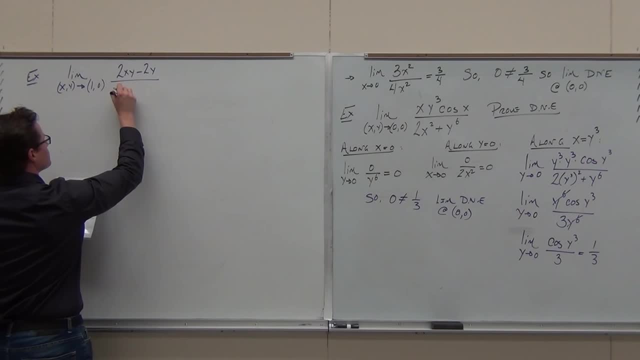 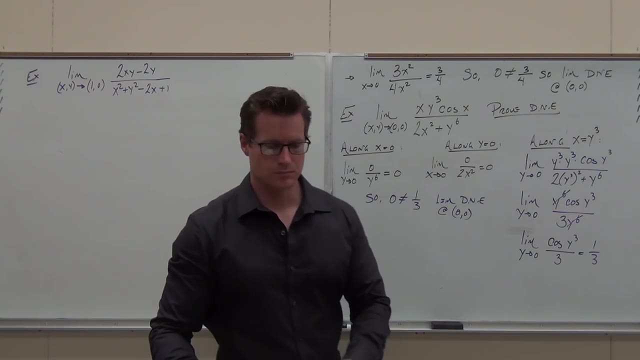 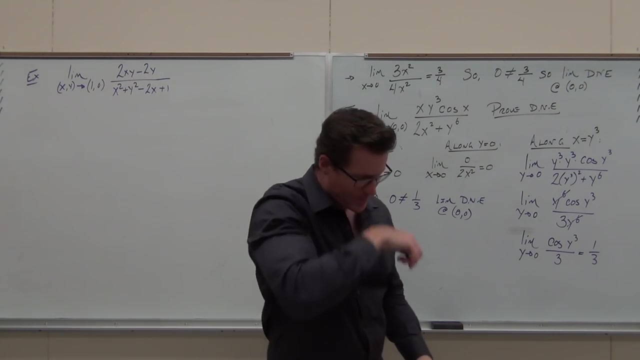 Okay, Let's see, Because this is some like. I don't just think that I'm maybe not going to take this. I'm just going to put it at the first of the limits so we can see how it acts. Okay. 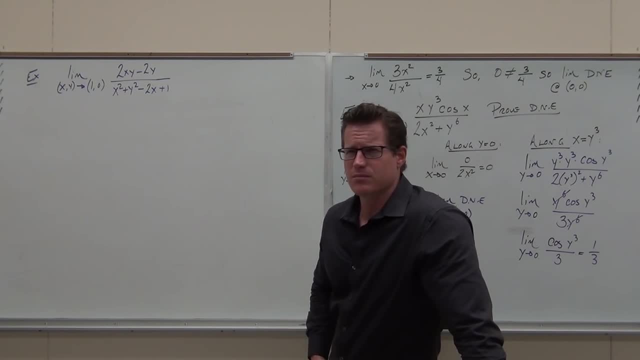 That's one word. Okay, Ill lines x and this is y and this is X here You see that. Yeah, you see for a second that we're going to get 0 over 0.. Act as 1, so that's well in the numerator we get 0, 0.. 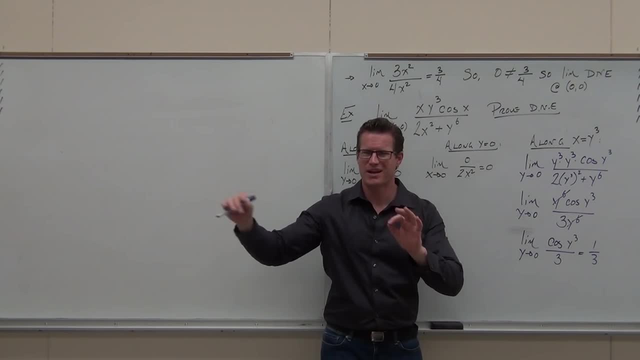 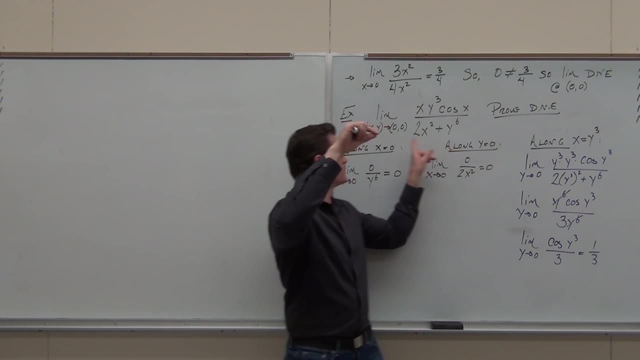 on the. this is weird, right? This is like S curve. So we're floating on the surface above the S curve And we're getting to this value, that point We're getting to that value, And then we're right above either one of these axes. 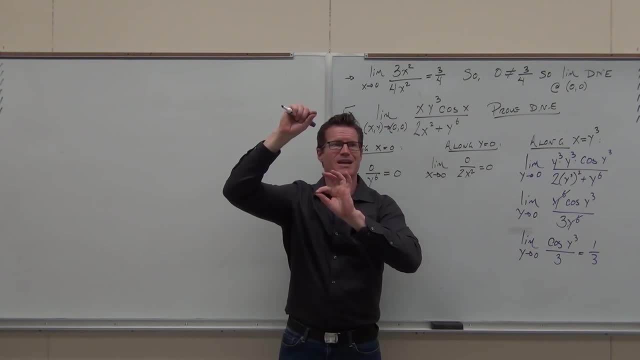 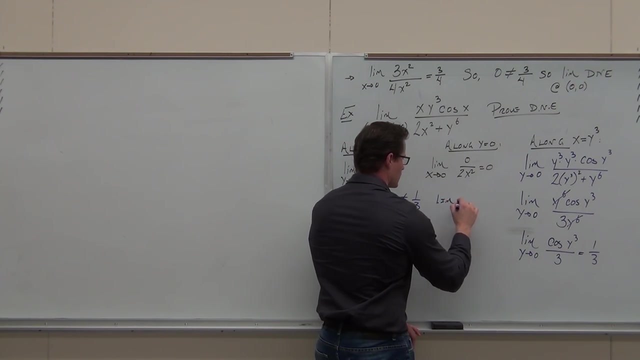 And we're getting to a different value. So the height of the surface is a different value as I'm approaching along the surface over those two curves. So since 0 does not equal 1, third limit does not exist at that point. Yes, 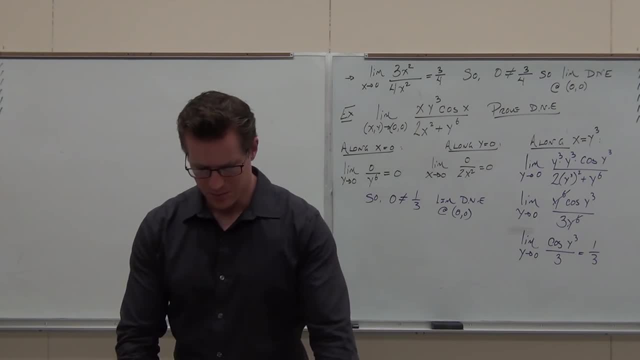 So, OK, tell you what One more I'm going to. I'm basically just going to do this one for you. I'm going to talk through it just to show you some weird things that can happen, Because this doesn't tell the whole story. 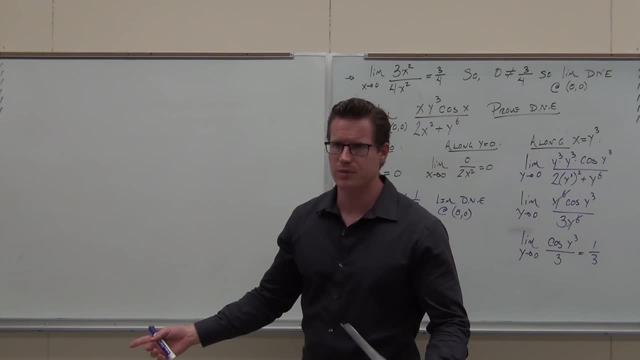 We're not always going to 0, 0.. Your substitution is not always going to be x equals y or y equals x. It's not how it is all the time. So I want to do one more, at least to give you that. 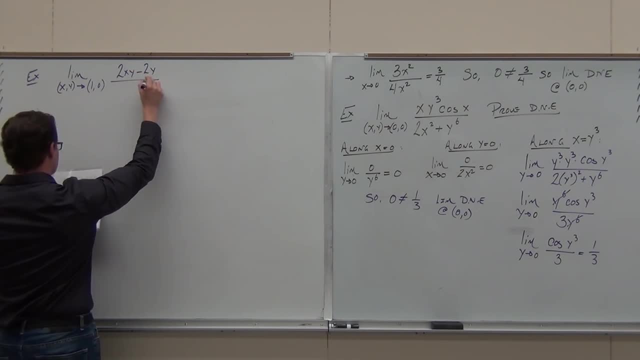 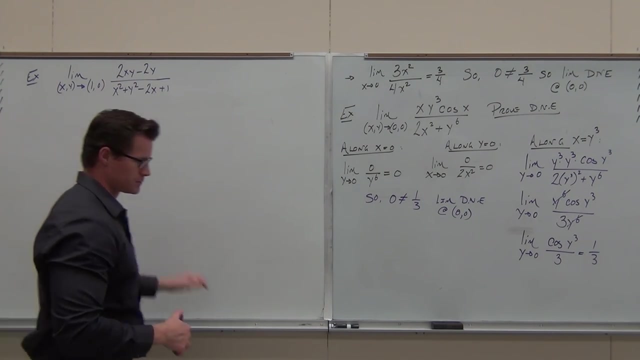 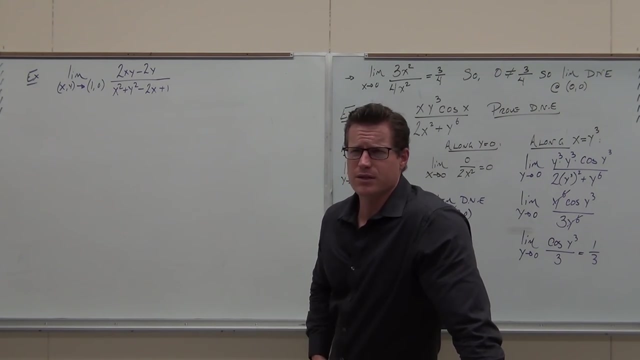 There we go. What's the first thing you do with limits, like all the time? If we plug that in, for x equals 1 and y equals 0.. Do you see- maybe you can think about it for a second- that we're going to get 0 over 0?? 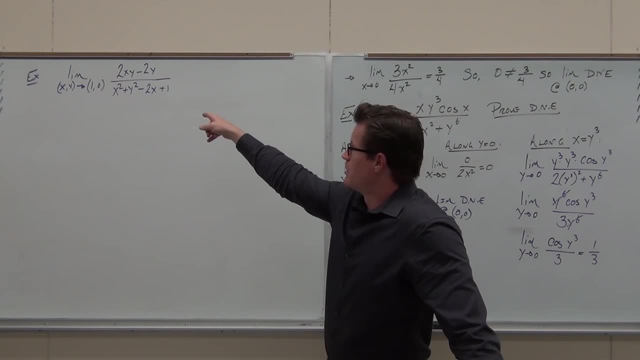 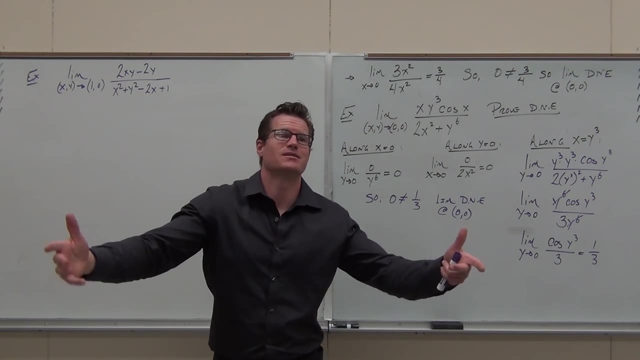 x is 1, so that's well. in the numerator you get 0, 0. But down here we got 0. We got 1 minus 2 plus 1. That's 0 over 0.. If it wasn't, you'd be done. 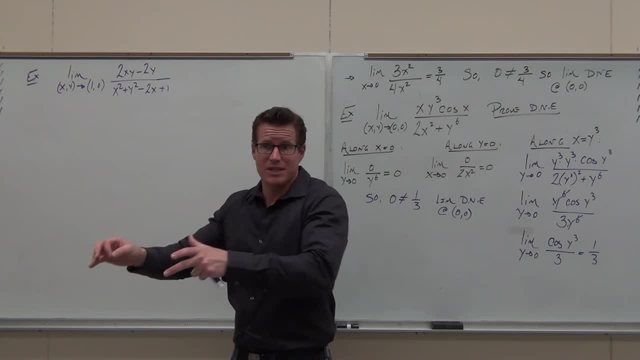 Just plug it in, You'd be done. We'll talk about y later, But you'd be done, Just plug it in. So since we get 0 over 0, we go. well, let's show this limit doesn't exist. 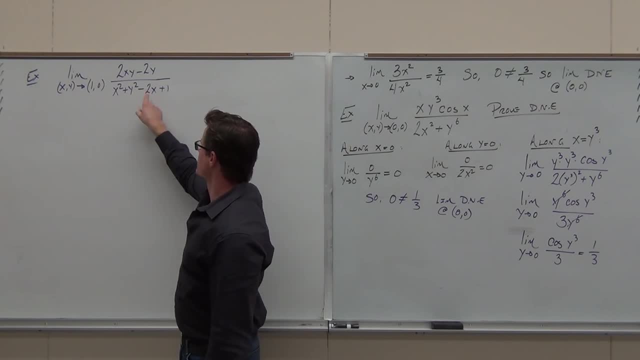 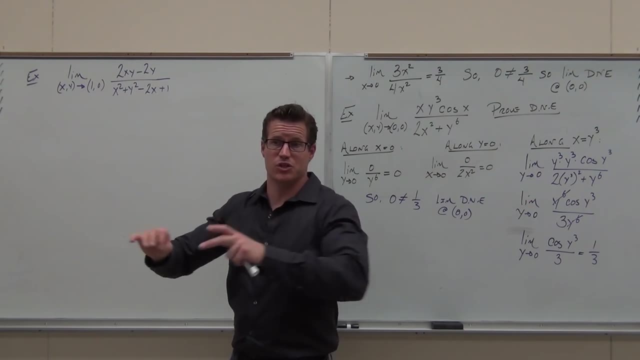 But down here we got 0, and we got 1 minus 2 plus 1.. That's 0 over 0.. If it wasn't, you'd be done. Plug it in, you'd be done. We'll talk about why later, but you'd be done. 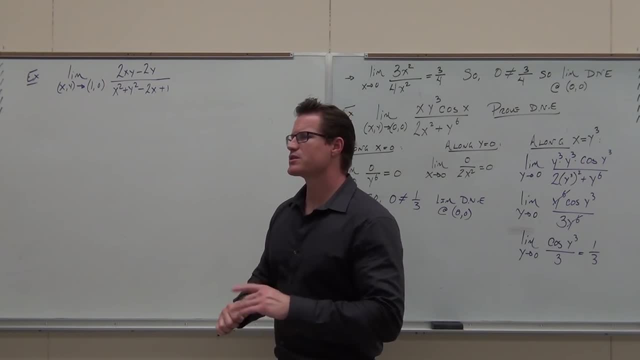 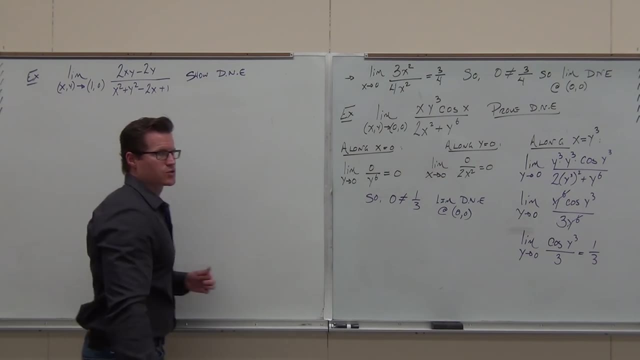 Just plug it in. So since we get 0 over 0, we go: well, let's show this limit doesn't exist, or let's try: Everyone in the class right now. what path do you use? at least what path do you use? 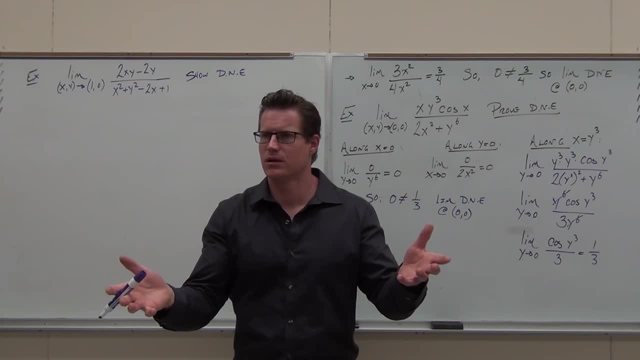 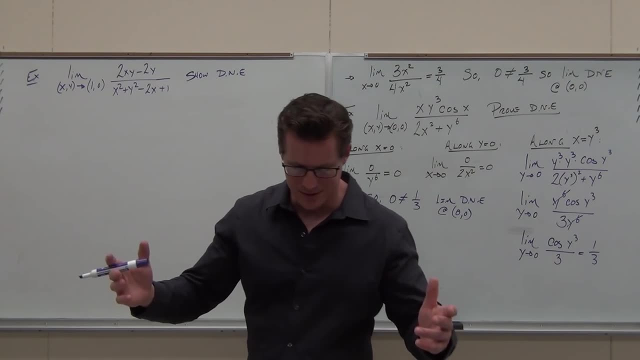 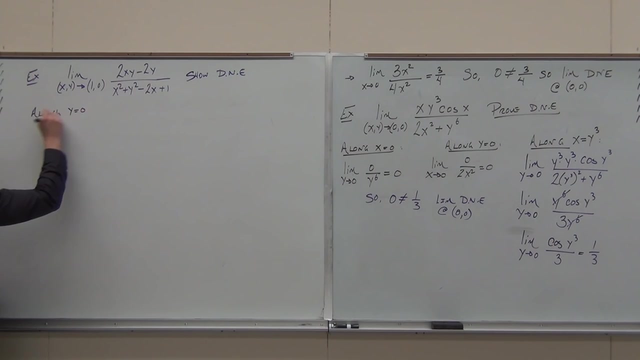 You use at least one of these all the time. What is it? Well, either one, either x is 0 or y is 0. So pick one. In this case, I think I did y equals 0.. So y equals 0.. 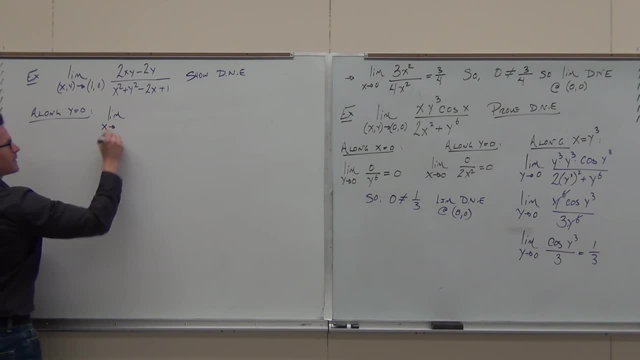 What's y equals 0?? What's y equals 0?? We got limit. oh wait, now wait a second. If we're going along, y equals 0,, this is 0, and that's 0. That's true. 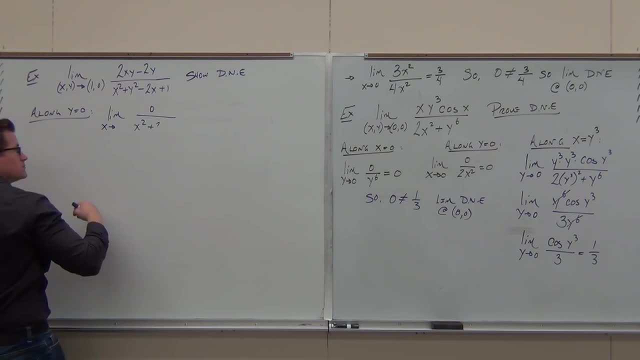 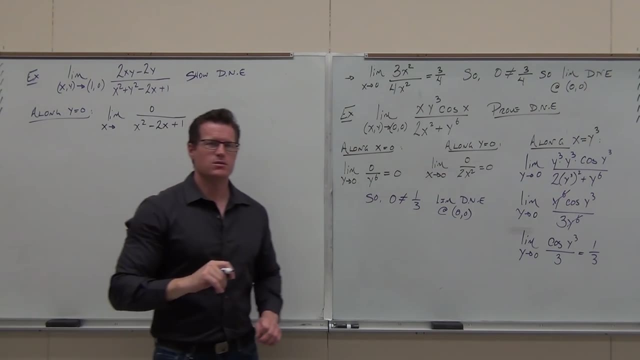 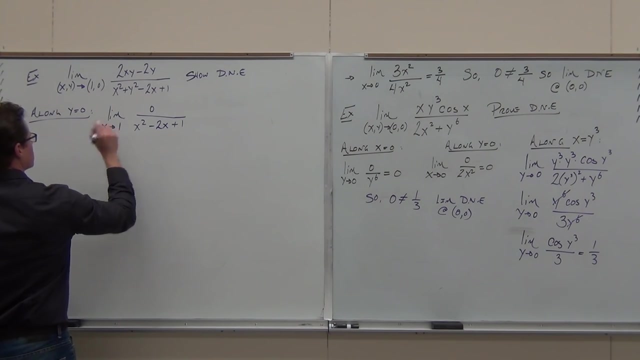 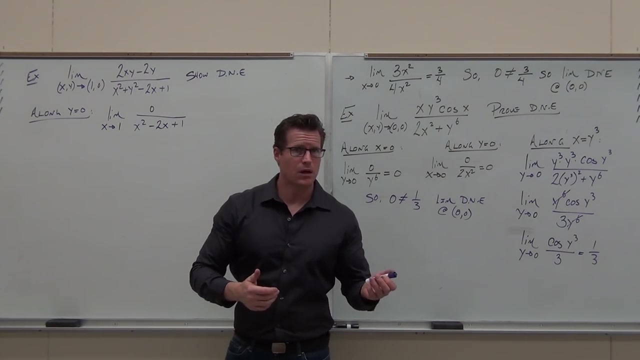 This is 0.. I get x squared plus. oh, I get that. Can you tell me where the x should be approaching? Is it true that along x equals 0,? I'm going to hit this point: 1, 0?. 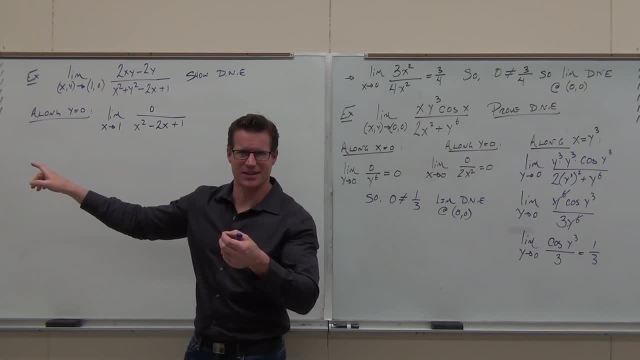 Notice that y equals 0 is the x-axis. Do you guys get that? So that point is on the x-axis: 1, 0, it's on there. So I'm going to be going through that point, But you've got to make sure you're going to the right value. 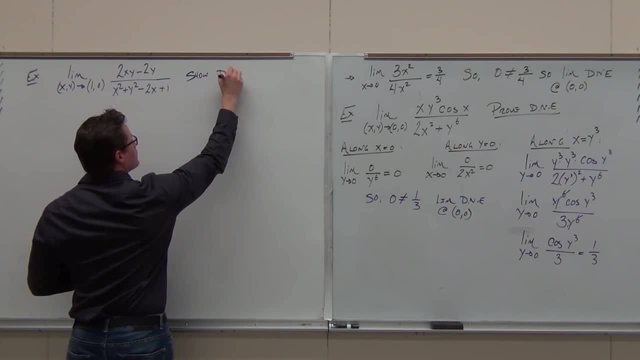 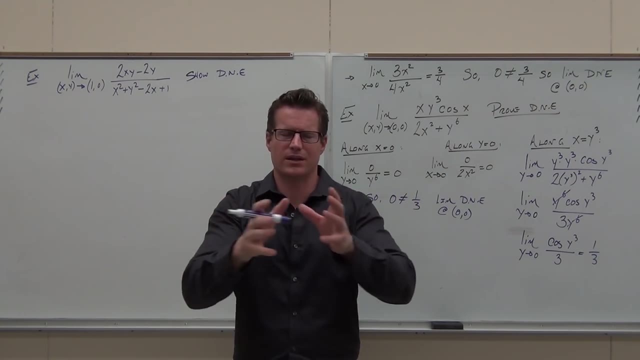 Or let's try Everyone in class right now. what path do you use at least? What path do you use? You use at least one of these all the time. What is it? Well, either one. Either x is 0 or y is 0.. 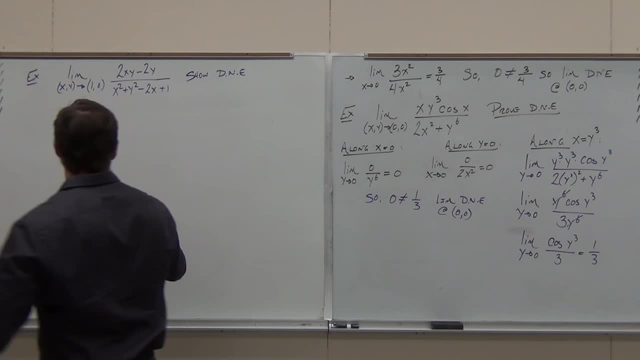 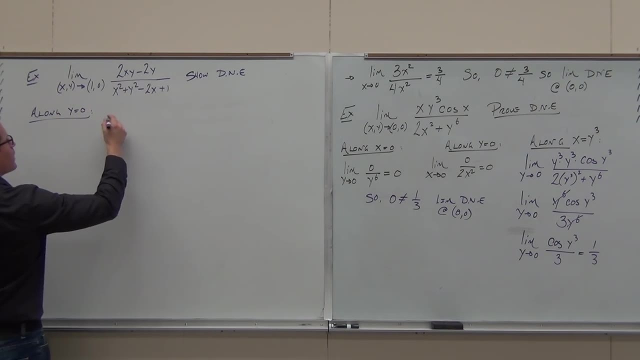 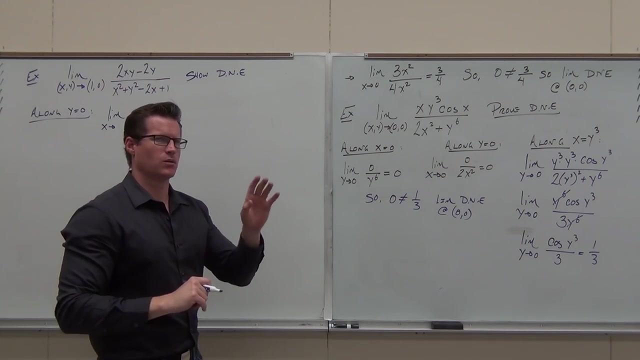 So pick one. In this case, I think I did, y equals 0.. So if y equals 0, we got limit. Oh wait, Now wait a second. If we're going along, y equals 0, this is 0 and that's 0.. 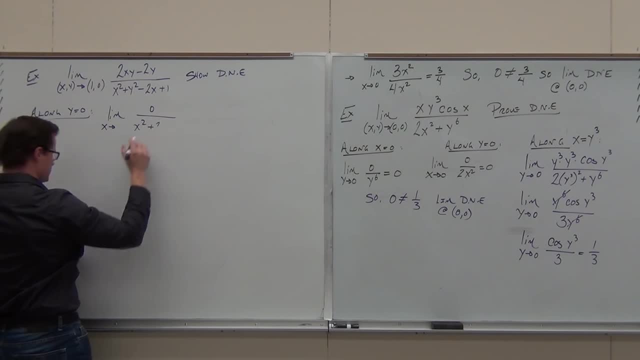 That's true, This is 0.. I get x squared plus 1.. I get that. Can you tell me where the x should be approaching? 1. 1. 1., 1., 1. 1. 1.. 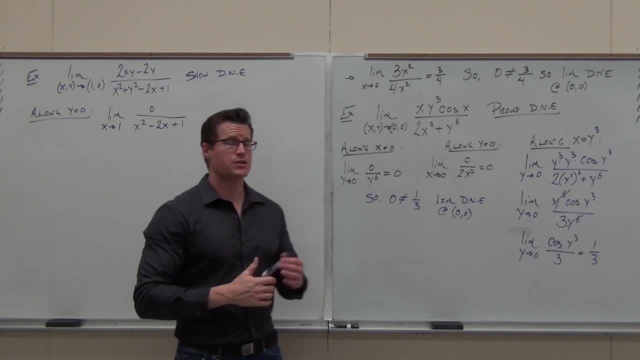 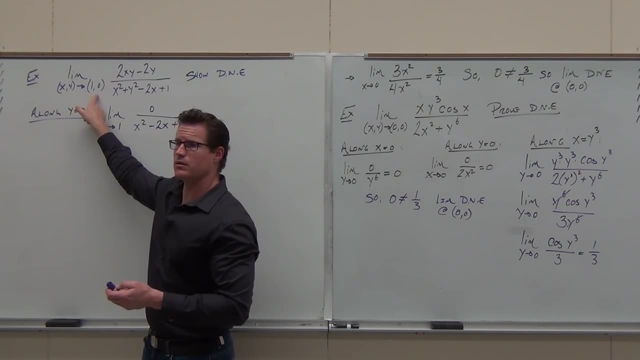 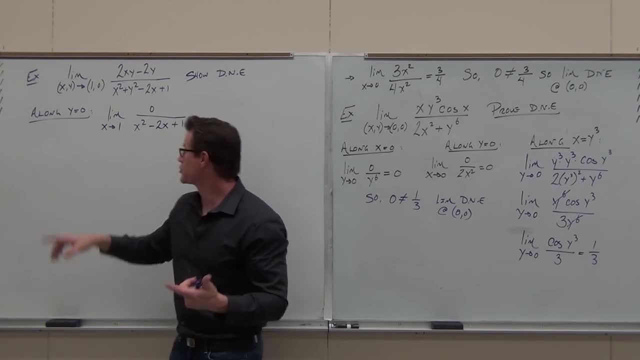 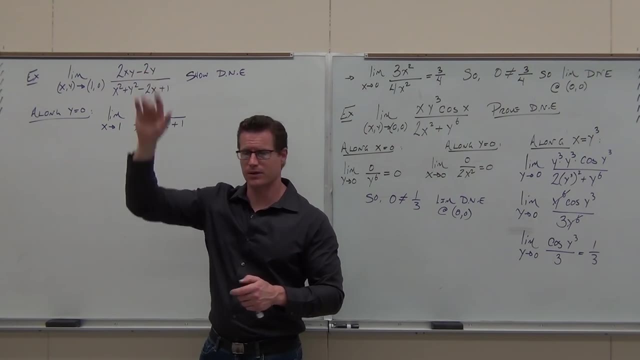 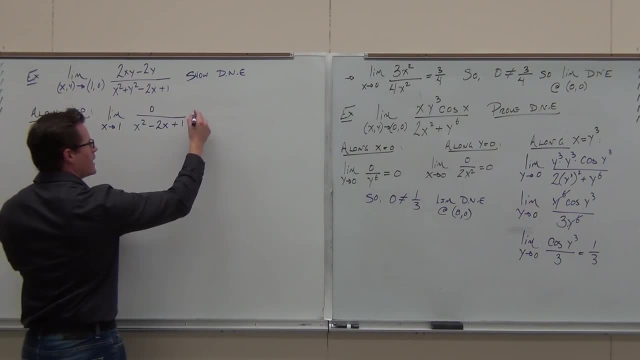 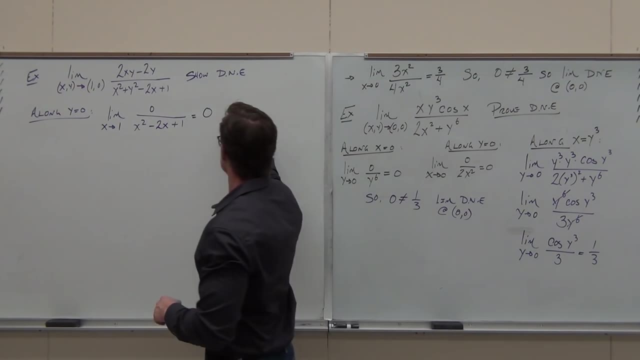 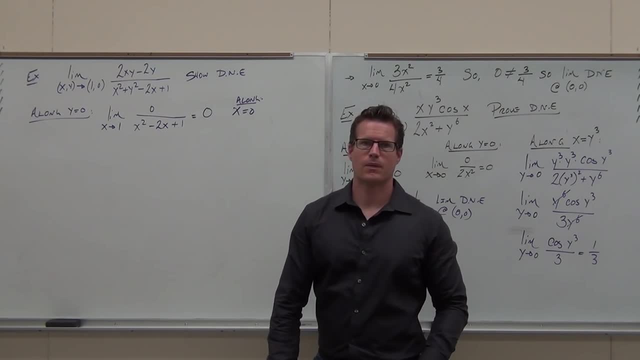 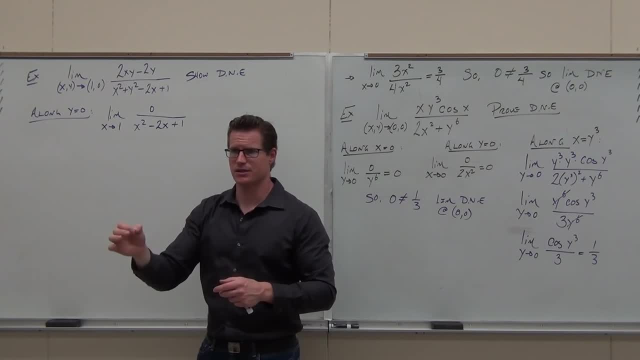 So x still has to be on the x-axis. So x still has to approach 1, since I'm fixing y equals 0.. x still has to approach 1.. So it makes me look good with that one. Okay, so what's it give you? 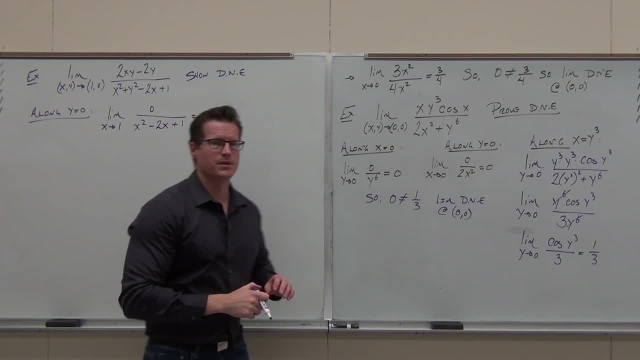 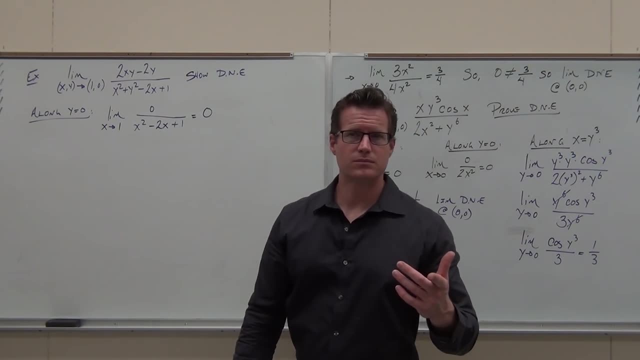 It gives you 0, not 0 over 0. It gives you 0 because if you do low retalls or whatever you have, you actually do get the 0 out of that. Now, if I go along, let's just see if you're paying attention. 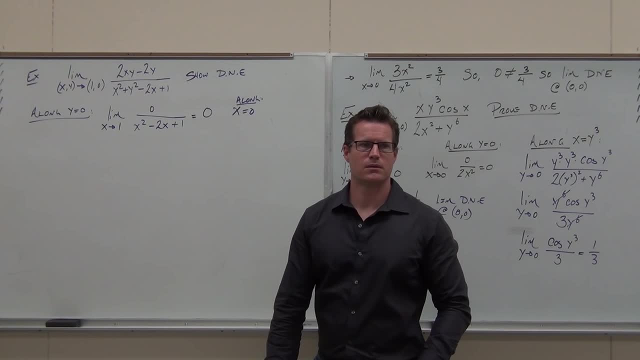 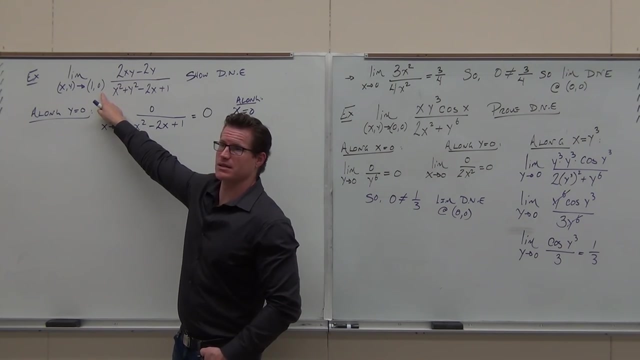 Should I do it? Should I? Why? At least you? That point's not even on that curve. Does that right there? go through that point? No, Then don't do it. That's silly. You're wasting your time. You're wasting your time. 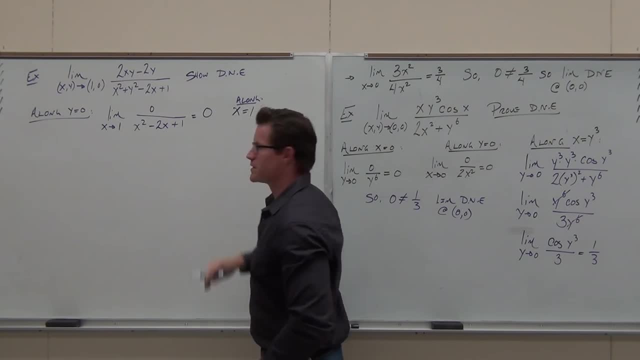 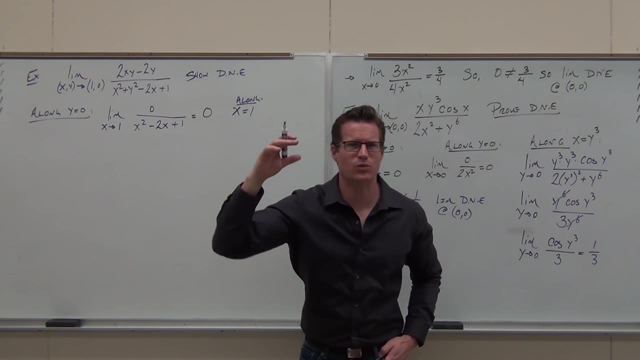 What about this? Would that be something I could do? Yes, Yeah, That goes through that point. That's fine. Now let's just try it in our heads. Okay, you don't have to write it out, but try it in your heads. 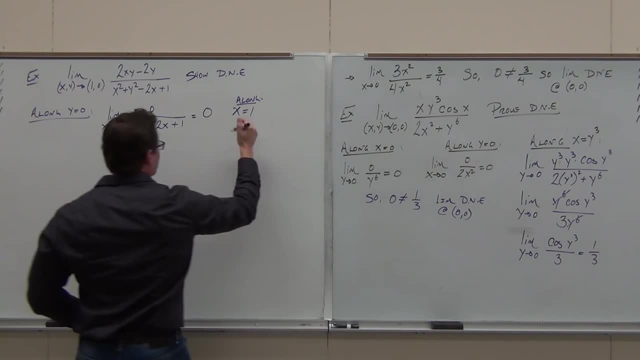 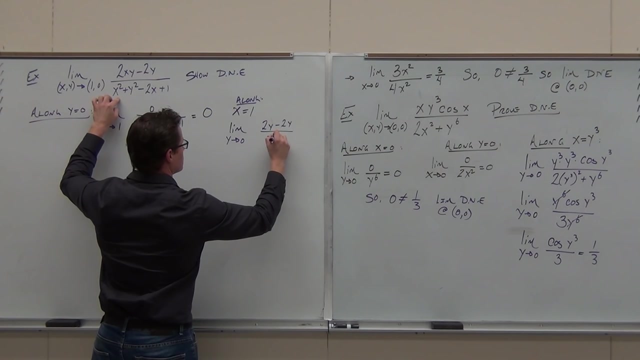 If you did, if x equaled, you know what fine. write it down Why we'd have to go to 0 if x is 1.. We get that Because we have 1 minus 2 plus 1, you'd get that. 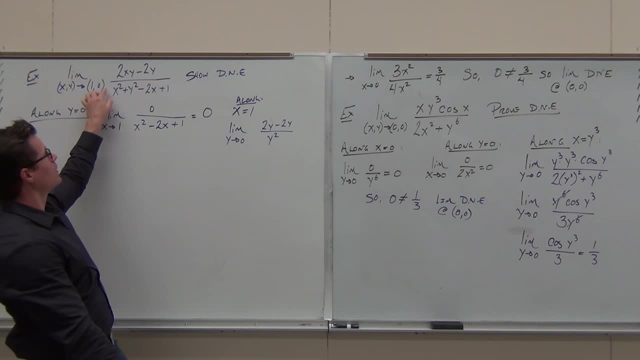 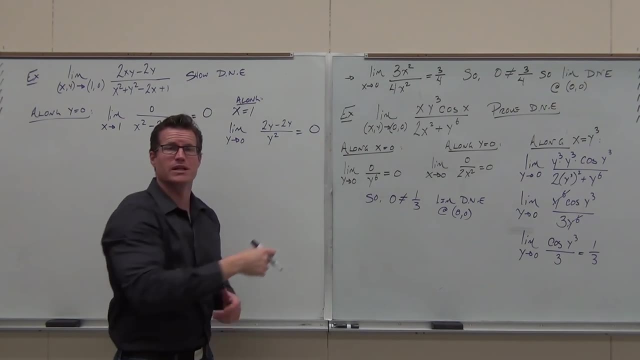 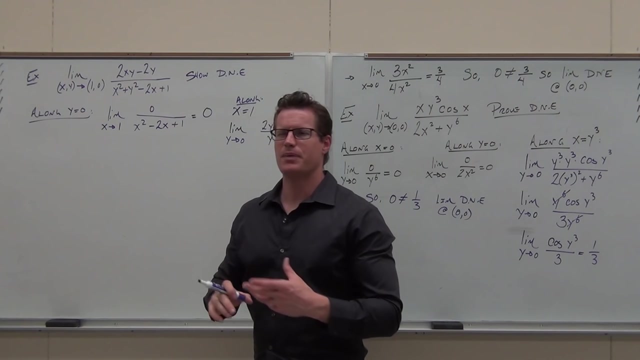 The only independent variable left is y. y has to approach 0. I got 1 here, so we get what's that limit? Come on 0. Does it do anything? No, So we need another path Now sometimes to get your path, because right now it's not obvious. 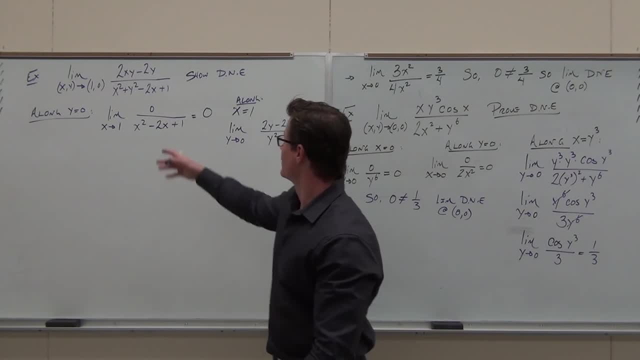 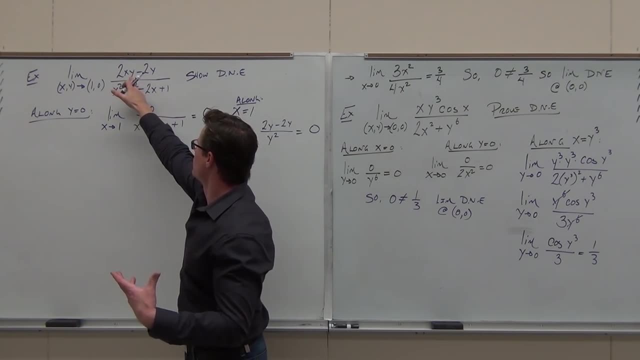 You go, man. I have no idea what path I should take, because if I go try to match up variables, I start having 1's here. That doesn't really help me. If I let x equals y, that doesn't really help me. 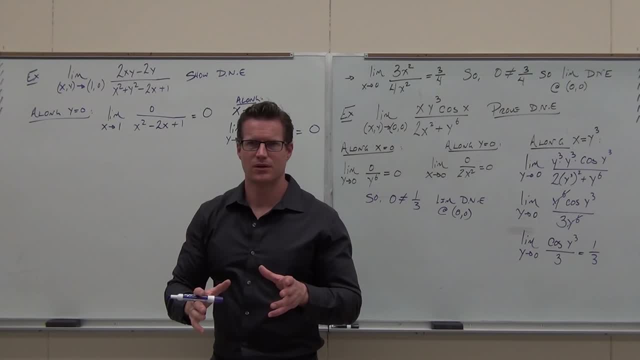 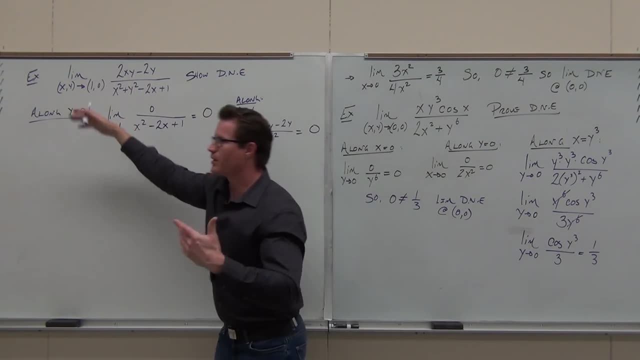 I get some squares. Do you guys see the problem that I'm talking about? No, Are you sure? So here we go. y equals 0, done, No problem. x approaches 1, got to go through the point. x equals 1, got to go through the point. 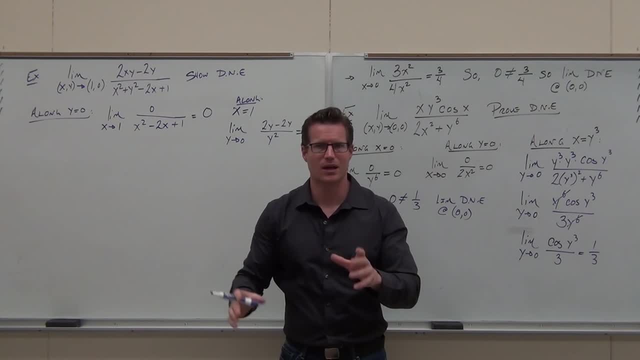 y's got to approach 0.. Either way 0, 0.. It's not telling us anything. Sometimes some tricks like this help. Not tricks, but some simple math. Try factoring, See if you can factor this stuff. 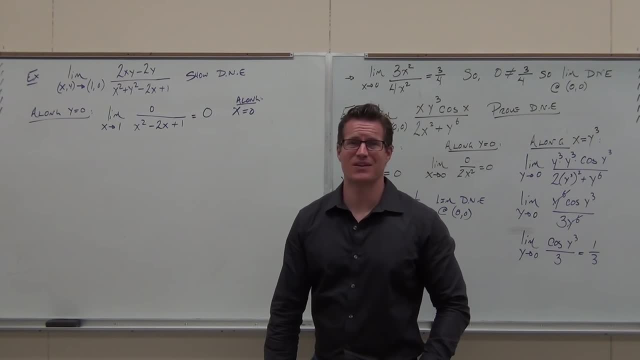 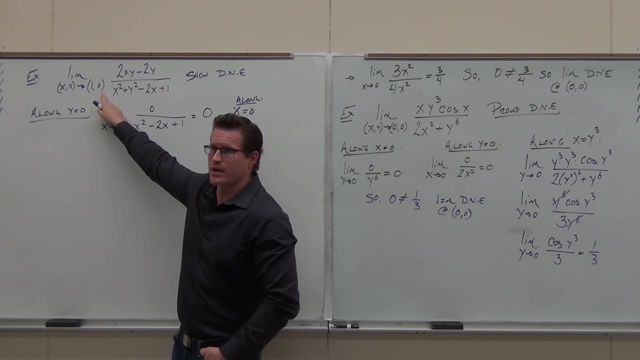 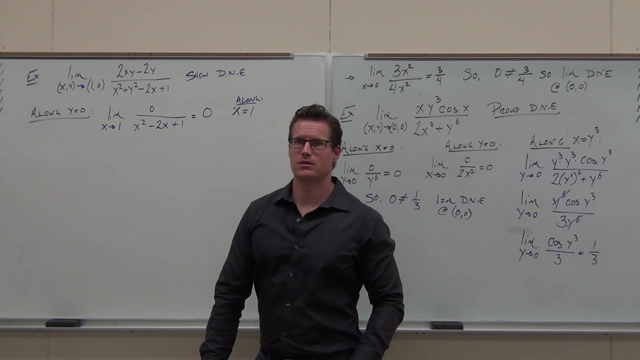 That point's not even on that curve. Does that right there? go through that point? No, Then don't do it. You're wasting your time. You're wasting your time. What about this? Would that be something I could do? Yes, 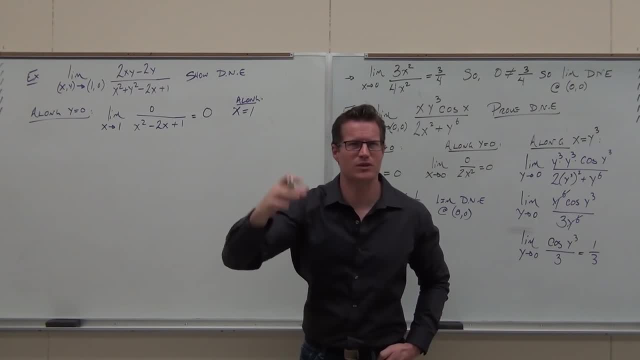 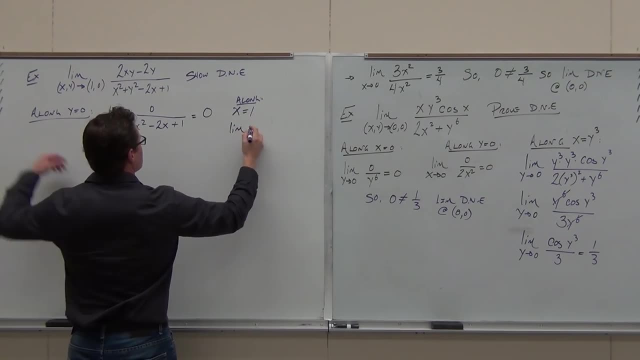 Yeah, That goes through that point. That's fine to write it out, but try it in your heads. If you did, if x equaled- oh you know what? fine, write it out over here: Y would have to go to 0 if x is 1.. 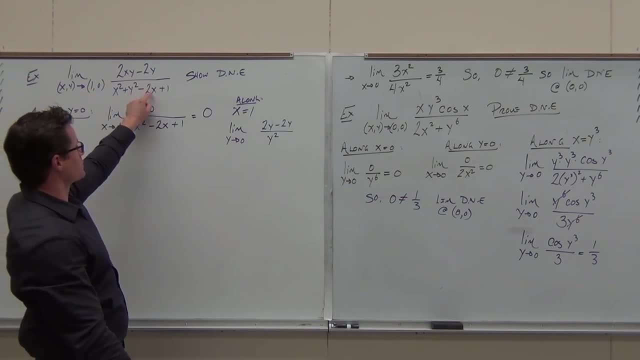 We get that Because we have 1 minus 2 plus 1, you get that The only independent variable left is y. Y has to approach 0.. I got 1 here, so we get what's that limit? Come on. 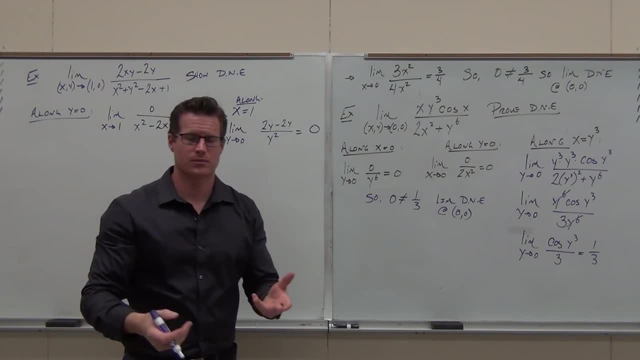 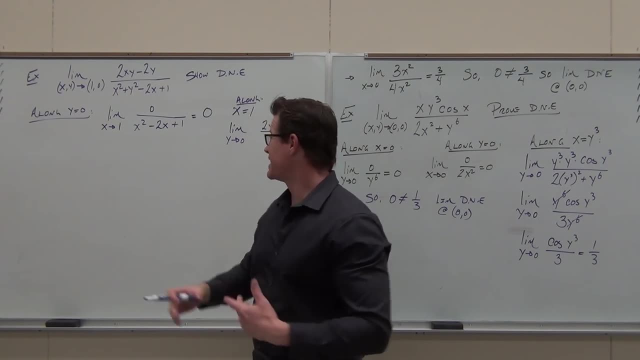 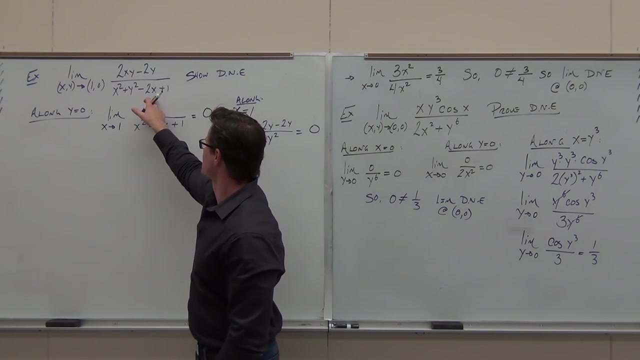 It doesn't do anything. So we need another path Now sometimes to get your path, because right now it's not obvious. You go, man, I have no idea what path I should take, Because if I go try to match up variables, I start having 1s here. 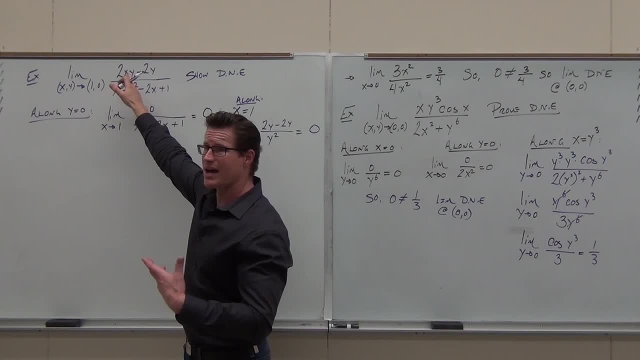 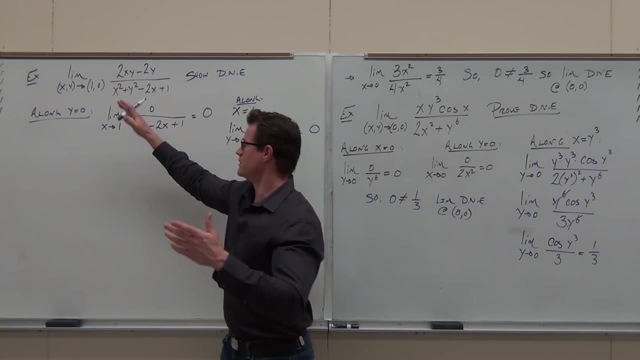 That doesn't really help me. If I let x equals y, that doesn't really help me. I get some squares. Do you guys see the problem that I'm talking about? No, Are you sure? So here we go: Y equals 0, done. 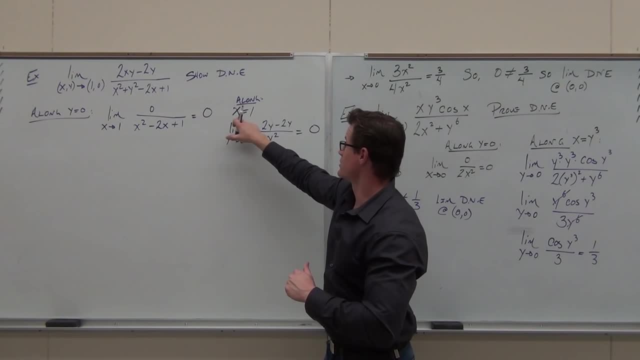 No problem, X approaches 1, got to get to the point X equals 1, got to go through the point. Y's got to approach 0. Either way, 0, 0. It's not telling us anything. 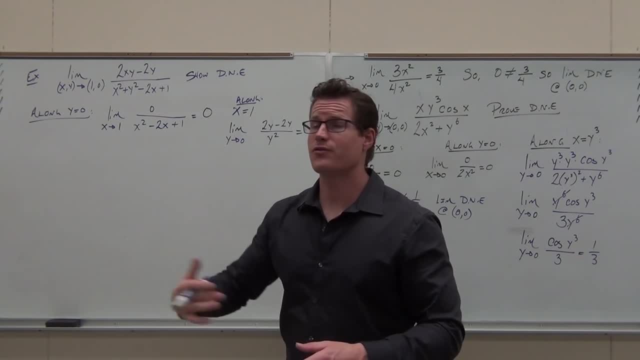 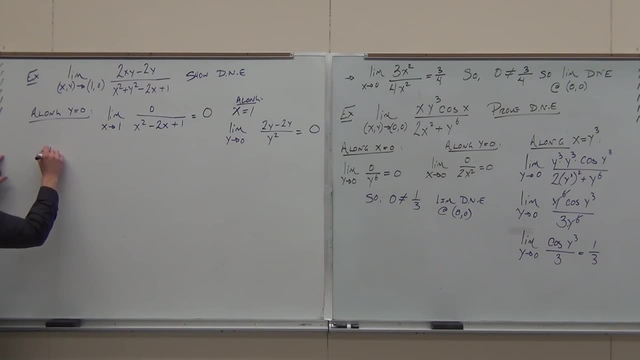 Sometimes some tricks like this help. Not tricks, but some simple math. Try factoring, See if you can factor this stuff. Sometimes that gives you a path to go along. For instance, if I factor, And if I factor this, pull the y squared. 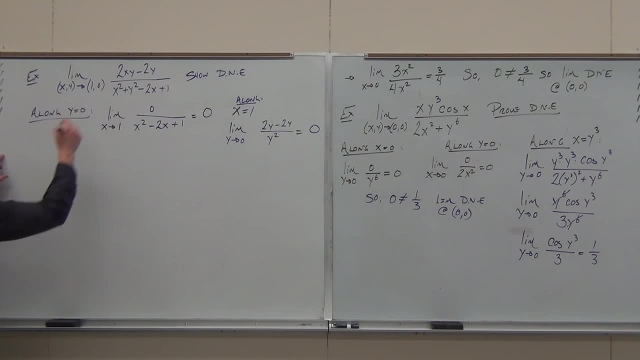 Sometimes that gives you a path to go along. For instance, if I factor, And if I factor this, pull the y squared, but notice how x squared minus 2x plus 1, it's still here. That's a perfect square trinomial. 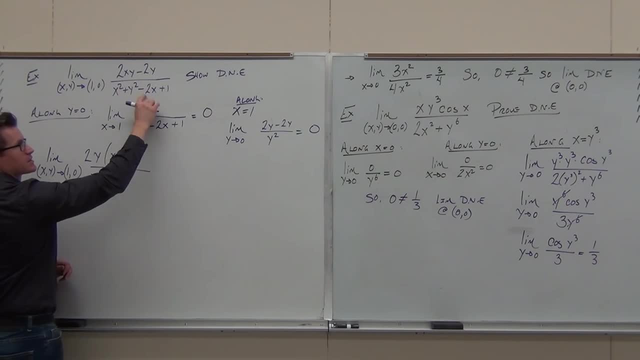 but notice how: x squared minus 2x plus 1, it's still here. That's a perfect square trinomial. In fact, it's x minus 1.. Y squared: Oh shoot, Hope you saw the little change there. 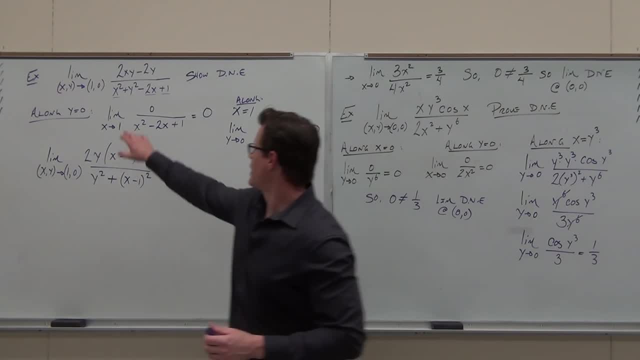 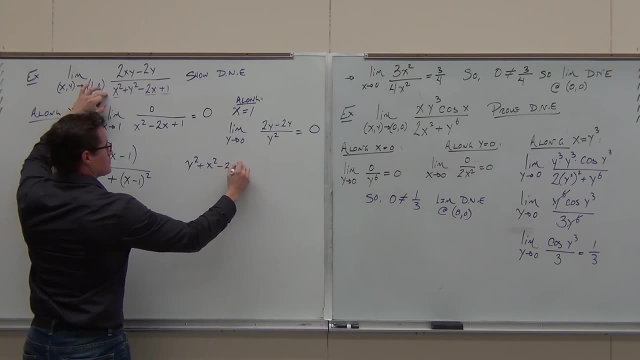 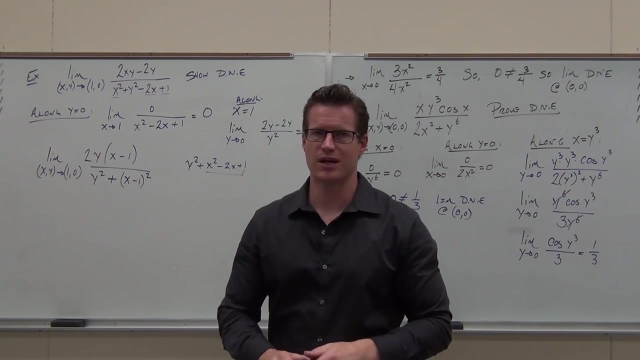 You guys? okay with that one. It should be a plus. It should be a plus because you have y squared Plus this. This is that p. You should have a plus 9 times. Does that make sense to you? I know it's just algebra, but just algebra is what messes you. 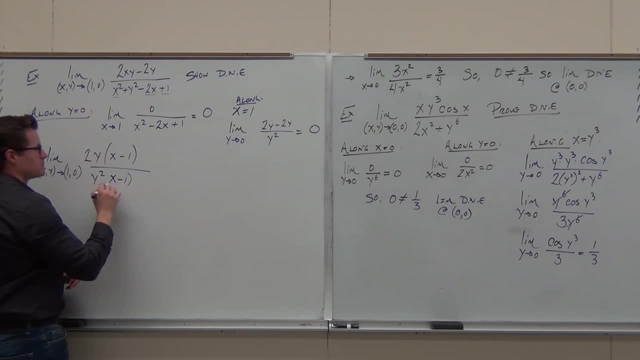 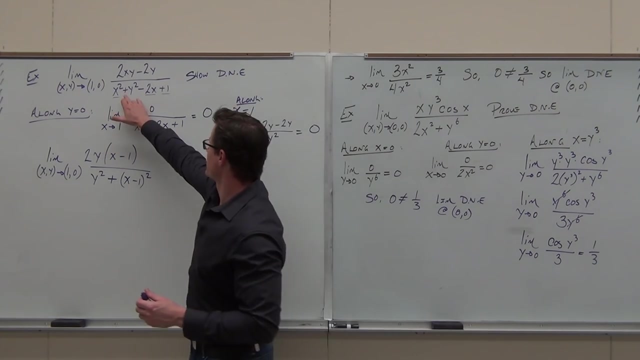 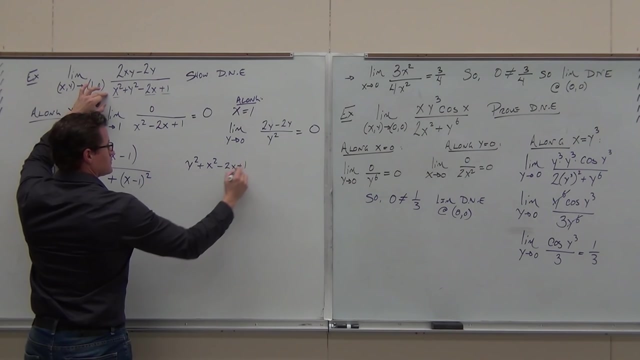 In fact, it's x minus 1 squared. Hope you saw the little change there, You guys. okay with that one, It should be a plus. It should be a plus because you have y squared Plus this. this is that piece. 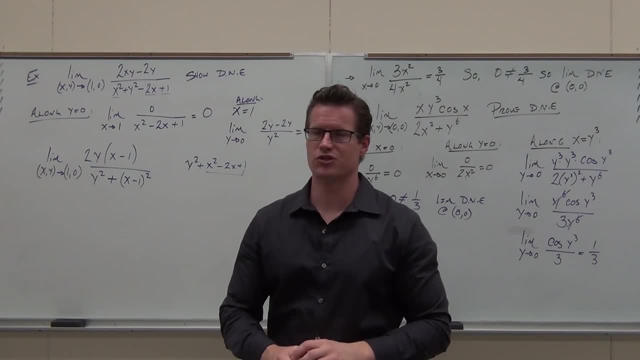 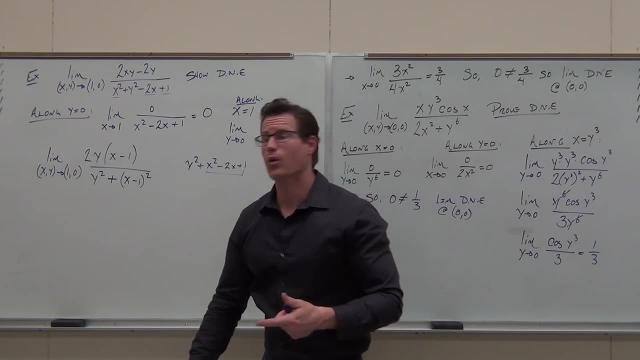 You should have a plus nine times. Does that make sense to you? I know it's just algebra, but just algebra is what messes you up, so be careful with that. Should we be okay with that one for real? Okay, now, if you have that, you go. well, how about this? 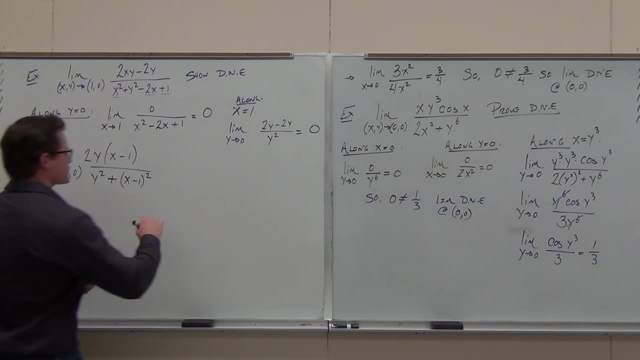 Is there a path that I can go along that's going to make my degrees the same? Notice, I have a power 2.. I've got a power 2.. I've got a power 1.. I want a power 2, and these are the same. 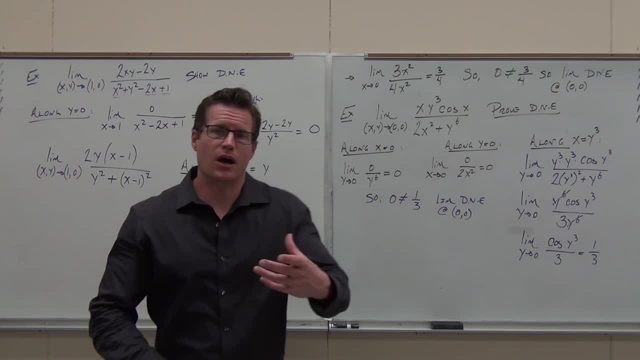 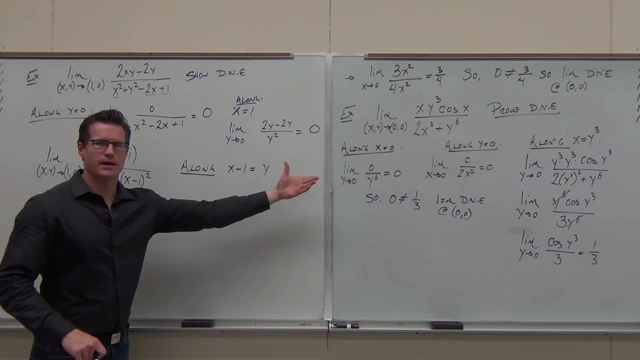 Go along that path. Let's change a whole piece of it. Let's change that ugly piece. If we change that ugly piece, we'll go. hey, let's just change x minus 1 into a y Now, if you're okay with that one. 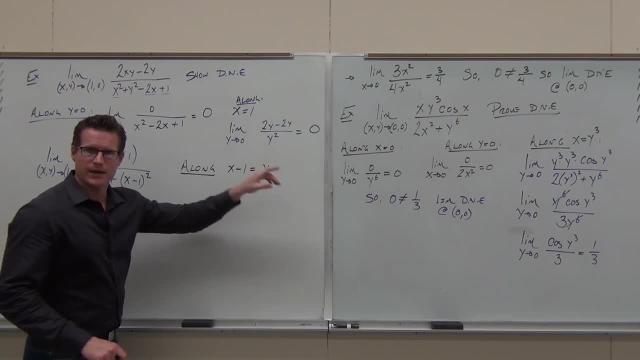 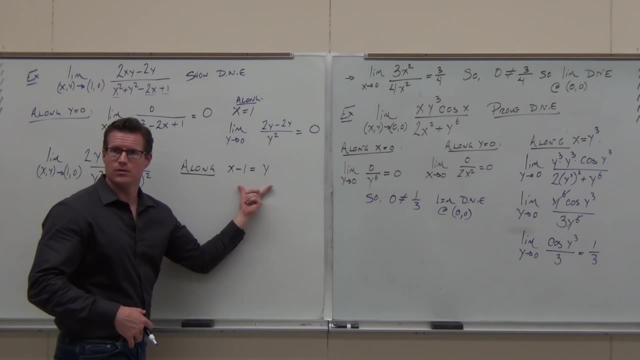 Now stop, right now Stop. Let's see. Is this point actually on that path? Plug in the 1 for the x, Plug in the 0 for the y. Does it equal? Yeah, 0 equals 0.. You know that point's on that path. 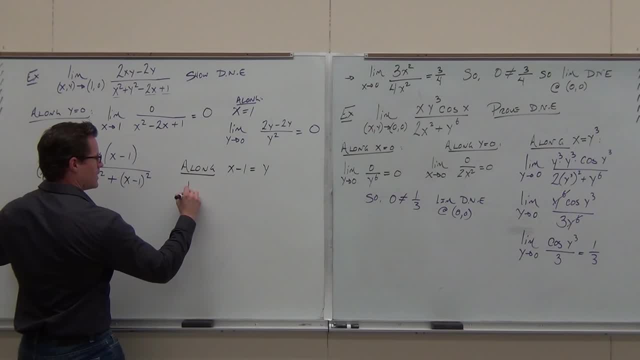 Does that make sense? It's going to work. So let's see We have limit. Let's talk about it in a second. Am I still going to have a 2y? I don't want to replace the y's, okay. 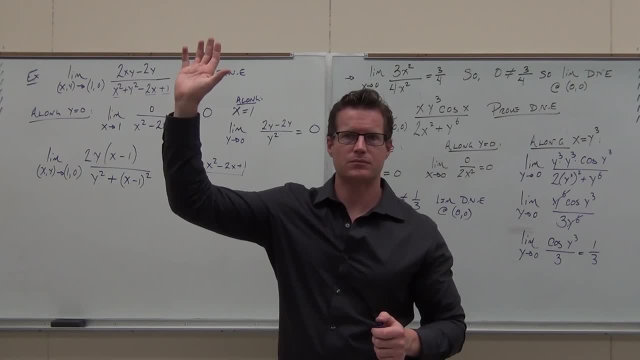 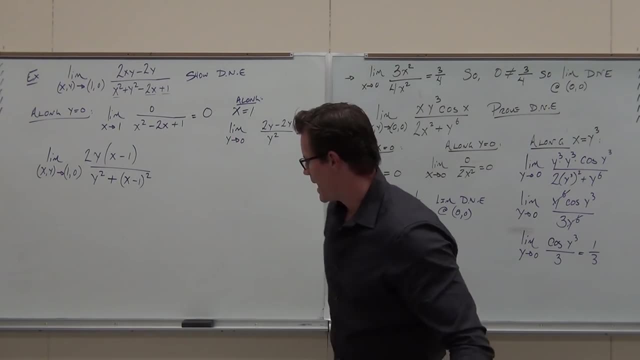 up, so be careful with that. So if you have that, you know well how about this? Is there a path that I can go along that's going to make my degrees the same? Notice I have a power 2.. 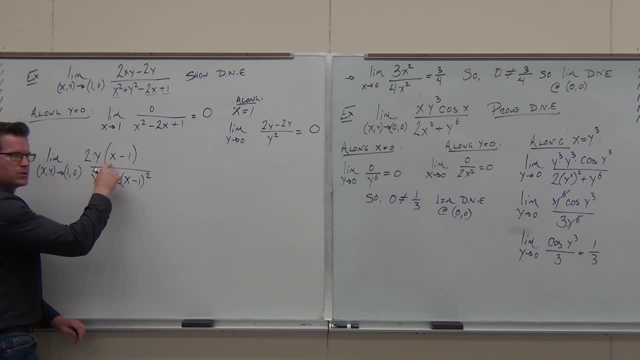 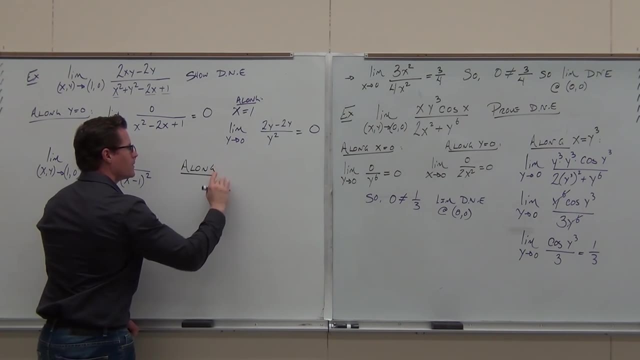 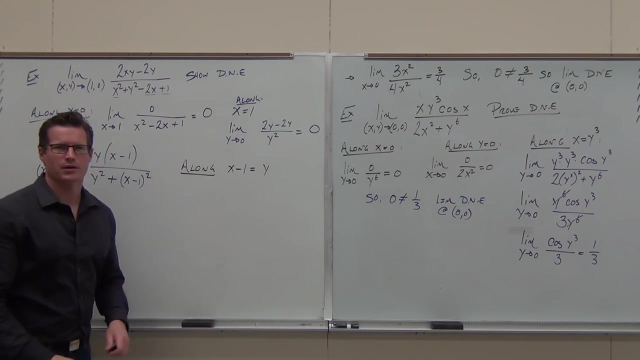 I've got a power. 2. I've got a power. 1. I want a power. 2. And these are the same. All right, so do it. Do it Here. we go, Go along that path. Let's change a whole piece of it. 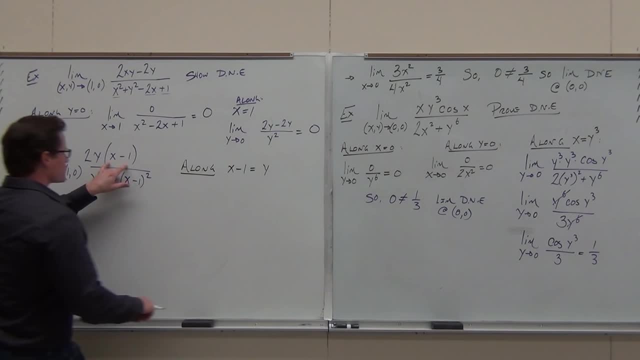 Let's change that ugly piece. If we change that ugly piece, we go: hey, let's just change x minus 1 into a y. Now, if you're okay with that one, Now stop, right now. Stop. Stop. 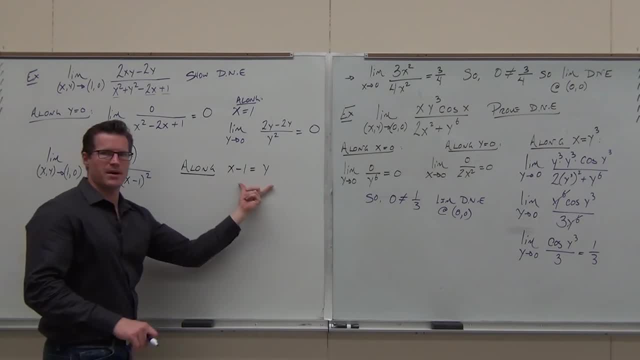 Let's see, is this point actually on that path? Plug in the 1 for the x, Plug in the 0 for the x, The 0 for the y, does it equal? yeah, 0 equals 0. You know that point's on that path. 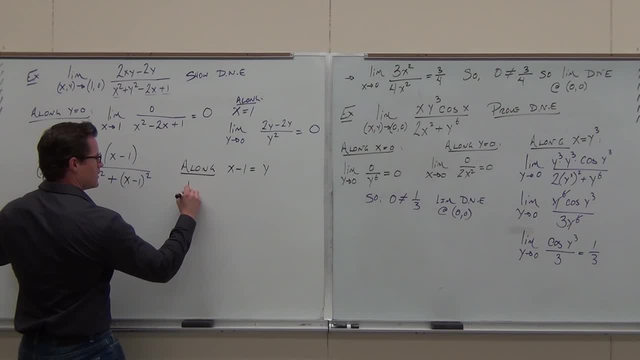 Does that make sense? It's going to work. So let's see We have limit. Let's talk about it in a second. Am I still going to have a 2y? I don't want to replace the y's, okay. 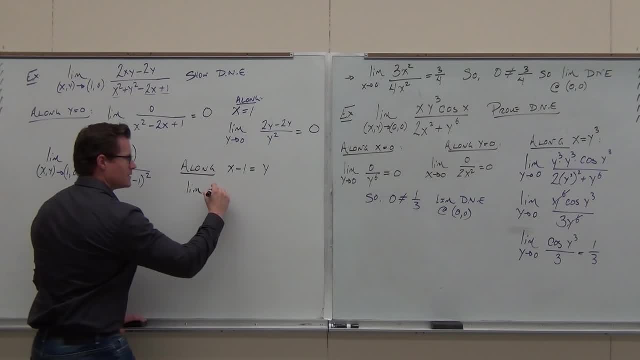 I want to replace this. Am I still going to have a 2y? Am I still going to have an x minus 1?? What am I going to have? y? This is a y squared plus. if this is a y, that's also y squared. 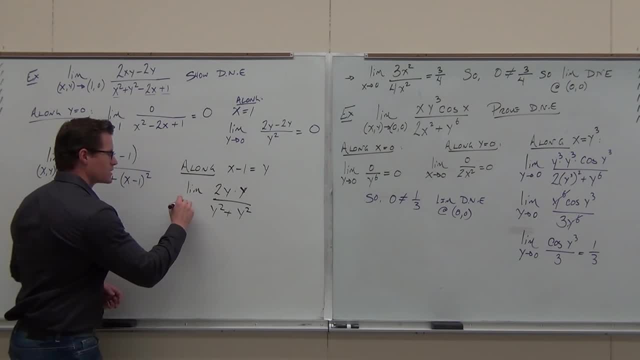 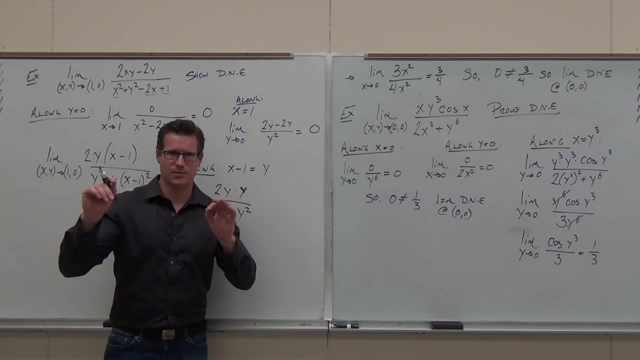 What's the only independent variable I have left? Come on folks quickly. And what's it going to? Zero because x. we fixed x along this path, So we said: along the surface, over this path, and now we're letting y go to 0.. 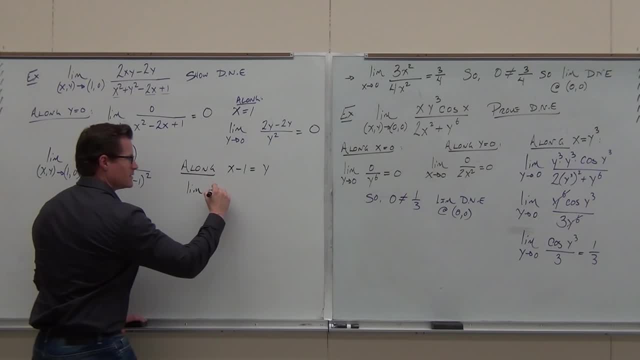 I want to replace the y's. I'm going to replace this. Am I still going to have a 2y? Am I still going to have an x minus 1?? No, What am I going to have? y? This is a y squared plus. if this is a y, 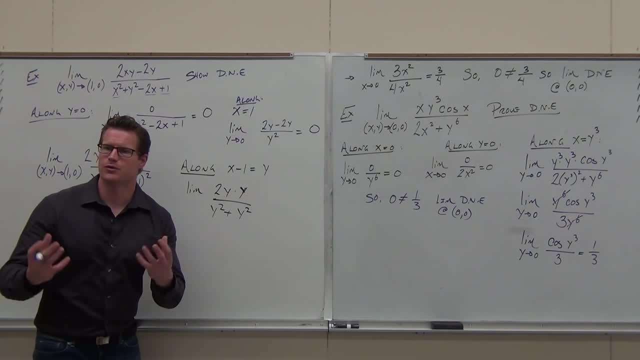 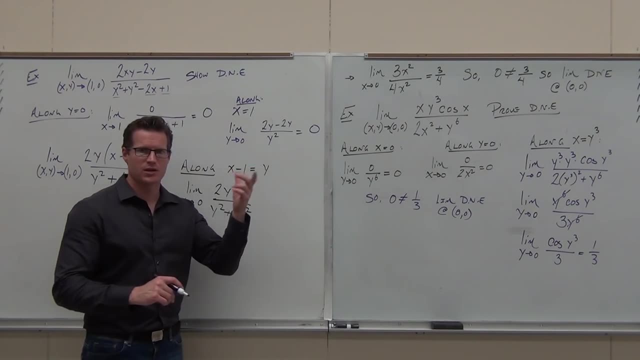 that's also y squared. What's the only independent variable I have left? Come on, folks, And what's it going to? 0.. Because x. we fixed x along this path, So it's along the surface, over this path. 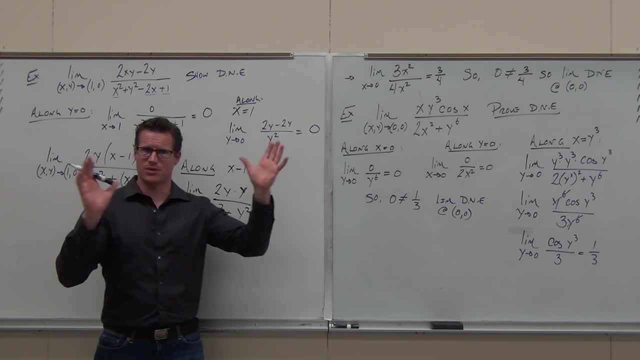 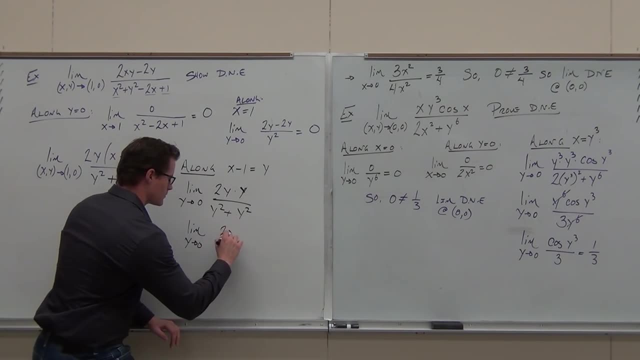 and now we're letting y go to 0.. The x is done. The x is tied up in the y's, We don't have to worry about it. It's just this independent variable that's moving. now We get 1.. 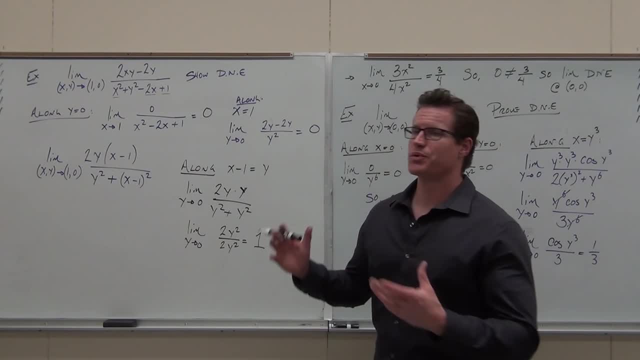 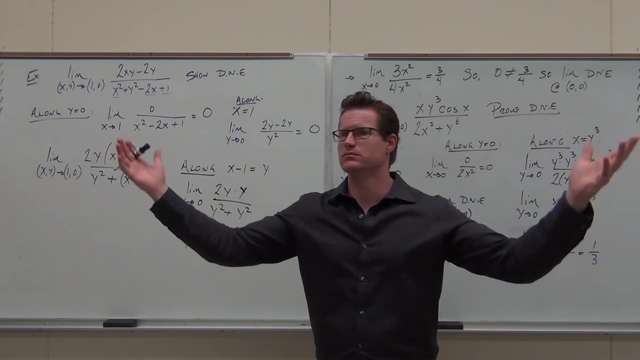 Big fat. 1. Question: Did it prove anything? Come on, put it together. Why? What did it prove? Does not exist. Does not exist. Why? Because? What's it mean? Why does it matter? 0 does not equal 1.. 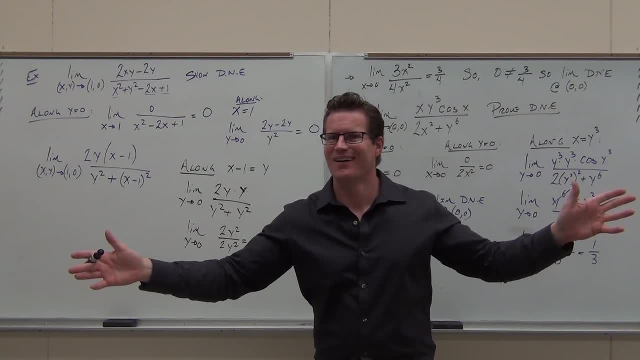 I know that 0 does not equal 1.. 1 does not equal 0.. You're saying the same thing. Because at that point they'll have different heights. Yeah, Because what? At that point they'll have different heights. 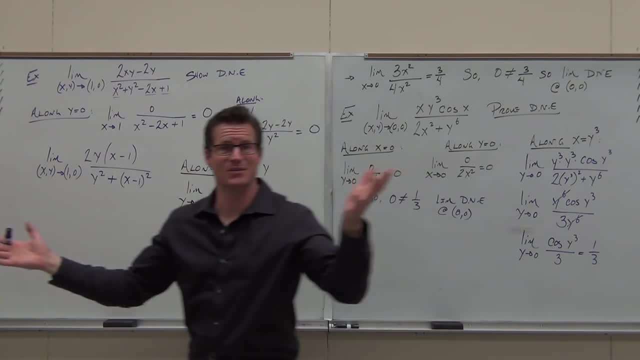 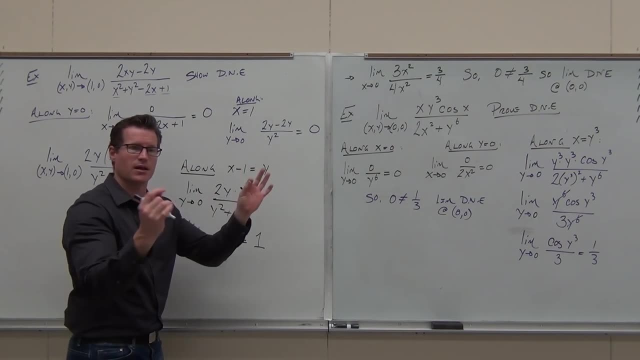 Different heights. That's all I'm doing Along these two paths, different heights, That's it. Limit doesn't exist. So 0 does not equal 1, because these are the heights of the function along those two paths, along the surface, over those two paths. 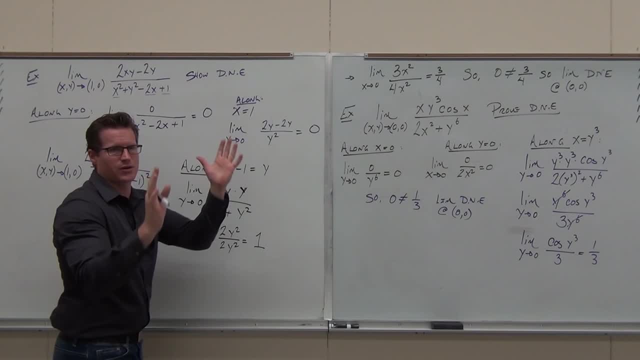 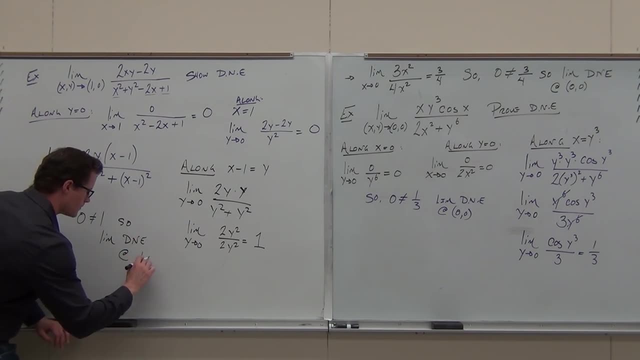 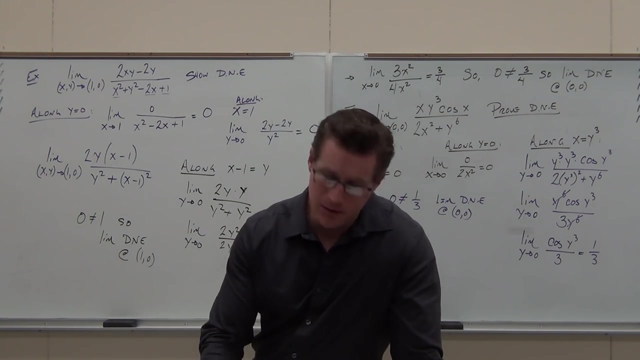 So along the surface, over those two paths, the function has different heights. Therefore the limit does not exist At that certain value. Do you feel like you fully understand this concept up to this point? Yes, Because limits can be tricky. 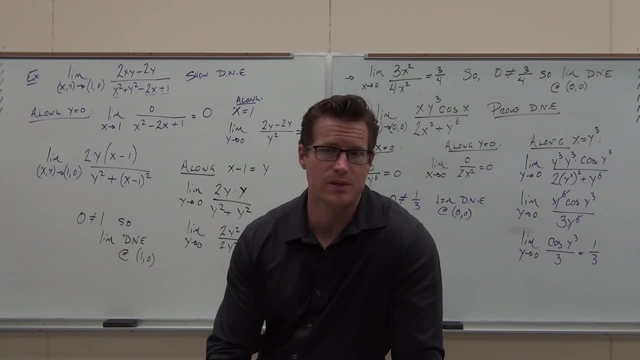 But I've given you some good techniques here. We've shown limits don't. how to show limits don't exist. When we come back, I'll do three variables. We'll talk about how to do that with three variables. We'll talk about continuity very quickly. 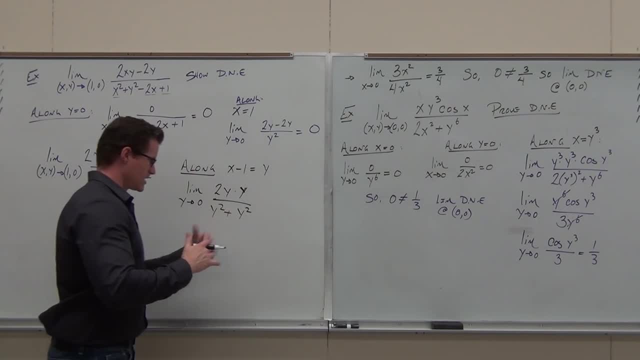 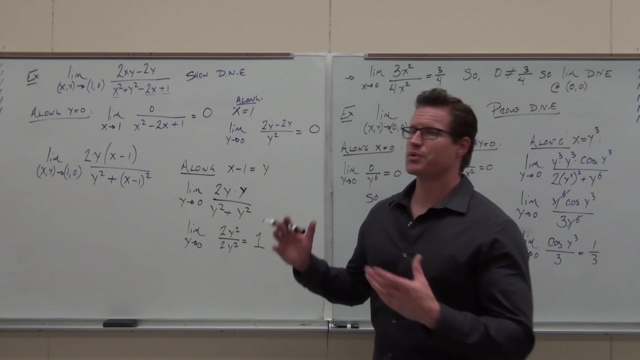 The x is done, X is tied up in the y's. We don't have to worry about it. It's just this independent variable that's moving. No, We need a 1, big fat 1. Question: did it prove anything? 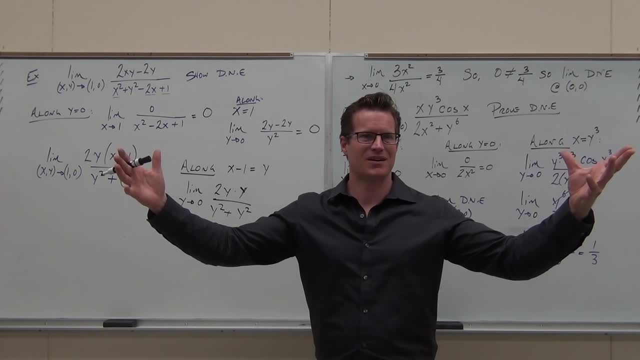 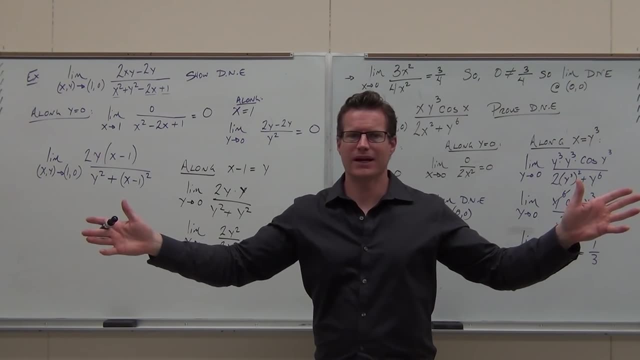 Come on, put it together. Why? What did it prove? Does not exist. Does not exist Why? Because 0 does not equal 1.. What's the name? Why is it not? Zero does not equal 1.. I know that 0 does not equal 1.. 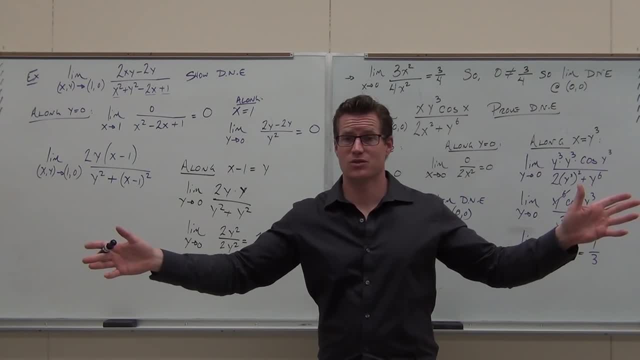 1 does not equal 0.. You're saying the same thing? Yeah, Because what? At that point they'll have different heights. Different heights, That's all I'm doing Along these two paths. different heights, That's it. 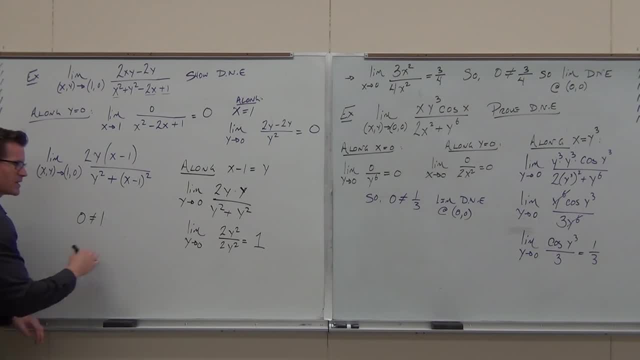 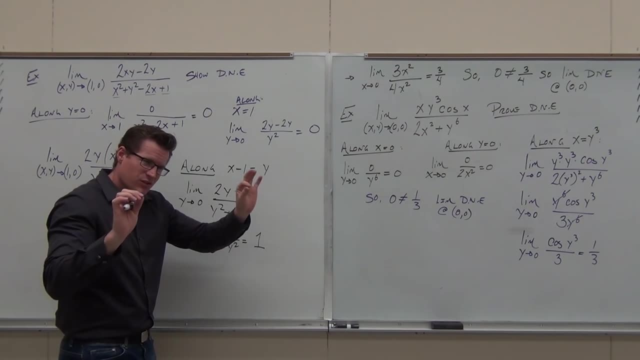 Limit doesn't exist. So 0 does not equal 1, because these are the heights of the function along those two paths, along the surface over those two paths. So along the surface over those two paths the function has different heights. 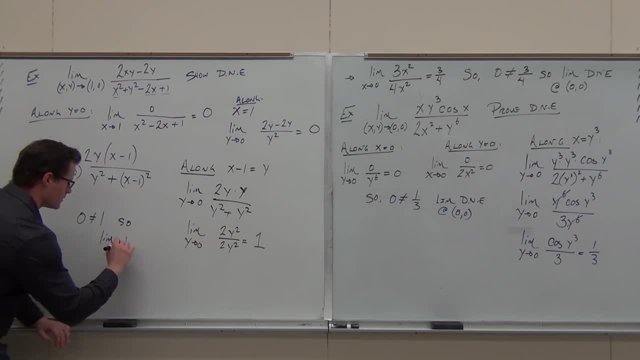 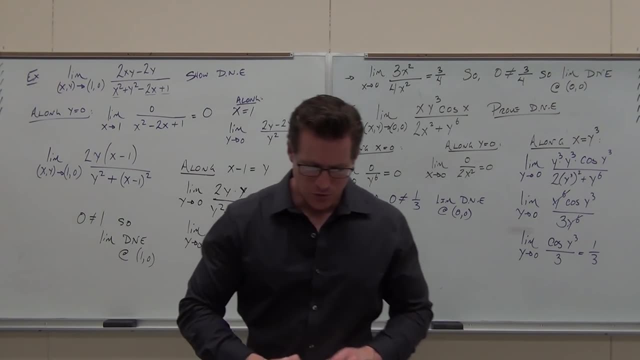 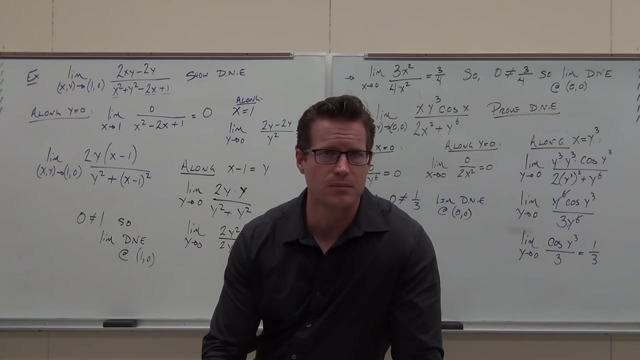 Therefore, the limit does not exist At that certain value. Do you feel Like you fully understand this concept up to this point? Yes, Because the limits can be tricky. But I've given you some good techniques here. We've shown limits don't how to show limits don't exist. 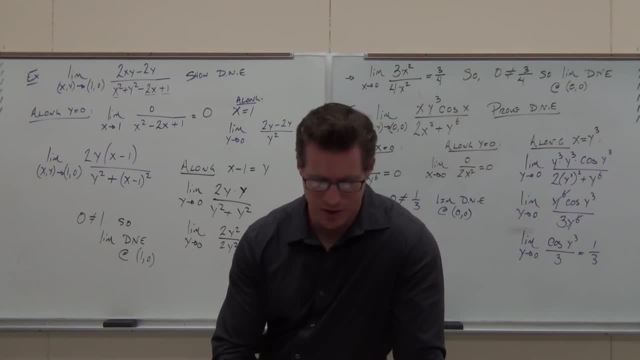 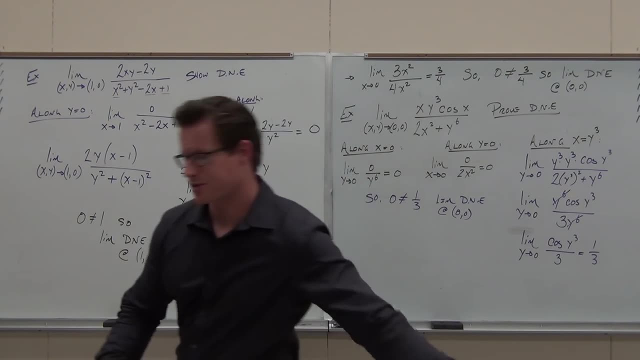 When we come back, I'll do three variables. We'll talk about how to do that with three variables. We'll talk about continuity very quickly, And then we'll talk- I'll do the squeeze theorem and show you some pretty pictures. All right, 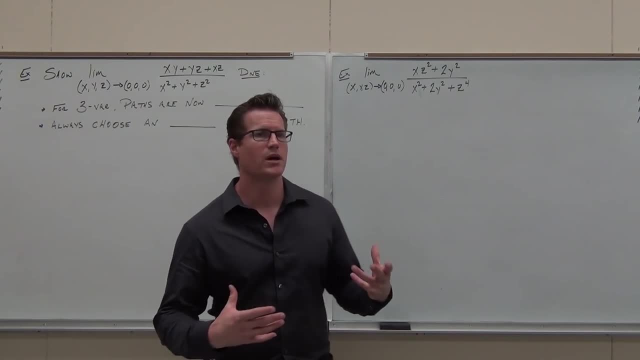 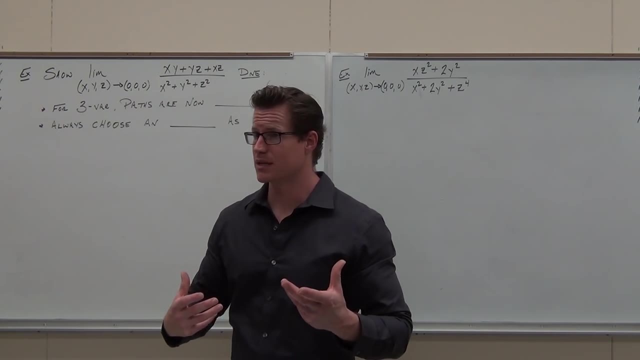 So how do we do this when you have more than two independent variables? We made the transition from one to two. One was easy, calc one Two. I showed you how to prove limits don't exist with two. Now we'll talk about what happens when you have functions. 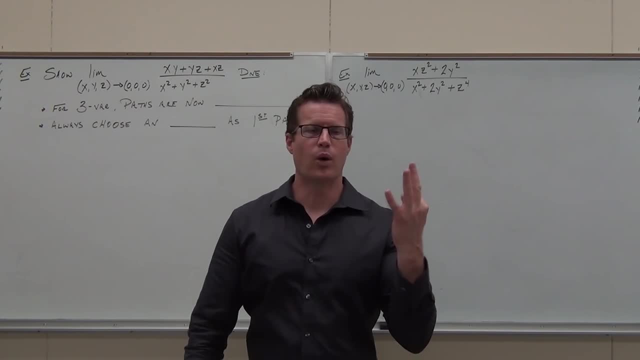 with three- count them three- independent variables. What type of a surface is that? Four dimensions, That's weird, because the paths now are in three dimensions. Does that make sense? So we're traveling along here, we? oh sorry, I'm. 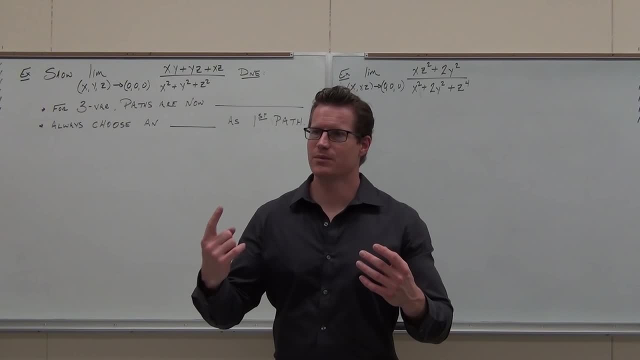 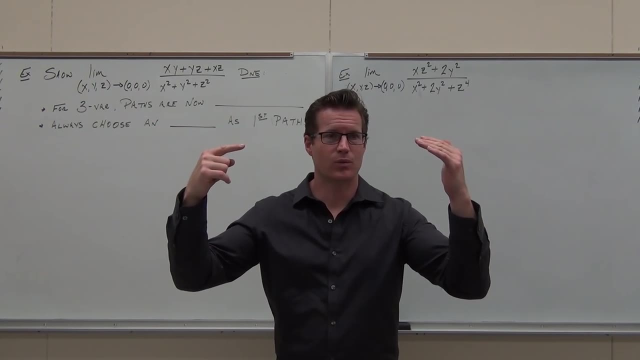 In one independent variable. you were along a curve. Basically, you only had one dimension of travel: left, right. that's it With two independent variables. you had two dimensions of travel. We were on a plane and then surface said: you're restricted. 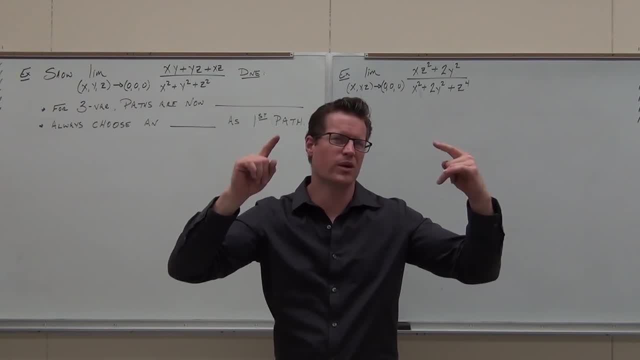 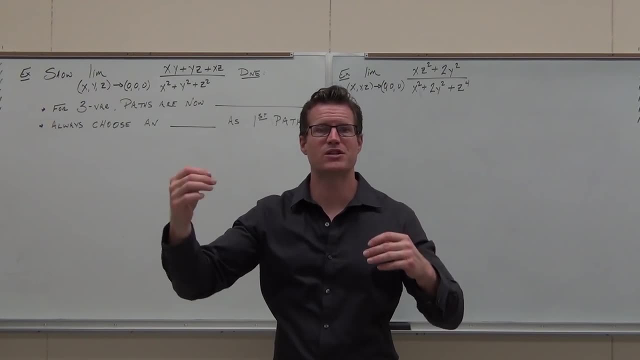 to these two-dimensional curves that were going, that were traveling above, With three independent variables. our curves, they're still curves, but they're space curves, They're now in 3D. Well, what's nice? it's actually nice, it's not hard. 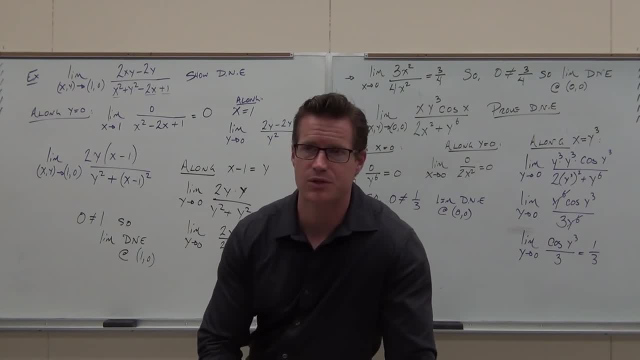 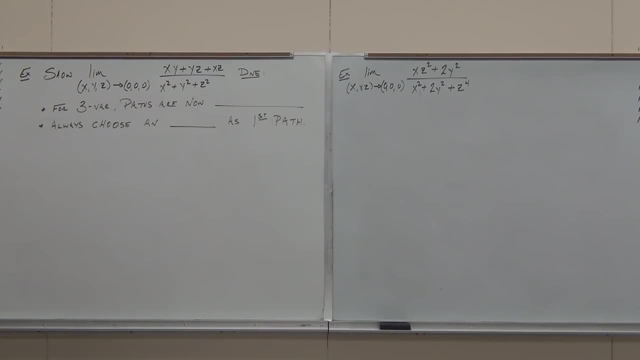 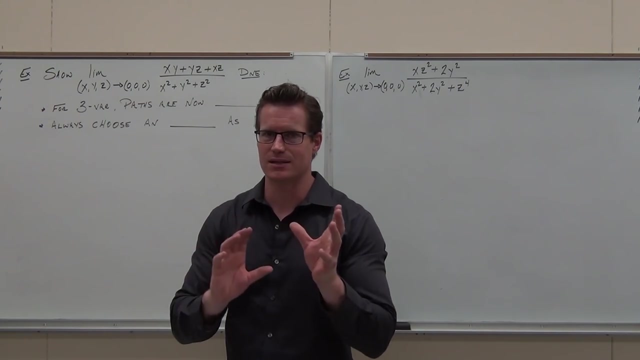 And then we'll talk. I'll do the squeeze theorem and show you some pretty pictures. All right, so how do we do this when you have more than two independent variables? We made the transition from 1 to 2.. 1 was easy, Calc 1.. 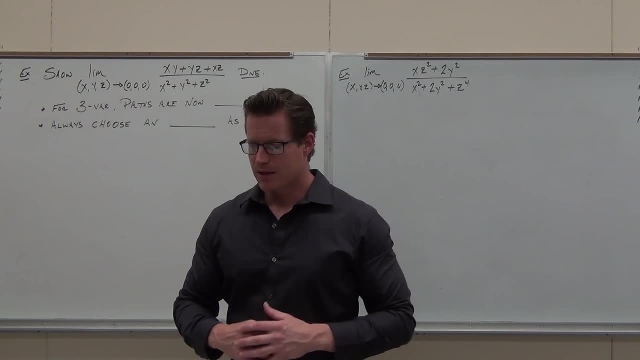 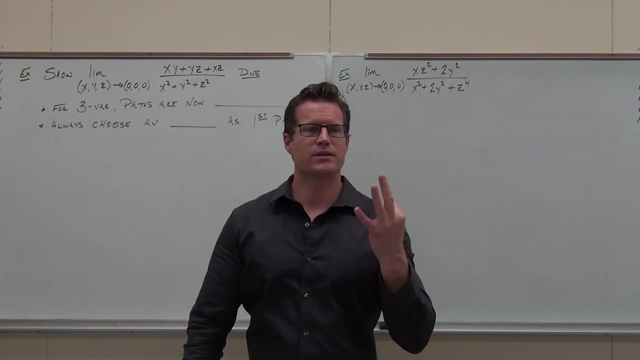 2,. I showed you how to prove limits don't exist with 2.. Now we'll talk about what happens when you have functions with three. count them three independent variables. What type of a surface is that? Four, Four dimensions. 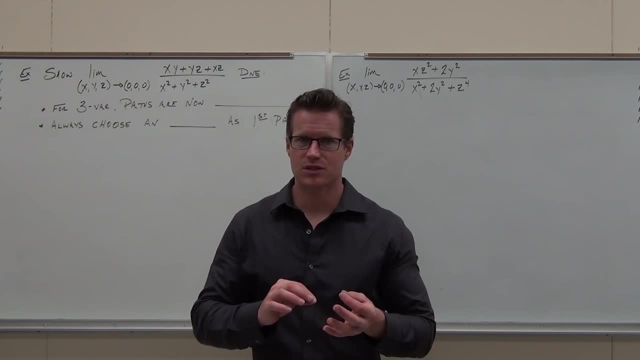 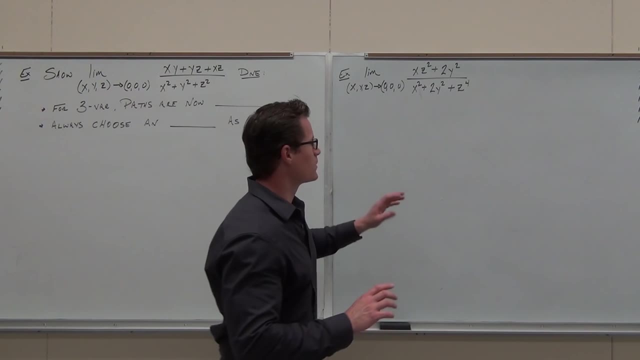 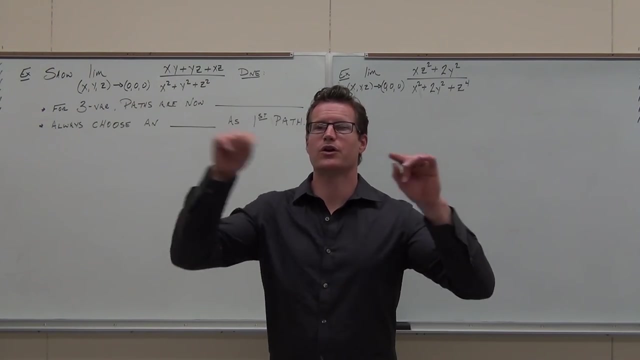 That's weird, Because the paths now are in three dimensions. Does that make sense? So we're traveling along? here we- oh sorry, I'm rational In in one independent variable. you were along a curve. Basically, you only had one dimension of of travel. 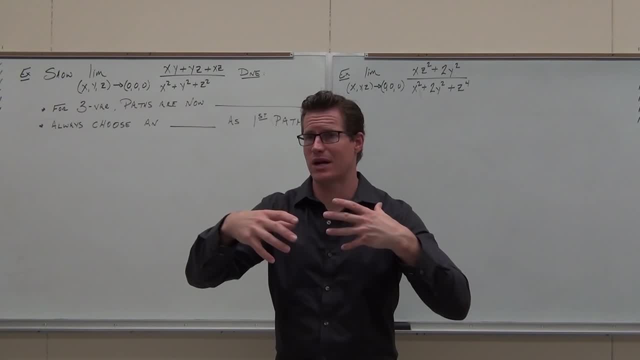 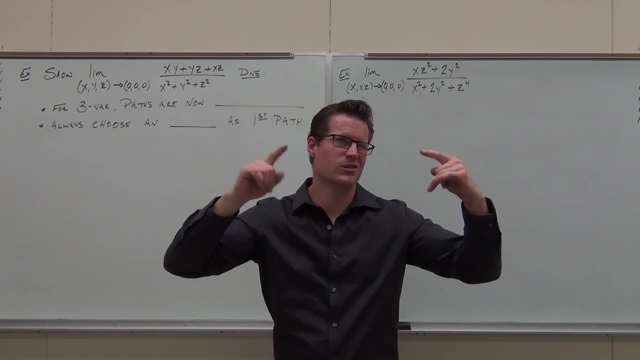 Left right. that's it, With two independent variables. you had two dimensions of travel. We were on a plane and then surface said: you're restricted to these two dimensional curves, That that we're going, that we're traveling above. 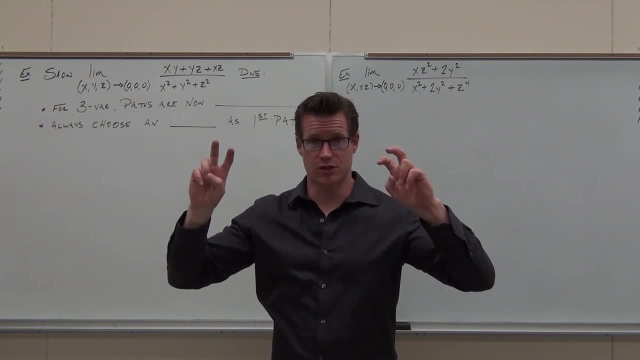 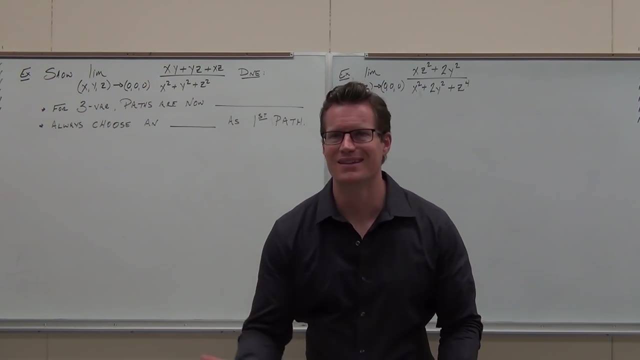 With three independent variables. our curves: they're still curves, but they're space curves. They're now in 3D. Well, what's nice? it's actually nice. it's not hard. What's nice? don't overthink this. 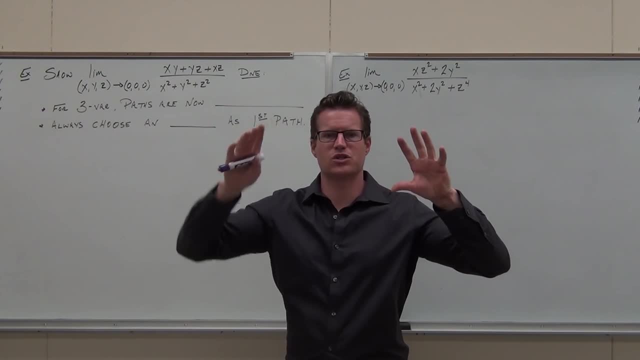 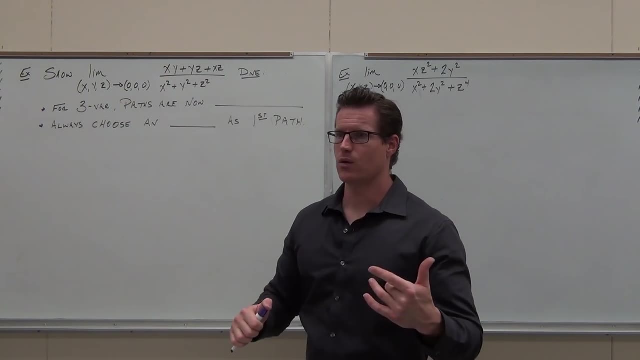 we're not traveling along surfaces. We're still traveling along curves over these 40 surfaces, But for three variables. the paths are now parametric, because that's how we defined curves in 3D. They're now parametric. Does that make sense to you? 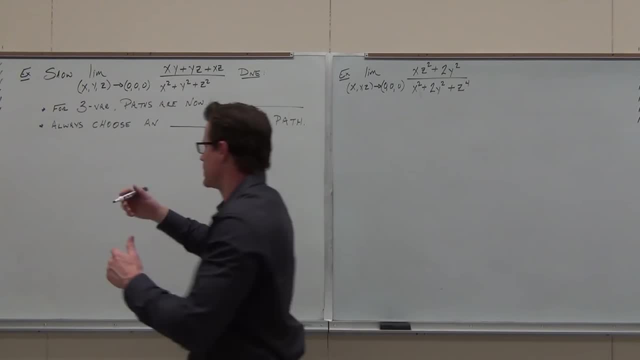 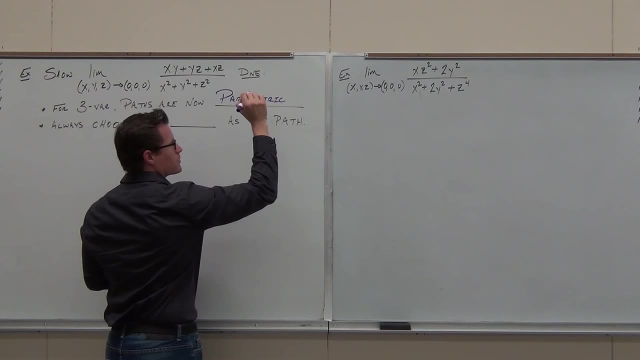 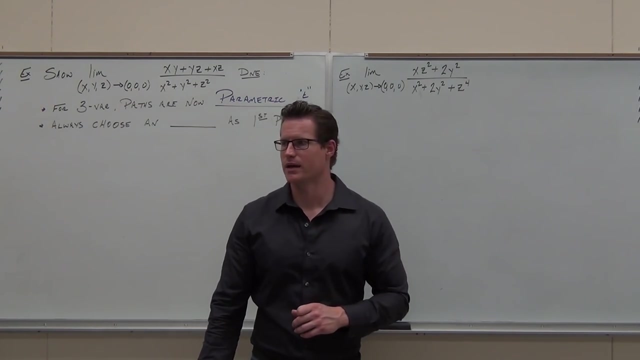 And that's what we're going to be traveling over: paths in 3D that are parametric curves. Quickly, everyone, what variable do we use for parametric curves? T, T, So your whole goal in life right now is to replace X, Y. 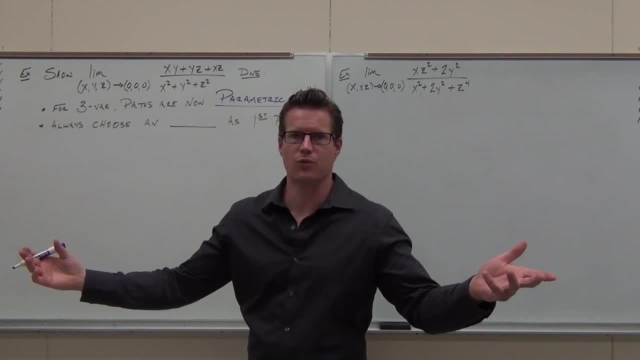 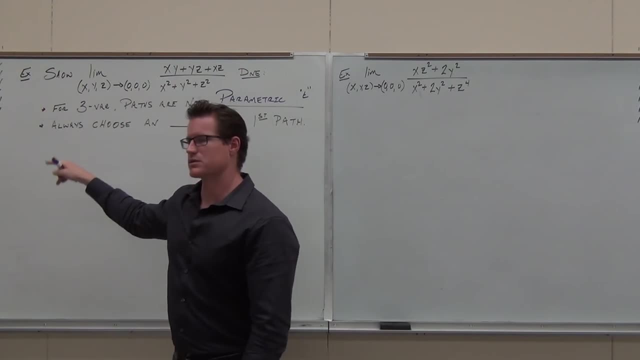 and Z with T. That's literally all we're going to be doing for for one of these things. That's it. We're going to be traveling along those paths. Now, this one, this is. this- is nice. Some people won't talk about this. talk about this. 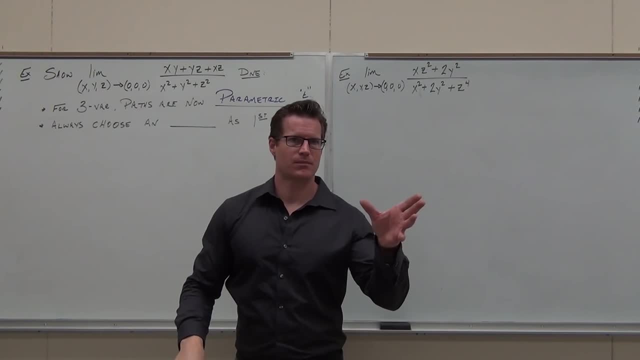 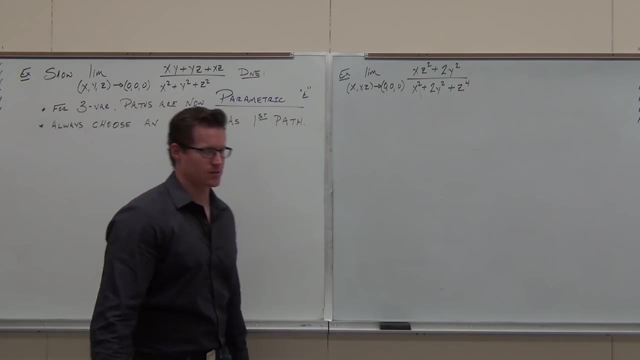 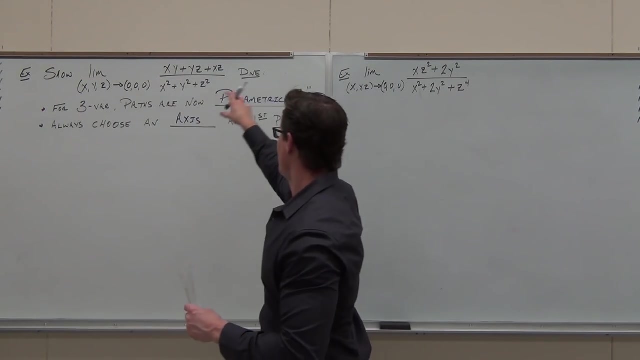 Always choose an axis as one of your paths. Always choose an axis as one of your paths because it's really easy to do that. So I want to show you how to choose an axis, and then we'll talk about how parametric should play a part. 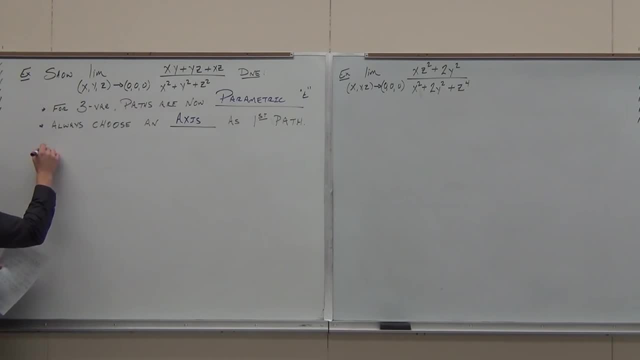 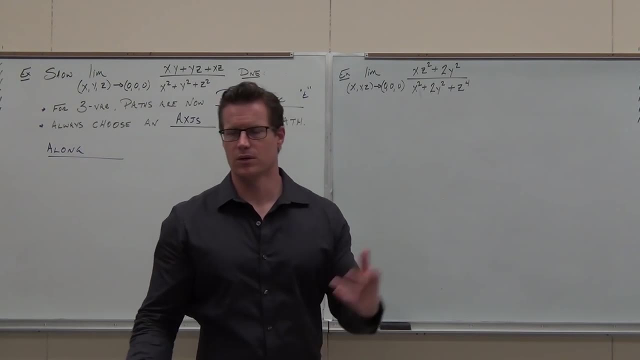 in this, because otherwise I'm literally confusing. So let's, let's start this. So the first thing I want you to do is go along an axis. What axis do you want to go along? X, X, Love it. 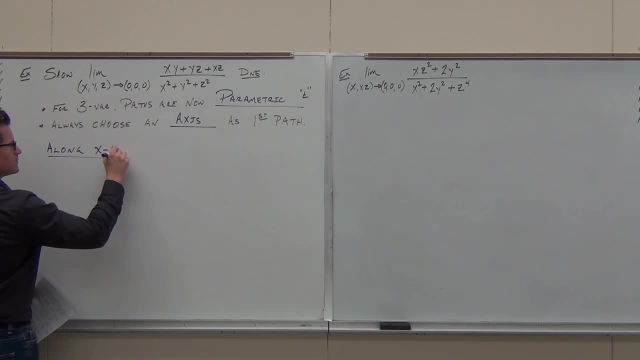 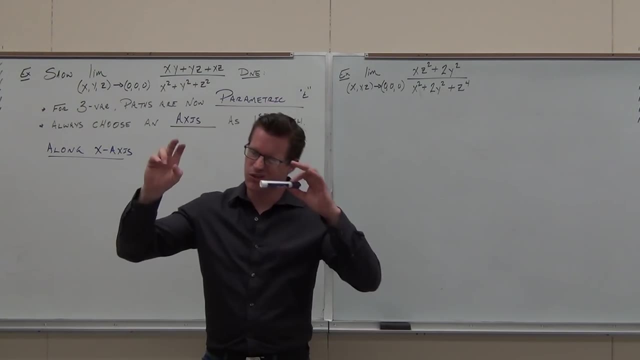 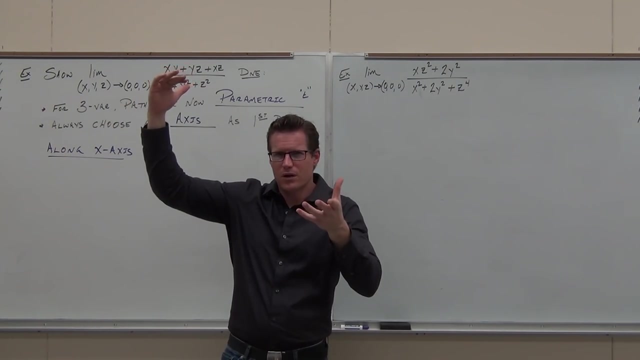 Let's go along. X. I want to explain what's going on. We are in 4, the curve the. it's not in the curve. The surface is in 4D, But we are traveling along that surface over paths in 3D. 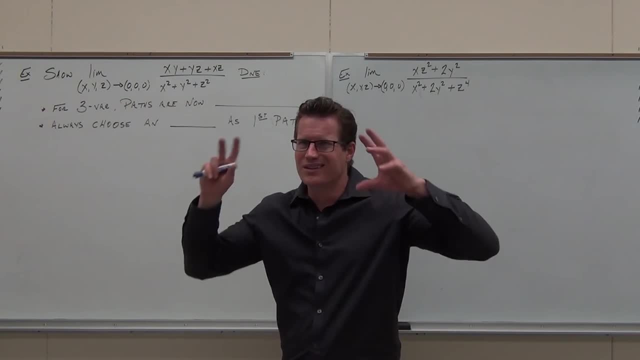 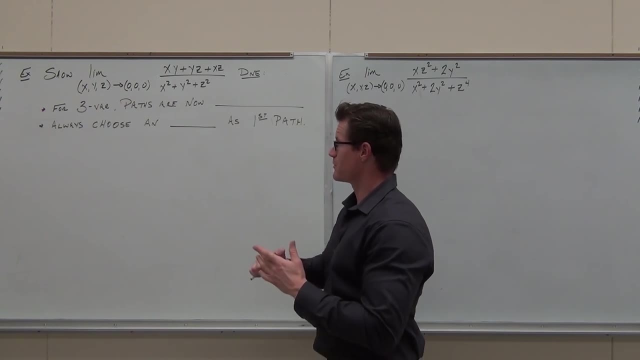 What's nice? don't overthink this. we're not traveling along surfaces. We're still traveling along curves over these 40 surfaces, But for three variables. the paths are now parametric because that's how we defined curves in 3D. 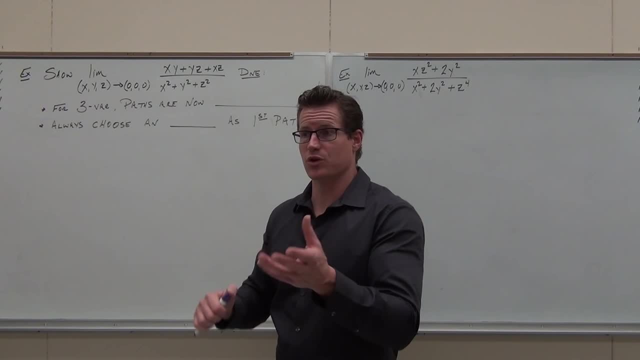 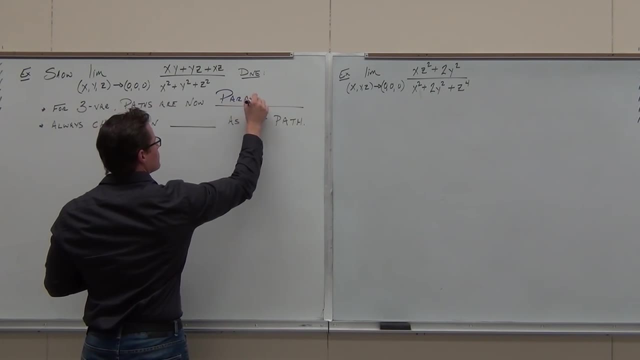 They're now parametric. Does that make sense to you? And that's what we're going to be traveling over? paths in 3D that are parametric curves. Quickly everyone, what variable do we use for parametric curves? T. 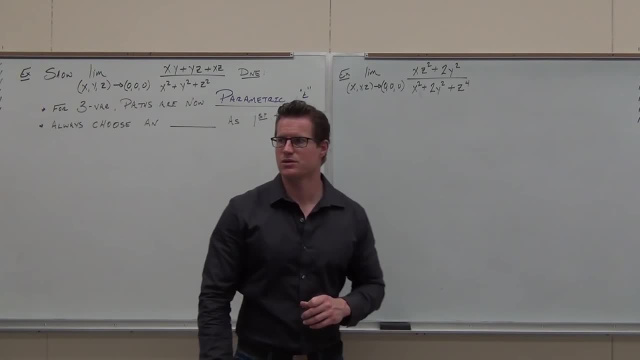 T. So your whole goal in life right now is to replace x, y and z with t. That's literally all we're going to be doing for one of these things. That's it. We're going to be traveling along those paths. 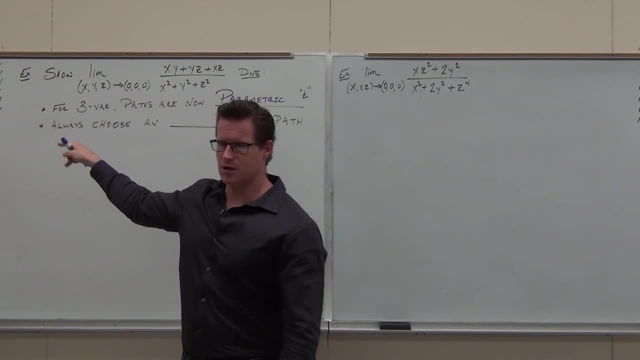 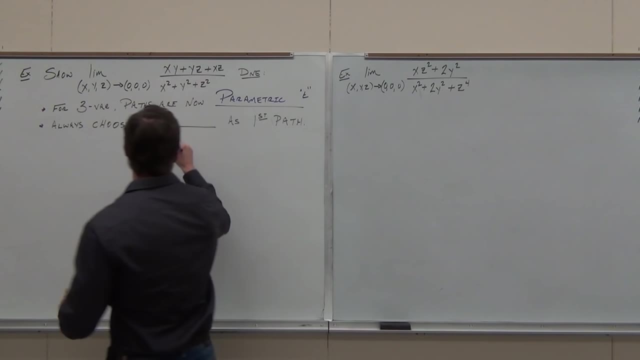 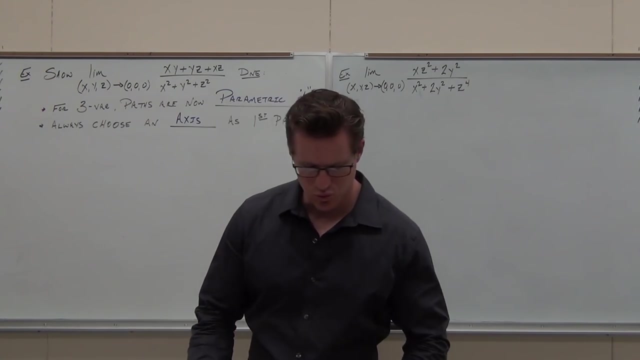 Now this one. this is nice. Some people won't talk about this. Talk about this: Always choose an axis As one of your paths. Always choose an axis as one of your paths, because it's really easy to do that. 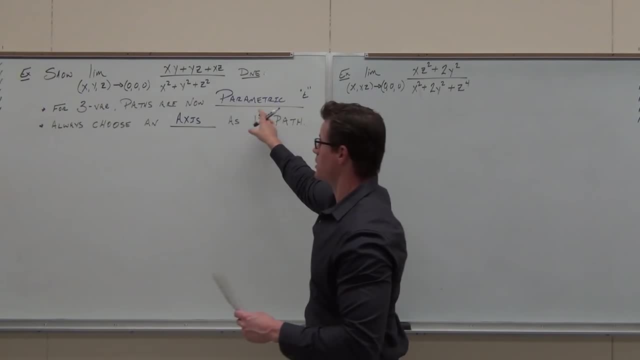 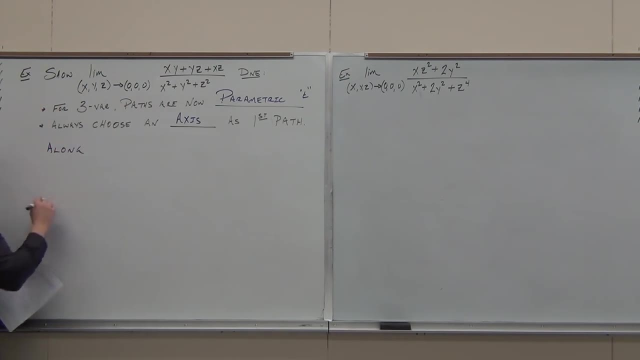 So I want to show you how to choose an axis, and then we'll talk about how parametric should play a part in this, because otherwise I'm literally confusing. So let's start this. So the first thing I want you to do is go along an axis. 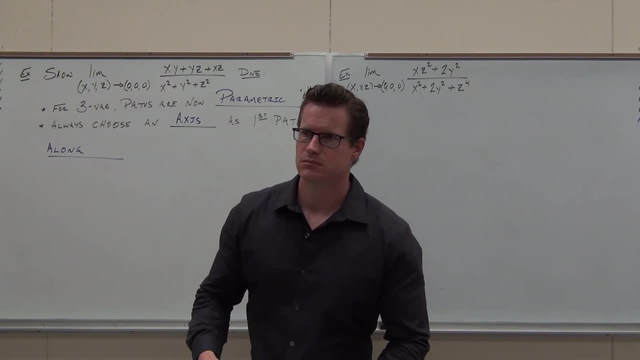 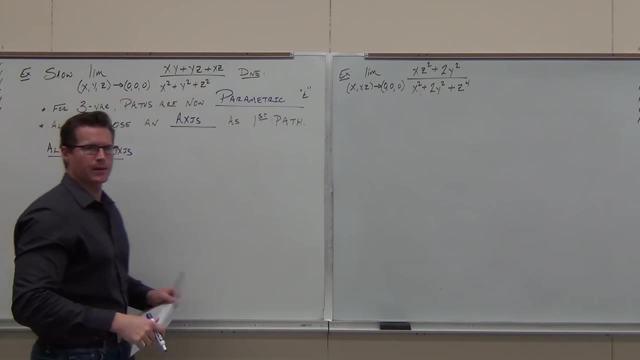 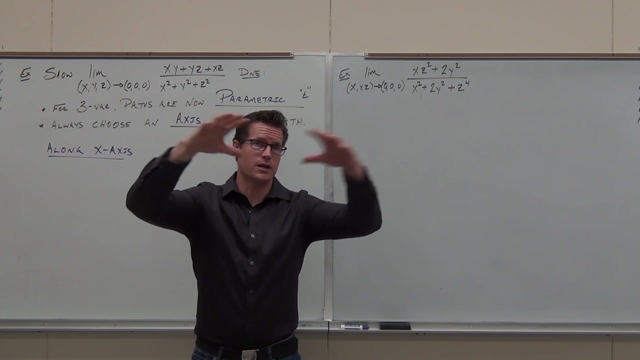 What axis do you want to go along? X, X, Love it, Let's go along. x. I want to explain what's going on. We are in 4D, the curve, the surface- sorry, not the curve, The surface is in 4D, but we are traveling along that surface. 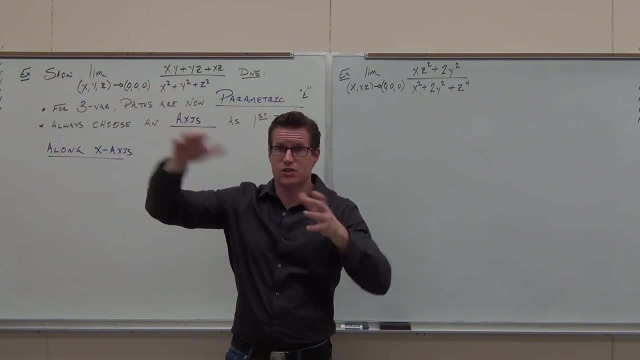 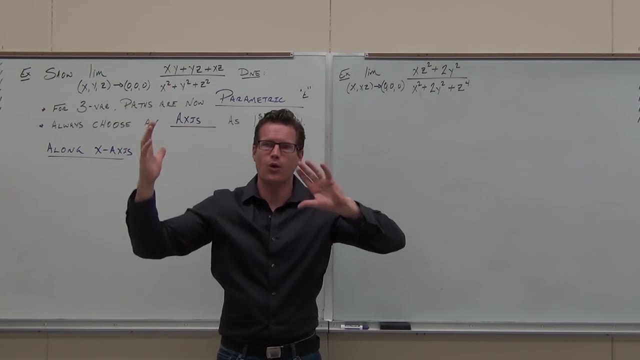 over paths in 3D. Just like in 3D, we are traveling over paths in 2D, Do you guys get it? So we're going to be traveling along this weird 4D surface over a three-dimensional curve. 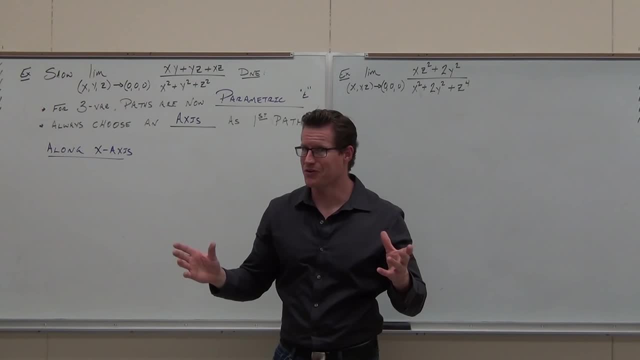 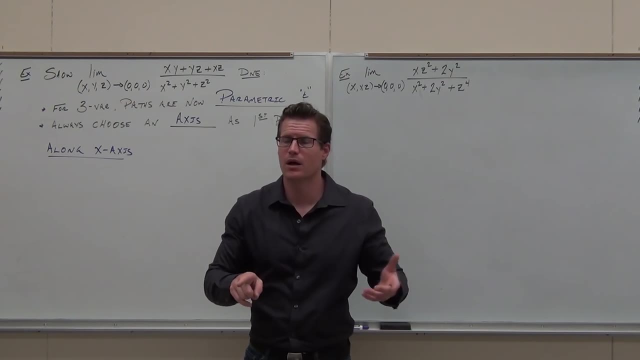 That's what we're trying to describe right now. One three-dimensional curve is simply the x-axis. That is a curve in 3D, isn't it? It's a boring one, but how do we describe it? Well, if we're talking about x's, y's and z's, 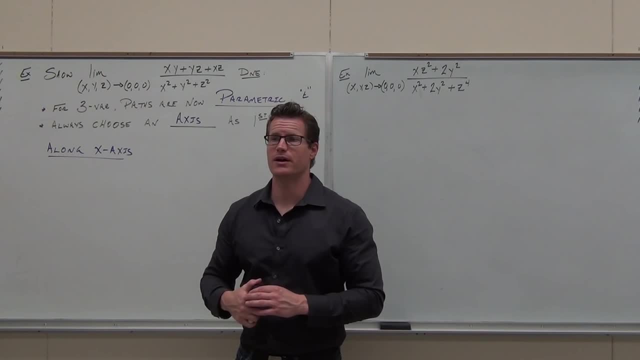 how do we get the x-axis? What's the y value for anything along the x-axis, What is it? Zero. And what's the z value for anything along the x-axis? Zero. So it's really easy. Just set x- sorry, set y and z, both equal to zero. 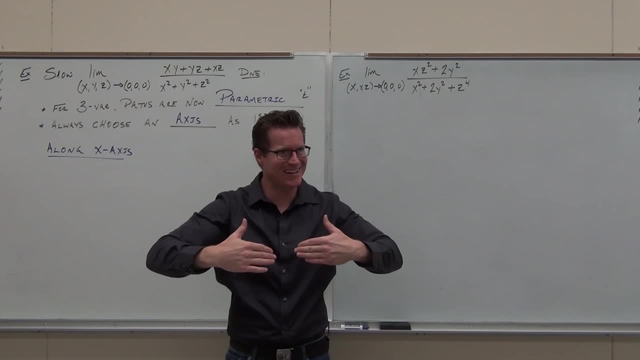 Just like in 3D, we are traveling over paths in 2D. Do you guys get it? So we're going to be traveling along that surface over paths in 3D. Do you get it along this weird 4D surface over a three-dimensional curve? 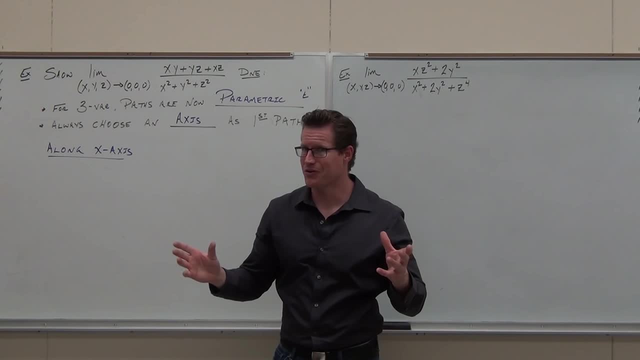 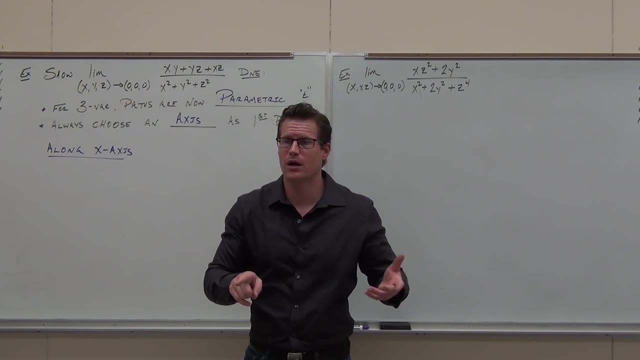 That's what we're trying to describe right now. One three-dimensional curve is simply the x-axis. That is a curve in 3D, isn't it? It's a boring one, but how do we describe it? Well, if we're talking about x's, y's and z's, 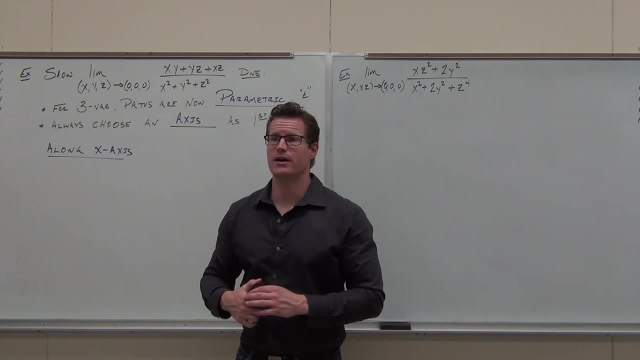 how do we get the x-axis? What's the y-value for anything along the x-axis, What is it? Zero. And what's the z-value for anything along the x-axis? Zero. So it's really easy. Just set y and z both equal to zero. 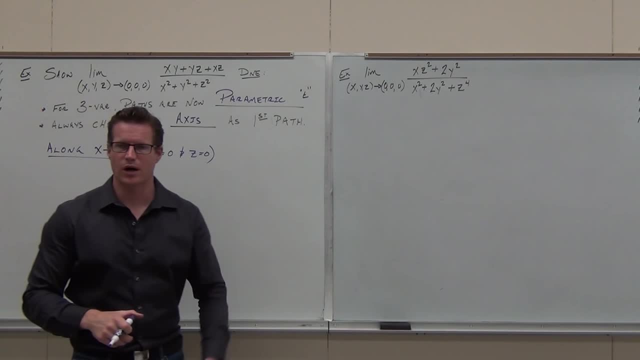 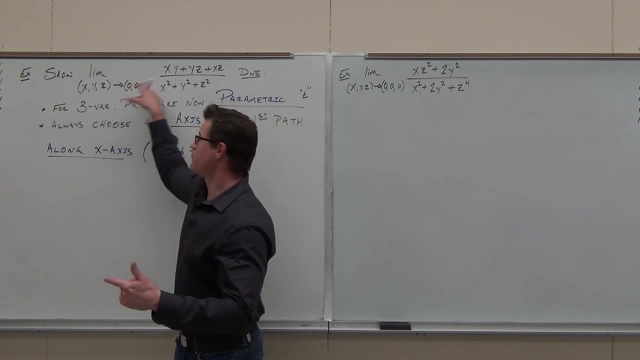 That's probably the easiest thing we've done all day. Just set both x and y equal to zero and you will be along the x-axis. I don't know that you understand that. So what we're looking at right now is what's the value of the function. 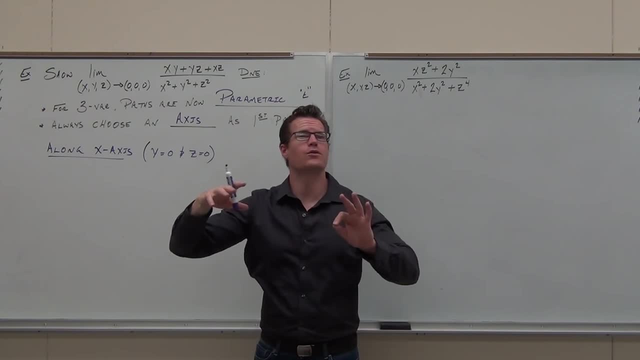 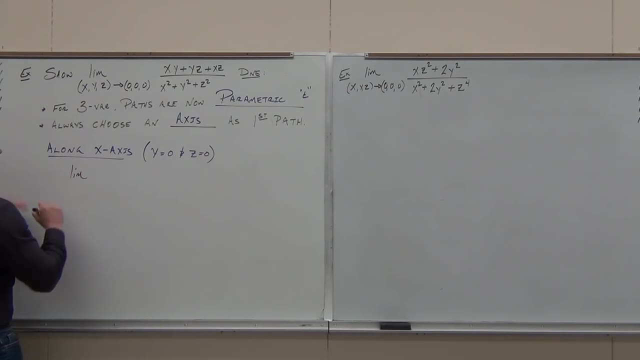 the 4D surface as it's traveling over the x-axis: a 3D curve through space. That's what we're doing. So if we do that, the limit is oh well, hey, if we let y equal zero and z equal zero, we have zero. 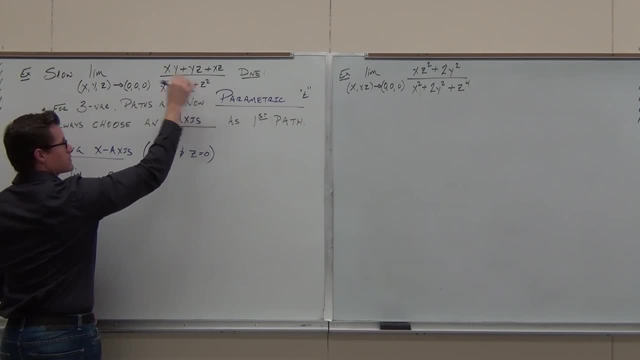 oh see, that's zero, zero, zero, zero, zero. over what? Zero? And what's our only independent variable left, ladies and gentlemen? The x-axis. And what's it got to approach Zero. How much is this limit? 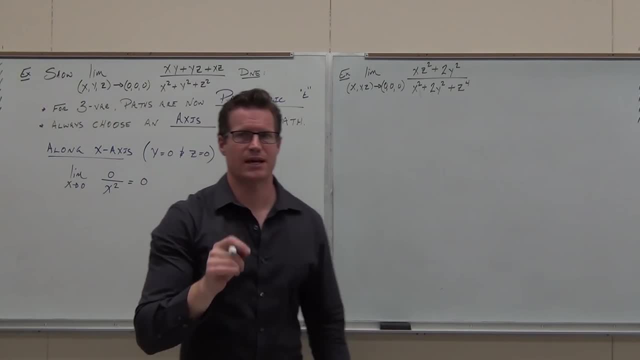 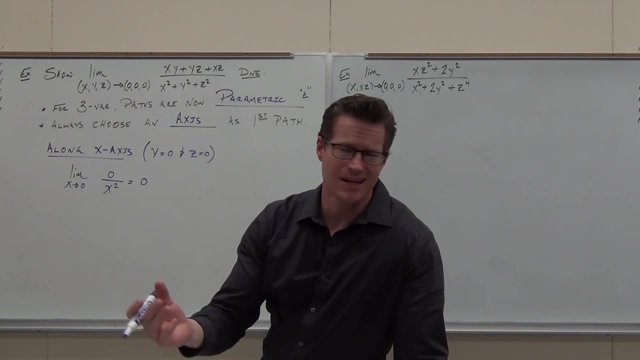 Zero, Perfect. That's why we always choose an axis first if we can. That's why we choose an axis first, Because it's really really easy. You just set y and z equal to zero, or x and z, any two of them. 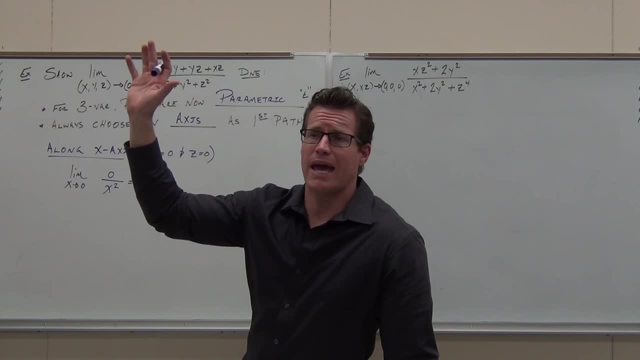 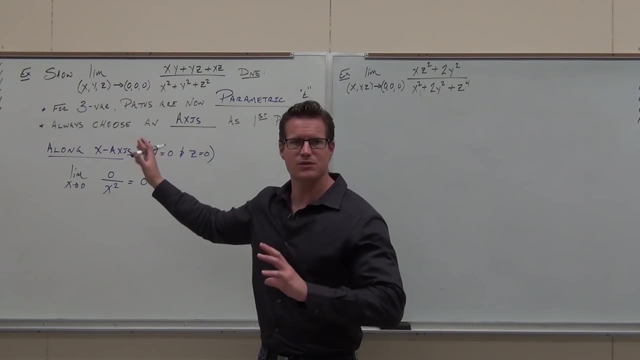 and you're traveling along an axis. So, if you're okay with that one, You can choose z-axis here, because z is now an independent variable, unlike before. okay, it's independent, so we can do that. You guys understand the concept of doing this. 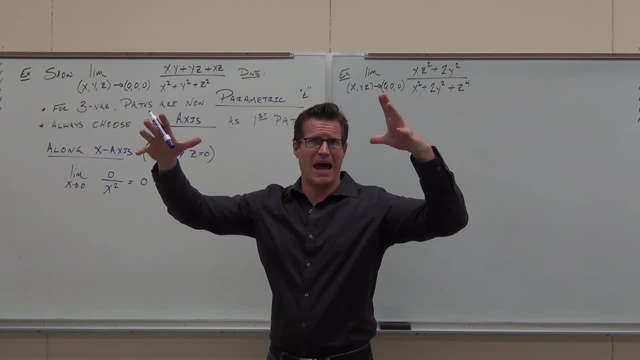 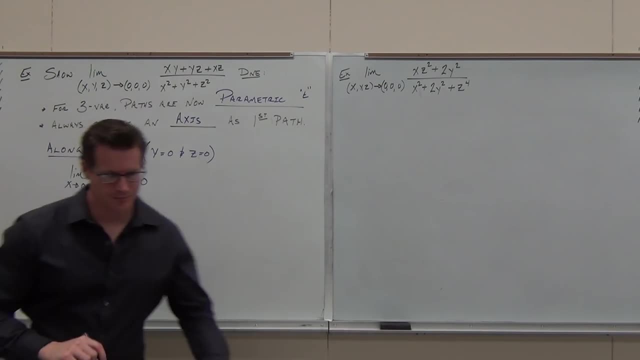 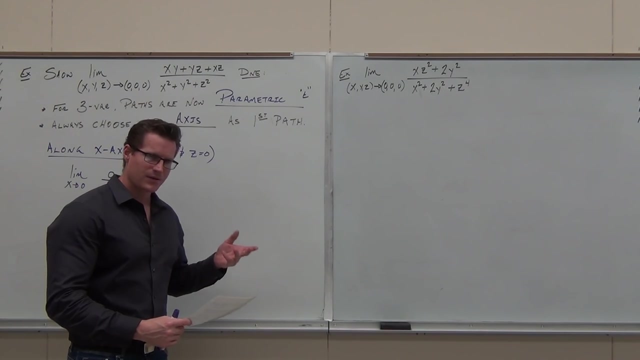 Weird concept of: we're now on a 4D surface and the path that we're over is a 3D path. So what's the other one? Well, the other one. We're going to have to go along a curve that's parametric. 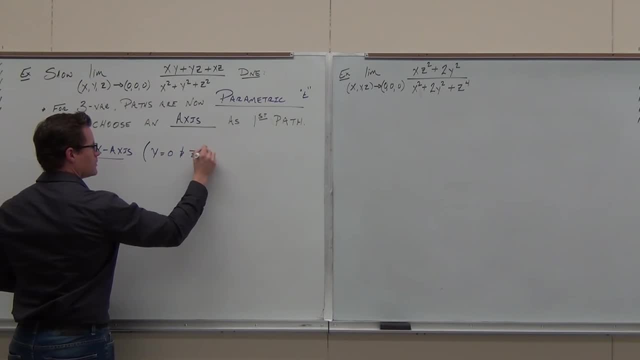 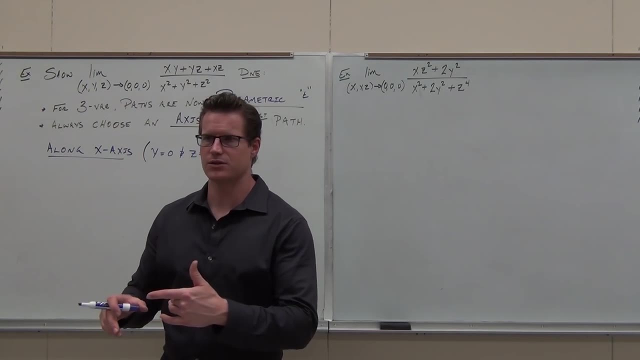 That's probably the easiest thing we've done all day. Just set both x and y equal to zero and you will be along the x-axis. I don't know that you understand that. So what we're looking at right now is: what's the value? 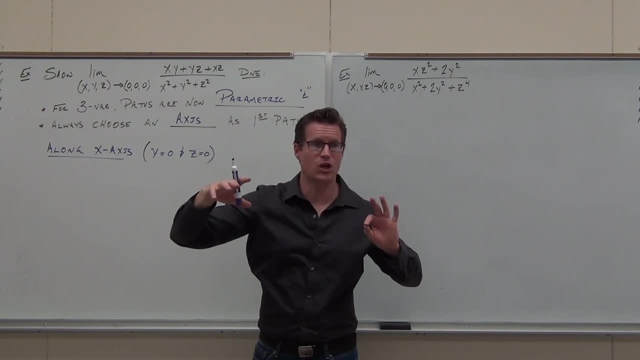 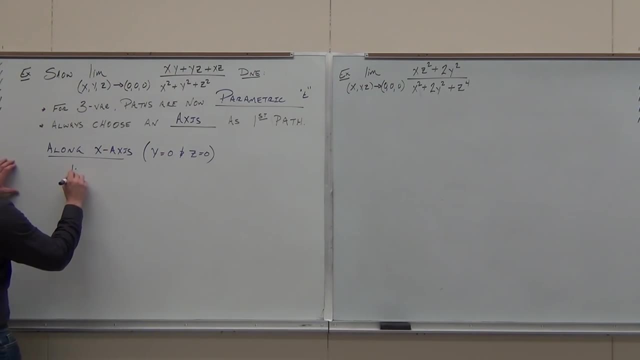 of the function, the 4D surface as it's traveling over the x-axis, A 3D curve through space. That's what we're doing. So if we do that, the limit is oh well, hey, if we let y equal zero. 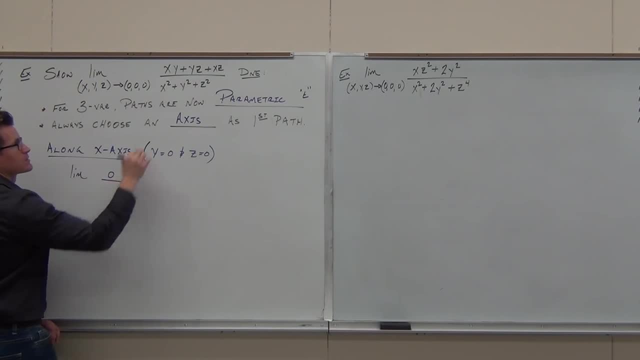 and z equal zero. We have zero. oh see, that's zero. zero, zero, zero, zero. over what? Zero. And what's our only independent variable left, ladies and gentlemen? X, And what's it got to approach? 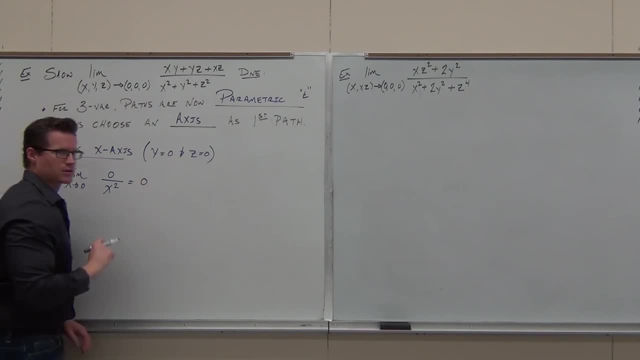 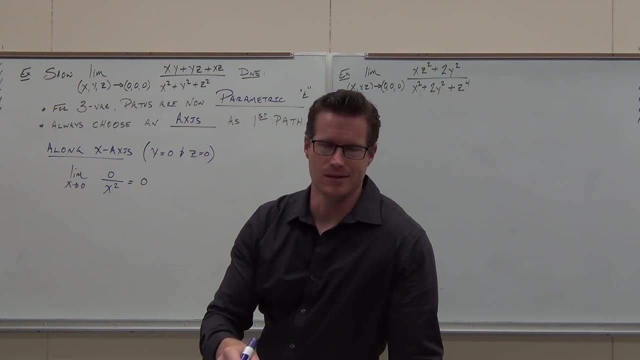 Zero. How much is this limit? Zero, Perfect. That's why we always choose an axis first, If we can. that's why we choose an axis first, because it's really really easy. You just set y and z equal to zero, or x and any two of them. 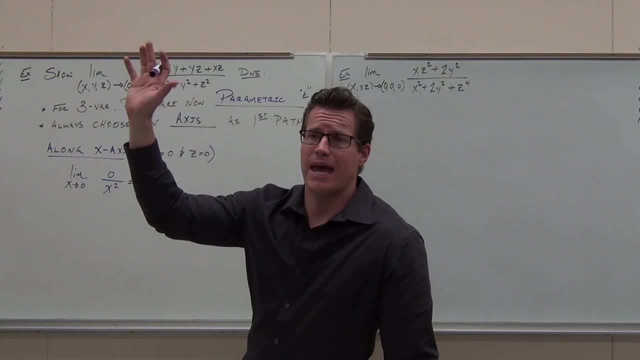 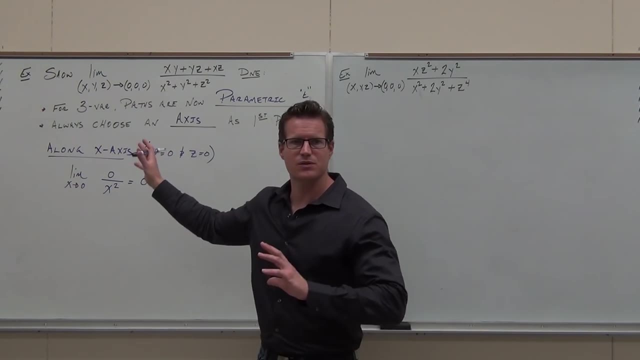 and you're traveling along an axis. So if answer, You can choose z axis here because z is now an independent variable unlike before. okay, It's independent, so we can do that. You guys understand the concept of doing this. 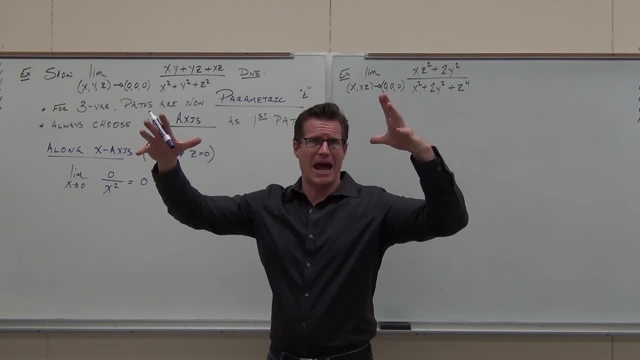 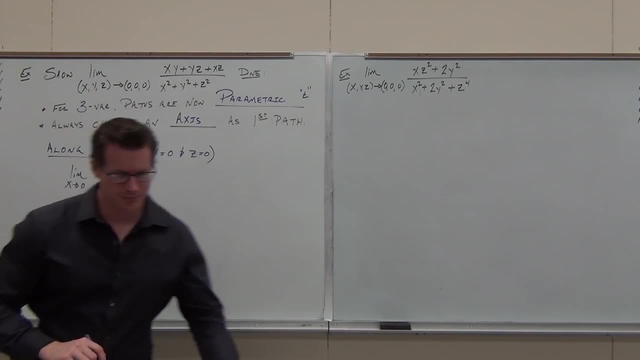 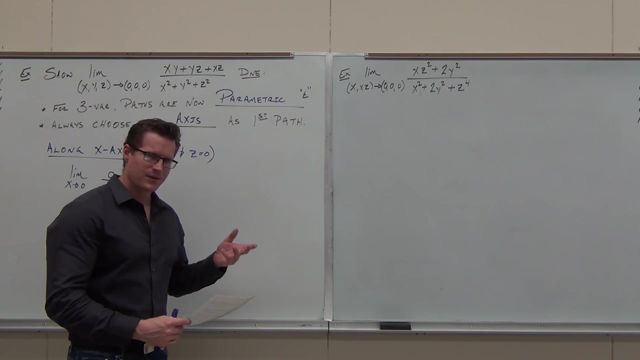 Weird concept of: we're now on a 4D surface and the path that we're over is a 3D path. So what's the other one? Well, the other one. we're going to have to go along a curve that's parametric. 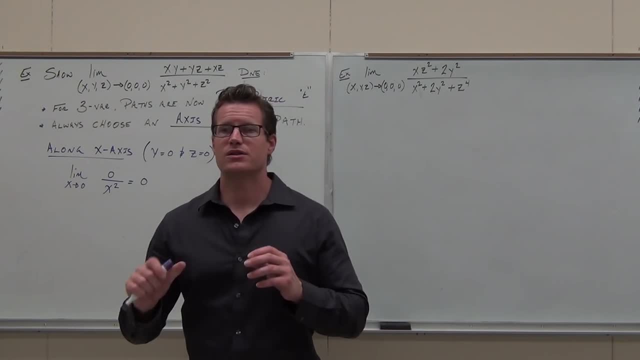 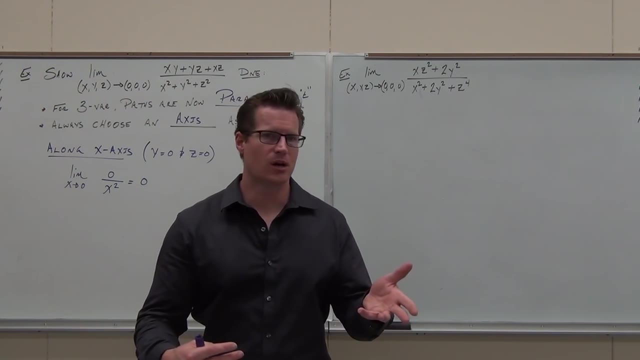 The biggest piece of advice I can tell you is: you're going to have to go along a curve that's parametric. The biggest piece of advice I can tell you is set all of your variables equal to a function of t, because that's a parameter such that your degrees match. 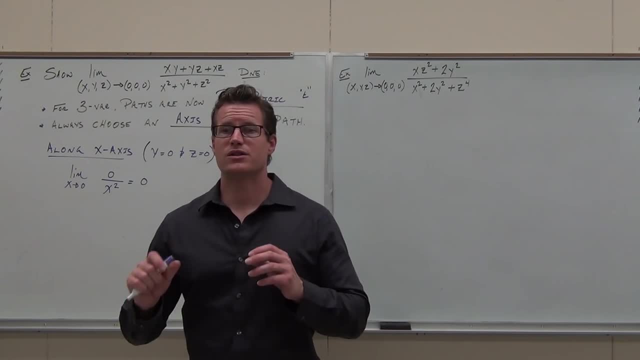 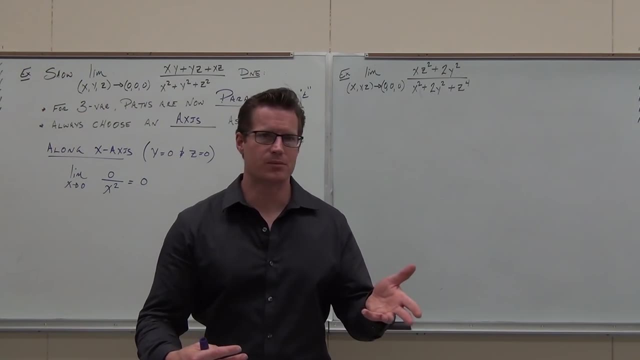 The biggest piece of advice I can tell you is set all of your variables equal to a function of t, because that's a parameter such that your degrees match up, just like we've practiced. So we're going to go along a curve, call it c. 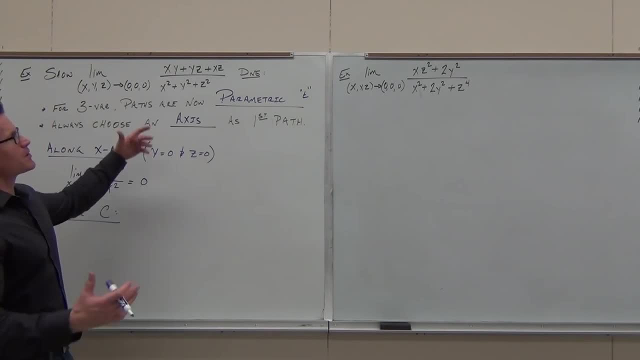 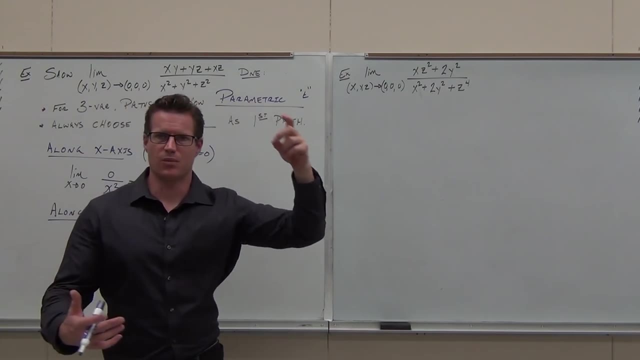 Go along a curve where- well, let's look at it, I'm going to replace x's, y's and z's with t's, what's going to let the powers match up? Well, what I'm looking at is this: is x squared? 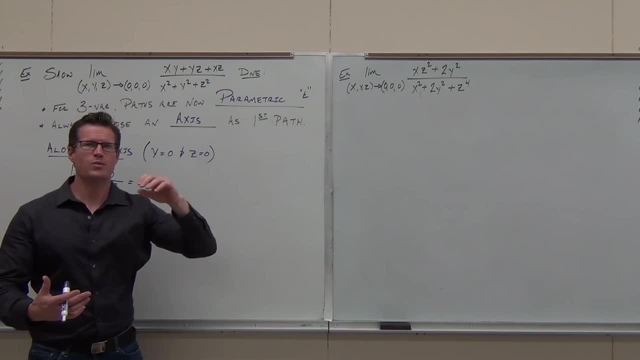 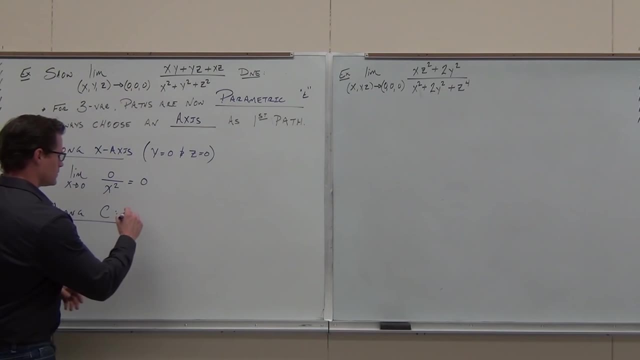 y squared and z squared. If x, y and z all become the same variable, will I be able to combine that stuff? Let's just let x and y and z all equal. t. x equals t, y equals t, z equals t. 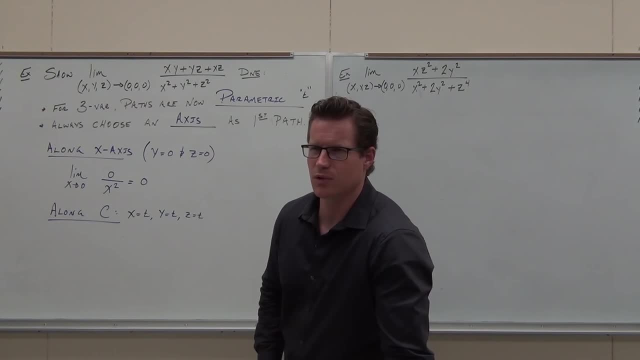 What is it? What is x equals t, y equals t and z equals t? What is that curve? It's a line. It's a line through space. That's all it is. Do you see the parametric line? That's what we're traveling over now. 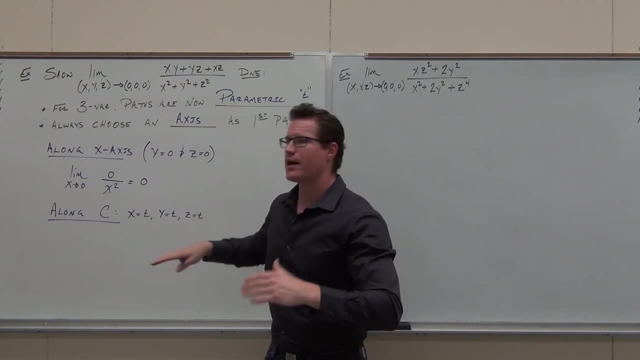 So in 4D we're going to be traveling along the surface over that three-dimensional line. That's it. That's why we use parametrics, because to travel through space we need parametrics. So we're going to be okay with that one. 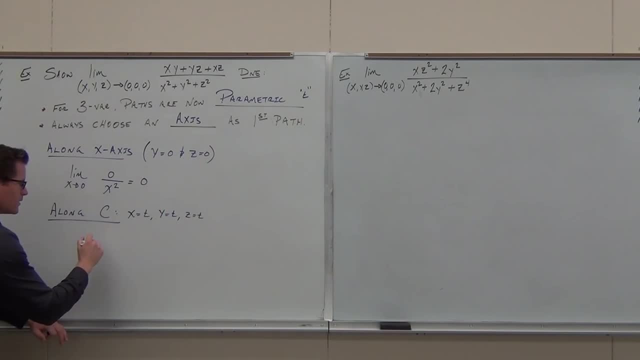 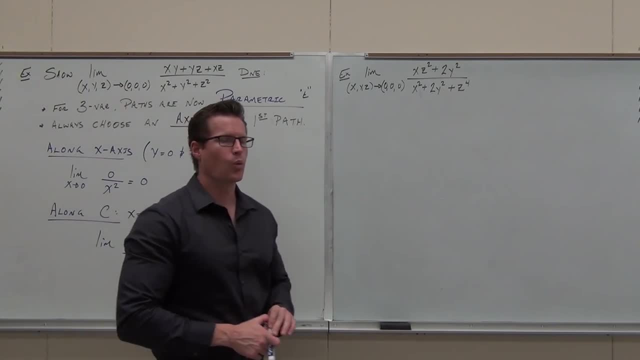 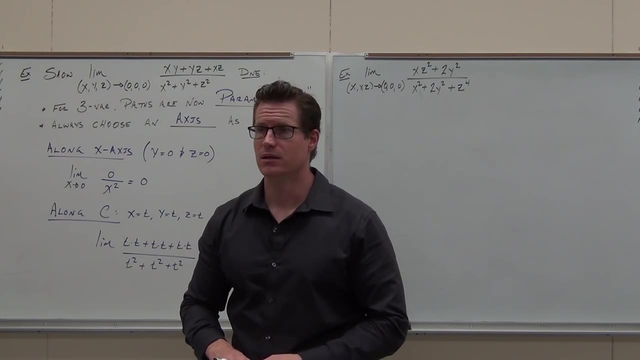 Super fun. Hey, what now? now? this is an interesting question. What is now our independent variable, since we basically just parameterized this function t? What's t approaching Zero? not zero, zero, zero, because if we let 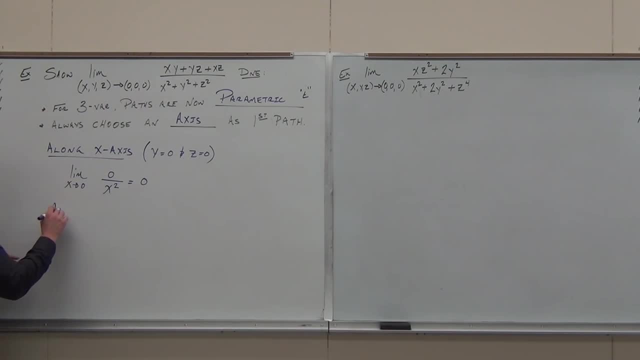 up, just like we've practiced. So we're going to go along a curve, call it c. Go along a curve where- well, let's look at it- I'm going to replace x's, y's and z's with t's. 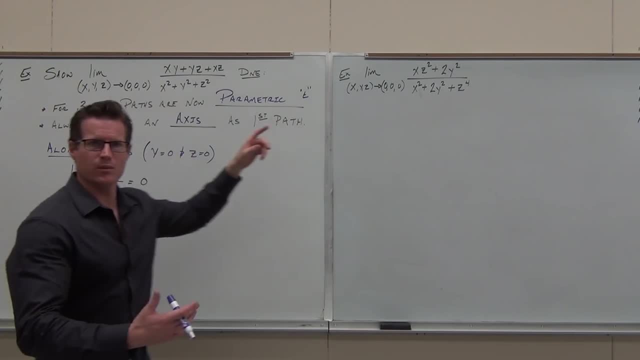 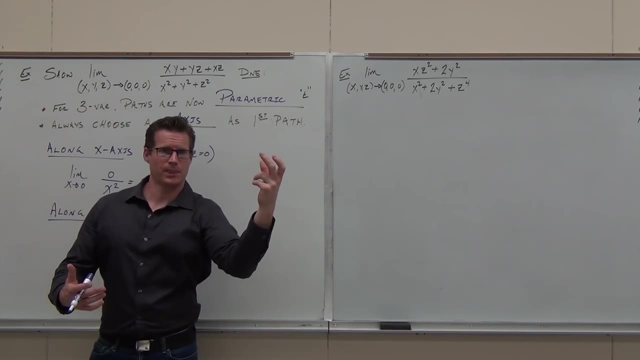 What's going to let the powers match up? Well, what I'm looking at is this: is x squared, y squared and z squared? If x, y and z all become the same variable, will I be able to combine that stuff? 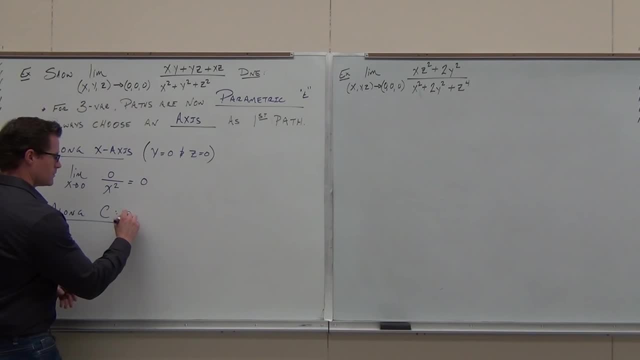 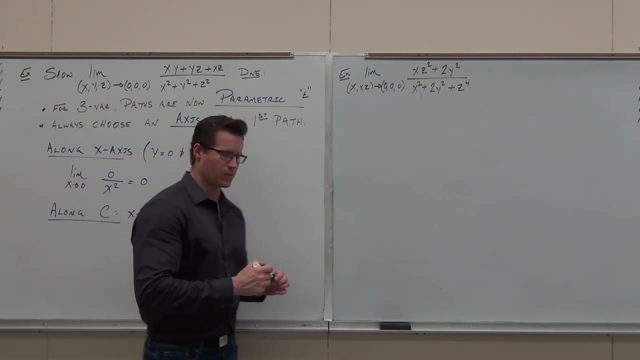 Let's just let x and y and z all equal t. x equals t, y equals t, z equals t. What is it? What is x equals t, y equals t and z equals t? What is that curve? It's a line through space. 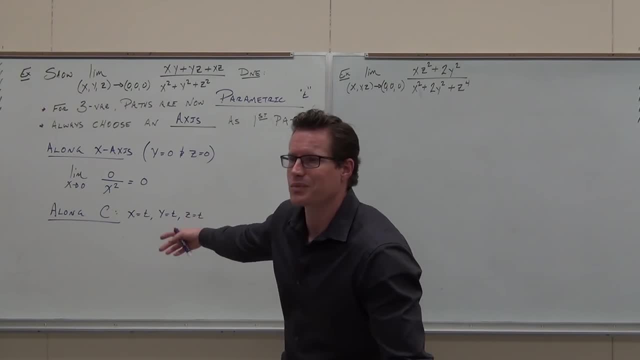 That's all it is. Do you see the parametric line? That's what we're traveling over now. So in 4D we're going to have to go along a curve. that's parametric. So in 4D we're going to have to go along a curve. that's parametric. 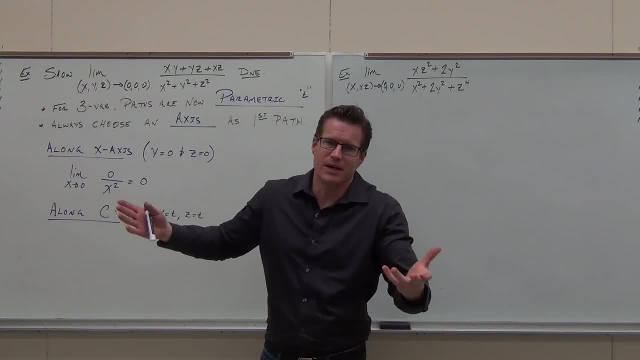 So in 4D we're going to have to go along a curve. that's parametric. So in 4D we're going to be traveling along the surface over that three-dimensional line. That's it. That's why we use parametrics. 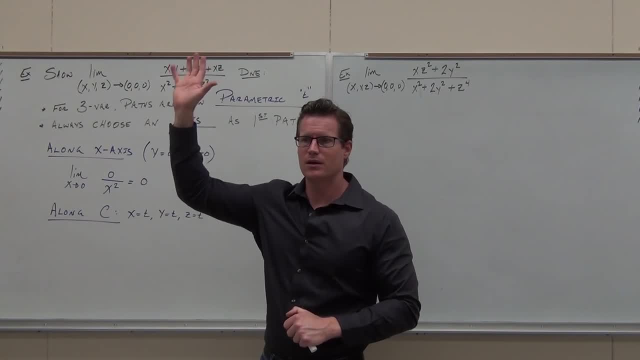 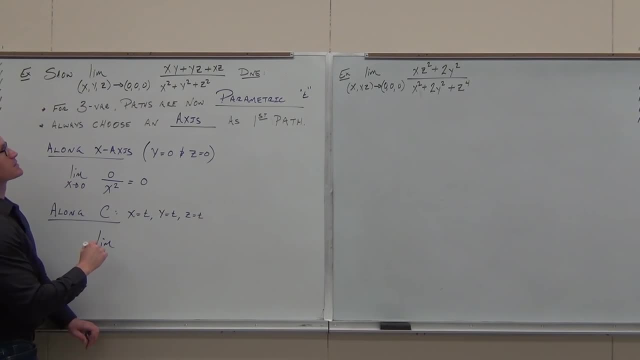 because to travel three-space we need parametrics. So we're basically okay with that one. Now let's make the substitution. If x and y and z are all t, then our limit becomes. well, let's see now. 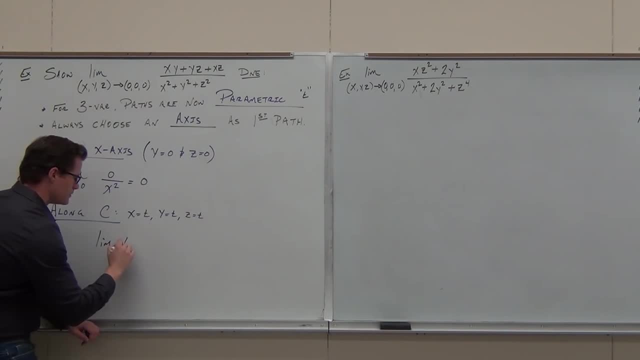 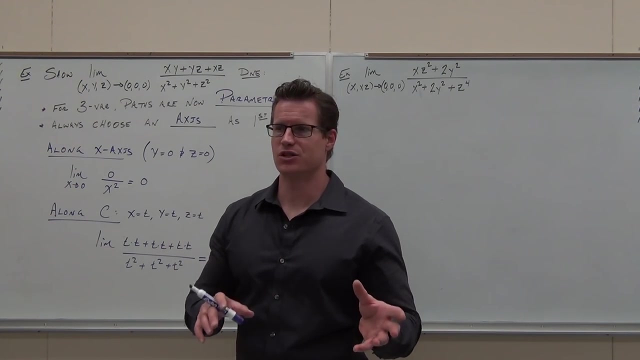 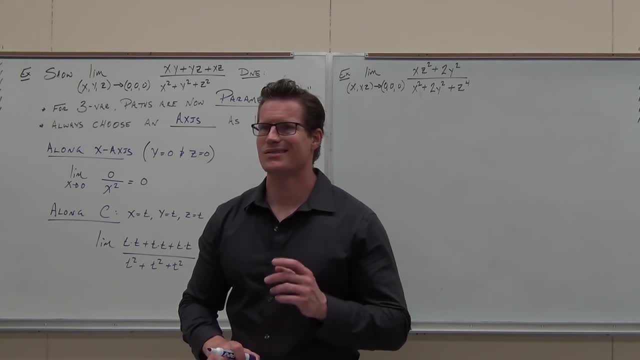 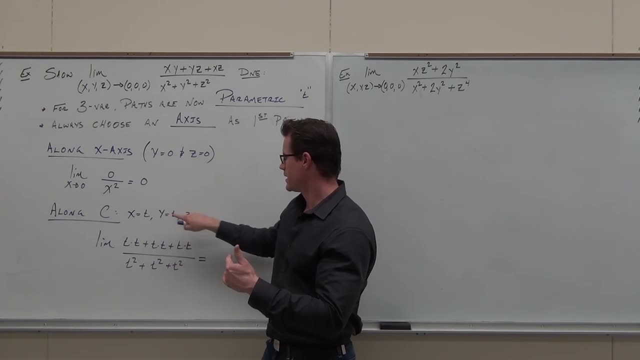 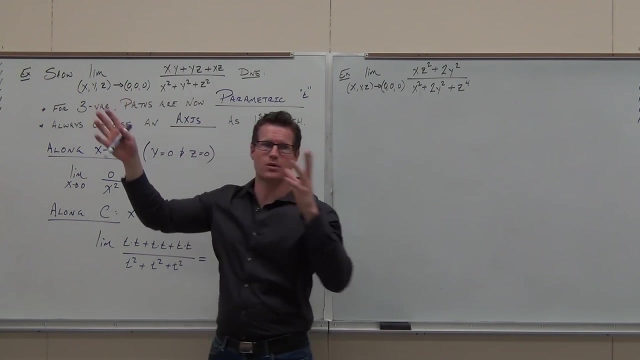 t. What's t approaching? Zero, Zero, Zero, Not zero, zero, zero. Because if we let watch carefully, If we let t approach zero, x and y and z also approach zero. So Letting t approach zero, lets the point approach zero, zero, zero. 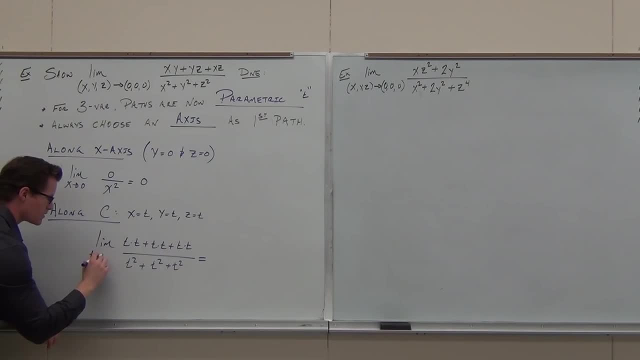 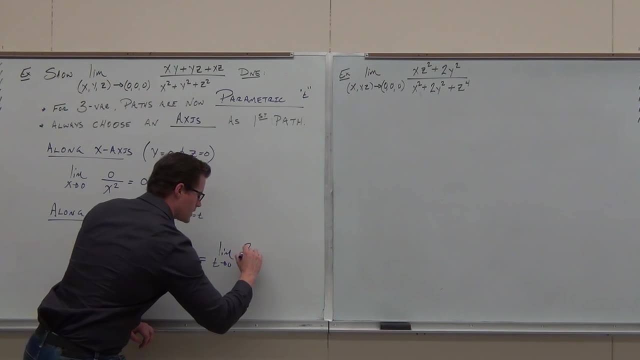 Does that make sense? So just kind of watch that sort of stuff. So t is approaching zero, So that's the limit as t approaches zero. of t squared, t squared, let's see 3t squared over 3t squared. 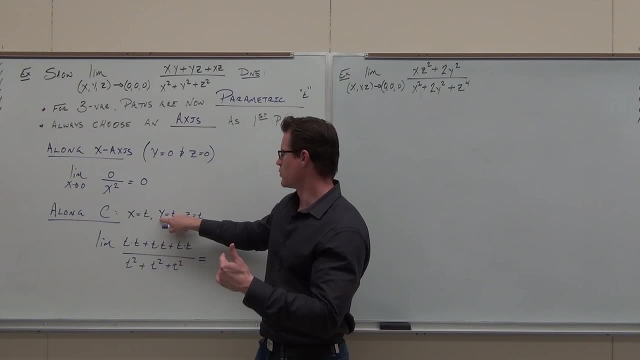 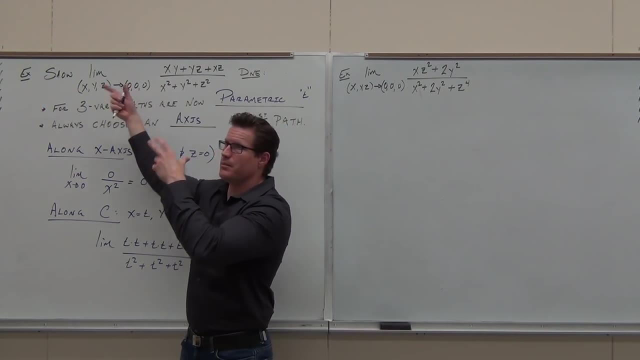 watch carefully. if we let t approach zero, x and y and z also approach zero. So letting t approach zero lets the point approach 0, 0, 0.. Does that make sense? So just kind of watch that sort of stuff. 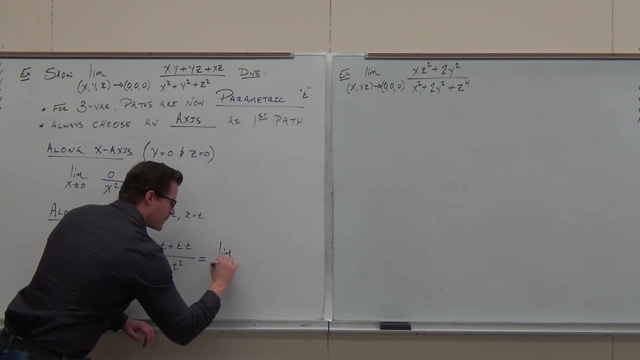 So t is approaching zero. So that's the limit as t approaches zero. of t squared, t squared, let's see 3t squared over 3t squared. How much does that equal? Come on, Does that prove something for us? 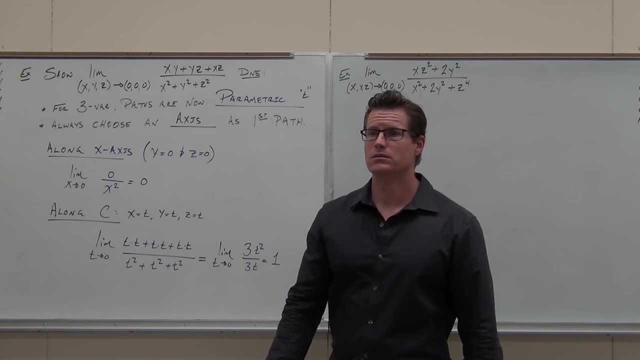 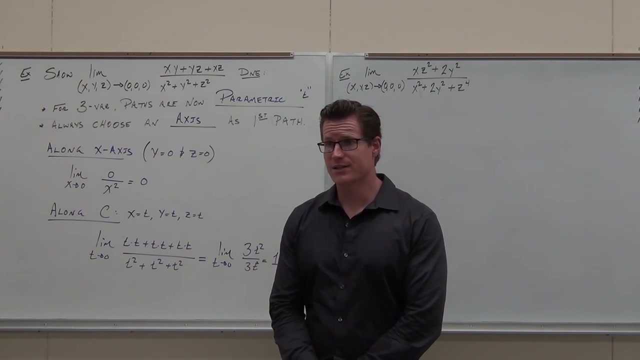 It's about the 3t squared over 3t squared. Oh Yeah, One. It wouldn't have been one before, Sorry. What does it prove for us That it doesn't? why Does not exist? Because, as I'm traveling along the 4d surface, 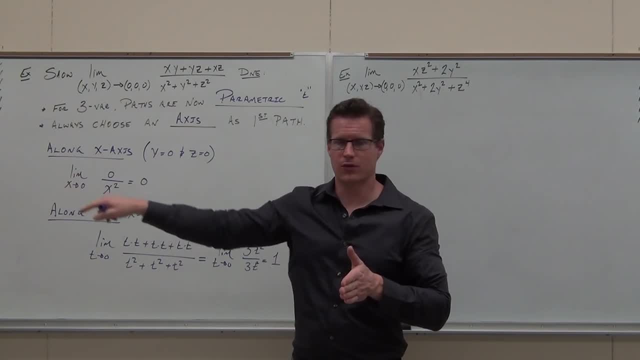 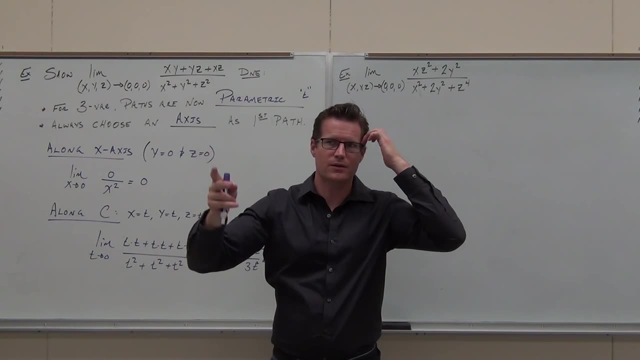 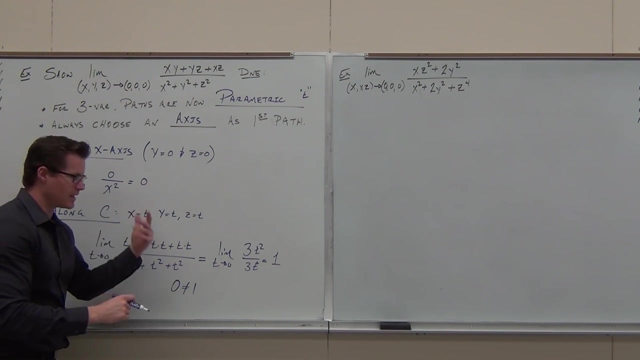 over that path, the x-axis- and over that, that path, which is a line through space, the value of the function is different. That's what we're proving here. Does it make sense to you? So, since zero does not equal 1, the limit does not exist. 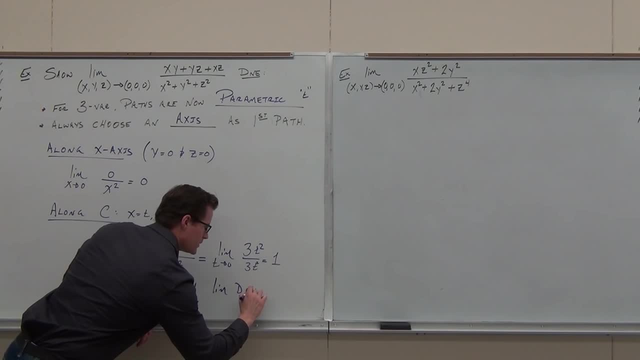 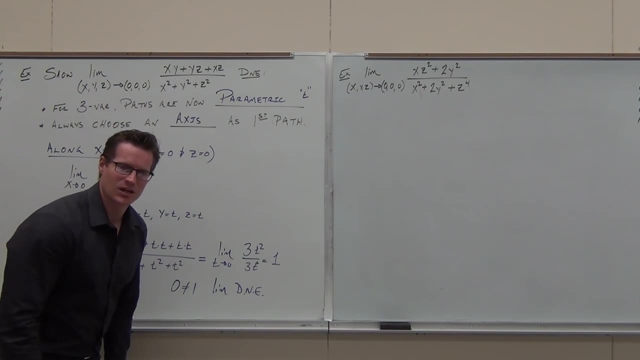 at 0, 0, 0.. Please wrap this up and at least for my class, I want a statement, at least something that you actually understand the concept. Do not just say doesn't exist, Doesn't exist ever. 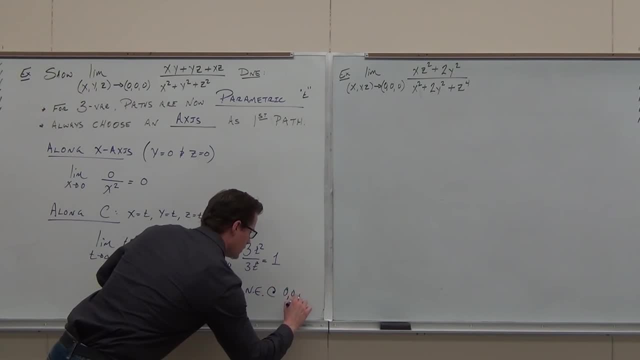 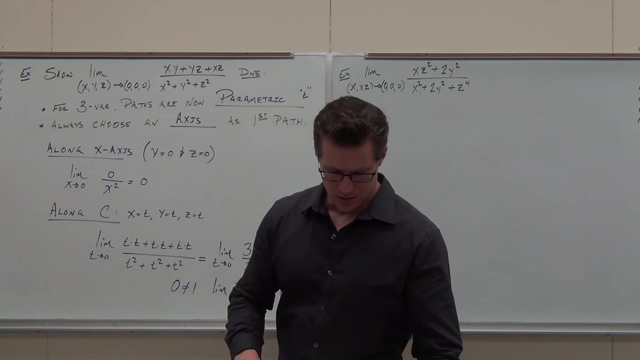 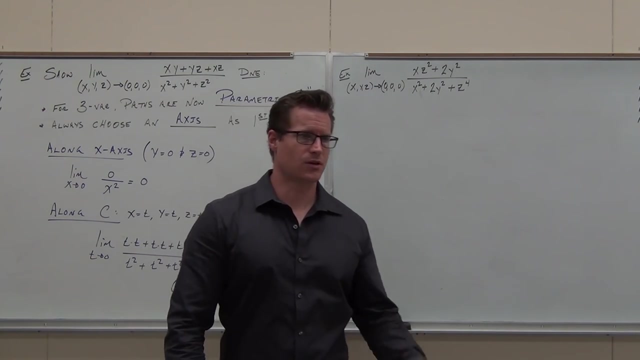 Come on, We just proved that because of these two paths, the limit doesn't exist as we approach that point. That's the idea. Listen, I'm not going to make it through the whole thing here. I just want to give you the blurb about how you start it. 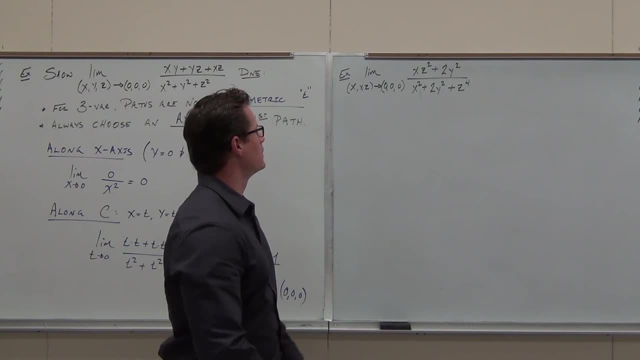 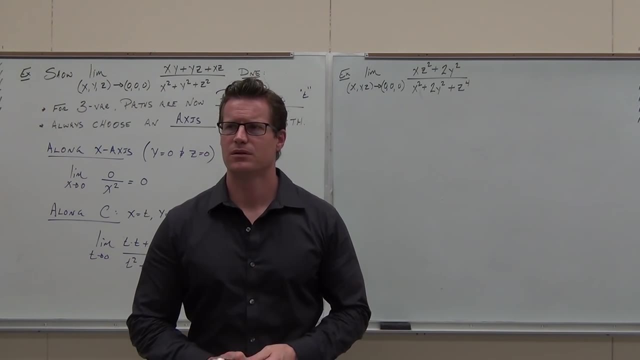 Don't worry, we'll show you that next time. What would you do first If I wanted to prove this doesn't exist? what would you do first? Go along, what An axis So you do. maybe the x-axis, Yeah. 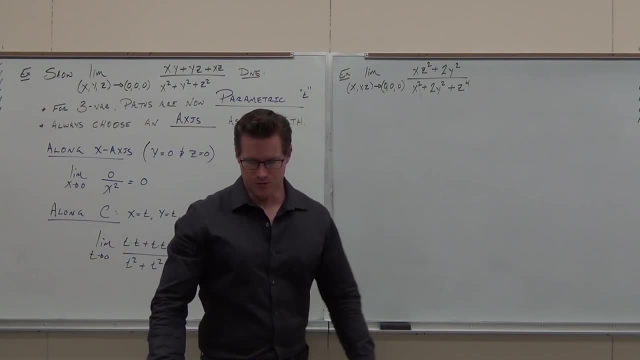 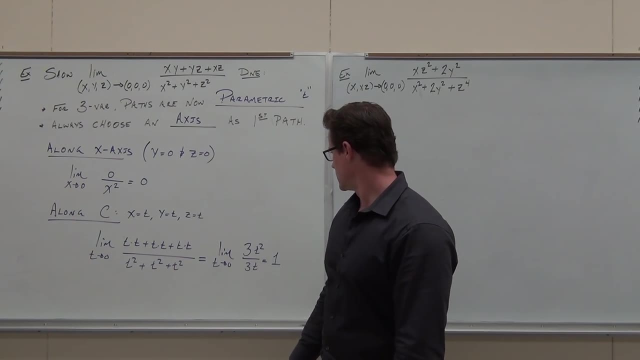 How much does that equal? Come on, Does that prove something for us? Yeah, How's about the 3t squared over 3t squared? Oh, Yeah, One. It wouldn't have been one before, Sorry. What does it prove for us? 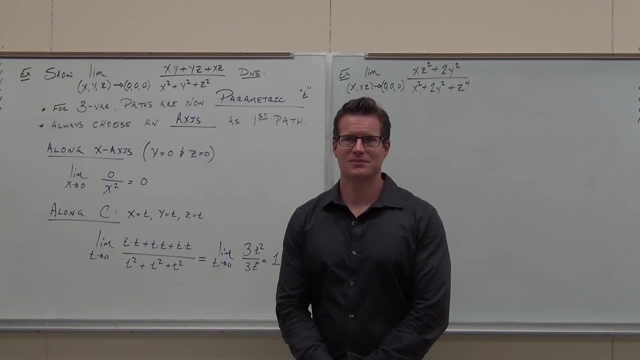 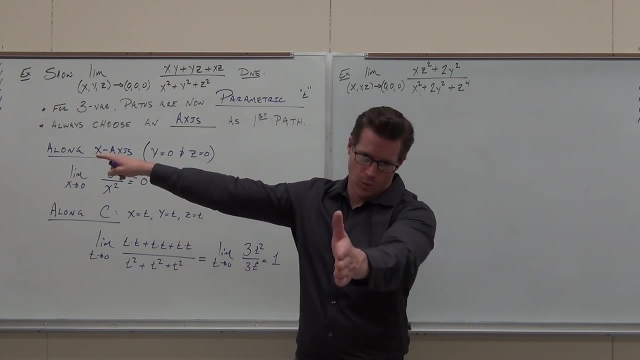 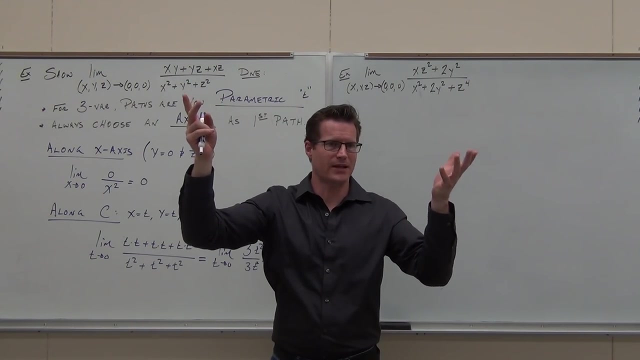 That it doesn't why? Because, as I'm traveling along the 4d surface, over that path- the x-axis- and over that path, which is a line through space, the value of the function is different. That's what we're proving here. 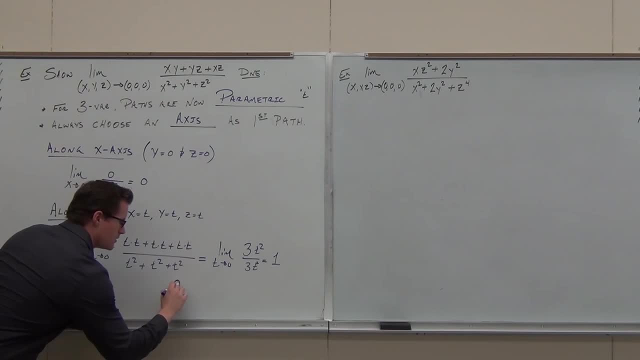 Does it make sense to you? So, since zero does not equal one, the limit does not exist at zero, zero, zero. Please wrap this up and, at least for my class, I want a statement, at least something that you actually understand the concept. 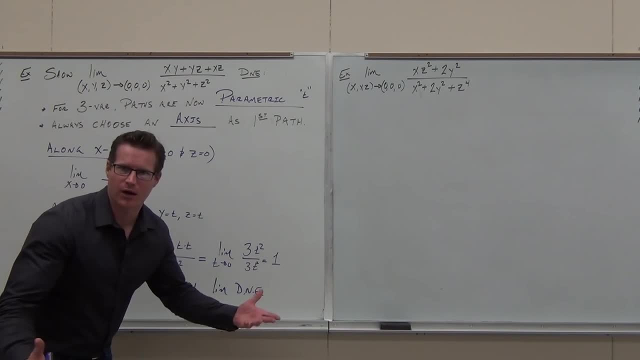 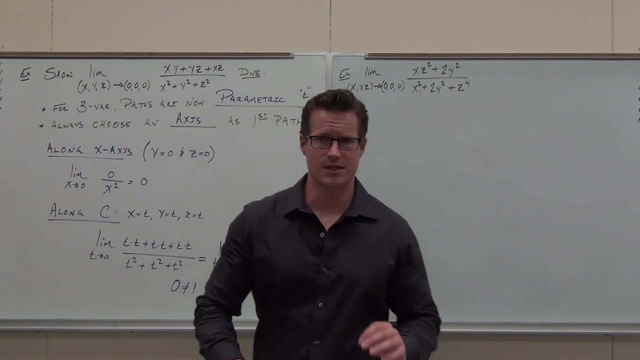 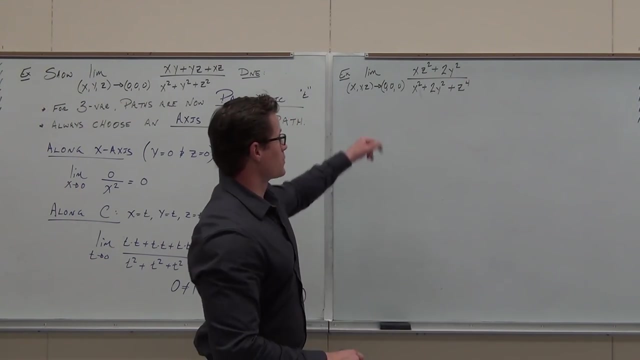 Do not just say doesn't exist, Doesn't exist ever. Come on, We just proved that because of these two paths, the limit doesn't exist as we approach that point. That's the idea. Listen, I'm not going to make it through the whole thing here. 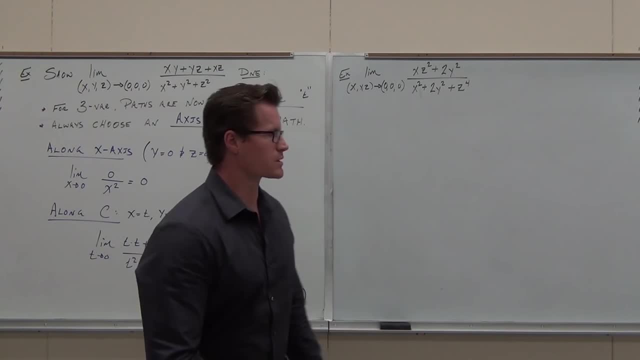 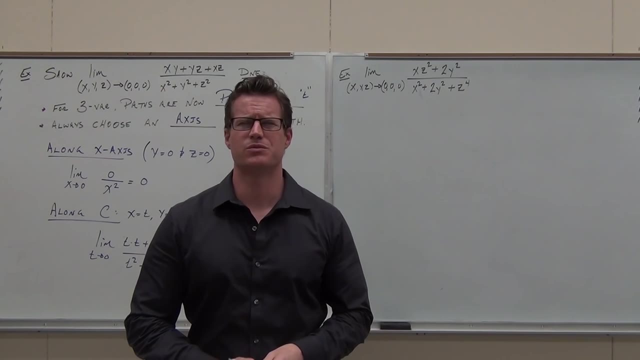 I just want to give you the blurb about how you start it. Don't worry, we'll show you that next time. What would you do first If I wanted to prove this doesn't exist? what would you do first? Go along what? 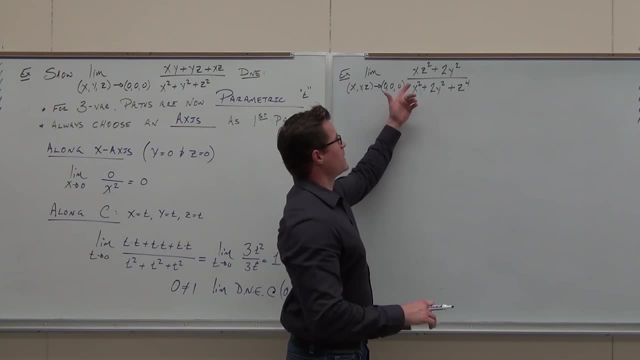 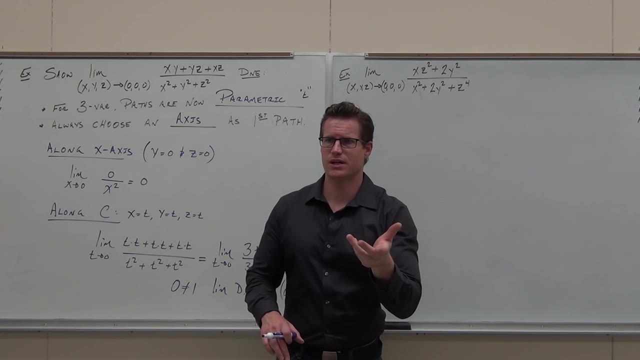 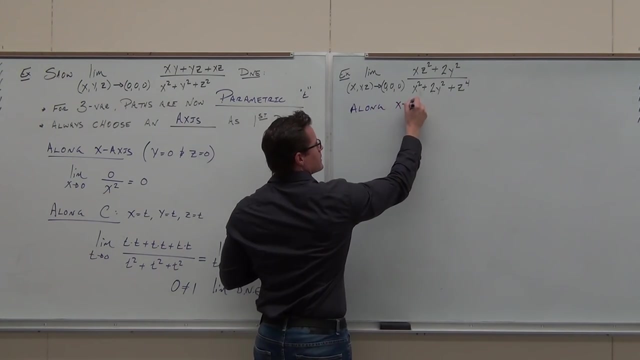 An axis, An axis, So you do maybe the x-axis. you'd get. y equals zero and z equals zero. You get zero over x squared, you'd still get zero. Do you guys see what I'm talking about? What I want to focus more? so one of them along x-axis, and we would get the limit. 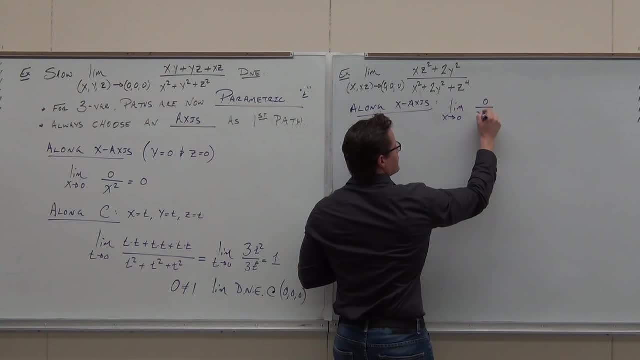 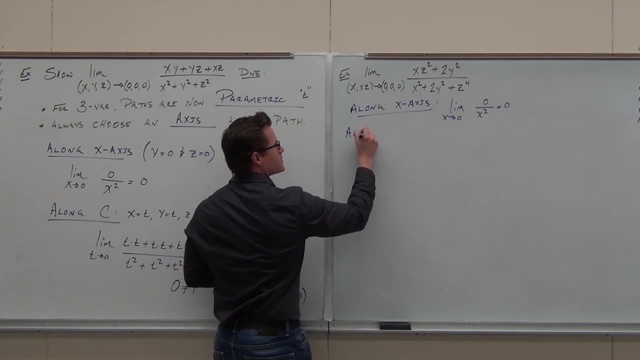 as x approaches zero of zero over x squared, and that's zero. That's still zero. That's an easy one. That's nice. You always- pretty much always- do that. What I want to focus on is the parametric curve that I want to create. 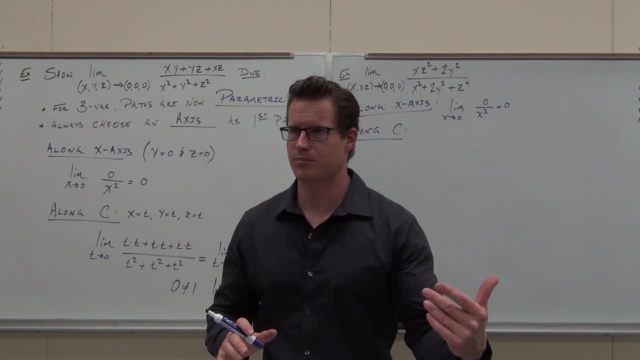 This is a little harder because you don't just do x, y and z all equal to the same parameter. What I want you to think about- I'm going to give you about 30 seconds. just think, Just think about it. 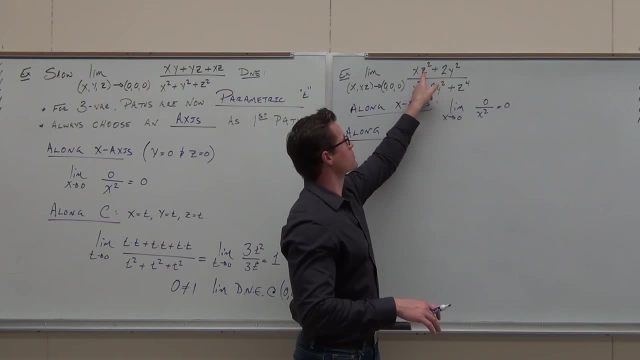 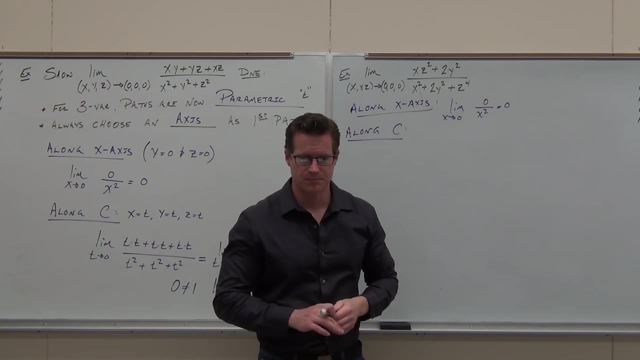 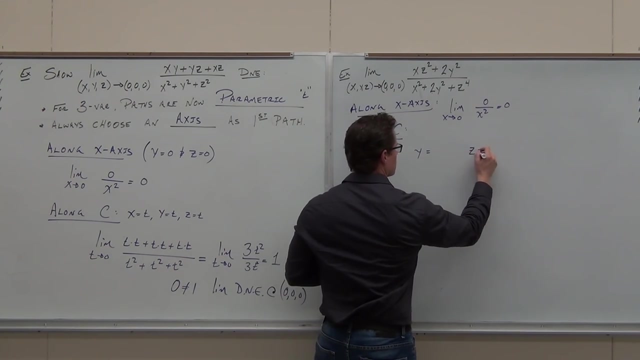 How can I make these powers all the same? How can I make those powers the same? If I can't, how can I do it? So think about it. What's the, what's the variable with the largest power right now? 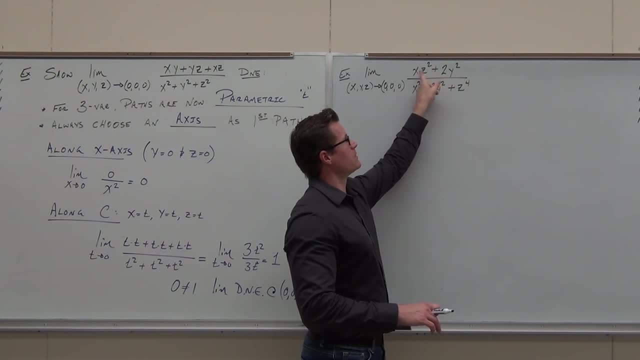 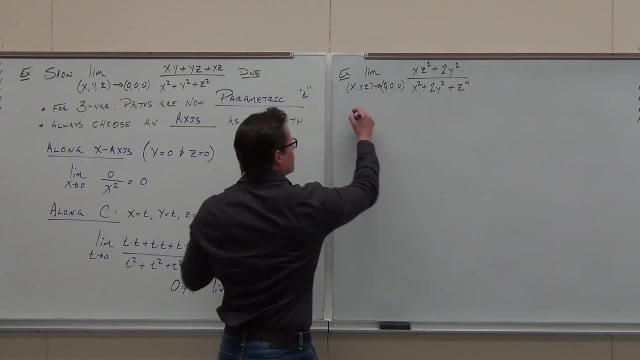 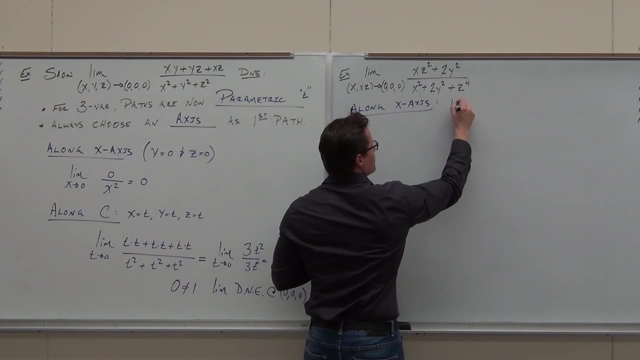 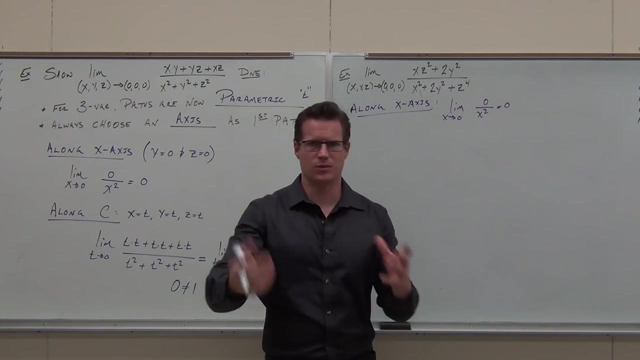 Do you guys see what I'm talking About? I want to focus more. so one of long x-axis, And we would get the limit as x approaches, zero of zero over x squared, and that's zero and still zero, You'd you, that's an easy one. 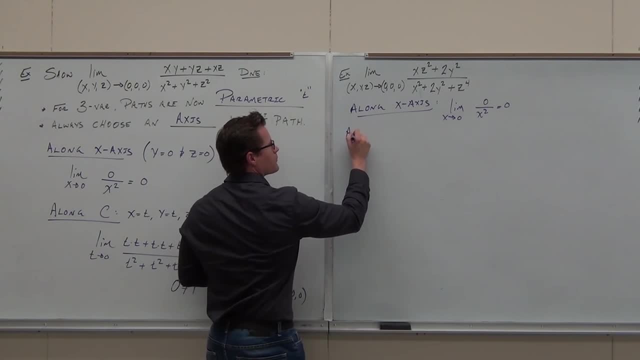 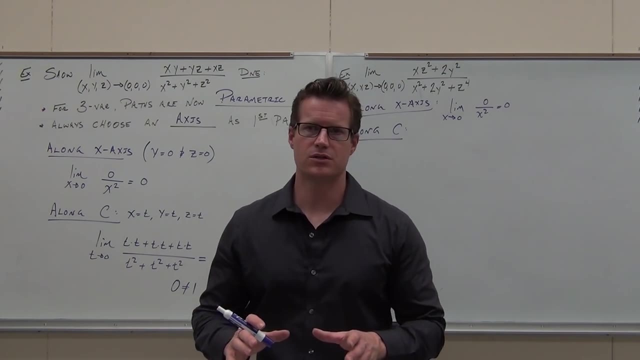 That's nice. You always- pretty much always- do that. What I want to focus on is that your number of x's is the parametric curve that I want to create. This is a little harder because you don't just do x, y. 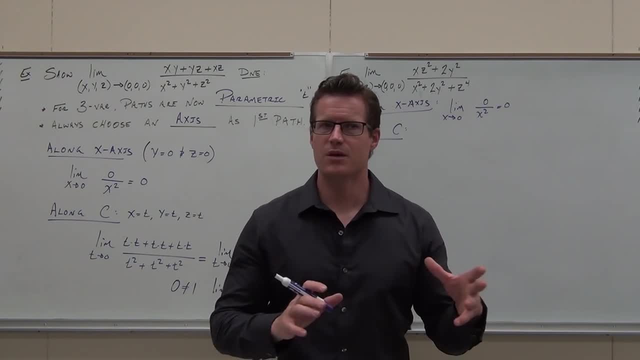 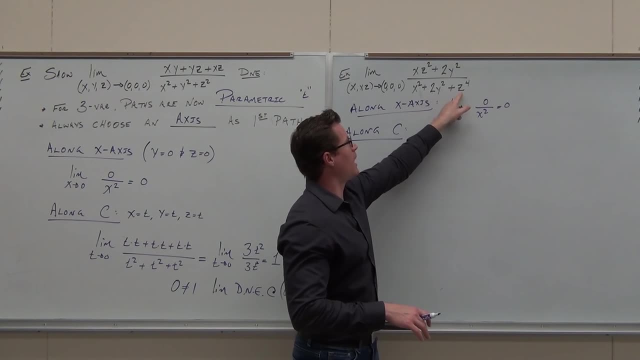 and z all equal to the same parameter, t. What I want you to think about. I'm going to give you about 30 seconds. just think, just think about it. How can I make these powers all the same? How can I make those powers the same? 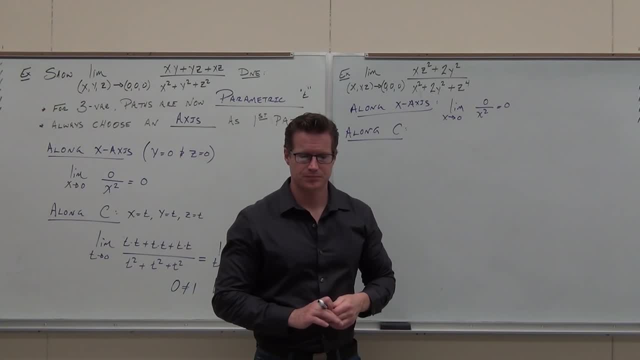 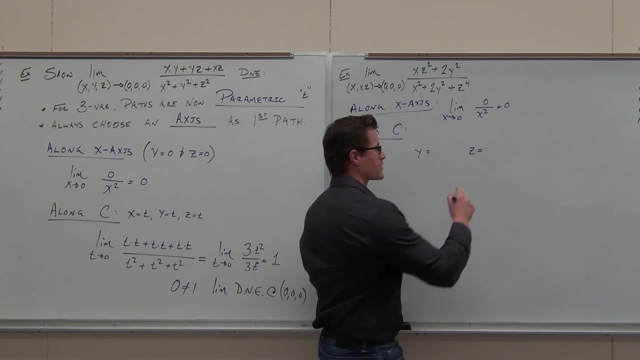 If I can't, how can I do it? So think about it. What's the? what's the variable with the largest power right now? Z, Try this. Try calling the variable with the largest power: t. Let it equal t. 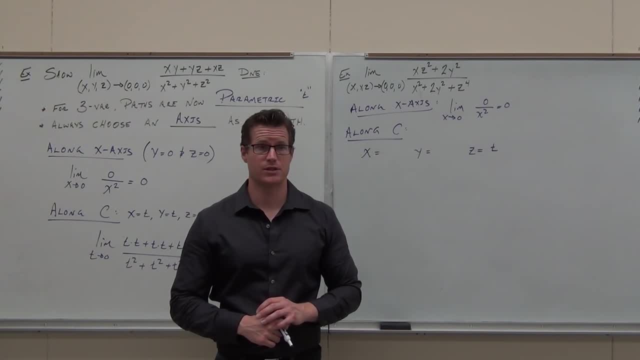 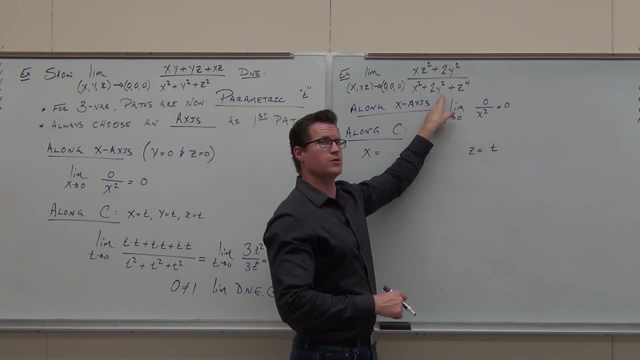 Then try to make the other ones match up. So, for instance, if z equals t, I would give t to the fourth. Does that make sense? I also want this to be t to the fourth. What would y have to equal in order to get t to the fourth? 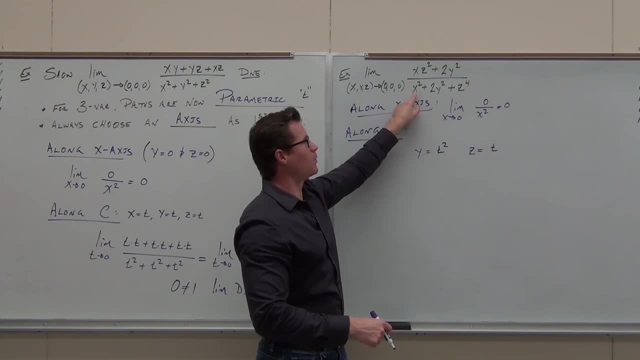 I also want this to be bless you: t to the fourth. What would x have to be to get t to the fourth? That would do it. That would do it. If we do that, the limit changes to t equals zero for sure. 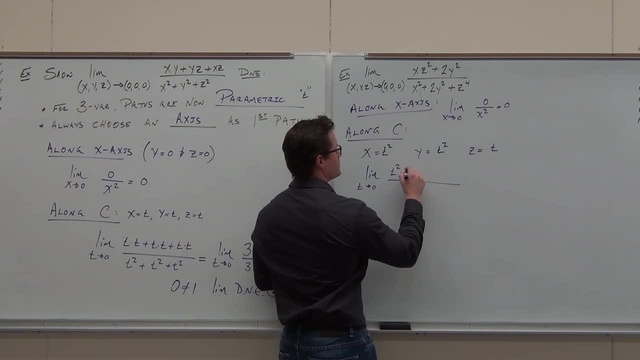 And we got t squared times. notice that Here's x, Here's y, Here's x is t squared, Z is t. So t squared plus 2 times. oh, hey, t squared squared, because that's y squared. Then we have t squared squared, t squared squared. 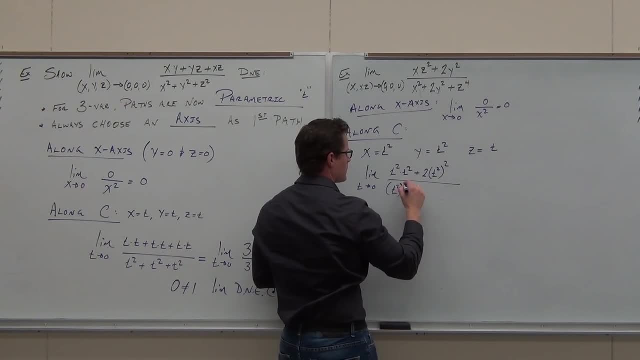 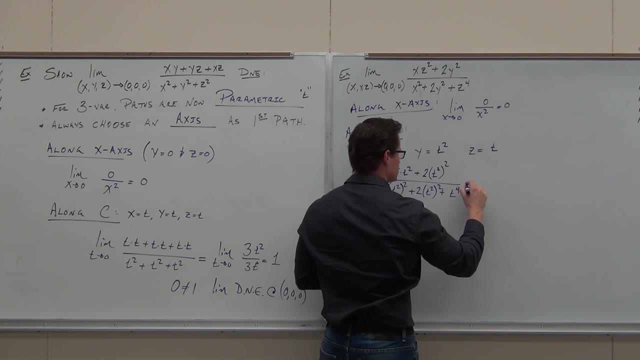 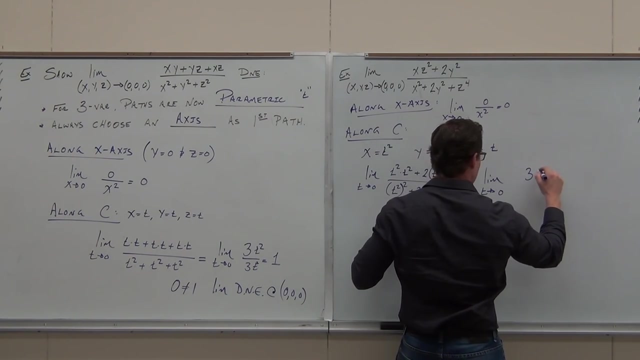 and t to the fourth. I guess I am doing the whole thing. I always do that. I should never say stuff like this. Can you double check my work? I did a lot of it in my day, That's all right. Triple check. 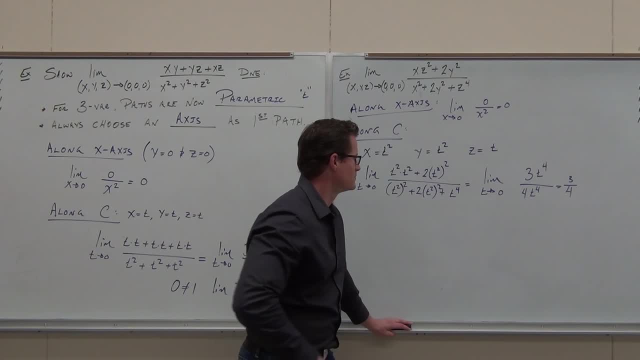 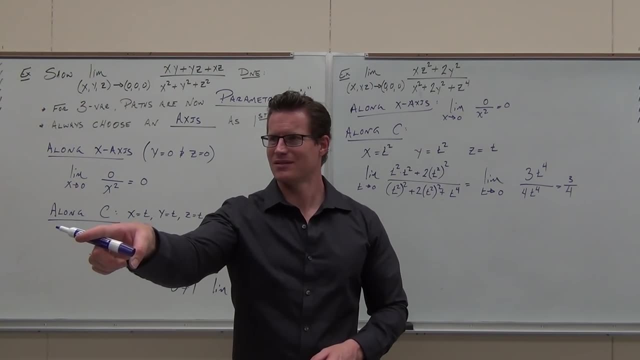 That's all right. Do the same person, That's all right, Doesn't count. when you do it twice, Did you get the same thing? Yeah, Does it prove anything? Yes, Zero, three-fourths, not the same Limit doesn't exist. done. 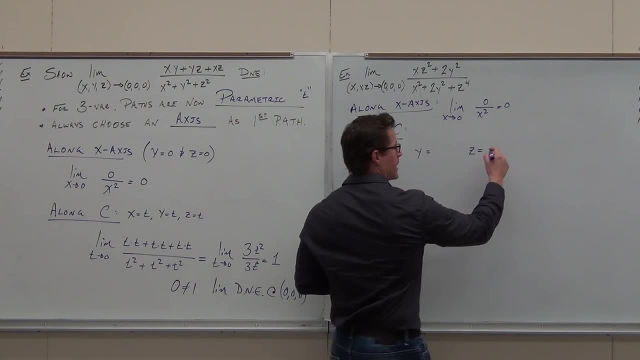 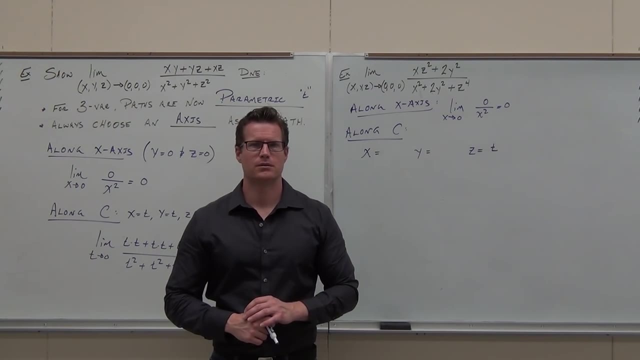 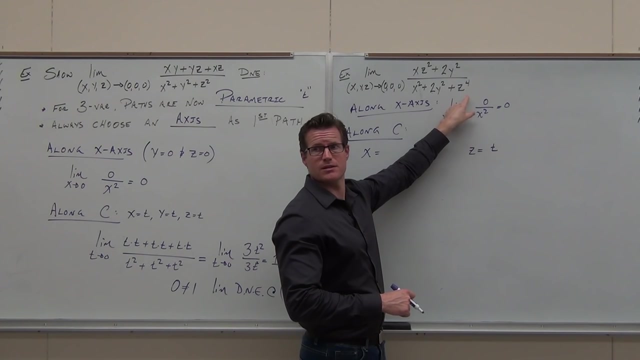 Z. Try this. Try calling the variable with the largest power, T. Let it equal T. Then try to make the other ones match up. So, for instance, if Z equals T, I would get T to the fourth. Does that make sense? 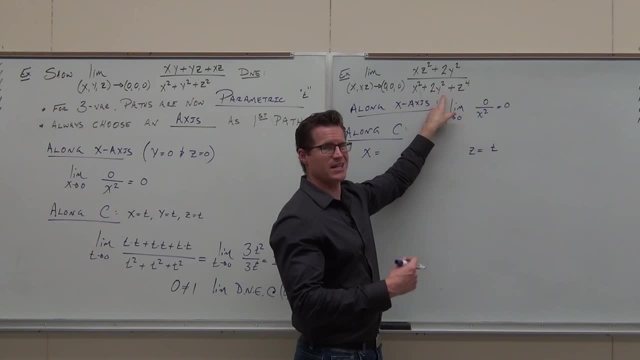 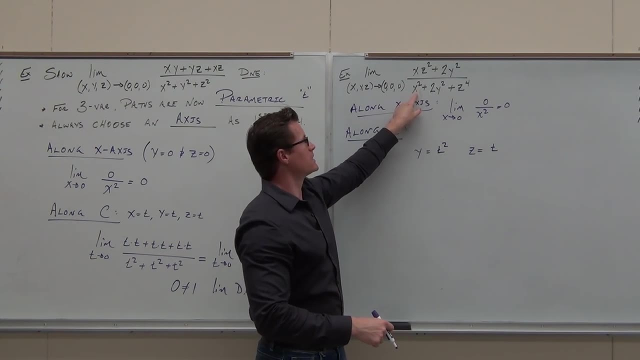 I also want this to be T to the fourth. What would Y have to equal in order to get T to the fourth? I also want this to be bless you. T to the fourth. What would X have to be to get T to the fourth? 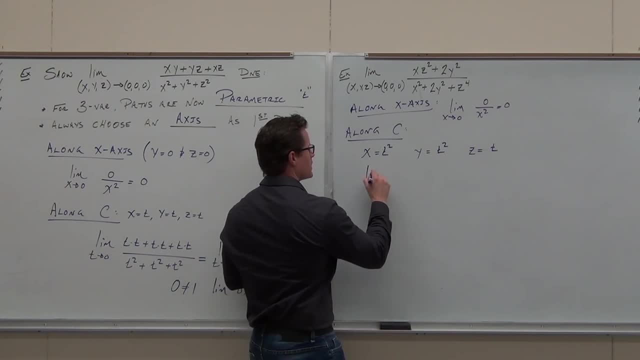 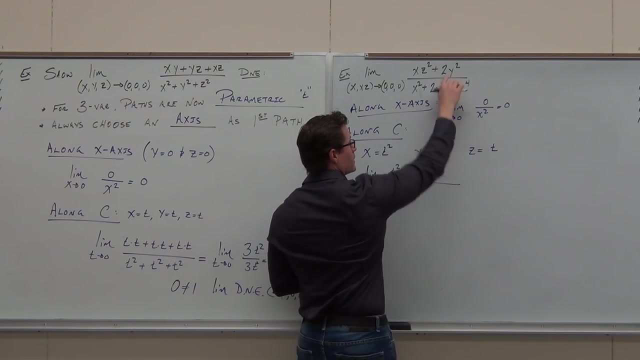 That would do it. That would do it. If we do that, the limit changes to T equals zero, for sure. And we got T squared times. notice that Here's: X is T squared, Z is T, So T squared plus two times. oh hey. 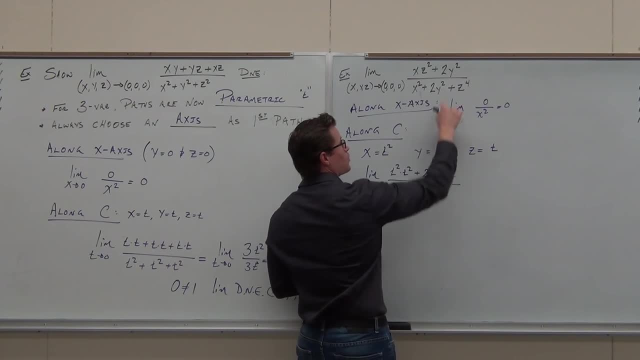 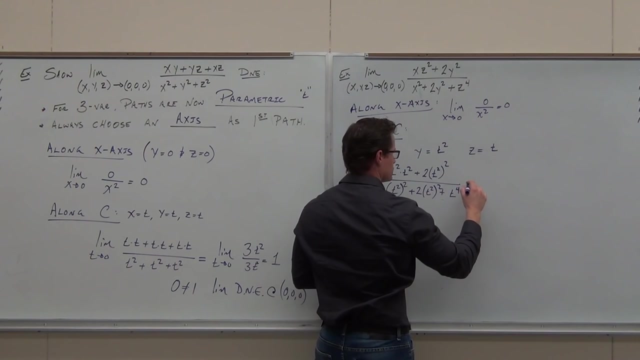 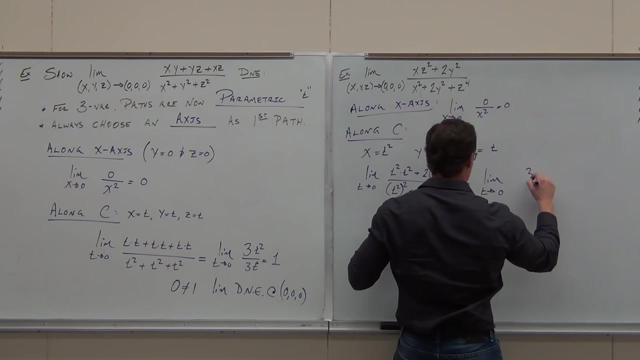 T squared Square, because that's Y squared. Then we have T squared squared, T squared squared and T to the fourth. I guess I am doing the whole thing. I always do that. I should never say stuff like this. Can you double check my work? 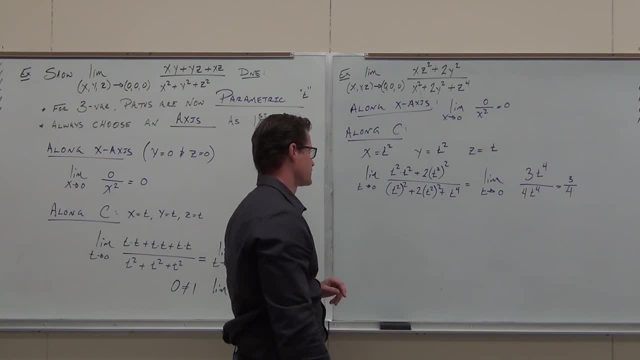 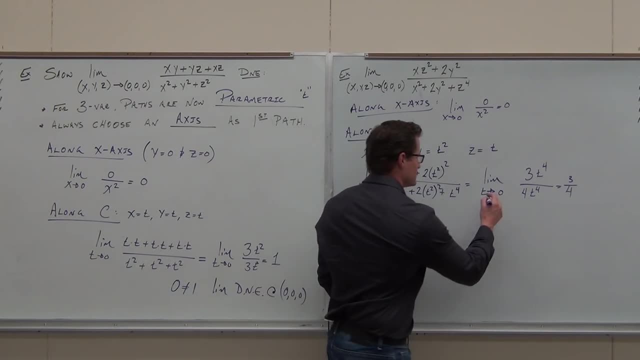 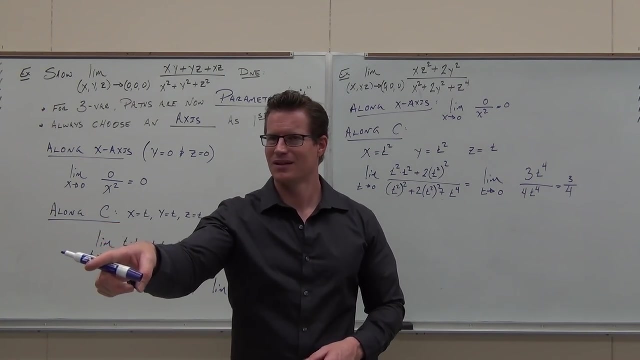 I did a lot of it in the day. That's right. Triple check: That's right. You're the same person. That's right. It doesn't count when you do it twice. Did you get the same thing? Yeah, Does it prove anything? 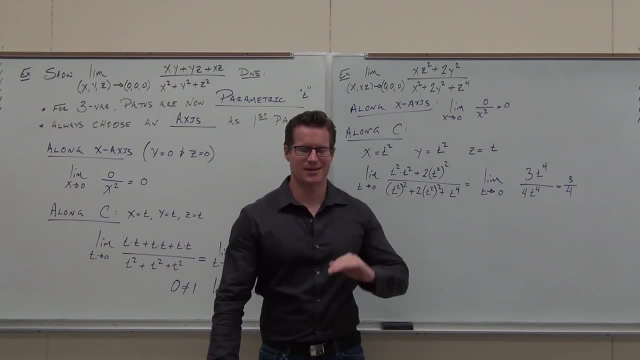 Yes, Zero, Three-fourths, Not the same Limit does exist, Done. So if answer is okay, with this one, Now we practice. Now we practice evaluating Limits. I need you to know that evaluating limits is exactly the same here as it is for Calc 1.. 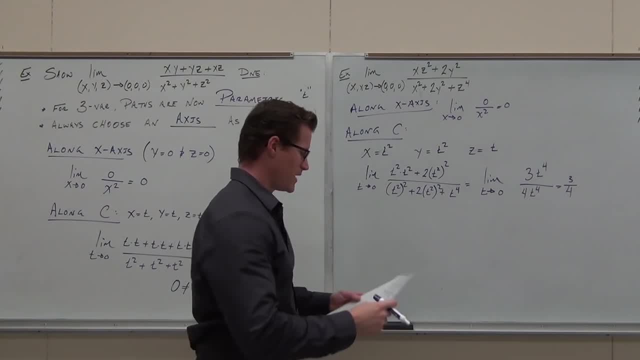 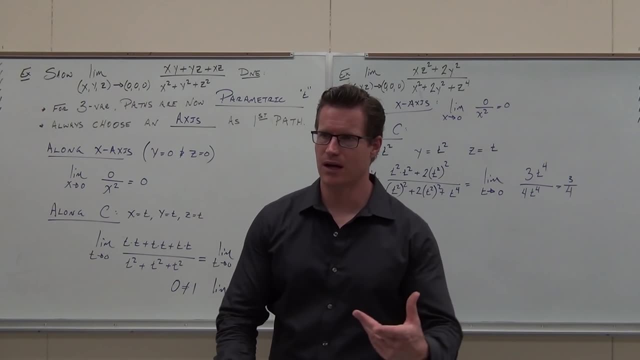 So we're okay with this one. Now we practice. Now we practice evaluating limits. I need you to know that evaluating limits is exactly the same here as it is for Calc 1, and I'm going to cheat. I told you I'm going to use some circular reasoning. 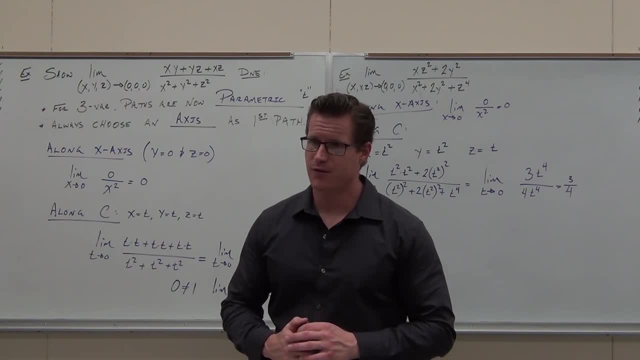 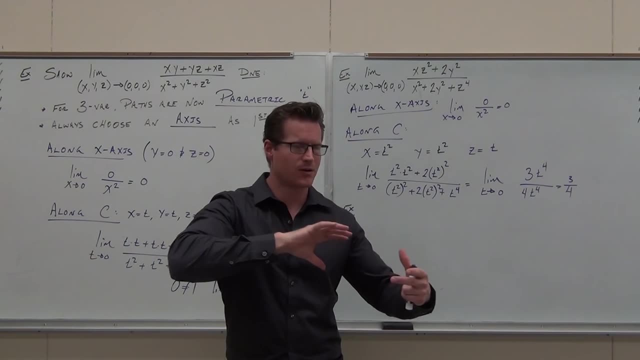 What I'm going to do is show you how to evaluate based on the fact that we have continuity. Then I'm going to talk about continuity and use that to kind of fill in the fact that we have continuity, The fact that we're able to do this. okay, 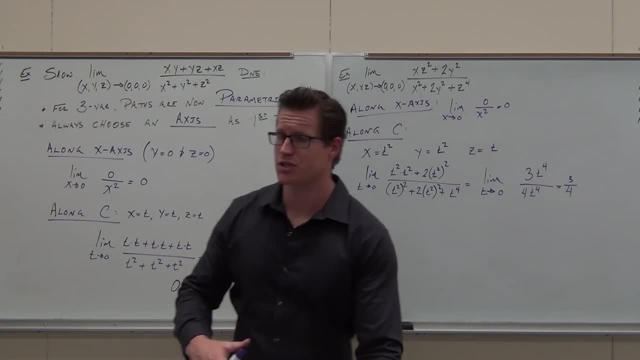 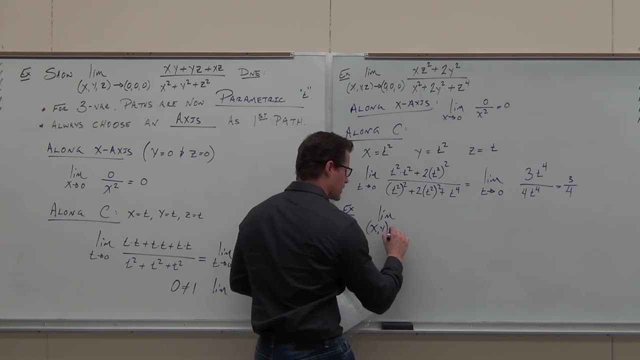 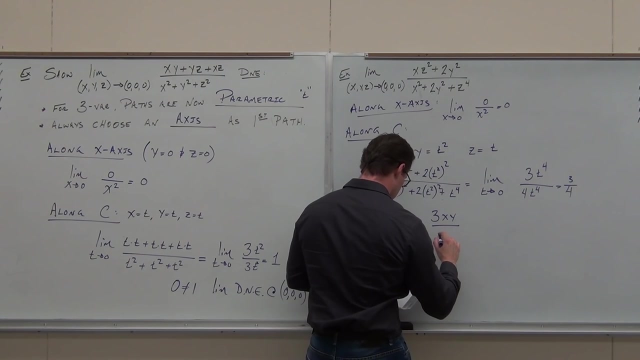 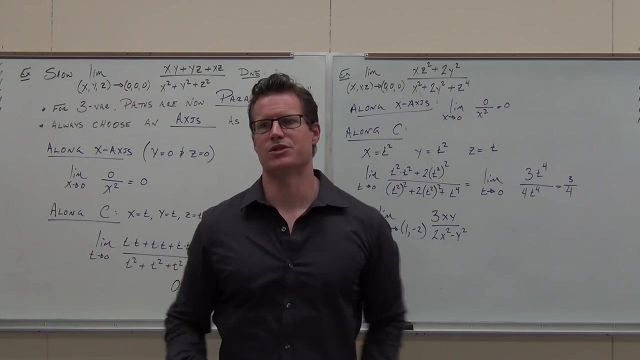 So here's the how. I'll talk about the why in just a little while. So the how. Whenever we're evaluating limits, I don't care what class you're in through calculus, The first thing I want you to do is plug the numbers in. 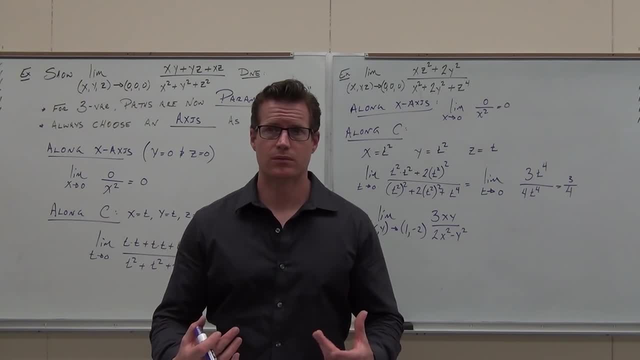 Just plug them in. If you don't get zero over zero or you don't get zero over zero- zero on a denominator- you're done, Plug them in. And we're using the fact that if you plug in a value and you get a number, a limit, then that function exists. 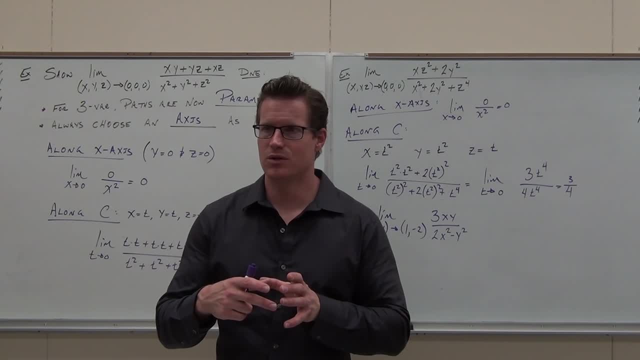 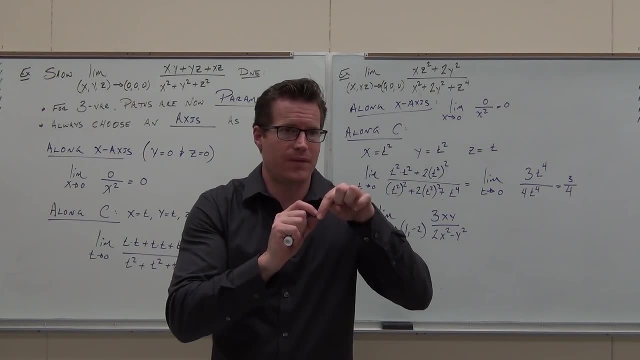 at that point and in a neighborhood around it, you can find continuity And in a neighborhood around it, it means all the paths lead to that same value. That's what we're using here. We'll talk about how that, how we're. 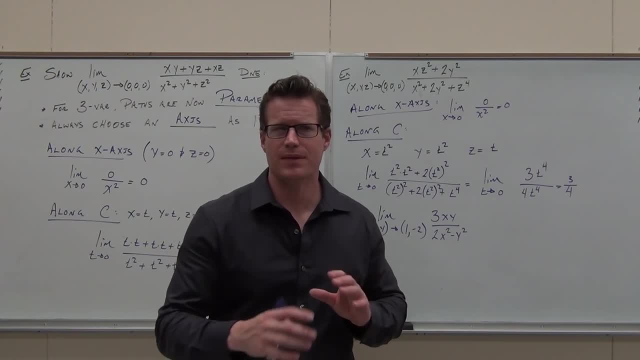 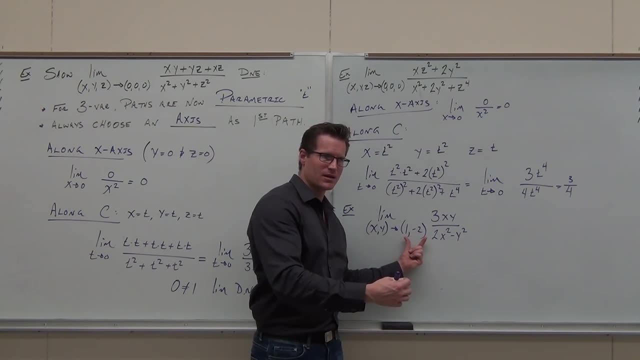 if we have a domain that's defined, we're continuous on that domain. we'll talk about that in a minute. but that's basically what we're doing, What we're using. we're saying, if this function exists, if it's defined, at that point you're going to be continuous. 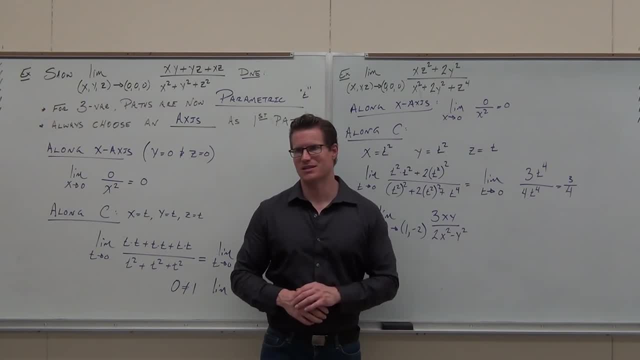 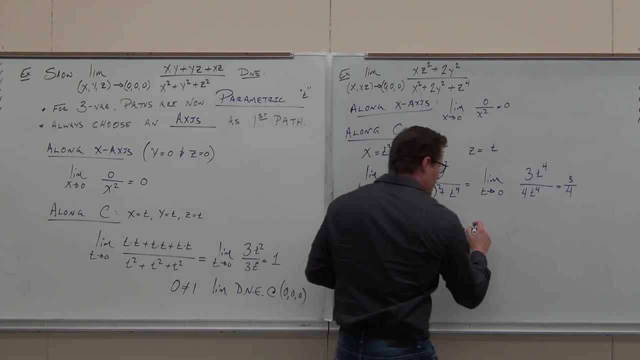 at that point, which means that the limit has to exist, Because if we're defined, the limit exists. sorry, if we're defined and continuous, the limit has to exist. Therefore, plug in a number: the limit has to equal the value of the function. 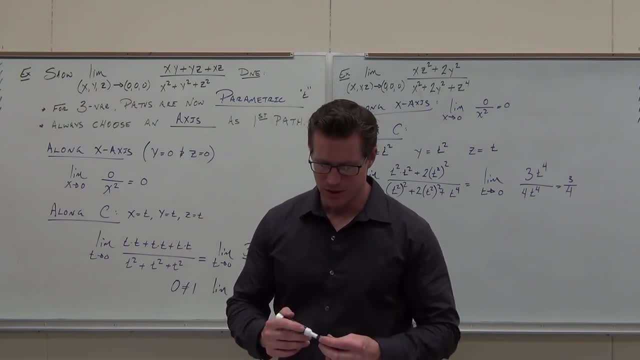 And I'm going to cheat. I told you I'm going to use some circular reasoning. What I'm going to do is show you how to evaluate based on the fact that we have continuity. Then I'm going to talk about continuity and use that to kind of fill in the fact that we're able to do this. 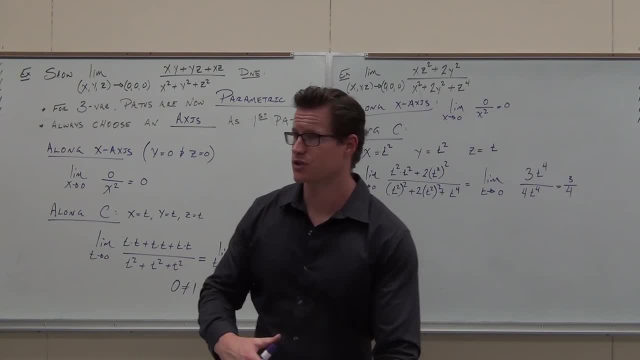 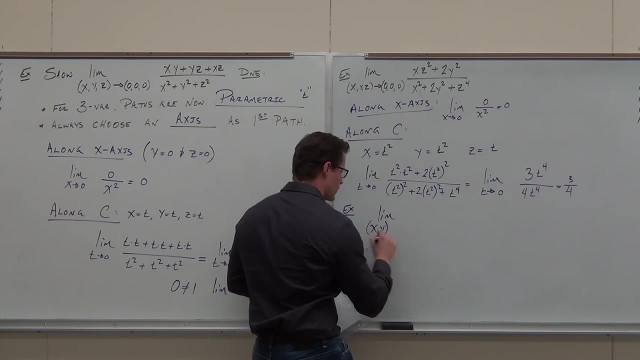 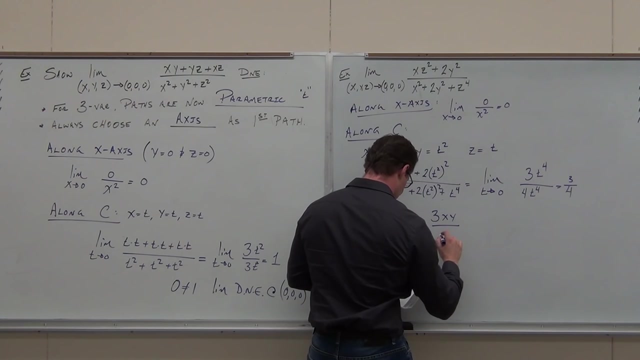 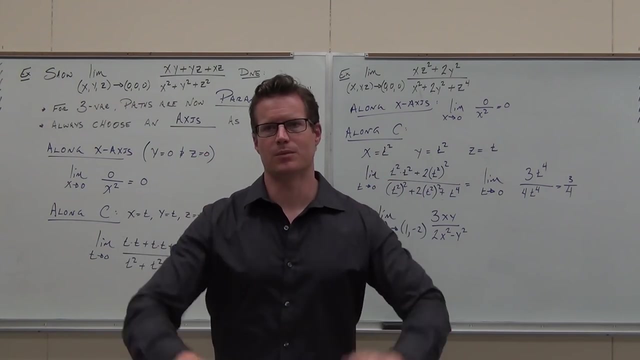 Okay, So here's the how. I'll talk about the why in a little while. So the how. Whenever we're evaluating limits, I don't care what class you're in through calculus- The first thing I want you to do is plug the numbers in. 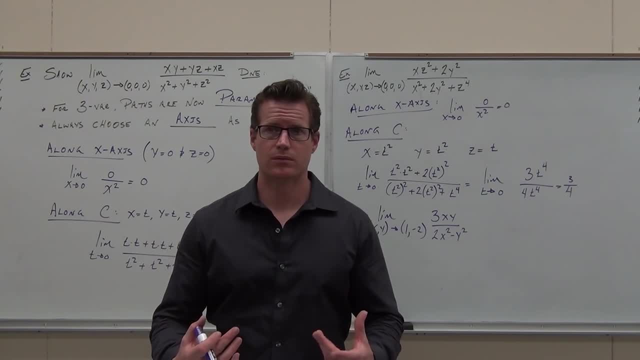 Just plug them in. If you don't get zero over zero or zero on a denominator, you're done, Plug them in And we're using the fact that if you plug in a value and you get a number, If you limit, Then that function exists at that point. 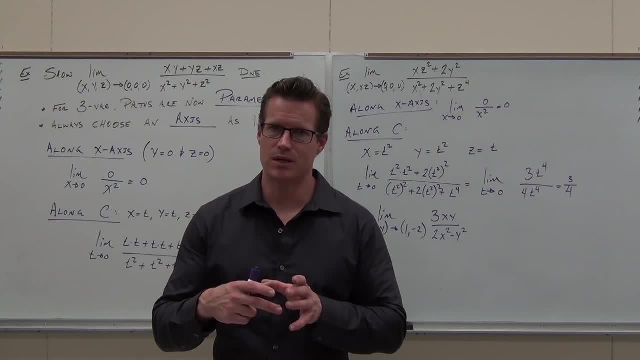 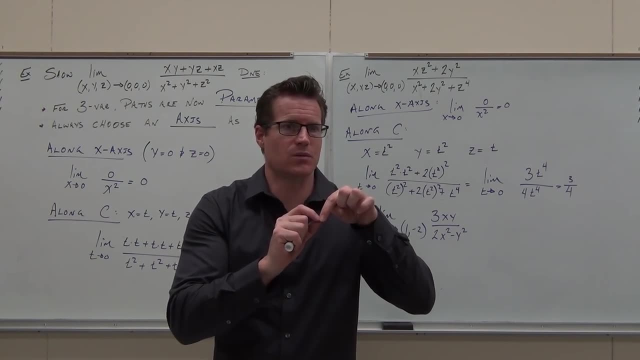 And in a neighborhood around it you can find continuity, And in a neighborhood around it it means all the paths lead to that same value. That's what we're using here. We'll talk about how we're. If we have a domain that's defined, we're continuous on that domain. 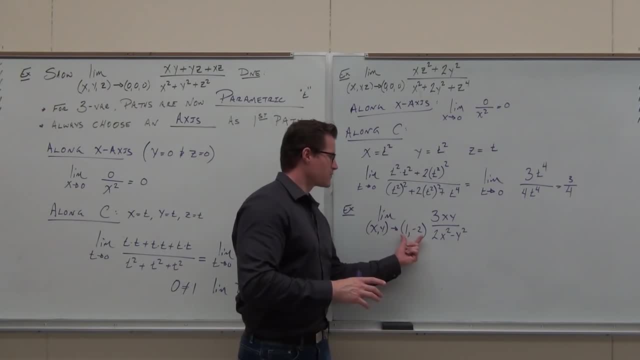 We'll talk about that in a minute, But that's basically what we're using. We're saying, if this function exists, if it's defined at that point, you're going to be continuous at that point, which means that the limit has to exist. 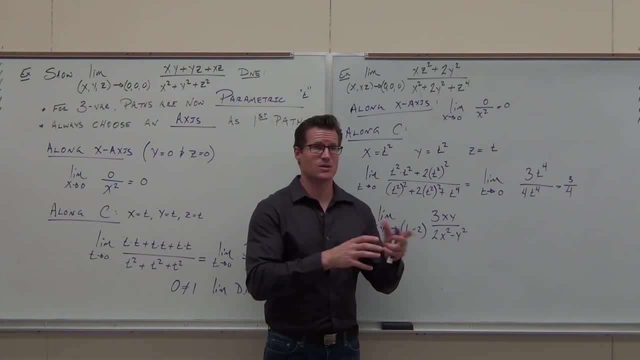 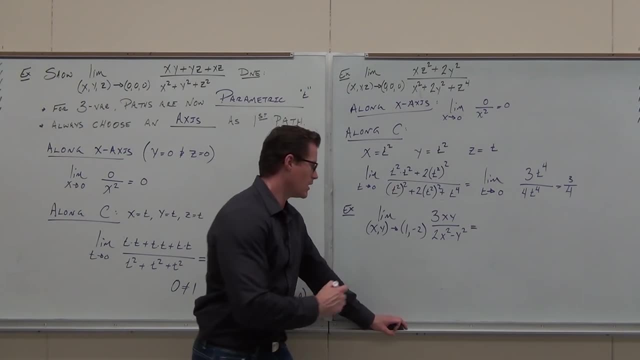 because if we're defined, the limit exists. Sorry, if we're defined and continuous, the limit has to exist. Therefore, plug in the number. the limit has to equal the value of the function. We're kind of cheating here. The idea from Calc 1 would be: if the point exists, 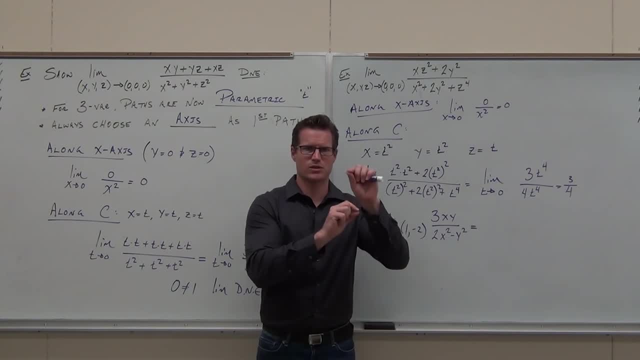 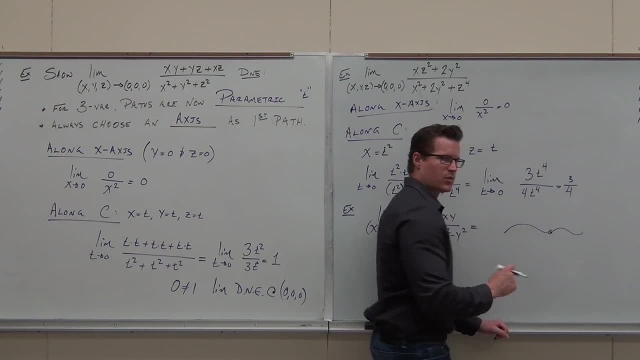 and the limit exists, and limit equals the point. you have continuity. If you have this, the limit exists, the point exists and the points in that little spot that creates continuity. So if we have continuity, ie it's defined. 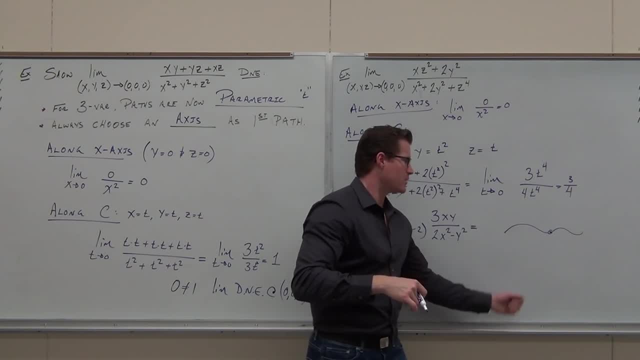 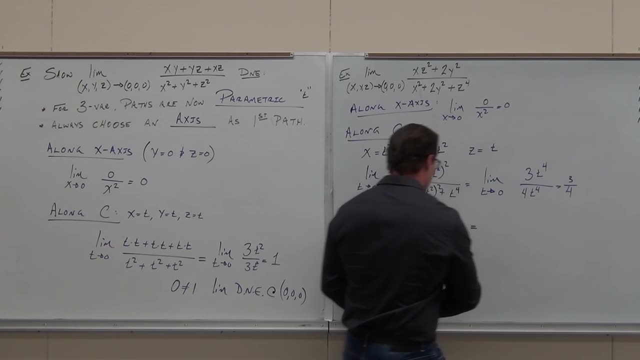 If it's defined, we have continuity. If we have that, then we can go backwards and say: if we have continuity, then the limit exists, And that's what I meant about. we're going backwards here, So let's try it. 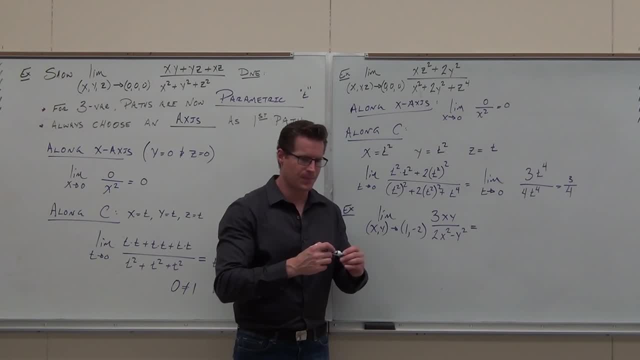 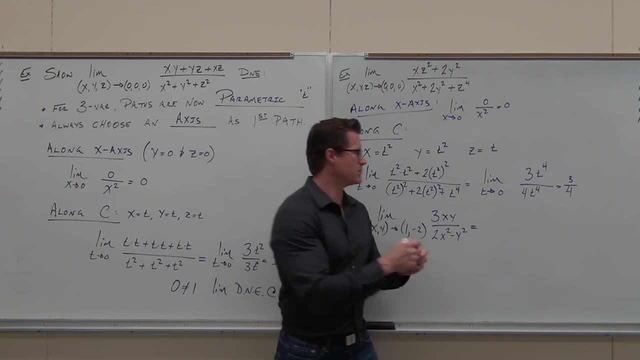 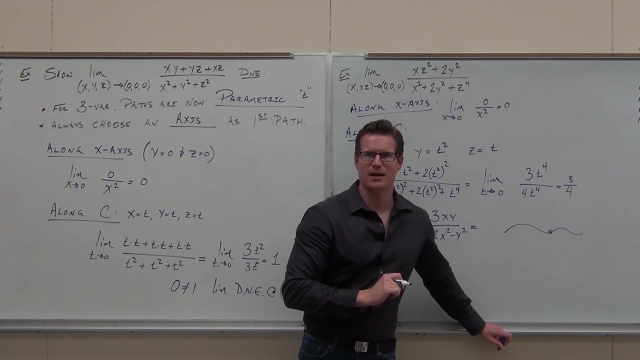 We're kind of cheating here. The idea from Calc 1 would be: if the point exists and the limit exists- and limit equals the point- you have continuity. If you have this, the limit exists, the point exists and the point's in that little spot. that creates continuity. 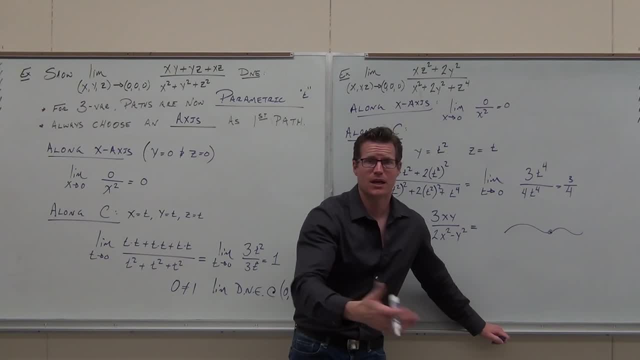 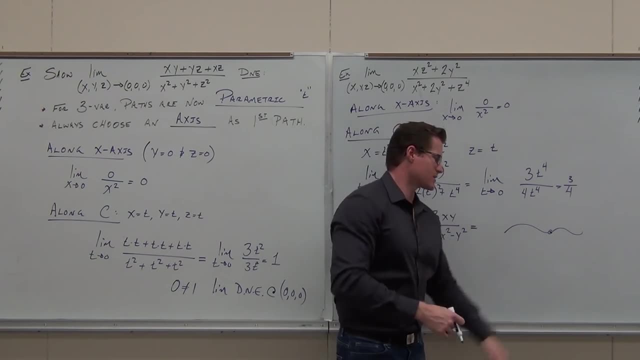 So if we have continuity- ie it's defined- if it's defined, we have continuity. If we have that, then we can go backwards and say: if we have continuity, then the limit exists. And that's what I meant about. we're going backwards here. 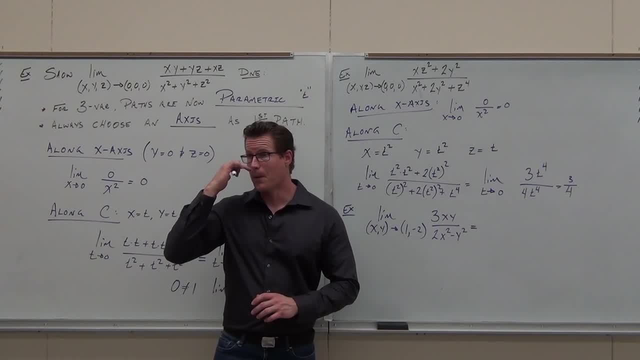 So let's try it. Can you plug in your x and your y value? What is your x value? What's your y value? Have you already plugged this in? How much do you get? Three, Three, Okay, I agree. 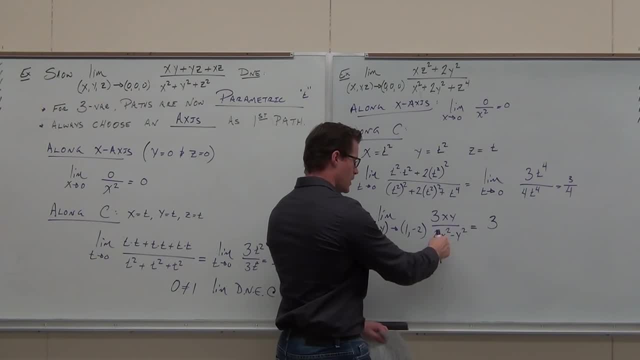 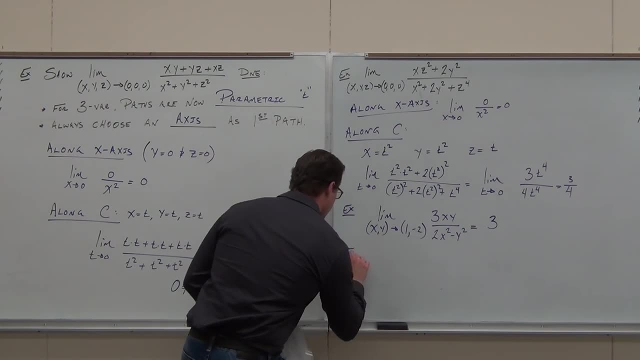 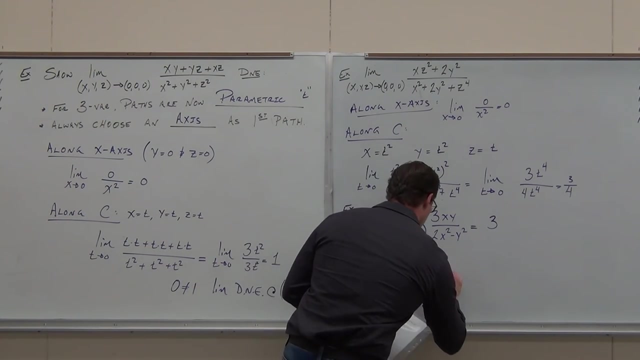 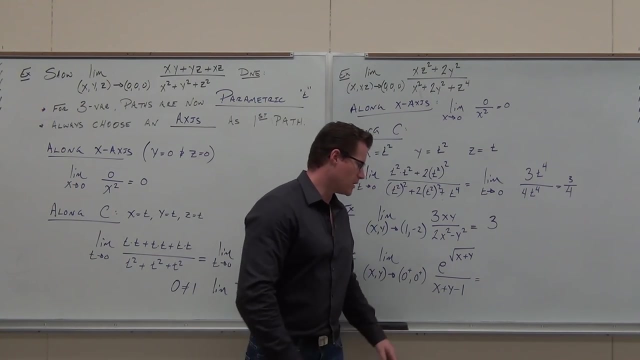 Why Well? 1, negative 2, okay, perfect. 1, negative 2,, plug in, you get 3.. Simplify: you get 3.. Are you guys okay with that one? All right, We also learned this from Calc. 1, right-sided and left-sided are super fine, as long. 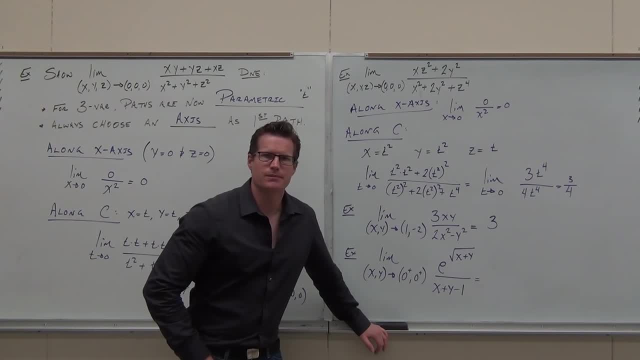 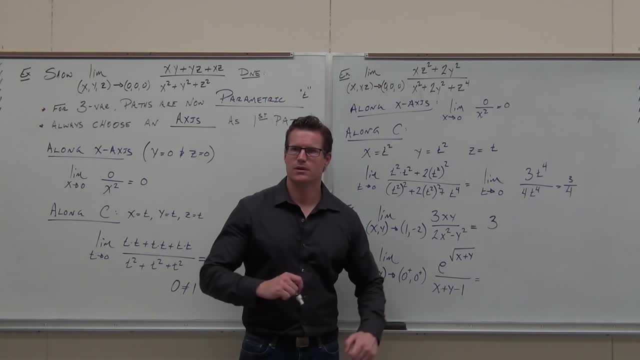 0. 0. 0. It's negative folks. Now, just this part, just that. What do you get here? So something close to 0 from the right, positive. Something close to 0 from the right, also positive. 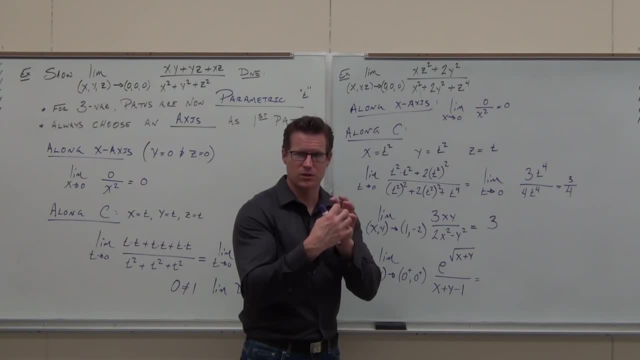 You're going to get something close to 0 from the right 0.. So you're going to get 0, really close to 0, but positive Reason why it has to be right-sided is you get it under the square root. 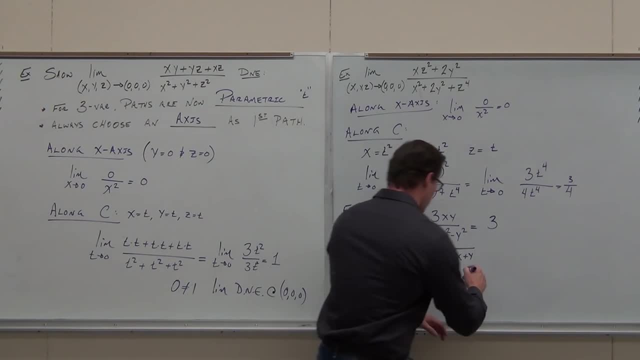 you can't get it from the other side, okay, So we can't have it. that's the only reason why it's there. So this is e to the 0 over negative 1.. How much do we get for that 0.? 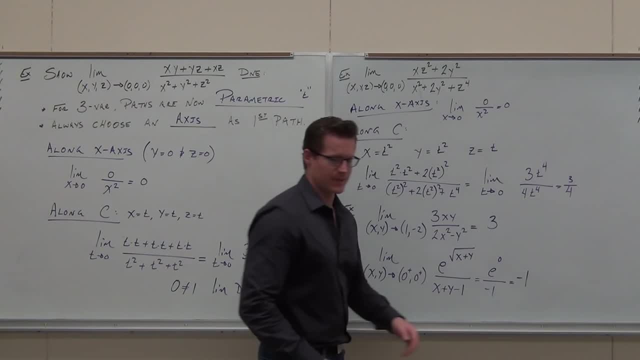 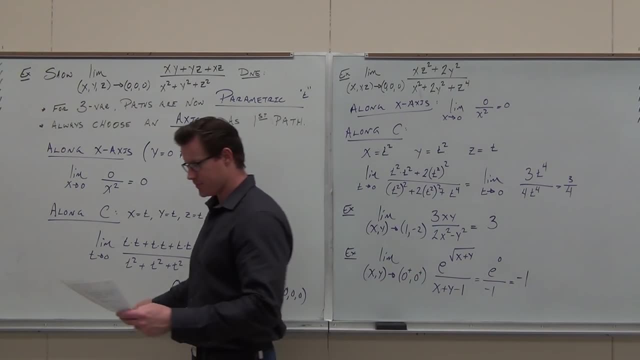 that's it. that's it. that's evaluating limits head down. if you're okay with with that one, we can make them nastier, but the idea is the same. so let's try. i'm going to give you one that's kind of nasty and and then i'll give you another one i want you to think about. 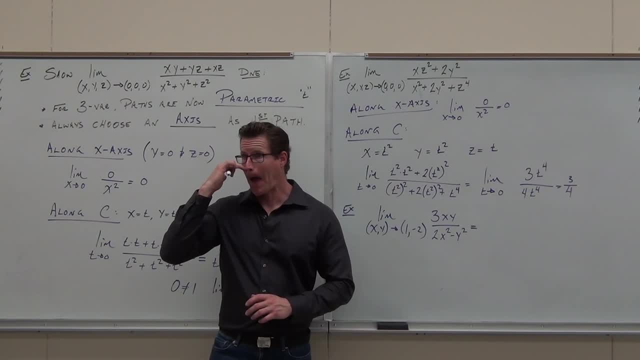 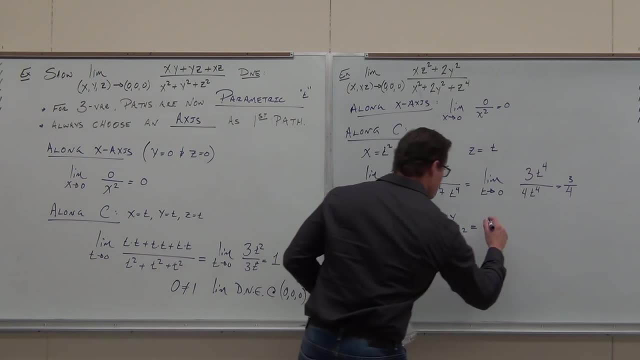 Can you plug in your x and your y value? What is your x value? What's your y value? Have you already plugged this in? How much do you get? Three, Okay, three Y, well, 1, negative, 2, okay, perfect. 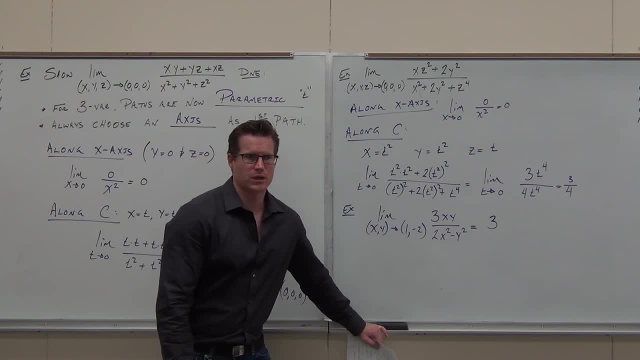 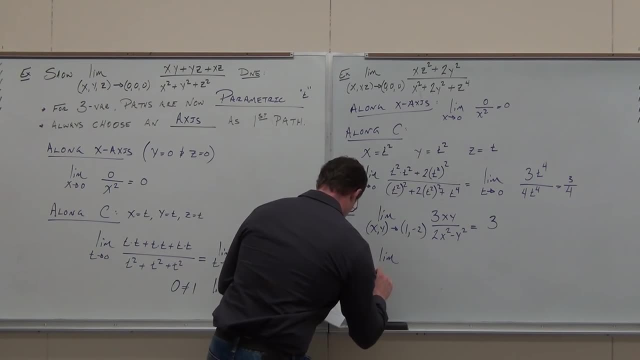 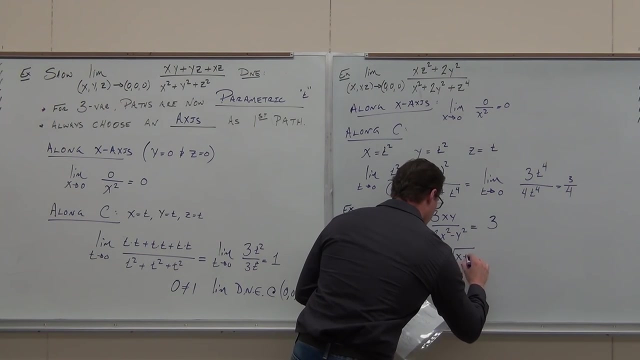 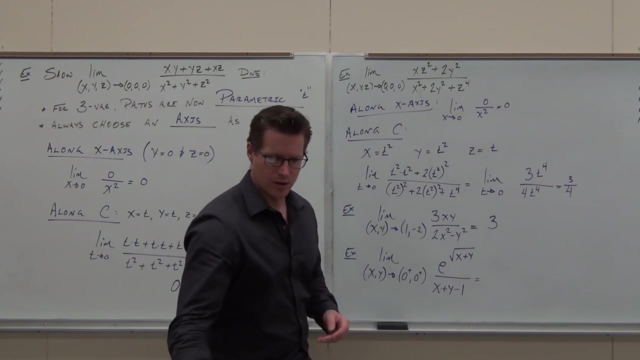 1, negative 2, plug in: you get 3.. Simplify, you get 3.. Are you guys okay with that one? All right, Boy, there's a weird one. We also learned this from Calc 1, right side and left side are super fine, as long. 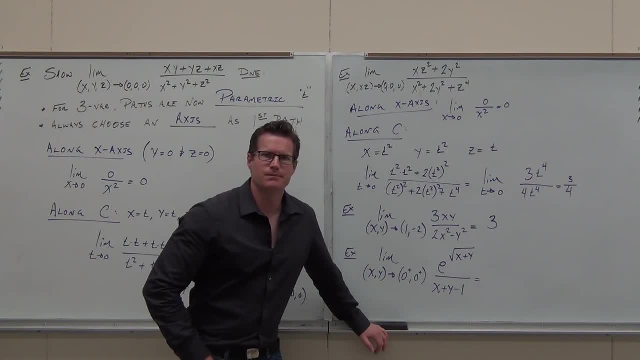 as you have continuous functions. So honestly, plug the numbers in and see if they work. So just plug in 0 and 0. Let's see if we can do that. Can you plug in 0 and 0? What do you get? 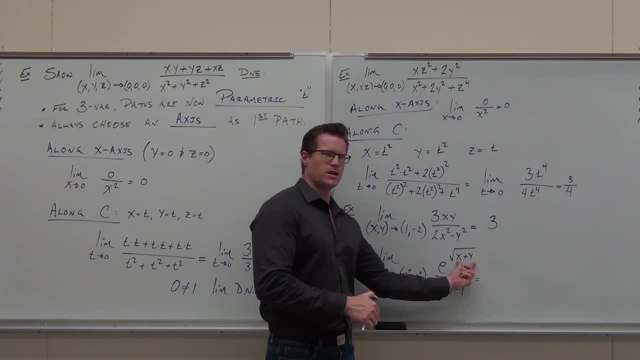 Come here folks. Just this part, just that. What do you get here? No, Okay, So something close to 0 from the right- positive. Something close to 0 from the right, also positive. You're going to get something close to 0 from the right- 0.. 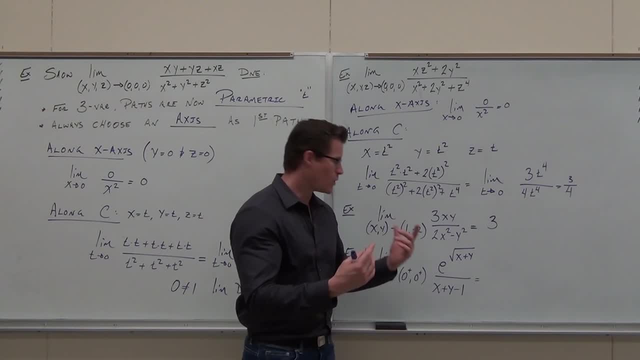 So you're going to get 0, really close to 0, but positive. Reason why it has to be right-sided is because you have it under a square root. You can't get it from the other side. okay, so you can't have it. 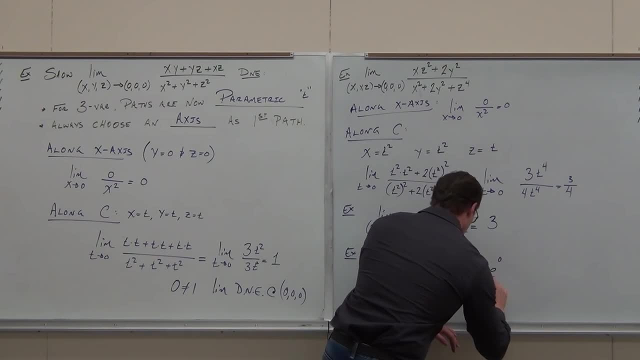 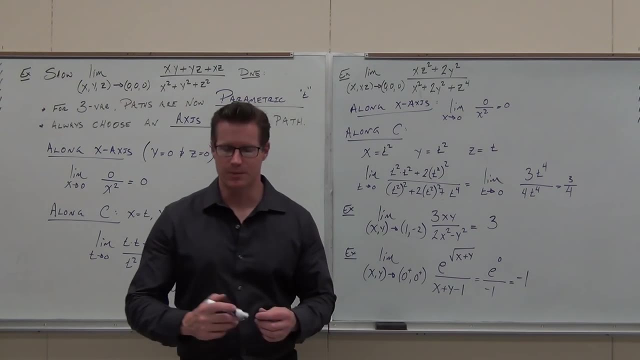 That's the only reason why it's there. So this is e to the 0 over negative 1.. How much do we get for that Negative 1.? That's it. That's it. That's evaluating limits Head down, if you're okay with that one. 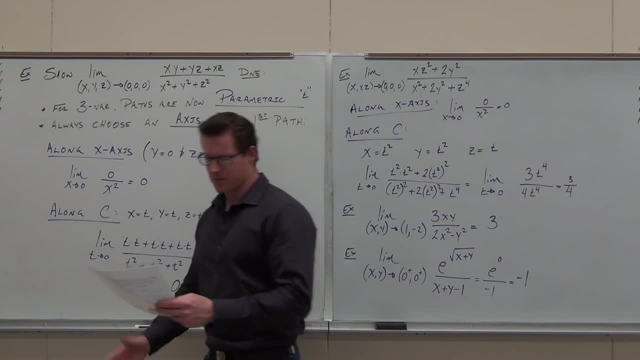 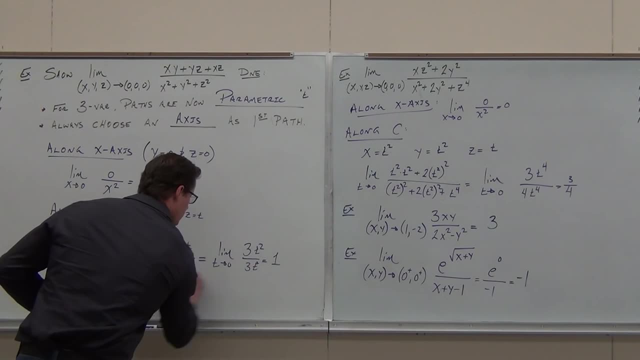 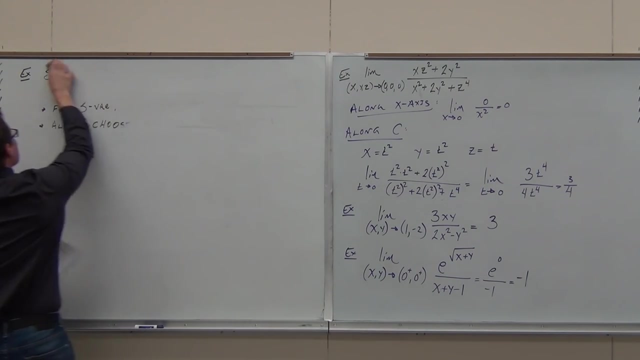 We can make them nastier, but the idea is the same. So let's try. I'm going to give you one that's kind of nasty, and then I'll give you another one I want you to think about. So give it a try. 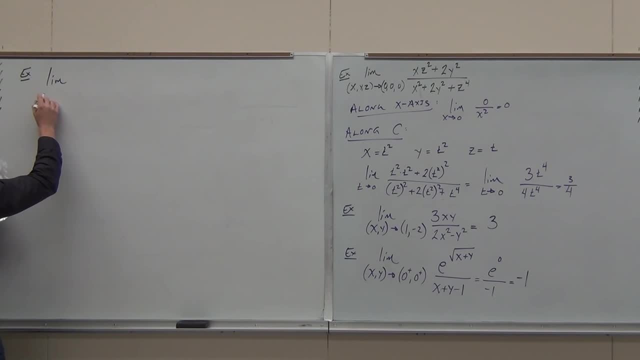 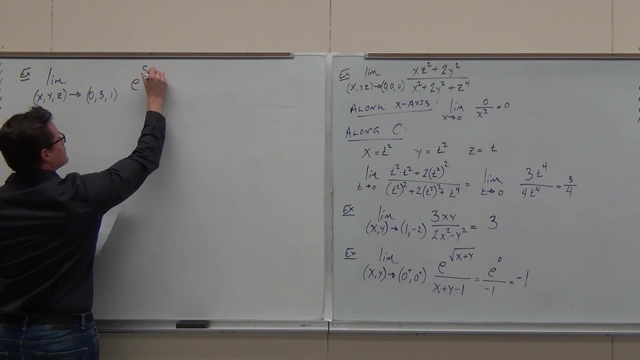 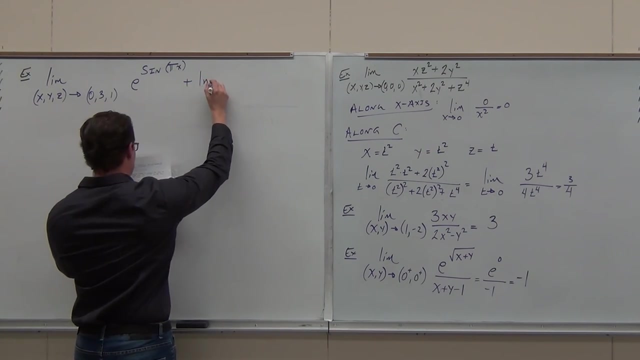 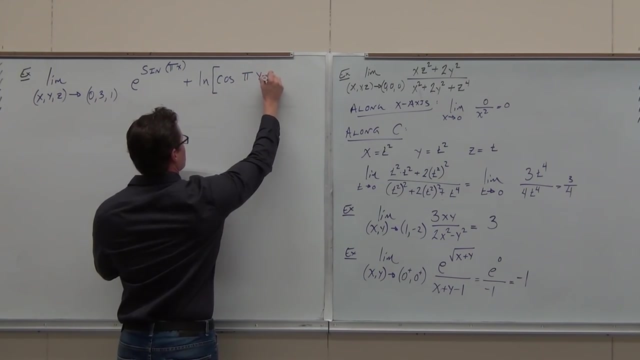 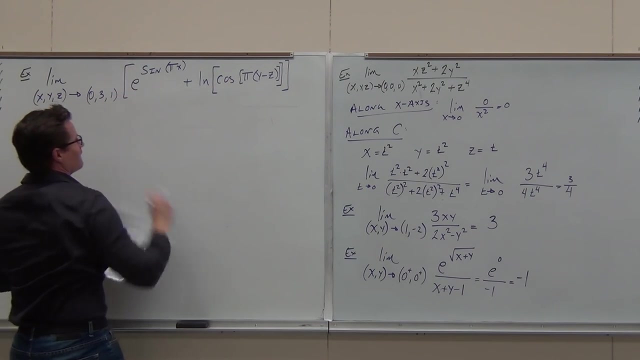 so give it a try. here's x, y, z. i want the limit of the following function as we approach the point zero, three, one, and the function is: oh, don't worry, worry you. yeah, that's what i'm talking about. what's the first thing you do with any limit? like ever. 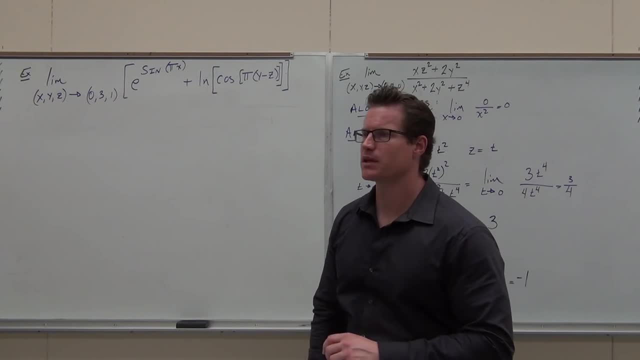 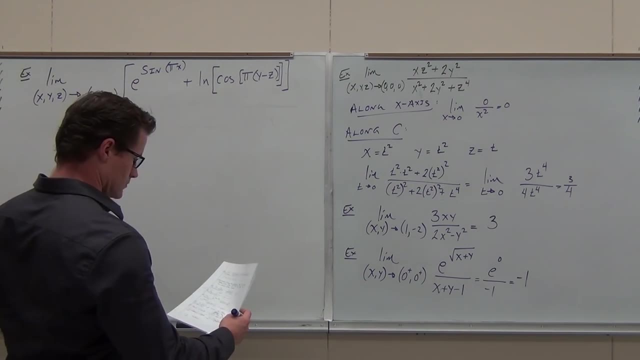 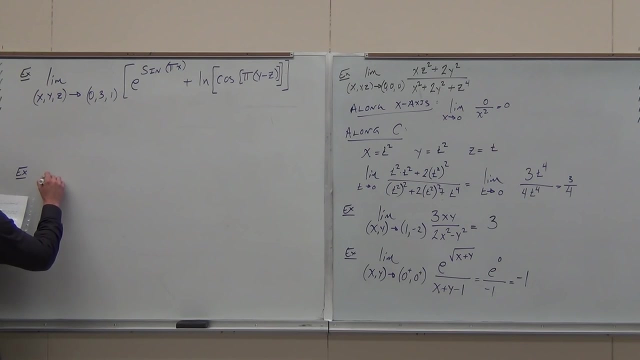 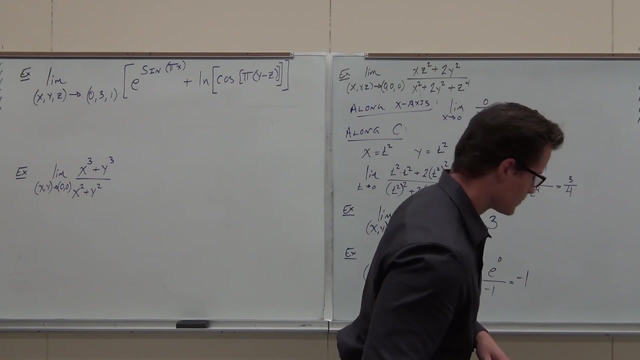 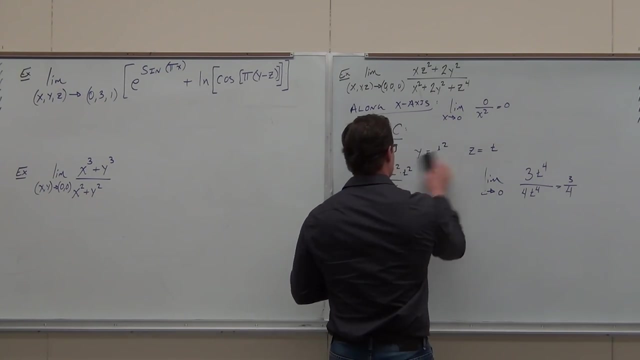 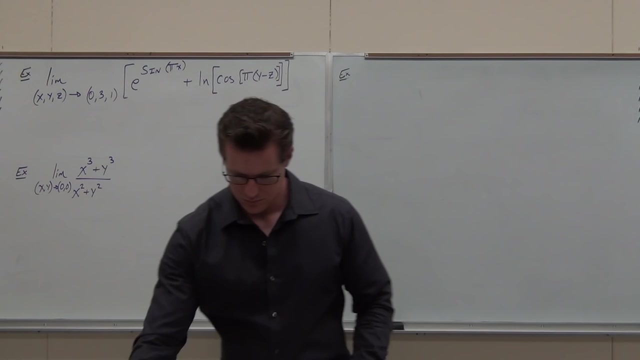 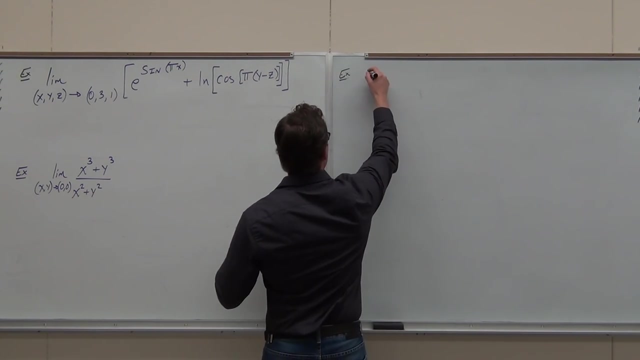 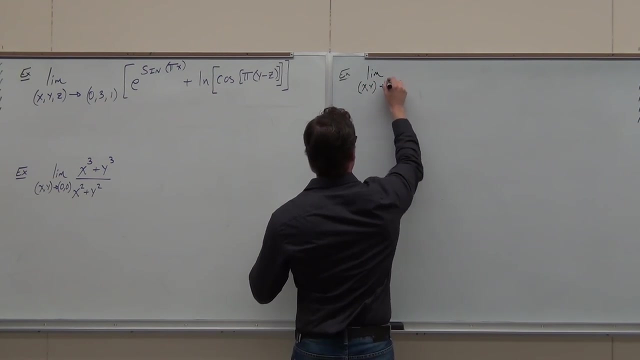 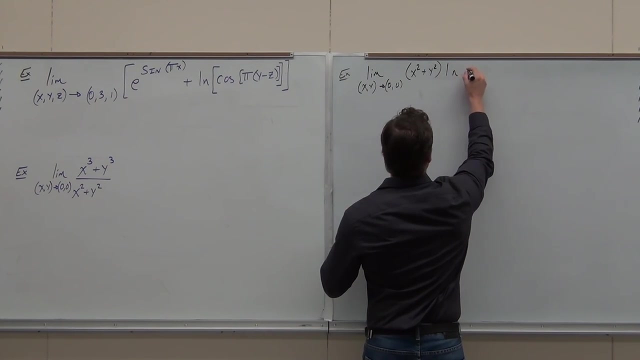 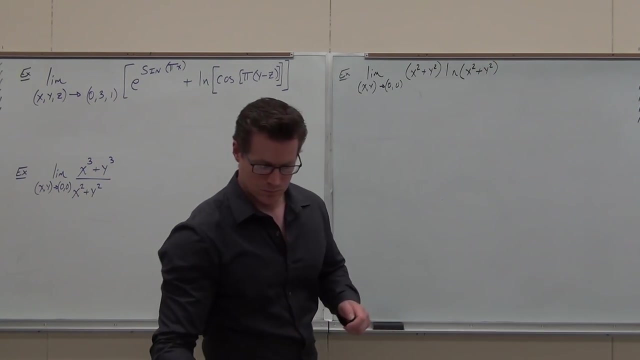 can you just do that. let's plug it. just plug it in, see what happens. hopefully i wrote down right. that would suck. so after you do that one, i want you thinking about the next example, please Thank you. What's the x value, Y value? 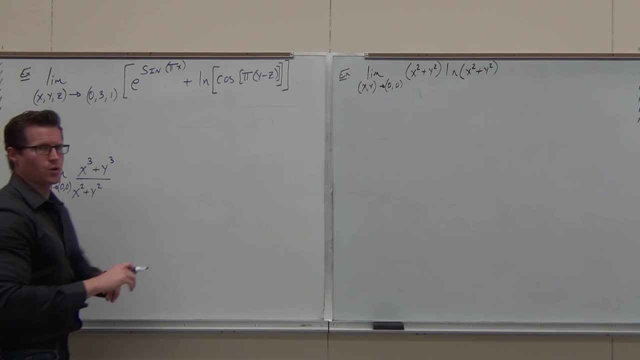 Z value. Instead of trying to do all of this math in your head- probably no good idea- at least write out some pieces of it. So here I'm writing out e to the sine of. I do know that's 0, so I'm going to put the 0. 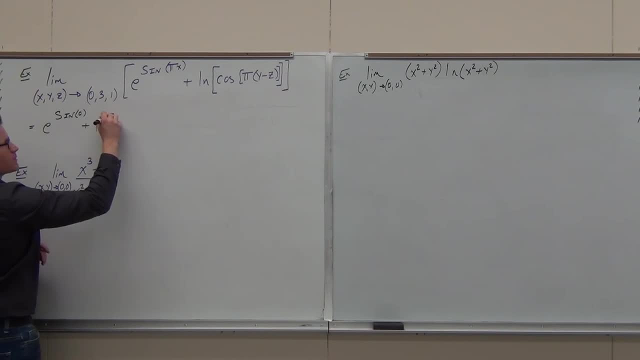 e to the sine of 0. Plus ln. that's got to be there, Cosine that's got to be there, Pi that's got to be there. But I would do things like this: 3 minus 1 is 2.. 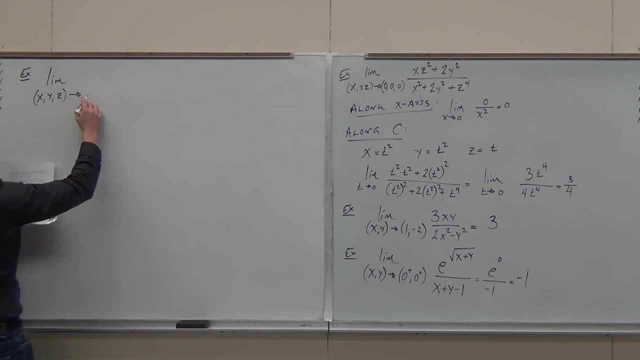 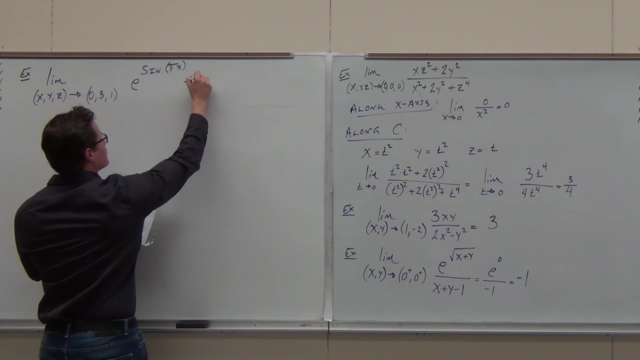 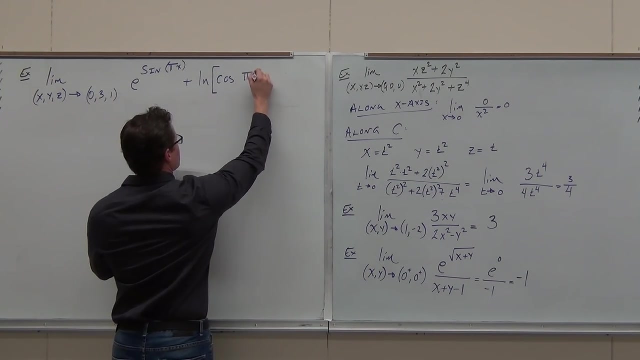 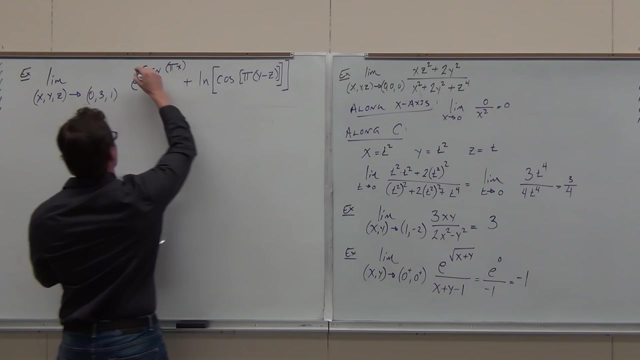 Here's x, y, z. I want the limit of the following function as we approach the point 0,, 3,, 1, and the function is: oh, don't worry, Worry, Worry, Yeah, That's what I'm talking about. 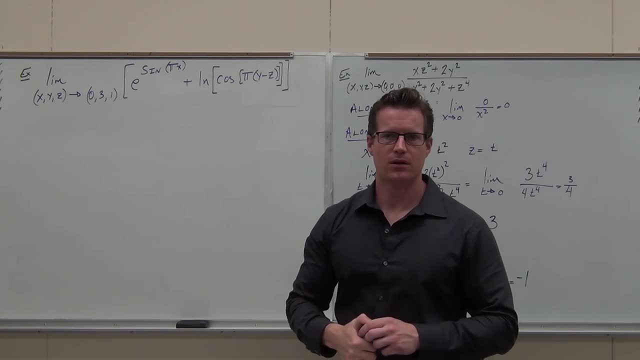 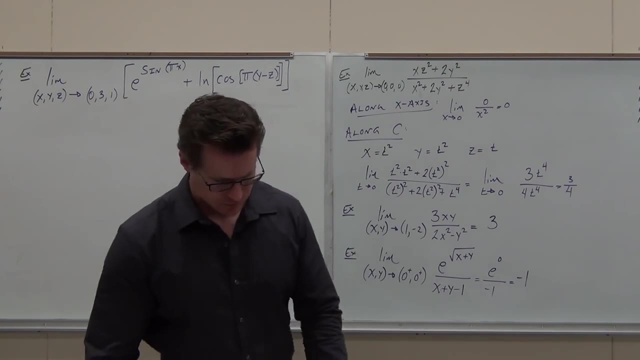 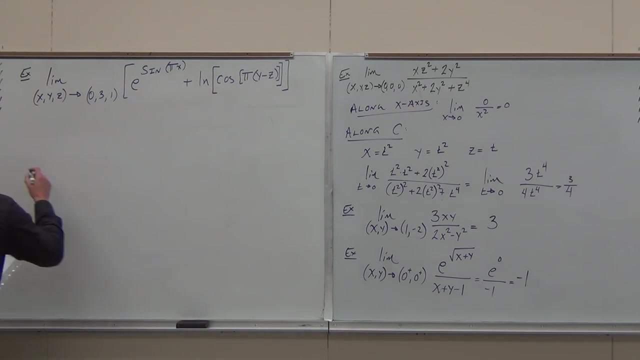 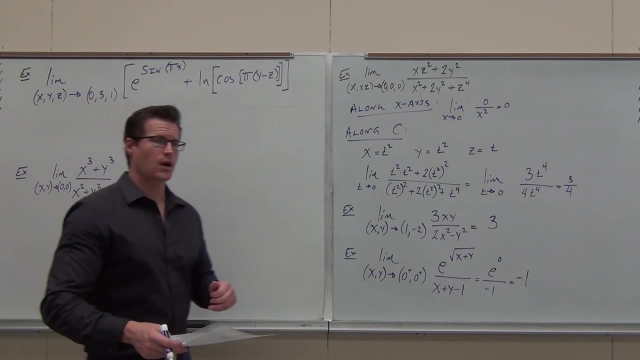 Woo, What's the first thing you do with any limit, like ever, Can you just do that? Let me plug it in. Just plug it in and see what happens. Hopefully I wrote it down right. That would suck. After you do that one, I want you thinking about the next example, please. 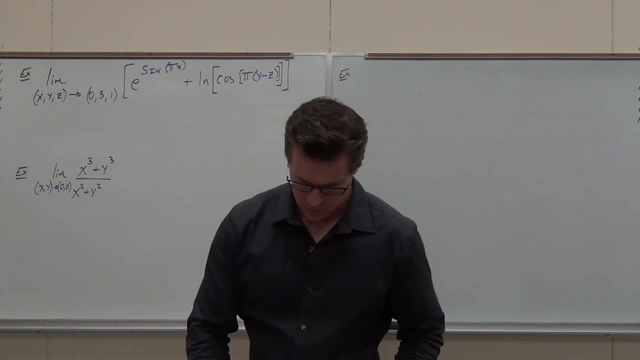 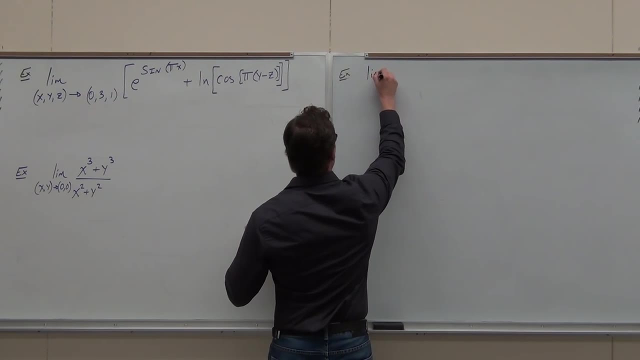 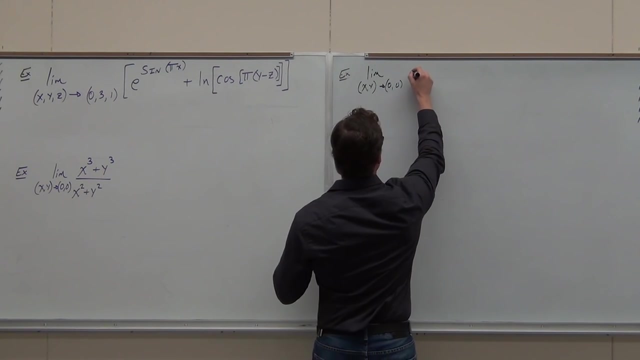 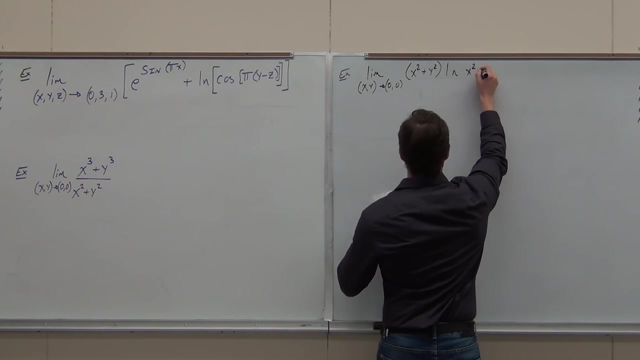 Oh, oh, oh, That's a hard one. How do you do that? I never know, but I'm not sure. Oh, oh, oh, Oh. no, I can't remember, but I'll give you a second. 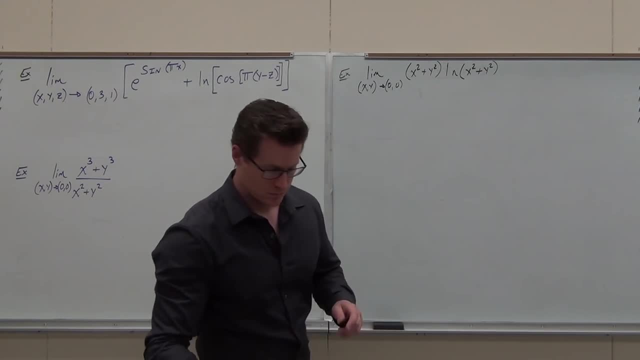 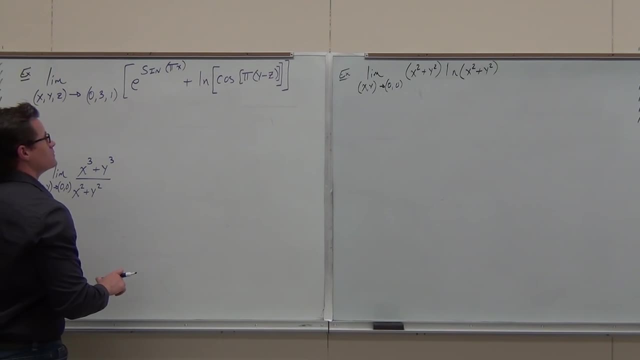 Oh, oh, oh, Oh, oh, oh, Thank you. Oh, oh, oh, Thank you, Thank you. Oh, oh, oh, Thank you. What's the X value, Y value, Z value? Instead of trying to do all of this math in your head, 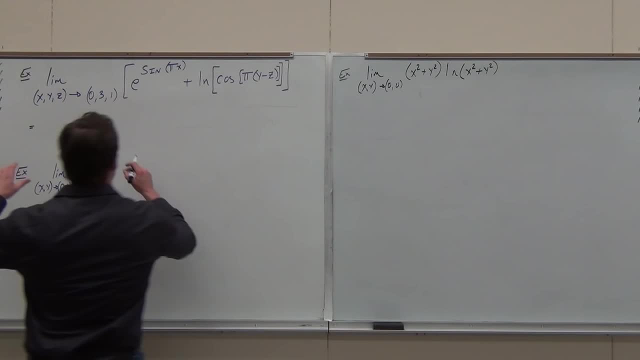 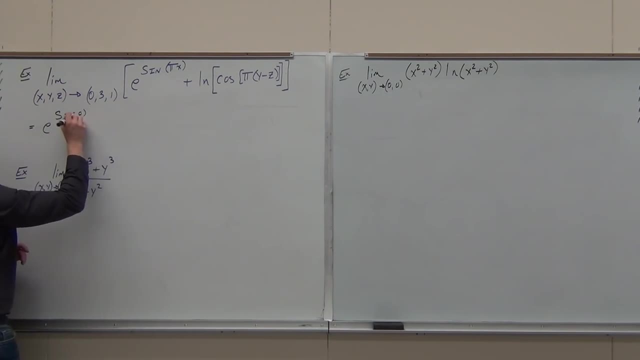 probably no good idea. at least write out some pieces of it. All right. so here I'm writing out E to the sine of. I do know that's zero, so I'm going to put the zero E to the sine of zero plus LN. that's got to be there. 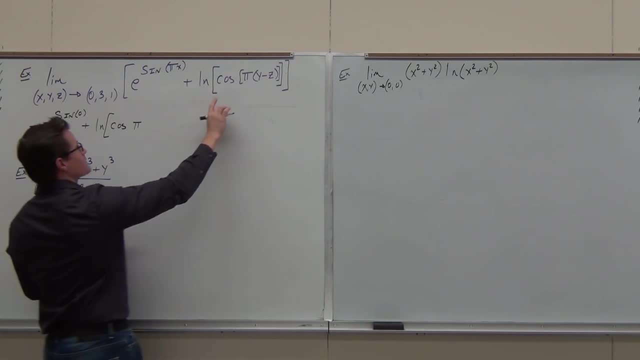 cosine, that's got to be there. Pi, that's got to be there. But I would do things like this: 3 minus 1 is 2.. So this is times 2, or you can put 2 pi. Does that make sense to you? 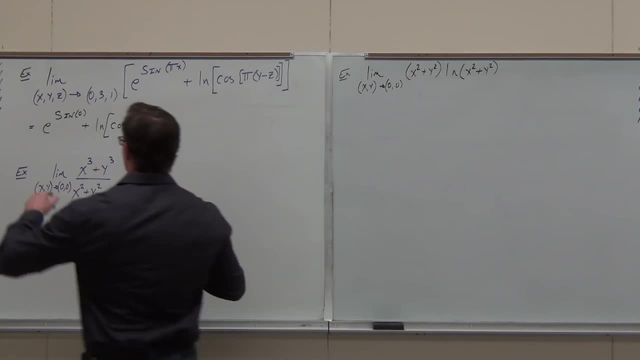 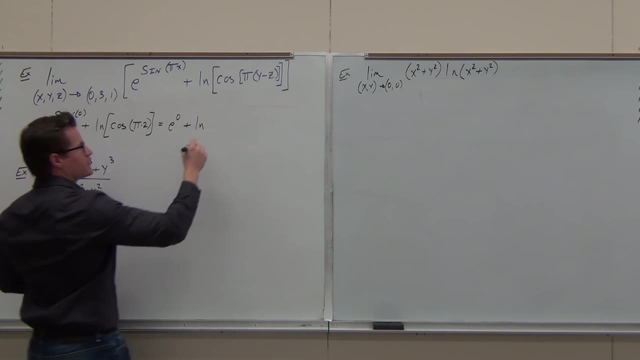 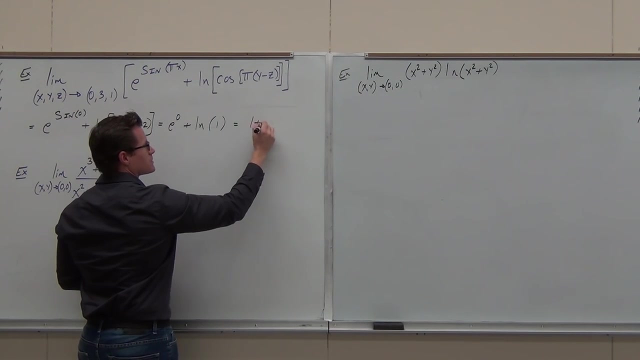 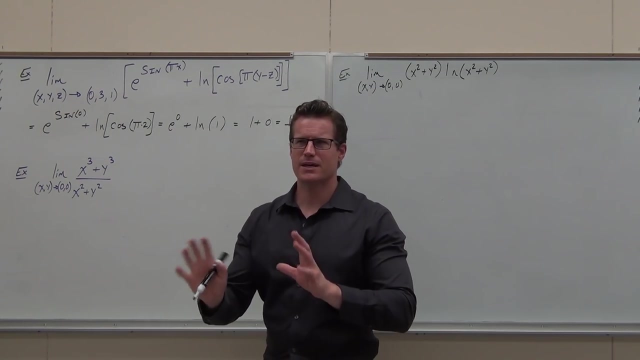 I do just little stuff, not a whole bunch. It's crazy too hard to do that. How much is sine of zero? How much is cosine of 2 pi? How much is that Plus zero equals That's one. Okay, yes, no. 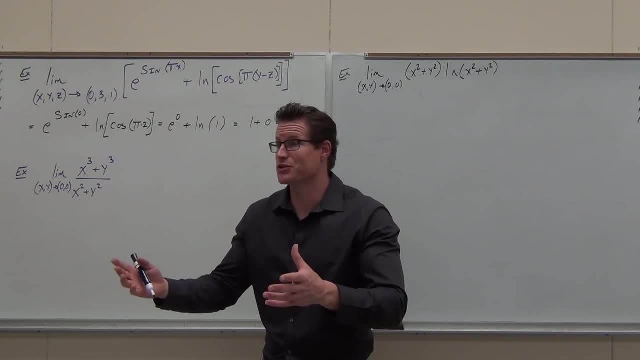 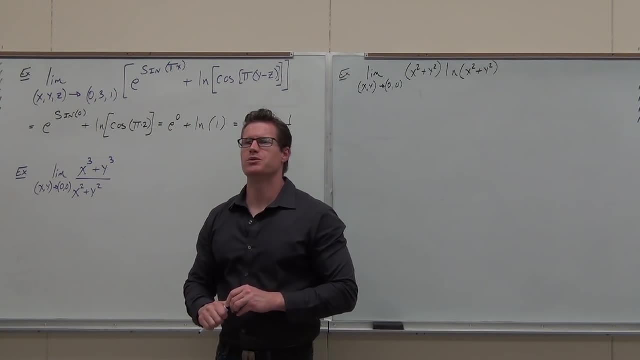 Easy, medium hard- Plugging stuff in- pretty easy as long as you know to do that. Now, did you think about that one? as we were doing the problem? Did you think about that one? What's the first thing you always do with limits? 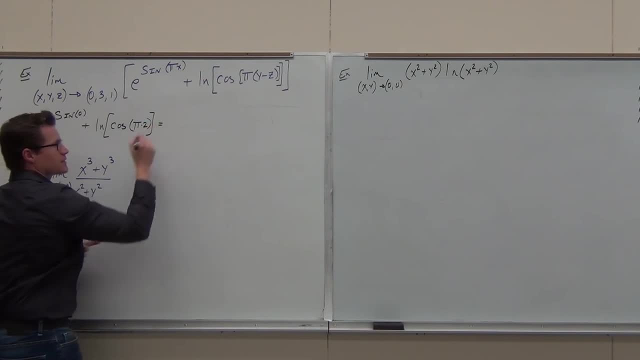 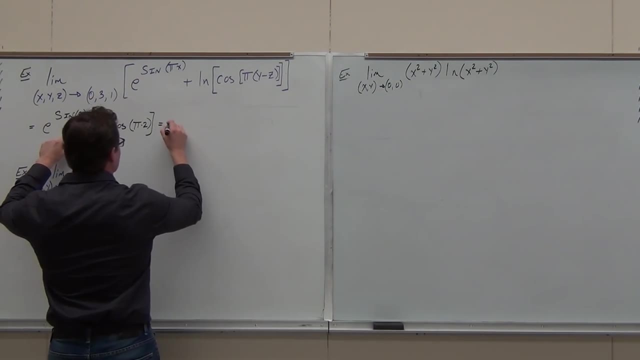 So this is times 2, or you can put 2 pi. Does that make sense to you? I do just little stuff, not a whole bunch. It's crazy too hard to do that. How much is sine of 0?? How much is cosine of 2 pi? 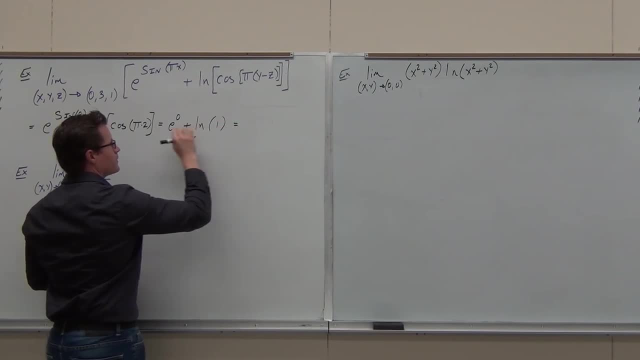 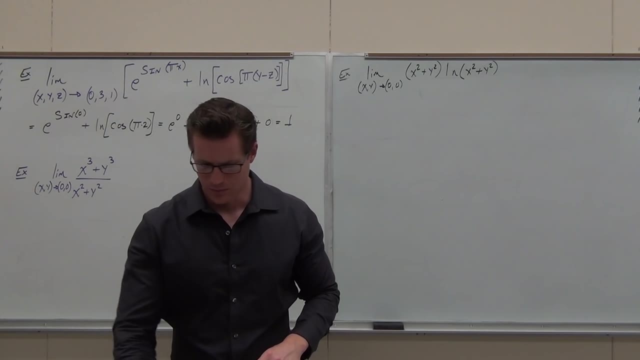 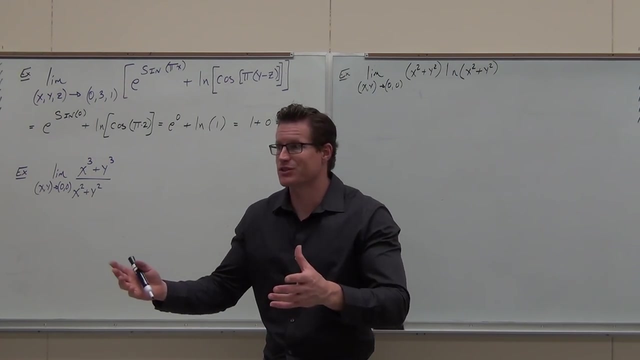 How much is that? 2 pi Plus Zero, Zero Equals 1. And then it's 1.. OK, yes, no, Easy, medium hard Plugging stuff in. pretty easy, as long as you know to do that. 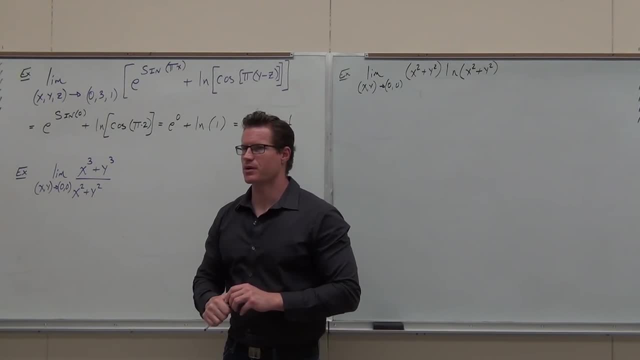 Now, did you think about that one as we were doing the problem? Did you think about that one? What's the first thing you always do with limits? Plug it in. Plug it in. What does it give you? There, there, there, there. 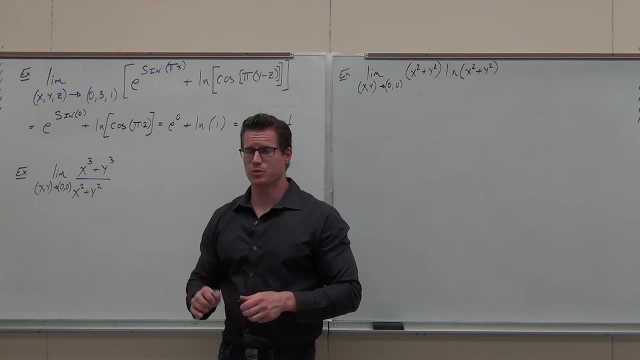 Crap. Every other time, we've tried to prove that this doesn't exist. Now we're going to try to prove it does exist. There's a few ways that we can go about thinking about this. One of them is the squeeze theorem, which we're not going to do right now. 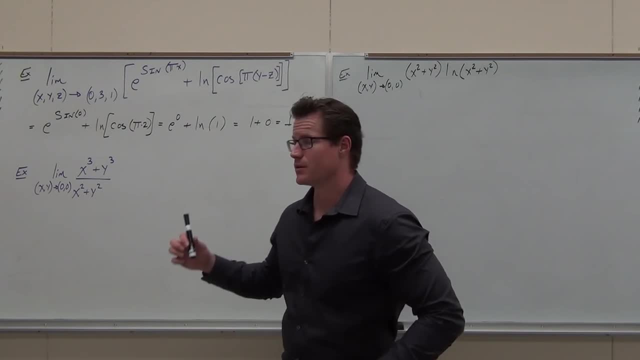 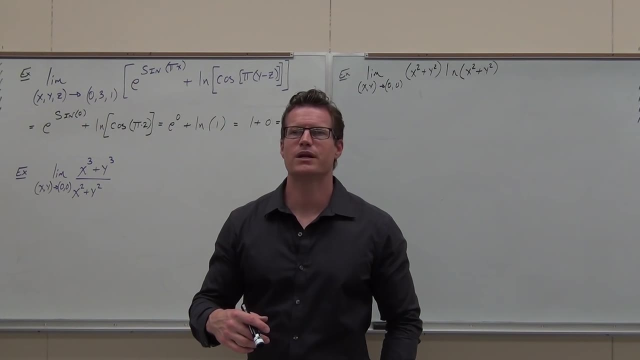 We'll do it later, a little bit later. One of them is the squeeze theorem. Another one is: well, you can do some algebraic manipulation or you can do a really cool trick. sometimes that helps a lot. If it's not working for you and you're like dang, I don't even know. 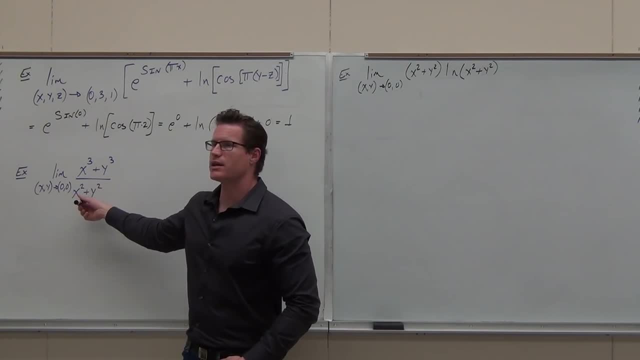 but you see a lot of x squared plus y squareds floating around. You see a lot of that. You see what I'm talking about. Number one thing: goodness, don't make me drink at night. Please don't start canceling this stuff out. 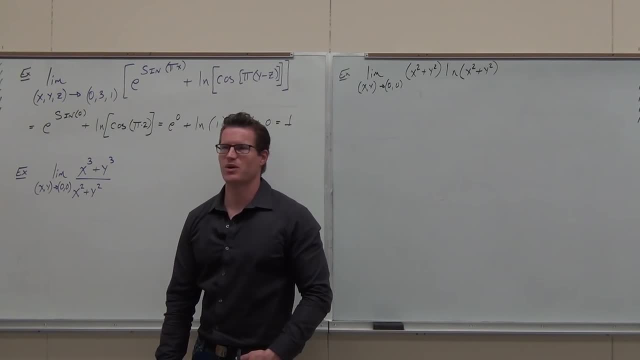 I like crossing stuff out. I've crossed it out. Please don't do that. I swear please. I'm begging, begging. Please don't do that. Also, I don't want you to start factoring. You can't factor this. 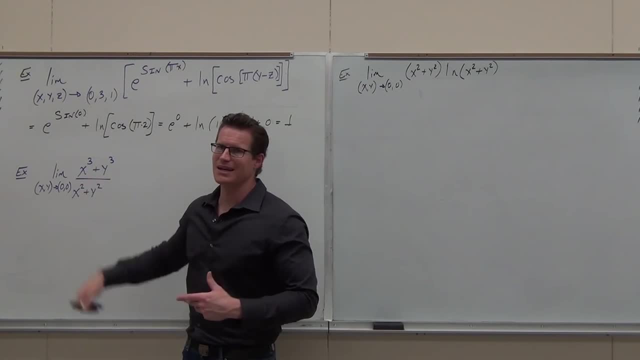 It's impossible. You can factor that, but it's not going to help you. You get your x plus y times this quadratic. that's not factorable, So you go. what am I supposed to do with that? That's not going to help. 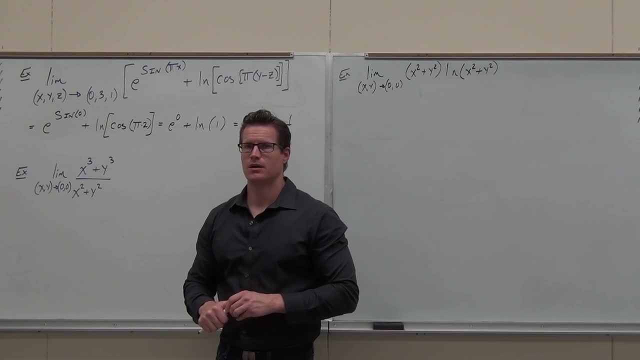 Plug it in. What does it give you Crap. Every other time we've tried to prove this doesn't exist. now we're going to try to prove it does. There's a few ways that we can go about thinking about this. 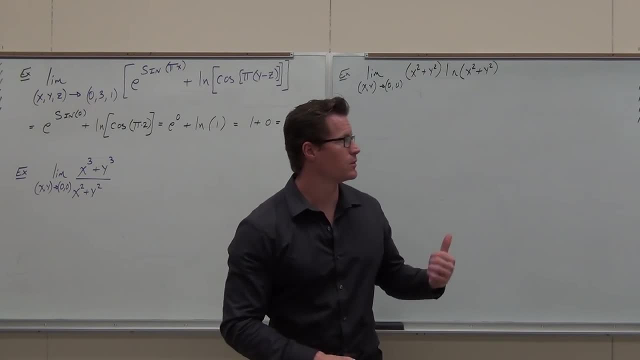 One of them is the squeeze theorem, which we're not going to do right now. we'll do it later, a little bit later. One of them is the squeeze theorem. Another one is: well, you can do some algebraic manipulation. 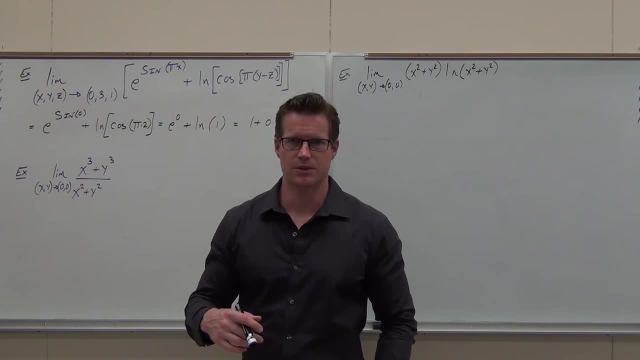 or you can do a really cool trick. sometimes that helps a lot If it's not working for you and you're like dang, I don't even know, but you see a lot of x squared plus y squareds floating around. You see a lot of that. 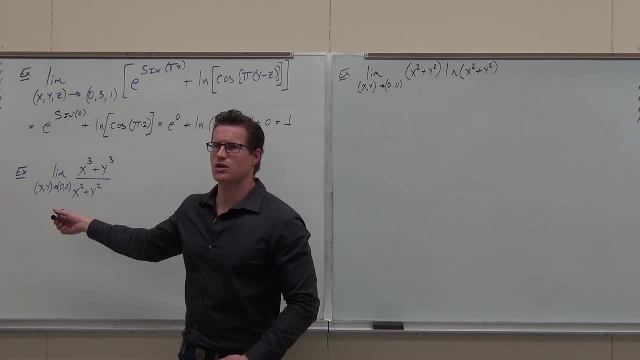 You see what I'm talking about. Number one thing: goodness, don't make me drink at night. Please don't start canceling this stuff out. I like crossing stuff out. I've crossed it out. Please don't do that, I swear, please. 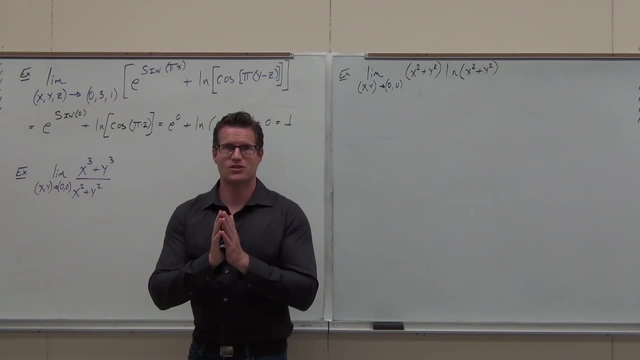 I'm begging, begging. Please don't do that. Also, I don't want you to start factoring. You can't factor this, It's impossible. You can factor that, but it's not going to help you. You get your x plus y times this quadratic. that's not factorable. 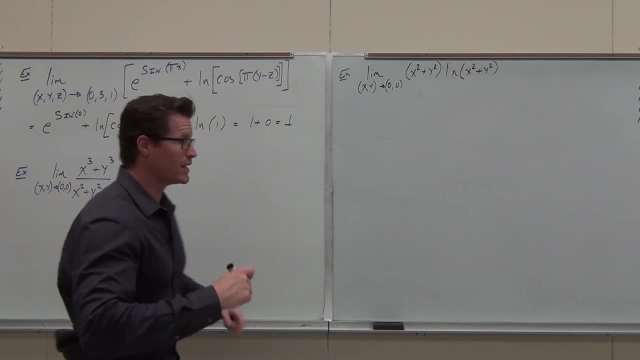 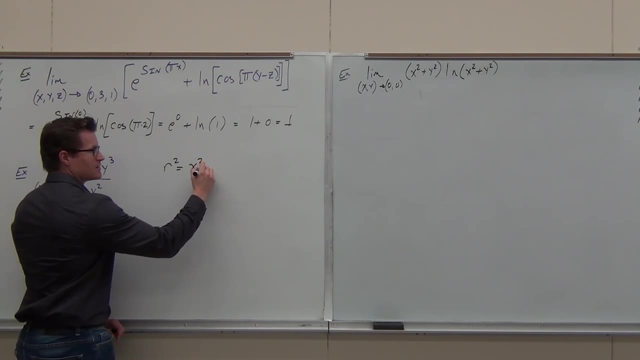 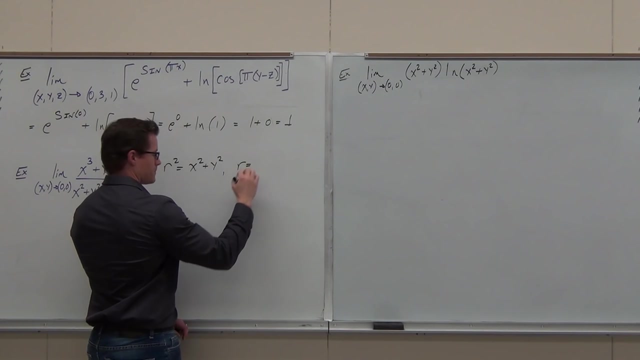 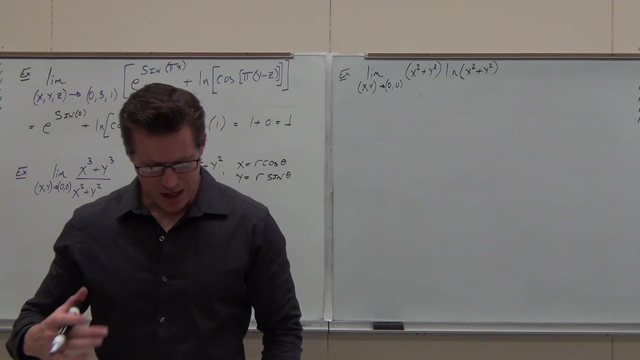 So you go. what am I supposed to do with that? That's not going to help. What I do see is that, goodness, I know that this is true As long as they let this and that also be true. Sometimes we can trick our problem into thinking that it's polar. 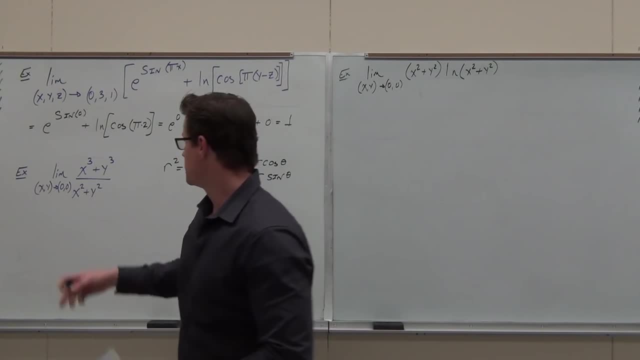 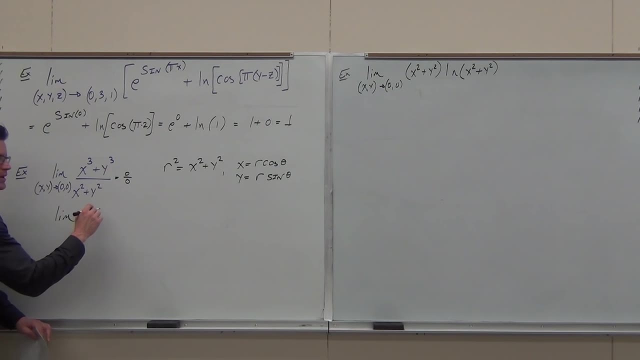 Make it polar. If you get zero over zero and you see a lot of x squared plus y squared, zero over zero, and you go. well, let's try to make this thing happen. If we do, we can let this go to r. 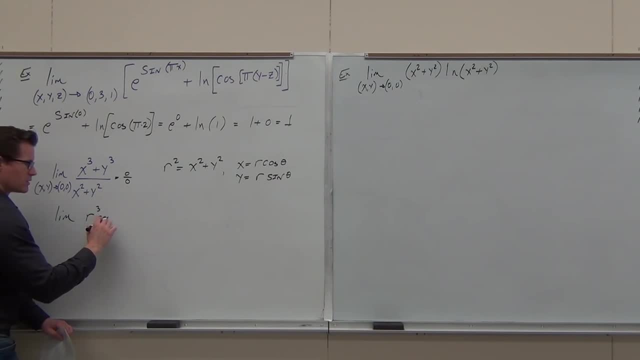 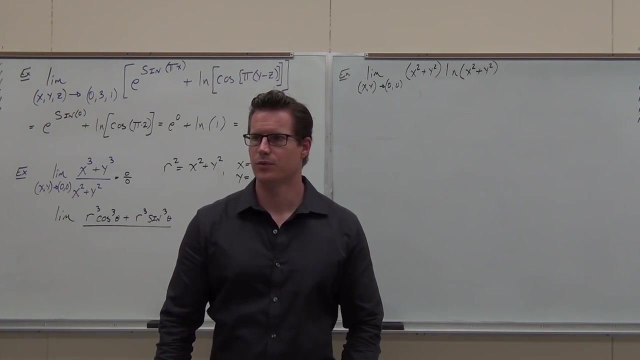 Well, x would be r cosine theta. So r cubed cosine cubed theta plus r cubed sine cubed theta. Now, if you're okay with that one for real, let us know. Do you see where this came from? 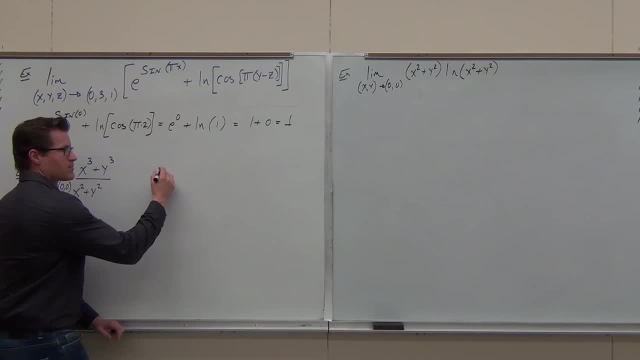 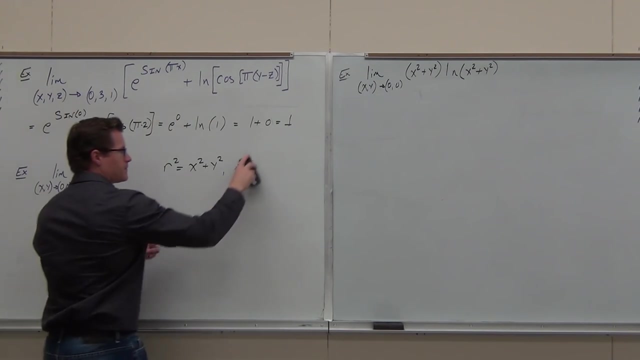 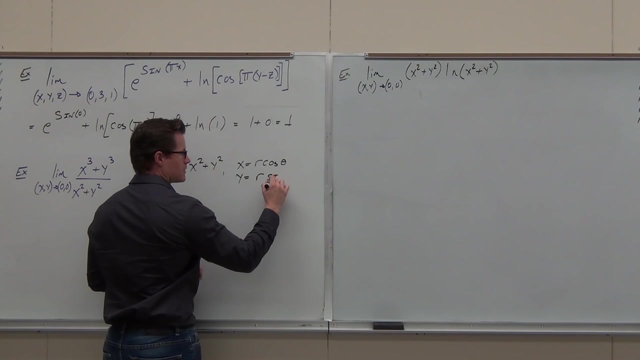 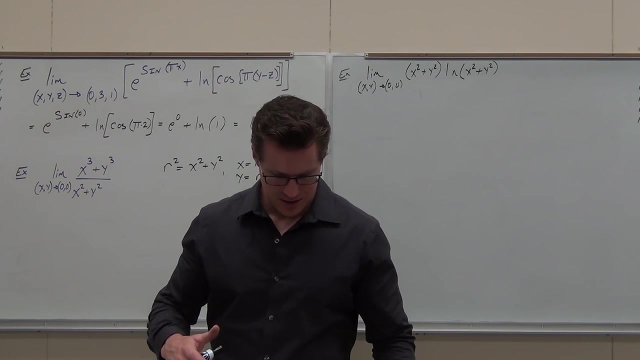 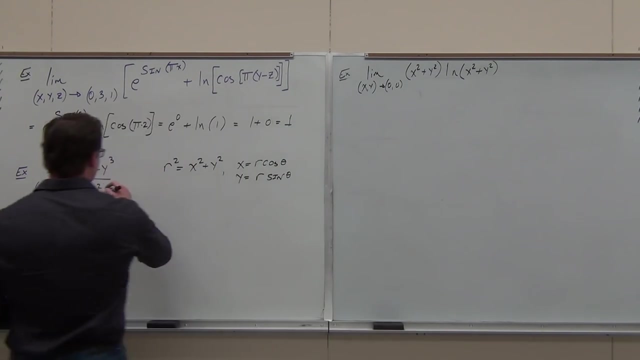 What I do see is that, goodness, I know that this is true As long as they let me Right This, and that all should be true. Sometimes we can trick our problem into thinking that it's polar, Make it polar If you get 0 over 0 and you see a lot of x squared plus y squared, 0 over 0, and you go. 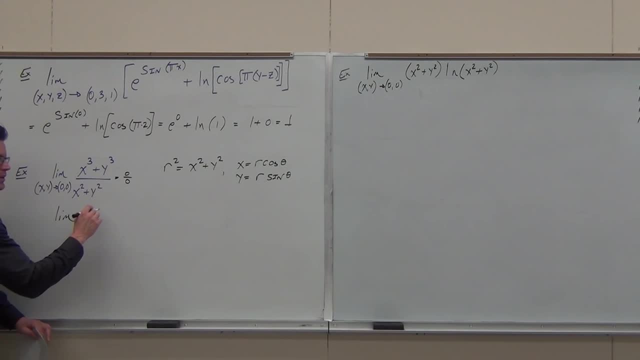 well, let's try to make this thing happen. If we do, we can let this go to r. Well, x would be r cosine theta, So r cubed cosine theta, So r cubed sine cubed theta, plus r cubed sine cubed theta. 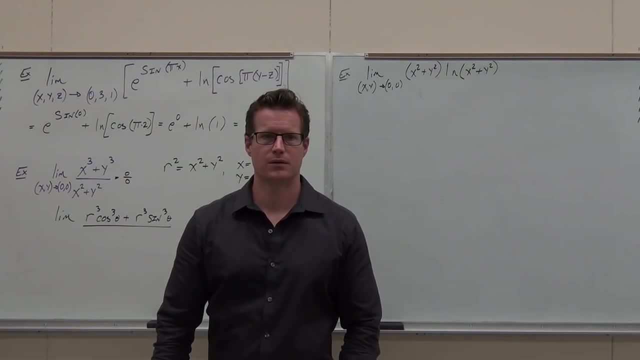 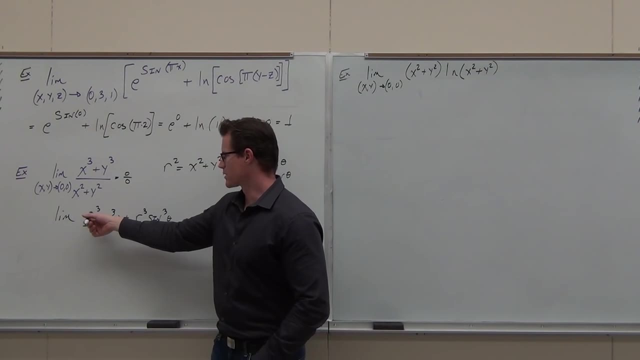 I don't know. if you're okay with that one for real, Let us know. Yeah, Do you see where this came from? If x is r cosine theta, then x cubed is r cosine theta cubed. r cubed cosine theta cubed. 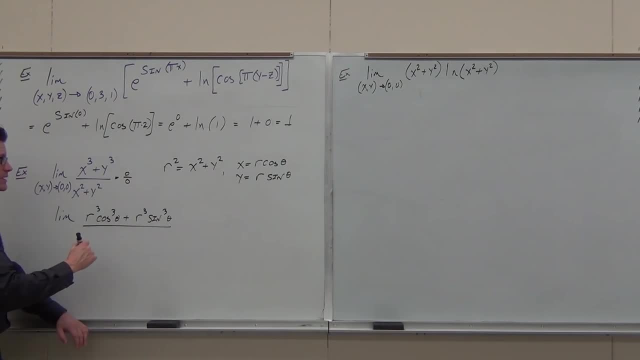 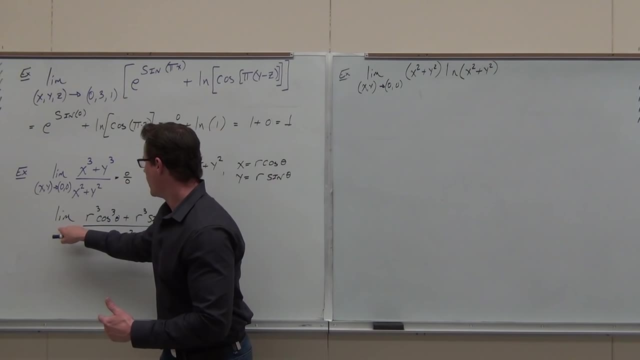 Same thing for the y. What's the denominator? What's that going to be My next question? This is a really kind of interesting question: What's my independent variable? What's it going? What's x and y relate to up here? 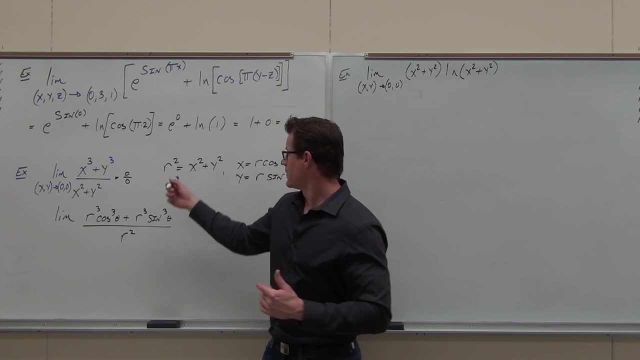 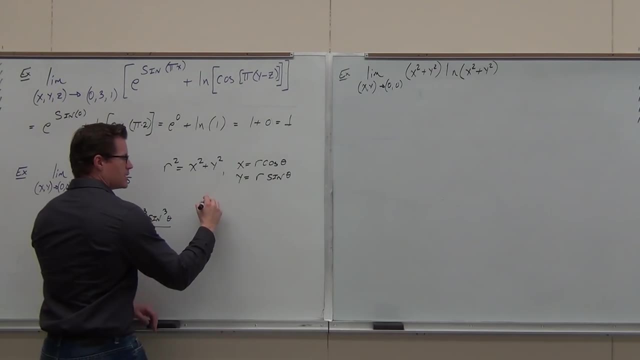 Say what Theta? x and y are only tied. well, they're tied to theta, but they're also tied to r. Well, let's see what happens If x and y go to 0, 0.. What's x squared plus y squared going to? 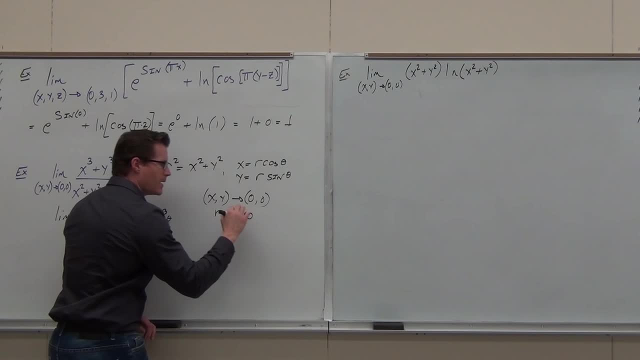 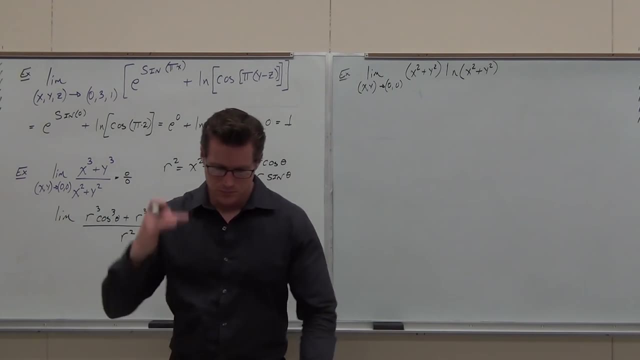 Then r would also go to 0, but look, it can't be negative. All right, This is going to give us something that's positive. so plus right hand side. So if we're going to use that, then our r is a thing that's going to 0,, but it's right. 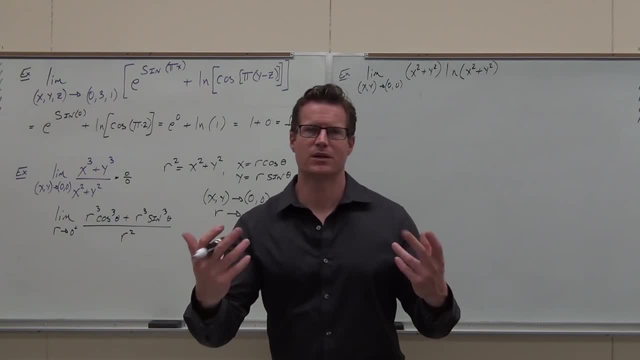 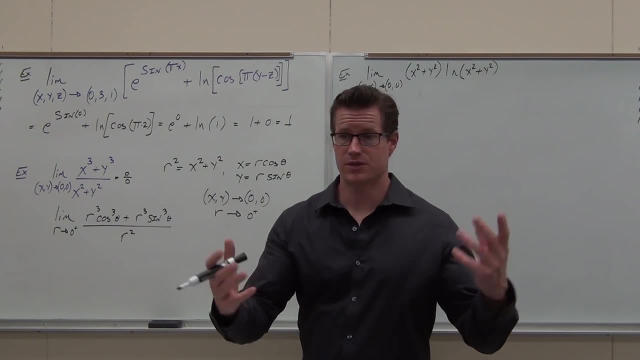 side Now. can you see something nice to do? Come on quickly, See something nice to do. What are you going to do? Not yet, What are you going to do? Simplify. You're going to simplify How. 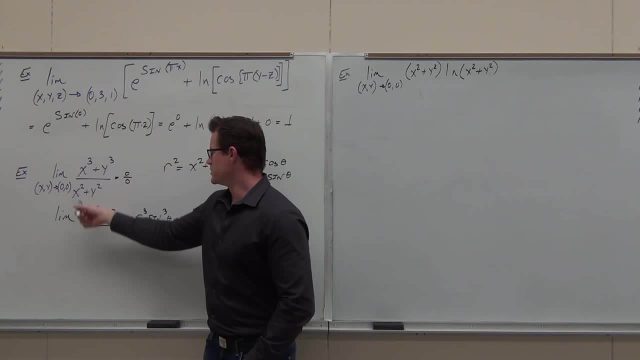 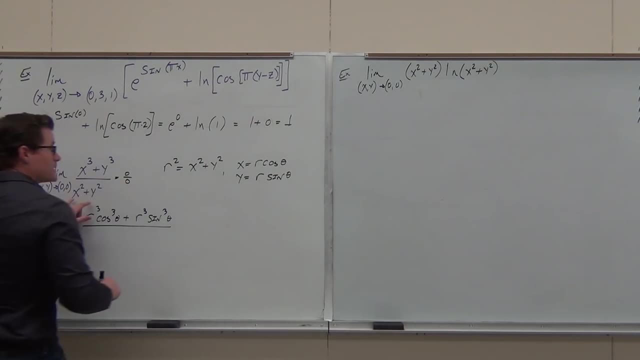 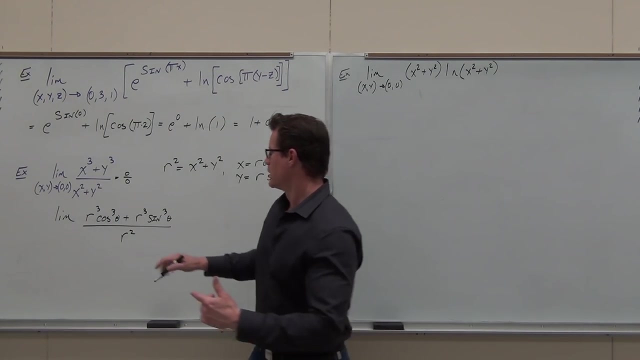 If x is r cosine theta, then x cubed is r cosine theta cubed, r cubed cosine theta cubed. Same thing for the y. What's the denominator? What's it going to be My next question? this is a really kind of interesting question. 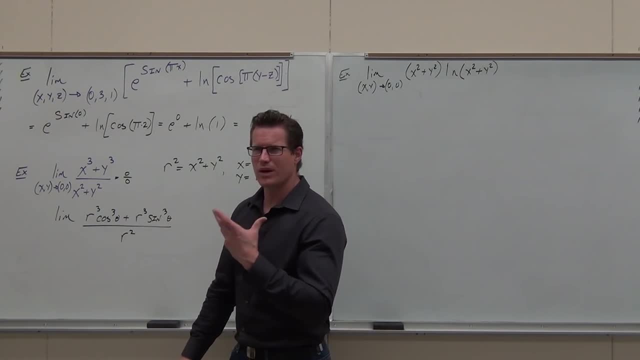 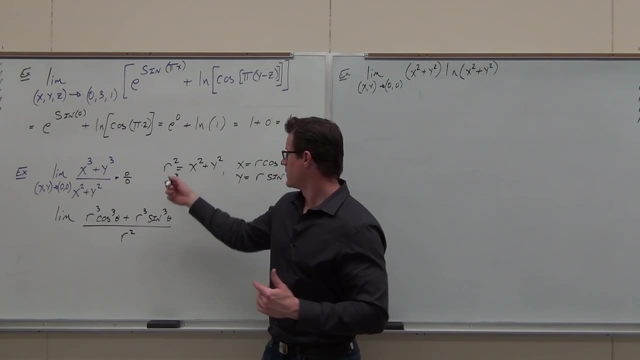 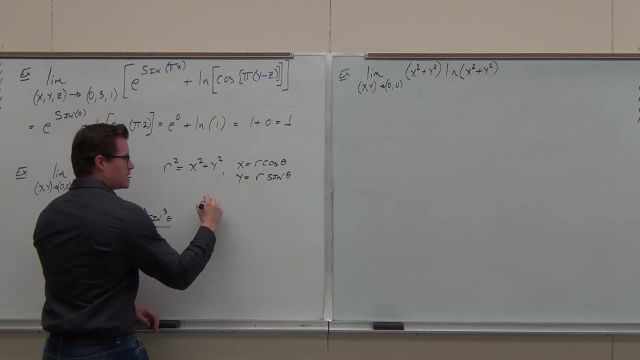 What's my independent variable? What's it going? what's x and y relate to up here? Say what X and y are only tied. well, they're tied to theta, but they're also tied to r. Well, let's see what happens. 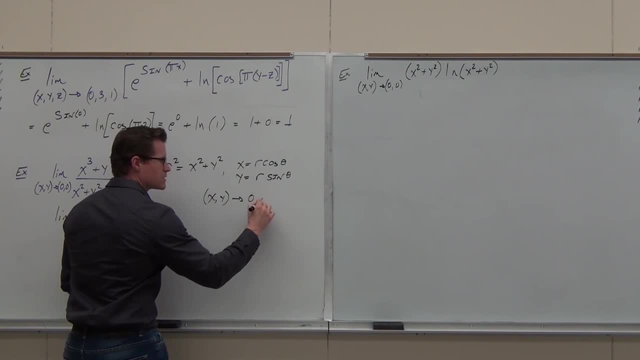 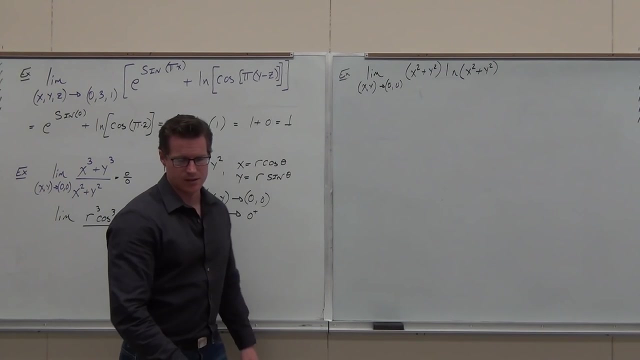 If x and y go to zero, zero, what's x squared plus y squared going to? Then r would also go to zero. But look, it can't be negative. all right, This is going to give us something that's positive. so plus right-hand side. 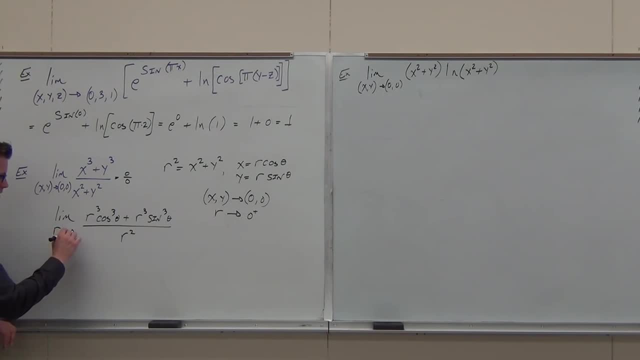 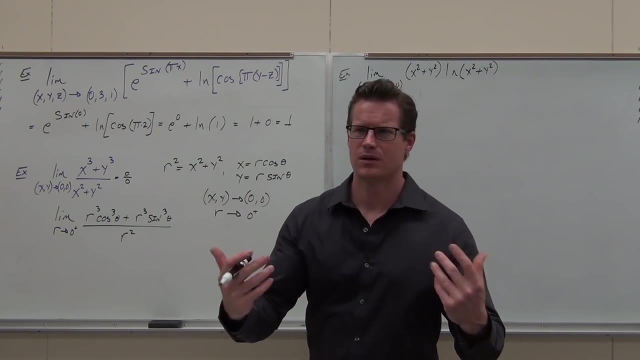 So if we're going to use that, then our r is a thing that's going to zero, but it's right-sided. Now, can you see something nice to do? Come on quickly, See something nice to do. What are you going to do? 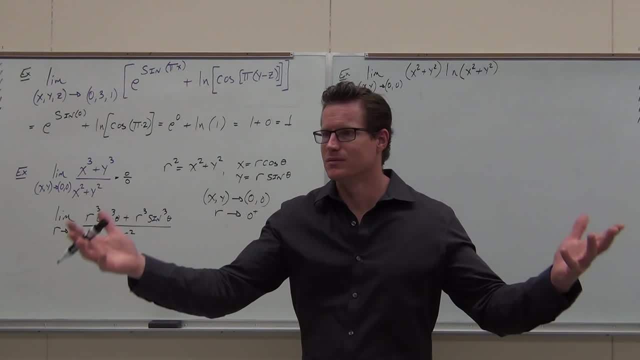 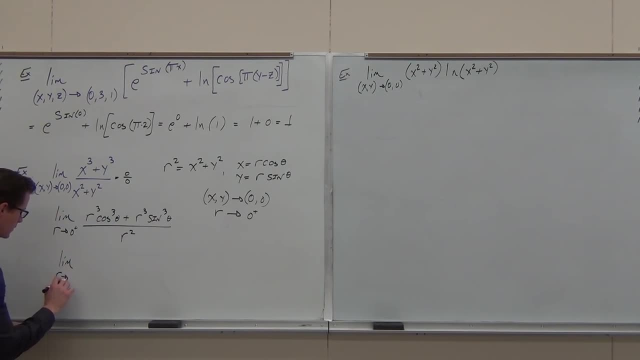 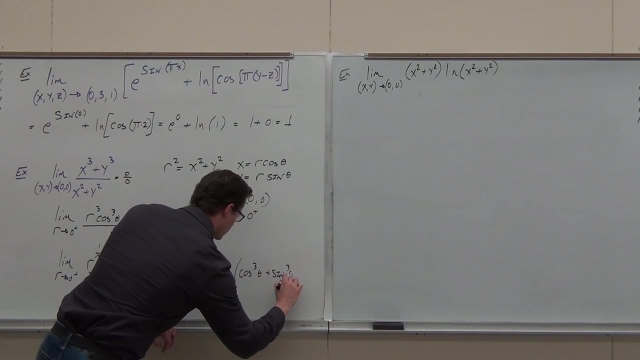 Not yet. What are you going to do? You're going to simplify How It's the F word. Come on, what are you going to do? So if we factor and we simplify? All right, Let's think about it. 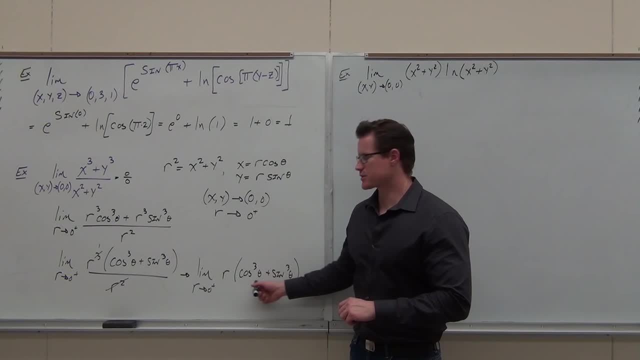 I don't even care what this is. Tell me why. I don't even care about what that is. What's the r doing? Zero, What's zero times? pretty much anything, Even if it's zero, I don't really care. So zero times anything is how much. 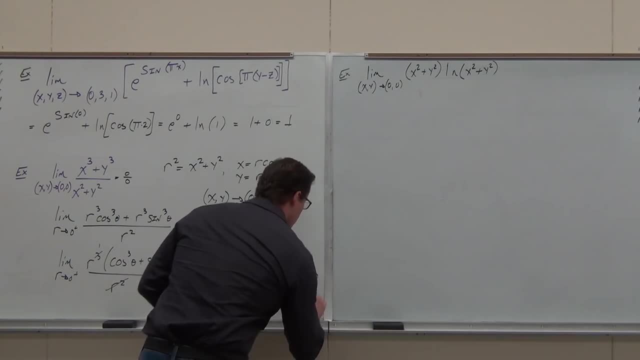 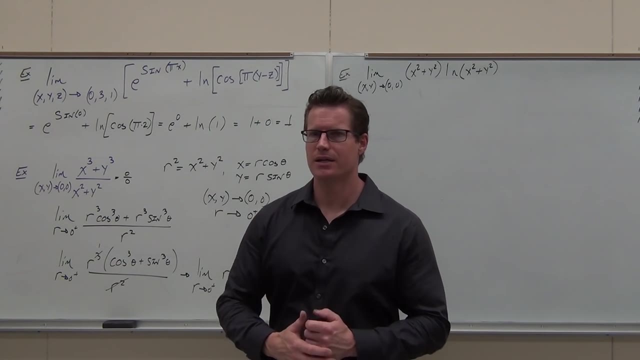 Zero, Zero. Does that prove the limit exists? Yes, Yes, it does. We plugged in a number. We actually got a number out That proves the limit exists And I feel okay with that. one Question: Why does the r have to go, or zero, from the right again? 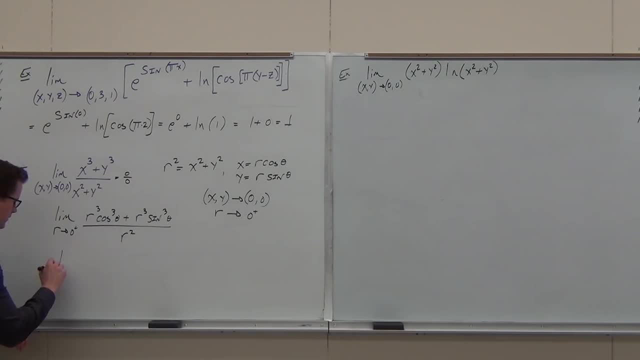 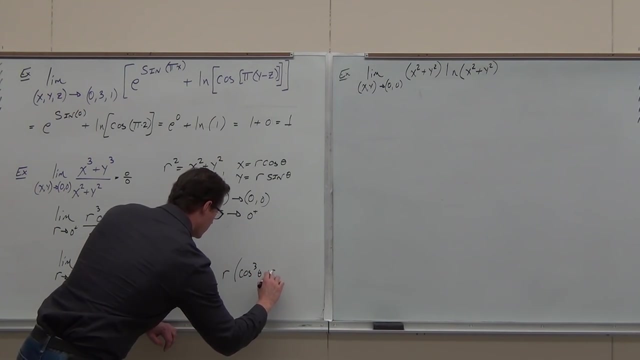 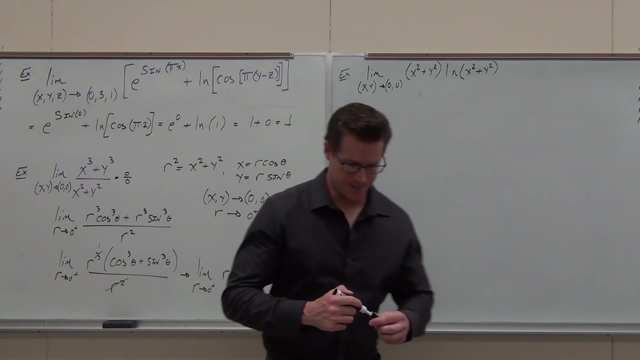 That's the F word. Come on, What are you going to do? So, if we factor And we simplify, Let's think about it. I don't even care what this is. Tell me why. I don't even care about what that is. 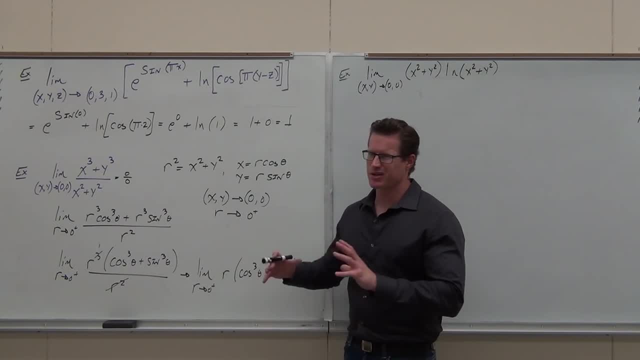 What's the r doing? 0.. What's 0 times? pretty much anything, And even if it's 0, I don't really care. So 0 times anything is how much? 0. 0.. Does that prove the limit exists? 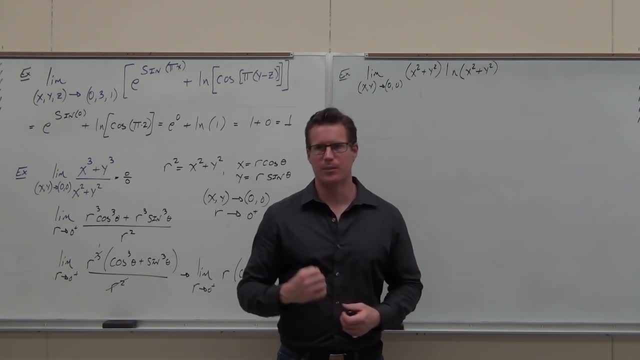 Yes, Yes, it does. We plugged in a number. We actually got a number out That proves the limit exists And I feel okay with that. one Question: Why does the r have to go, Or does 0 have to come right again? 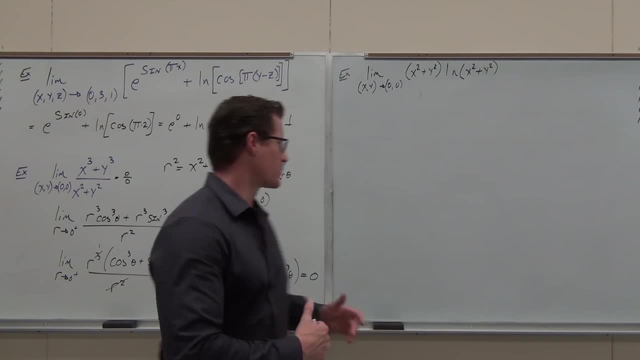 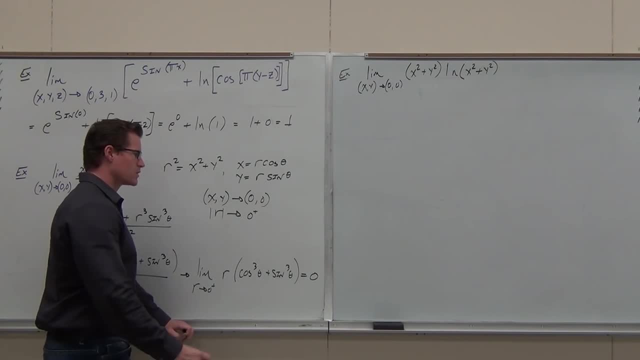 You could go absolute value. You could go absolute value. You could go absolute value, But you're never going to get a negative out of that. The absolute value of r. if you took the square root of both sides, you'd get the absolute value of that r. 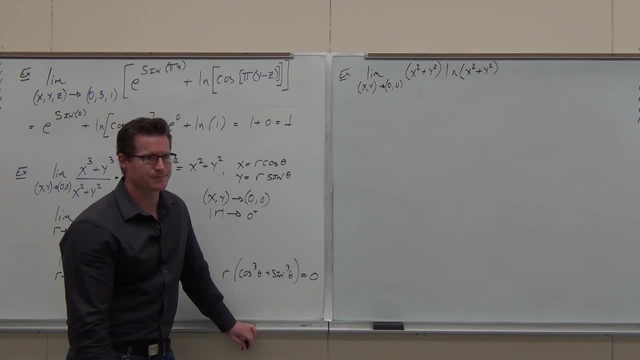 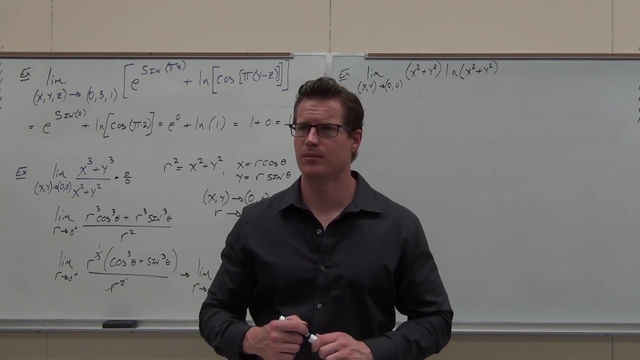 We just go 0 plus to not have to do with the negative, obviously, So that's why, Not a very big thing, Just make sure you go to 0.. Can you do it for the next one? Can you see the substitution for the next problem? 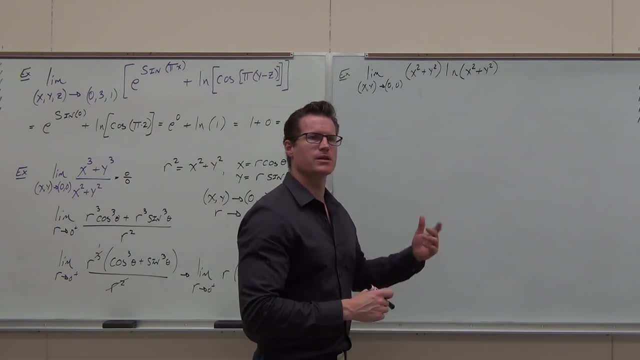 Because right now, if you plug this in, do you know what you get? if you plug this in, Plug in 0, 0. What do you get? Come on, folks, How much is this Times, how much is this? 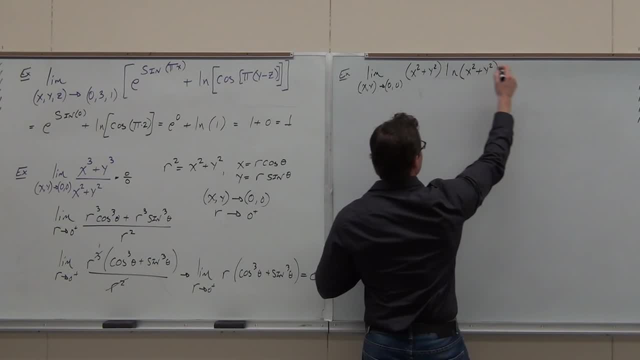 This is 0.. ln of 0 is negative infinity. ln as you approach 0, negative, it's doing this. That's what's happening. ln of 0, negative infinity. This is an indeterminate form, If only. 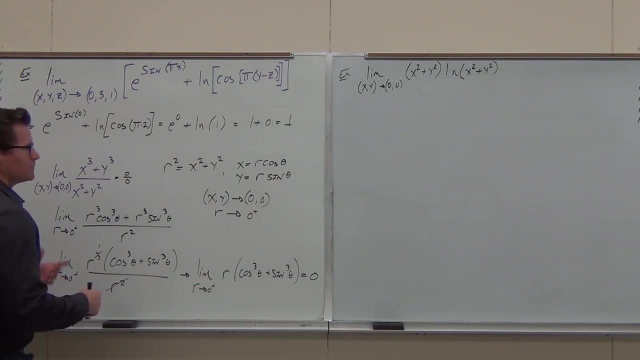 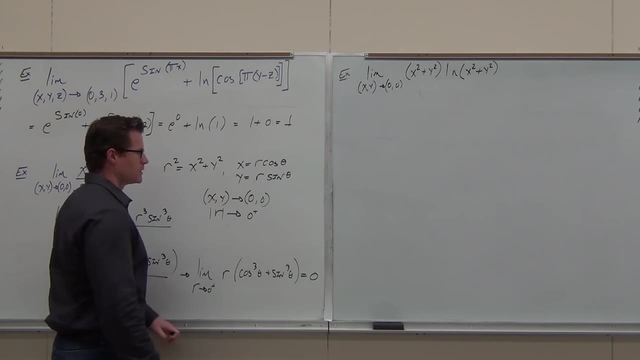 I missed that one. Well, a couple reasons. When we're man, you could go. You could go. absolute value, You could go, absolute value, But you're never going to get a negative out of that. The absolute value of r, if you took the square root of both sides. 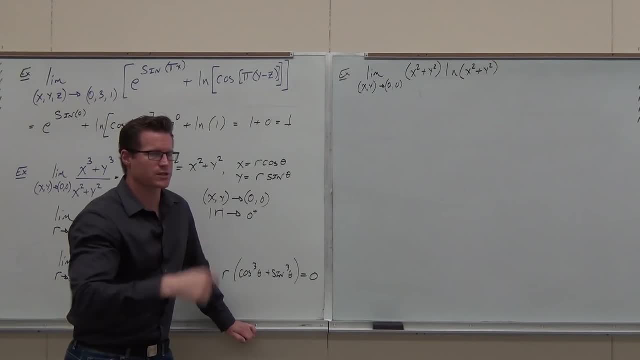 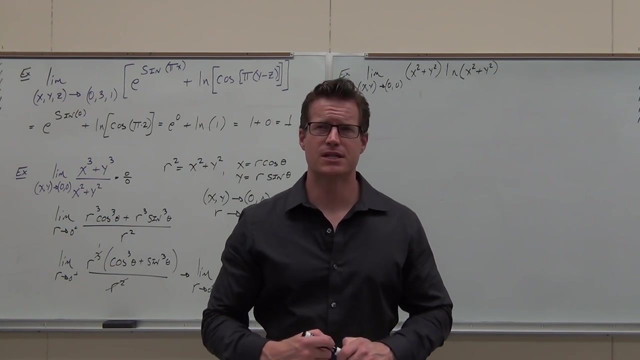 you'd get the absolute value of that r. We just go zero plus to not have to do with the negative, honestly. So that's why Not a very big thing, Just make sure you go to zero. Can you do it for the next one? 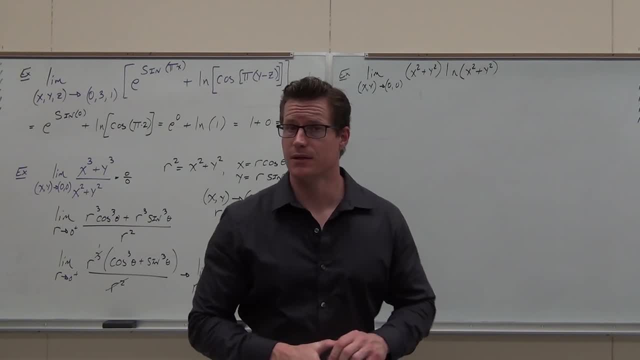 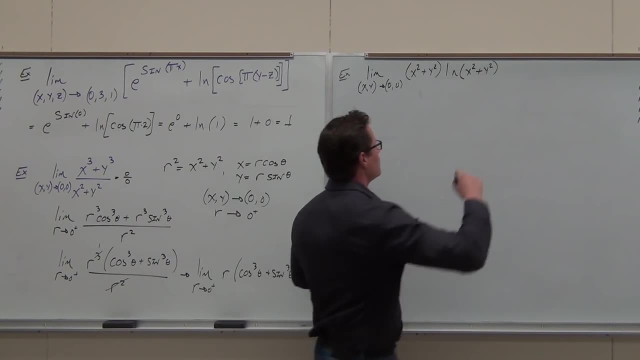 What's the substitution for the next problem? Because right now, if you plug this in, do you know what you get? if you plug that in, Plug in zero, Plug in zero to zero, What do you get? Come on, folks. 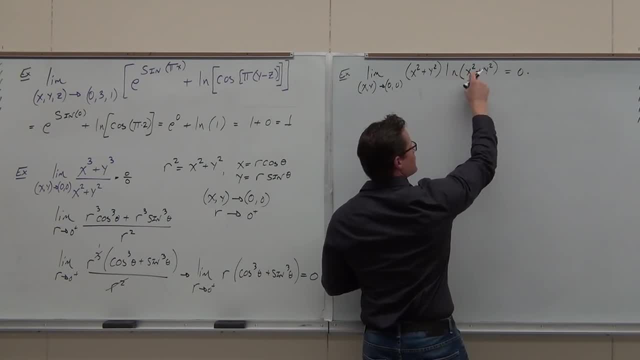 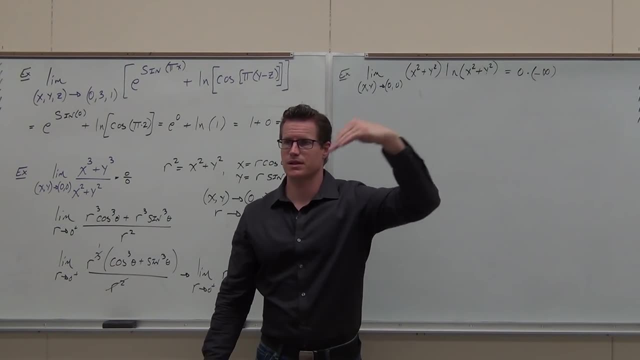 How much is this Times? how much is this? This is zero. ln of zero is negative infinity. ln. as you approach zero, it's doing this. That's what's happening. ln of zero: negative infinity. This is an indeterminate form. 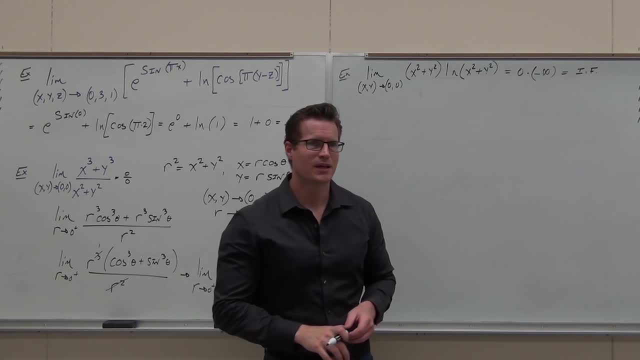 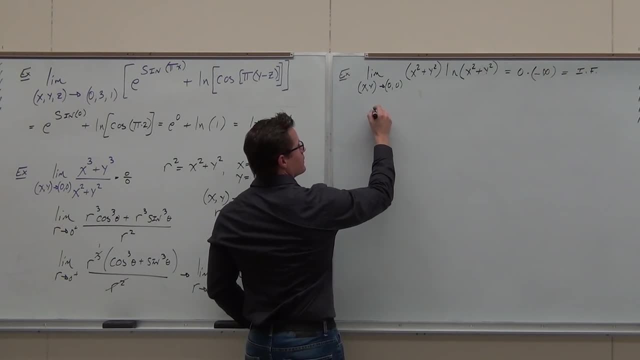 If only Indeterminate form. That's what that is. Well, if we start doing stuff like: all right, let's let x squared plus y squared equal r squared, then we can change our limit to ln r squared, Quick hint, and I'll be OK with the substitution. 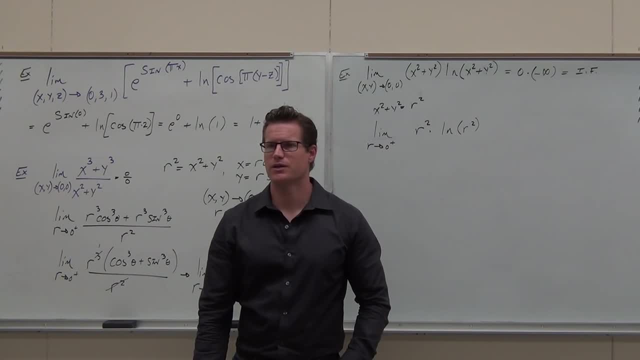 Please don't let your r squareds change to r's magically. Don't do that. x squared plus y squared is r squared. Are you following the math on this? Do you see why our r's going to go to zero? Now, that doesn't help you with the indeterminate form. 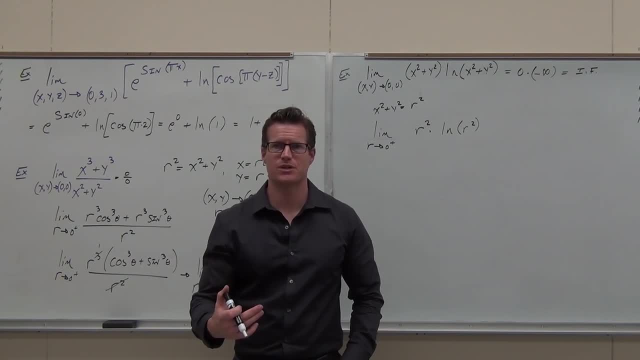 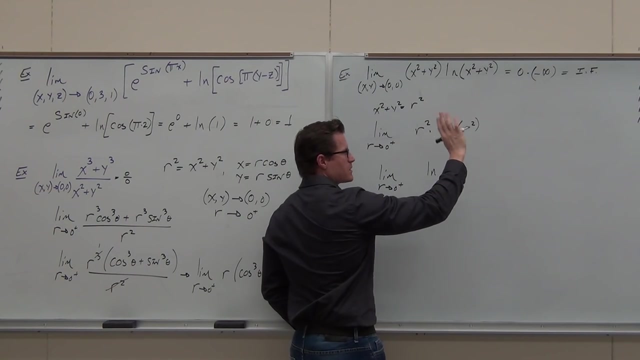 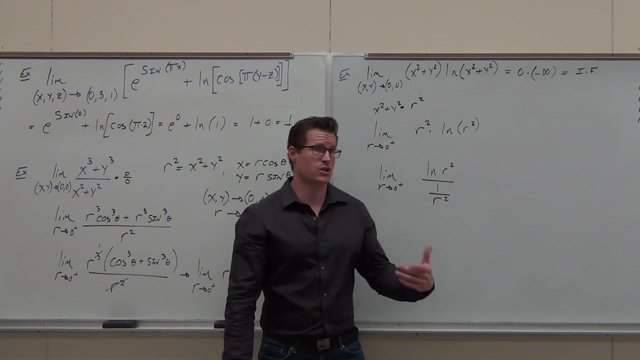 but if you ever did limits of indeterminate forms from section 6.7 from Calculus 2, then you know that at this point if you have zero times some type of infinity and you create this complex fraction, you change the zero into a different thing, change it into infinity. 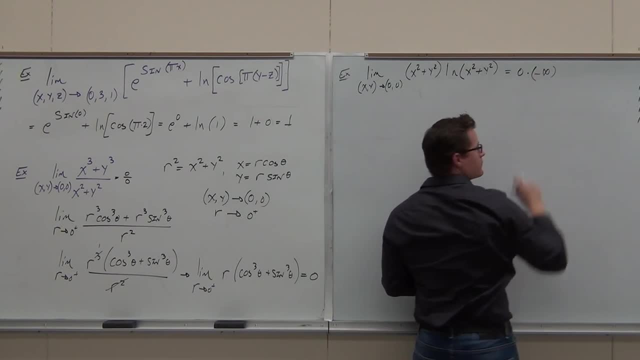 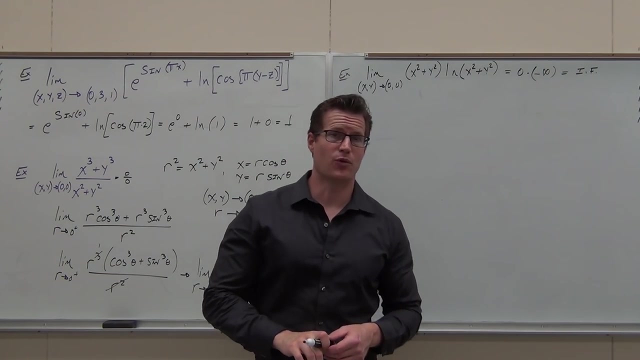 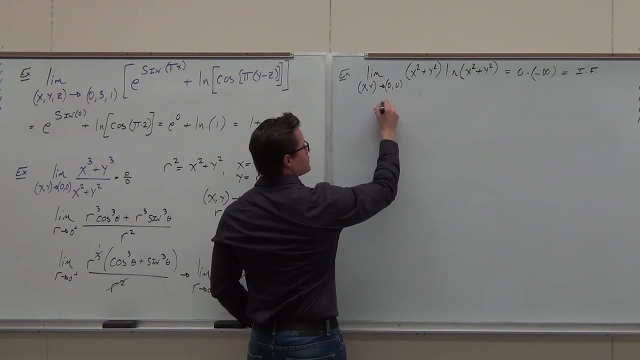 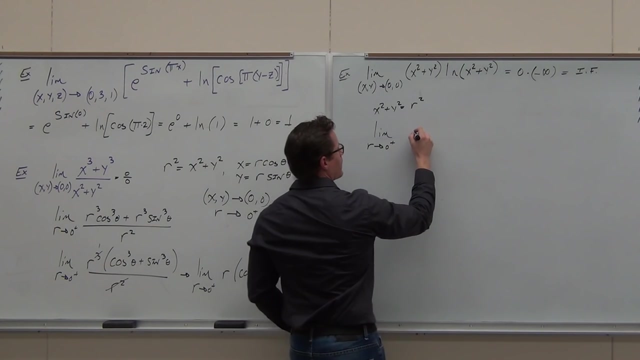 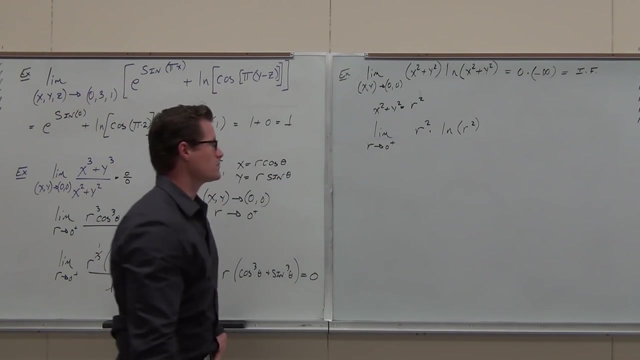 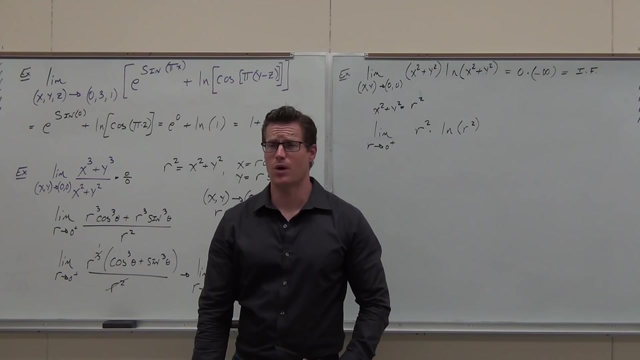 Indeterminate form that x squared plus y squared is r squared. 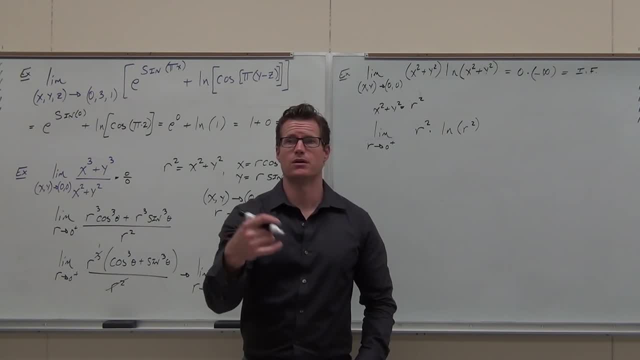 Are you following the math on this? Do you see why r is going to go to zero? Now that doesn't help you with the indeterminate form, but if you ever did limits of indeterminate forms from section 6.7 from Calculus 2, then you know that. 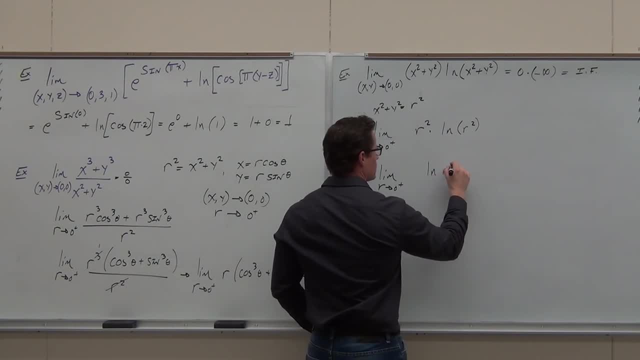 at this point, if you have zero times 1, some type of infinity, and you create this complex fraction, you change the zero into a different, you change it into a different thing, change it into infinity. Now you have infinity. Notice this. 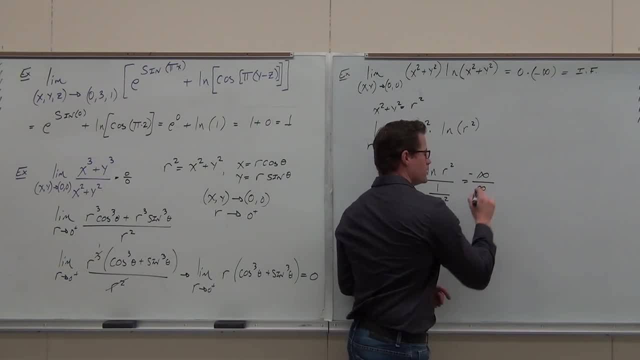 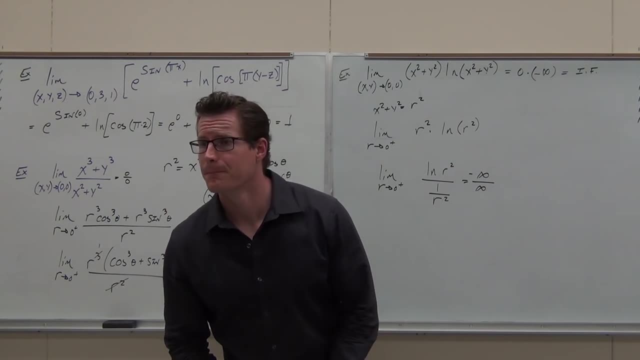 What's 1 over 0? Oh, it's infinity. What do you do any time you see infinity over infinity? Come on, open it up, Say what: L'Hopital, L'Hopital. So here, even if you move this down, L'Hopital. 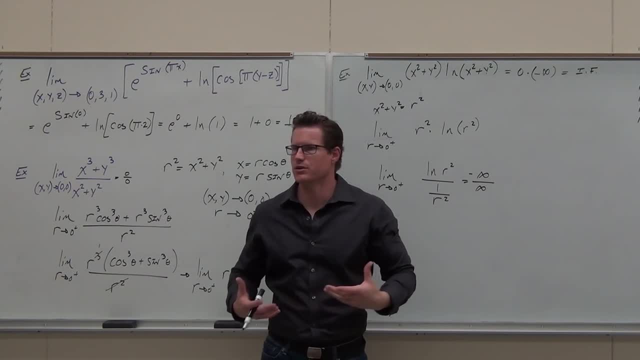 how are you going to do it? Because you've got two variables, two independent variables. How are you going to do that? But if we change it to one independent variable and we manipulate it, now you've got L'Hopital. I'm not going to finish it. 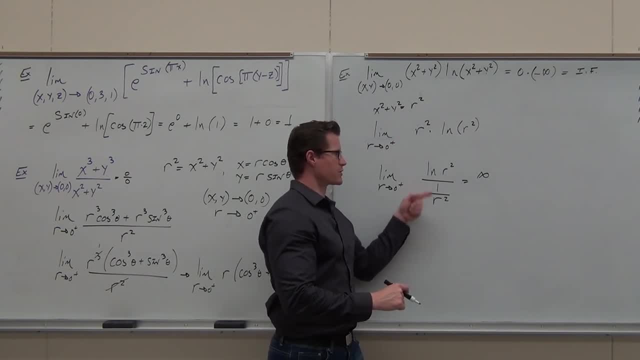 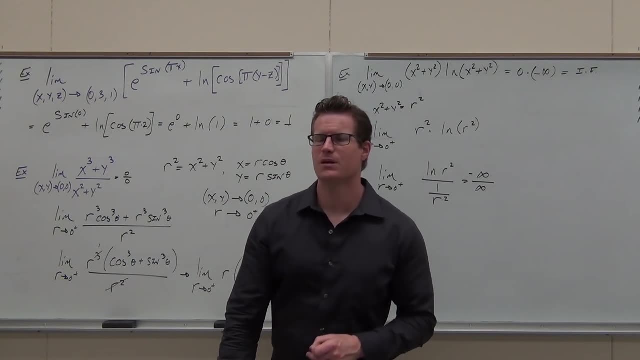 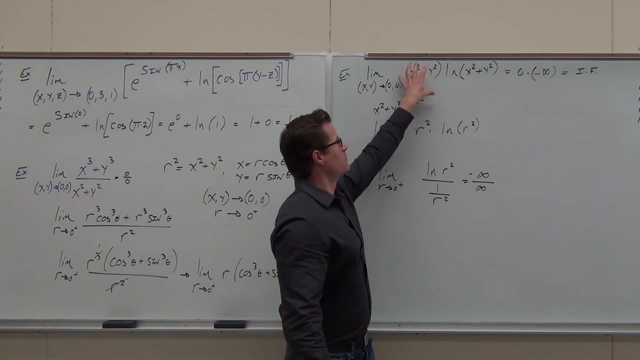 Now you have infinity. Notice this. What's one over zero? Oh, it's infinity. What do you do? any time you see infinity over infinity? Come on, open it up. Say what? Open it up, Open it up. So here, even if you move this down, 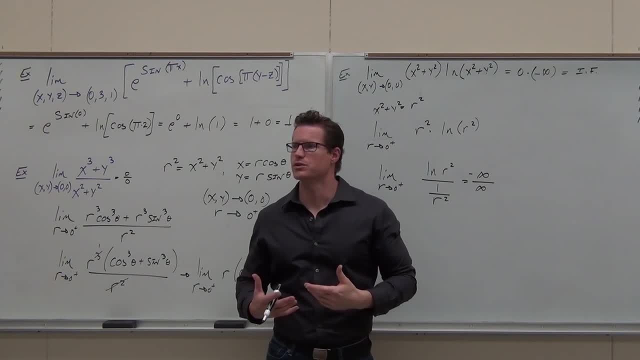 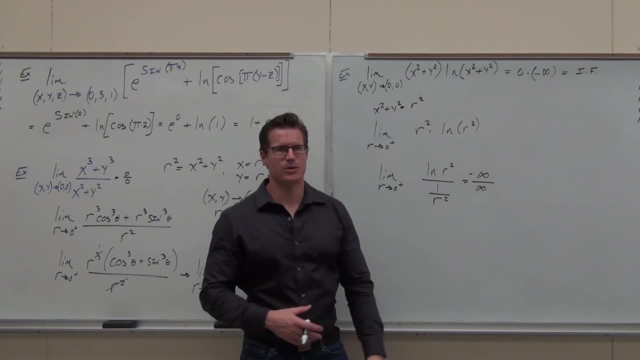 L'Hopital's. how are you going to do it? Because you've got two variables, two independent variables. How are you going to do that? But if we change it to one independent variable and we manipulate it, now you've got L'Hopital's. 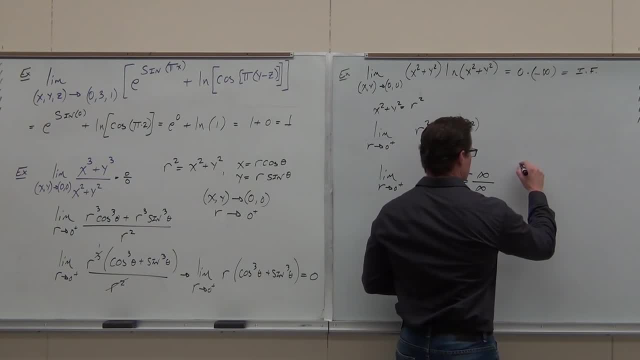 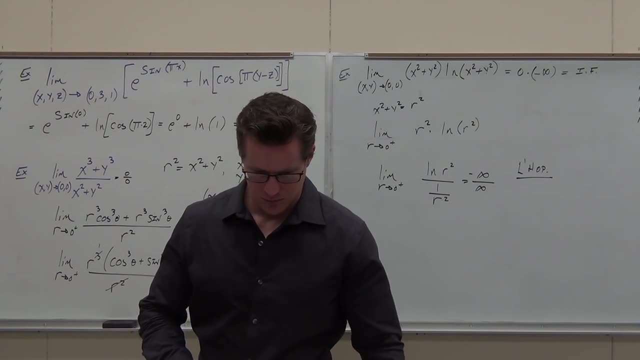 I'm not going to finish it. I want you to finish it. Try L'Hopital's here. So kind of a cool idea. I hope you like this idea. I liked it. the first time I saw it I thought it was pretty neat. 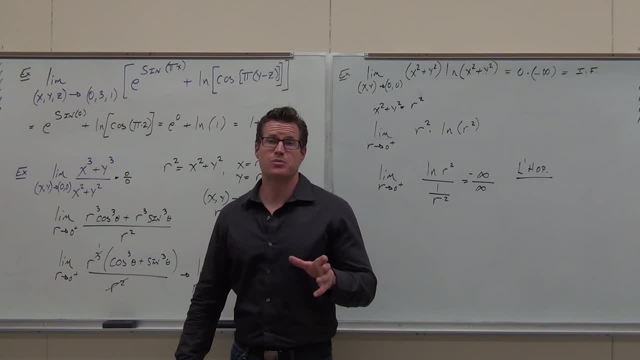 So what do I just do with this? I don't know. give up. No, Let's try to change it to polar. Let's make x squared plus y squared equal r squared. We've got some substitution for x and y. Same thing here. 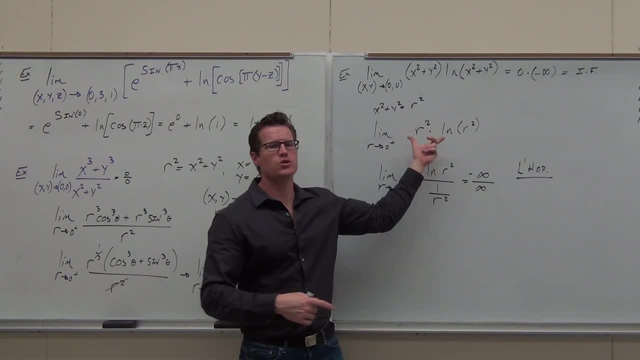 As soon as we do that, even if we have indeterminate forms, you know what to do with one variable. You can start creating from zero times infinity. infinity over change. it make a fraction over infinity, and then L'Hopital's. 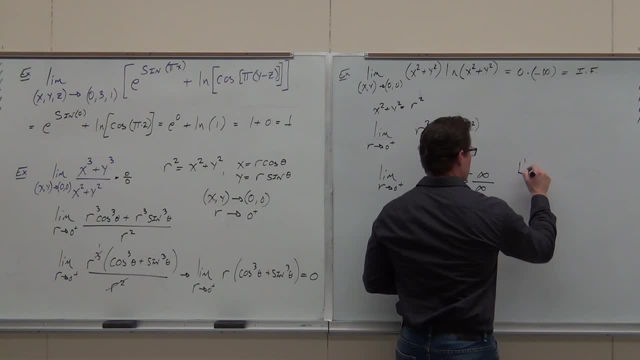 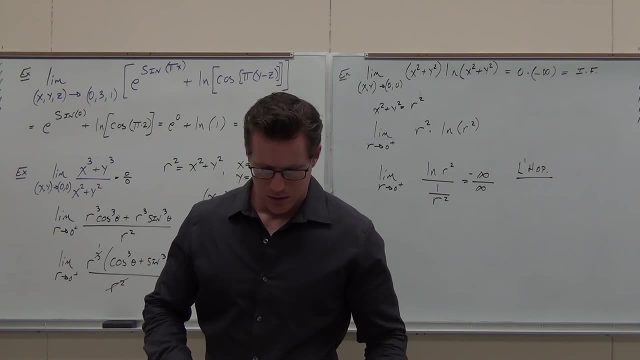 I want you to finish it. Try L'Hopital here. So kind of a cool idea. I hope you like this idea. I like it. It's going to be the first time I saw it. I thought it was pretty neat. 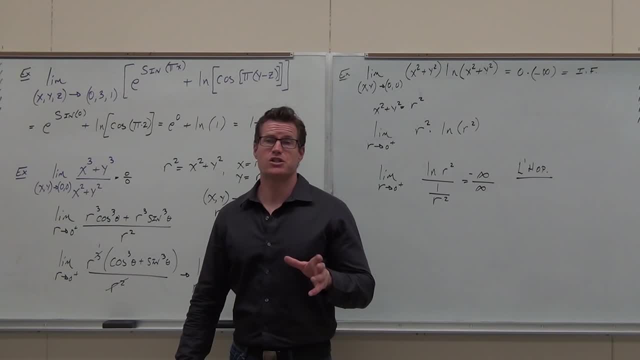 You go. what do I just do with this? I don't know. Give up. No, Let's try to change it to polar. Let's make x squared plus y squared equal r squared. We've got some substitution for x and y. Same thing here. 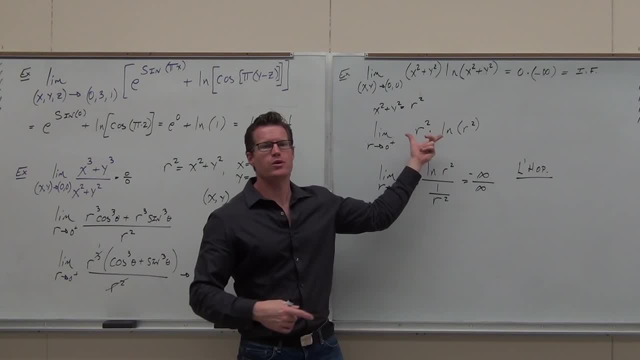 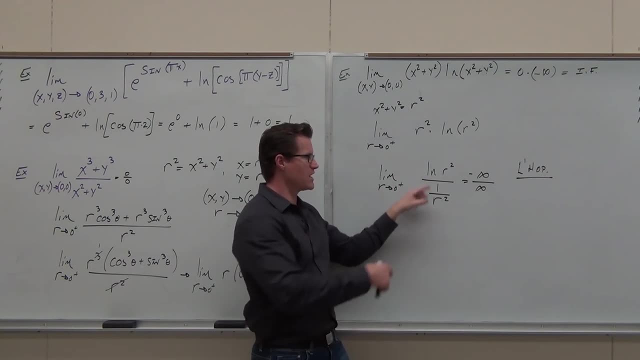 As soon as we do that, even if we have indeterminate forms, you know what to do with one variable. You can start creating from 0 times infinity. infinity over change. it make a fraction over infinity, and then L'Hopital's. 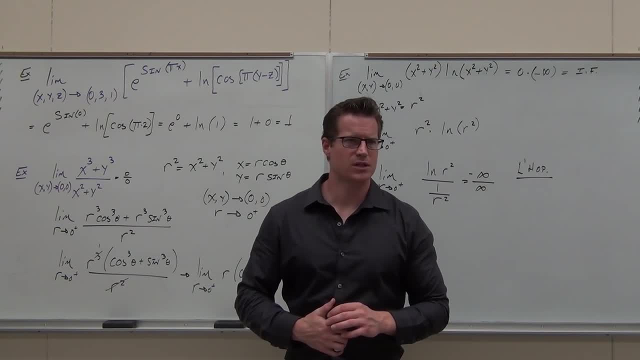 Head on, if you're okay with that. one for real Comments questions, comments, No Comments questions, anything. I can't help you if you don't ask Yeah, Okay, Anybody else Yeah. How do you get one over an R-discord? 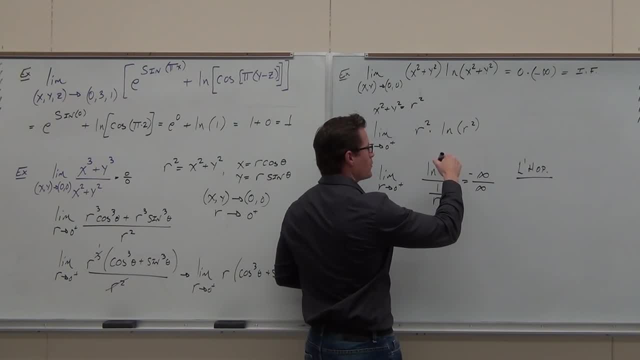 You force this thing down to a denominator. You force it, So you go. well, where do I want that? I want to create this, So forcing it to get the indeterminate form. It's already in the indeterminate form. What you're forcing it to be is: 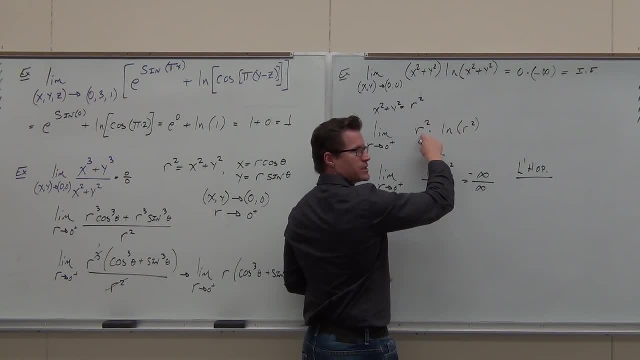 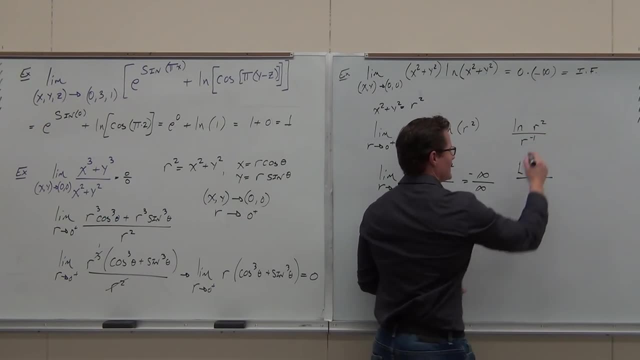 Is a form that allows L'Hopital's. So you go. how do I move this to a denominator? Well, you could do R to the negative 2. That forces it right. 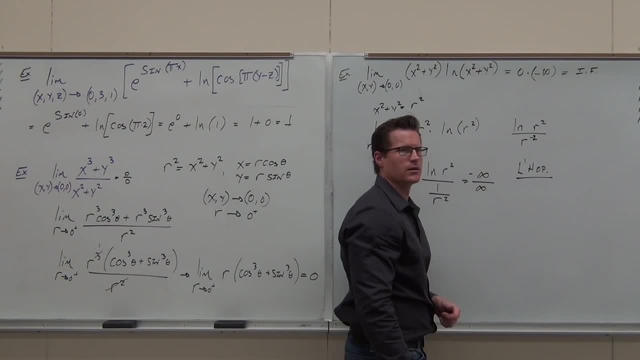 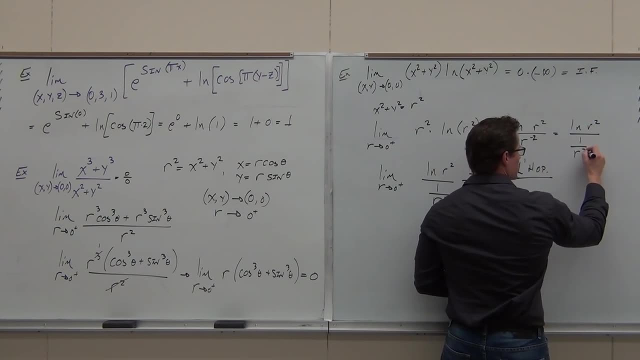 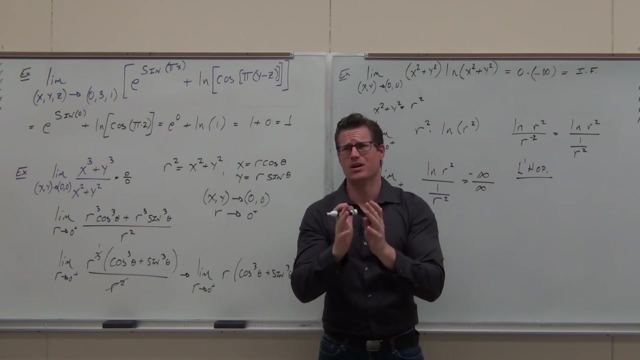 Yep, Yes, There's no negative exponent. Well, what is R to the negative 2?? Well, it's actually a complex fraction that you got. Now it's infinity over infinity. You can't do anything with this. Please, I'm begging you, don't go zero times infinity zero. 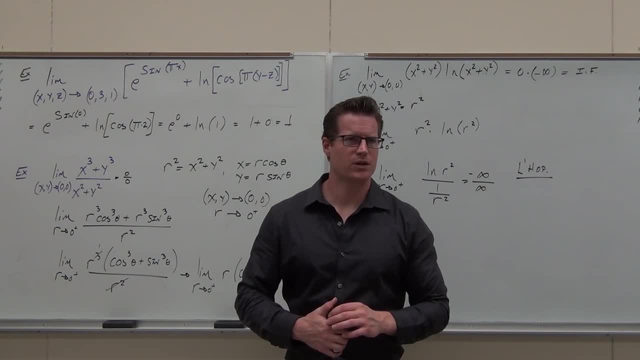 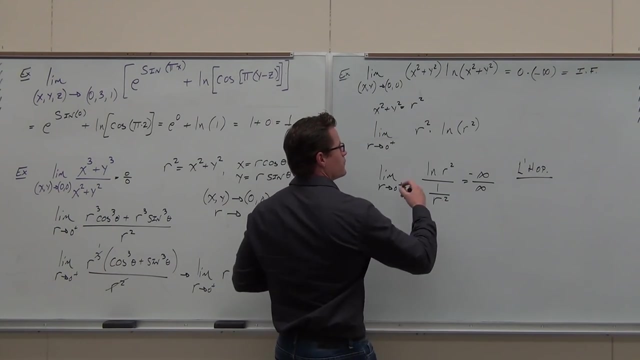 Head on, if you're okay with that one, for real Comments, questions, anything. I can't help you if you don't ask, yeah, Okay, Anybody else, Yeah. How do you get one over r squared? You force this thing down to a denominator. 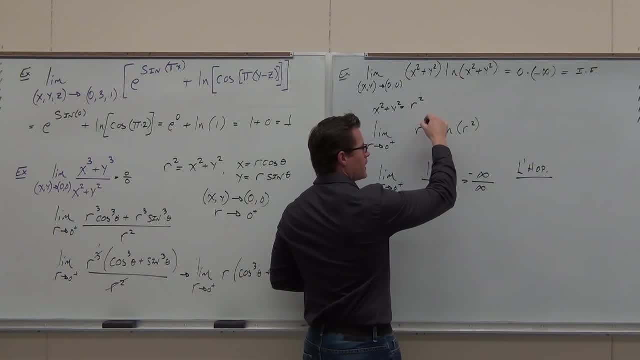 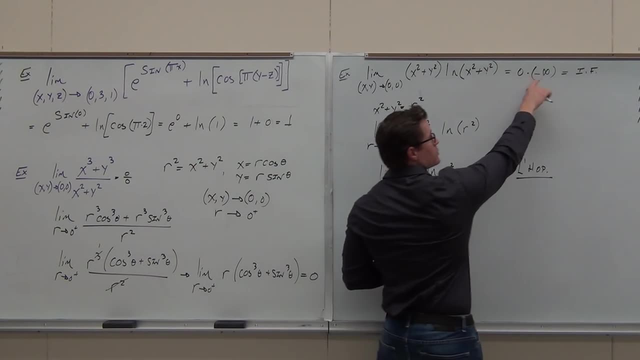 You force it, So you go. well, where do I want that? I want to create this, So you're forcing it to get the indeterminate form. It's already an indeterminate form. What you're forcing it to be is a form. 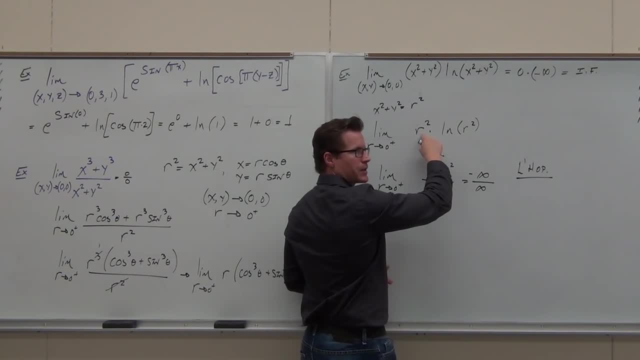 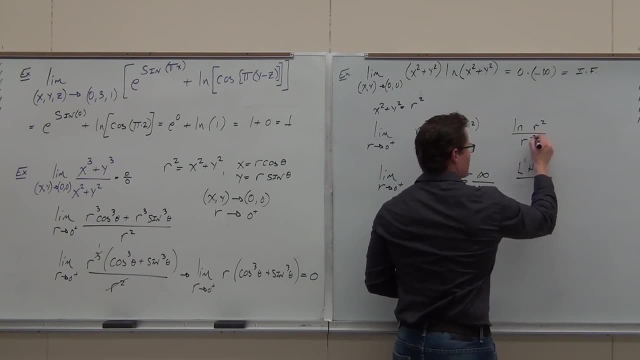 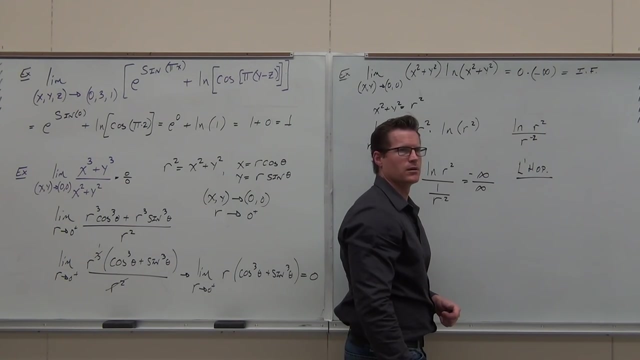 that allows L'Hopital's. So you go: how do I move this to a denominator? Well, you could do r to the negative 2.. That forces it right. Yeah, You guys know about negative exponents. Well, what is r to the negative 2?? 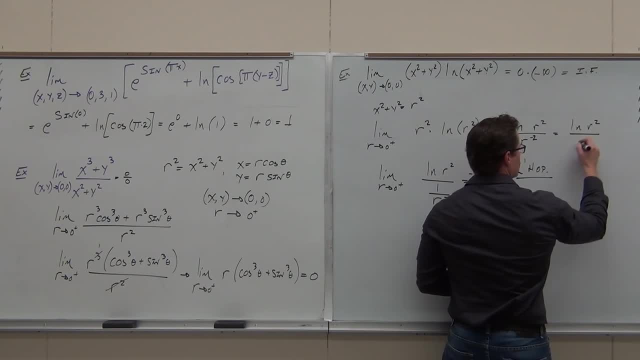 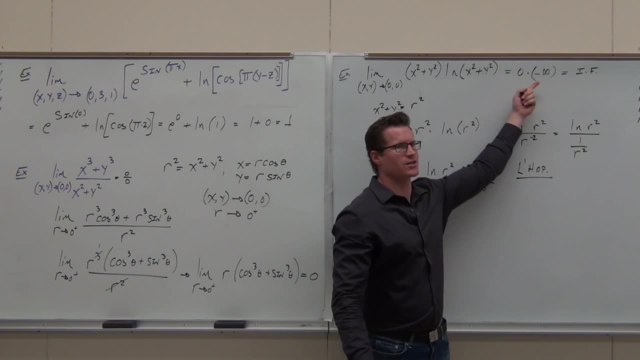 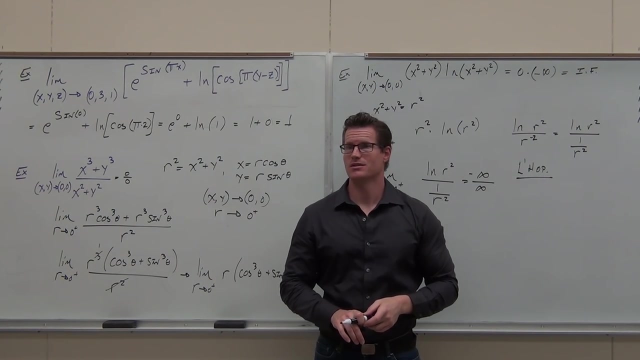 Well, it's actually a complex fraction. Now you got it. Now it's infinity over infinity. You can't do anything with this. Please, I'm begging you, Don't go zero times, infinity, Zero. Sometimes That's D for done, right there, though. 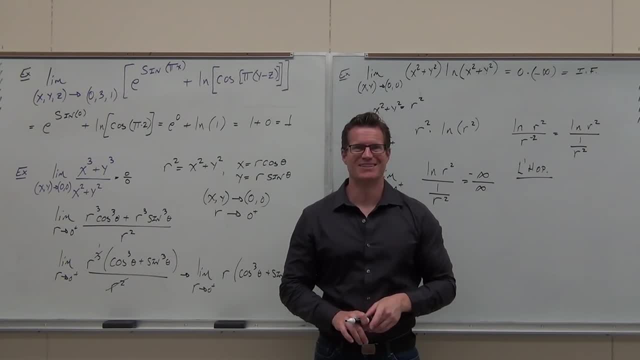 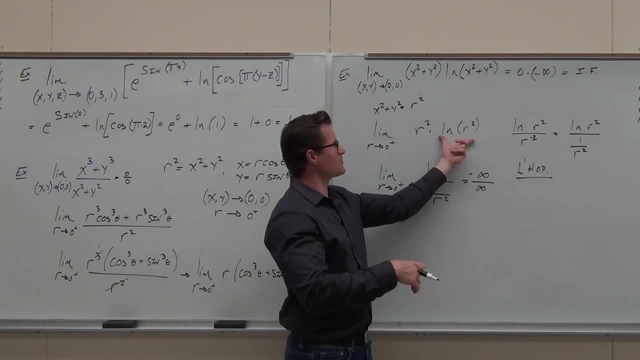 Sometimes that's D for done right there, though, You've heard that. okay, Sometimes, sometimes not, You've got to work with it. So you create this and you go, hey, let's make it zero times infinity. No, Let's make it infinity over one times zero. 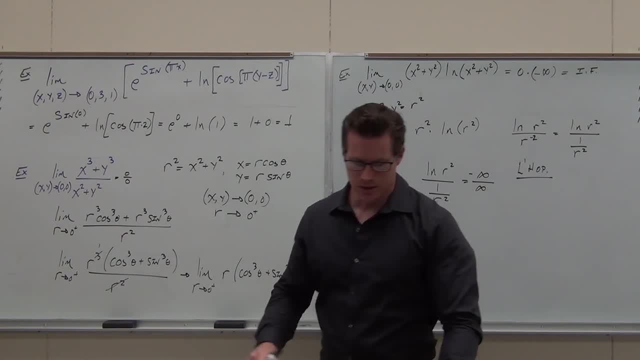 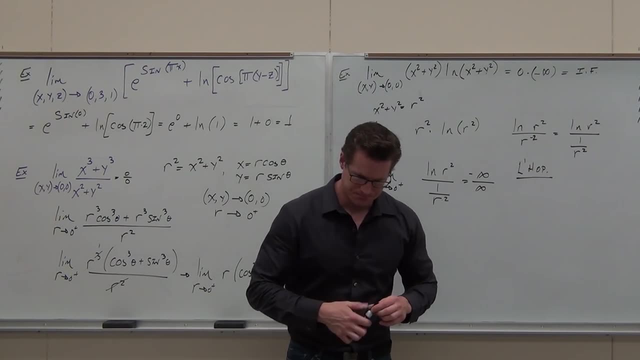 That's infinity, infinity, over infinity, and then L'Hopital's. Okay, we've got to get on with this stuff. We're going to talk about continuity right now. Listen, here's the rundown on continuity. A function's continuous on a region. 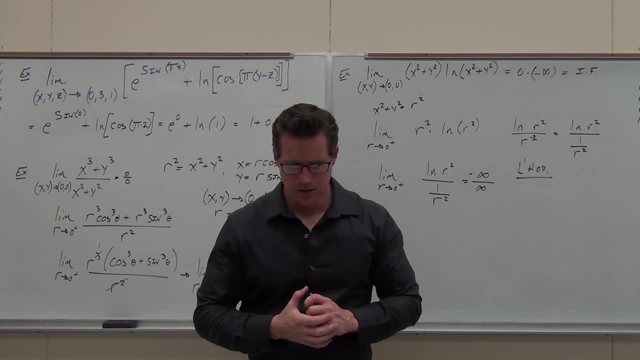 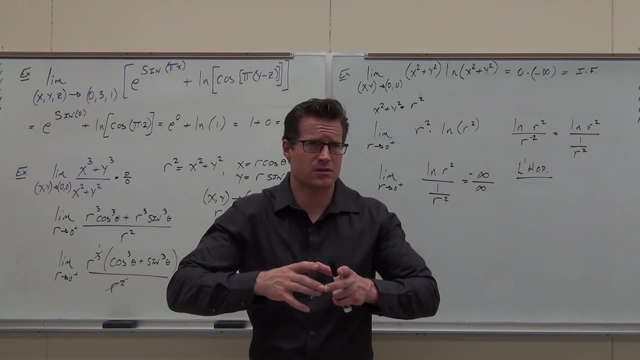 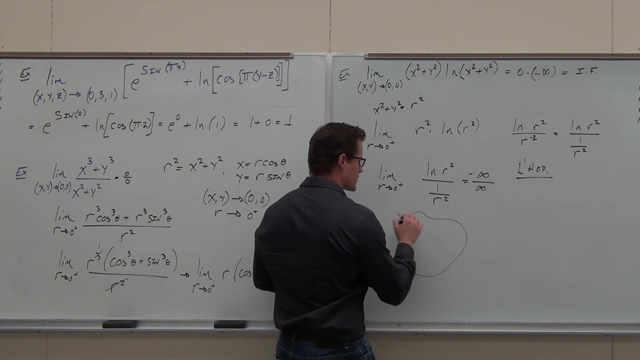 If at each point in the region we can find this little neighborhood around it where we don't have any gaps, jumps or boundaries. So basically they say, if we have this point on the interior of a region, You don't have to do that. 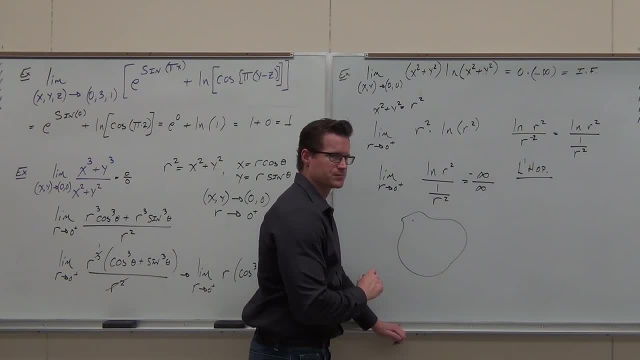 You don't have to do that, You don't have to draw this. I'm just going to explain it real quick. But if you have a point on the interior of a region, you can always draw a little neighborhood, neighborhood, delta A little, that just means a little neighborhood, okay. 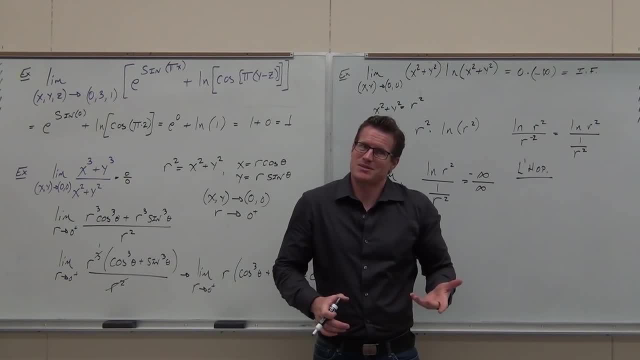 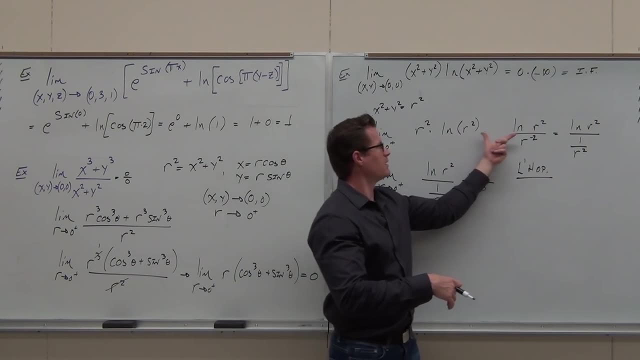 You heard that, Okay, Sometimes, Sometimes not. You got to work with it. So you create this and you go: hey, let's make it zero times infinity. No, Let's make it infinity over one times zero. That's infinity. 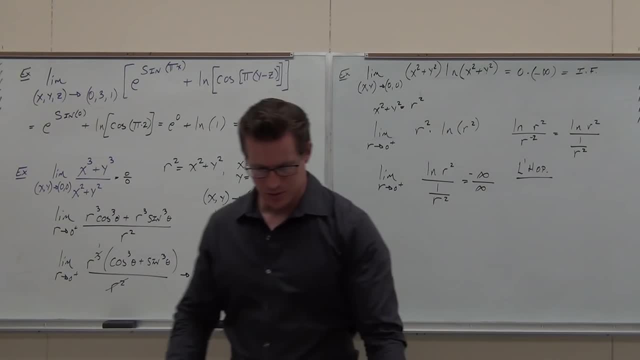 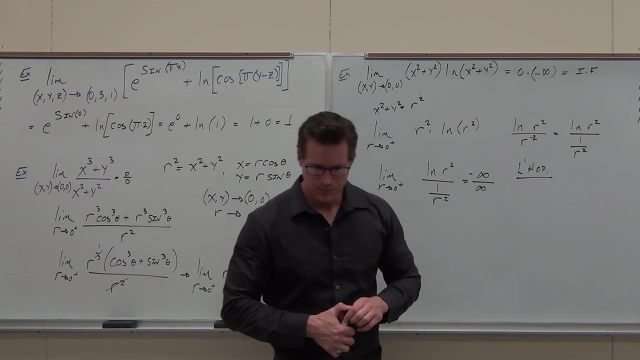 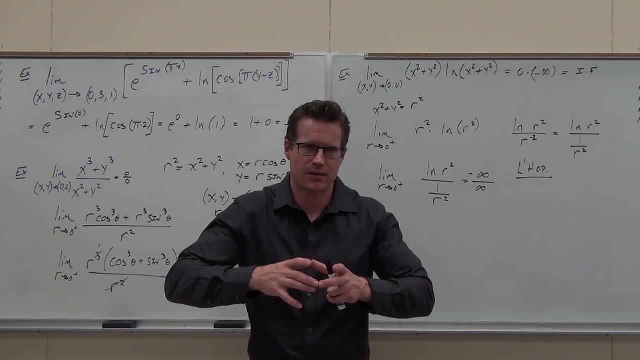 Infinity over infinity, And then L'Hopital's: Okay, We got to get on with this stuff. We're going to talk about continuity right now. Listen, here's the rundown on continuity. It functions continuous on a region If at each point in the region, we can find this little neighborhood around it. 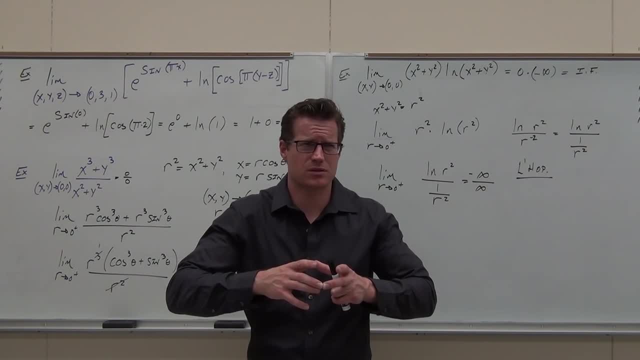 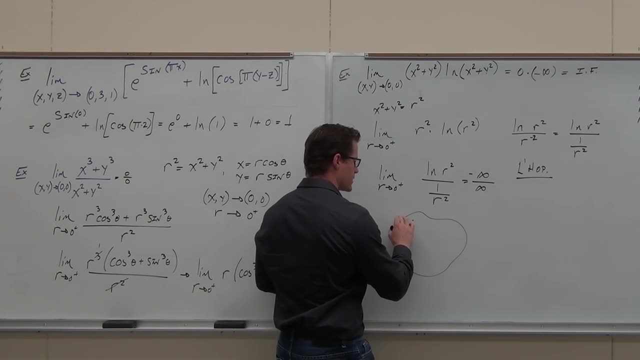 where we don't have any gaps, jumps or boundaries. So basically, let me say, if we have this point on the interior of a region, You don't have to draw this. I'm just going to explain it real quick. But if you have a point on the interior of a region, 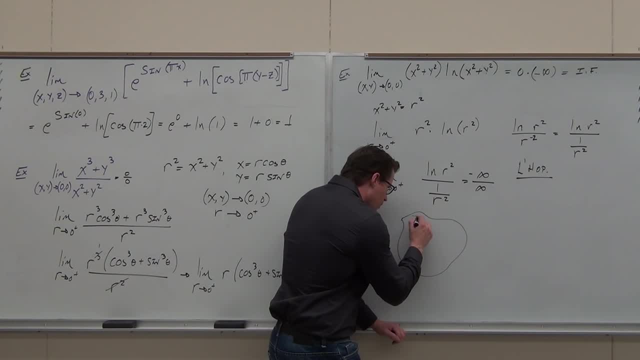 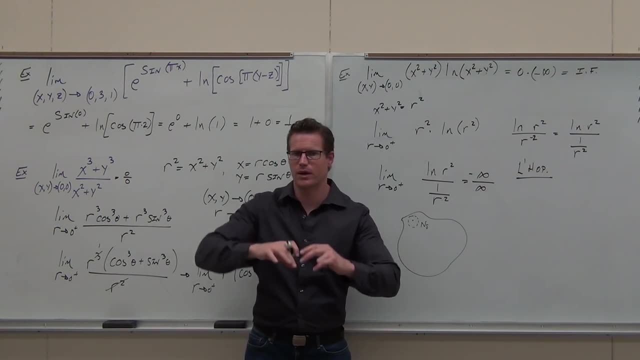 you can always draw a little neighborhood, neighborhood delta A little. that just means a little neighborhood, okay, Just a little circle around it, And even if you get really super teeny close, you could still draw a little teeny circle around that. 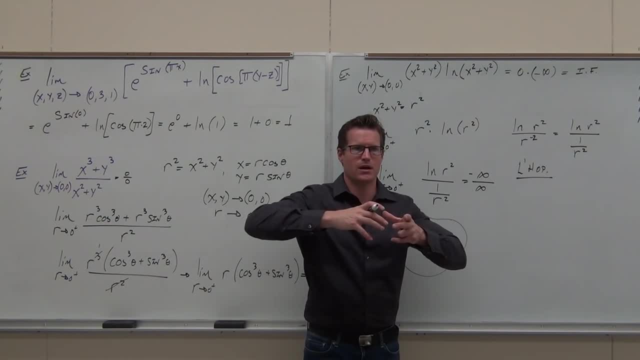 Does that make sense to you? You can define some points around it, which means that at that point that we can draw this neighborhood around. we can get to that point no matter what path. That means that we're continuous on that surface, over that region. 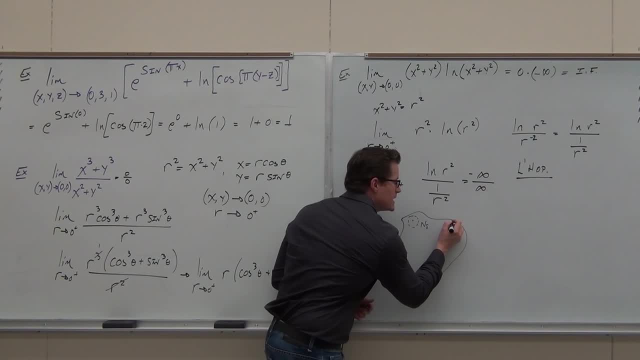 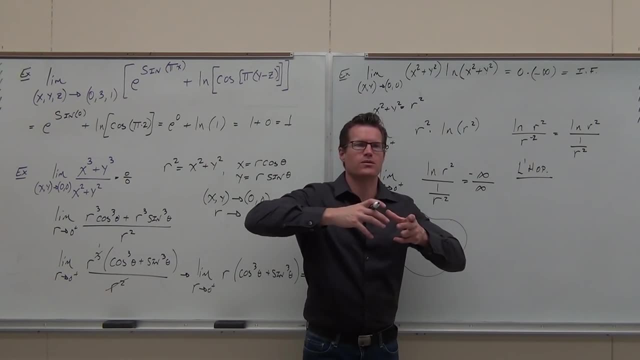 Just a little circle around it And even if you get really super teeny close, you could still draw a little teeny circle around that. Does that make sense to you? You can define some points around it, which means that at that point that we can draw this neighborhood around, we can get. 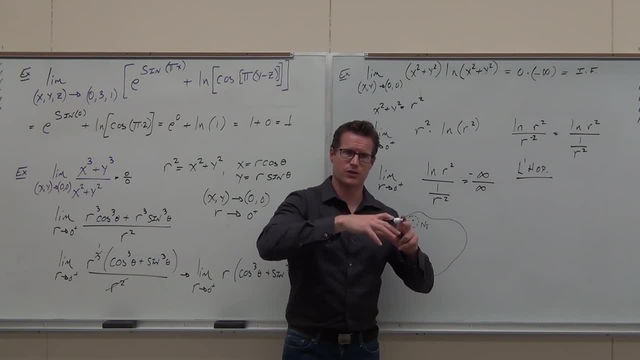 to that point, no matter what path. That means that we're continuous on that surface, over that region, On boundary points. so if you're actually on there, you go. well, this looks pretty good, but these points out here don't look so hot. 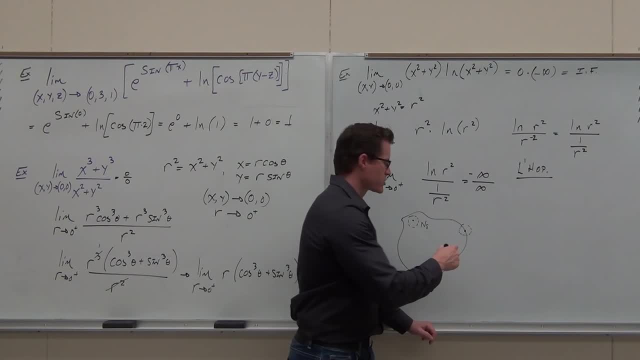 In that case we say: you know what? we're going to restrict our paths. Just restrict our paths to all paths that come from the inside, sorry, inside the neighborhood. like this, We say paths outside, don't worry about those paths outside. 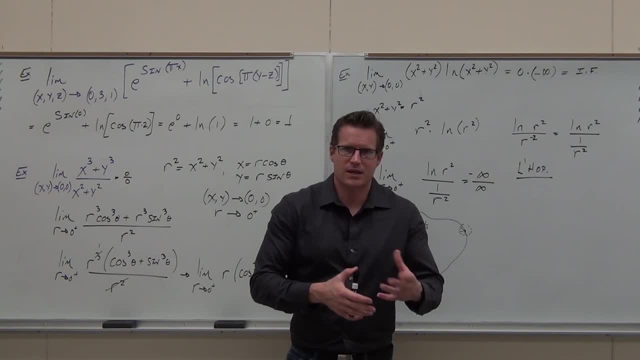 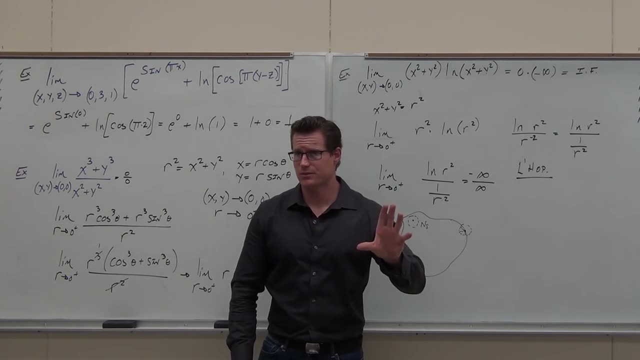 So boundary points, boundary points are okay As long as we restrict our paths. All this basically says- I know I'm going speeding through it because it matters- it does matter, But it's easier than some of these definitions make it. Here's what this says: 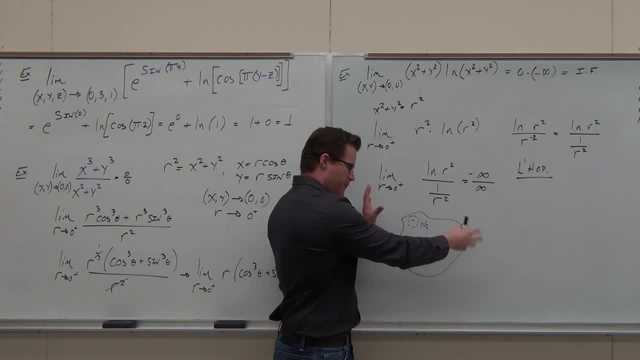 If you have a region, you have a function that's defined over this region. it's going to be continuous at any point in that region. Why? Because you draw a little circle around it. that's continuous within that circle. That's why. 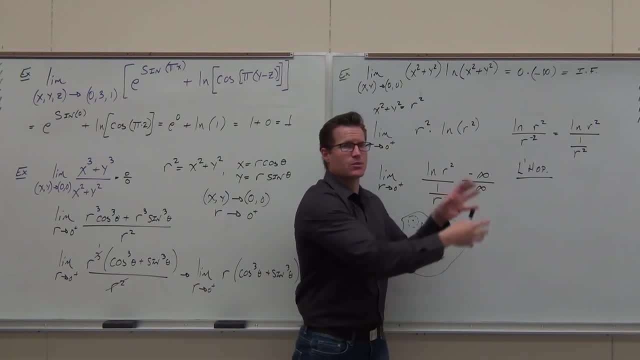 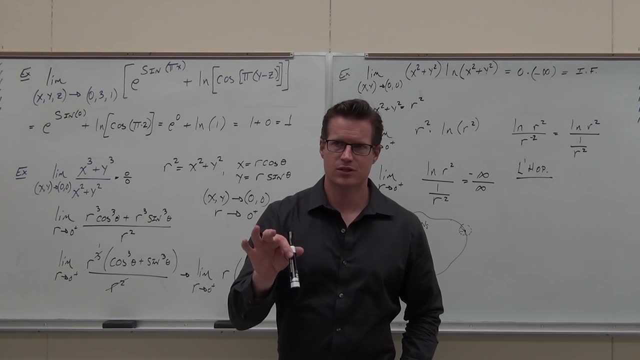 On the boundary, you're still fine because you can find some paths from inside the region that get there. In other words, all of this stuff says the following: A function is continuous at any point inside of its domain. That's all it says. 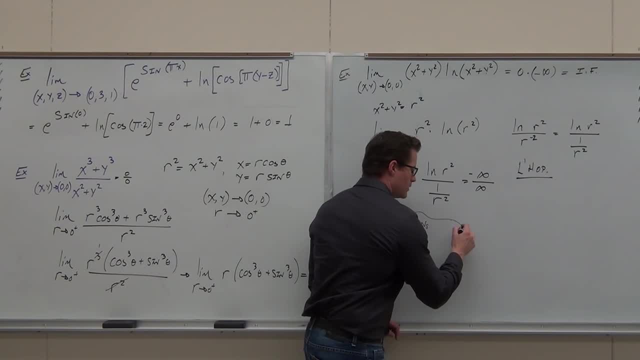 On boundary points. so if you're actually on there, you go. well, this looks pretty good, but these points out here don't look so hot. In that case we say: you know what? we're going to restrict our paths. 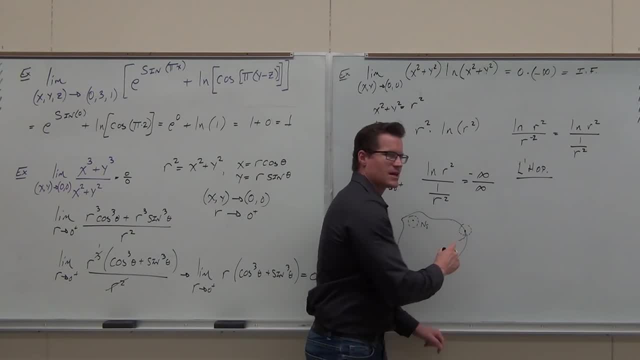 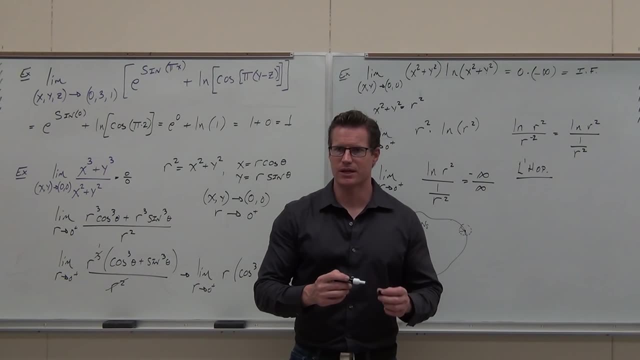 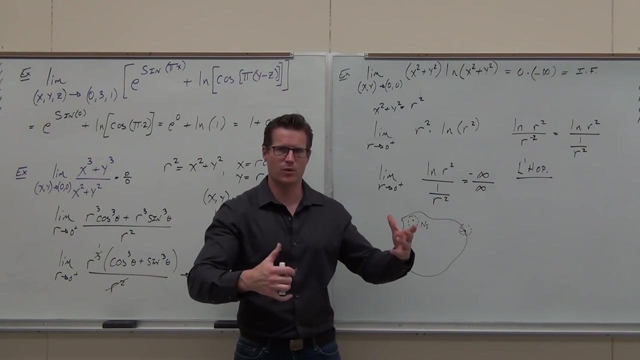 Just restrict our paths to all paths that come from the inside, sorry, inside the neighborhood, like this: When we say paths outside, don't worry about those paths outside. So boundary points are okay as long as we restrict our paths. All this basically says I know I'm going speeding through it. 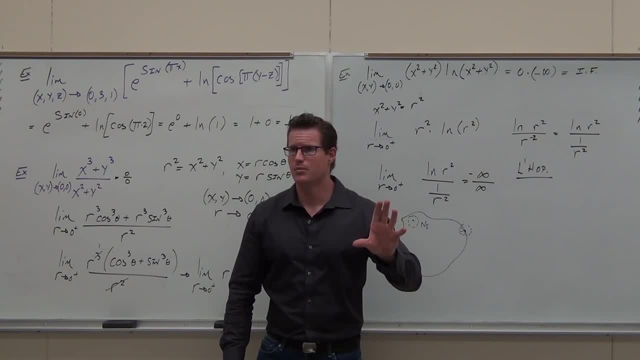 because it matters. it does matter, but it's easier than some of these definitions make it. Here's what this says: If you have a region, you have a function that's defined over this region. it's going to be continuous at any point in that region. 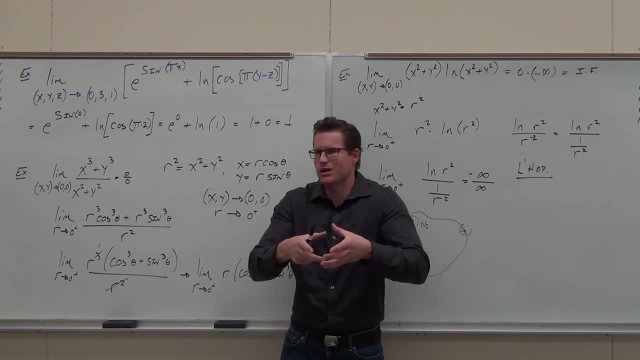 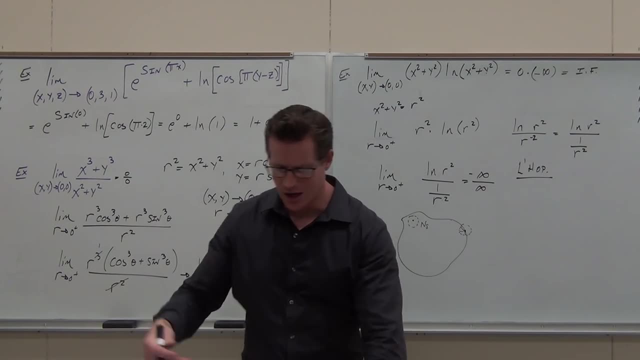 Why? Because you draw a little circle around it that's continuous within that circle. That's why On the boundary you're still fine, because you can find some paths from inside the region that get there. In other words, all of this stuff says the following: 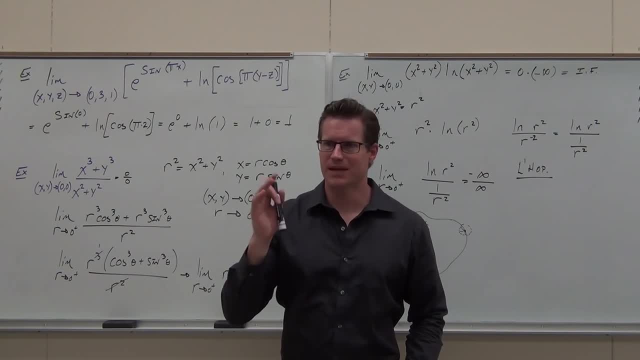 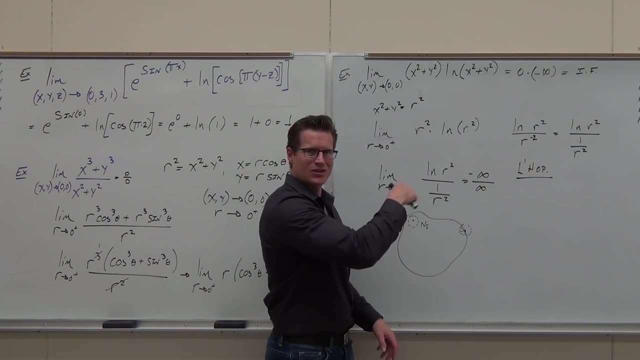 A function is continuous at any point inside of its domain. That's all it says. Here's a domain, Here's a point: Continuous. Draw a little neighborhood around there. All the paths go to that point. Well, to get to that point, by any path, it's going to be there. 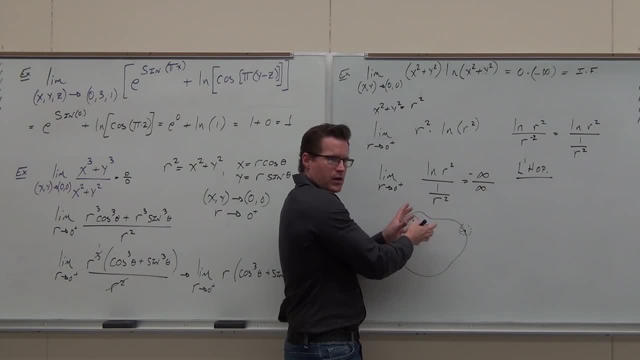 There's no jumps, There's no gaps, There's no asymptotes. There's nothing wrong in that if we're completely defined in that domain. Same thing on the boundary: There's no jumps or gaps within this part of it. We can find continuity there. 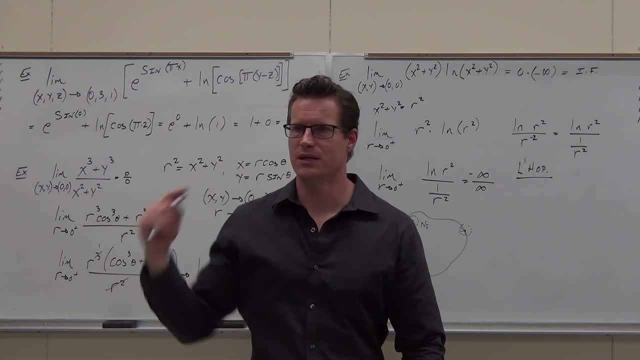 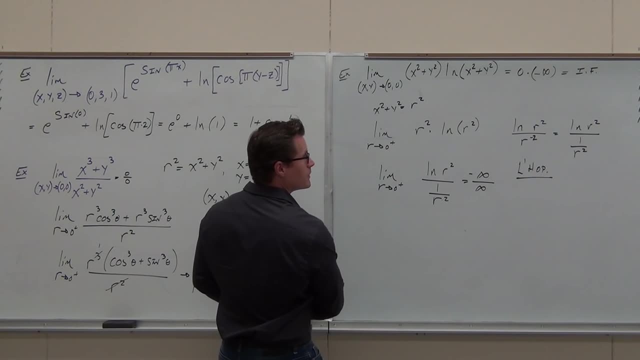 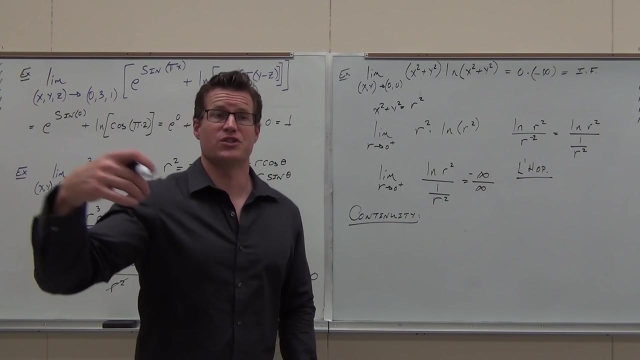 All it says is that a function is continuous at any point inside the domain. That's what I want you to write down right now. So, as far as continuity goes, a function is continuous at any point inside the region for which it's defined. 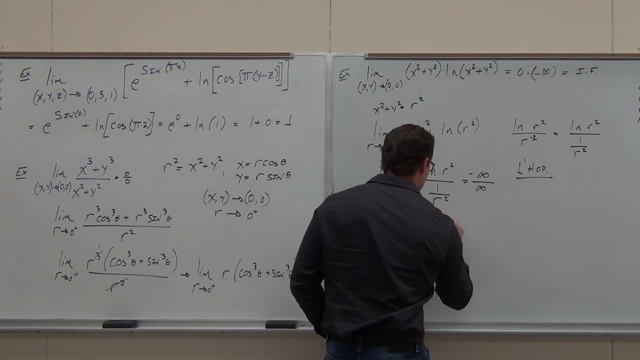 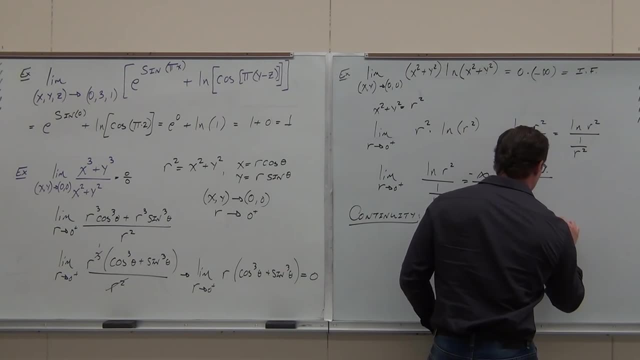 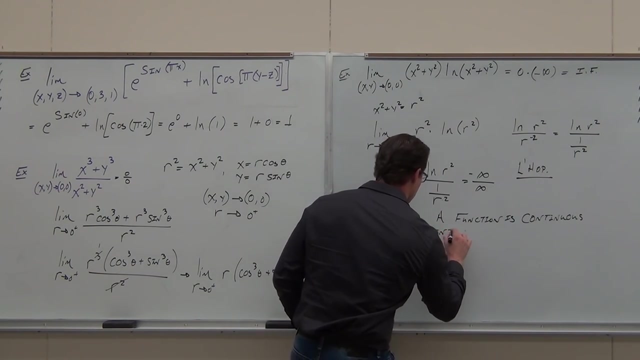 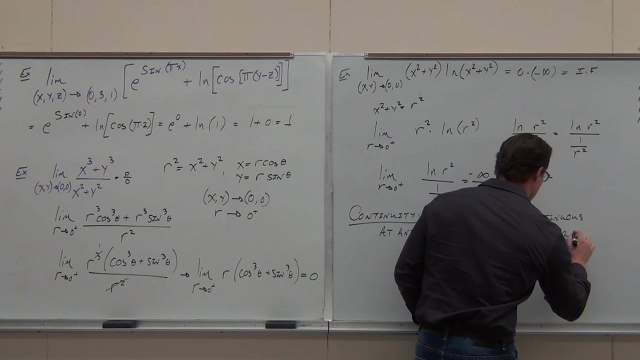 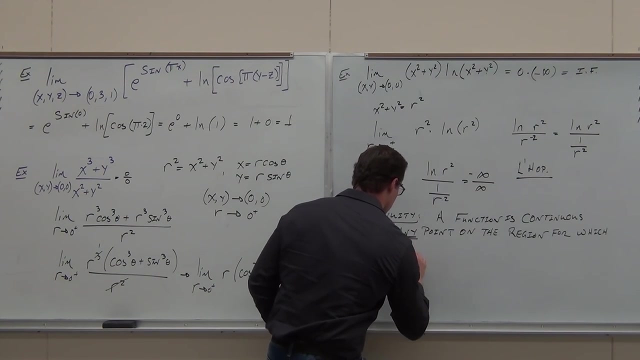 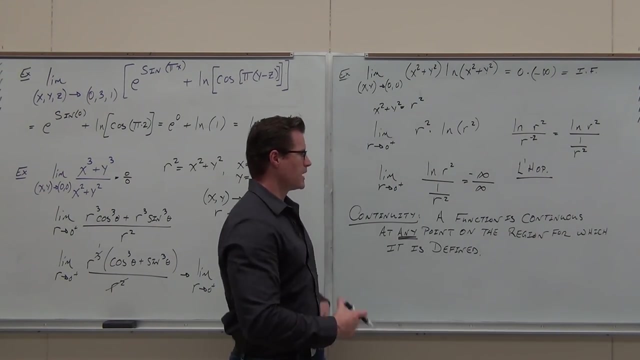 Domain. Well, how do we define the regions? Well, how do we do that? On what regions are functions defined? We already did that. It's called the domain. Find the domain, You find out where the function is continuous. Do you remember that? back from Calc 1 when you're like. 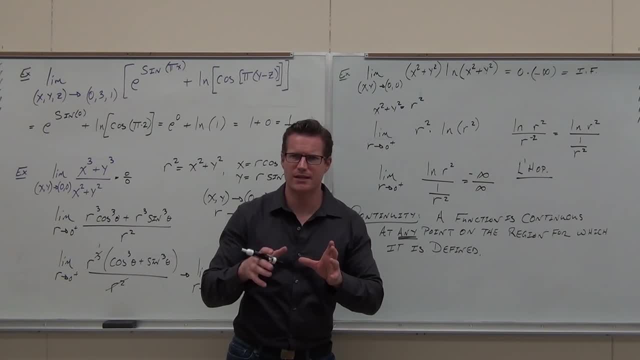 wait a minute- finding continuity issues. Remember the holes and asymptotes from Calc 1? You watched them on the videos. You probably saw that. But where we found discontinuities were exactly where we found domain issues. They were basically one and the same until we started restricting our domain. 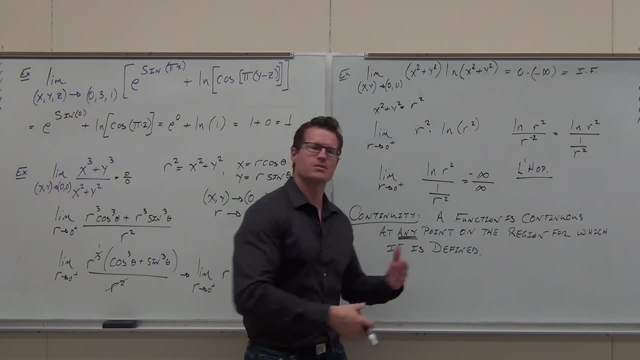 If we don't restrict the domain, domain and continuity give you the same region, And that's what I'm saying here. I'm saying that a function is continuous at any point on the region for which it's defined. The region for which a function is defined is defined to be the domain. 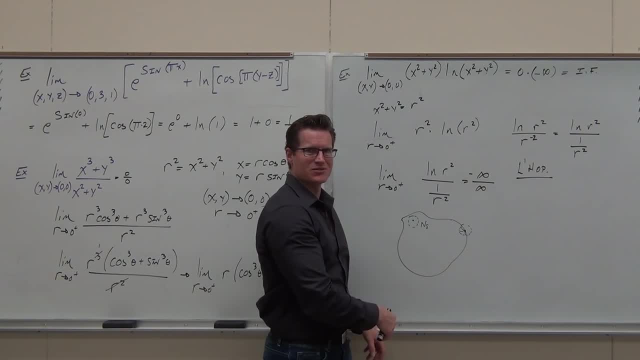 Here's a domain, Here's a point, Continuous Throw a little neighborhood around there. All the paths go to that point, No problem. Well, to get to that point by any path it's going to be. there's no jumps, there's no gaps, there's no asymptotes. 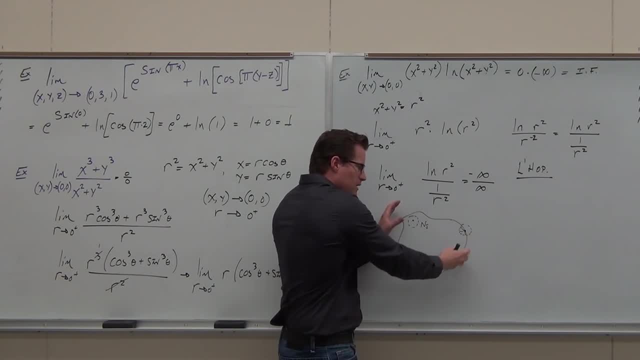 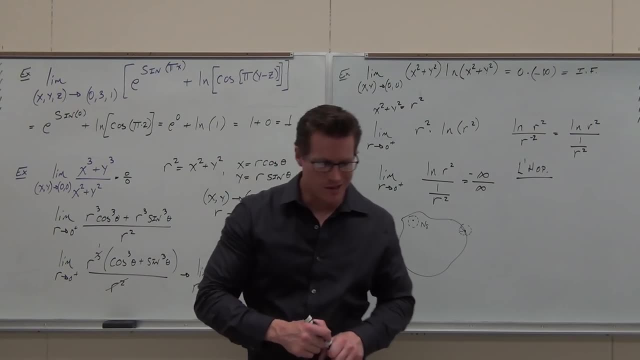 there's nothing wrong in that, If we're Okay, Completely define that domain. Same thing on the boundary. There's no jumps or gaps within this part of it. We can find continuity there. All it says is that a function is continuous. 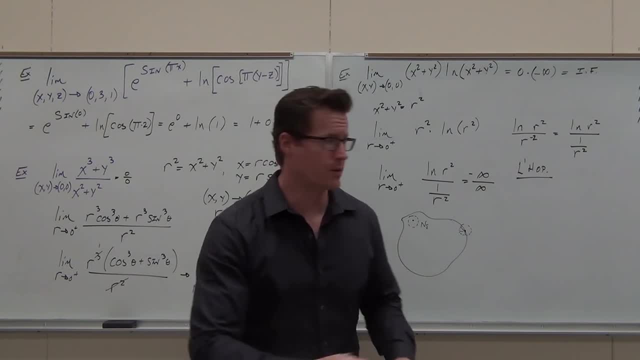 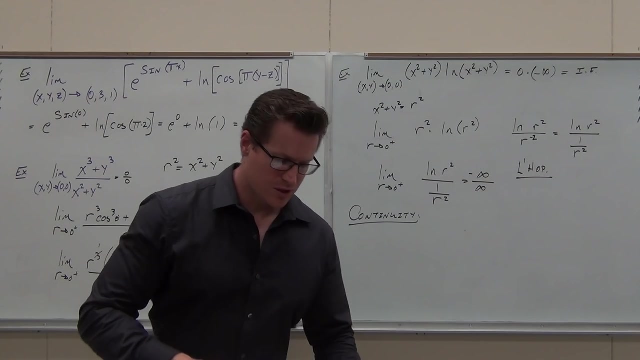 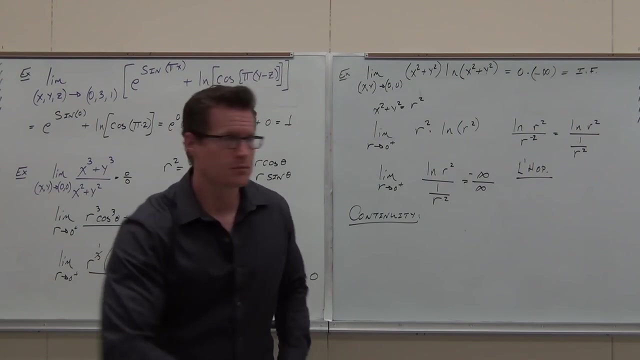 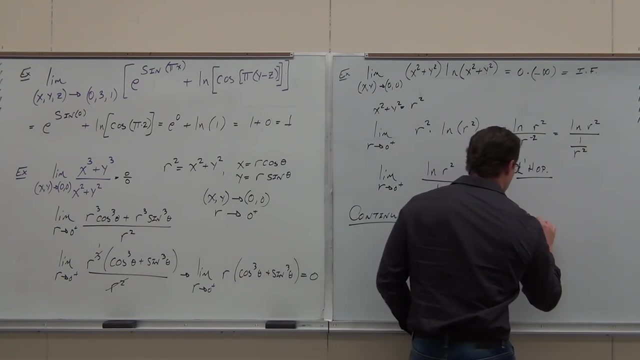 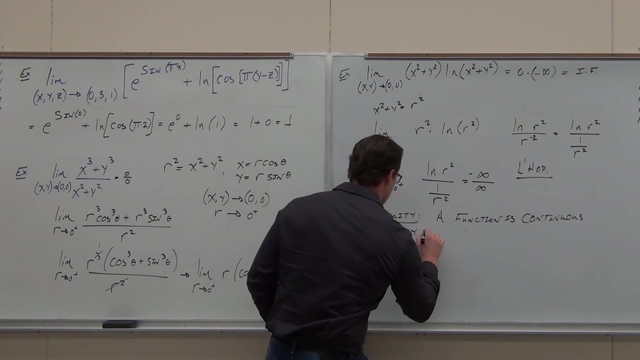 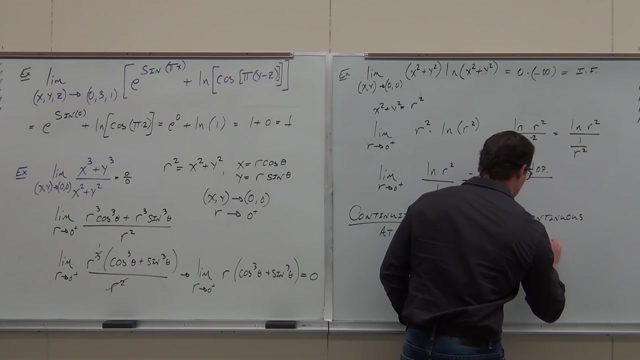 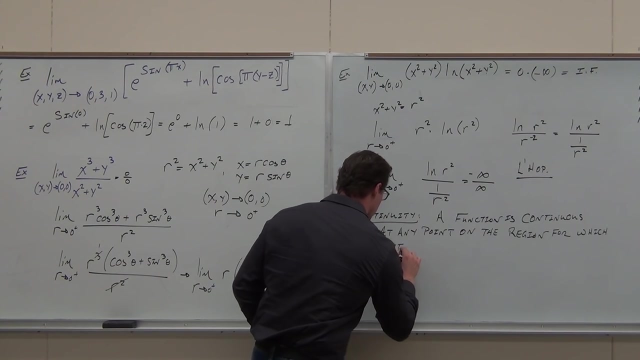 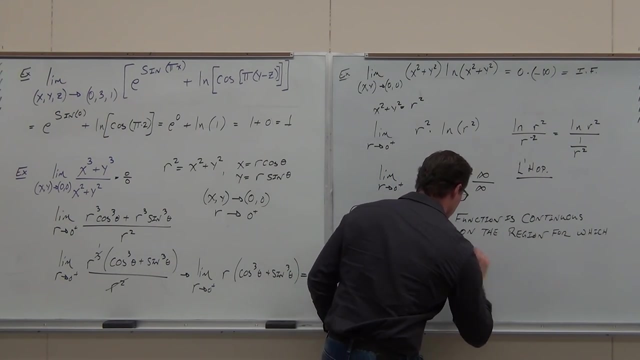 at any point inside the domain. That's what I want you to write down right now. So, as far as continuity goes, A function is continuous at any point inside the region for which it's defined Domain. Well, how do we define the regions? 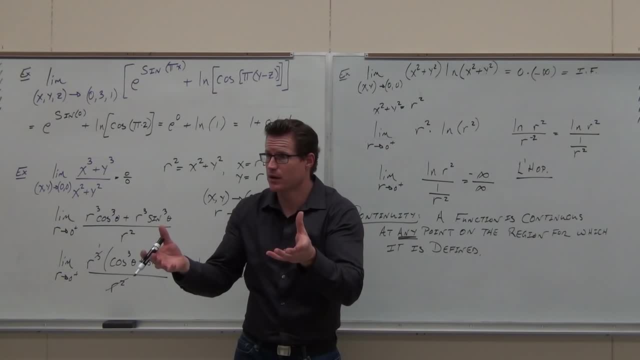 Well, how do we do that? On what regions are functions defined? We already did that. It's called the domain. Find the domain. You find out where the function is continuous. Do you remember that? back from Calc 1 when you're like: 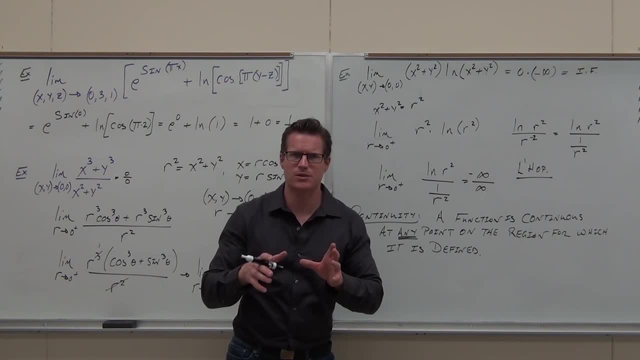 wait a minute- finding continuity issues. Remember the holes and asymptotes from Calc 1? You watched them on the videos. You probably saw that. But where we found discontinuities were exactly where we found domain issues. They were basically one and the same. 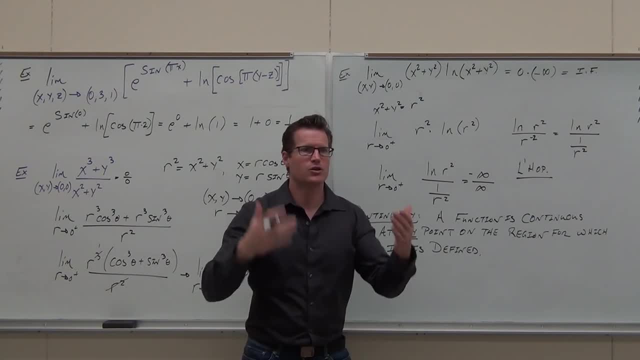 until we started restricting our domain. If we don't restrict the domain, domain and continuity give you the same region, And that's what I'm saying here. I'm saying that a function is continuous at any point on the region for which it's defined. 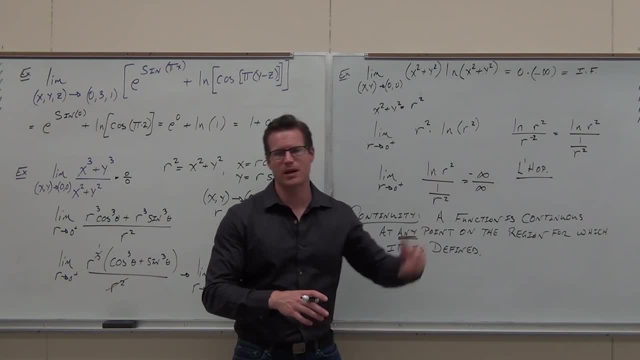 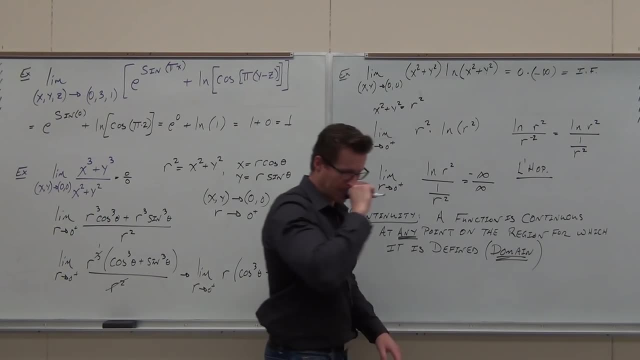 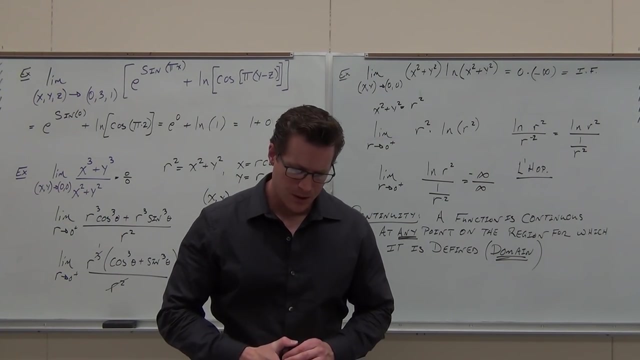 The region for which a function is defined is defined to be the domain. This is domain, And that's kind of beautiful because we get a lot of the continuity properties we had before. They still work. All we have to look for are the same exact things we looked. 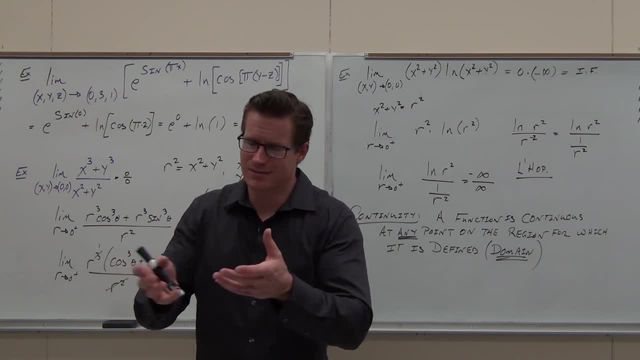 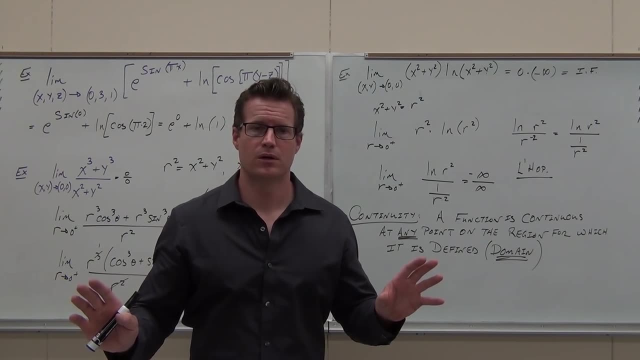 for before holes, these weird things that would be like denominators equal to zero negatives inside square roots. So just look for the same problems we looked for for domain. Does that make sense to you all? Okay, There's a couple things. 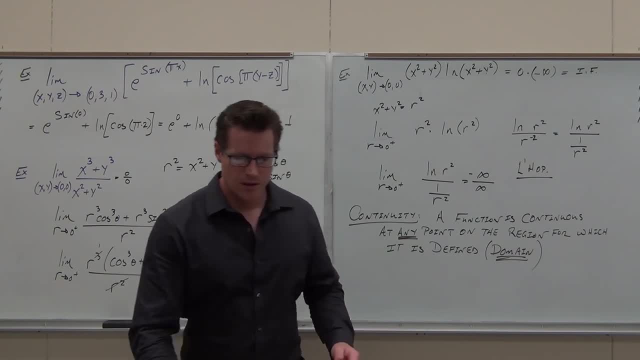 I want you to write down here a couple things that we get to use. the first one: Polynomials are continuous everywhere, Rational functions are continuous everywhere. The denominator is not zero And continuity holds for compositions of continuous functions. So just put: continuity holds for compositions. 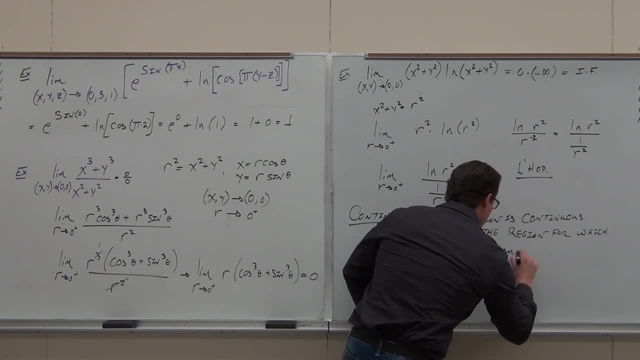 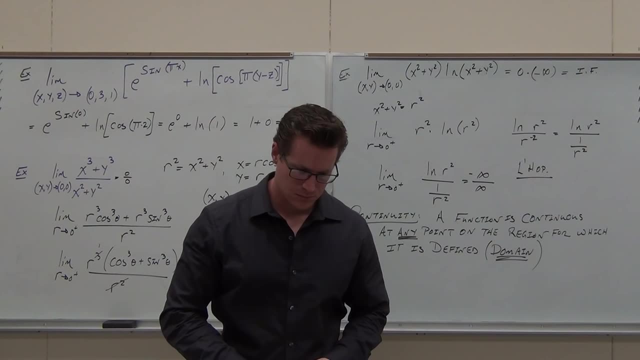 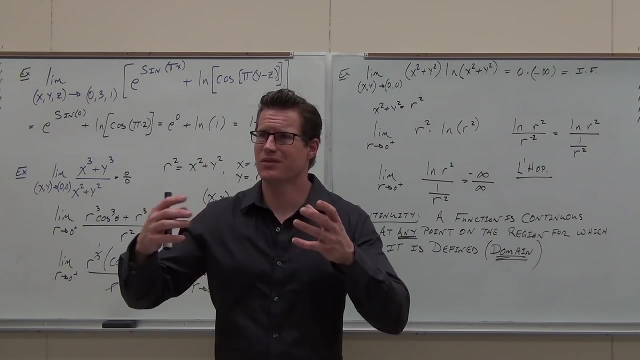 This is domain, And that's kind of beautiful Because we get a lot of the continuity properties we had before. they still work. All we have to look for are the same exact things we looked for before: Holes, these weird things that would be like denominators equal to zero negatives inside square roots. 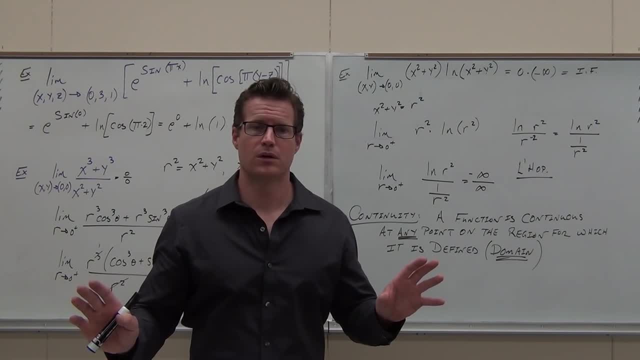 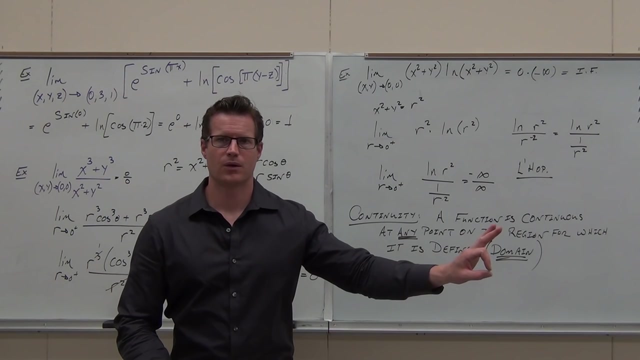 So just look for the same problems we looked for for domain. Does that make sense to y'all? Okay, there's a couple things I want you to write down here, A couple things that we get to use. The first one: polynomials are continuous everywhere. 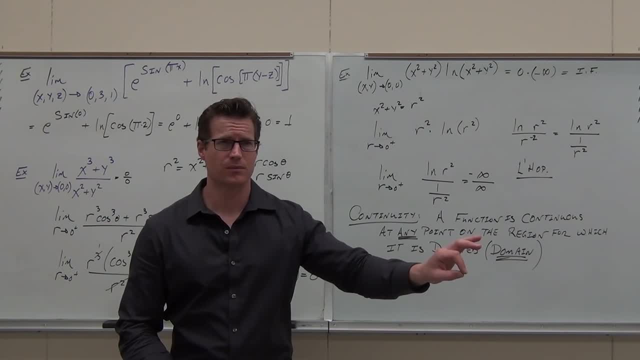 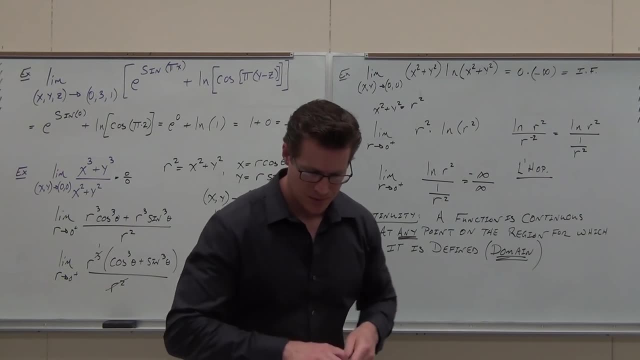 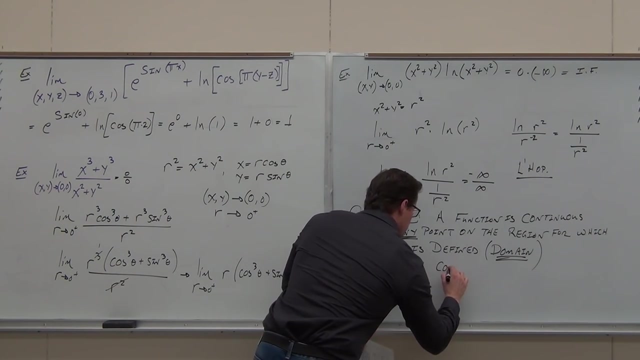 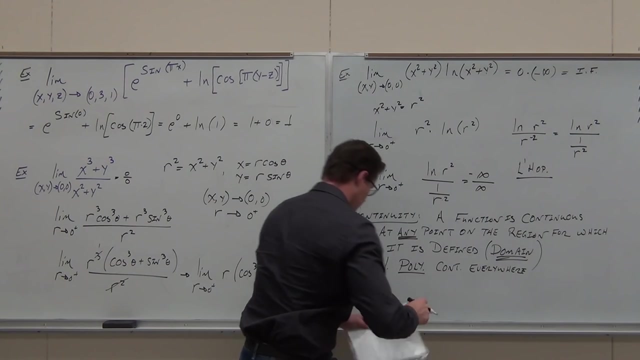 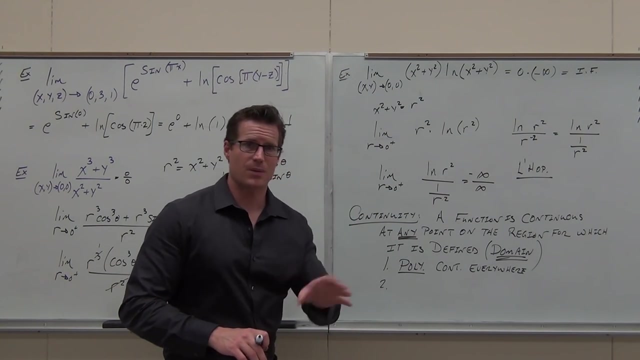 Rational functions are continuous everywhere The denominator is not zero And continuity holds for compositions of continuous functions. So just put: continuity holds for compositions. So those are the three things that I want you to put. Polynomials are continuous everywhere. Rational functions are continuous everywhere where the denominator is not zero. 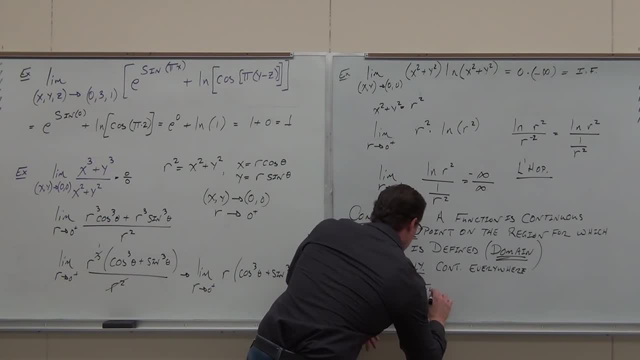 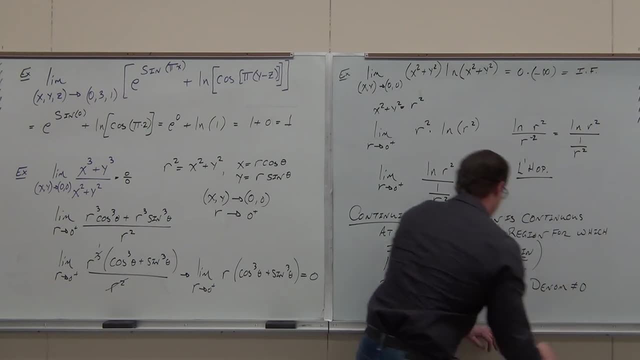 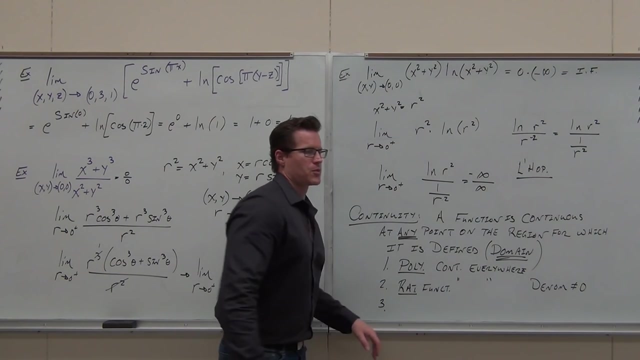 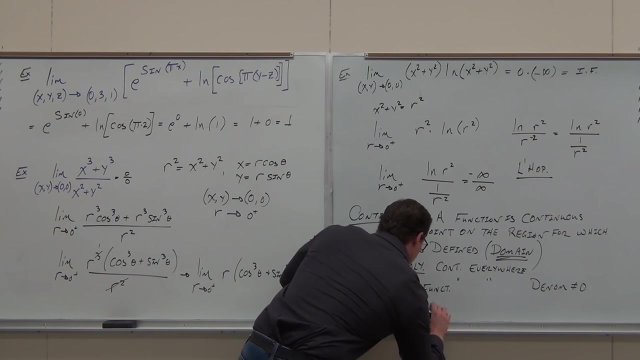 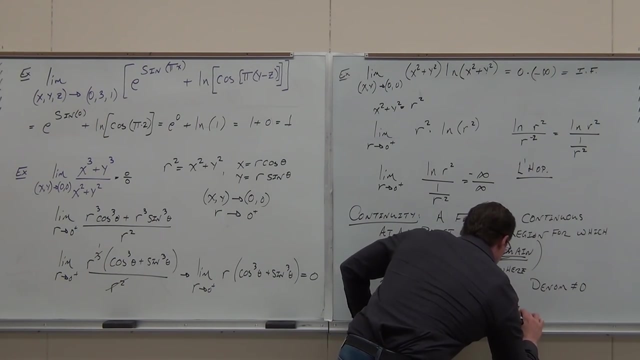 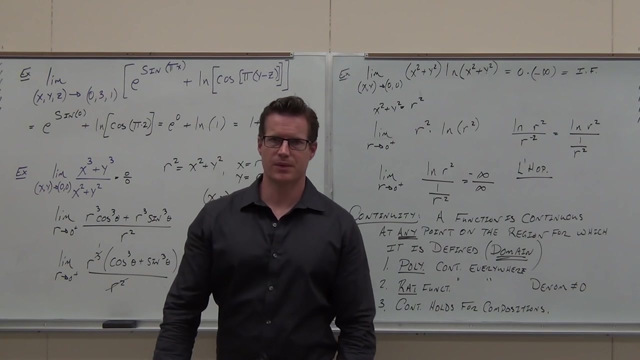 And three continuity holds for compositions of continuous functions. Polynomials are continuous everywhere, Rational functions are continuous everywhere where the denominator is not zero. And three continuity holds for compositions of continuous functions. This last statement is why I can't do the squeeze theorem until like right now. 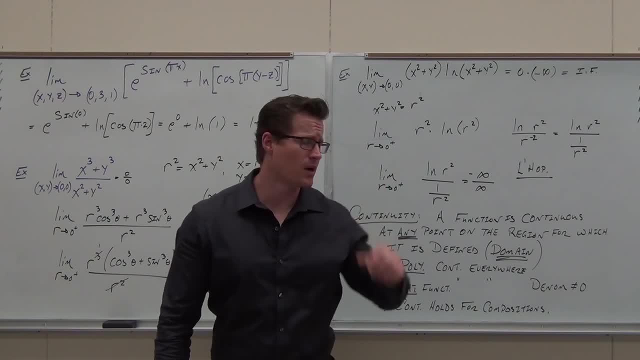 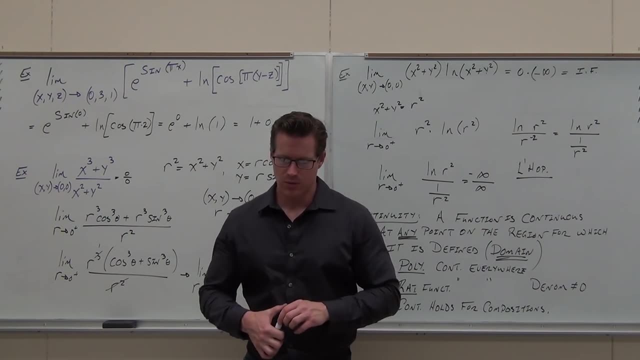 We're going to do some continuity and then we'll talk about squeeze theorem, Because this continuity holds for compositions of continuous functions. I need that to prove it. So we're going to do that in a little bit. Right now I'd like to do one example. 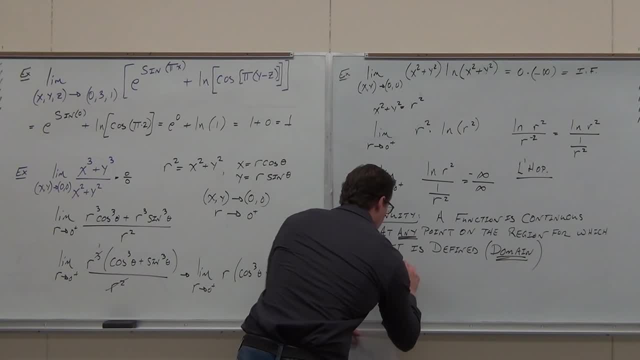 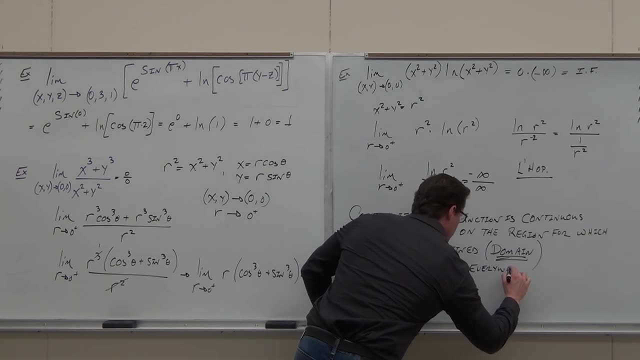 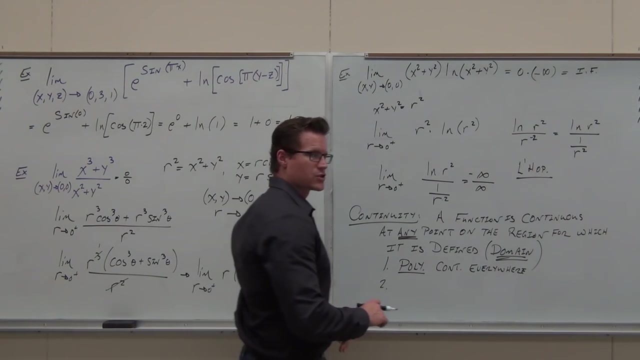 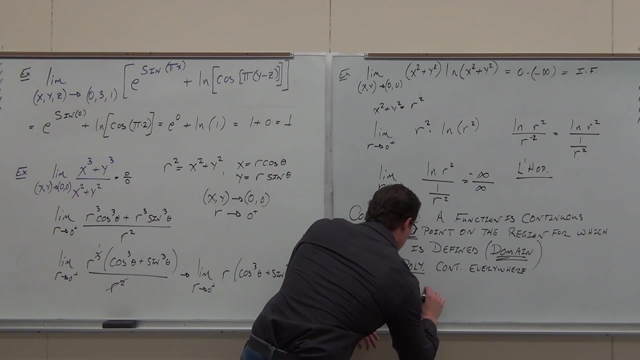 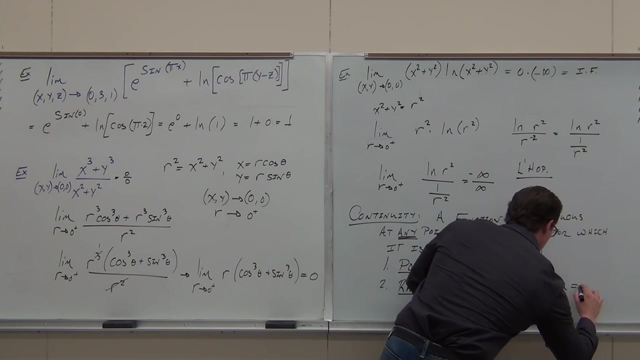 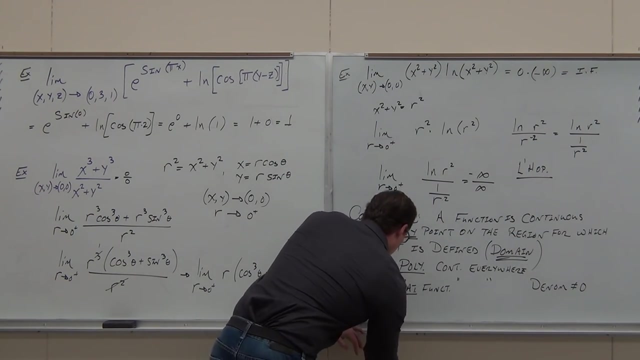 So those are the three things that I want you to put. Polynomials continuous everywhere. Rational functions are continuous everywhere where the denominator is not zero. Polynomials continuous everywhere, Rational functions continuous everywhere The denominator is not zero. And three: 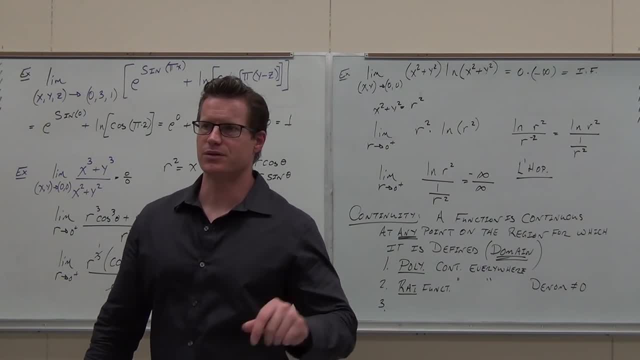 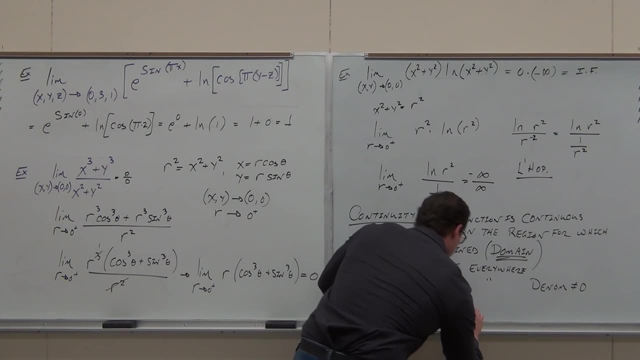 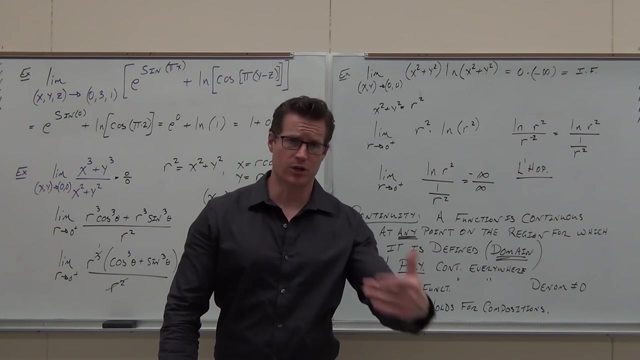 Polynomials are continuous everywhere, Rational functions are continuous everywhere where the denominator is not zero. And three Continuity holds for compositions of continuous functions. This last statement is why I can't do the squeeze theorem until like right now. We're going to do some continuity and then we'll talk about squeeze theorem. 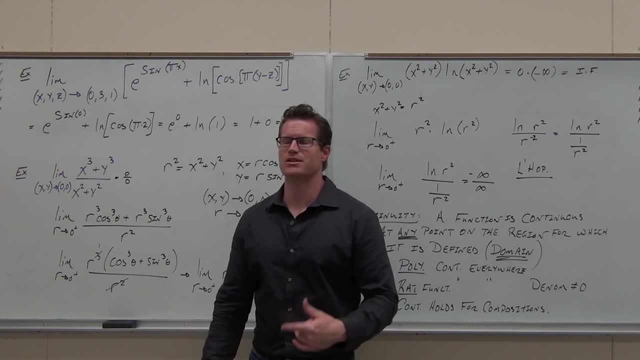 because this continuity holds for compositions of continuous functions. I need that to prove it. So we're going to do that in a little bit. Right now I'd like to do one example, just one. Okay, by one I mean two. 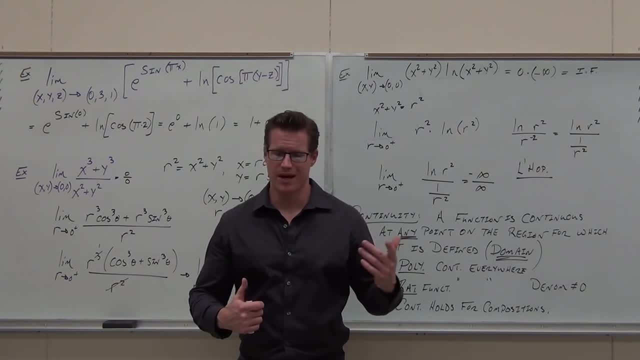 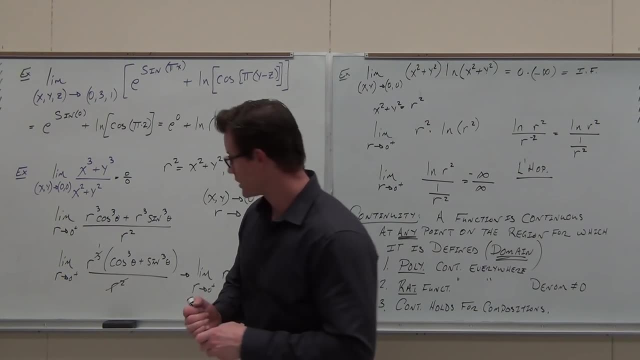 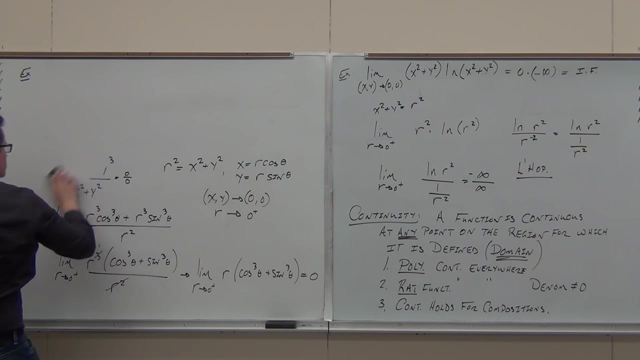 Two examples about continuity. then we'll take a break, We'll come back and maybe do one more. We'll do that squeeze theorem thing, I'll talk about compositions, and that'll be it Pretty close. I do want some more energy out of you guys, though. 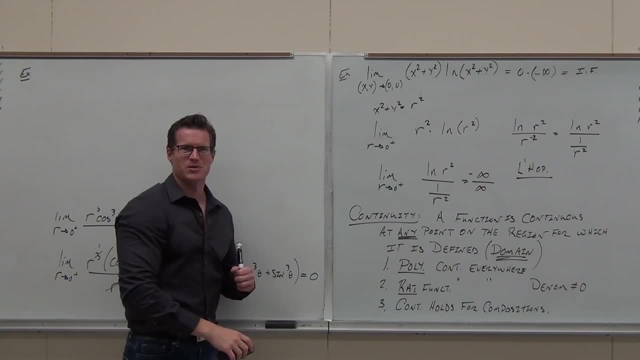 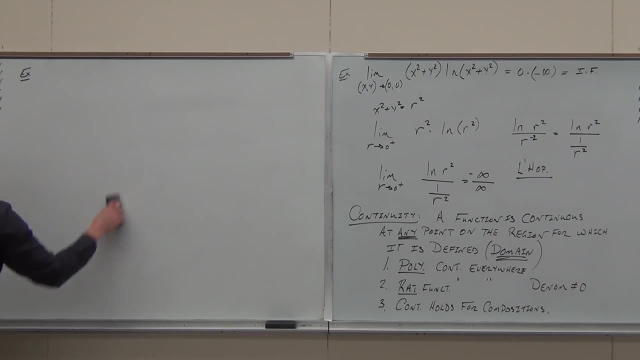 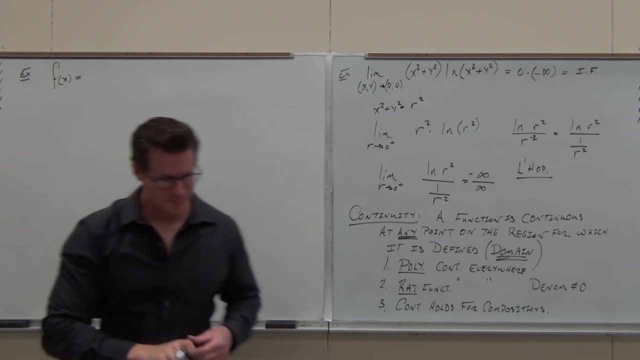 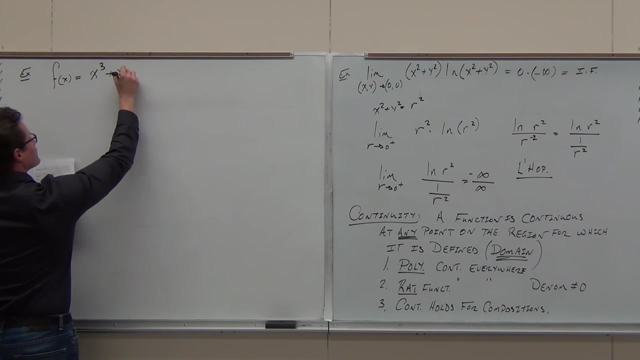 You're making me feel like I'm punching. I'm going to do it. I'm going to do it. I'm punishing you. Oh crap, you do feel like I'm punishing you. Yeah, me too. 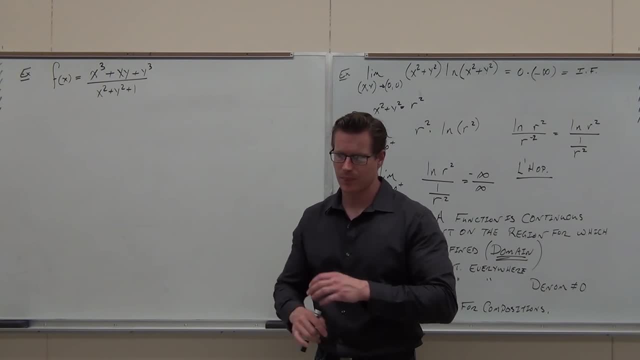 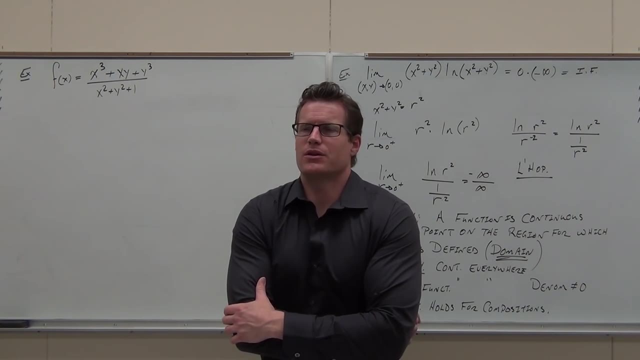 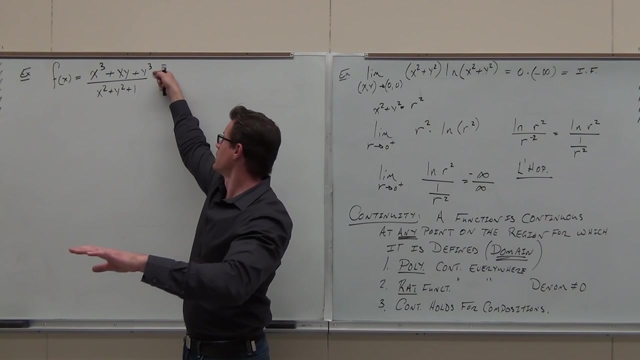 Question: where would domain issues and so likewise, where would continuity issues exist on this problem? If anywhere, where would they be? The denominator Good polynomial: continuous everywhere. perfect Polynomial: continuous everywhere. rational function: continuous everywhere, unless the denominator. 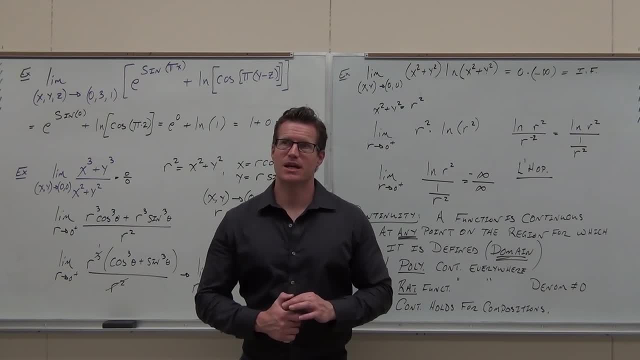 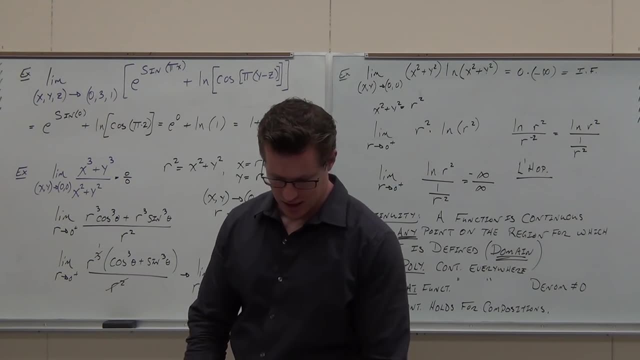 Just one. Okay, by one I mean two, Two examples about continuity. then we'll take a break, We'll come back and maybe do one more. We'll do that squeeze theorem thing. I'll talk about compositions and that'll be it. 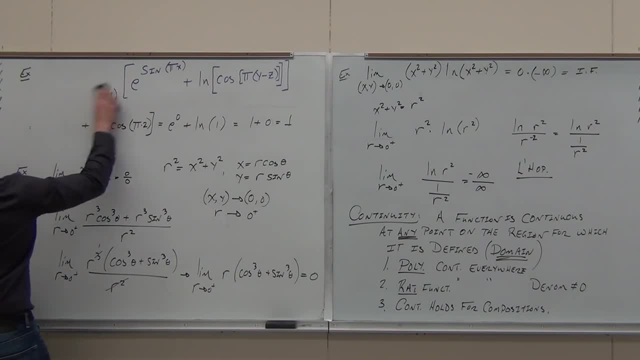 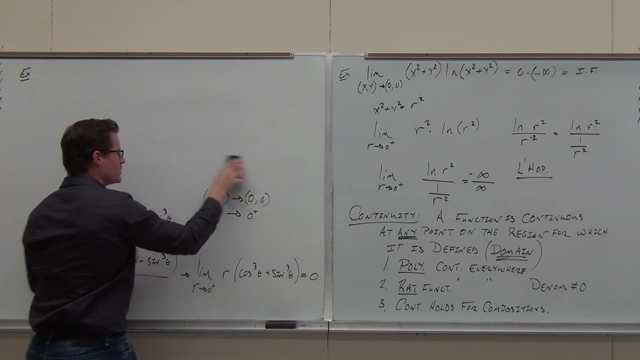 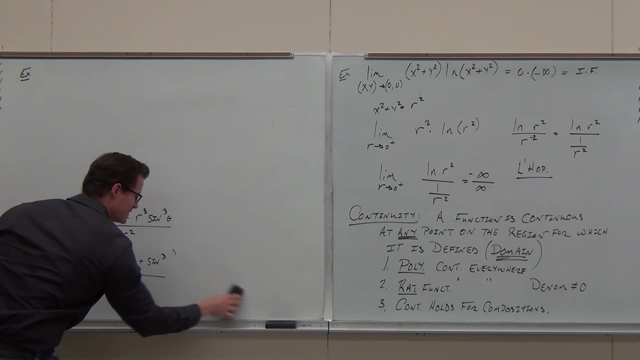 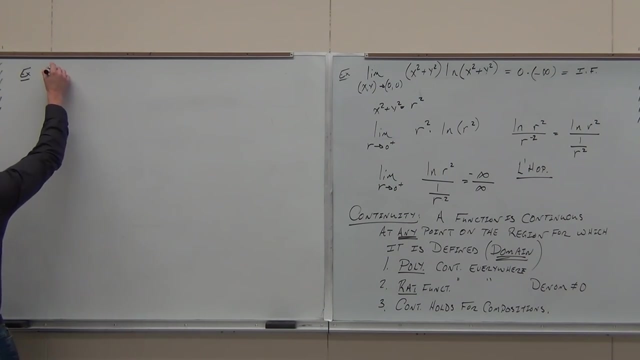 Pretty close. I do want some more energy out of you guys, though You're making me feel like I'm punishing you. Oh crap, you do feel like I'm punishing you. Okay, Okay, Okay, Okay, Okay, Okay, Okay. 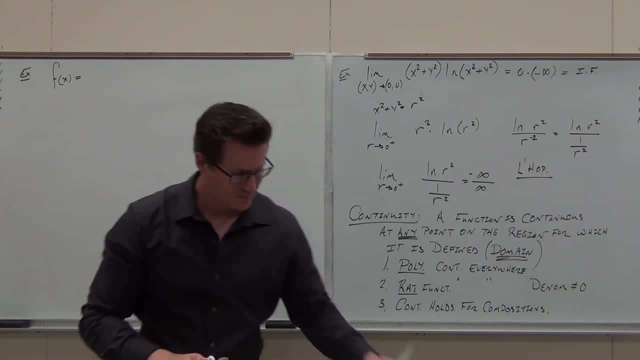 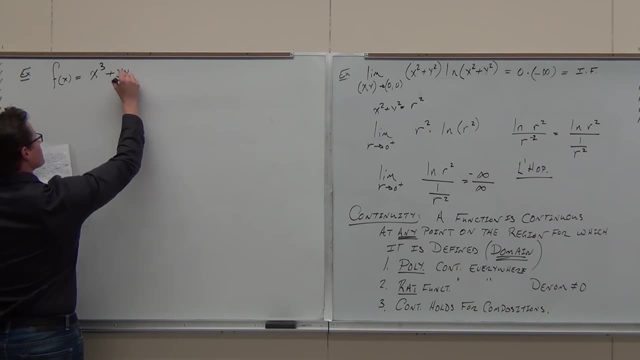 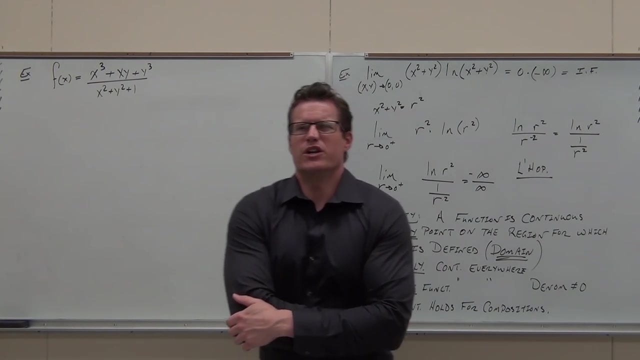 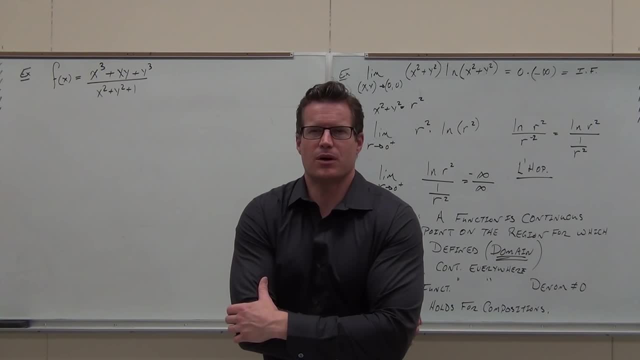 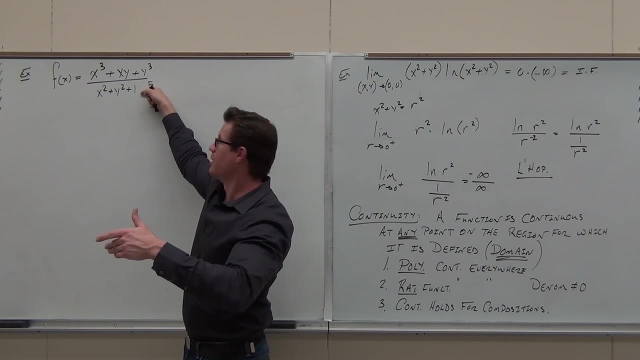 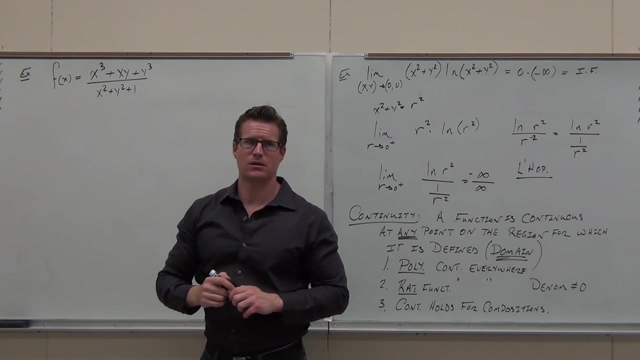 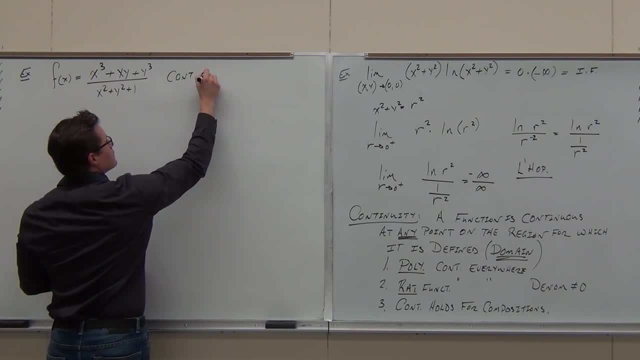 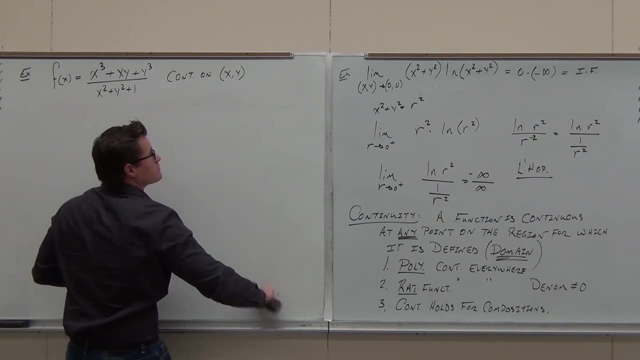 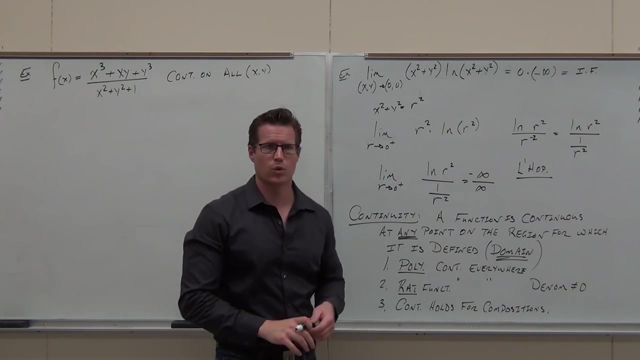 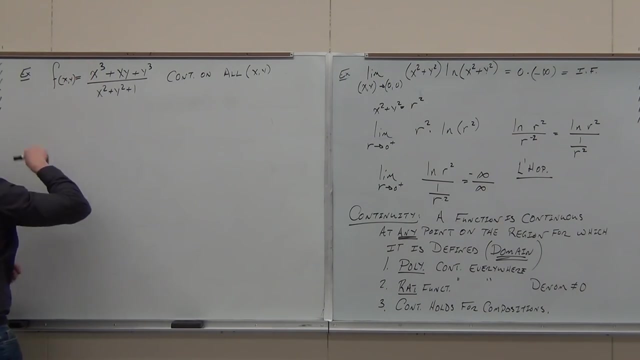 So this would be continuous On- let's put it this way- on all points. Continuous on all ordered pairs: XY. Question- Xy. Oh yeah, I'm sorry. Thanks for that. I didn't know if you were okay with that one. 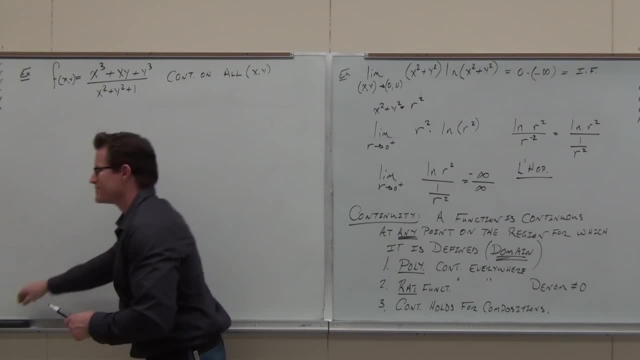 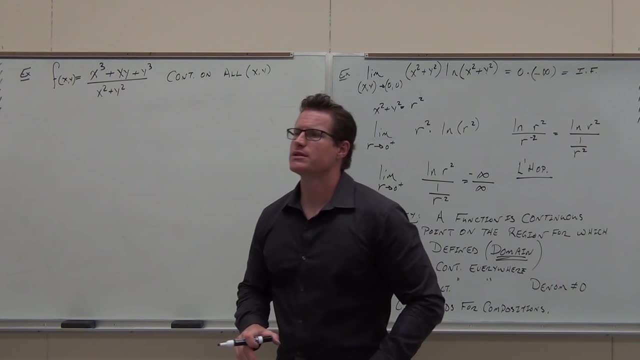 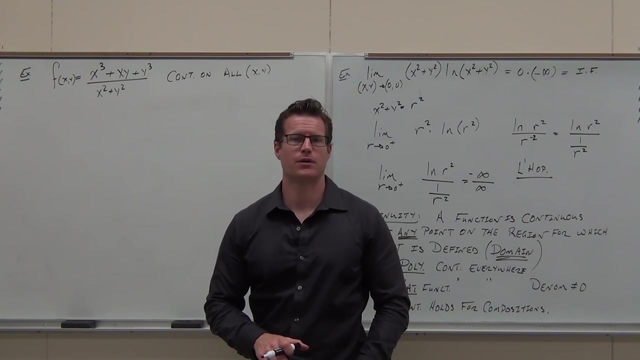 How about this? What if I just do one thing? Is that still continuous? So notice the change, please. Is that still continuous on all ordered pairs? No, What's the one point that I couldn't have? Zero, zero, Zero, zero. 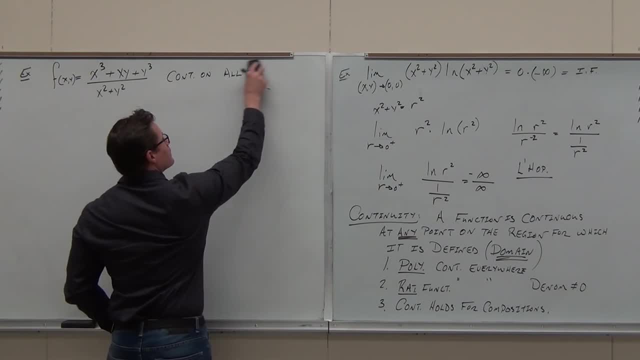 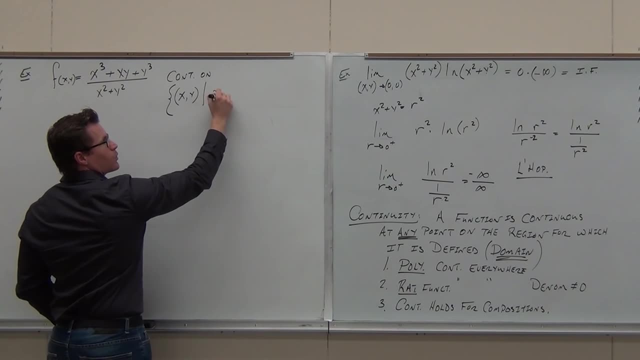 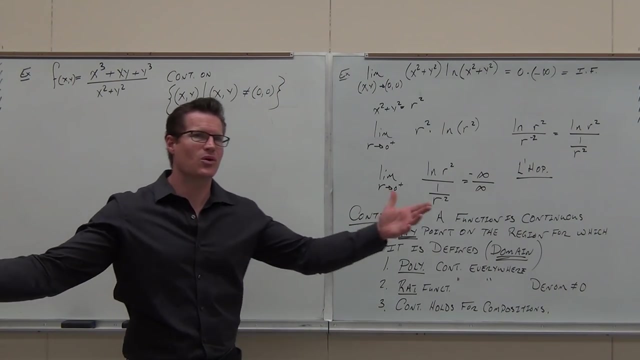 So this would be continuous. and here's how you'd write that: Write continuous on any ordered pair, such that that ordered pair does not equal the point zero, zero. That's how we'd show the continuity. Say, hey, anything works. 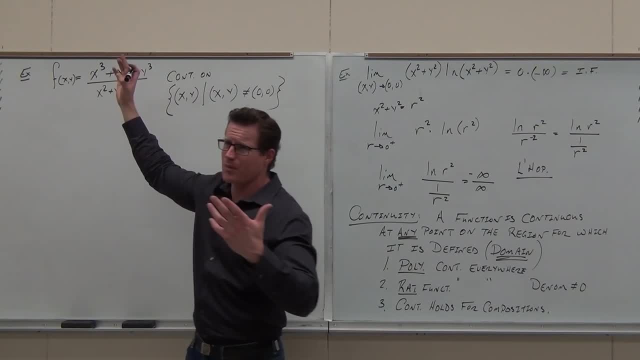 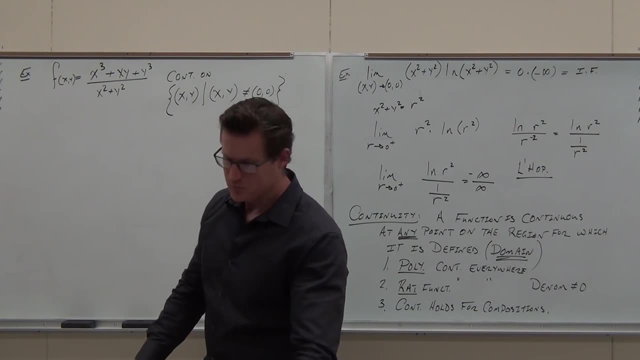 The only one that doesn't work is when the denominator is zero. That's a polynomial In December, no problem. If it's zero, who cares? But this one can't equal zero. That only exists at one spot. That only exists when xy equals the exact point: zero, zero. 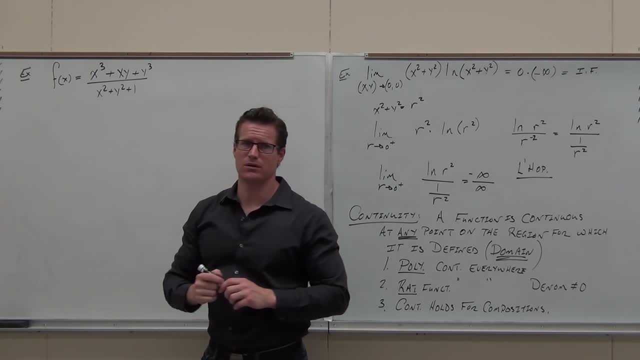 can equal zero. Now here's my question: can the denominator equal zero? Not with our imaginary numbers? Do we have imaginary numbers? Thank goodness no, so we don't even have those. So are there any continuity issues? So this would be continuous. 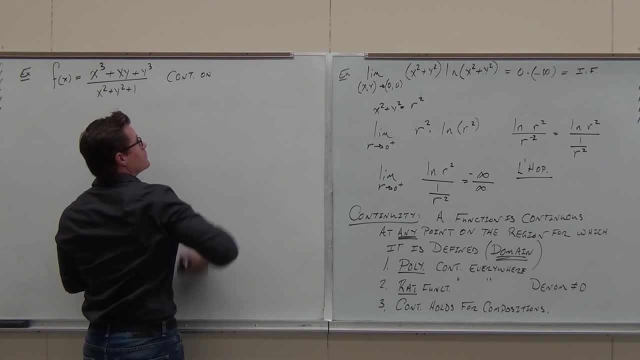 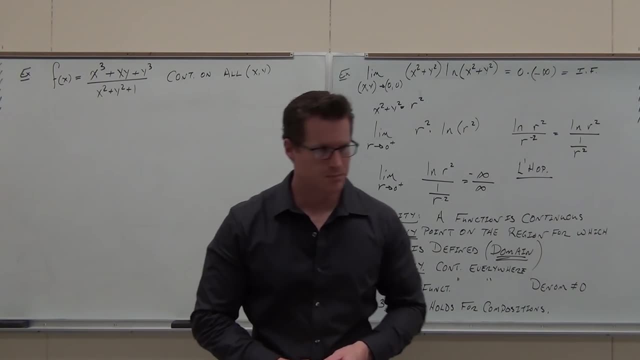 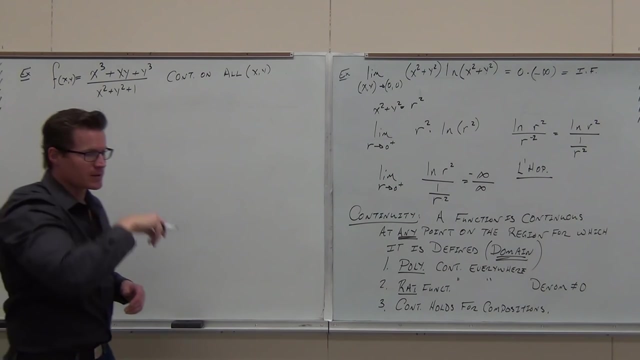 Let's put it this way: on all points, Continuous. on all ordered pairs: x, y. Question The x y. Oh yeah, I'm sorry, Thanks for that. I didn't know if you were okay with that one. 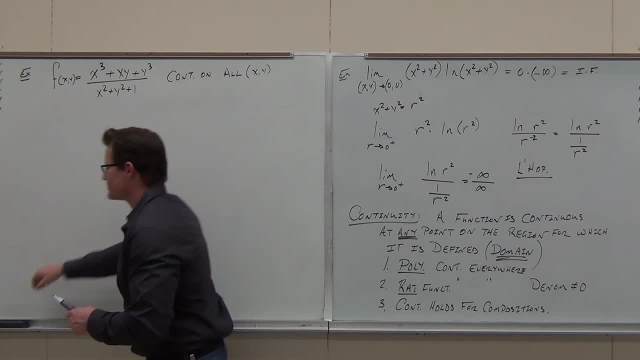 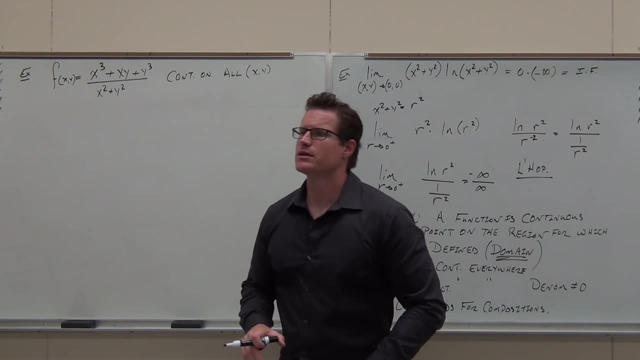 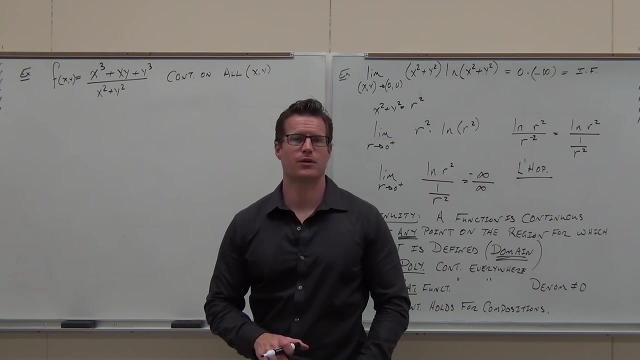 How about this? What if? what if I just do one thing? Is that still continuous? so notice the change, please. Is that still continuous on all ordered pairs? No, What's the one point that I couldn't have? Zero, zero. 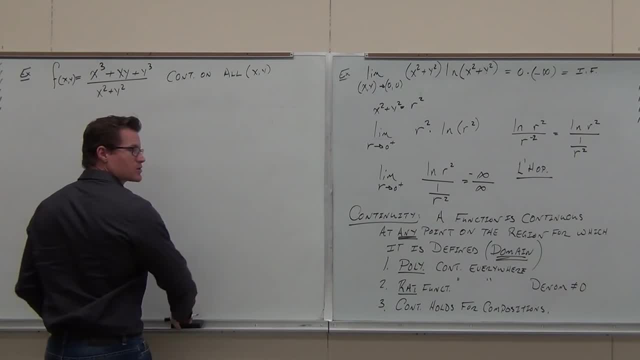 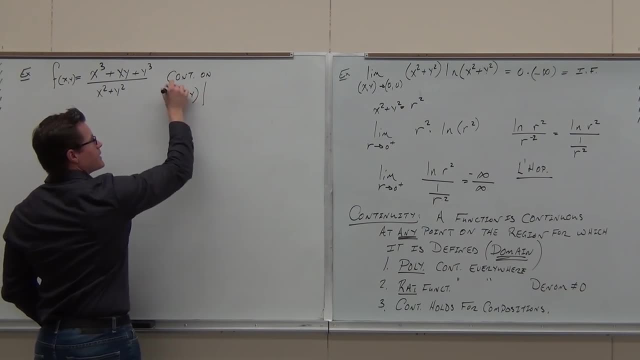 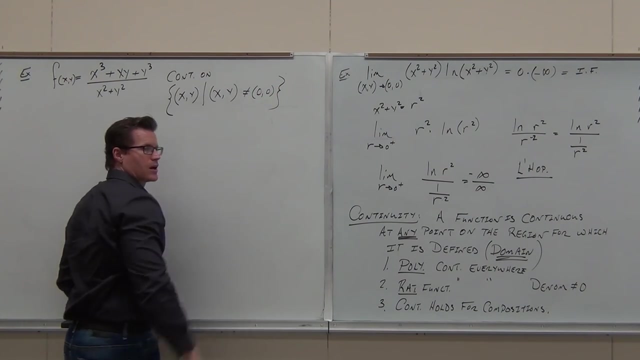 Zero, zero. So this would be continuous. and here's how you'd write that: Write continuous on any ordered pair, such that that ordered pair does not equal the point zero, zero. That's how we'd show the continuity. Say, hey, anything works. 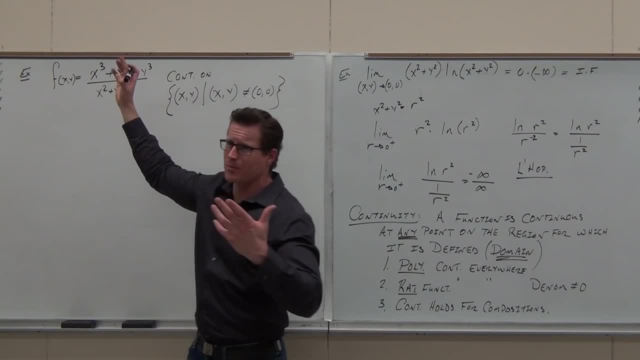 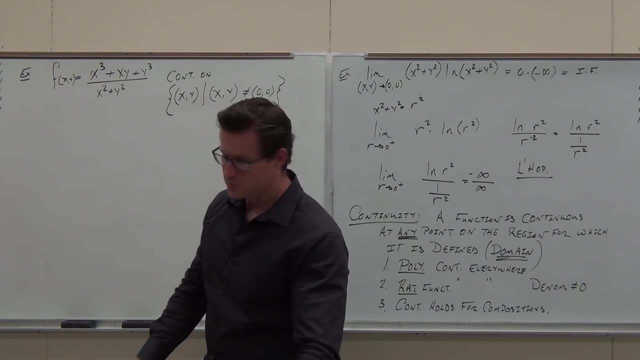 The only one that doesn't work is when the denominator is zero. That's a polynomial in December, no problem. If it's zero, who cares? But this one can't equal zero. That only exists at one spot. That only exists when x- y equals the exact point: zero, zero. 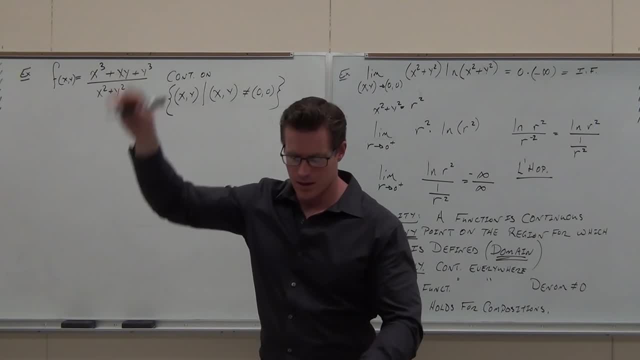 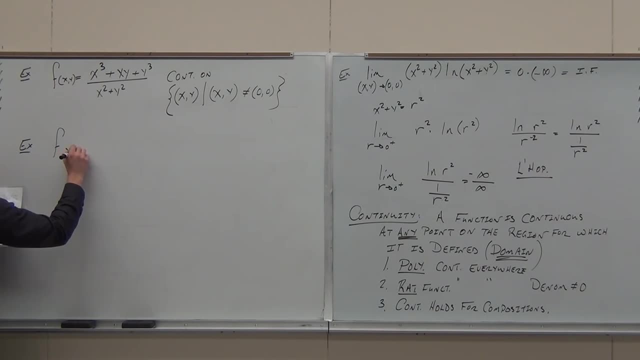 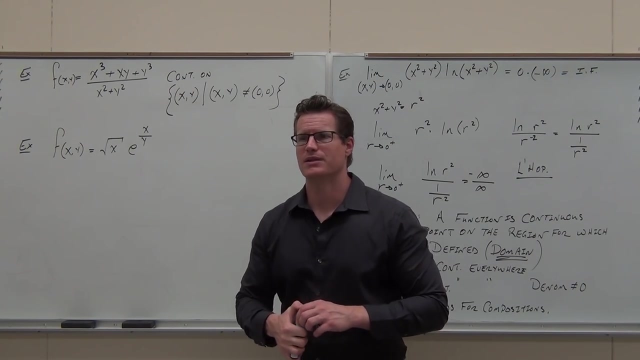 That's my only discontinuity. Should fans be okay with that one? Okay, here's the second example. Let me take a break. Please notice the compositions. Please notice that they're really not an issue as far as creating for you more discontinuities. 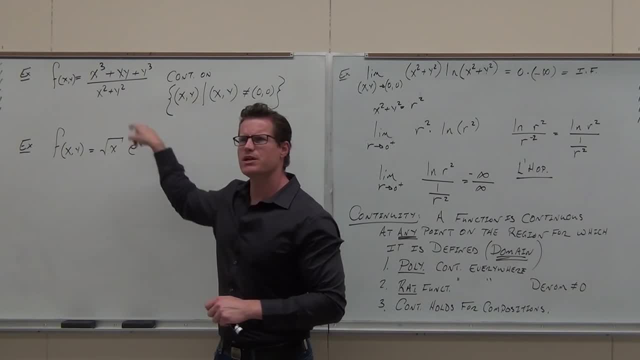 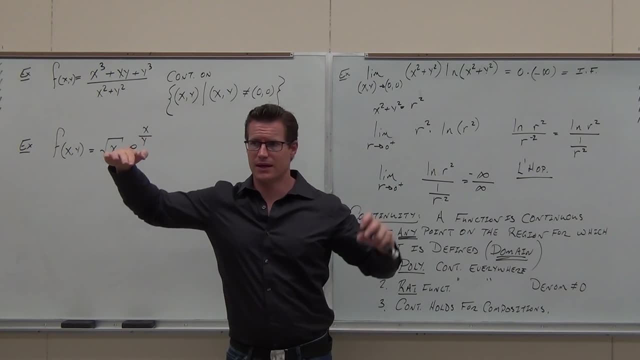 All they do is they might have some within. So let's take a look at it. What do we know about this thing right now? Firstly, is e to the x continuous everywhere? E to the x is a function That's continuous everywhere, for sure. 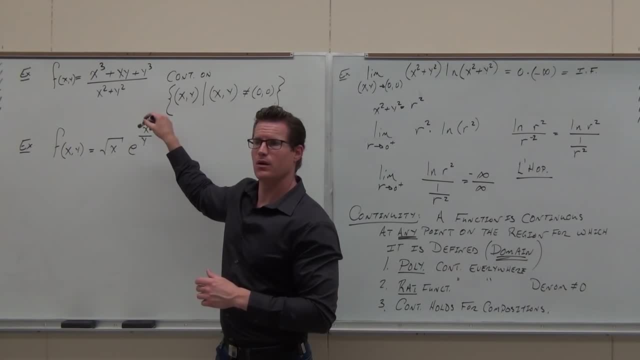 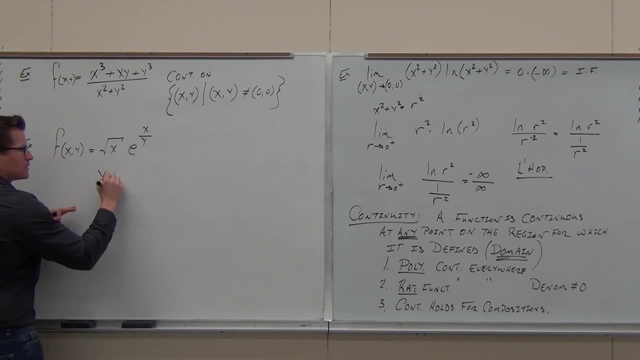 Is x over y, continuous everywhere. What's the problem here? What couldn't we have? Well, come on quickly. What couldn't we have? So we can't let y equal zero, So y cannot equal zero. Tell me, write something else quickly. 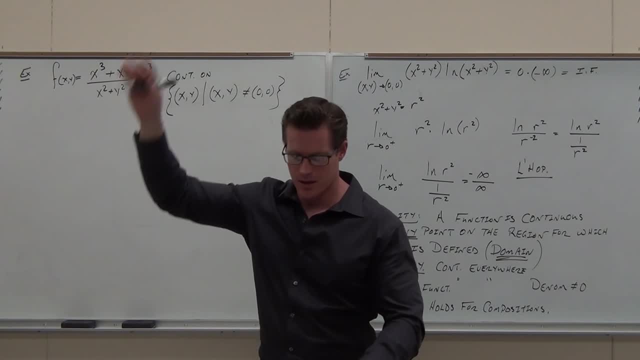 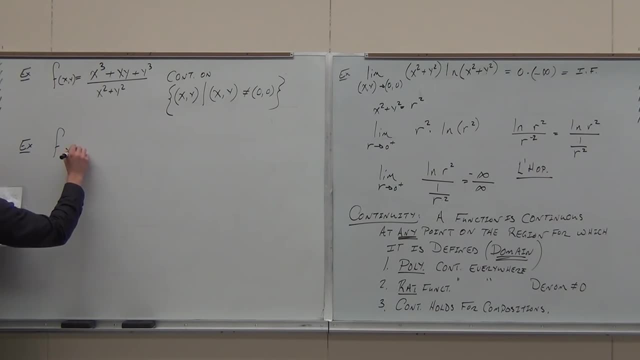 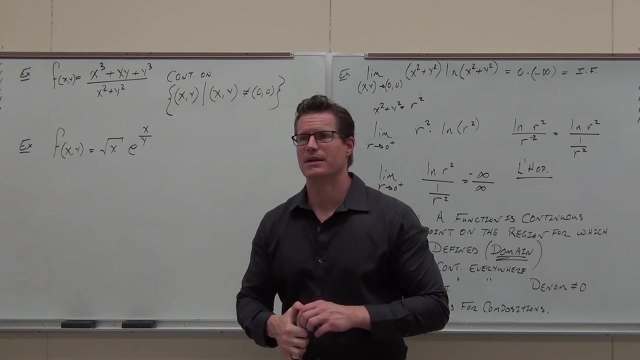 That's my only discontinuity. Should fans feel okay with that one? Okay, here's the second example. Let me take a break. Please notice the compositions. Please notice that they're really not an issue as far as creating for you more discontinuities. 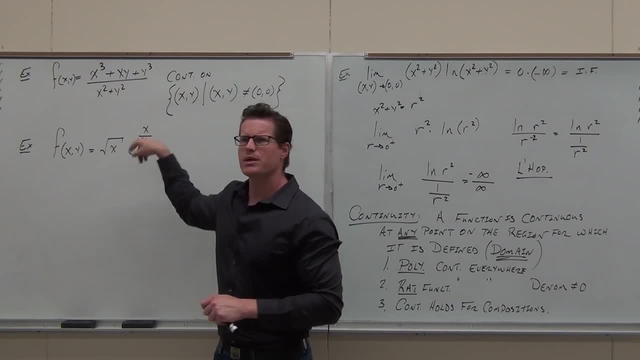 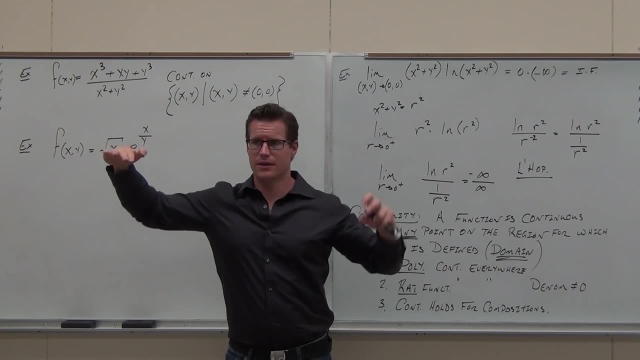 All they do is they might have some within. So let's take a look at it. What do we know about this thing right now? Firstly, is e to the x continuous everywhere? e to the x is a function That's continuous everywhere, for sure. 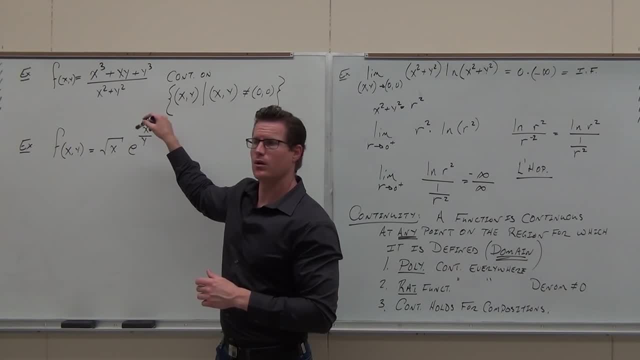 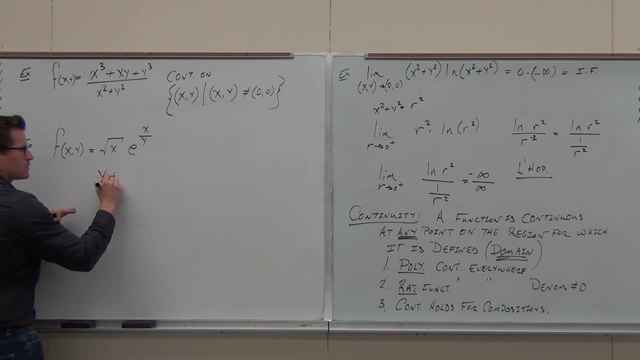 Is x over y, continuous everywhere. What's the problem here? What couldn't we have? Come on quickly, What couldn't we have? So we can't let y equal zero. So why can that equal zero? Tell me, right side, something else quickly. 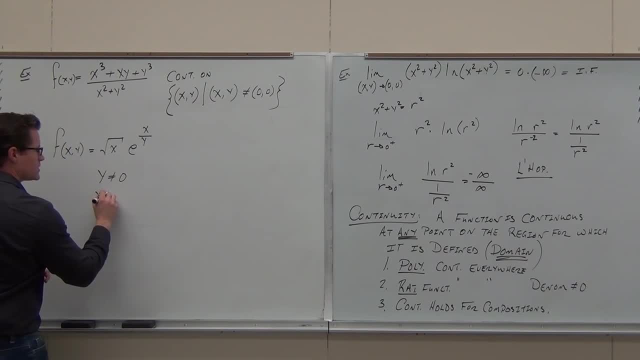 What else do you know about this thing? Could it be zero? Yes, Yes, Yes. So that's it. That's literally it. The only things we have here are x got to be greater than or equal to zero. y cannot be zero. 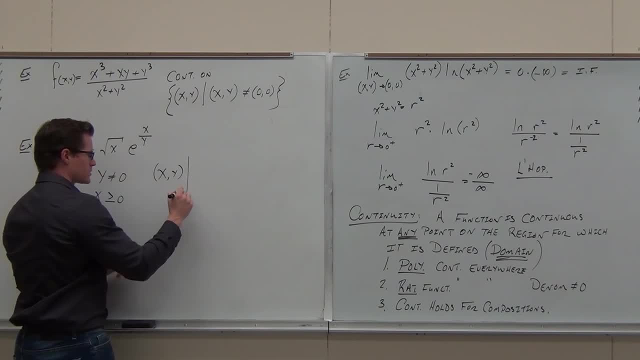 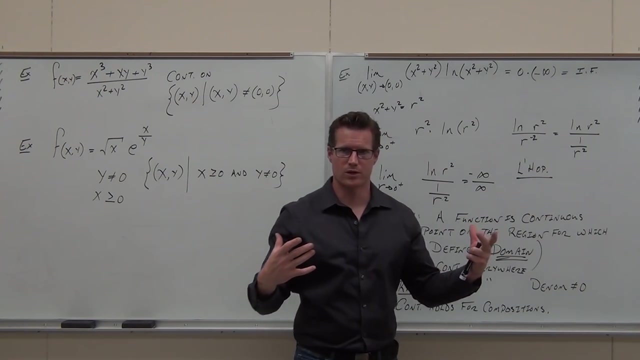 So we have any ordered pair such that x must be positive and y cannot equal zero, Since domain. basically, since domain gives you the region where your function is defined, Mm-hm. And since the region where your function is defined, so it's giving you continuity. 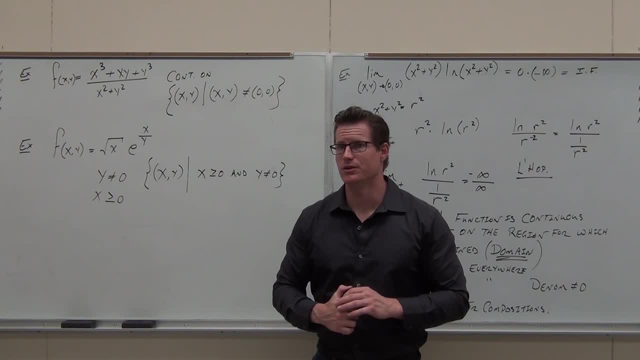 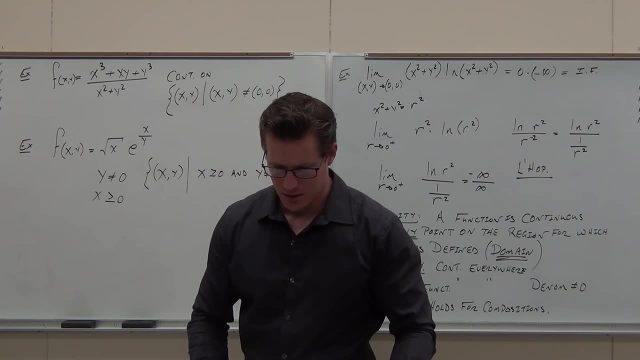 basically, finding your domain is practically the same as finding your continuity in almost every single case, and that's what we deal with. We'll do maybe one more when we come back from our break, but I think we need a break here real quick. 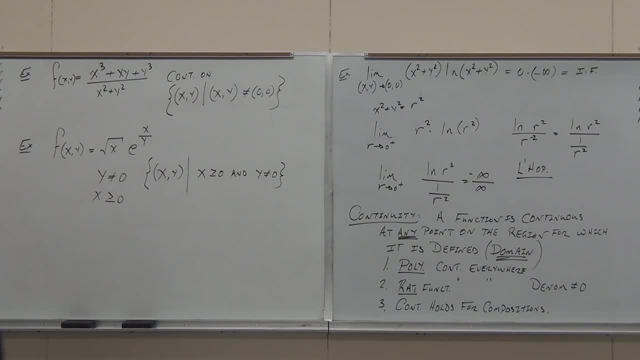 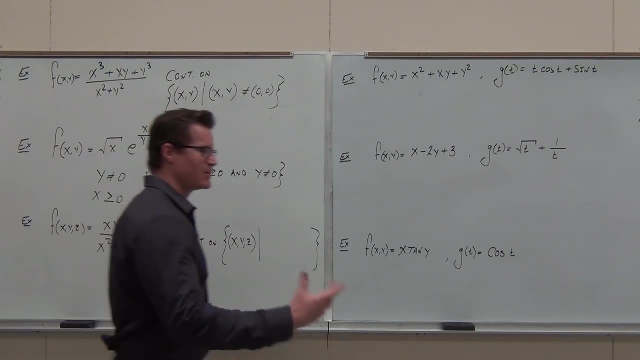 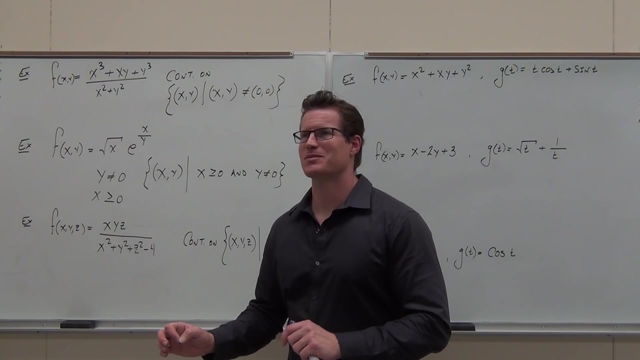 Show fans feel okay with what we're doing so far. Okay, So a few examples. We're talking about continuity. What we're finding out is that finding continuity and finding the domain most of the time are pretty much one and the same. Oh, almost rhymes. 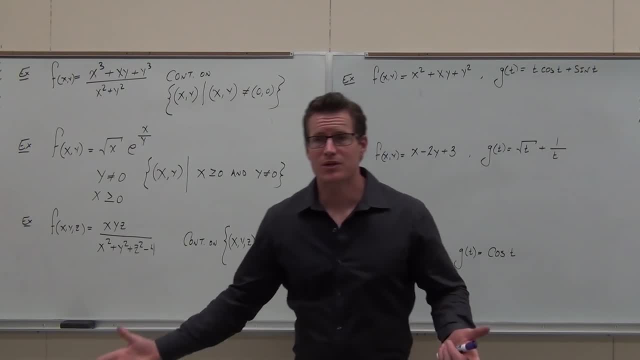 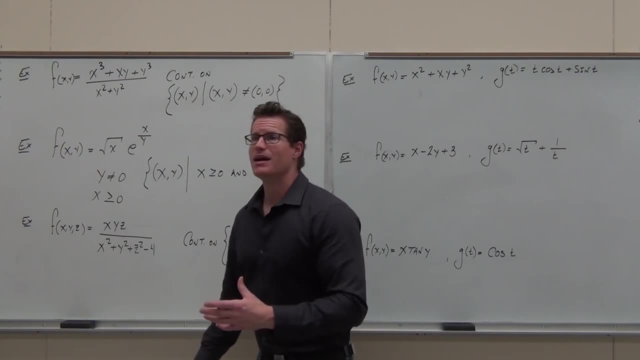 I like that. So you're just looking for the problem issues. That's all we're doing Now. that holds true for functions in three independent variables. So let's take out this domain. Here's the problem. Here, let's check out the continuity. 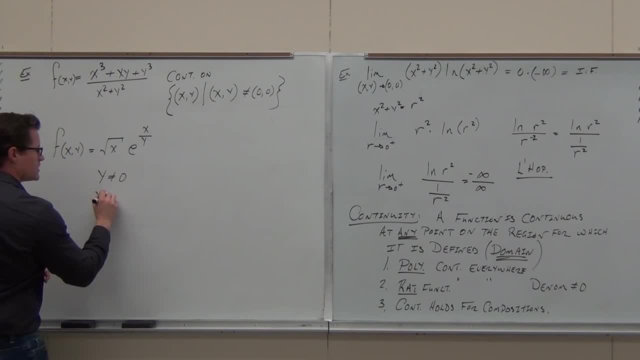 What else do you know about this thing? Can't write something else quickly. Could it be zero? Yes, So that's it. That's literally it. The only things we have here are x got to be greater than or equal zero. y cannot be zero. 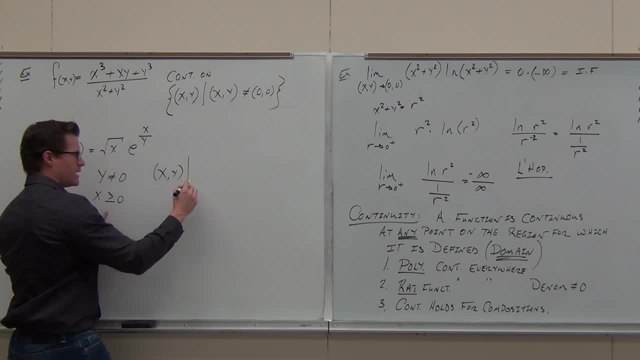 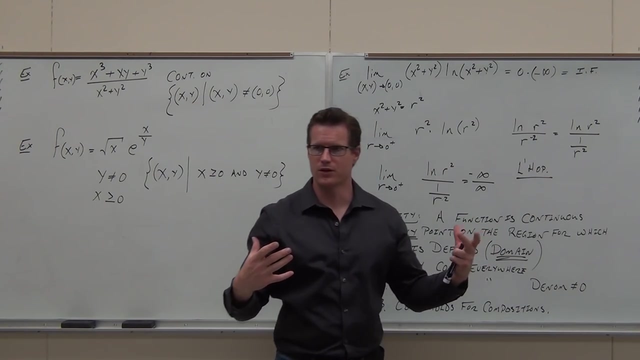 So we have any ordered pair such that x must be positive and y cannot equal zero Sense domain. basically, sense domain gives you the region where your function is defined, and since the region where your function is defined is what's giving you continuity. 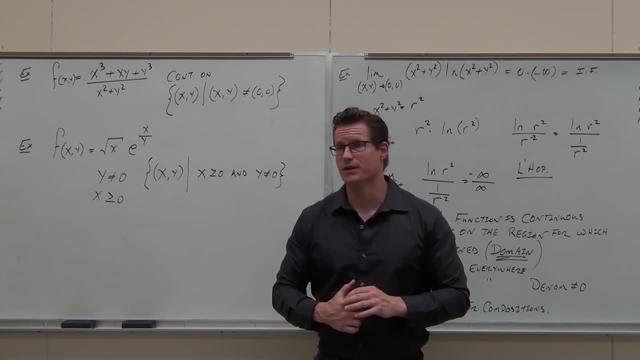 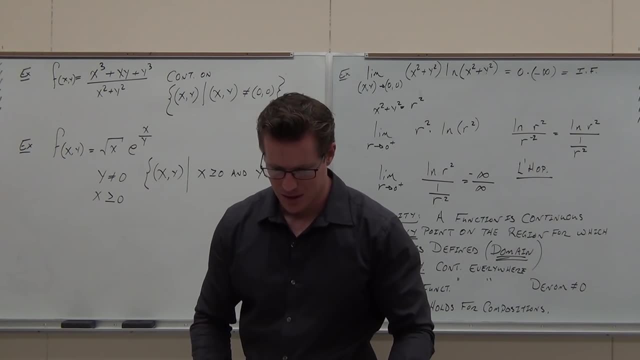 basically, finding your domain is practically the same as finding your continuity in almost every single case, And that's what we deal with. We'll do maybe one more when we come back from our break, but I think we need a break here real quick. 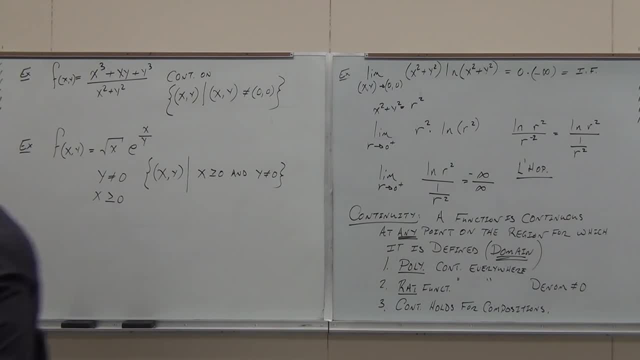 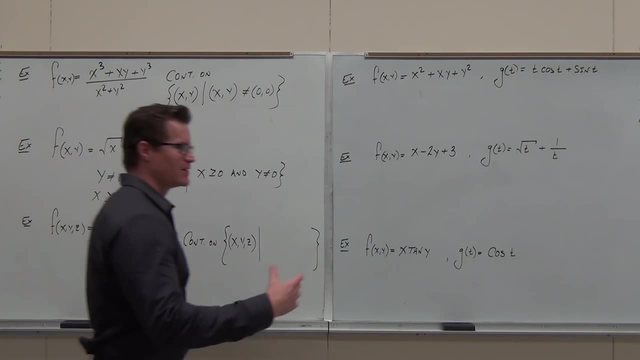 Show fans feel okay with what we're doing so far. Okay, So a few examples. We're talking about continuity. What we're finding out is that finding continuity and finding the domain most of the time is the same as finding the domain. 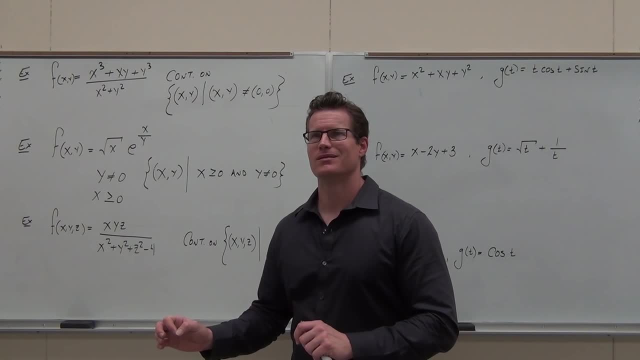 So we're talking about continuity. We're finding out is that finding continuity and finding the domain most of the time are pretty much one and the same. Huh, almost rhymes. I like that. So you're just looking for the problem issues. 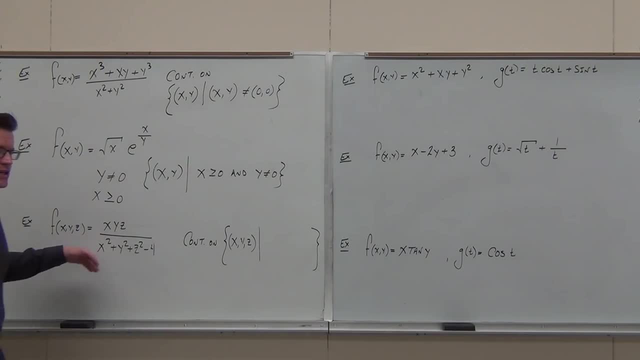 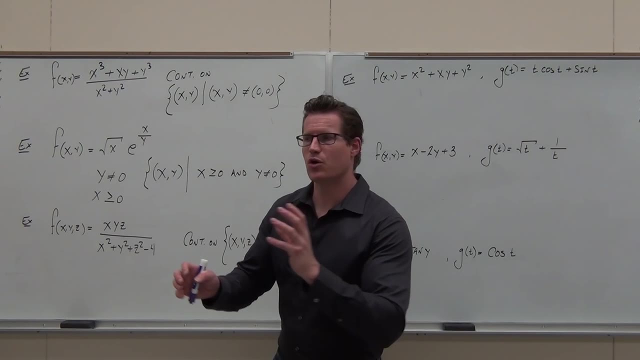 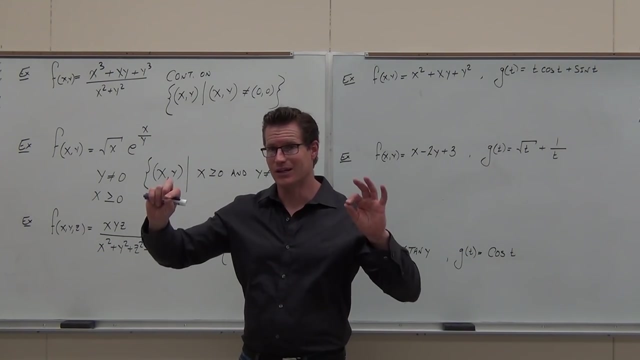 That's all we're doing Now. that holds true for functions in three independent variables. So let's take out this domain. Here's the problem. Here let's check out the continuity. Here's the issue. Just like domain of two variables is on a plane 2D, domain of one variable is on a line 1D. 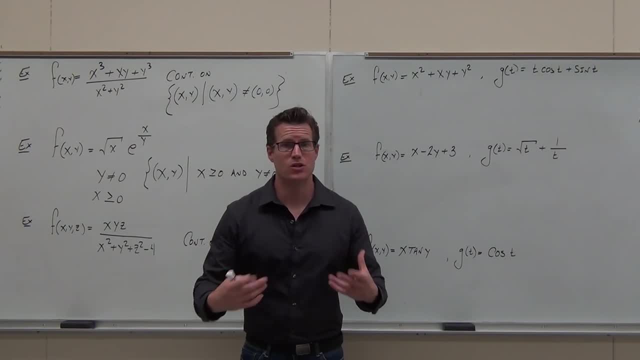 domain of three independent variables is 3D, which means continuity is also a 3-D issue. So let's take a look at this. Do we have any domain issues on the numerator: Yes, No. Denominator: Yes, No. 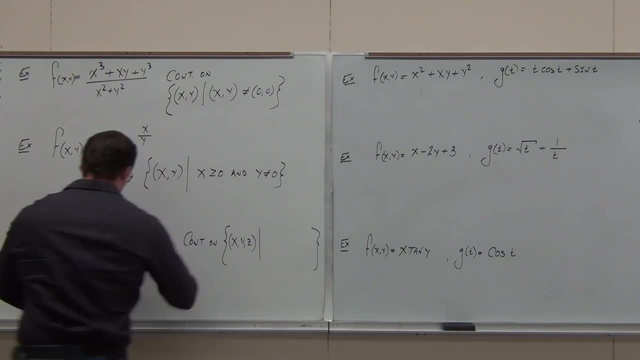 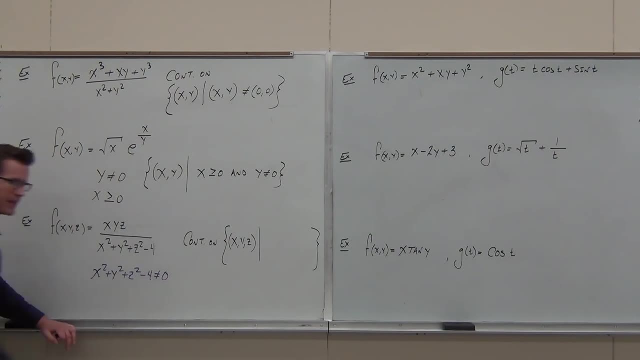 What do you know about denominators? Everybody? come on quickly. I know zero, So I know that That's true. That's it. That's the only continuity issue we have. so write it down. We want all sets of order triples, such that X squared plus Y squared plus Z squared. 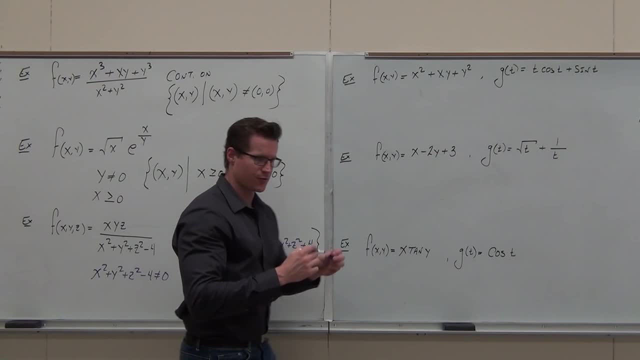 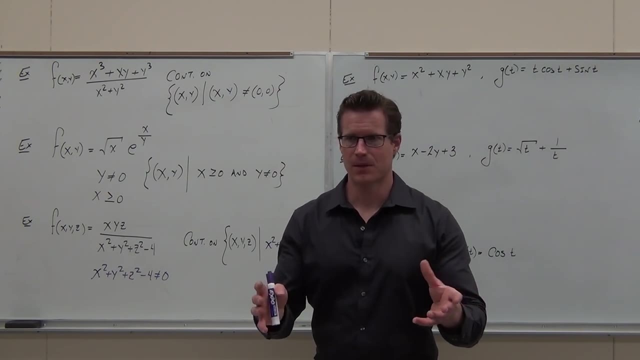 Sorry, Twoh X squared cannot equal 4. if you add 4 to both sides, I don't know if you're okay with that one. Now think about what this means. Think about what this means. Can you tell me what shape I'm going to ask you what shape this isn't. 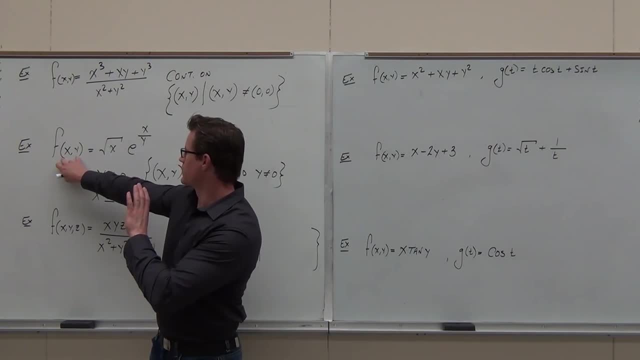 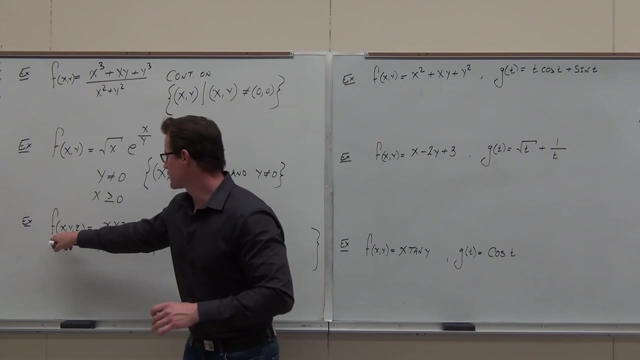 Here's the issue: Just like domain of two variables is on a plane 2D, domain of one variable is on a line 1D, domain of three independent variables is 3D, which means continuity is also a 3D issue. 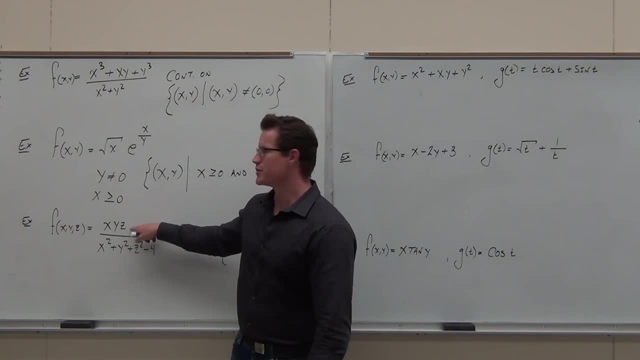 Okay, So let's take a look at this. Do we have any domain issues on the numerator: Yes or no? Denominator: Denominator Yes or no, Yes. What do you know about denominators? Everybody, come on quickly. 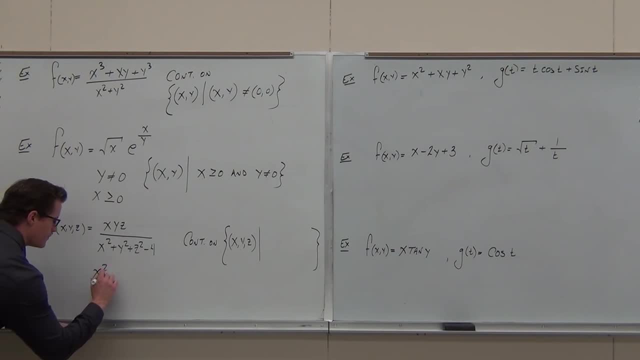 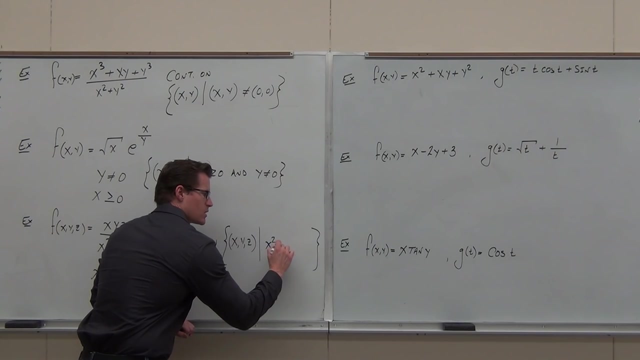 I equals zero, So I know that That's true. That's it. That's the only continuity issue we have, So write it down. We want all sets of order triples, such that X squared plus Y squared plus Z squared cannot equal 4 if you add 4 to both sides. 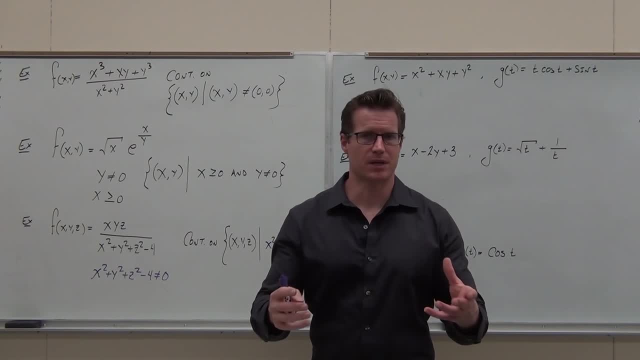 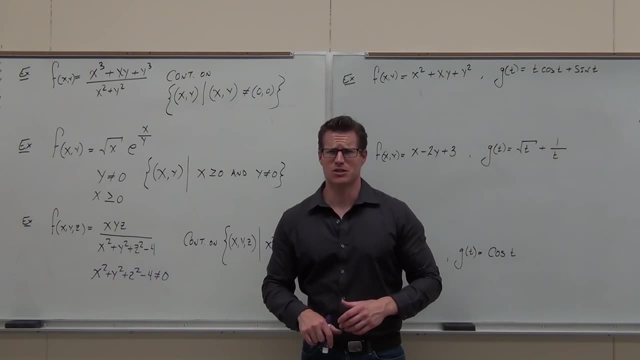 I don't know if you're okay with that one. Now think about what this means. Think about what this means. Can you tell me what shape I'm going to ask you what shape this isn't? What shape is? X squared plus Y squared plus Z squared equals 4?? 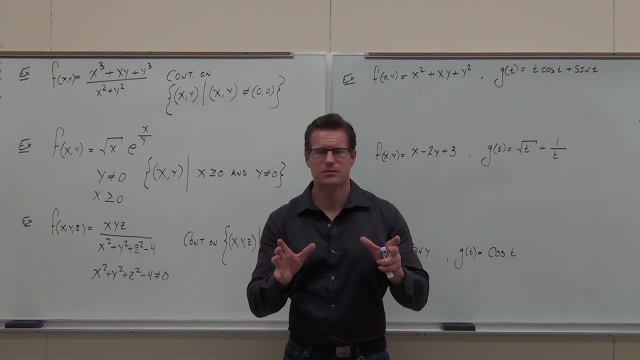 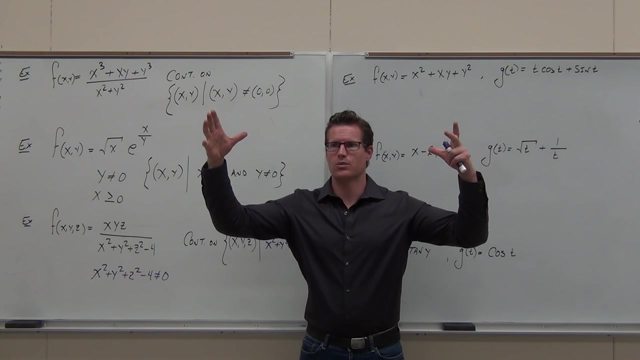 What shape is that? It's a what Ellipsoid? What type of ellipsoid, since all of our numbers are exactly the same. It's a sphere. It's a sphere. Okay, Here's what this says. It says: any point in all of 3-space will work. 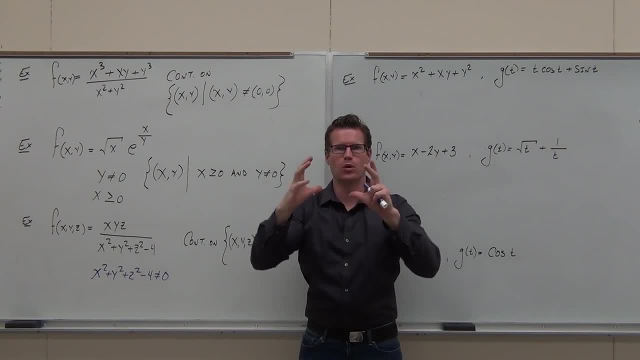 We have no discontinuities there, except for this bubble of that sphere. All it says is that the points you can't plug in, all those points, are on that sphere. Does that make sense to you? It's all of the 3-D space. 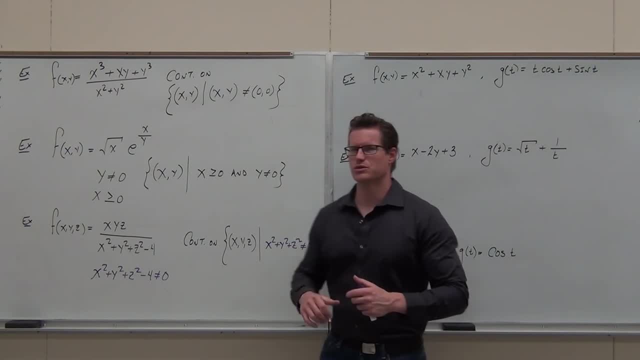 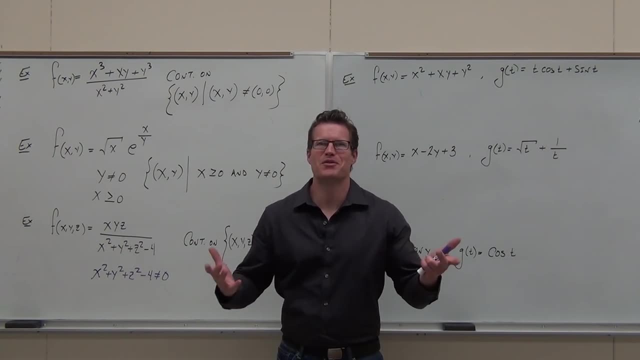 What shape is? X squared plus Y squared plus Z squared equals 4?. What shape is that? It's a. what Ellipsoid? What type of ellipsoid, since all of our numbers are exactly the same Square. It's a sphere. 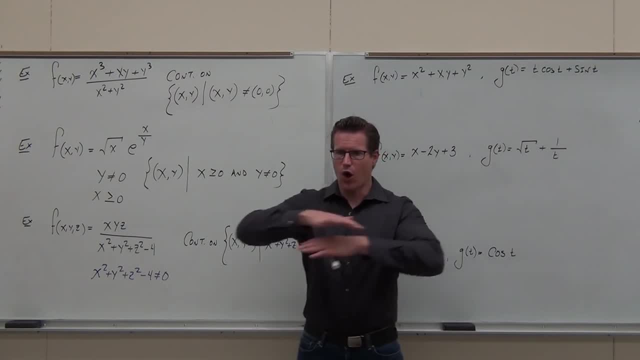 Here's what this says. It says: any point in all of 3 space will work. We have no discontinuities there, except for this bubble of that sphere. All it says is that the points you can't plug in, all those points are on that sphere. 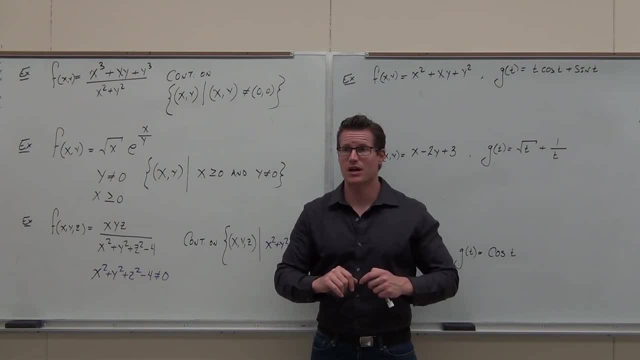 Does that make sense to you? It's all of the 3D space. The discontinuity exists on that sphere. The points that create discontinuities are on that sphere. That's why we can't let it equal. That's why we can't let it equal to the radius of 2.. 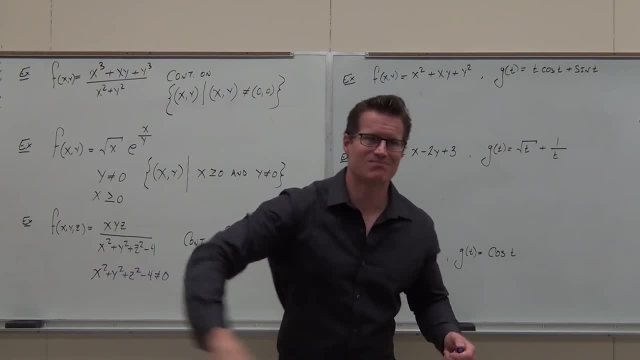 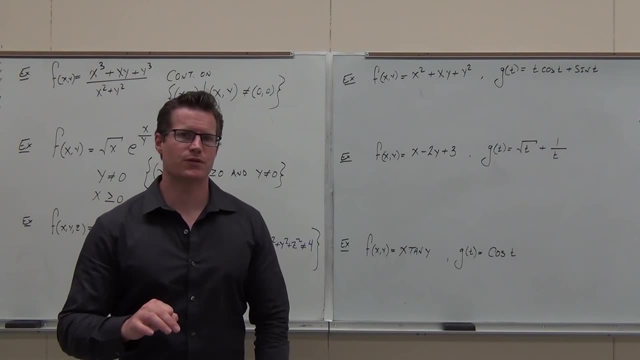 So if you guys feel okay with that, That's it. that's all we're doing. It's just regular continuity. Now, what I do want to tell you- the statement 3 down here from a little while ago: continuity still holds for compositions and parametrics are all compositions. 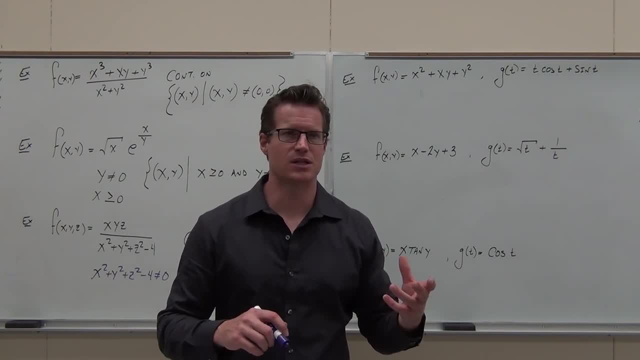 So when we're going to try to figure out some continuity that has compositions in it, just remember one thing: You can't ever make domain or continuity issues better. You can only make them worse. That's encouraging, right. You can't ever make domain or continuity issues better. You can only make them worse. That's encouraging, right. 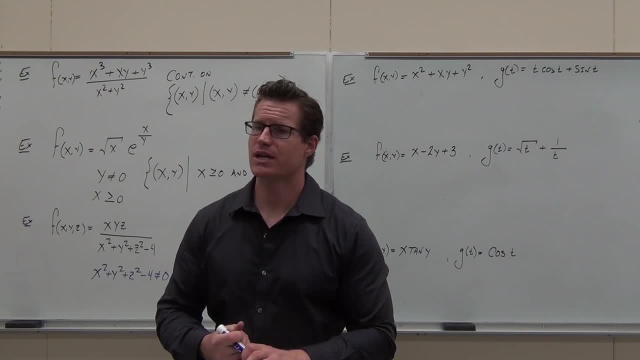 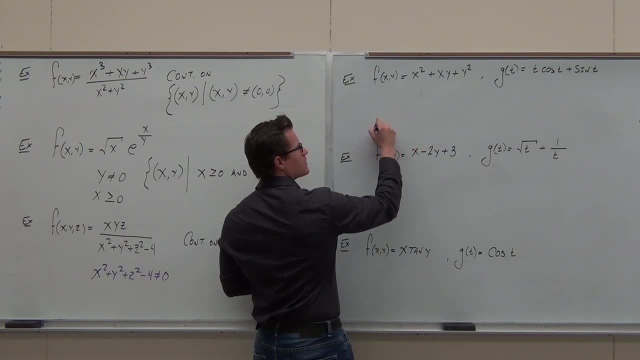 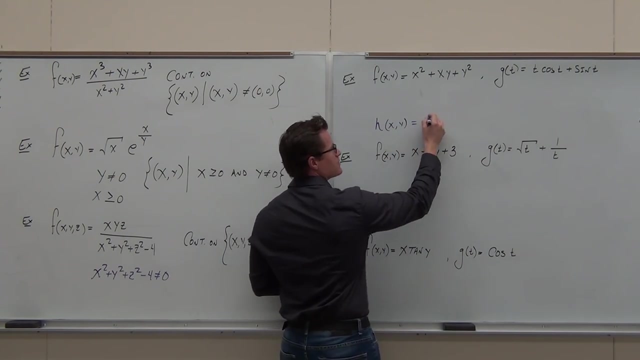 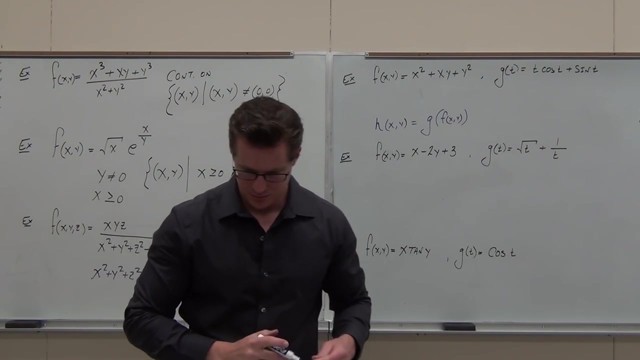 You can't fix a continuity issue ever. Here's how to do: some parametrics, some compositions, whatever you want to call them. Let's focus on finding h of xy such that this equals g of f of xy. In other words, what I want to do is: 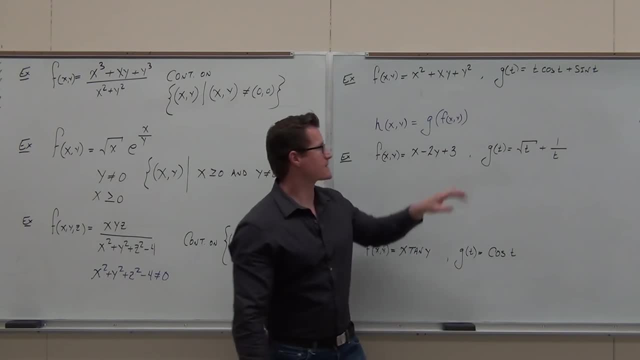 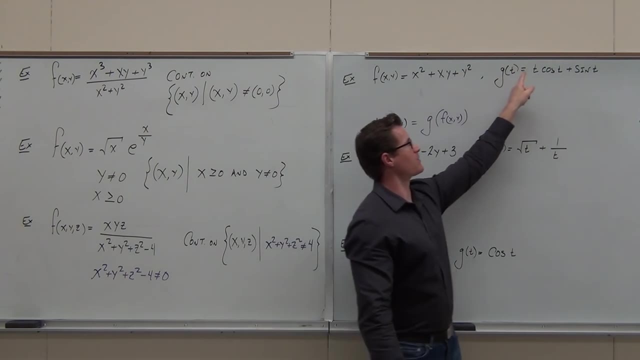 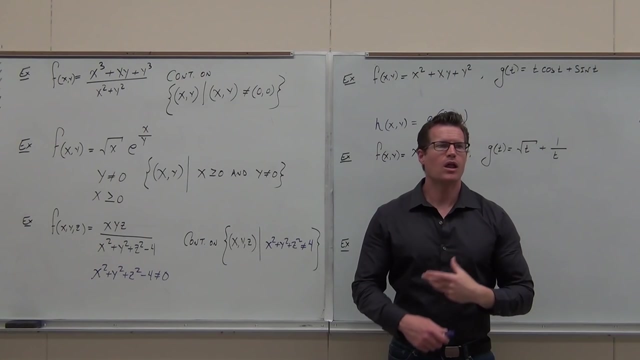 do you know how compositions work? No, This says: take the f thing, put it in for the g thing. So take this entire thing and replace this variable and this and this with it. Do you actually want to do that? No, No really. 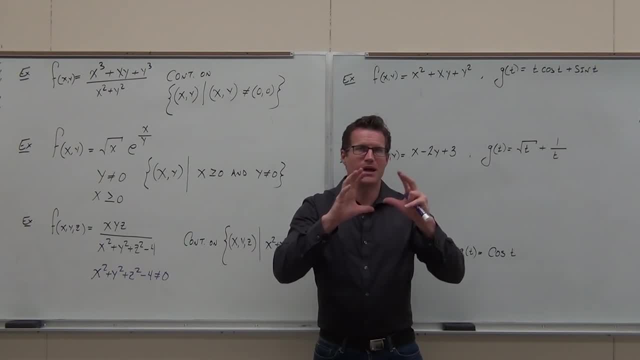 The discontinuity exists on that, you know, on that sphere. The points that create discontinuities are on that sphere. That's why we can't let it equal the radius of 2.. So if you feel okay with that, that's it. 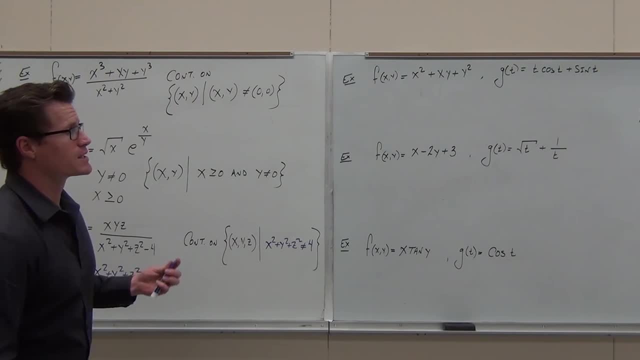 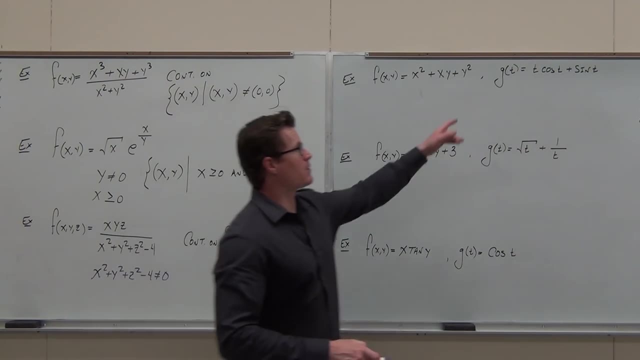 That's all we're doing. It's just regular continuity. Now, what I do want to tell you- the statement 3 down here from a little while ago. continuity still holds for compositions and parametrics are all compositions. So when we're going to try to figure out some continuity that has compositions in it, 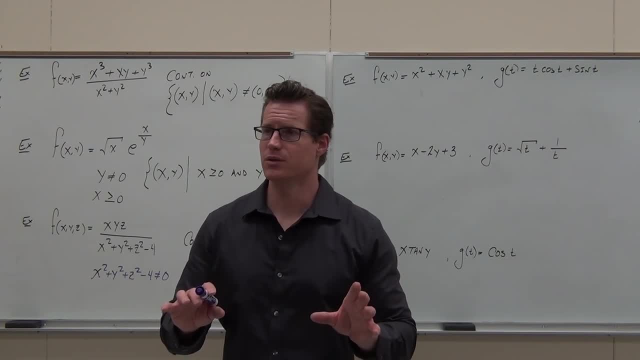 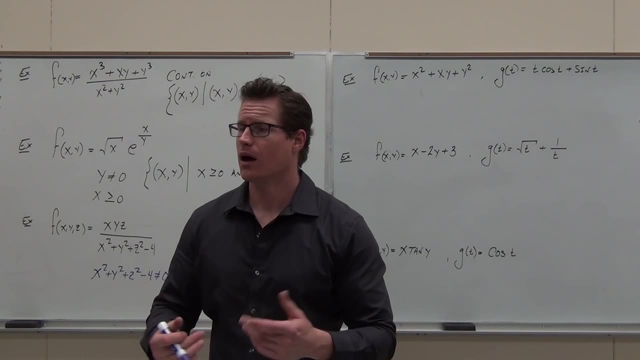 just remember one thing: You can't ever make domain or continuity issues better. You can only make them worse. That's encouraging, right? You can't fix a continuity issue ever. Here's how to do: some parametrics, some compositions, whatever you want to call them. 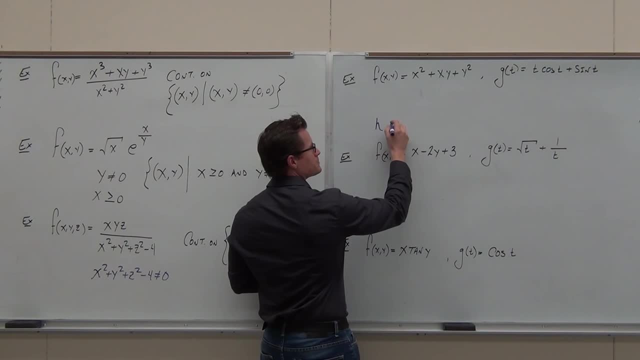 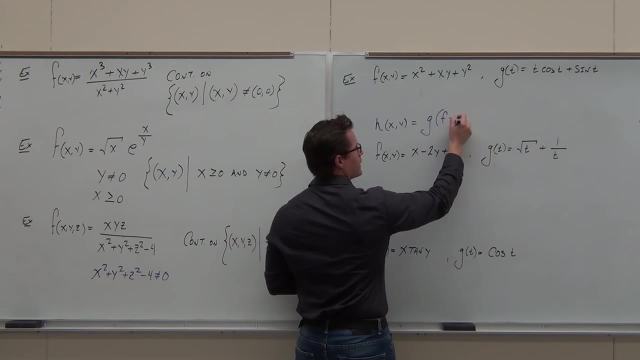 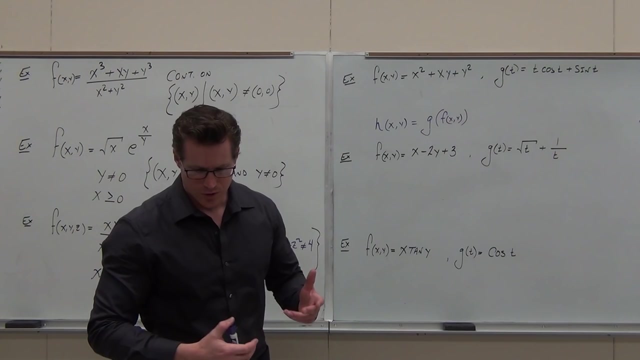 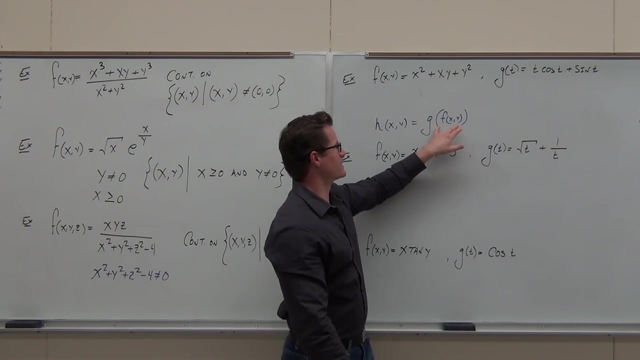 Let's focus on finding h of xy, such that this equals g of f of xy. In other words, what I want to do is: do you know how compositions work? No, This says: take the f thing, put it in for the g thing. 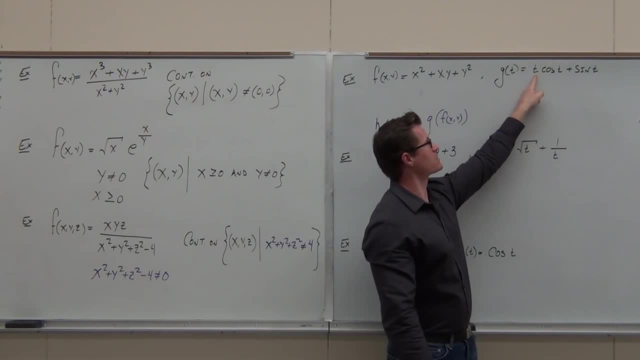 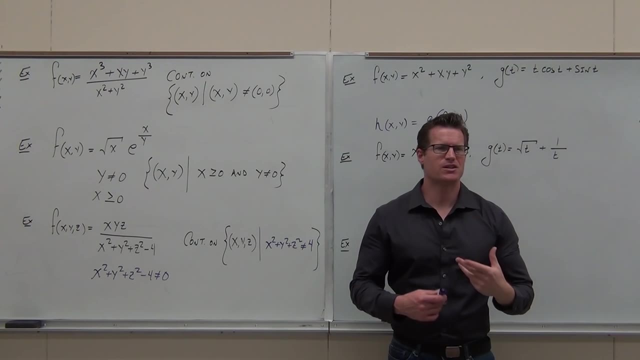 So take this entire thing and replace this variable and this and this with it. Do you actually want to do that? No, No, really. All I'm worried about is what's the continuity going to be for this composed function that we're going to get? 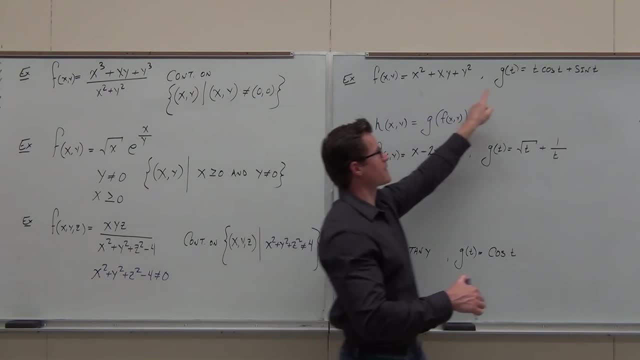 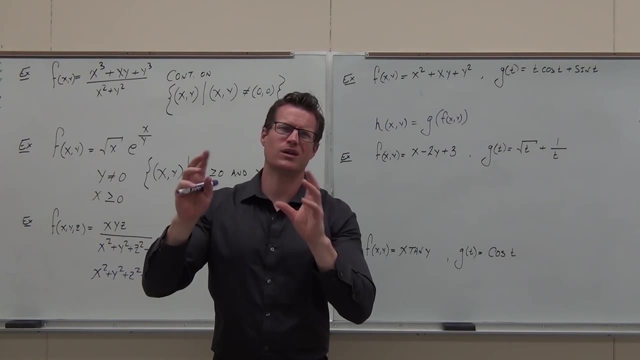 Here's how to do that. Firstly, find the continuity here. find the continuity here and I'll show you how to work with it. What's the continuity? Oh, we don't know Great Why. I don't want to say all real numbers, all ordered pairs. 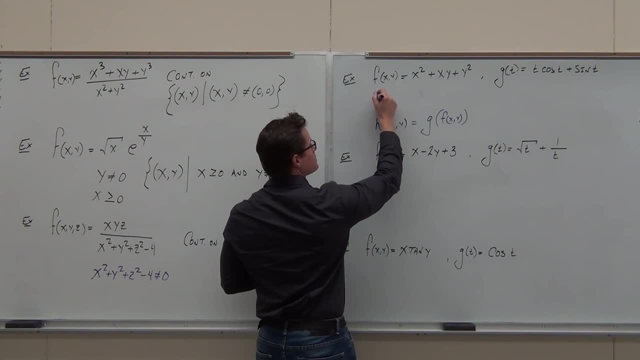 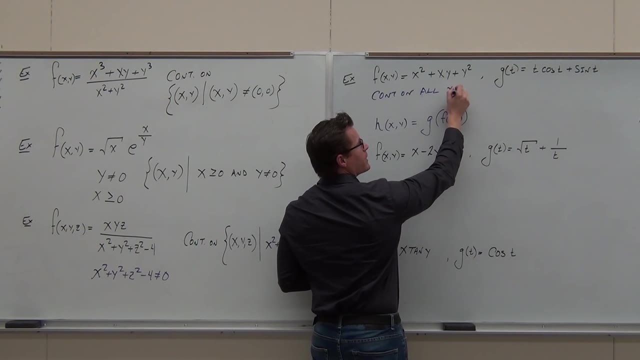 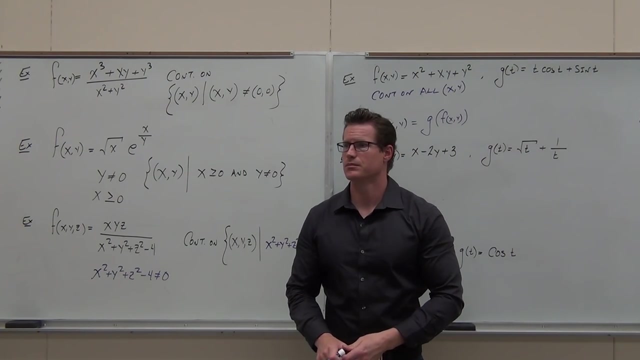 That's a better way to say it, because these are ordered pairs, So this is continuous on all ordered pairs, True or false? This is continuous on all t. Yes, no, Okay. what's it not continuous at? What's it not continuous at? 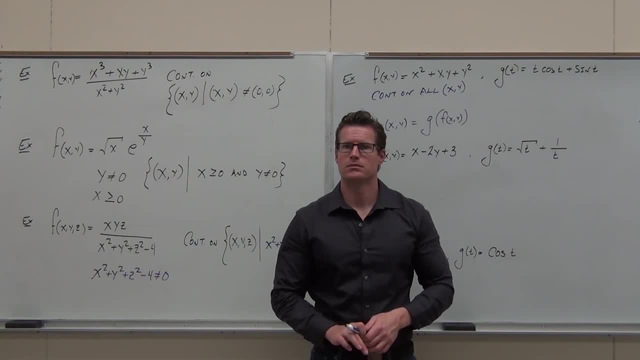 Inverse to higher plus zero. Say what: Over 2 pi is 1 pi less than zero to the power of t. No, plug in anything you want, Can you do it? Can you plug in anything to cosine? Can you plug in anything to sine? 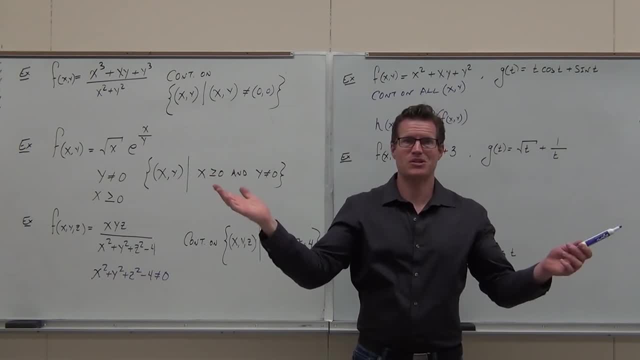 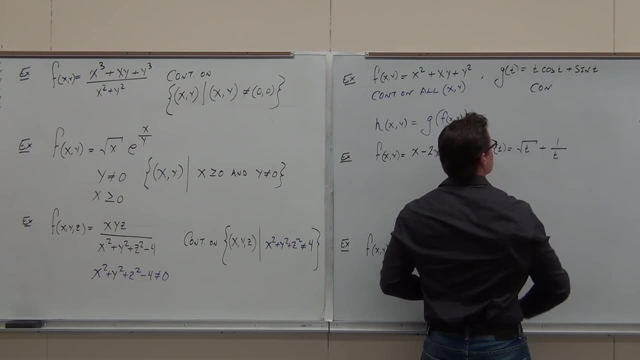 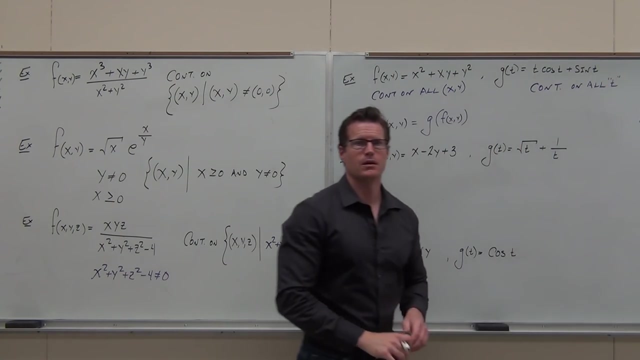 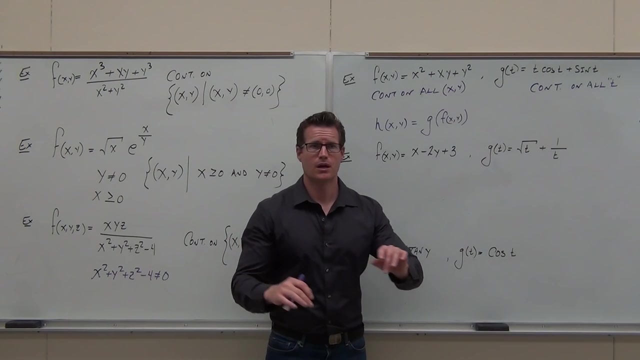 Can you plug in anything to t? No issues Continuous On all t. Here's what I want to tell you. if this, please watch carefully what we're going to do. You're not watching. you should be watching. please watch carefully. 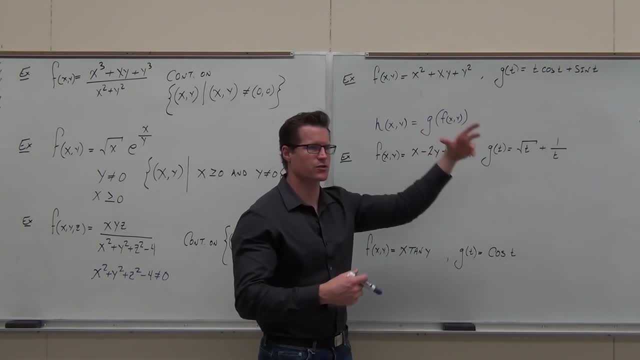 All I'm worried about is what's the continuity going to be for this composed function that we're going to get? Here's how to do that. Firstly, find the continuity here. find the continuity here and I'll show you how to work with it. 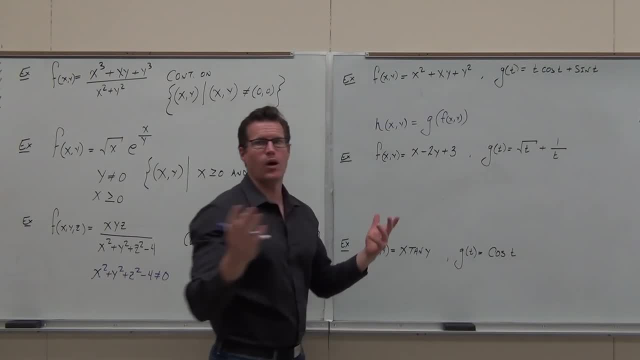 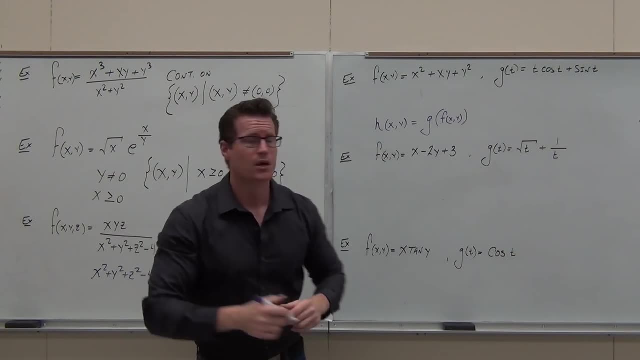 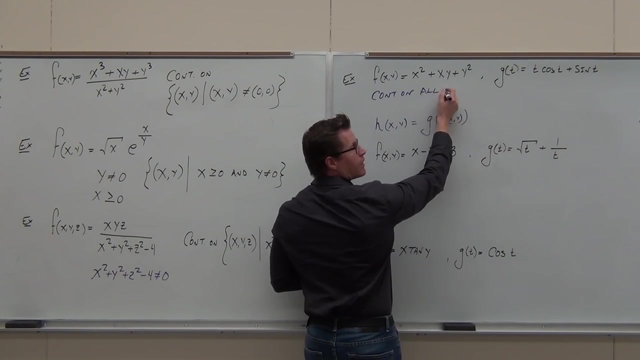 What's the continuity? Continuity, Great. Why? Well, I don't want to say all real numbers, all ordered pairs. That's a better way to say it, because these are ordered pairs, So this is continuous on all ordered pairs. 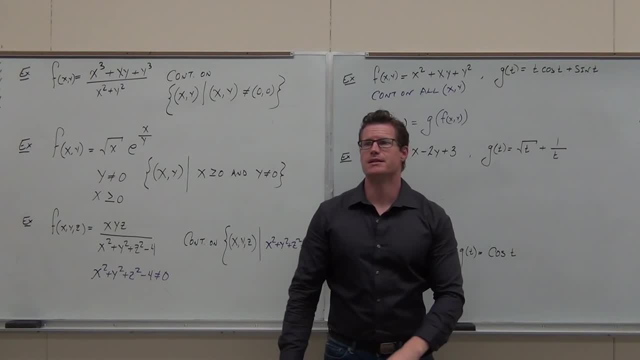 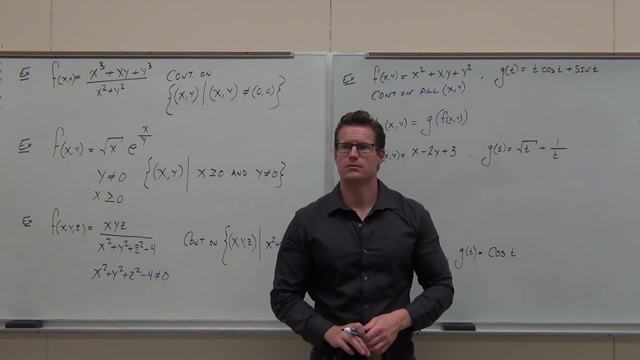 True or false. This is continuous on all t, Yes or no? No, Okay, What's it not continuous at 0. 0.. Oh, that's 0.. So what capit – 0 pi is pi less than 0, right. 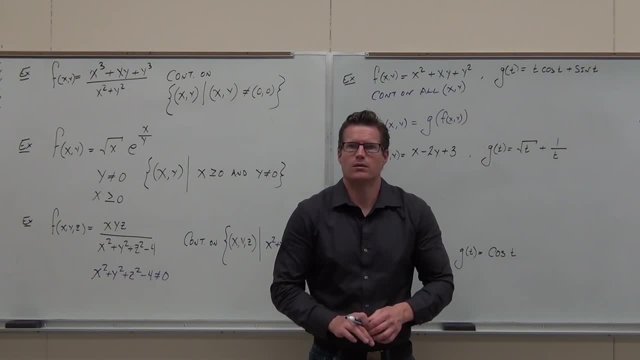 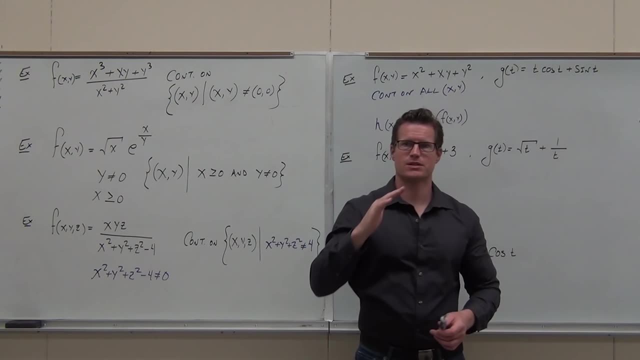 No plug in anything you want. Can you do it? Can you plug in anything to cosine 하고? Can you plug in anything to sine? It's a step. Can you plug in anything to t? It's a smoked height. No issues. 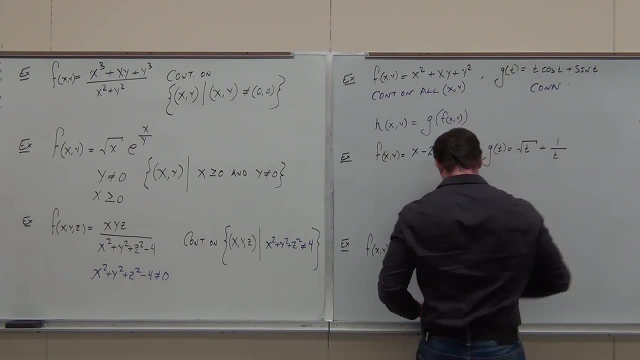 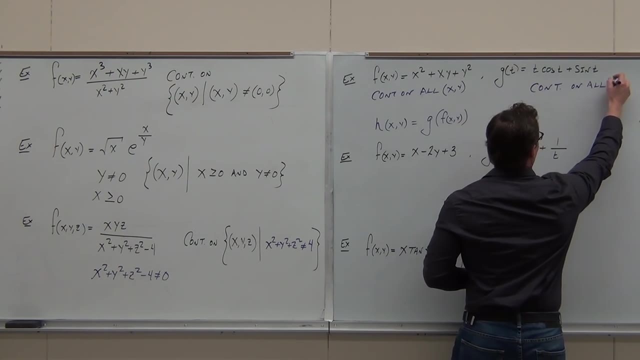 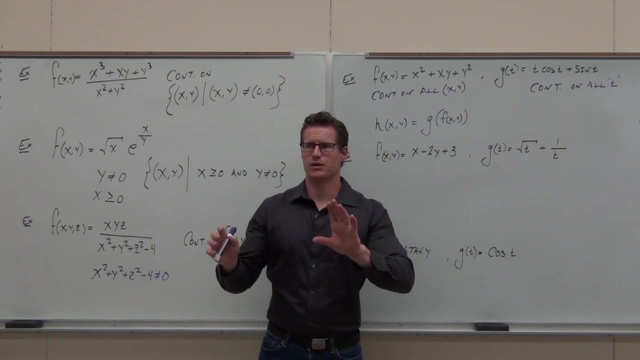 Continuous. It's continuous to t. It's continuous to t right here. Continuous on all t. Here's what I want to tell you. If this, please watch carefully what we're going to do. You're not watching. you should be watching. 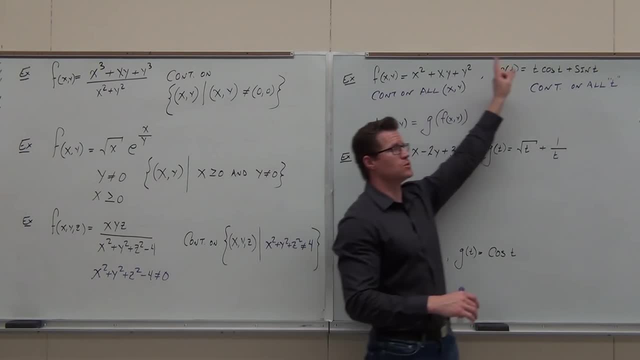 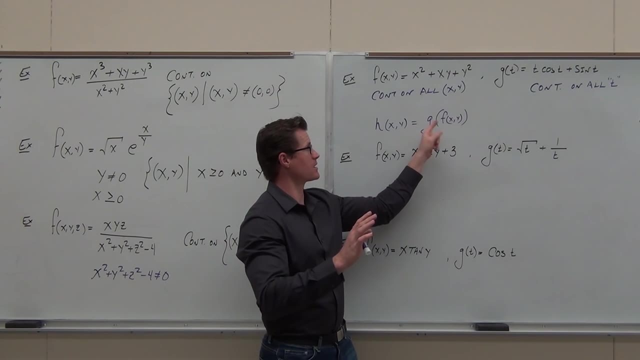 Please watch carefully. We're going to be taking this function and plugging it into this function. Does that make sense? Everything would be ending with x's and y's. The t's would disappear. That's what this says. Replace t's with xy stuff. 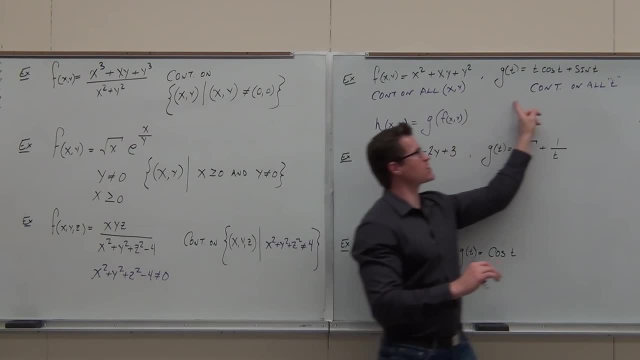 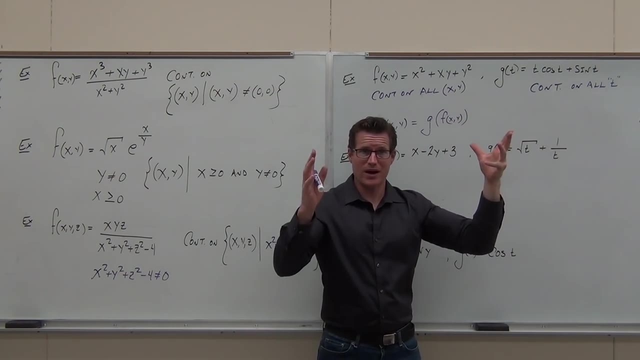 You get me So lots of xy's. If this is continuous everywhere, and this is continuous everywhere, tell me where. this is continuous Everywhere, Everywhere. But we're going to be in terms of whatever that says, So a to xy. that's why it says xy. 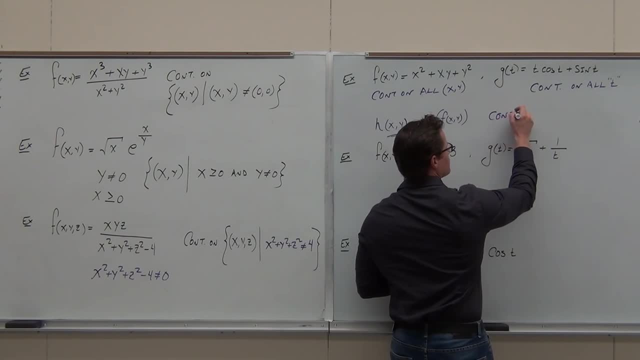 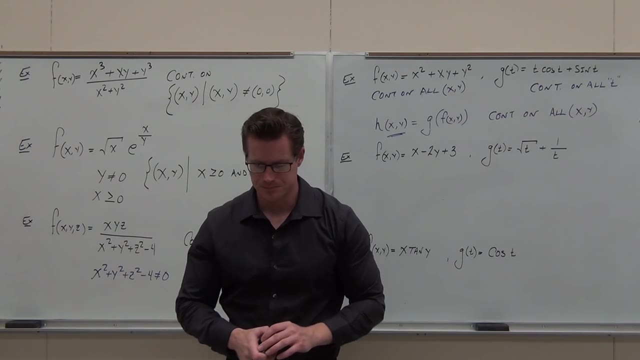 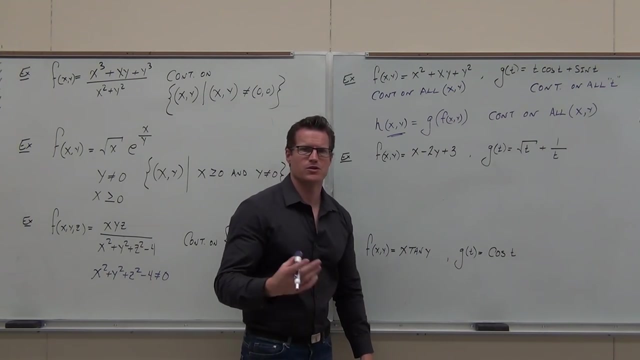 because you're going to be ending with xy's. This would be continuous, also on all ordered pairs. Does that make sense to you, that track? Yes, Now let's try this one. It's a little bit more complicated. The first part's really easy. 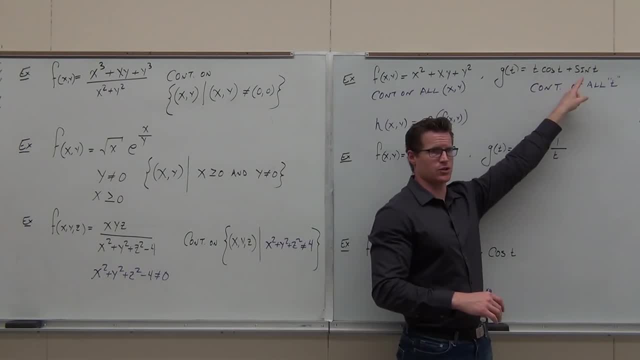 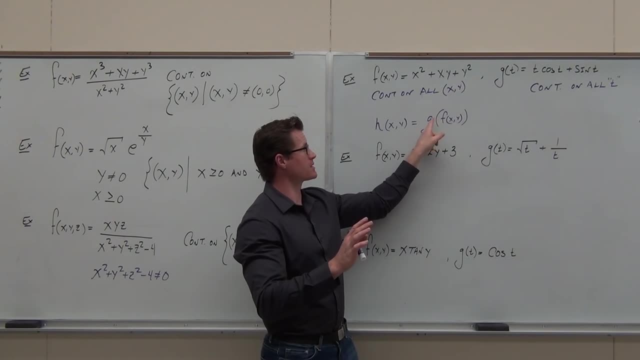 We're going to be taking this function and plugging it into this function. does that make sense? Everything would be ending with x's and y's. the t's would disappear. That's what this says. replace t's with xy stuff, you get me. 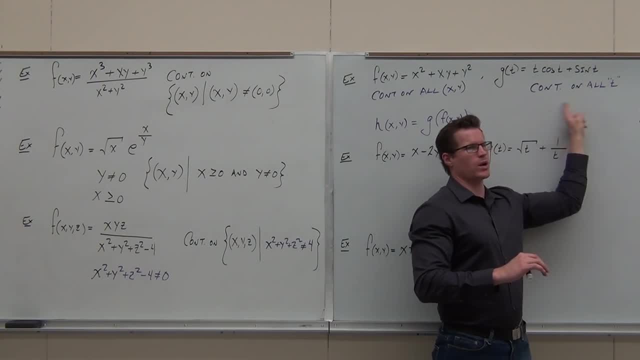 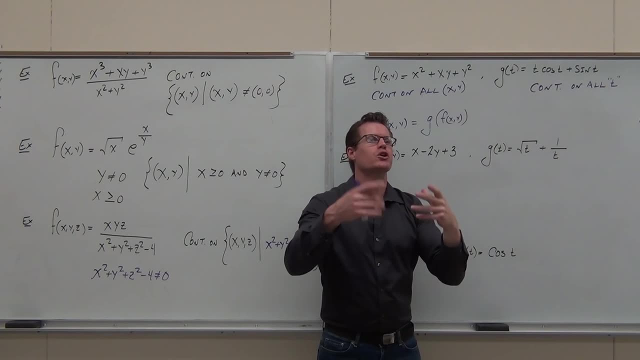 So lots of xy's. If this is continuous everywhere, and this is continuous everywhere, you're going to get a lot of xy's Everywhere. tell me where this is continuous: Everywhere, Everywhere. but we're going to be in terms of whatever that says. 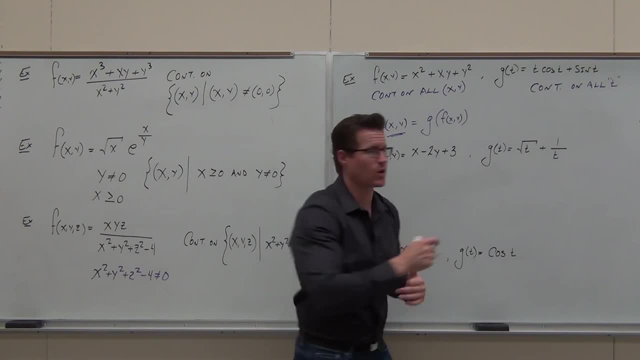 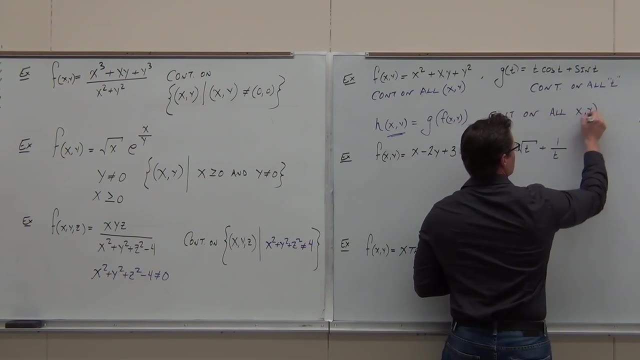 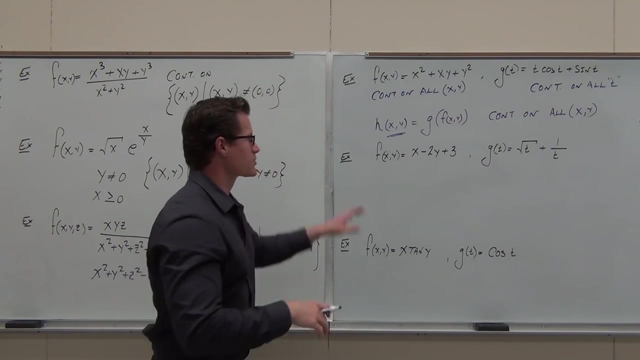 So a to xy. that's why it says xy, because you're going to be ending with xy's. This would be continuous, Also on all ordered pairs. Does that make sense to you, that track with you? Now let's try this one. it's a little bit more complicated. 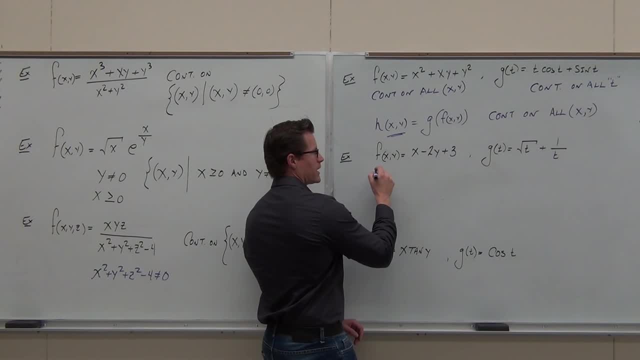 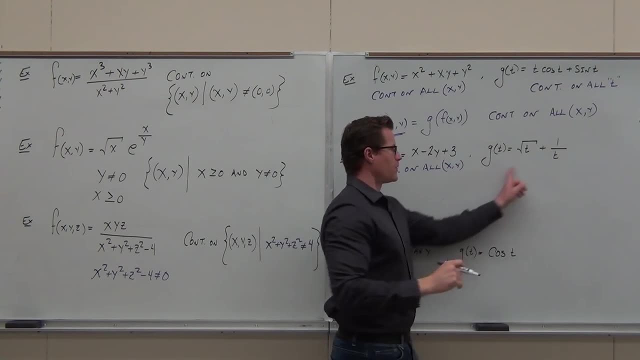 The first part's really easy: True or false? this is continuous on all xy's. No Yes, True or false. this is continuous on all t's. yes or no, No, False. Oh, Continuous on t, such that what? 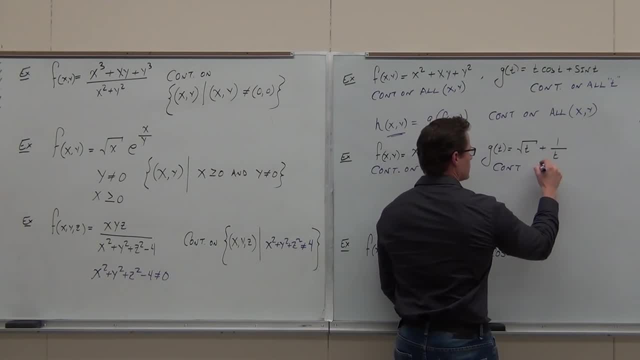 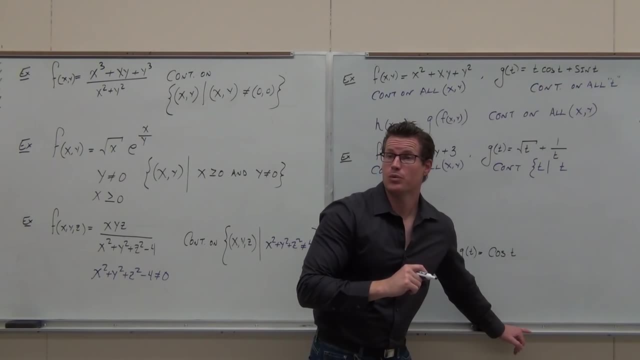 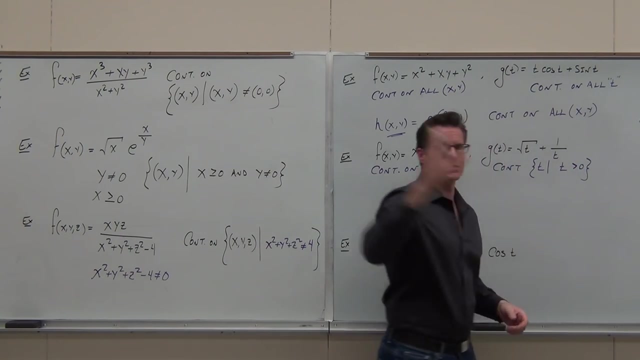 Zero, Such that t is Greater than zero. Yes, make it really simple. This says greater than or equal to zero. this just takes away the equal, So it makes me feel okay with that one. Now here's what's going on. 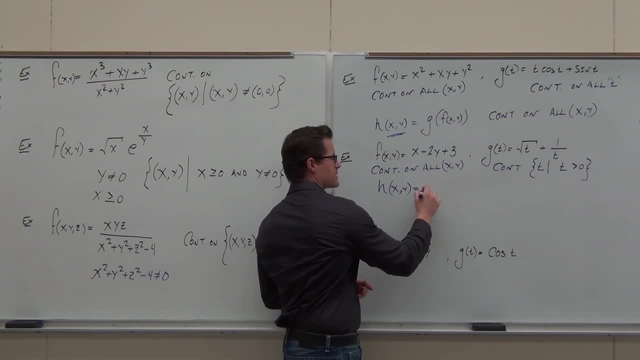 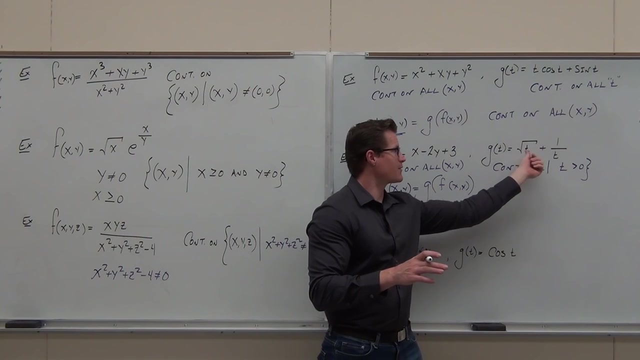 When we find the continuity for h of xy such that this equals g of f of xy. what this says again: take your f function and plug it into your t function. Here's what that means. It means every place you have t. what are you going to have? 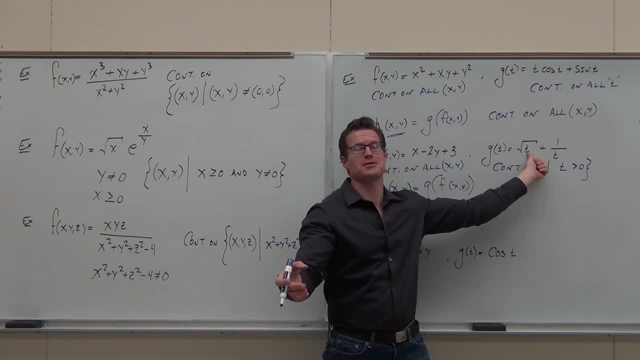 You're not expecting t. You're not expecting t. You're not going to be excited. You should be excited Every place you got t. you're going to have what? No, you're not going to have xy, You're going to have an entire function. 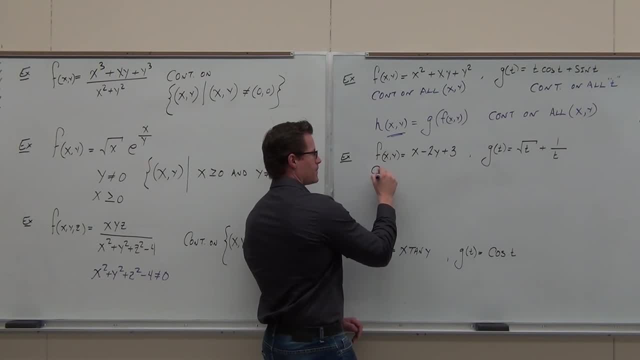 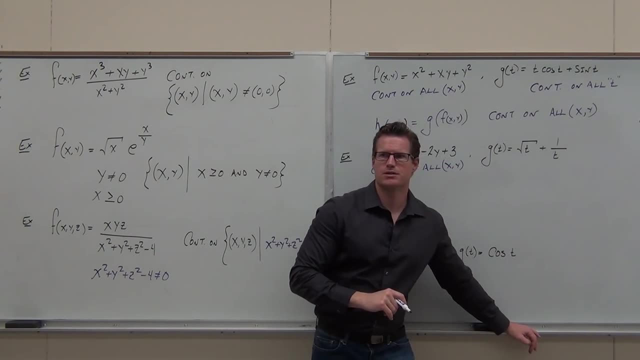 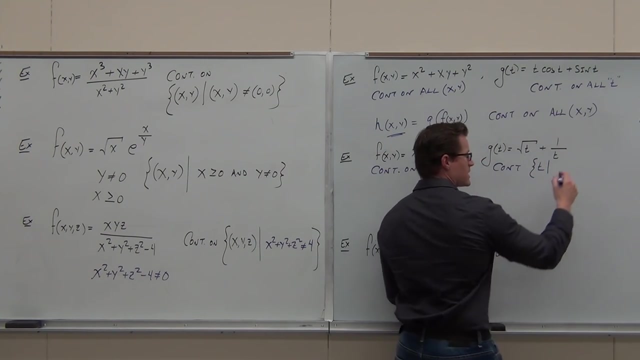 True or false. this is continuous on all xy. Yes or no. Yes, True or false. this is continuous on all t, Yes or no. False. Continuous on t such that: what Zero? Zero Such that t, T is greater than or equal to zero. 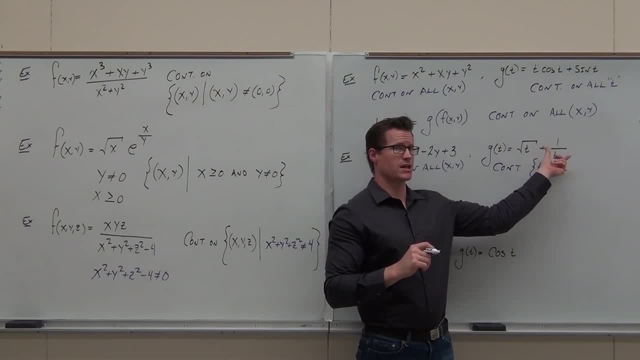 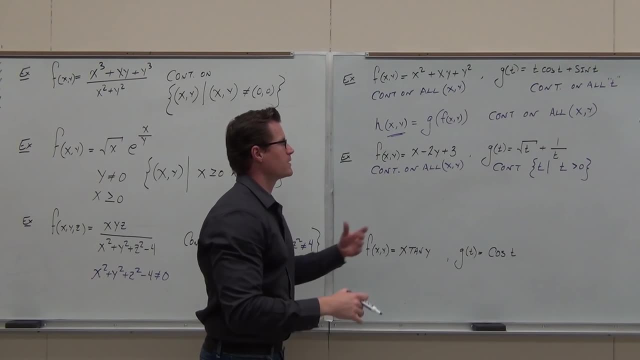 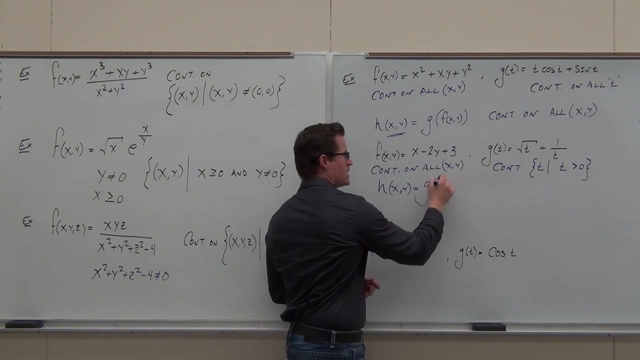 Let's make it really simple. This says greater than or equal to zero. This just takes away the equal. So if that's real key with that one, Now here's what's going on. When we find the continuity for h of xy such that this equals g. 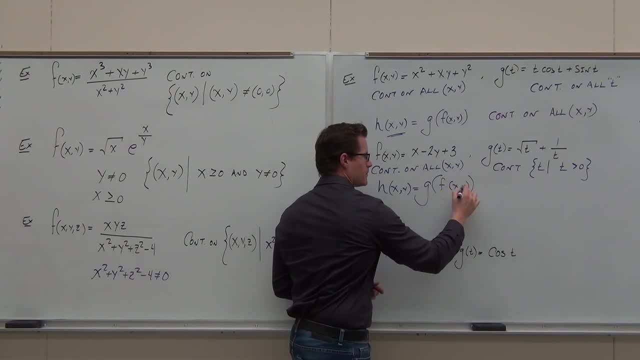 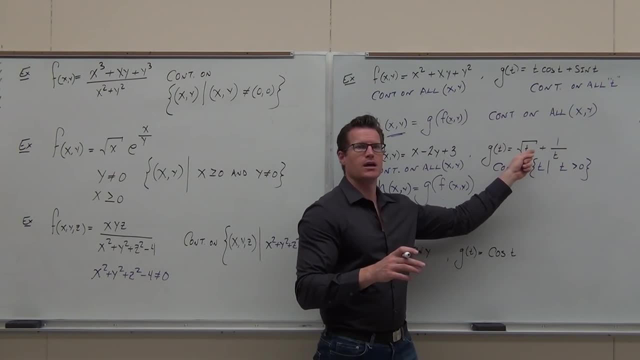 of f, of xy, what this says again, take your f function and plug it into your t function. Here's what that means. It means every place you have t. what are you going to have? You're not excited. You should be excited. 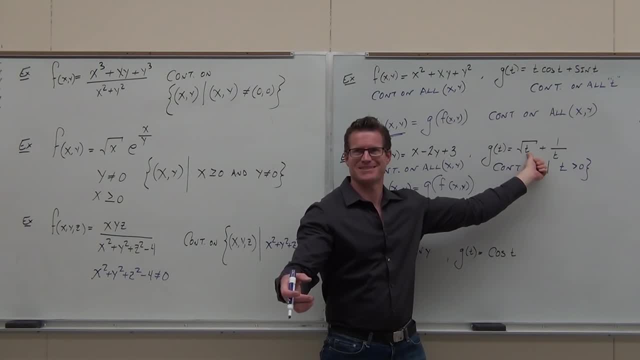 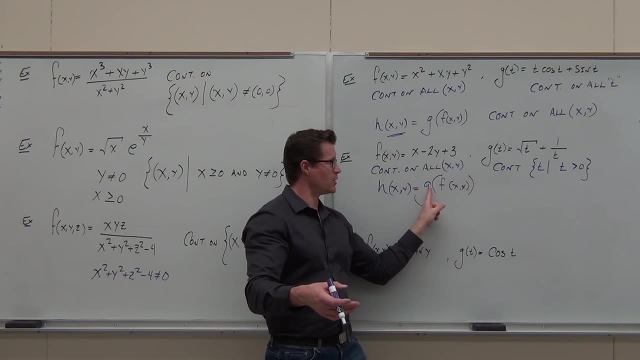 Every place you got t, you're going to have what. No, you don't have xy, you're going to have an entire function. What entire function? This says for every variable in this function. you're going to plug in this entire freaking function. 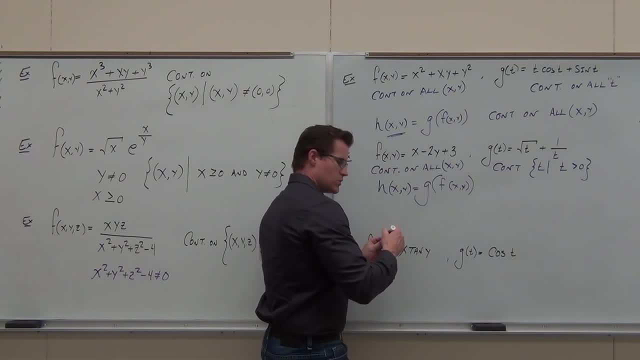 There and there. Does that make sense? In other words, you're going to let T equal x minus 2y plus 3.. 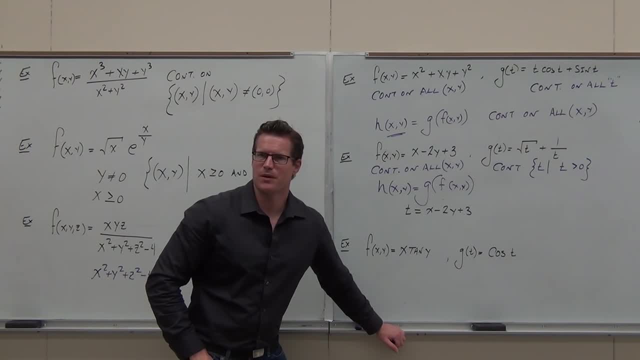 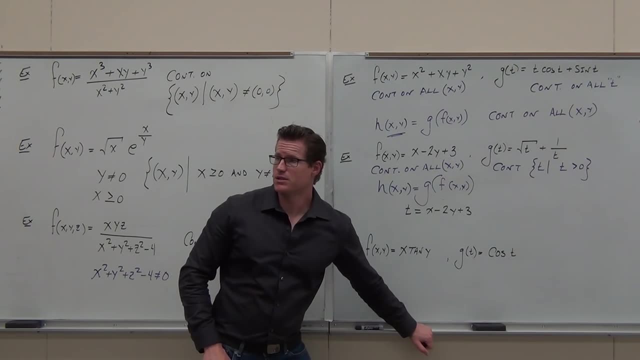 Does that make sense to you? Now, here's the magic part about that. What do you know about t? Read it. What do you know about t? It's got to be greater than 0. So that means that t must be greater than 0.. 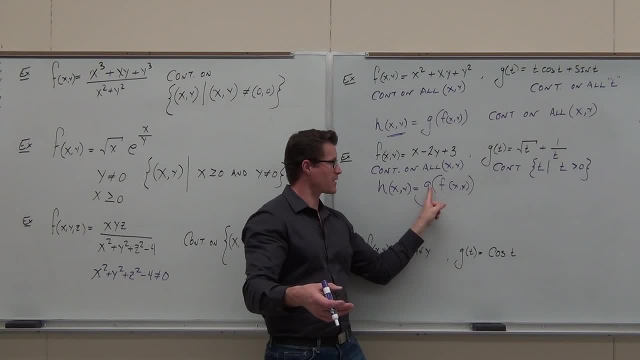 What entire function This says for every variable in this function. you're going to plug in this entire freaking function There and there. Does that make sense? In other words, you're going to let t equal x minus 2y plus 3.. 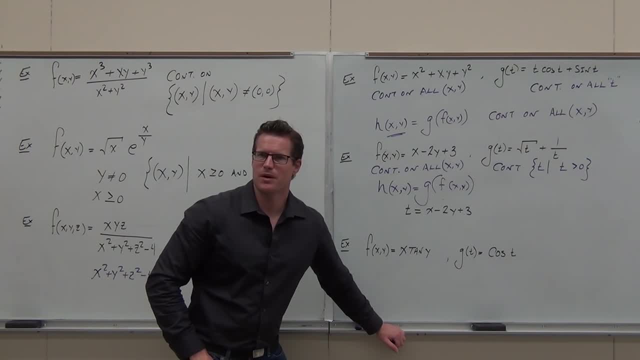 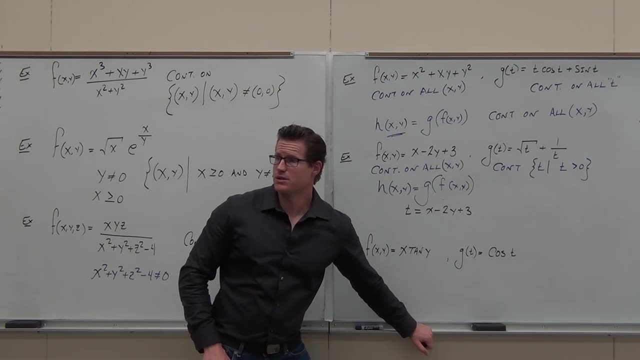 Does that make sense? Does that make sense to you? Now, here's the magic part about that. What do you know about t? Read it. What do you know about t? It's got to be greater than zero. So that means that t must be greater than zero. 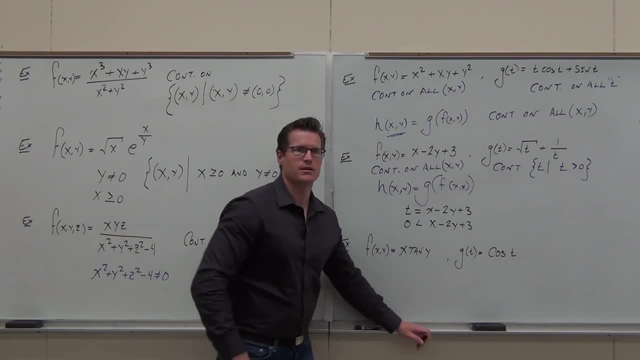 Therefore, this thing must be greater than 0.. If you can see that substitution, then you've got it made. Can you see how to get from here to here? T is going to equal this right, because we're going to take that function and plug it in for t. 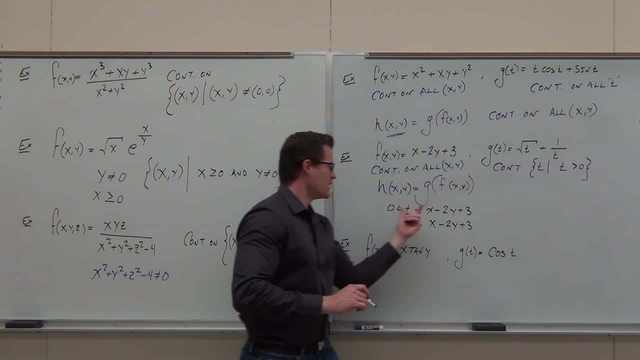 If t has got to be greater than 0 by what we have, if t has got to be greater than 0 and t equals this thing, then this thing has got to be greater than or equal to 0.. Why are we doing that in terms of x and y? 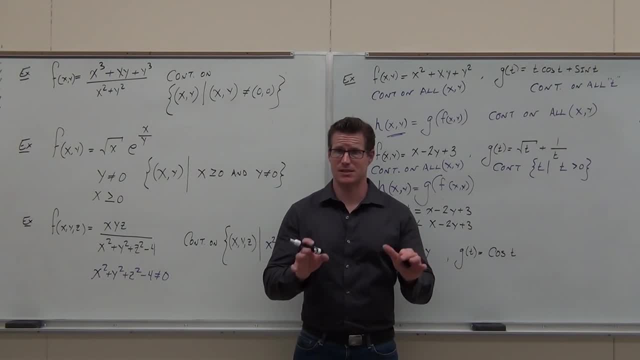 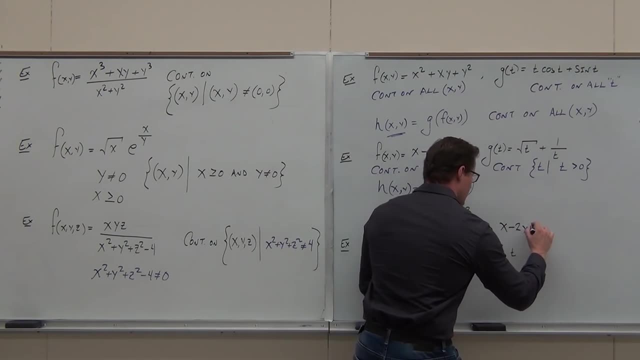 Because the function is going to end in terms of x and y. Does that make sense? Now, solve it, Do something. Just subtract the 3 or something. So we've got x minus 2y is greater than yeah. I flipped it around. 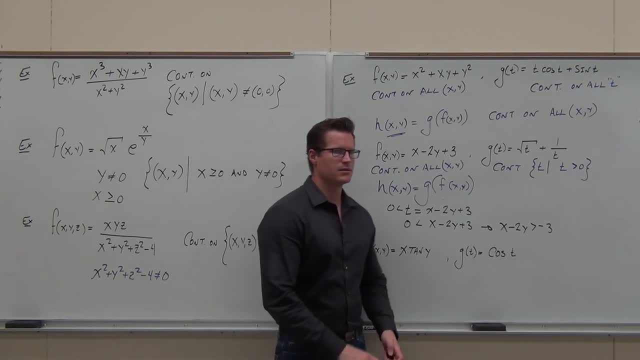 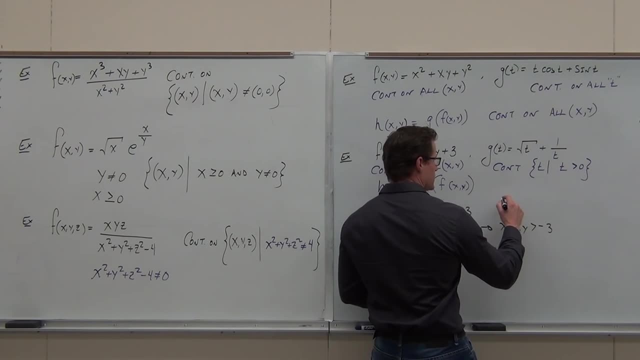 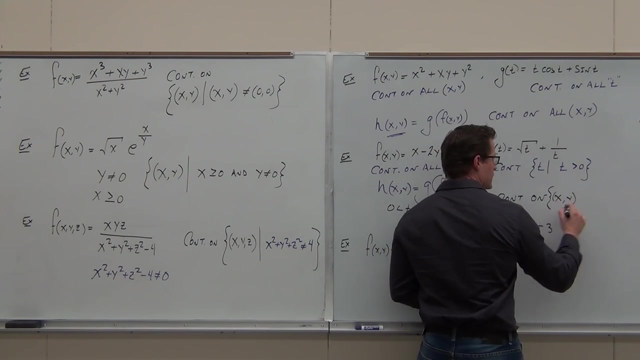 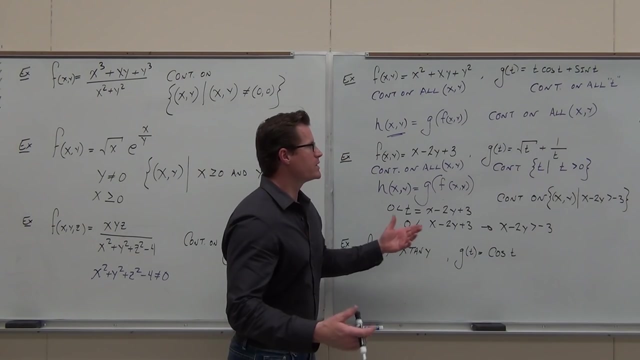 x minus 2y is greater than negative 3.. Does that make sense? So we found continuity. This will be continuous on all ordered pairs x- y, such that x minus 2y is greater than negative 3.. So what we do is we figure out continuity. 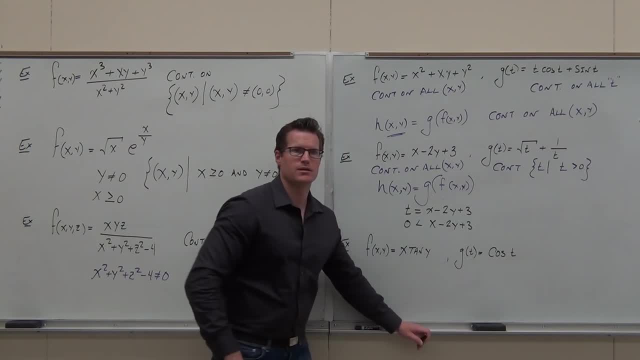 Therefore, this thing must be greater than zero, Can you? if you can see that substitution, then you've got it made. Can you see how to get from here to here? t is going to equal this right, because we're going to take that function and plug it in for t. 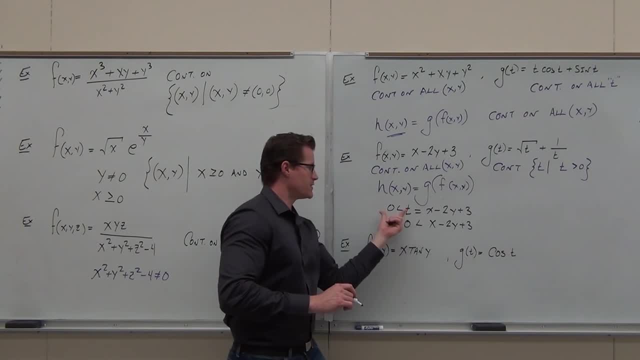 If t has got to be greater than zero, If t has got to be greater than zero by what we have, if t has got to be greater than zero and t equals this thing, then this thing has got to be greater than or equal to zero. 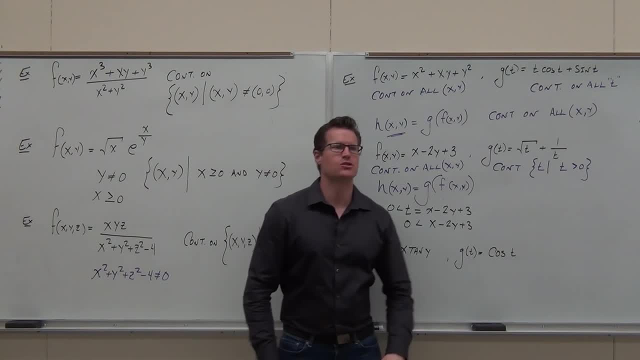 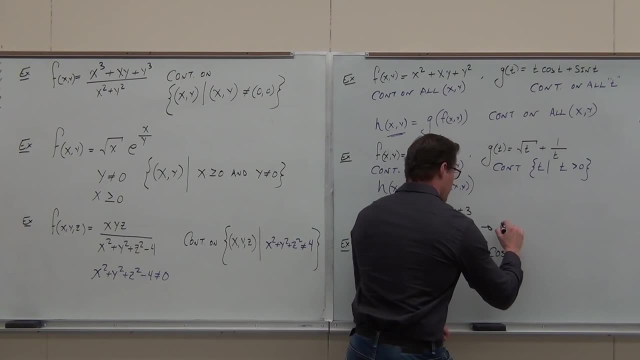 Why are we doing that in terms of x and y? Because the function is going to end in terms of x and y. Does that make sense? Now, solve it. Do something. Just subtract the 3 or something. So we've got x minus 2y is greater than yeah. I flipped it around. 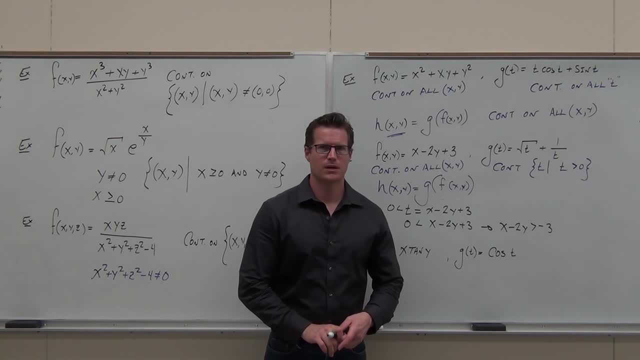 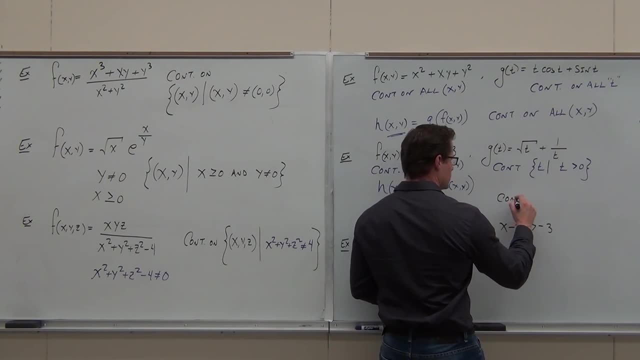 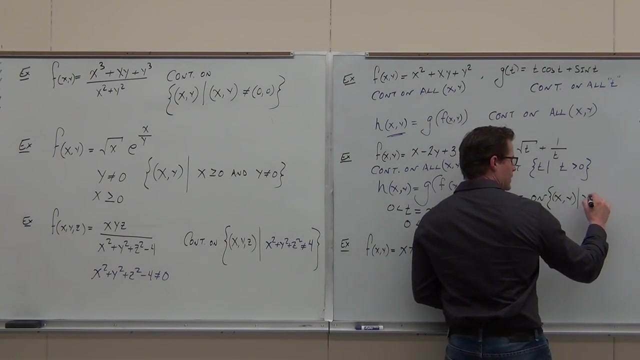 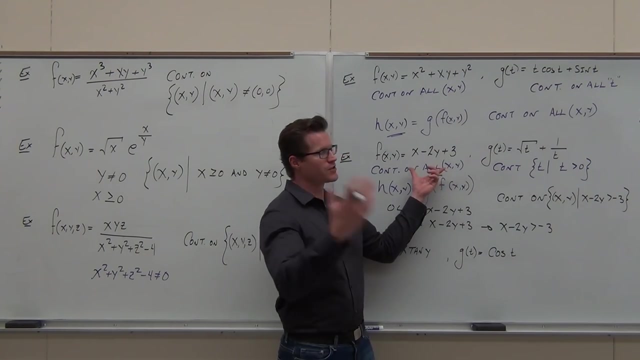 x minus 2y is greater than negative 3.. Does that make sense? Yeah, So we found continuity. This will be continuous on all ordered pairs x- y, such that x minus 2y is greater than negative 3.. So what we do is we figure out continuity. 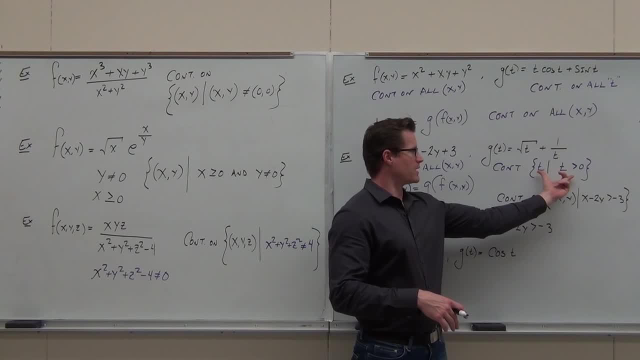 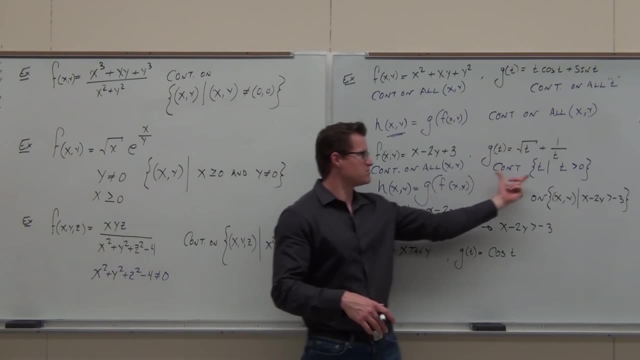 If it's all real numbers, great, All ordered pairs, I should say: Figure out continuity here, If it's not just set the parameter equal to what you're plugging in for that parameter, And then you have this: It's an equality. 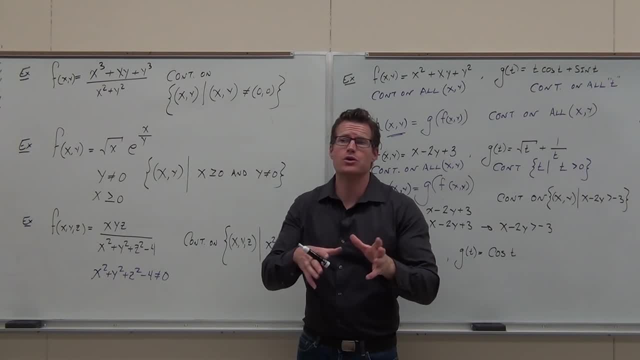 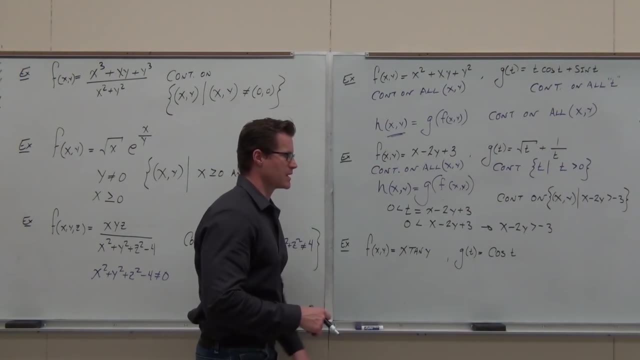 Solve for the inequality And you have the domain and the continuity for that second composed function. That one. Now, last one, This is going to be the opposite case. Let's start here. Is this continuous on all t, Yes or no? 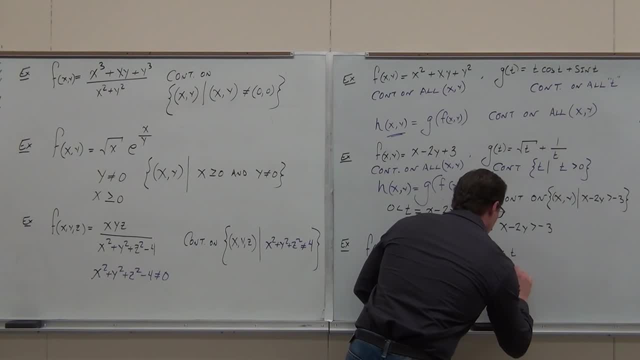 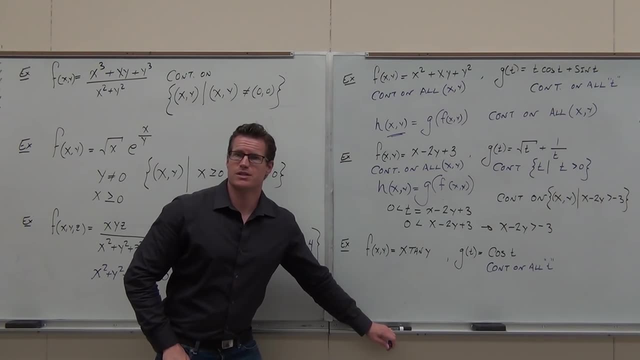 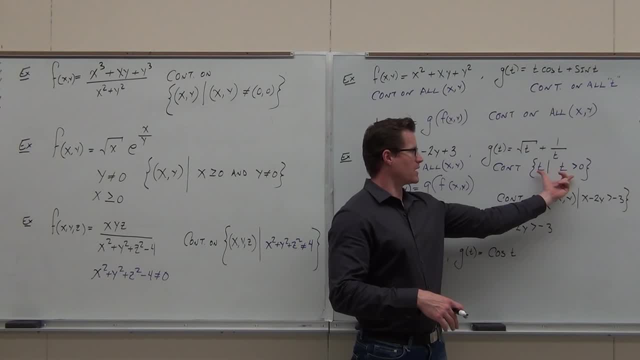 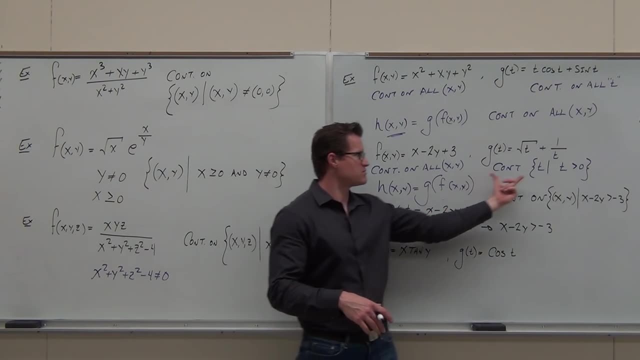 If it's all real numbers, great, All ordered pairs, I should say. Figure out continuity If it's not just set the parameter equal to what you're plugging in for that parameter, And then you have this inequality. Solve for the inequality. 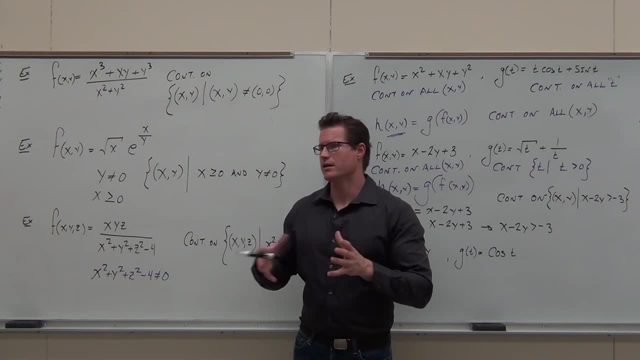 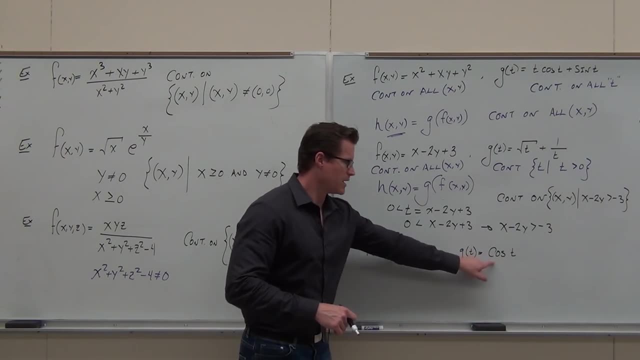 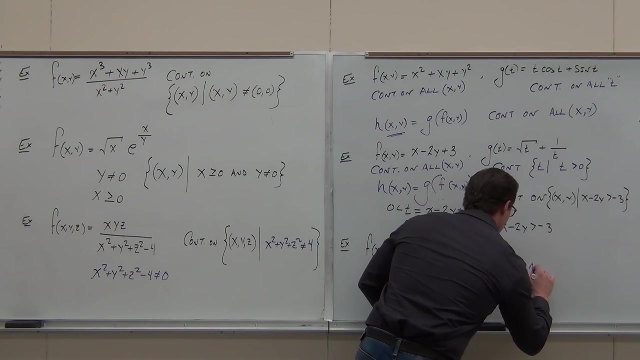 And you have the domain and the continuity for that second composed function, That one. Now, last one, This is going to be the opposite case. Let's start here. Is this continuous on all t? Yes or no? Yes, Is this continuous? 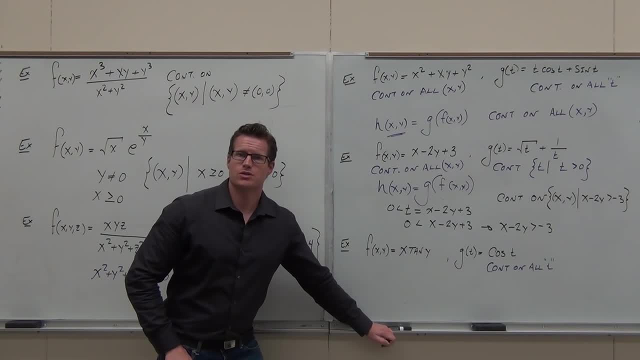 Yes, Notice it's everywhere. No, Notice it's tangent. Is it continuous on all x? Yes, Continuous on all y? No, What's wrong with it? Isomtotes. Isomtotes where Pi over 2.. 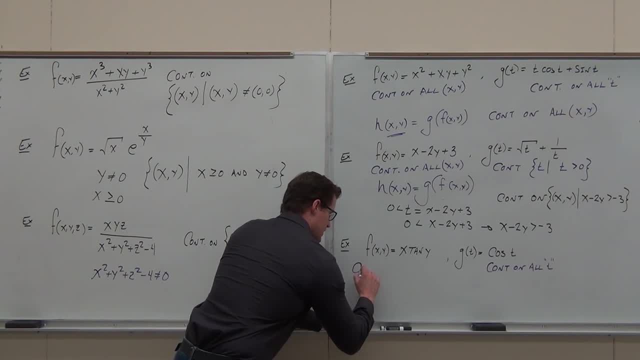 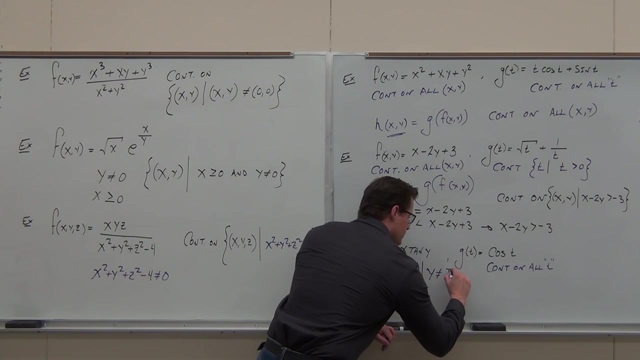 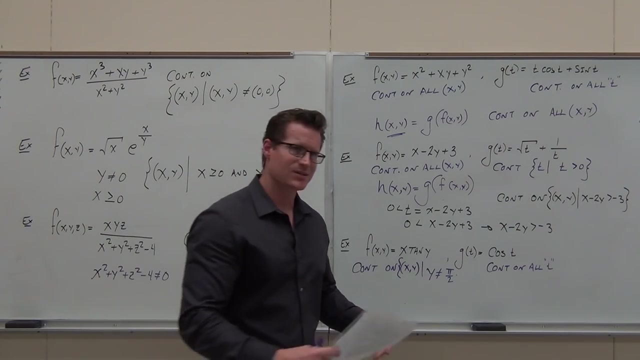 All values of pi over 2.. So we have- this is continuous on ordered pairs- x, y, such that x- I don't care about, X- is good, But I just can't have y equaling pi over 2.. I can't have y equaling pi over 2 or any multiple of that. 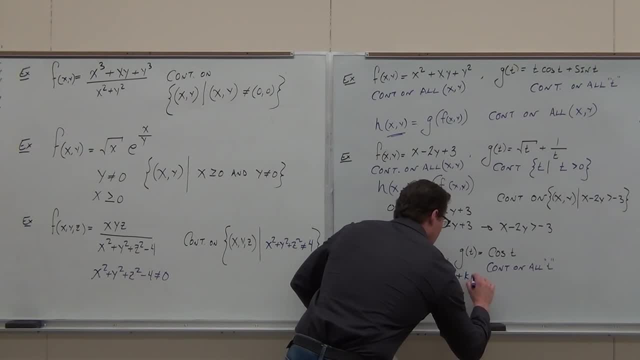 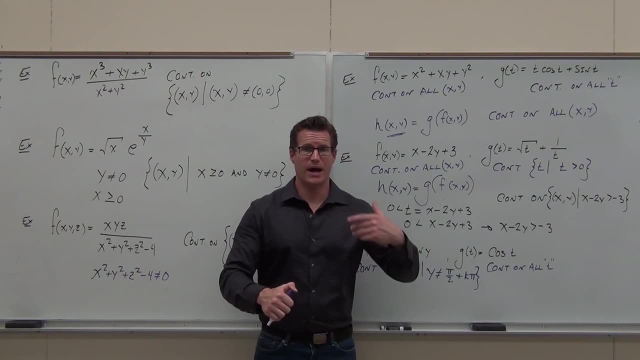 So we're going to say plus k pi And what that says is if you add or subtract pi to it, you still have a problem. Any multiple where k is an integer Pi, you go. okay. so negative pi over 2.. 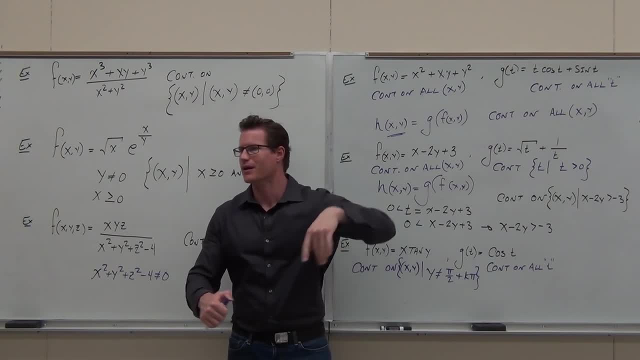 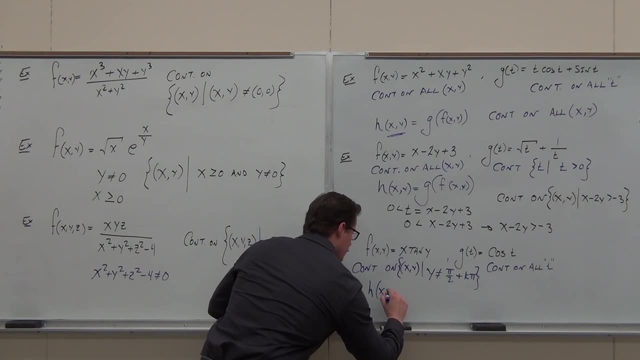 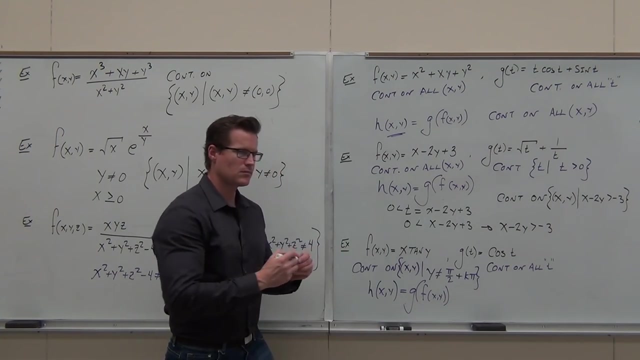 Or 3 pi over 2. Or any circle, any like half circle around there. You can't have any of those Now, here's the deal. Here's the deal. Watch carefully If I want to talk about This. 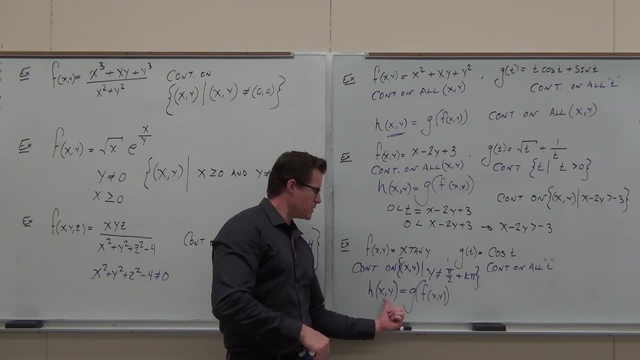 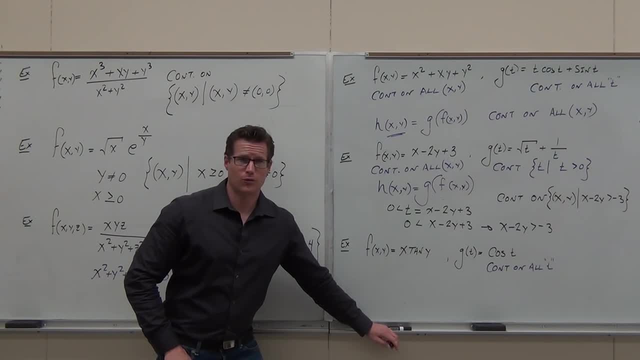 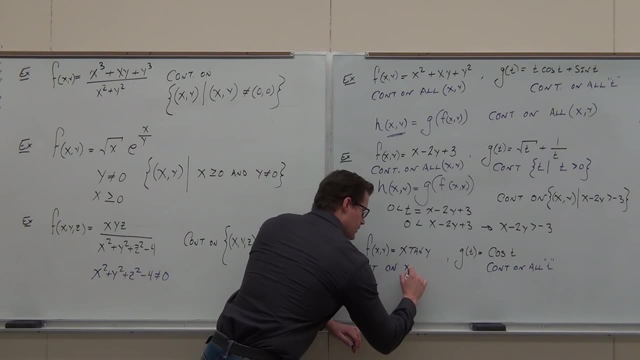 Isomtotes where Pi over 2. All values of pi over 2.. So we have- this is continuous on ordered pairs- x, y, such that x- I don't care about, X- is good, but I just can't have y equaling pi over 2.. 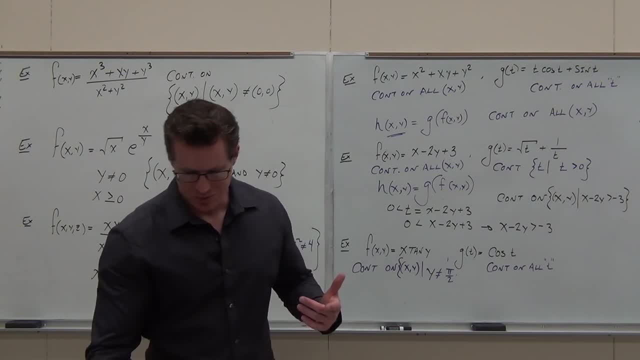 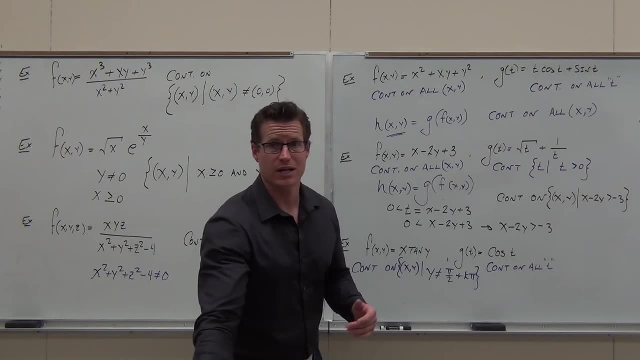 I can't have y equal to pi over 2 or any multiple of pi over 2.. I can't have y equal to pi over 2 or any multiple of that. so we're going to say plus k pi, And what that says is: if you add or subtract pi to it, you still have a problem. 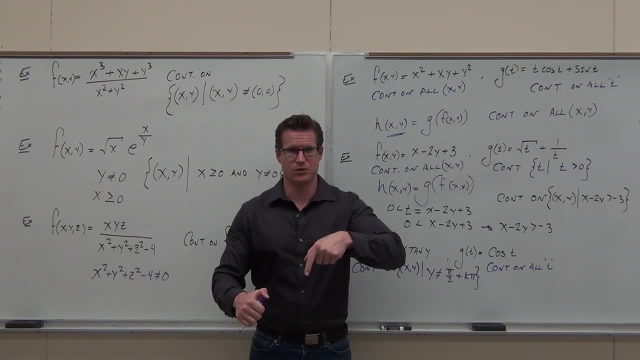 Any multiple where k is an integer pi, you go. okay, so negative pi over 2 or 3, pi over 2 or any circle, any like half circle around there. You can't have any of those. No, here's the deal. 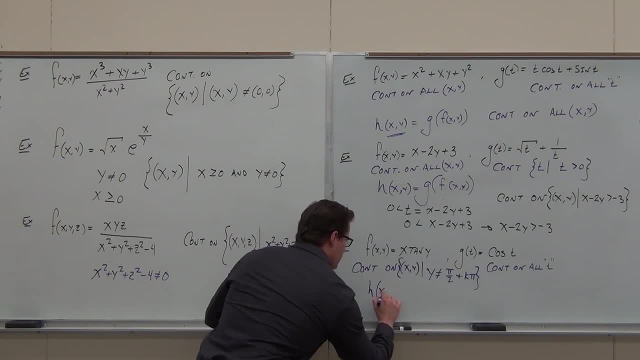 Here's the deal. Watch carefully, If I want to talk about this, This, This, This, This, Here's what I want you to see. This is going to be in terms of x- y, correct? Is this going to add any more continuity issues to this situation? 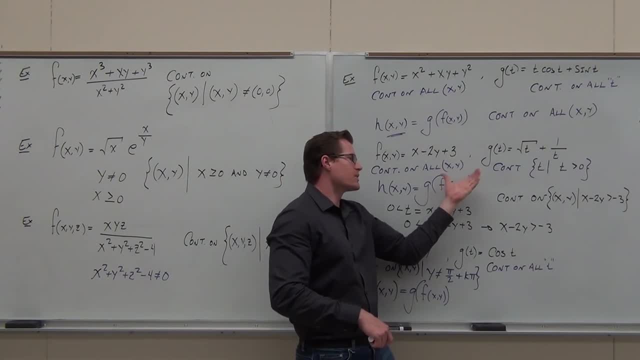 So this added, okay, this said I have continuity issues that I didn't, So we have to set it equal to this continuity issue. We have to figure it out. If I say I'm taking this whole thing and I'm just going to substitute this in for T, This 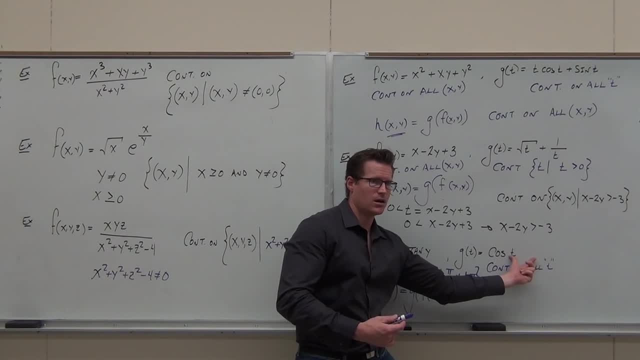 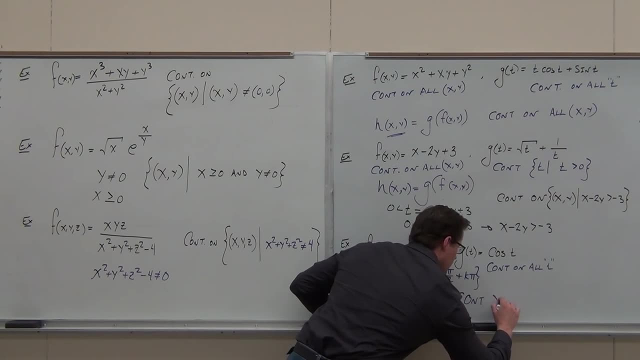 doesn't add any more problems. All it says is that, yeah, you're going to have. you know, this is the derivative of pi over 2.. You're going to have continuity, basically the same region. you had this. This was the only problem there. 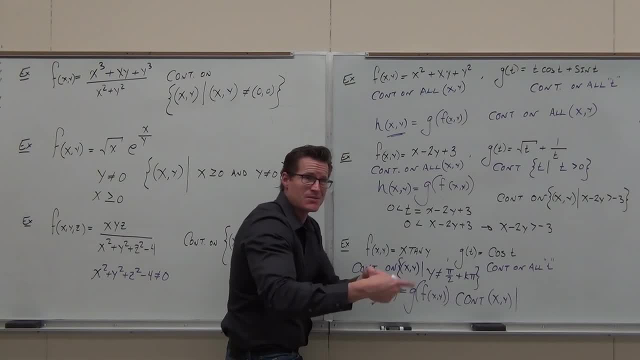 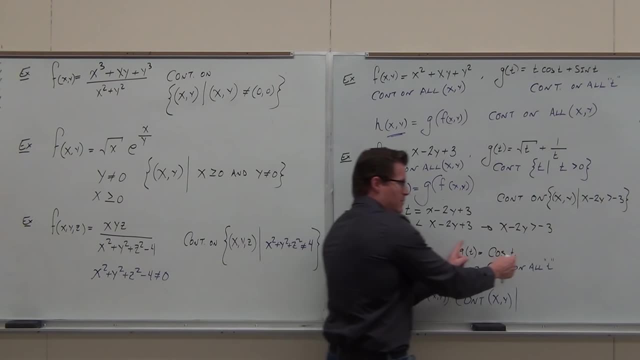 It was already in terms of x's and y's, so it's going to be the exact same value of points. Does that make sense to you? The cosine is continuous everywhere. It's not making a difference for us. It's this piece that, even when I put it here, I still can't have the y equally in those multiples of pi over 2.. 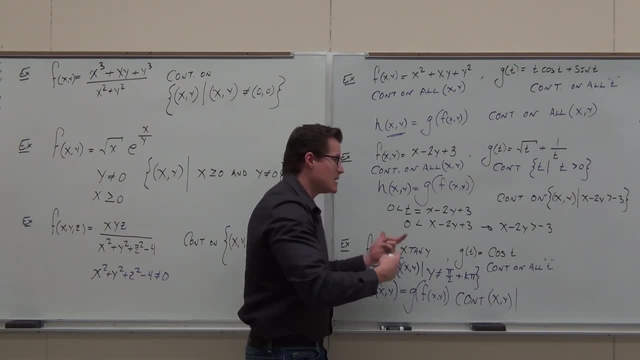 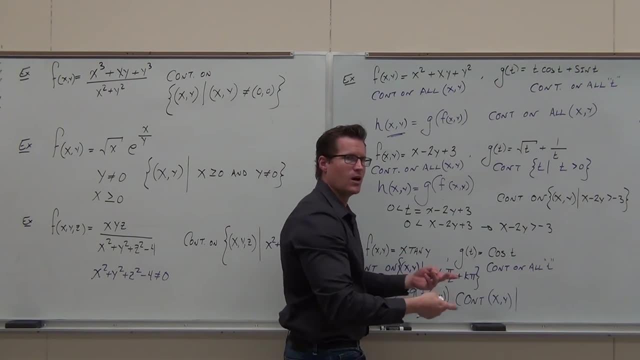 Do you guys catch that? So, composing, you basically keep the same continuity. Sometimes you have to work with it and say, okay, well, my t's are changing to x's and y's, Figure that out. But for the most part we just take continuity from both of them and kind of jam them together. 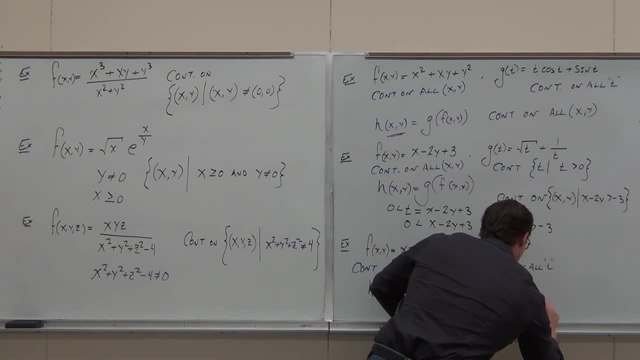 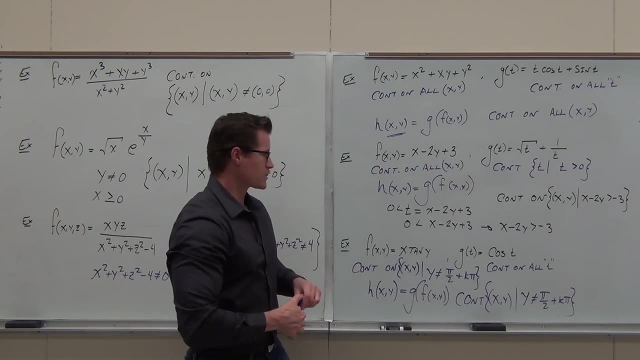 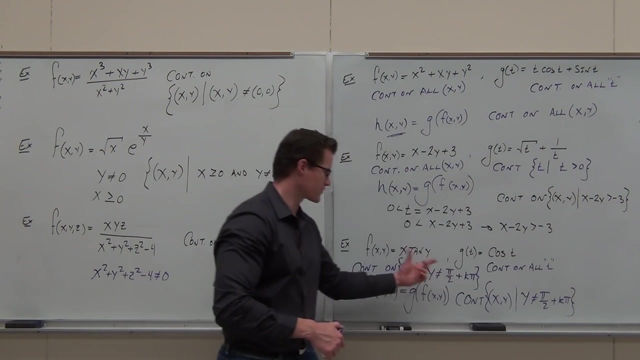 That's basically what we're doing. So this says continuous everywhere. That means I'm not going to have any issues when I plug into this function, But I'm not going to have any issues when I plug into this function. We look at this function and go, okay, this is what I'm plugging into that. 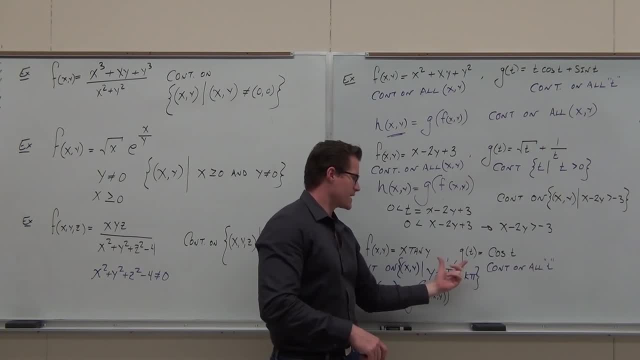 So we have to set it equal to this continuity issue and we have to figure it out. If I say I'm taking this whole thing And I'm just going to substitute this in here, I'm just going to substitute this in for t. 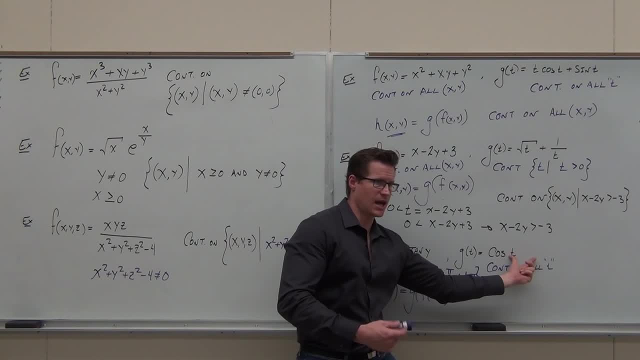 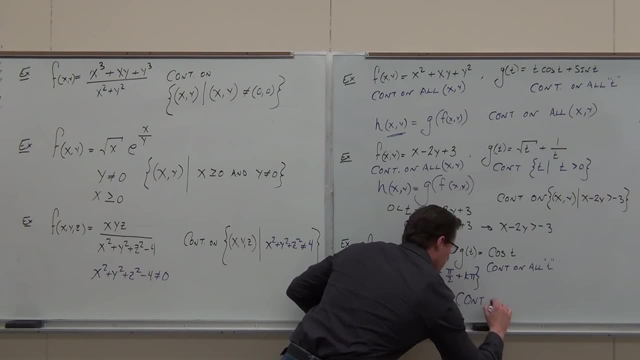 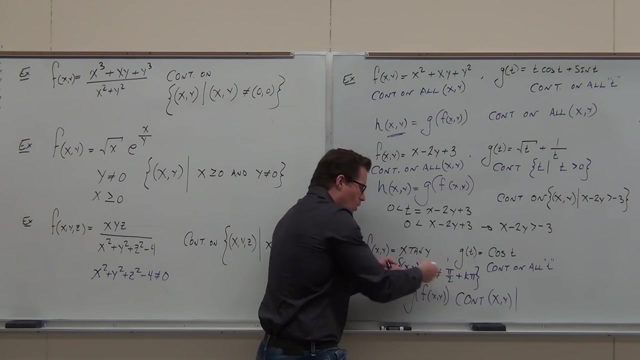 This doesn't add any more problems. All it says is that, yeah, you're going to have, you're going to have continuity, Basically the same region. you had this. This was the only problem there. It was already in terms of x's and y's. 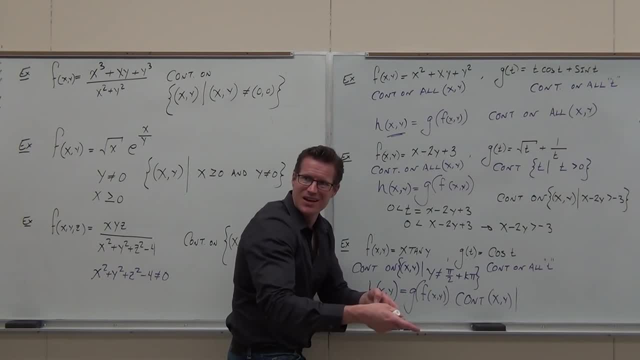 So it's going to be the exact same value of points. Does that make sense to you? The cosines continue to stay everywhere. It's not making a difference for us. It's this piece That, even when I put it here, I still can't have the y equally in those multiples of pi over 2.. 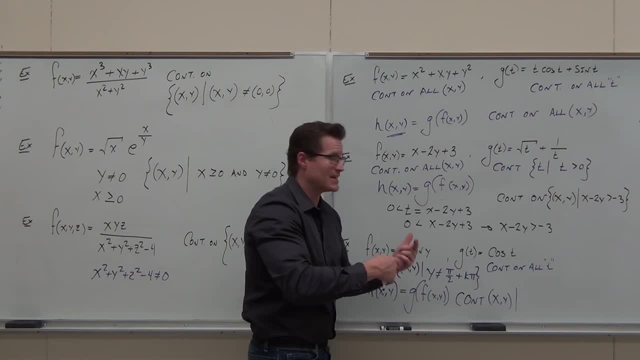 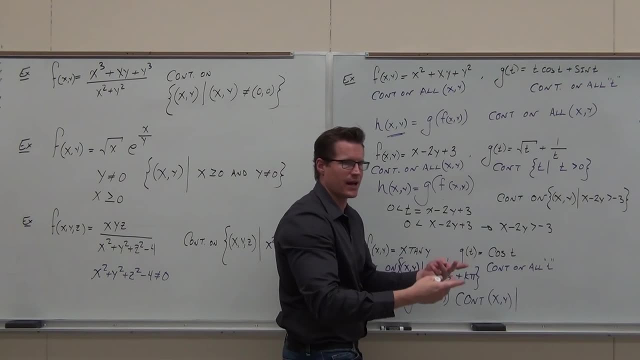 Do you guys catch that? So, composing, you basically keep the same continuity. Sometimes you have to work with it and say, okay, well, my t's are changing to x's and y's, Figure that out. But for the most part we just take continuity from both of them and kind of jam them together. 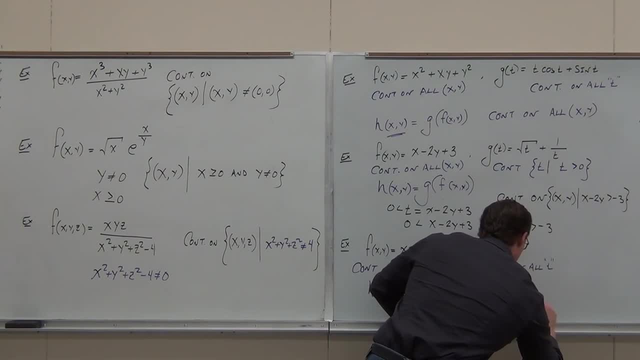 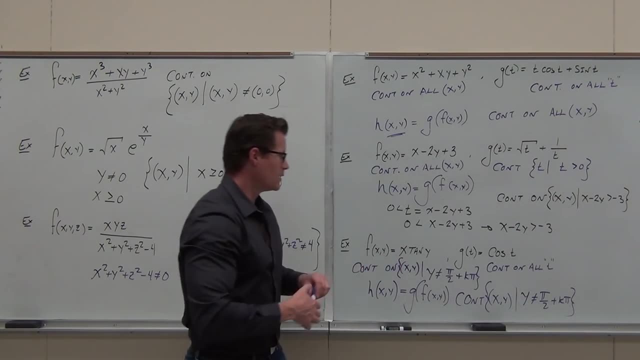 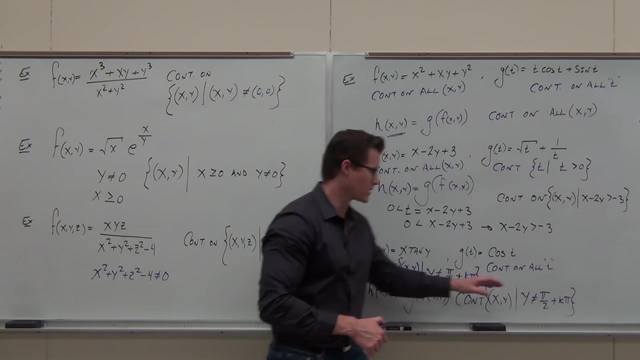 That's basically what we're doing. So this says continuous everywhere. That means I'm not going to have any issues when I plug into this function. But I'm not going to have any issues when I plug into this function. We look at this function. 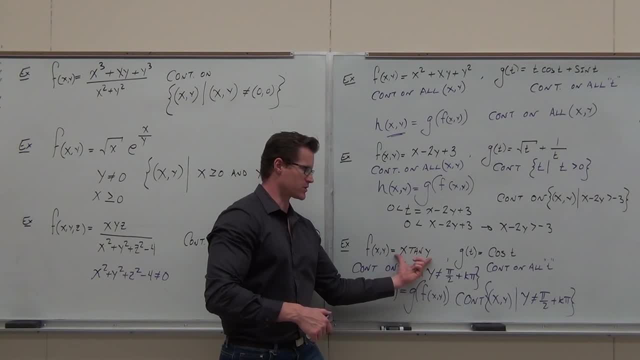 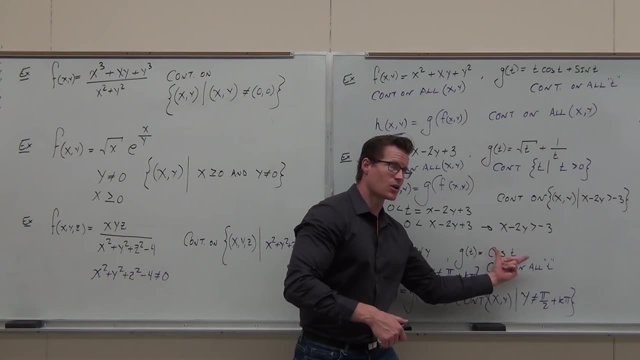 Okay, this is what I'm plugging into that. Where is this not continuous? Well, it's continuous everywhere, except this. Therefore, since this doesn't create any more issues, this is also continuous everywhere, except that, Should fans feel okay with that one. 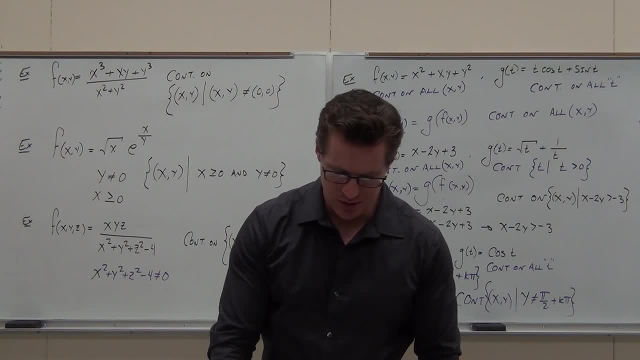 Okay, I promised you this. I promised that we were going to talk about the squeeze there. I'm going to show you one example. I said: you know what, When we started this, I said: it's really, really hard to prove that limits exist. 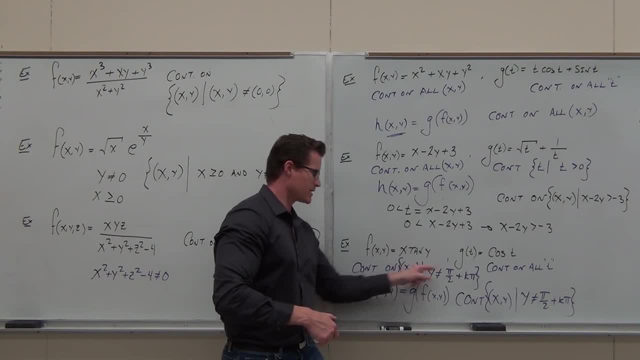 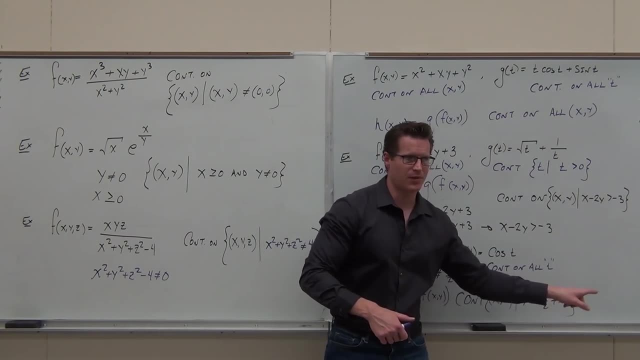 Where is this not continuous? Well, it's continuous everywhere, except this. Therefore, since this doesn't create any more issues, this is also continuous everywhere, except that, Should fans feel okay with that one? Okay, I promised you this. I promised that we were going to talk about the squeeze there. 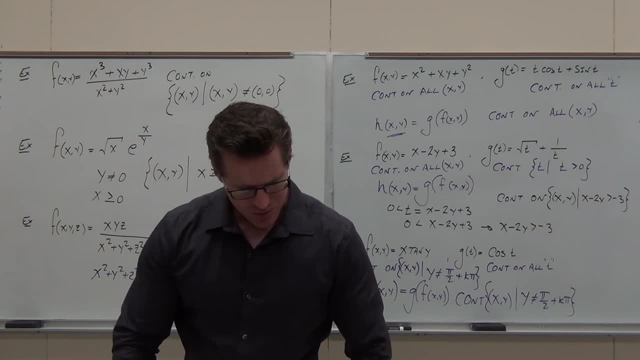 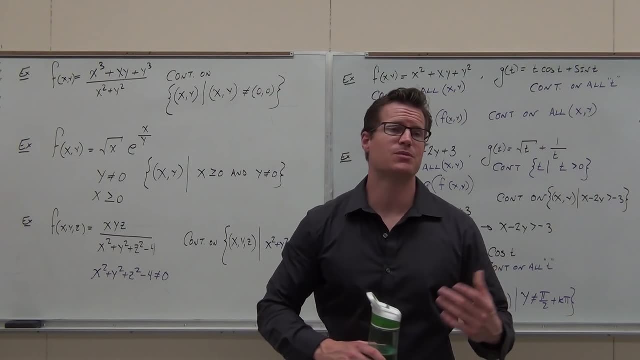 I'm going to show you one example. I said: you know, when we started this, I said: it's really really hard to prove that limits exist. It's really easy to prove they don't exist. We spent most of the time doing that. 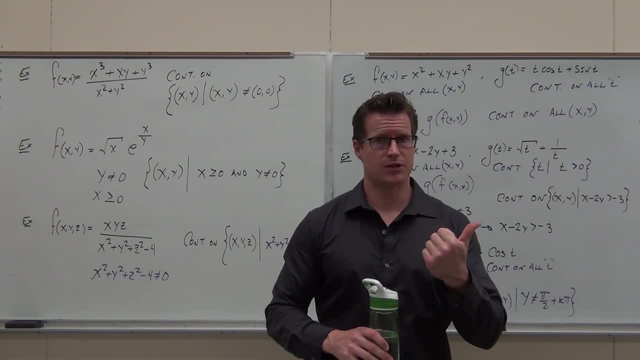 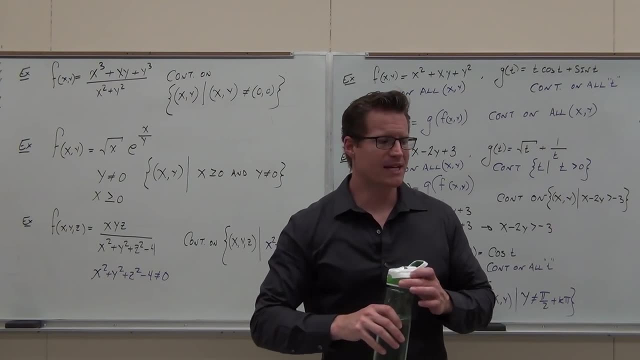 How we prove limits exist is by using continuity and just plugging in the number that uses continuity. We talked about that a little bit. We said if a function is defined, then it's got continuity. If it's got continuity, the limit exists. 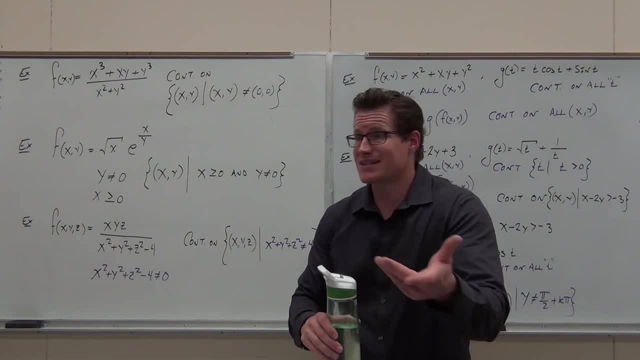 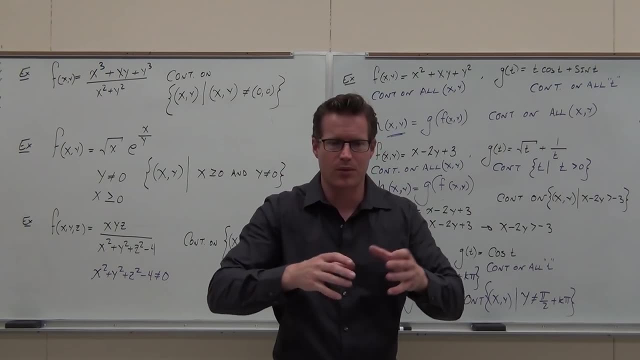 So just plug the number in And if the function is defined there, then it's continuous. there We talked about the region, We talked about how, if we're defined and we plug that point in over the defined region, then we find a neighborhood of points and we're continuous. 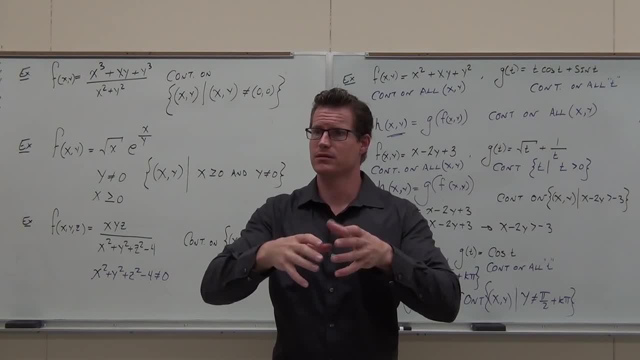 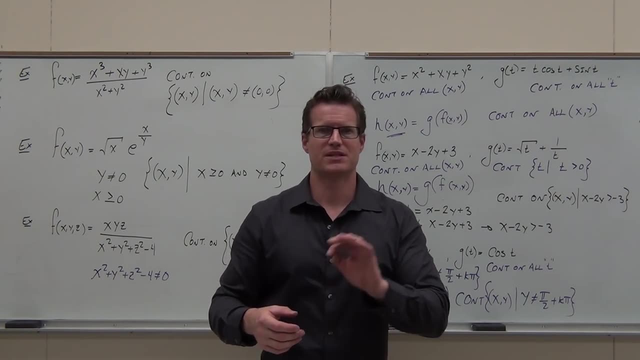 The limit has to exist. So if we're defined continuity, no problem, Just plug the number in. You got it. Well, what if we can't do that? and what if the limit still exists and we didn't have the magic trick of polar? 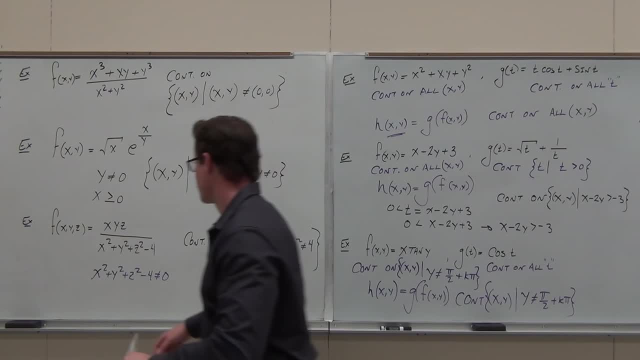 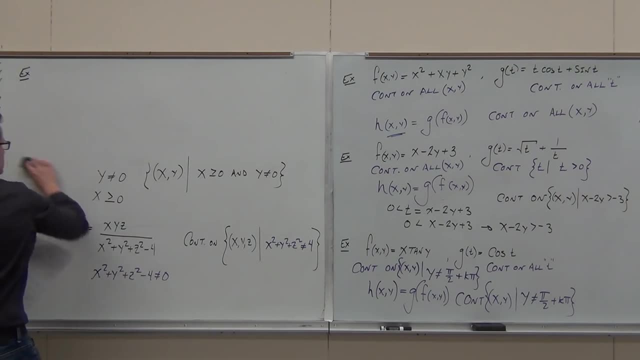 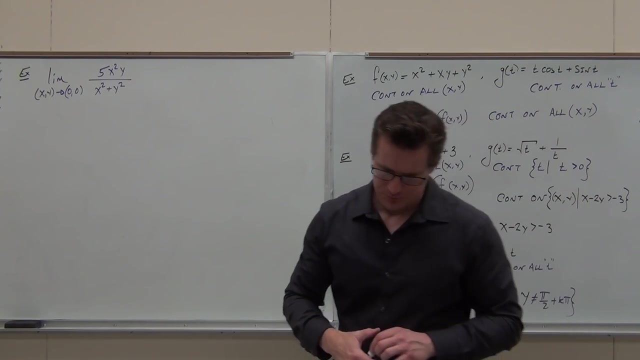 This is the case that you use. So if we go, if we don't have that stuck, for example, Let's talk about this limit, only one First thing you should always do with limits is what Plug them in. Plug it in. 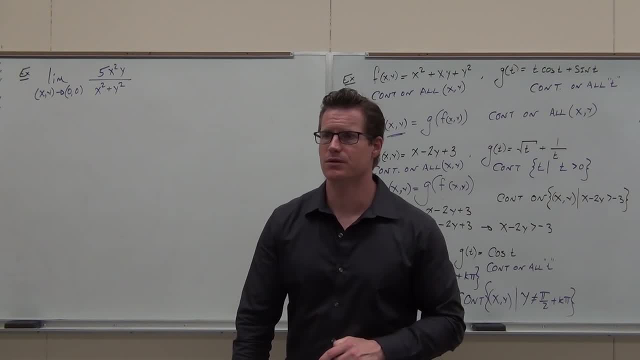 And you plug it in, you get zero over zero. You can verify that form if you want to. And then we go: okay, we're saying things: Don't Limits don't exist in this case, but this one does. How do you prove it? 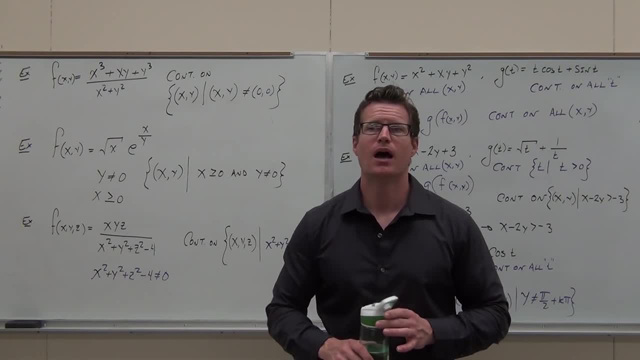 It's really easy to prove they don't exist. We spent most of the time doing that. How we prove limits exist is by using continuity and just plugging in the number that uses continuity. We talked about that a little bit. We said if a function is defined, then it's got continuity. 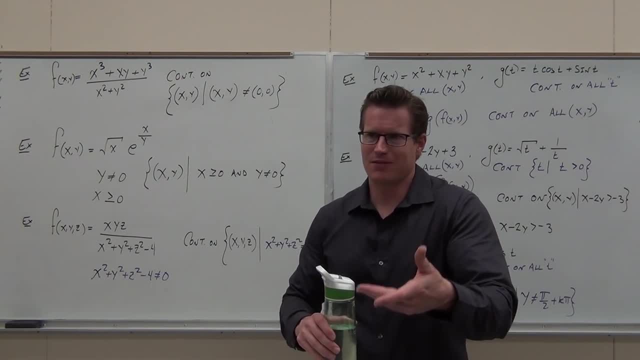 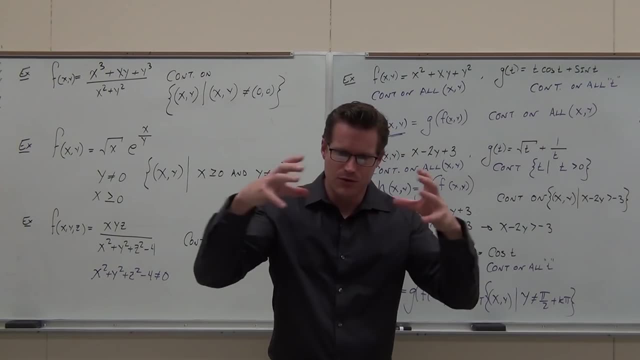 If it's got continuity, the limit exists. So just plug the number in And if the function is defined there, then it's continuous there. We talked about the region. We talked about how, if we're defined and we plug that point in over the defined region, 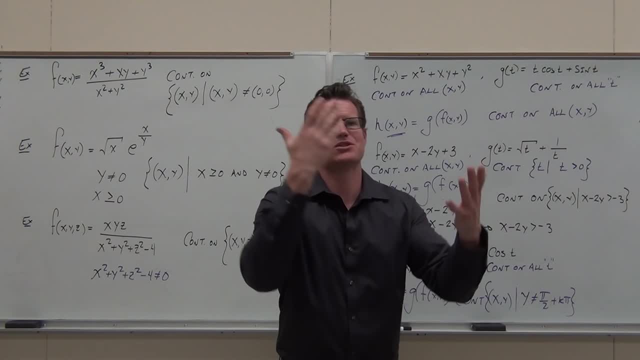 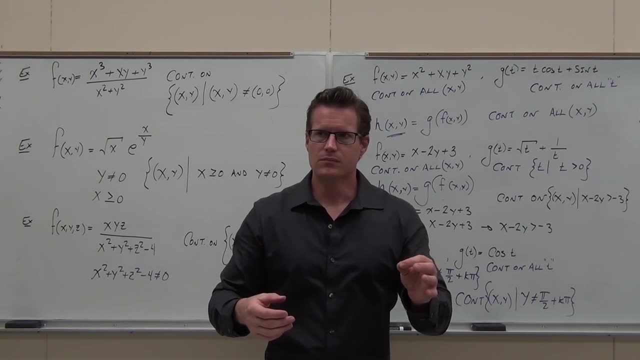 then we find a neighborhood of points and we're continuous there. The limit has to exist. So if we're defined continuity, No problem, Just plug the number in. You got it. Well, what if we can't do that? and what if the limit still exists and we didn't have the magic trick of polar? 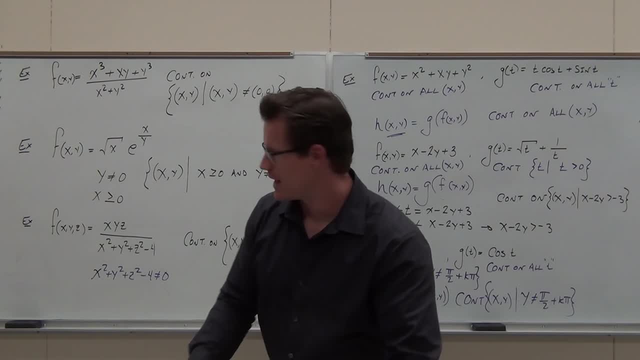 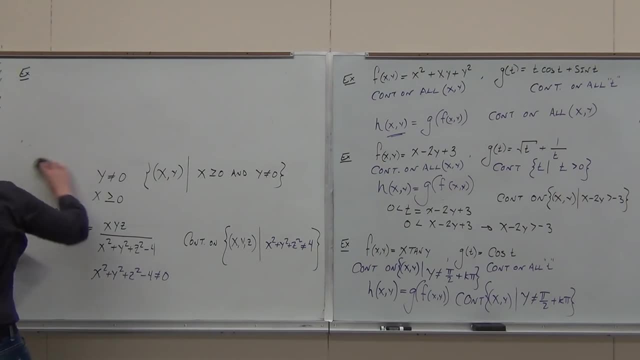 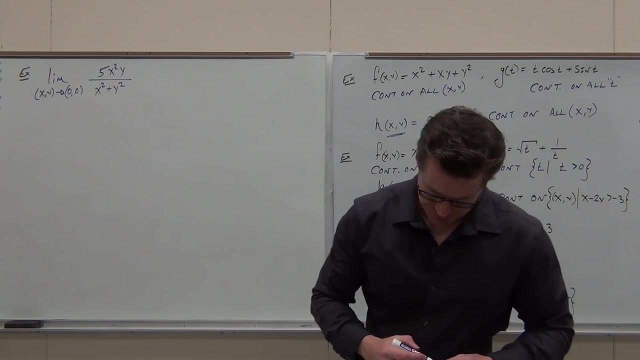 This is the case that you use. So if we don't have that stuff, for example, Let's talk about this limit Only. one First thing you should always do with limits is what Plug them in And you plug it in. 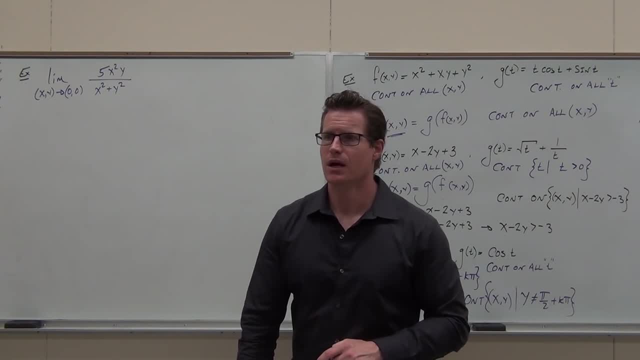 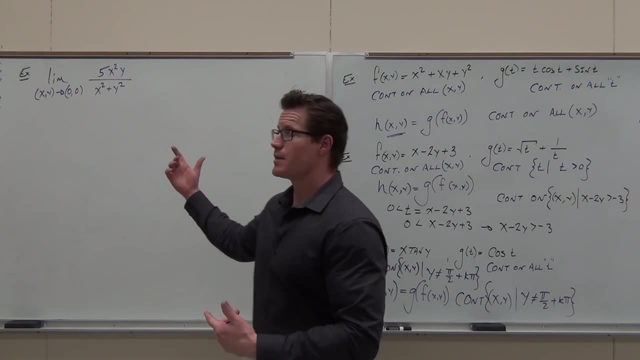 You get 0 over 0.. You can verify that form if you want to, And then we go: okay, we're used to saying things don't exist in this case, but this one does. How do you prove it? You might try polar and see what that gives you. 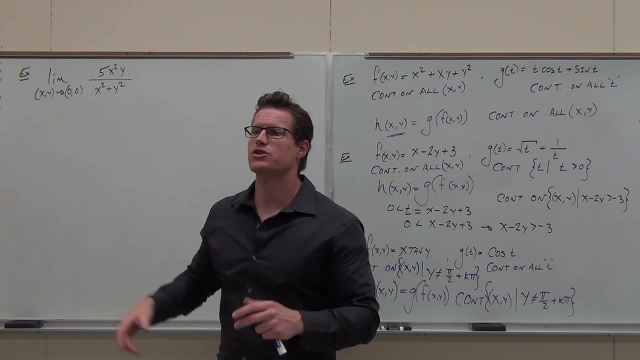 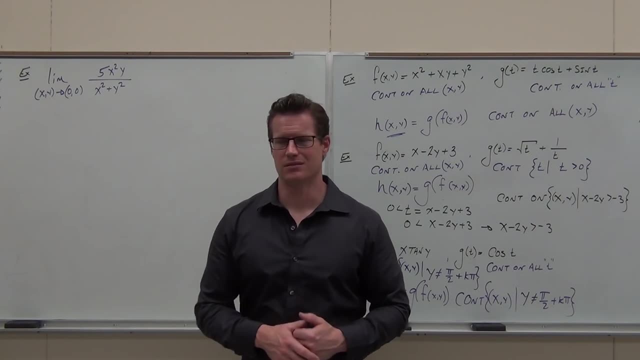 You could try it. That might work, I don't know. I want to show you in this case how to use a squeeze theorem to your advantage. This is the other way. So the things we do with limits: First plug it in. 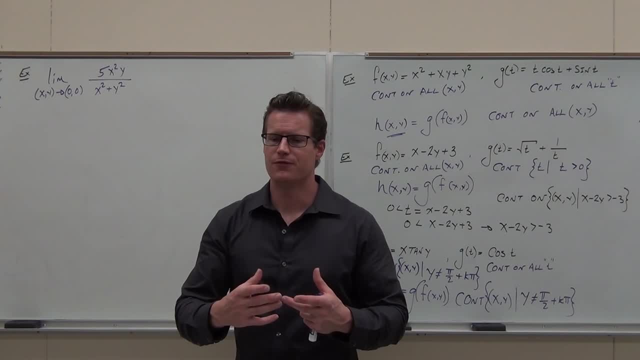 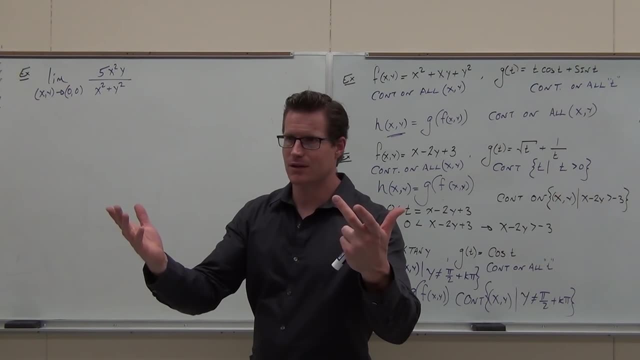 If you can plug it in and you get a number, then the function is defined there, which means we're continuous there. We just plug it in and we're good, because if we're continuous the limit exists, Got it? That's fantastic. 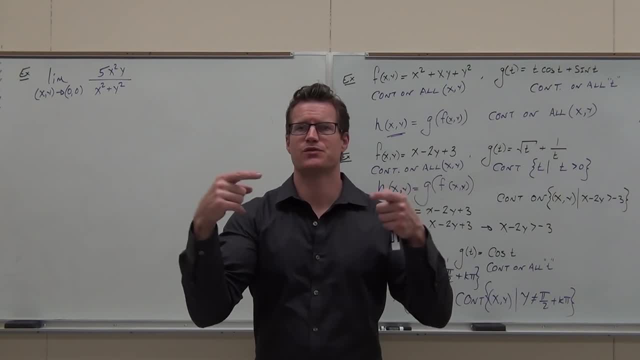 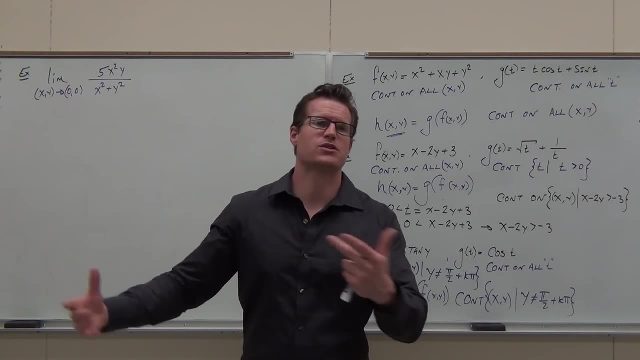 Or we try to prove it doesn't exist by finding those different paths. We spent most of our time doing that. Or using the polar trick that we created- That was pretty cool- Or the squeeze theorem. Those are basically the things we do with limits. 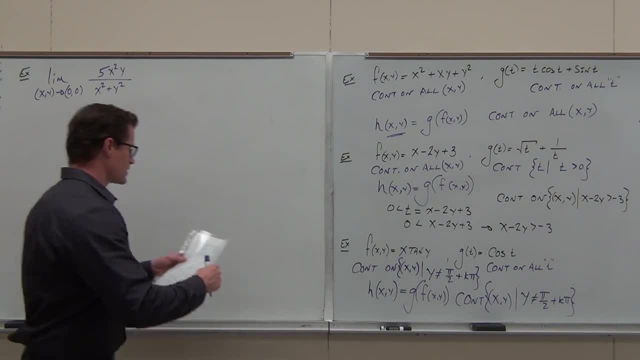 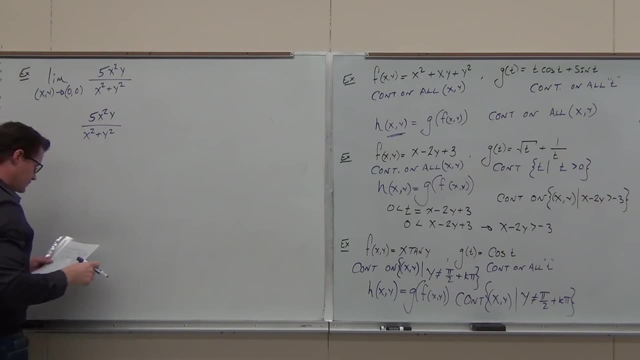 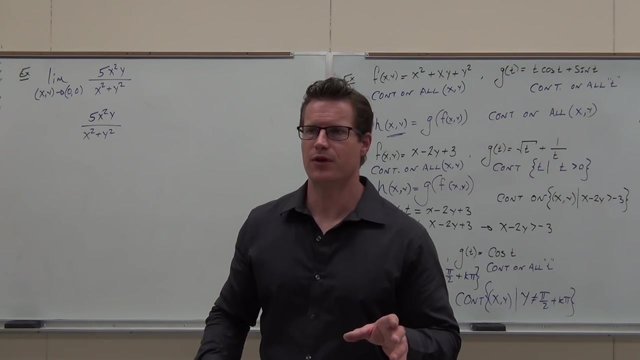 I'm going to show you the squeeze theorem right now. So let's take a look at this, Let's look at our function, And I want to consider the absolute value of the function. Where are you getting that from? I'll show you where. 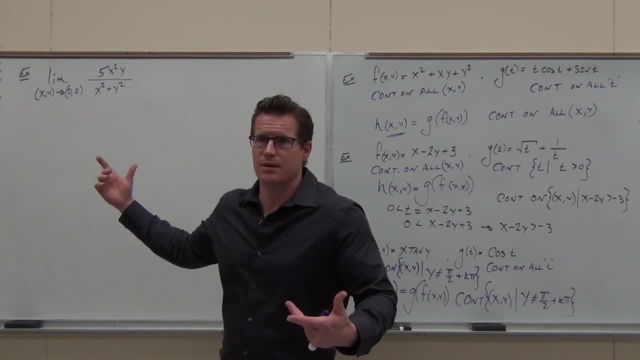 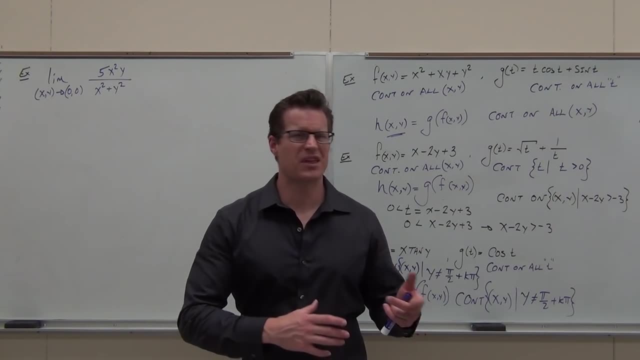 You might try polar and see what that gives you. You could try it. That might work, I don't know. I want to show you in this case how to use a squeeze theorem to your advantage. This is the other way. So the things we do with limits. 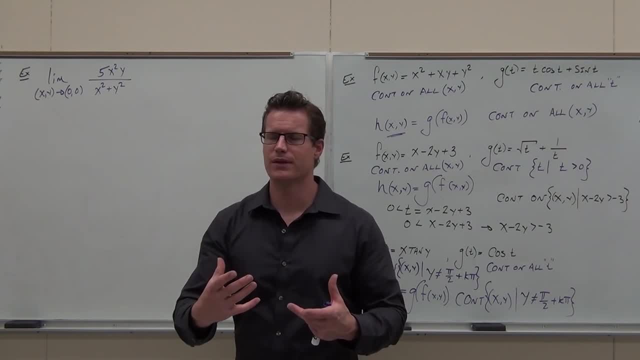 First plug it in. If you can plug it in and you get a number, then the function is defined there, which means we're continuous there. We just plug it in and we're good, Because if we're continuous the limit exists. 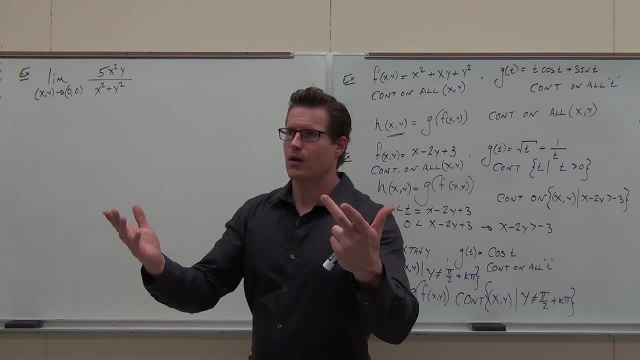 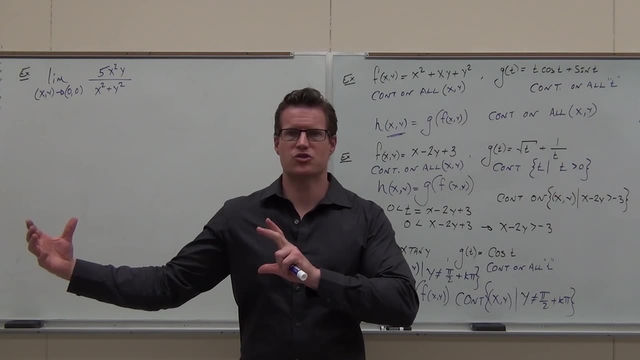 Got it, That's fantastic. Or we try to prove it. It doesn't exist. By finding those different paths, we spend most of our time doing that, Or using the polar trick that we created- That was pretty cool. Or the squeeze theorem. 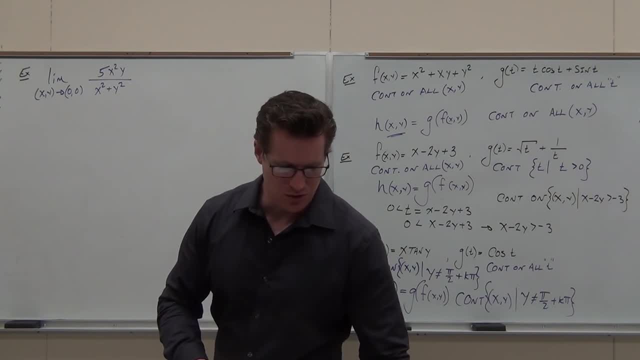 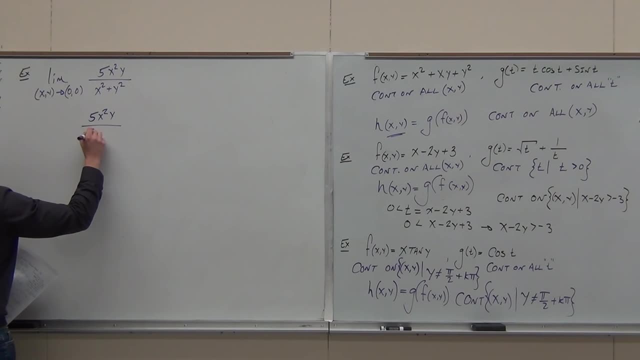 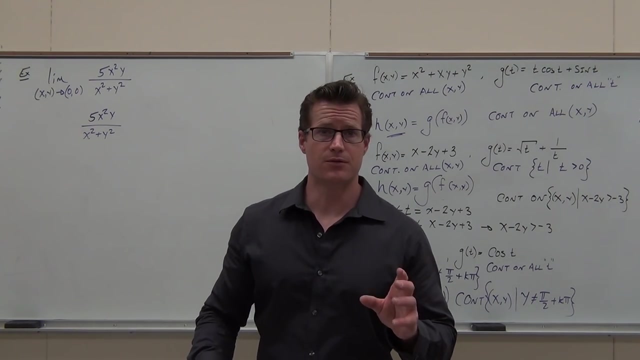 Those are basically the things we do with limits. I'm going to show you the squeeze theorem right now. So let's take a look at this, Let's look at our function And I want to consider the absolute value of the function. Where are you getting that from? 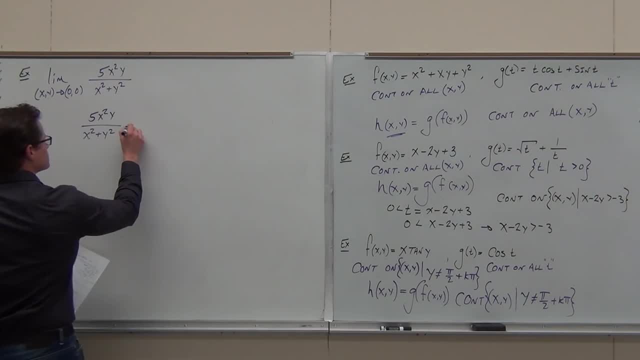 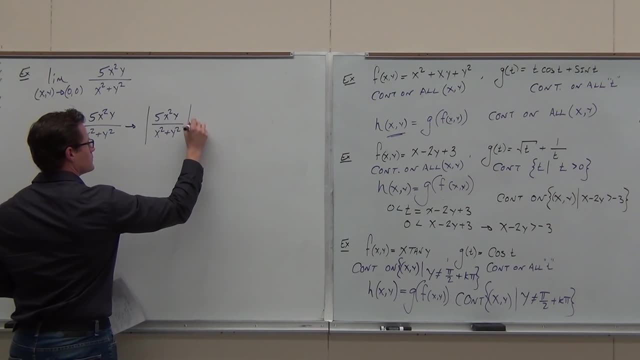 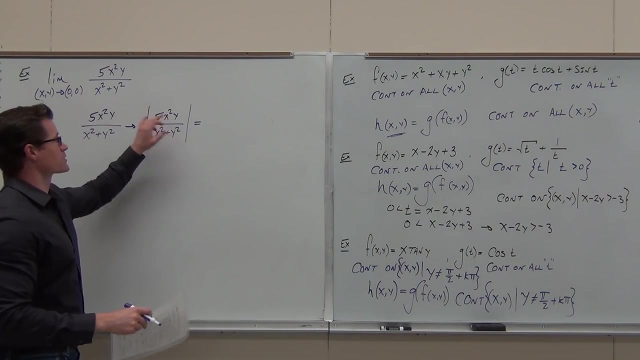 I'll show you where. I'll show you where, in a second. True or false, this denominator is always positive, no matter what. True, That absolute value doesn't really matter. True or false, 5x squared is always positive, no matter what. 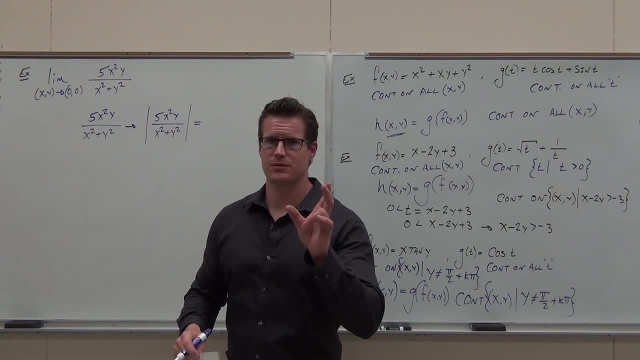 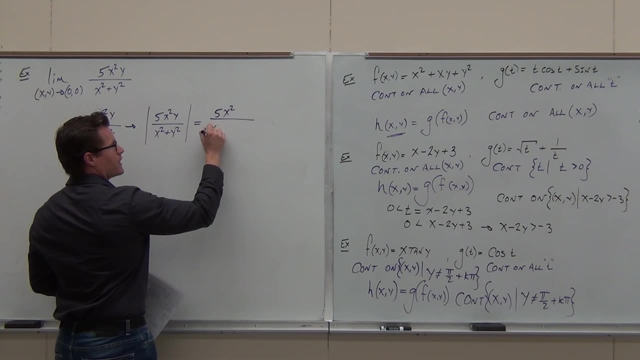 Yeah, That doesn't really matter. True or false, y is positive, no matter what False False. So this would equal 5x squared Over x squared plus y squared absolute value of y. Does that make sense to you? 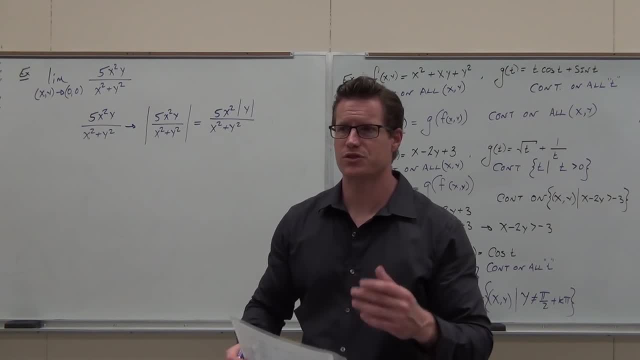 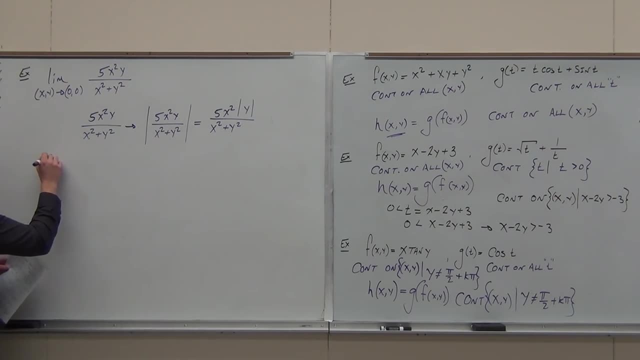 Now we're going to build some stuff here. I don't want to confuse you, but we're going to build from scratch and try to get back to this thing. We're going to try to get here. So here we go. This is going to seem kind of nonsense, but you understand this, right. 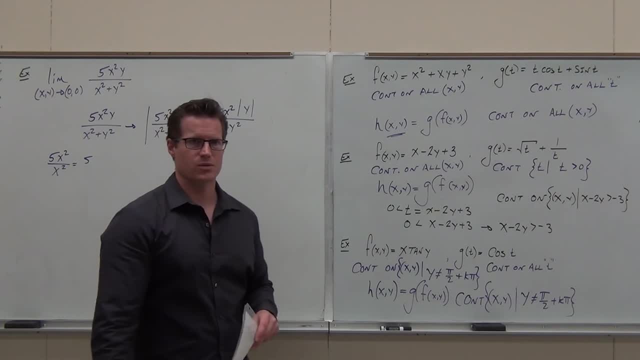 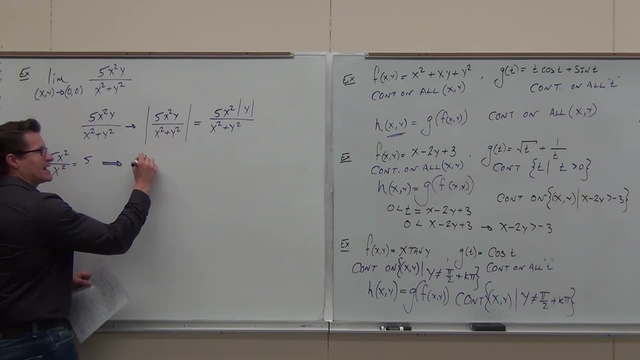 That this is equal to 5.. 5x squared plus x squared is equal to 5.. You go okay. why are we doing that? Well, that implies this: If I add anything to the denominator, if this equals 5 and I add something that's greater than, 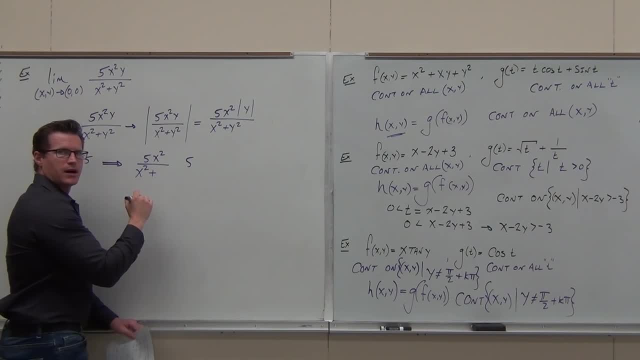 or equal to 0 here. is it still equal to 5?? What would it be? Smaller than 5.. Smaller than, or, if it's 0,, it would be equal to 5.. Does that make sense, True or false? y squared is greater than or equal to 0?. 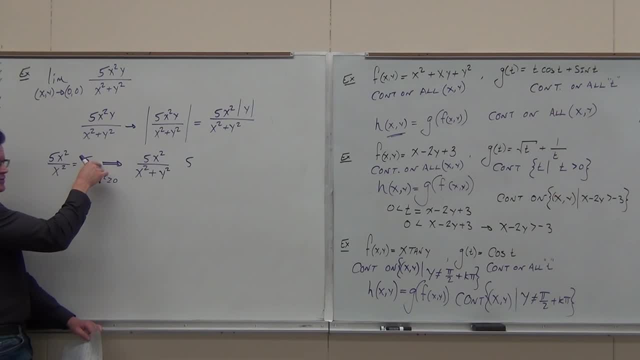 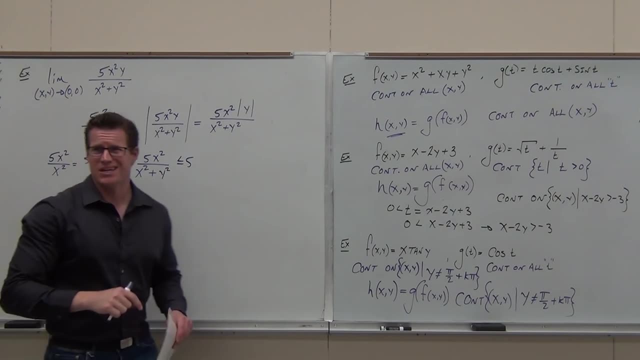 So, since y squared is greater than or equal to 0, if this equals 5 and I add something to the denominator, I make the denominator bigger, I make the fraction smaller. it's got to be less than 5 or at most equal to 5.. 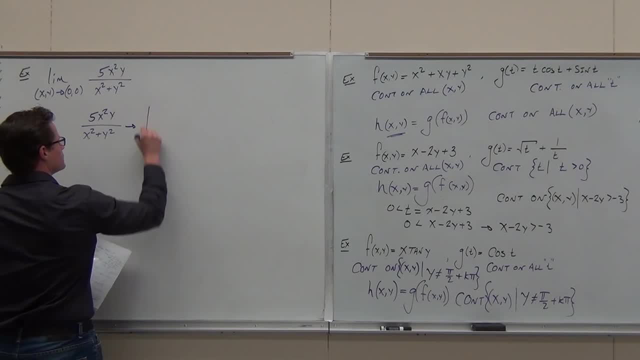 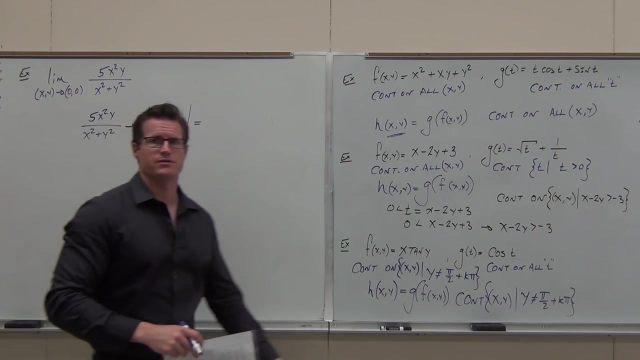 I'll show you where in a second. True or false, This denominator is always positive, no matter what, That absolute value doesn't really matter. True or false, 5x squared is always positive, no matter what, That doesn't really matter. 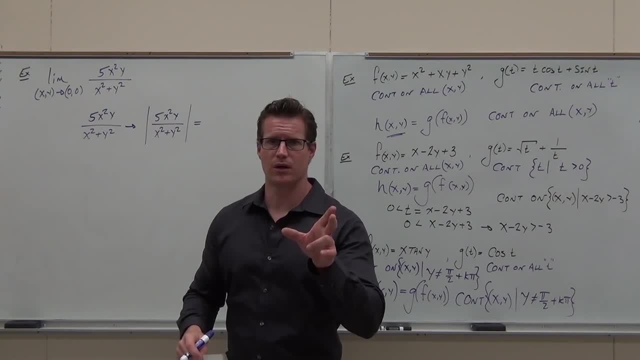 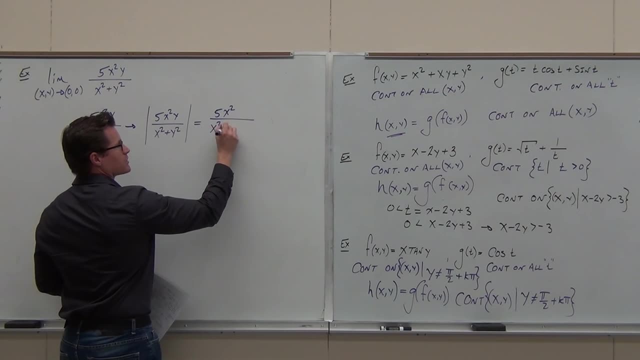 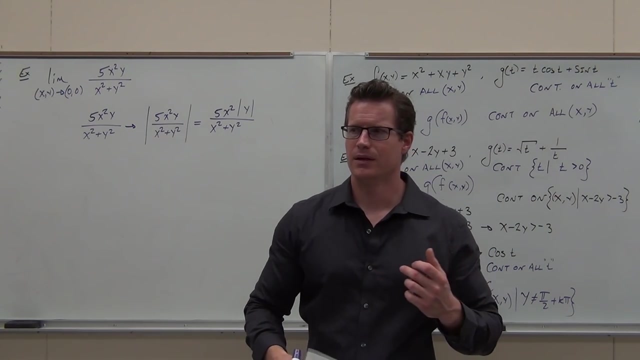 True or false, Y is positive, no matter what False False. So this would equal 5x squared over x squared plus y squared absolute value of y. Does that make sense to you? Now we're going to build some stuff here. 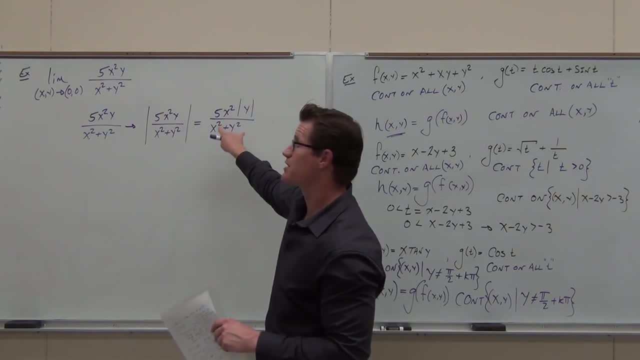 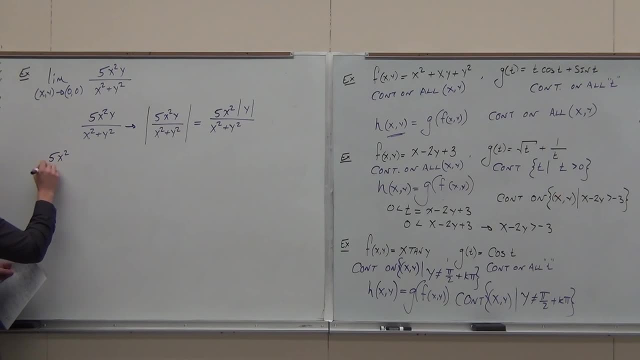 I don't want to confuse you, But we're going to build from scratch and try to get back to this thing. We're going to try to get here, So here we go. This is going to seem kind of nonsense, But You understand this right. 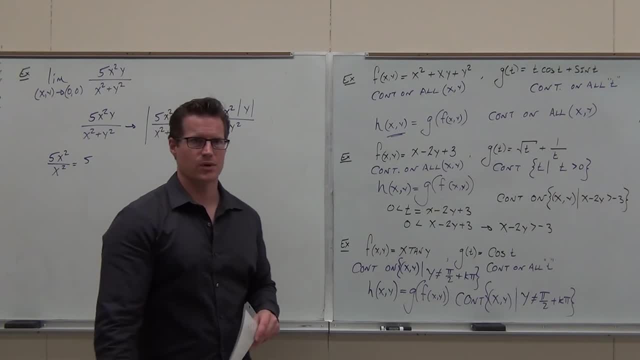 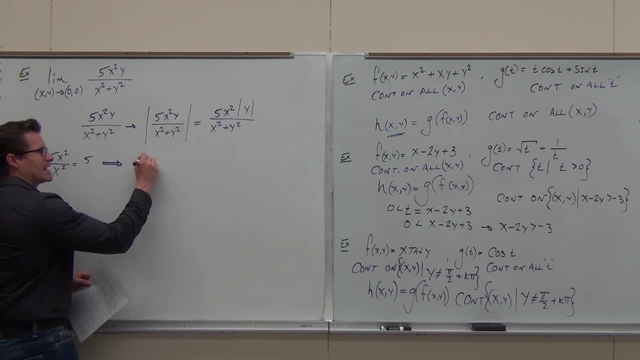 That this is equal to 5?? 5x squared plus x squared is equal to 5.. You go okay. Why are we doing that? Well, that implies this: If I add anything to the denominator, if this equals 5, and I add something that's greater, 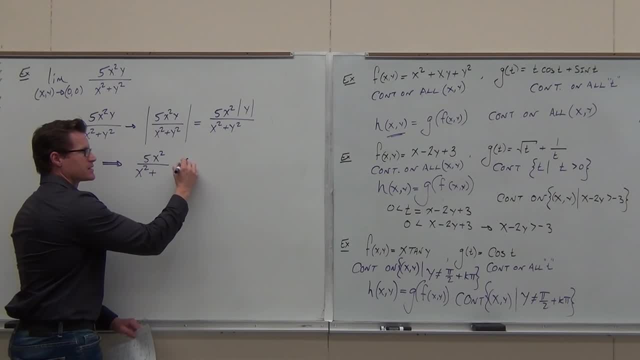 than or equal to 0. here is it still equal to 5?? What would it be? Smaller than 5.. Smaller than Or, if it's 0,, it would be equal to 5.. Does that make sense? 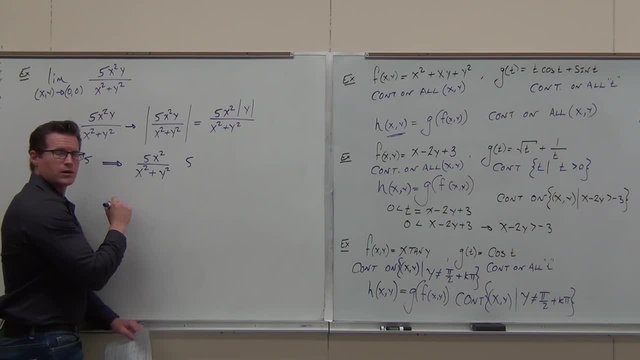 True or false, Y squared is greater than or equal to 0.. So, since y squared is greater than or equal to 0,, if this equals 5, and I add something to the denominator, I make the denominator bigger, I make the fraction smaller. it's. 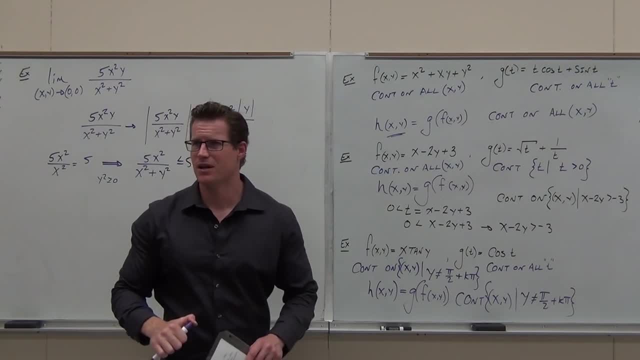 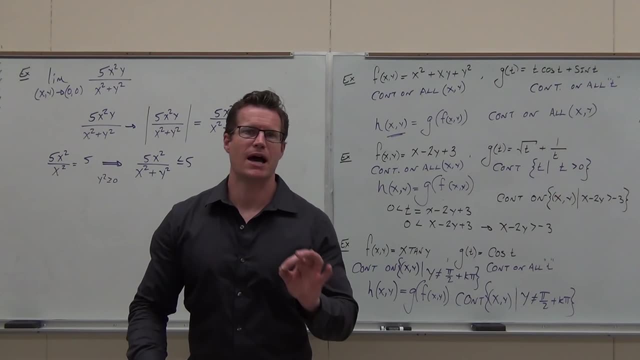 got to be less than 5 or at most equal to 5.. Head nod if you're okay with that one. Okay, we're going to use that in a second. Now, this is why we have to have the absolute value. What am I? 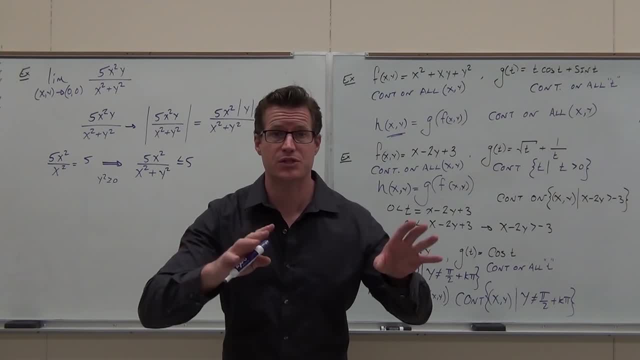 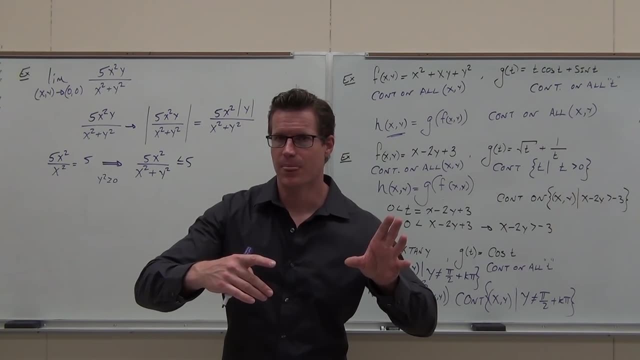 I can do anything I want to with inequalities, as long as I do it to both sides. And if I multiply by a negative, I've got to flip them, right? Do you know that? Yeah, Okay, I'm going to multiply by y. 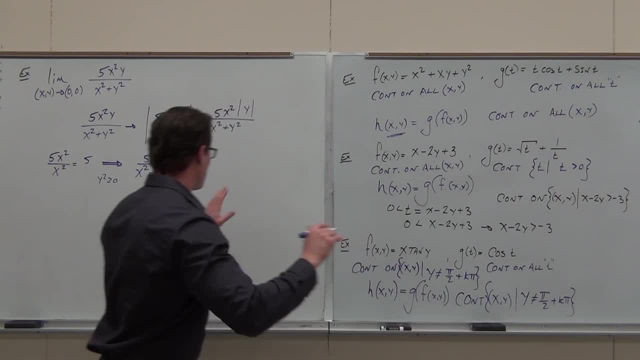 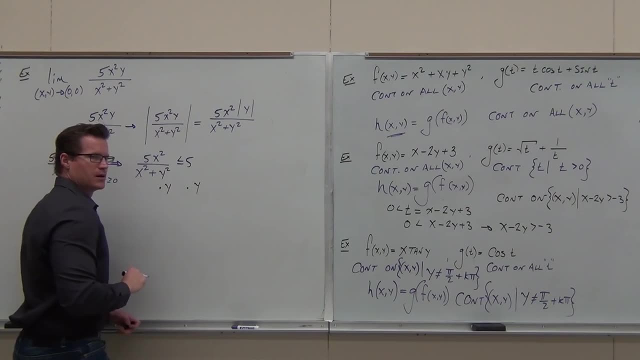 Now that's a problem. It's a problem if I do this. What's the problem If I multiply by just times this by y and times this by y? that's a problem, because y could be positive, y could be negative. 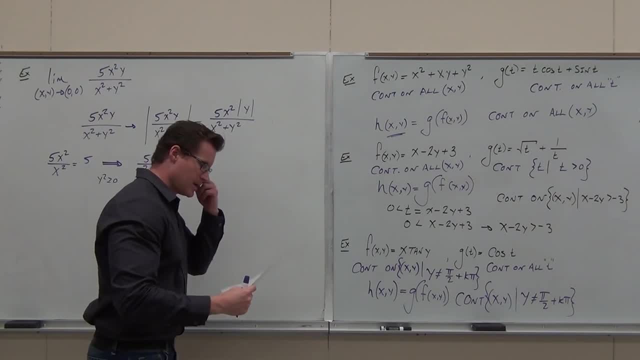 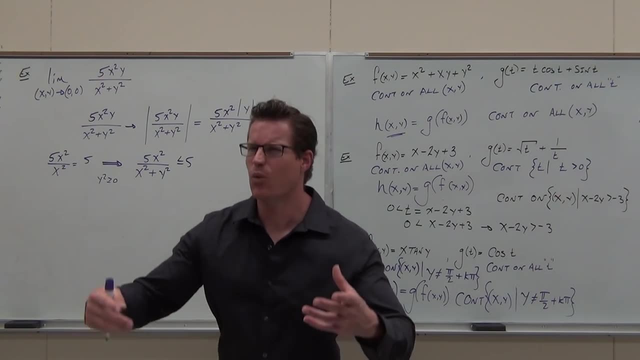 Head nod if you're okay with that one. Okay, we're going to use that in a second. Now, this is why we have to have the absolute value. What am I? you know I can do anything I want to with inequalities, as long as I do it to both sides. 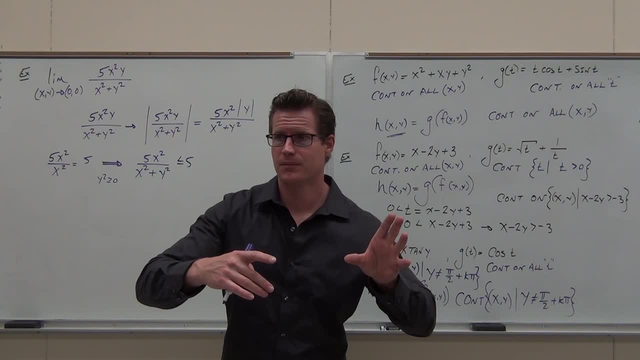 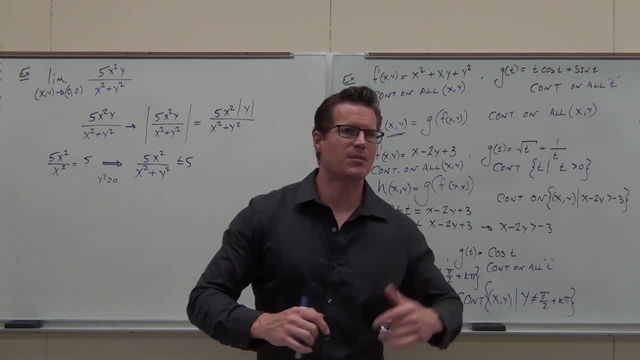 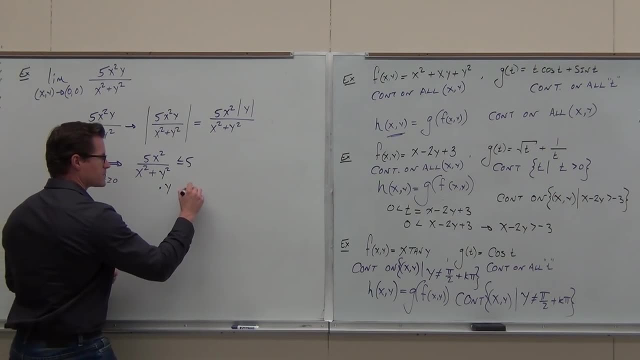 I'm going to work this out. I'm going to work this out. I'm going to work this out. If I multiply by y, now that's a problem. It's a problem if I do this. What's the problem If I multiply by just times this by y and times this by y? that's a problem. 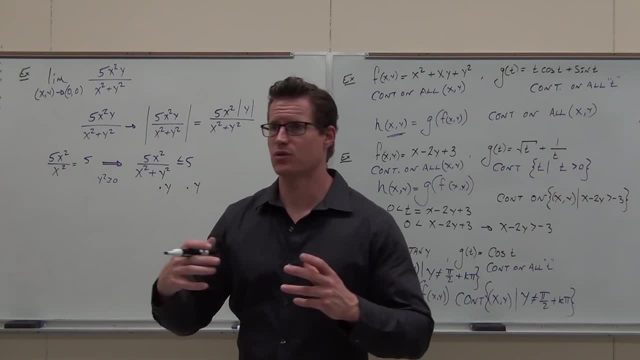 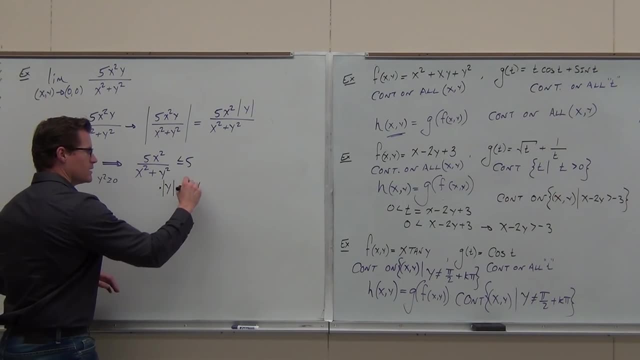 because y could be positive, y could be negative. I wouldn't know. I wouldn't have a correct inequality. That would be a big, big situation. Does that make sense? However, if I force this thing to be absolute value, now I'm multiplying by what type of number? 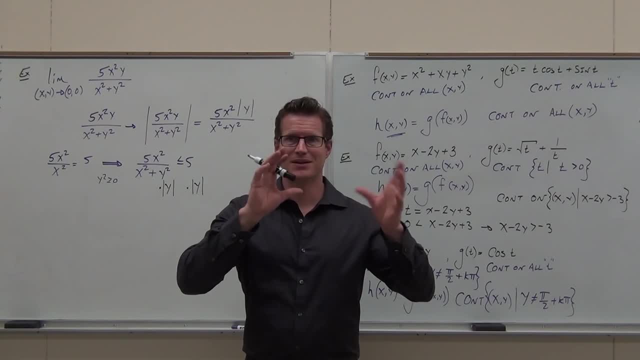 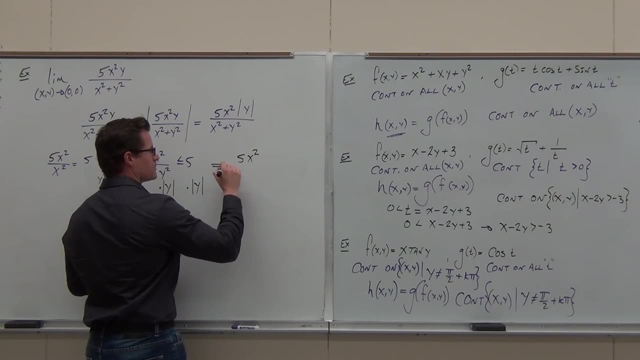 Positive, positive, For sure, positive. Do I have to flippy-dippy the inequalities? No, No, Okay, What it gives us is 5x squared absolute value. oh my gosh, over x squared plus y squared is less than or equal to 5 absolute value y. 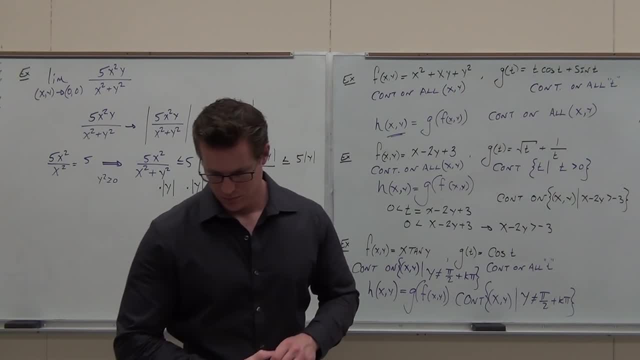 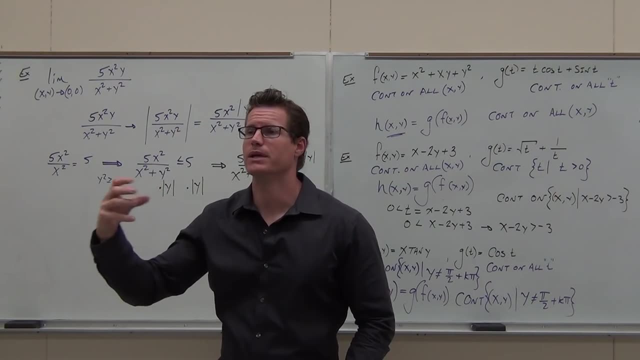 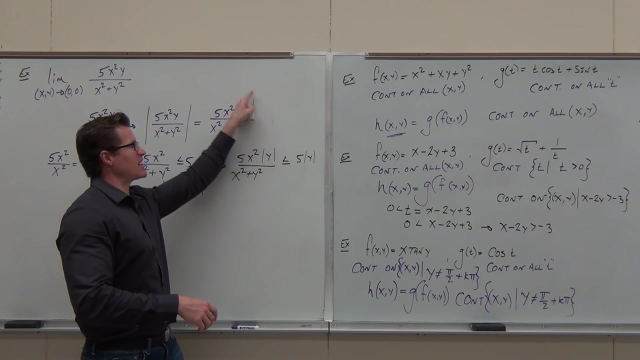 Can I have an honest show of hands, if you feel okay with this? so far, Yes. This is the reason why we needed the absolute value was so that I could multiply by something and not flip that inequality and get the same thing out of it. 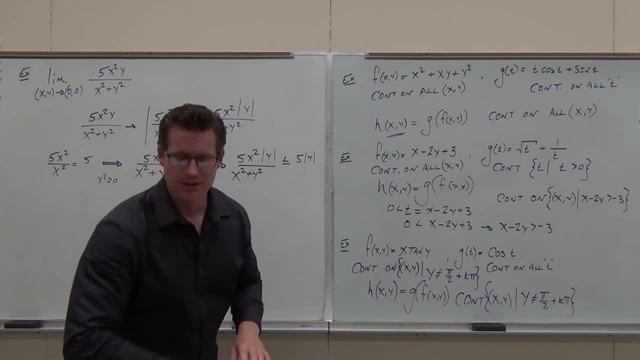 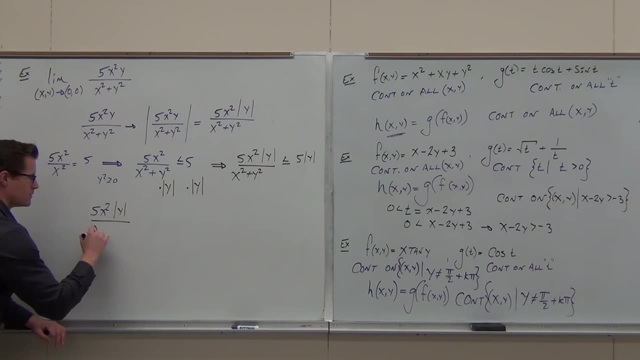 Do you guys get the idea? That's why I needed that. Now let's think about this. Tell me something We're going to start with this. Tell me something about. tell me one thing about that that you know It's on the board already. 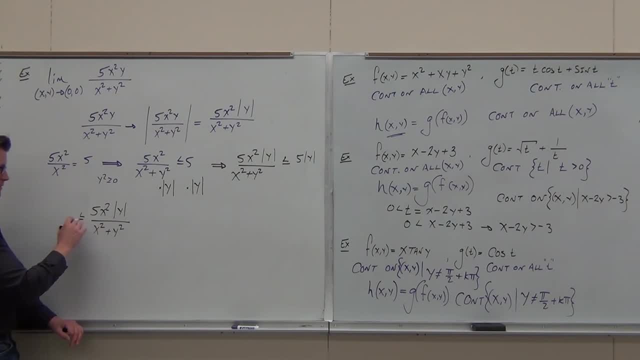 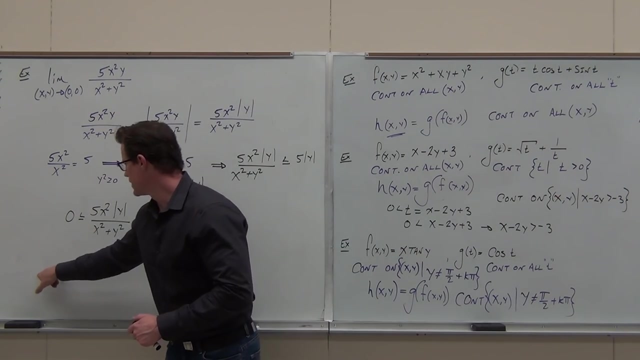 Tell me one thing about that that you know: Always positive. It is always positive, So it's greater than zero. Tell me the other thing that we just found out. Say that again. How the squeeze theorem works is this: It says: if you take the limit of this and you take the limit of this, and they go to the same number. 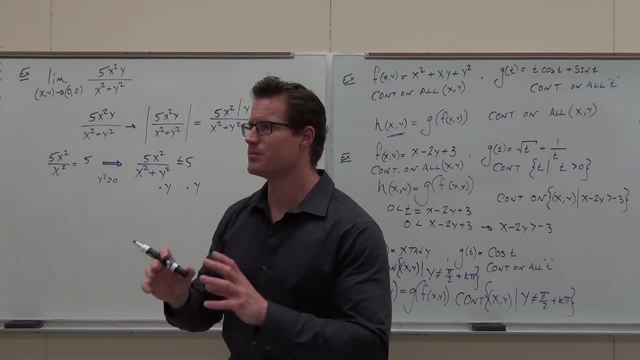 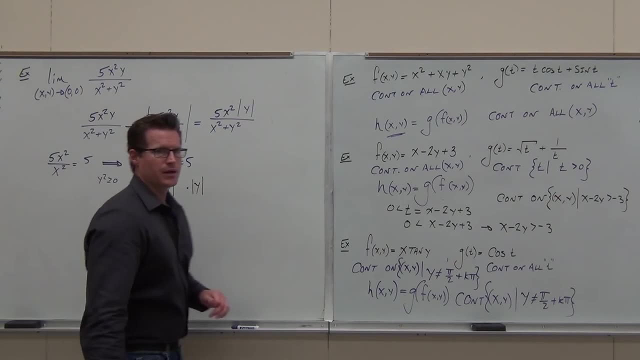 I wouldn't know. I wouldn't have a correct inequality. That would be a big, big situation. Does that make sense? However, if I force this thing to be absolute value now I'm multiplying by what type of number Positive? 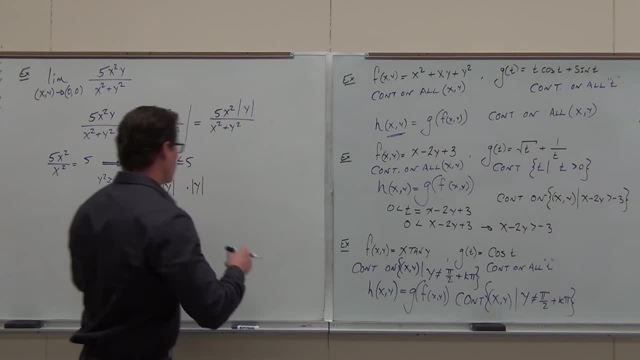 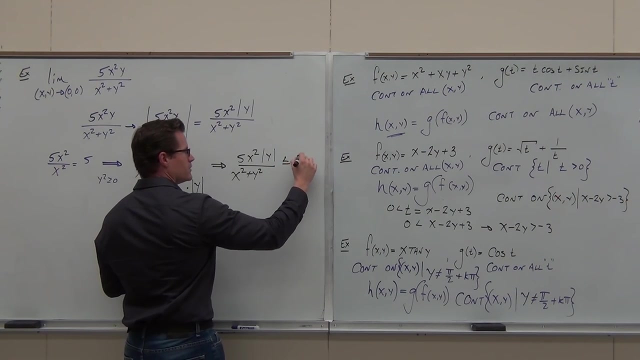 For sure, positive. Do I have to flippy-dippy the inequalities? No, No, Okay. What it gives us is 5x squared absolute value. oh my gosh. over x squared plus y squared is less than or equal to 5x absolute value of y. 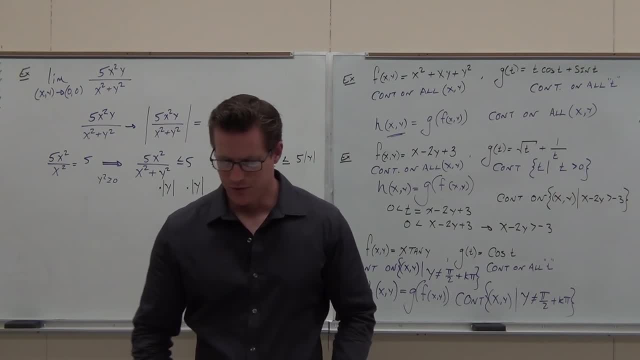 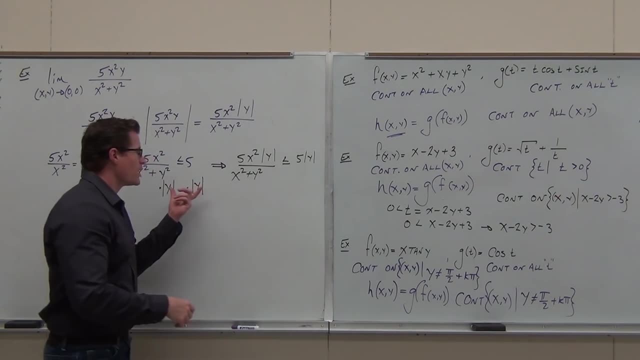 Can I have an honest show of hands, if you feel okay with this? so far? This is the reason why we needed the absolute value was so that I could multiply by something and not flip that inequality and get the same thing out of it. Do you guys get the idea? 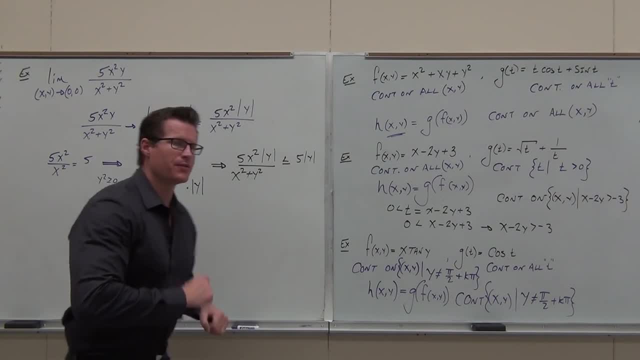 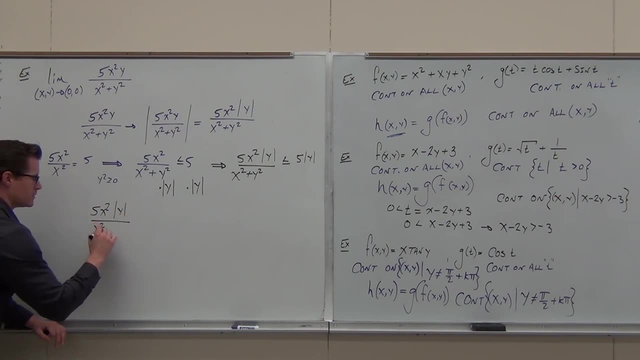 That's why I needed that. Now let's think about this. Tell me something- We're going to start with this. Tell me something about. tell me one thing about that that you know It's on the board already. Tell me one thing about that that you know. 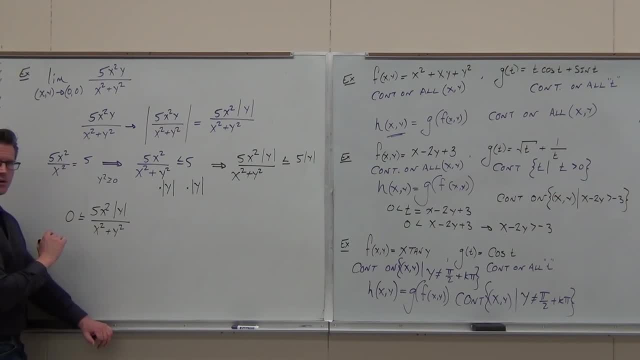 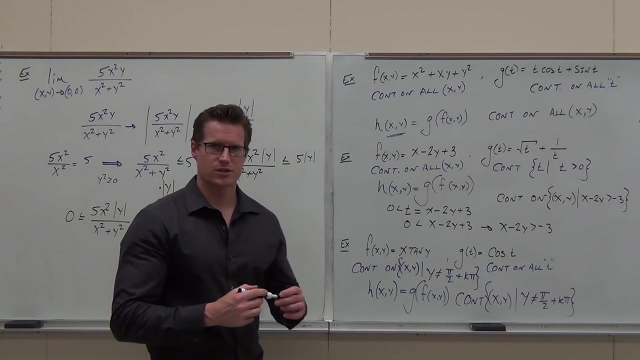 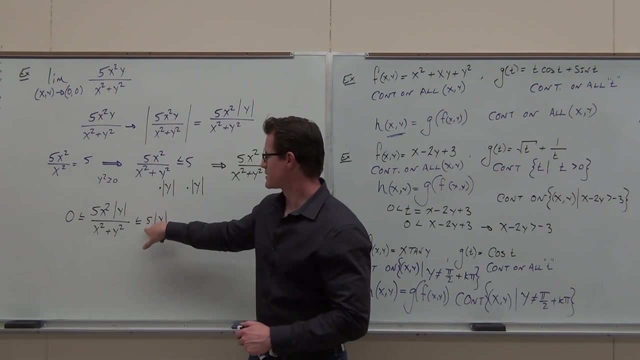 Always positive. It is always positive, So it's greater than zero. Tell me the other thing that we just found out. Say that again. Say that again. How the squeeze theorem works is this: It says: if you take the limit of this and you take the limit of this, and they go to the same number. 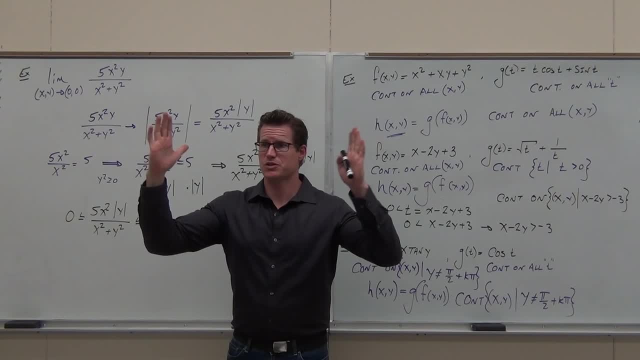 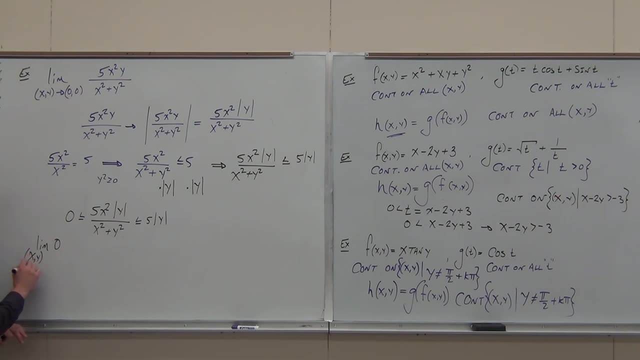 the thing squeezed or sandwiched- there some people call it the thing sandwiched or squeezed between them- has to go to the same value. What's the limit of zero as x, y approaches? I don't even care. Come on, it's not your question. 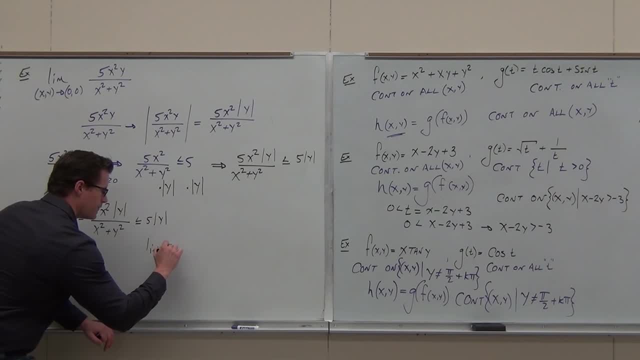 What is it And what's the limit of five? absolute value of y as x. y approaches zero, zero, Notice there's no x. I don't even care What's it. go to By the squeeze theorem, since the limit of this function goes to zero. 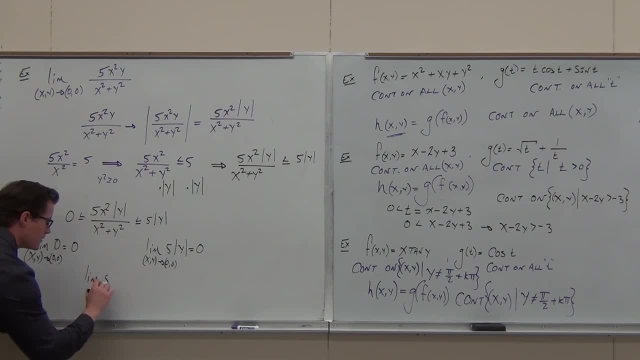 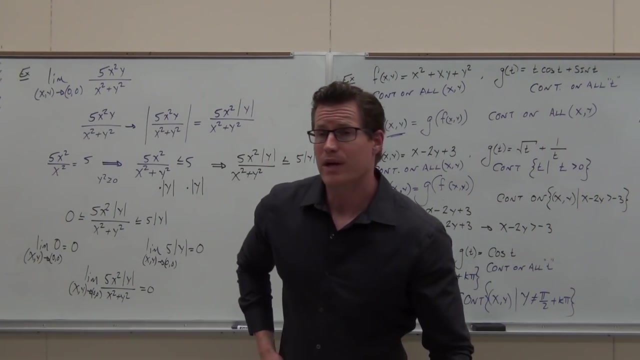 and the limit of this function goes to zero. the limit of this function: zero, zero by the squeeze theorem: zero. we built it. zero, zero. the middle's going to be zero. Now, we haven't proved a darn thing right now, but we're about to. 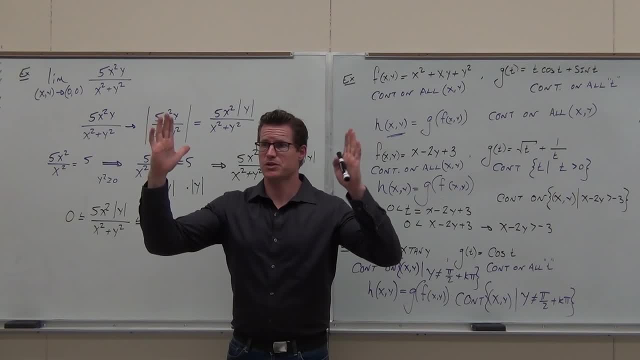 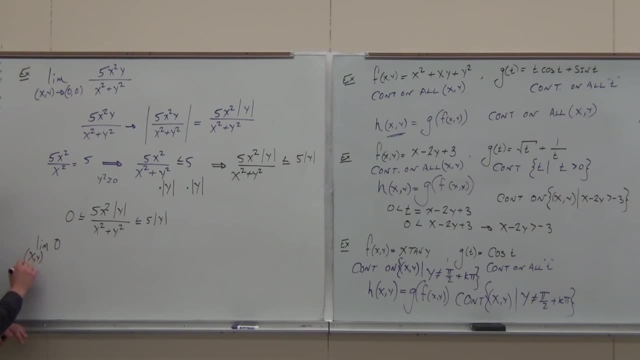 the thing squeezed or sandwiched- there some people call it the thing sandwiched or squeezed between them- has to go to the same value. What's the limit of zero as x, y approaches? I don't even care. Come on, that's not your question. 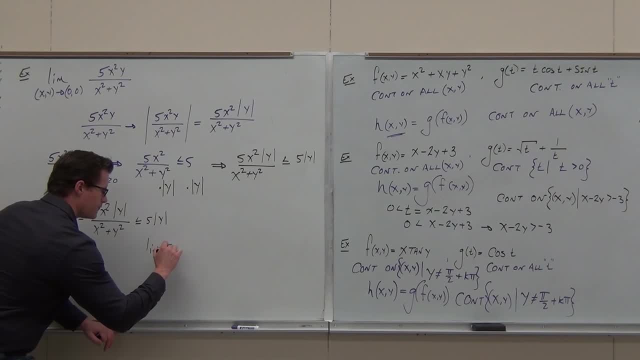 What is it? Zero And what's the limit of five? absolute value of y as x, y approaches zero. zero, Notice there's no x, but I don't even care. What's it. go to By the squeeze theorem, since the limit of this function goes to zero. 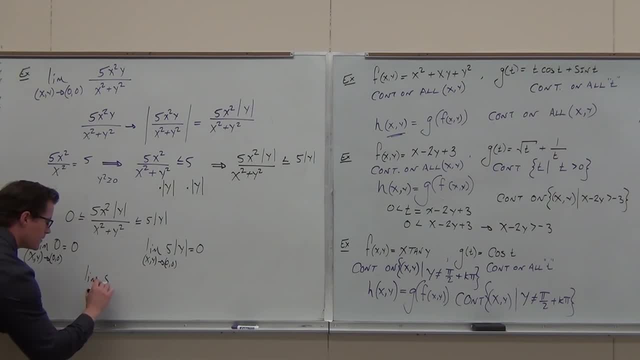 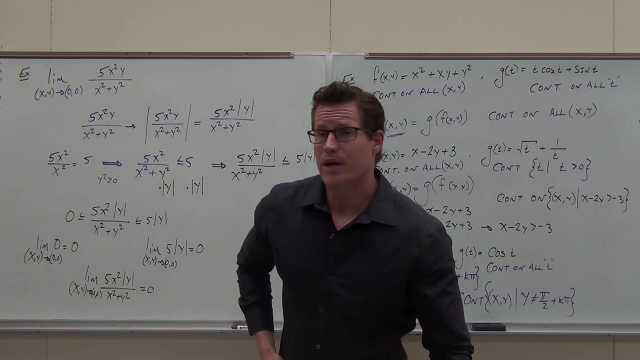 and the limit of this function goes to zero. The limit of this function is zero By the squeeze theorem: zero, zero. we built it. Zero, zero, middle's going to be zero Now. we haven't proved a darn thing right now, but we're about to. 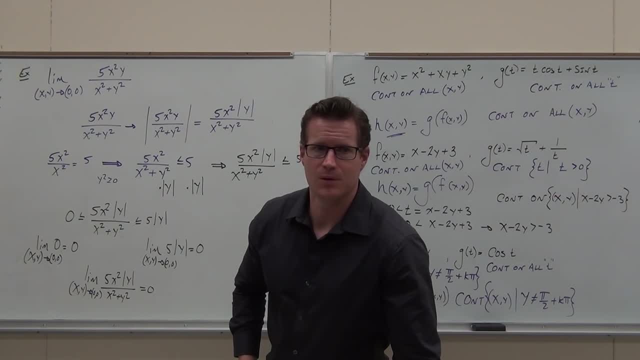 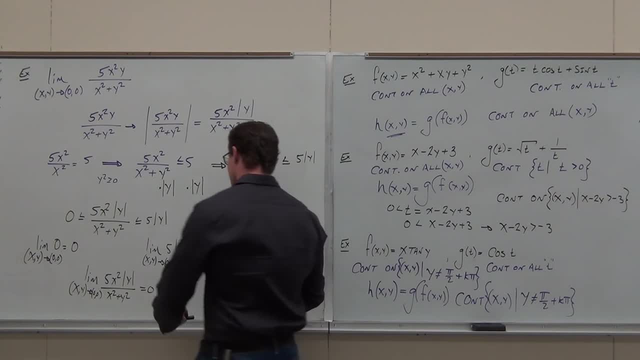 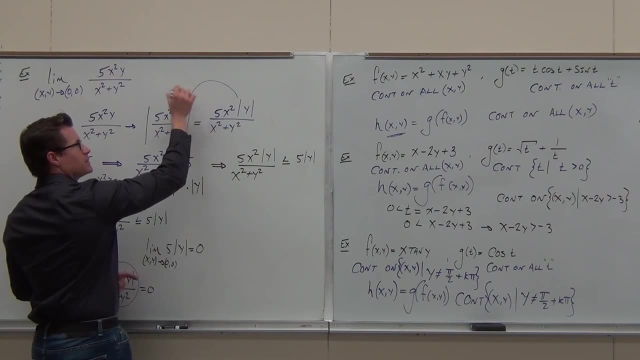 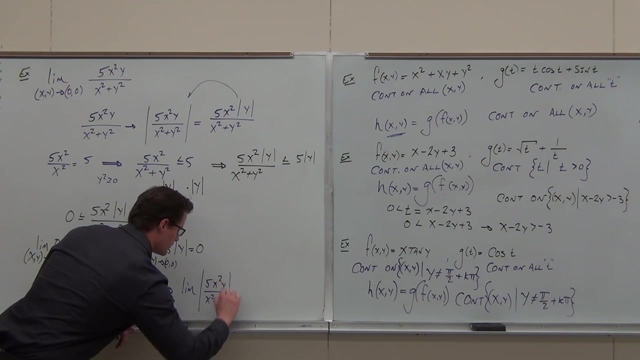 No, Yes. I want you to look back at this piece. This piece is equal to that piece. Do you guys follow that? Yeah, no, Yes. Therefore, the limit of the absolute value of all this junk? It is zero. 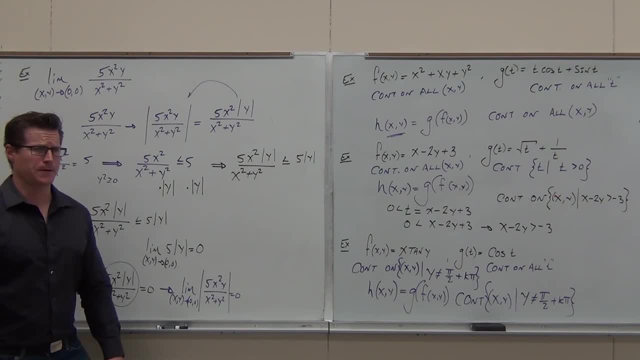 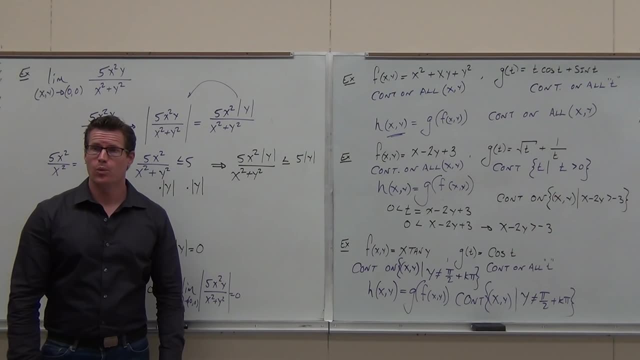 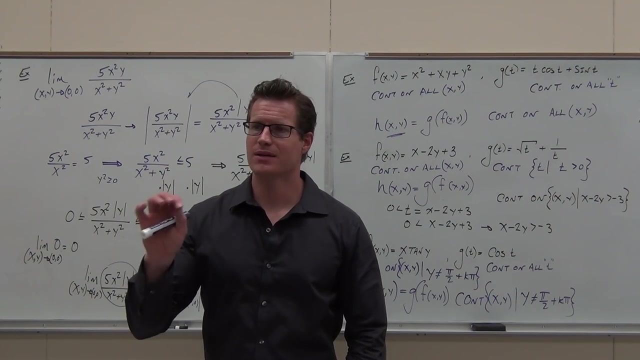 And you go awesome. But wait Leonard, Wait the Leonard. Is this exactly the same as that? No, But this is why we had statement number three over here, like 25 minutes ago. It was this: Continuity holds for compositions of continuous functions. 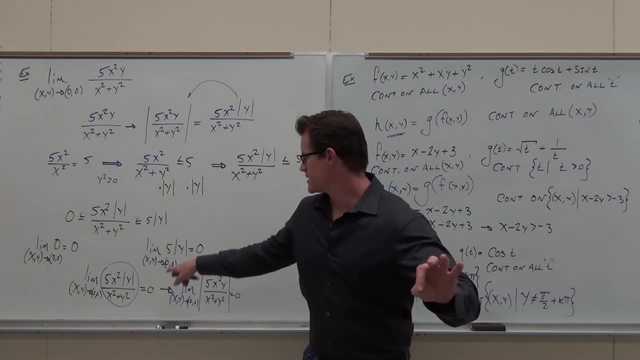 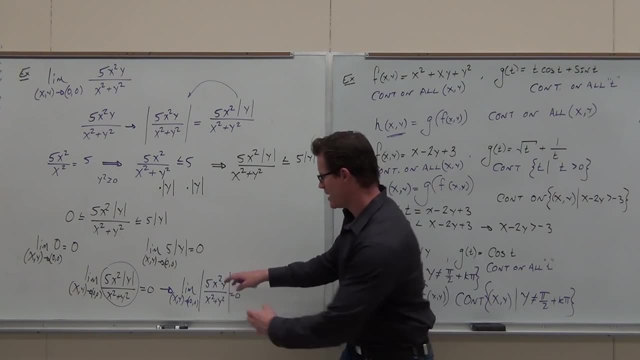 Here's my question to you: Is the absolute value function a continuous function? Do you see that this is a composition of this crappy function inside the absolute value function? Do you guys see that Continuity holds? That means we can do this stuff with it. 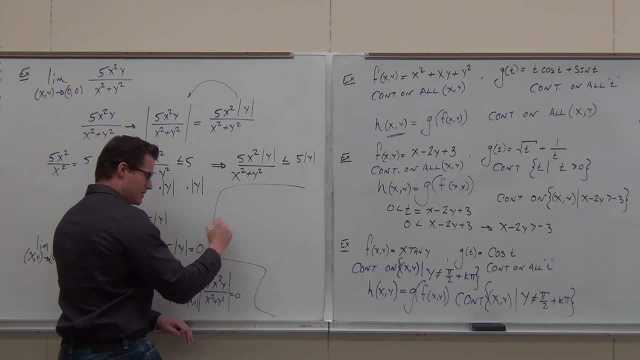 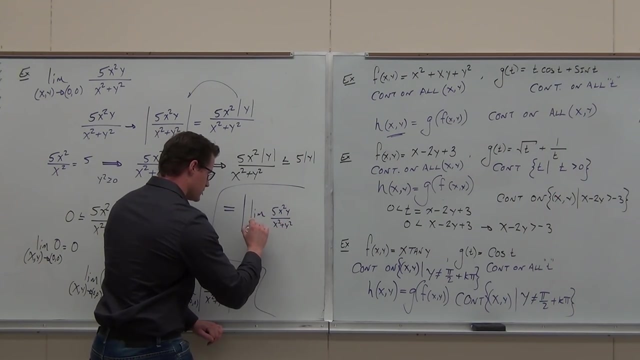 But the big point Here says that means that this limit equals the absolute value of the limit of 5x squared y, x squared plus y squared x, y- 0, 0.. Awesome, That's the same thing. 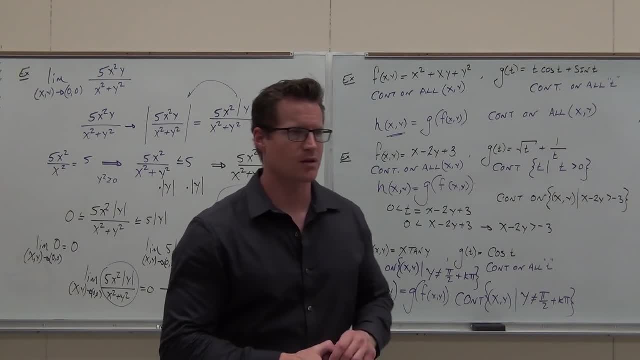 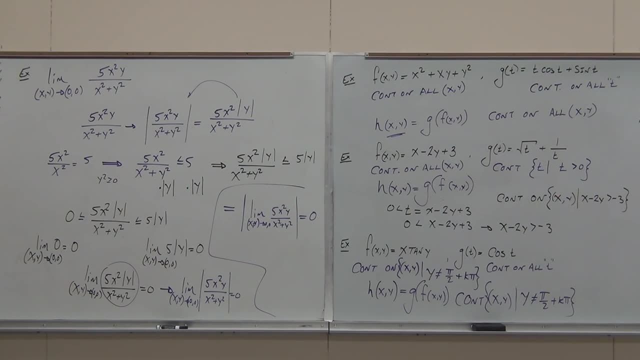 Absolute value of 0 is 0. We get the same exact thing. So we have this composition of continuous functions. We can prove that limit exists by the Swiss theorem. I guess stop it right here and we're going to call it good on this section. 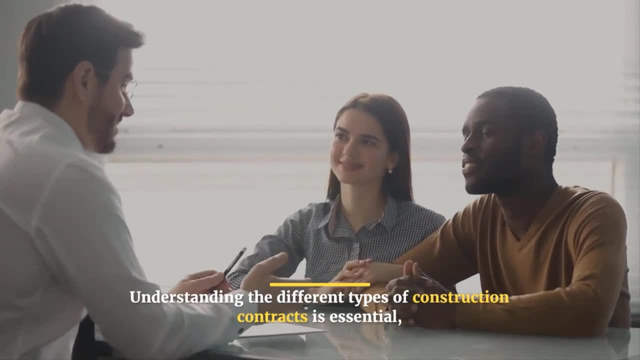 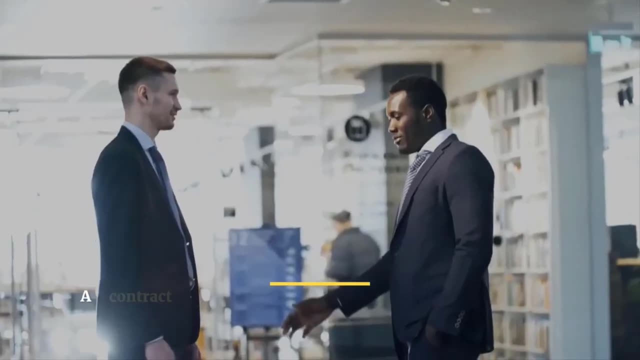 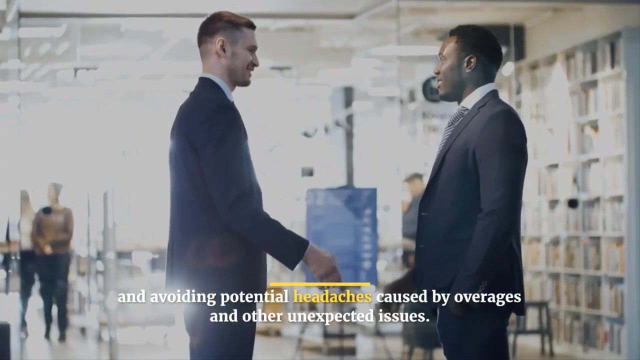 Understanding the different types of construction contracts is essential, as they determine what you pay, what you are liable for and many other aspects of the job. A contract protects both the builder and the owner by ensuring expectations are clear from the beginning and avoiding potential headaches caused by overages and other unexpected issues. 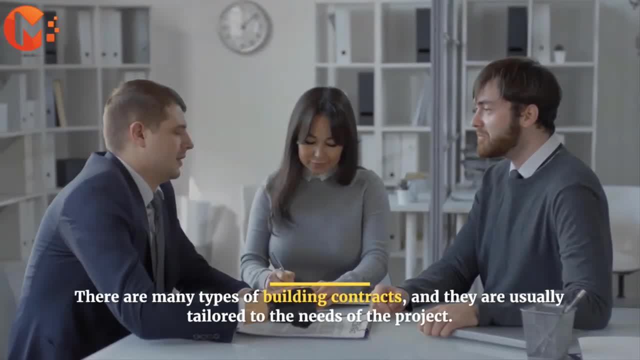 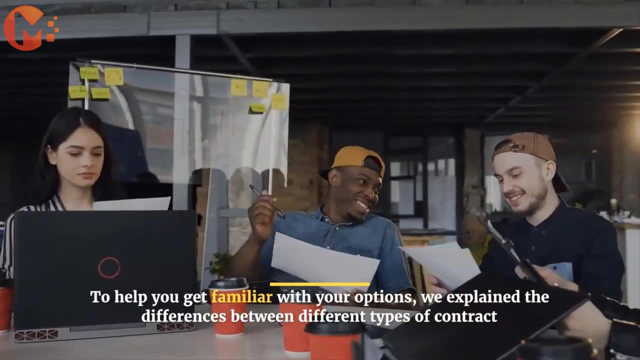 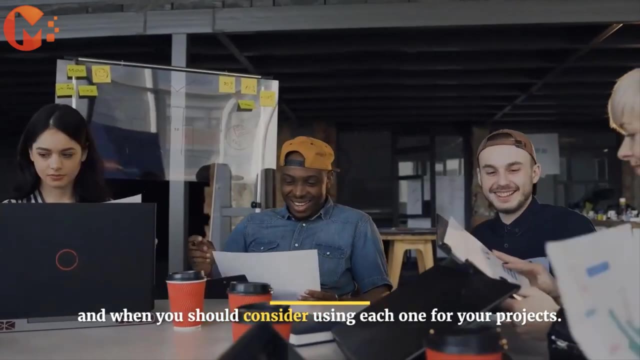 There are many types of building contracts and they are usually tailored to the needs of the project. To help you get familiar with your options, we explain the differences between different types of contract and when you should consider using each one for your project. We use builder to refer to the entity carrying out the construction services. 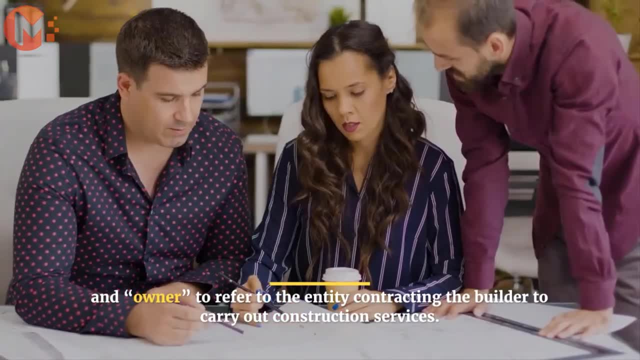 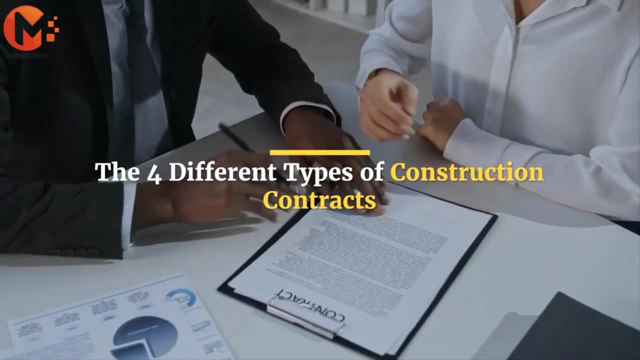 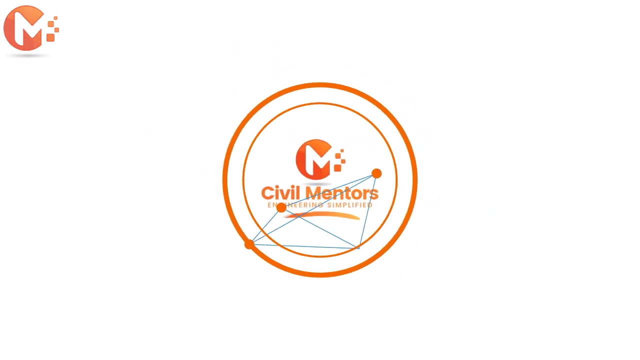 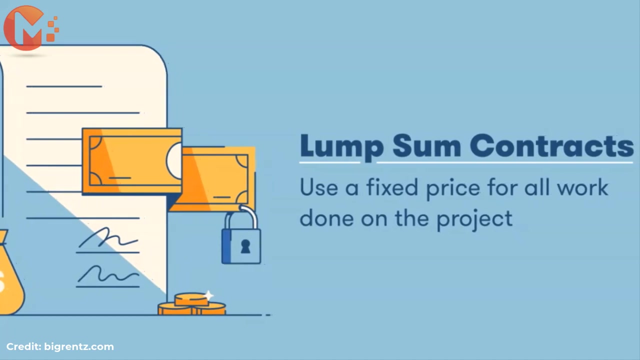 and owner to refer to the entity contracting the builder to carry out construction services. So now let's dive into the four different types of construction contracts. Number 1. Lumpsum Contracts. Lumpsum contracts use a fixed price for all work done on the project. 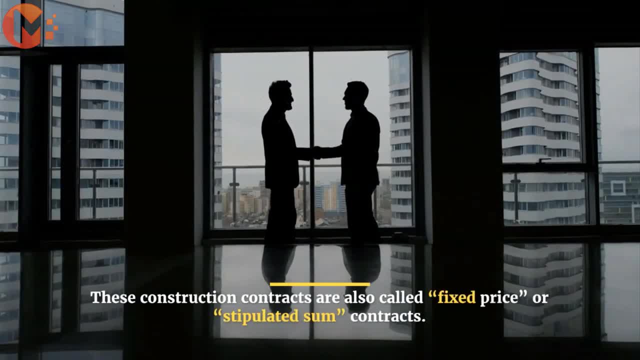 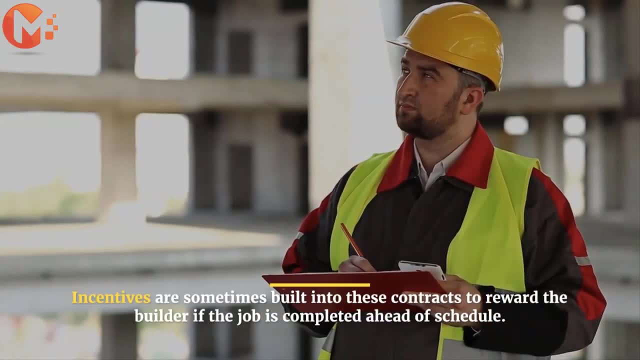 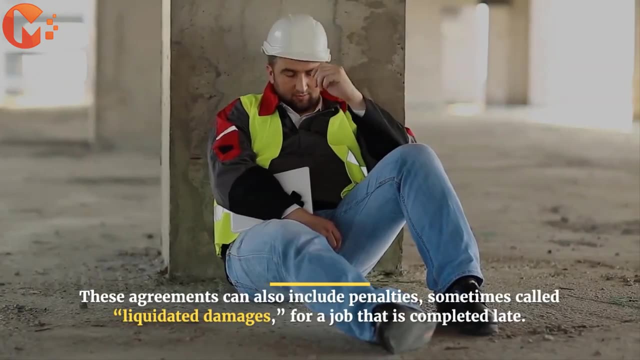 These construction contracts are also called fixed price or stipulated sum contracts. Incentives are sometimes built into these contracts to reward the builder if the job is completed ahead of schedule. These agreements can also include penalties, sometimes called liquidated damages, for a job that is completed late.